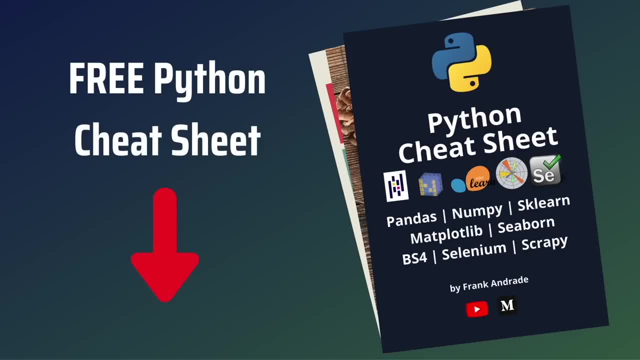 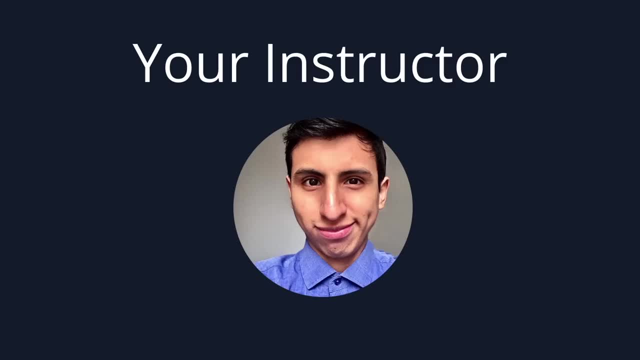 There you will find the concepts, methods and functions we will see in this course. By the way, I'm Frank and I will be your instructor in this course, So let's get started To download Anaconda. we go to anacondacom. 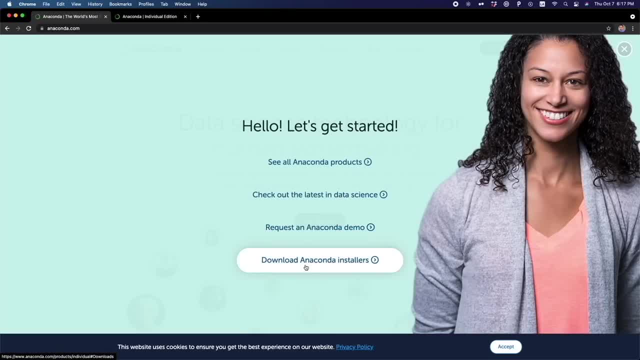 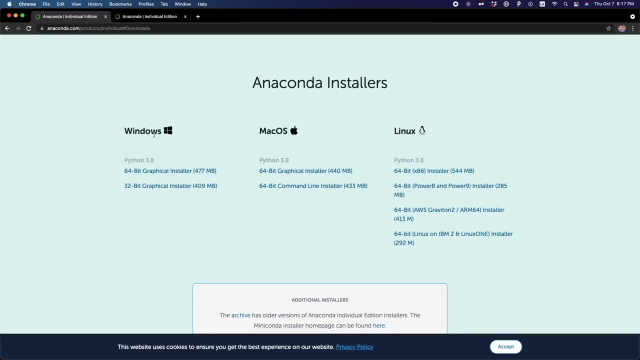 and click on get started. Then we choose the last option- download Anaconda installers- And then we have here that different Anaconda installers. So there are Windows, Mac and Linux. So in my case I'm going to choose Mac And I'm going to choose the 64 bit graphical installer. So now I'm 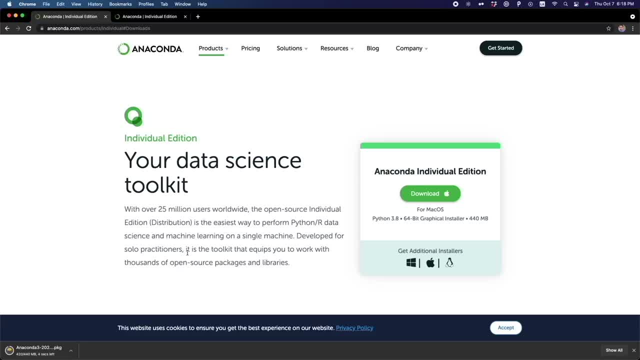 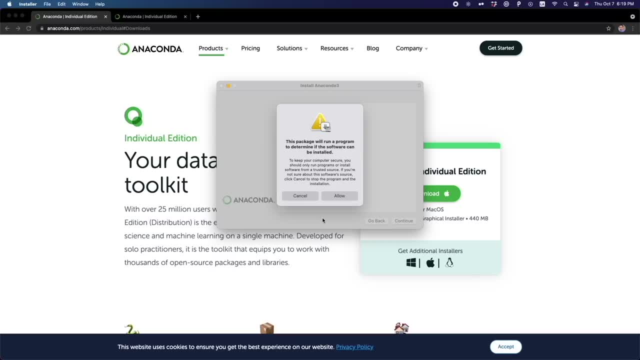 downloaded Anaconda And once it's downloaded, I'm going to click on it And a message will pop up. you just have to click on allow, As I'm going to do right now. So just click on allow and then click on continue until the. 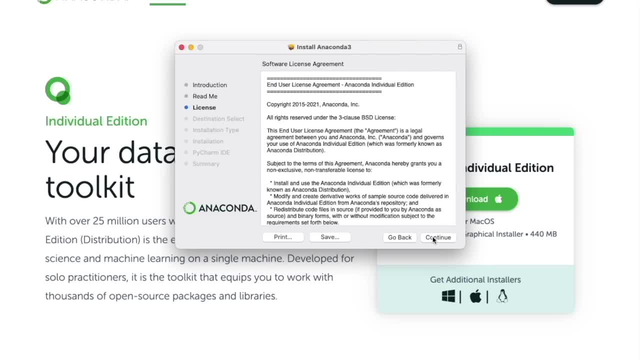 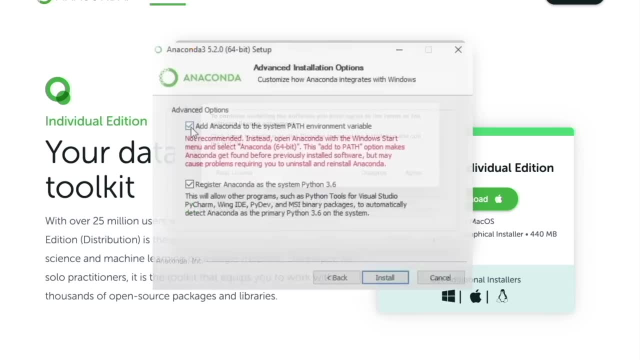 installation starts. So I just click Continue and then agree and then continue, And it's going to start installing Anaconda. In case you're on Windows and you're installing Python or Anaconda for the first time, make sure to check the first box you see now on screen. So I'm going to speed. 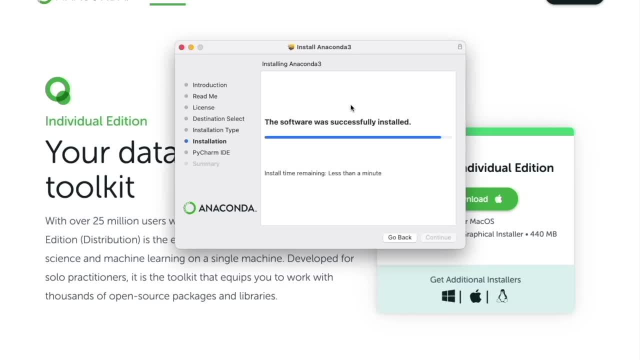 up the video now. Okay, the installation is almost done And now it's time to install the Anaconda. So I'm going to click on continue to finish the installation. So I click on continue And then we'll see just a summary of what was installed. And now I'm going to close this window And I'm 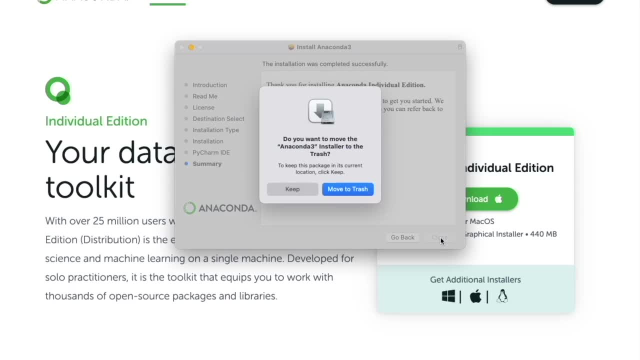 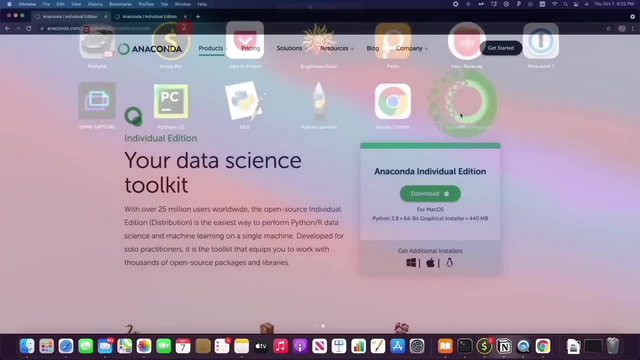 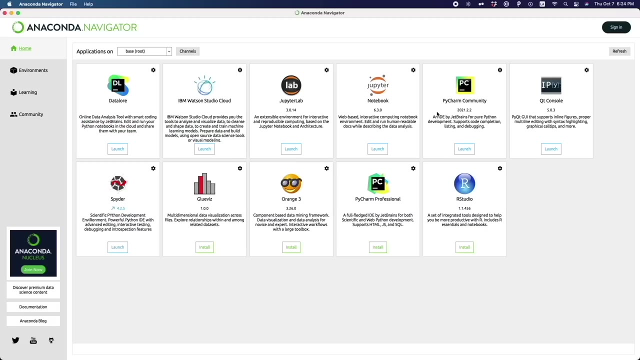 going to open Anaconda, So I'm going to locate the icon. it's a green icon, this one that you see here, And I'm going to open Anaconda. I'm going to wait a couple of seconds And let's see what was installed. So here we have. 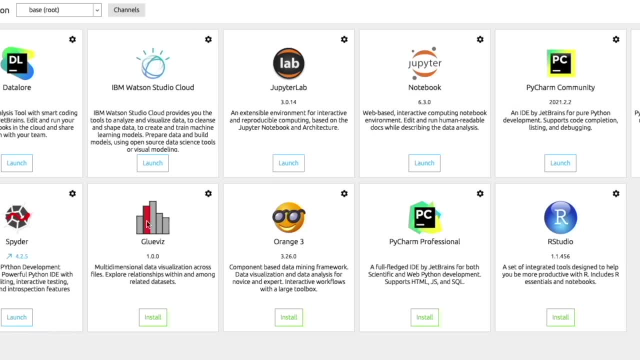 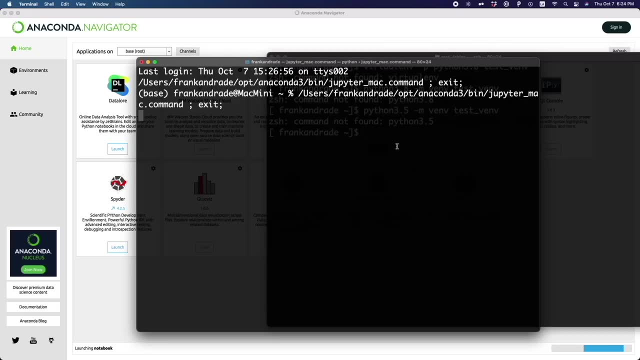 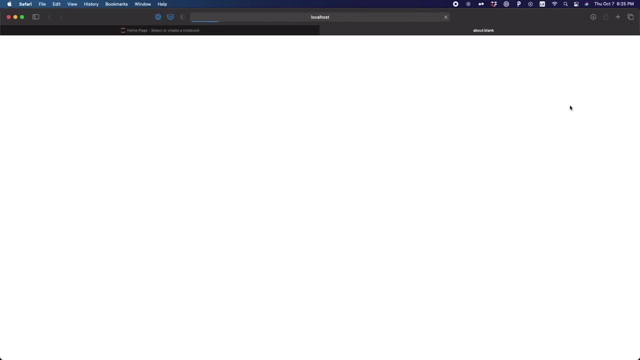 the Jupyter lab and Jupyter notebook, which are widely used in data science. So I'm going to launch Jupyter notebook. So here it's, opening Jupyter notebook. Let's give it a second. And now we open a new notebook with Python three. So Python three was installed too, And that's it In. 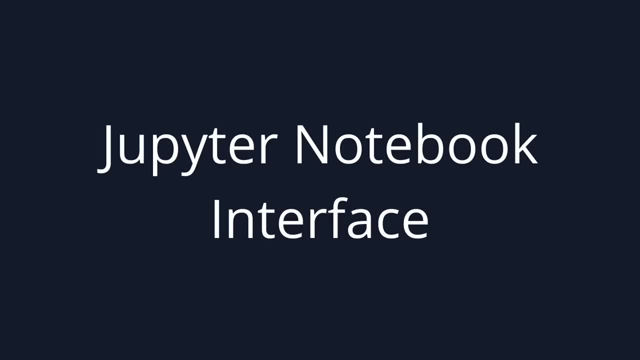 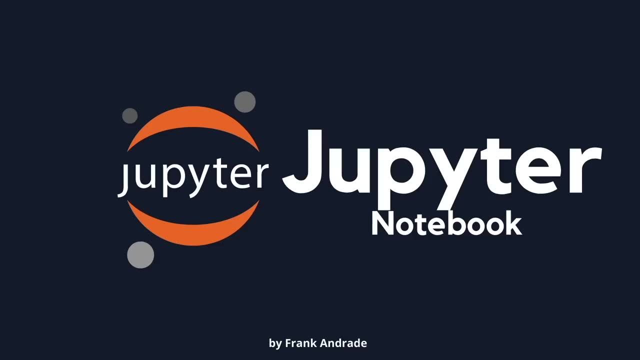 the following videos, we'll learn how to use Jupyter notebooks. In this video, I will introduce you to the Jupyter notebook interface. Jupyter notebook is an open source web application that allows us to create and share documents that contain live code, equations, visualizations and text. This is a perfect text editor for doing data. 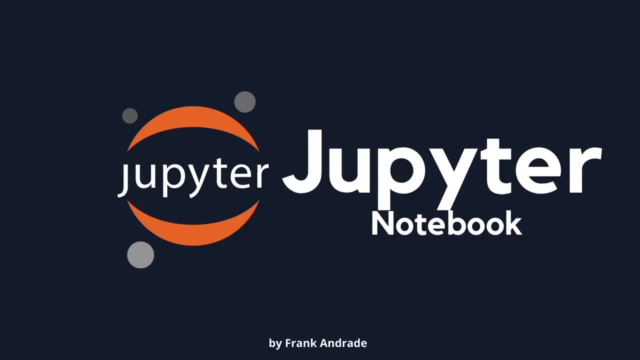 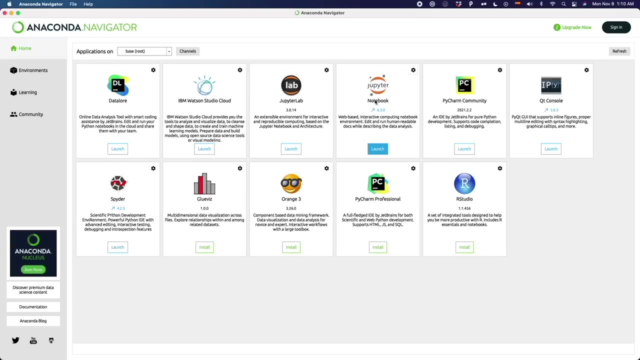 cleaning and transformation, data visualization and data analysis. This is why Jupyter notebook is widely used in data science And also machine learning. As you might remember, we installed Jupyter notebook in Python with the Anaconda navigator, And this means that we already have installed some popular libraries. 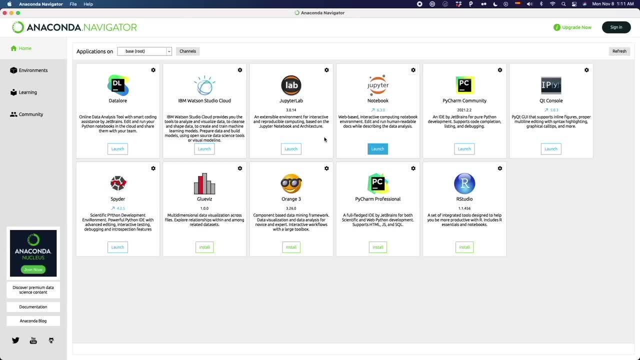 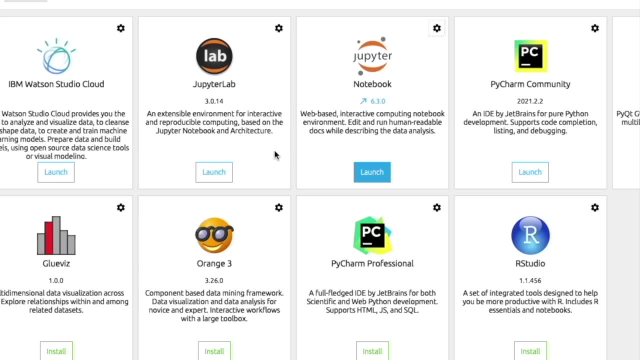 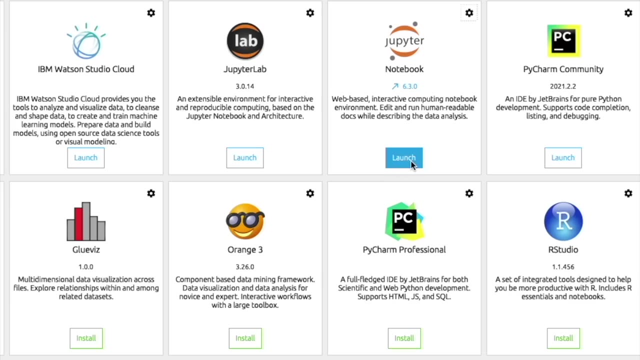 used in Python for data analysis. By the way, one of the alternatives of Jupyter notebook is Jupyter lab. Both are similar, but we're going to use Jupyter notebook in this course because of its simplicity. So let's open Jupyter notebook, And to do that we have to click here on the launch. 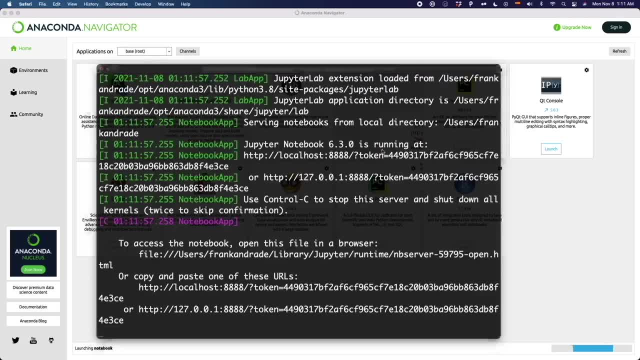 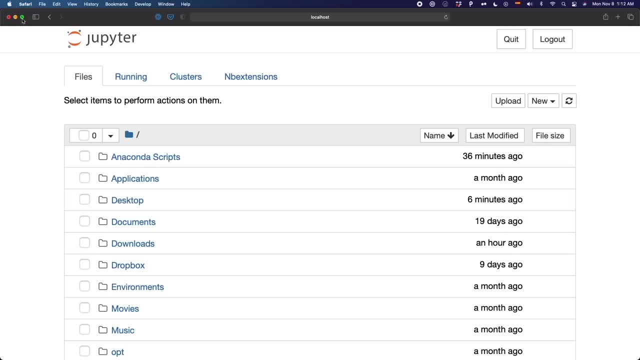 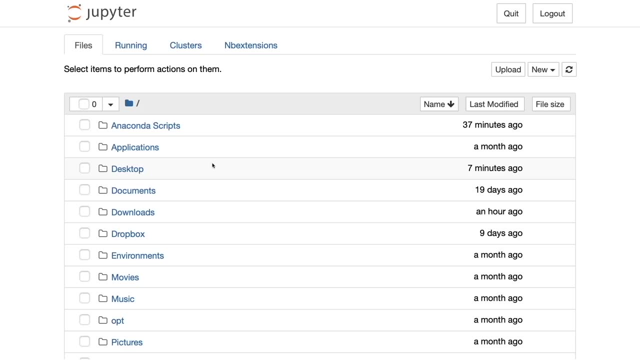 button. So I click here. you know we wait a couple of seconds And now we have here the interface of Jupyter notebook. So I'm going to maximize this And by default Jupyter notebook opens the root directory of your computer. it's a good idea to create a folder where all your 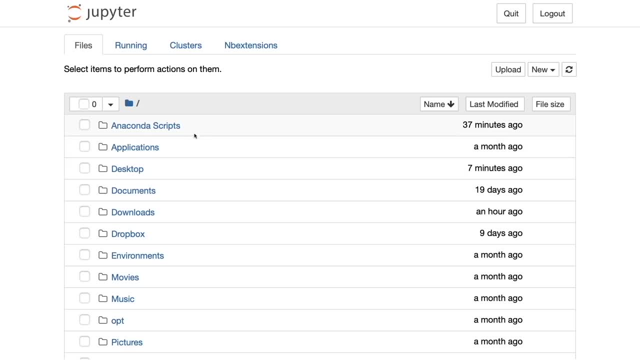 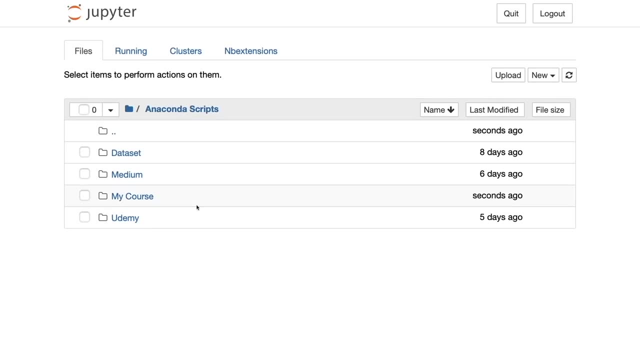 Python scripts will be located. In my case, this folder is called Anaconda scripts, So I click here And now I can navigate through the folders, and the folder I'm going to use for this Example is this one that says my course, And here we're going to create our first Python script. 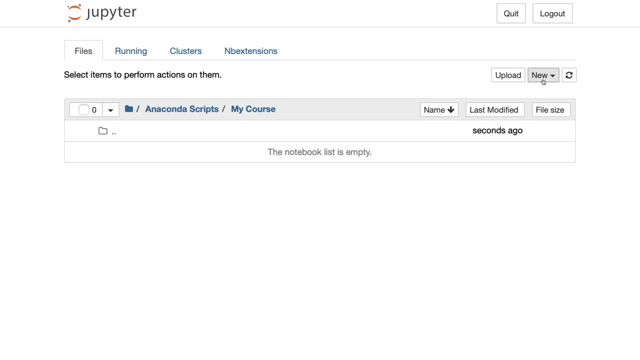 To do that, we click here, on the new button. So click here, and we have to click on the first option that says Python three. there are other options, like text file folder or the terminal, but we're not going to use these options in this course, So click on Python three. 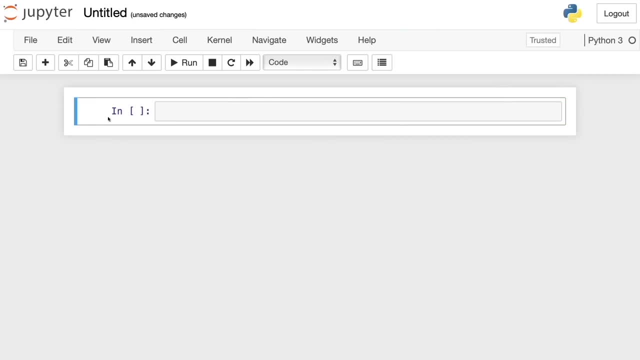 And now we have a Python script powered by Jupyter notebook. So here on the right you can see that it says Python three And also there is the Python logo, And on the left you can see here the Jupyter notebook logo and also the name of this Jupyter notebook file. 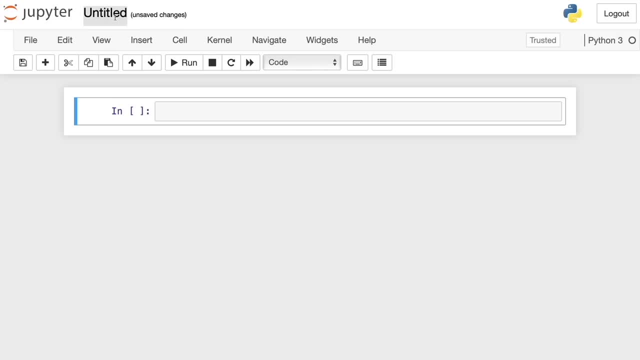 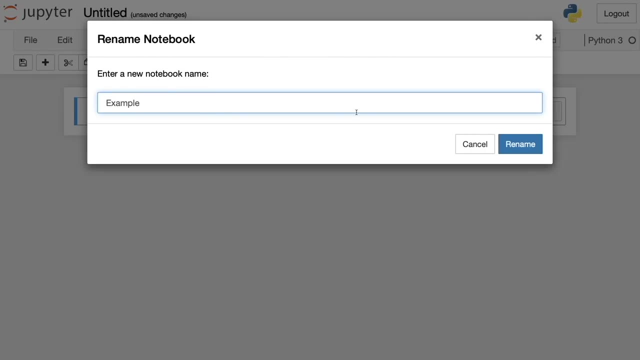 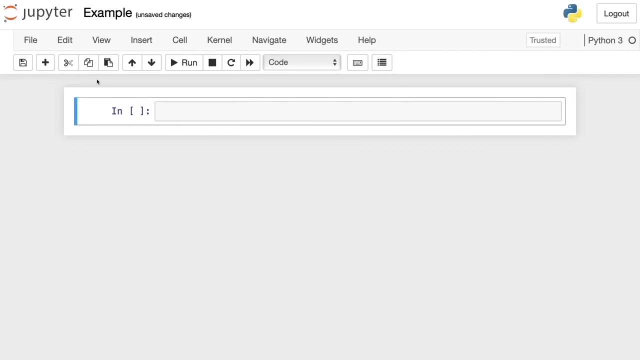 we can change the name of the file by clicking here on untitled. So I click here and I can change it to, let's say example: So I write example and I click on rename, And now we rename this Jupyter notebook file. Alright, now let's navigate through this menu bar that we have. 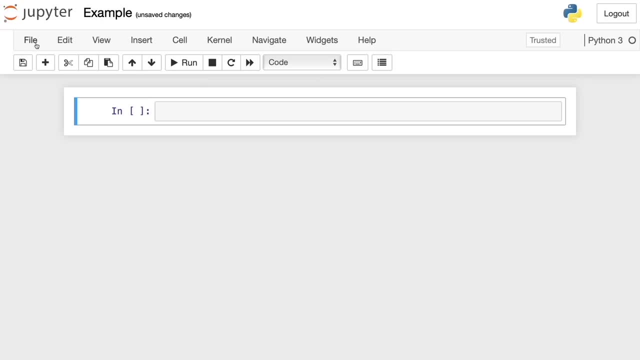 here in this Jupyter notebook file. So the first option is the file. In here we can create a new notebook with Python three. So if we click here, we're going to open a new Jupyter notebook file from scratch, as we did before. then we have the open And in this case we can open a Jupyter. 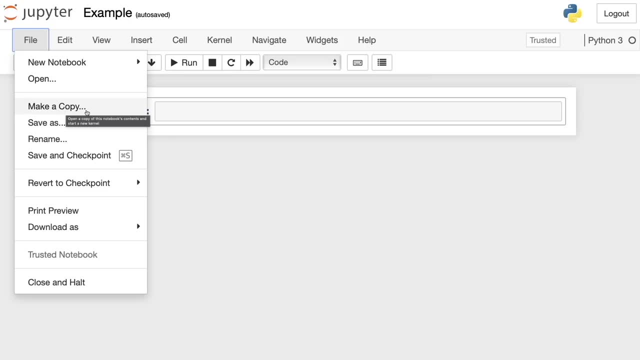 notebook we created before. we can also make a copy to a Jupyter notebook And then change the name. we can save a Jupyter notebook file and rename the file as we did before. we only click here and rename the file. then we can save all the progress we make in Jupyter. 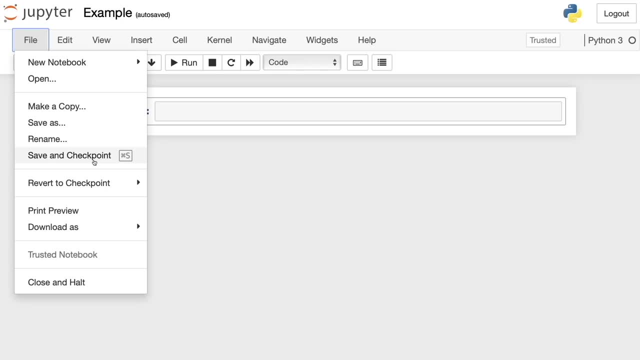 notebook. For example, after writing many lines of code, you can save all the progress you make by pressing Ctrl S or Command S on Mac and you're going to create a checkpoint And later you can revert to a previous checkpoint by using this option here. 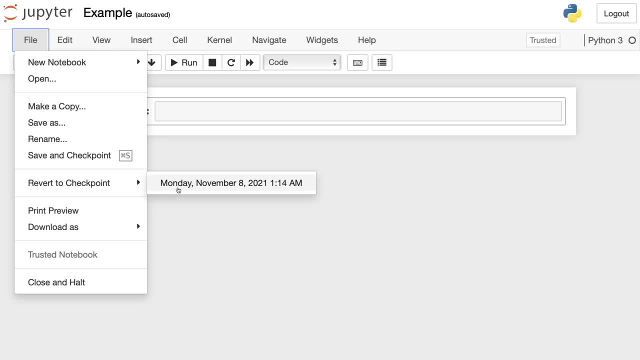 So here you will see many checkpoints and you can revert to a previous checkpoint. By the way, by default Jupyter notebook makes saves every 30 seconds or maybe one minute, So there is no need to press Ctrl S every time. So keep that in mind. 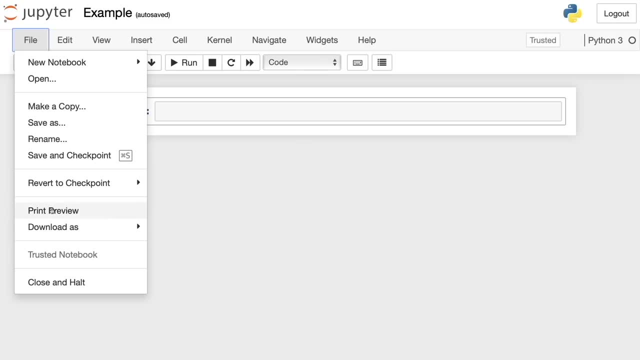 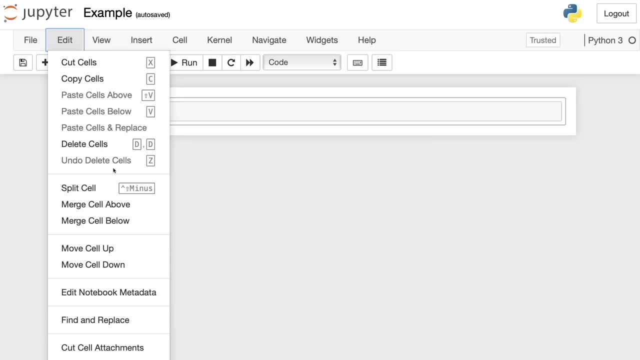 Then we have other options that I don't use so much, like print this Jupyter notebook or export that Jupyter notebook file to HTML or PDF, and so on. Okay, now let's see the second option that says edit, And here we can edit all the cells we have here in this Jupyter. 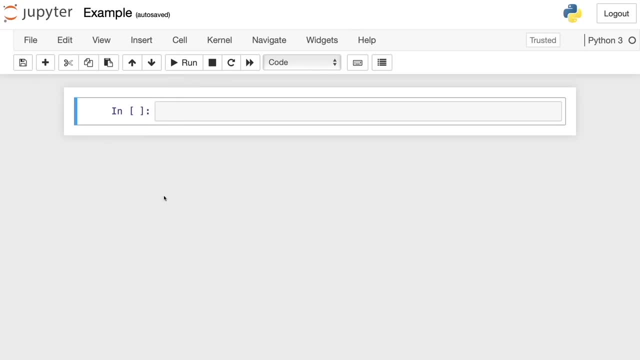 notebook, By the way, here. what you see here on the screen is a cell, So we can edit with this edit option. For example, we can cut cells, we can copy cells, paste cells above and delete cells. On the right you can see the shortcuts that we're going to see on the next video in detail. 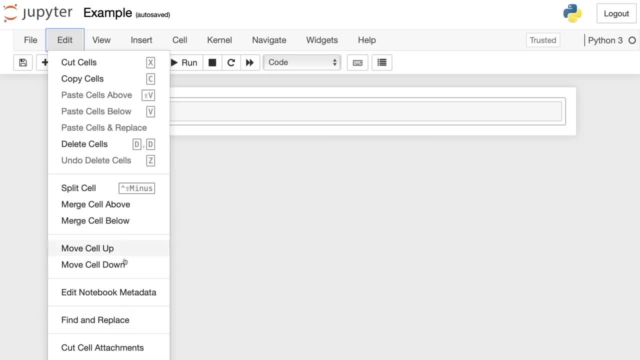 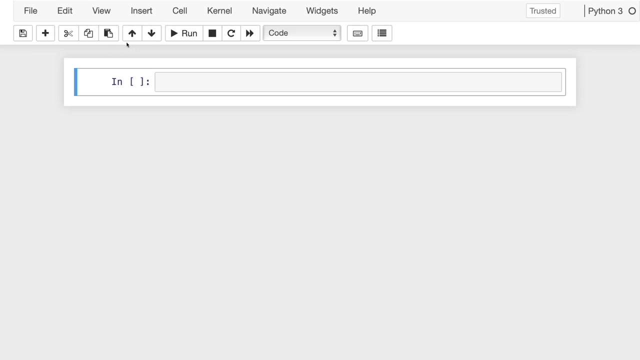 And well, you can check all the edit options that you can perform on Jupyter notebook here. then in the view option we can toggle the header, the toolbar and also line numbers. So here if I click on toggle header, the header is going to disappear, And if I click on toggle toolbar, 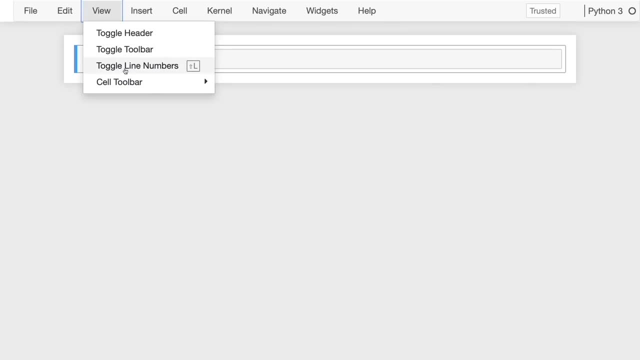 this toolbar disappears to also here in toggle line numbers. we can show here line numbers. So if I write anything, we can see that it says 123 and so on. And I'm not going to use this for this course. I'm going to leave it with the default options. So 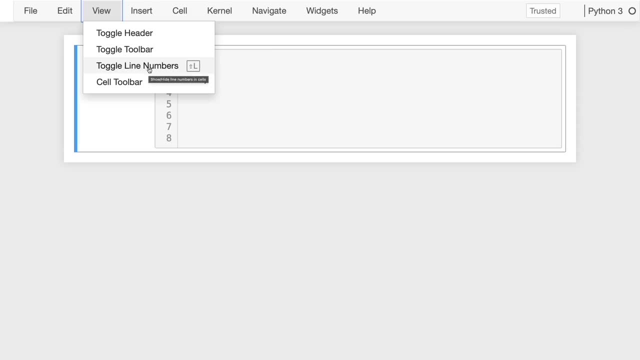 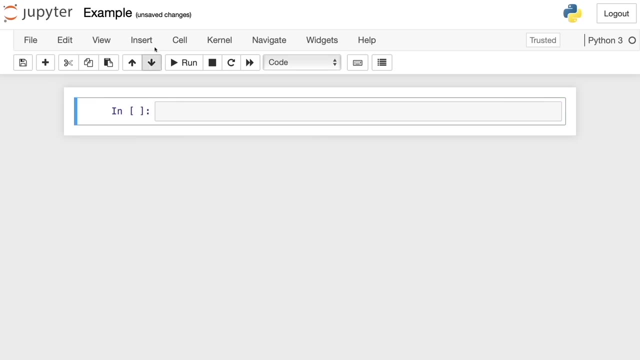 here I'm going to revert to the original option, So without line numbers, and I want to show the header and also the toolbar, but you can personalize it as you want. Next, in the insert options, we can insert cells above or below. we only click here And well, we're going to see the 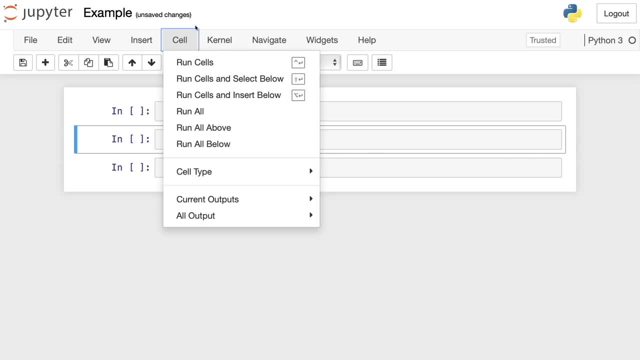 shortcuts later in the next video. then we have the cell options. we can run cells or run all the cells in this Jupyter notebook, And here we can see that we have all the cells that we want to use in this Jupyter notebook file. And then we have that kernel option, And a kernel is a. 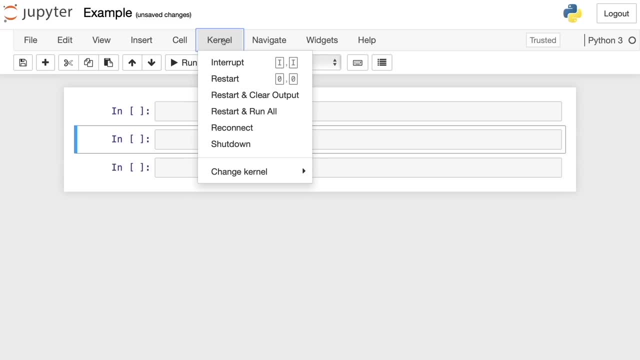 computational engine that executes the code contained in a notebook document. When we open Jupyter notebook, a kernel is automatically launched And we can interrupt this kernel by clicking here. So by interrupting we can pause the execution of a code. we can also restart. 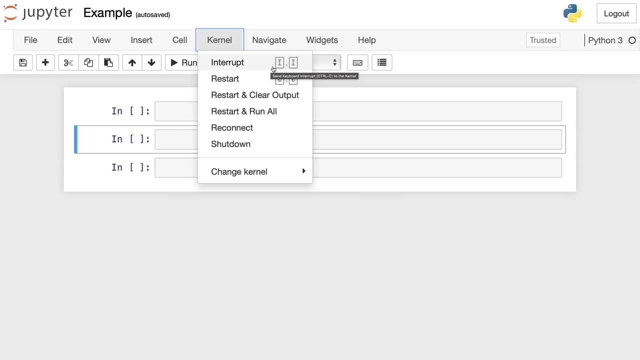 everything and do more things here. Sometimes, for example, I interrupt the kernel when a line of code, a cell, takes too much time to execute. And well, you can do the same here with restart or interrupt. Then we have the navigate option. that doesn't actually have anything here. 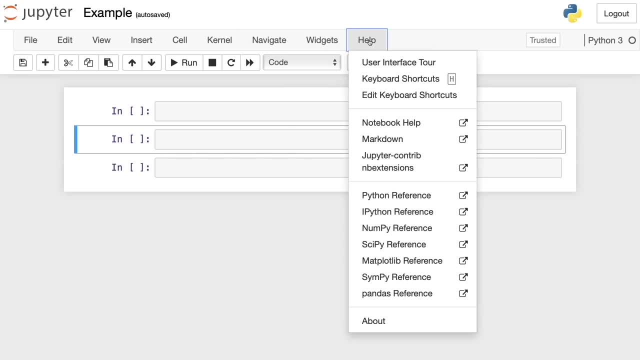 widgets that I don't use so much and will help that. I think it will send you to that documentation of Jupyter notebook and you can read it if you want. All right here. then we have the toolbar, And here you will find some shortcuts of the menu bar that we've seen. 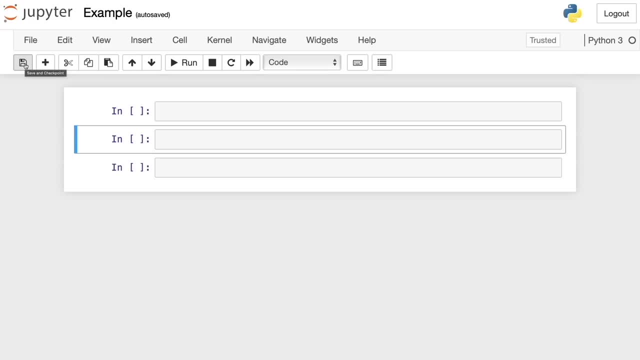 for example, here you can save and make a checkpoint. So here I click here And as you can see here it says checkpoint created or something like that: Yeah, checkpoint created and the time that it was created. then you can hear with this plus button insert cell below. 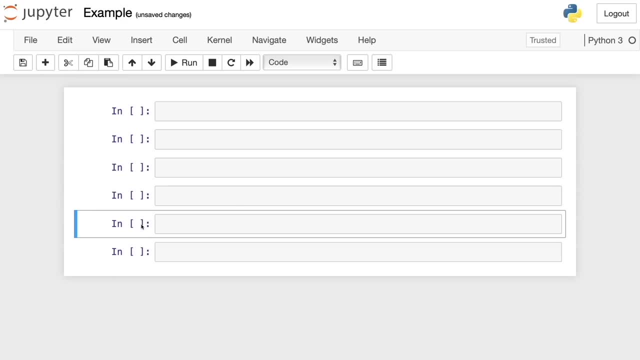 So I click here And, as you can see, we can insert a cell below And also you can use shortcuts, but that I'm going to show you in the next video. then we can select its pose with this button. we can copy a cell with this button And also we can paste cells. 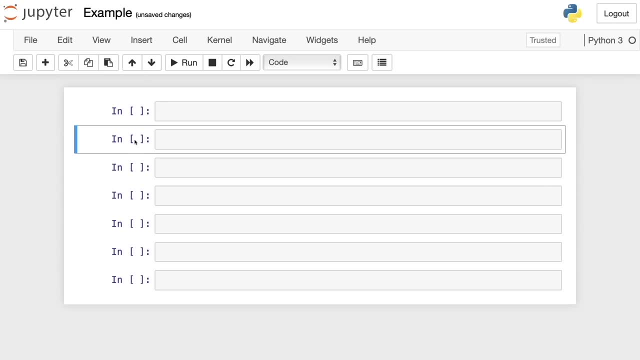 below. Also, we can move a cell above or below. For example, I'm going to write anything here in this cell. I can move it above with this button or below, As you can see here. then we can run this code. For example, I can write the number one and then run the code. And, as you can see here, 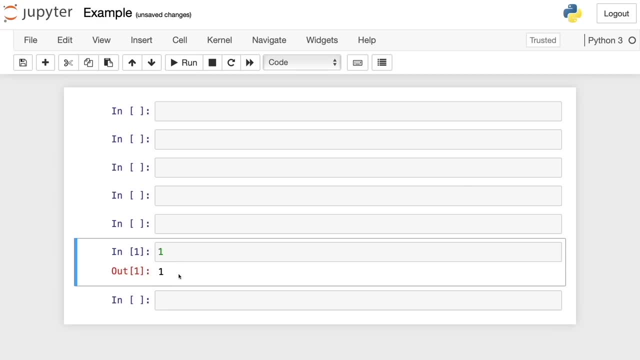 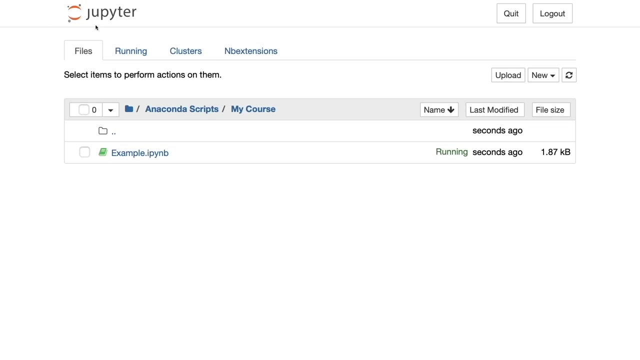 the code ran shows the number one. And well, those are some of the frequently used buttons in the toolbar, And that's everything you need to know about this Jupyter Notebook file. Okay, now, before finishing this video, I'm going to show you some other options that you can find here in the Jupyter. 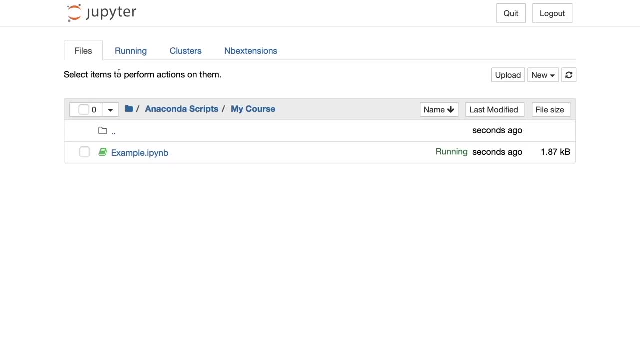 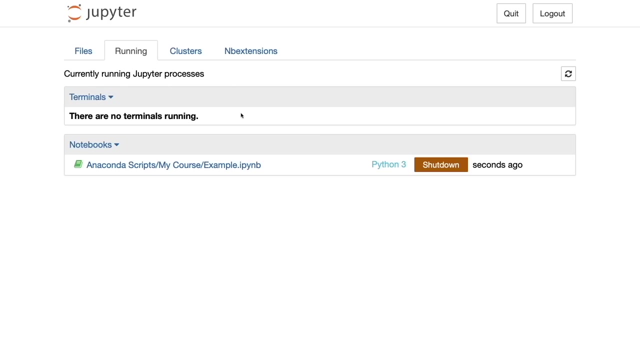 Notebook interface. In here you can see that there are some other options. So right now we're in the files tab And we can change to the running tab here And here you can see all the currently running Jupyter Notebook processes. For example, we can see here that Jupyter Notebook file we 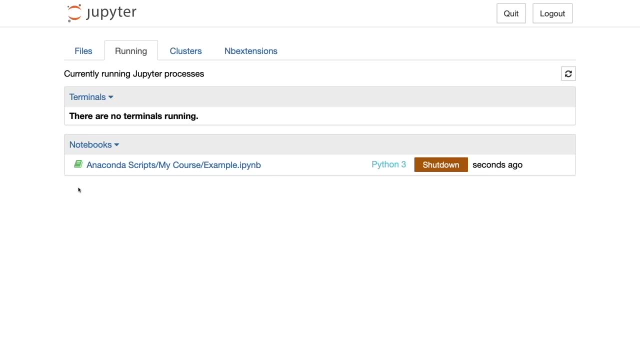 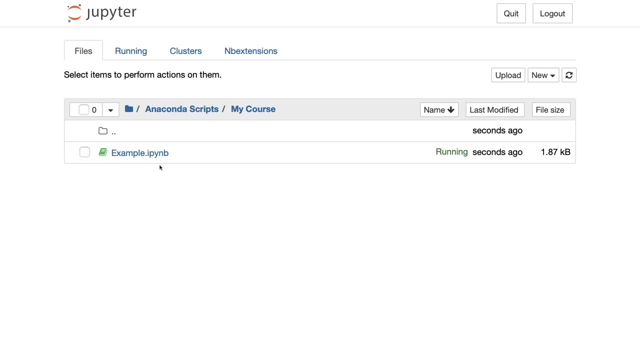 created and that we opened, So you can recognize that a Jupyter Notebook file is open or that is running, because here the icon will be in green. So here, if we go back to the files tab, we can see that this Jupyter Notebook file, which by the way has the IP, Y and B extension, is in green. So the icon. 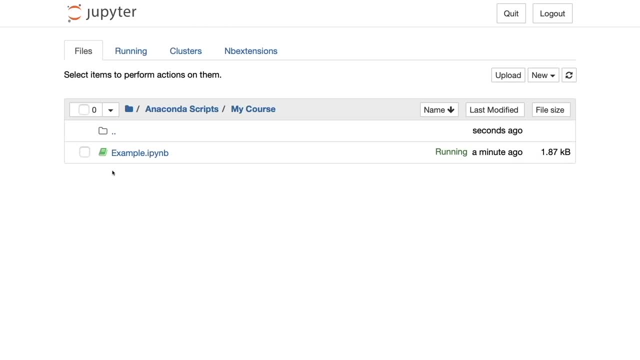 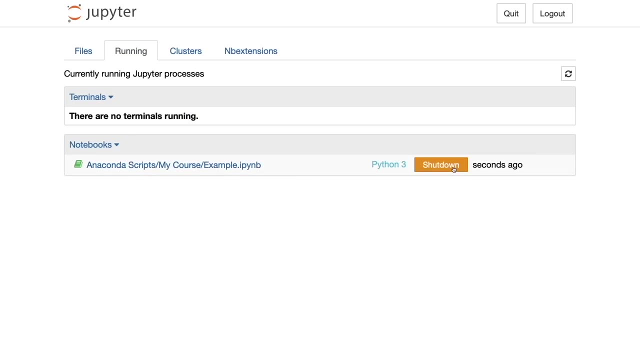 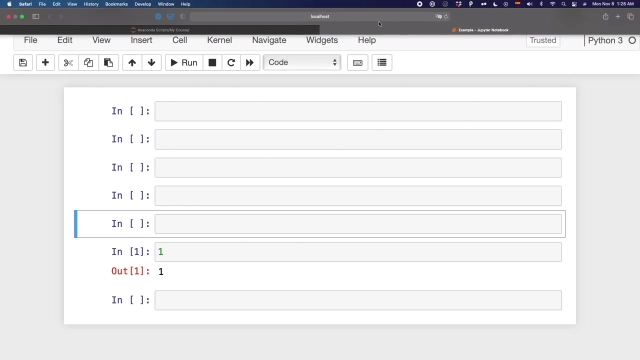 is in green, So this indicates that the file is running And well, it was opened. So here we can see that is open And we can shut down this file. And this is different from closing this file. For example, here I have the file And if I close this file, here we can see that the file 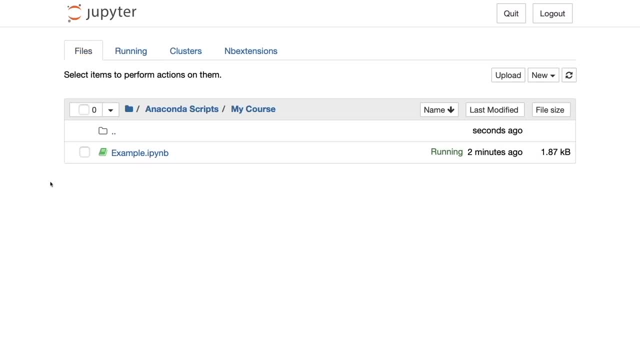 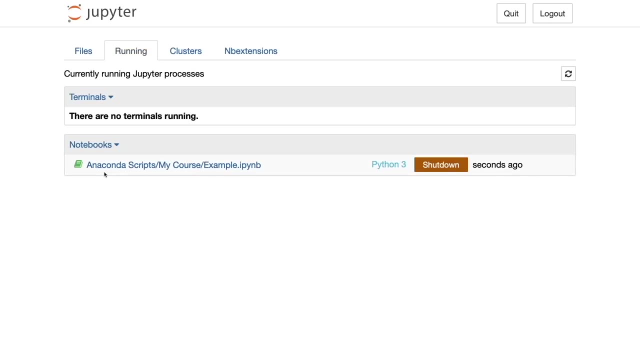 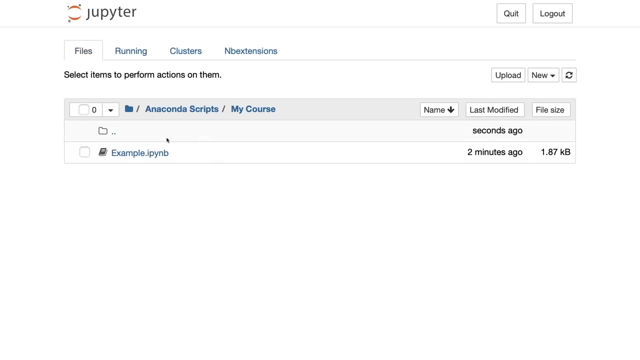 is a still running. Here we see running and is in green And in the running tab it still shows up. So if we want to shut down this file, we click here and it says that there are no notebooks running And we can see here that the notebook 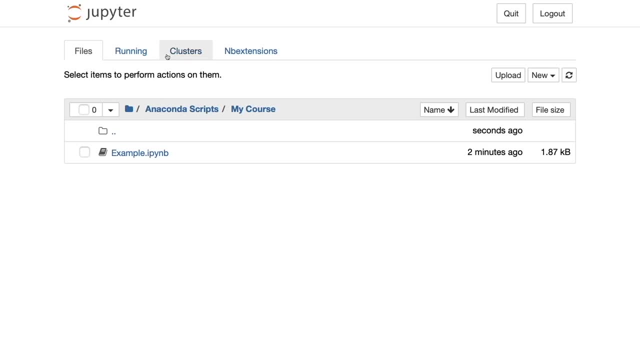 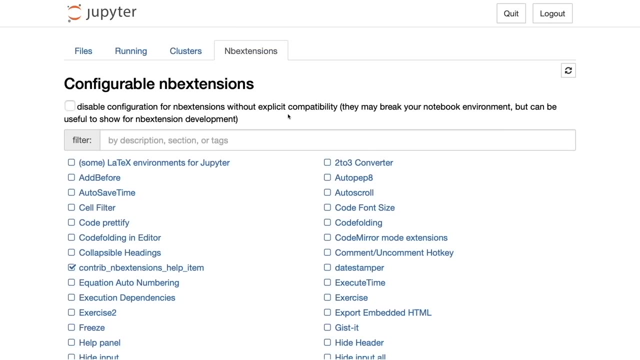 has a great icon Alright. then we have the clusters tab, And this tab I don't use so much And actually it doesn't show anything here. And then we have the NB extensions tab. Here you can can install any extension to personalize Jupyter Notebook even more, And we're going to see some 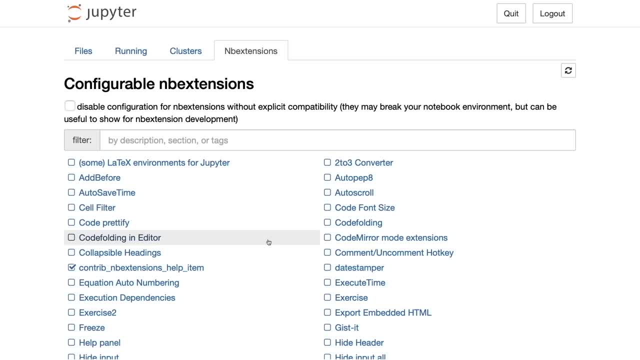 cool Jupyter Notebook extensions in the next videos. And, by the way, this nb extensions tab doesn't show up in some versions of Jupyter Notebook, but we can easily install it And we'll also see how to install this nb extensions tab in the next videos. Finally, we have this box. 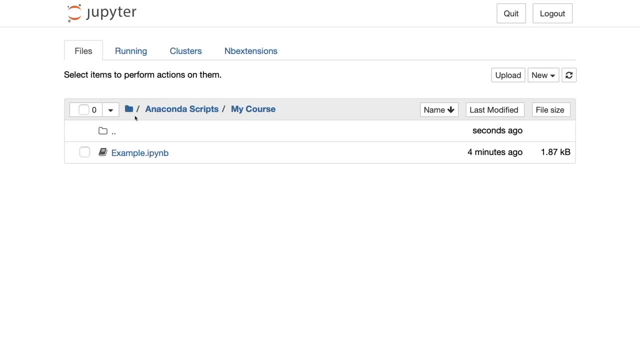 that shows our directory. So here this folder indicates the root directory. So if I click here, we are not in the root, And if I click on the folders- anaconda script- and then my course, I go to the folder where I was before And that's it. These are all the things you need to know. 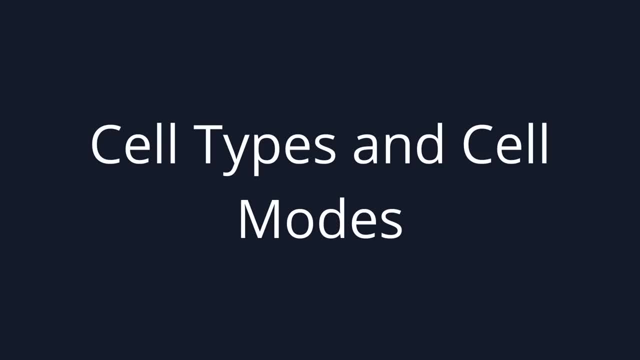 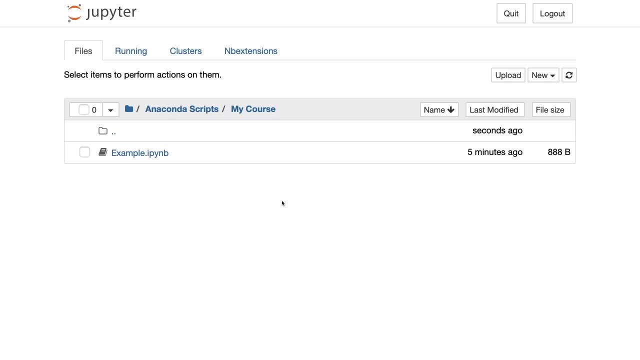 about the Jupyter Notebook interface. Okay, in this video we're going to see some cell types and cell modes in Jupyter Notebook. So first we're going to open the Jupyter Notebook file that we created in the previous video, which is this one example, that's. 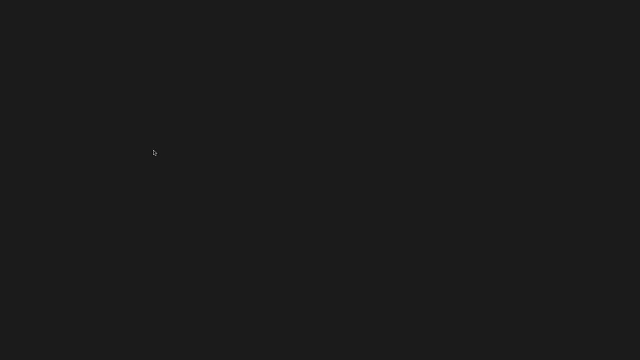 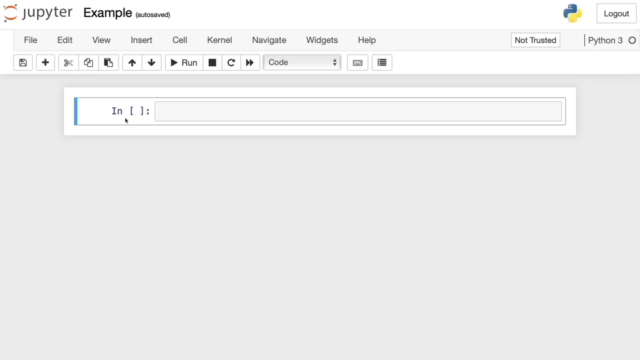 at I P y n b. So we click on it And here we have the Jupyter Notebook file opened And here by default we have this four sold in Command Mode. And we can say that this is Command Mode, because here this blue color indicates that the cell is in Command Mode. And when we are in Command Mode 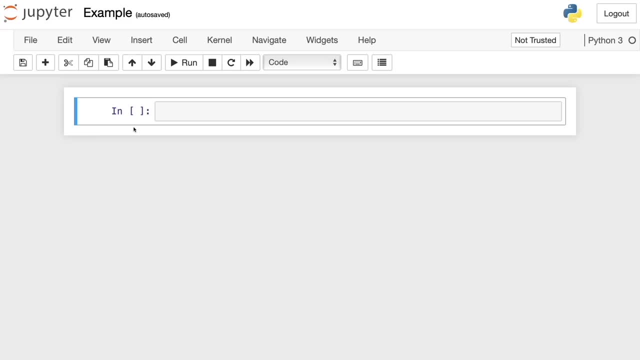 we can do things outside the scope of any individual cell. So basically, all the tools we see here in the toolbar, we can apply it in command mode. Also, in command mode we can apply some shortcuts that I'm going to show you later. And, for example, if we want to see the shortcut window, we press. 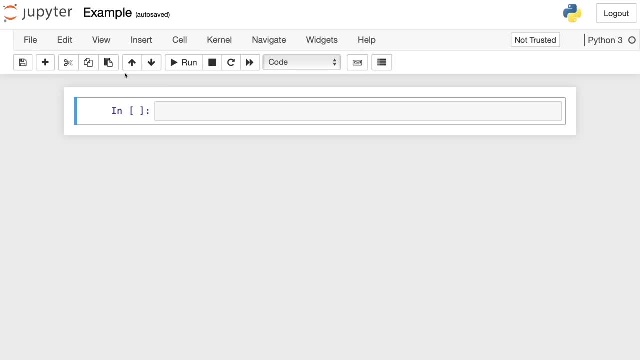 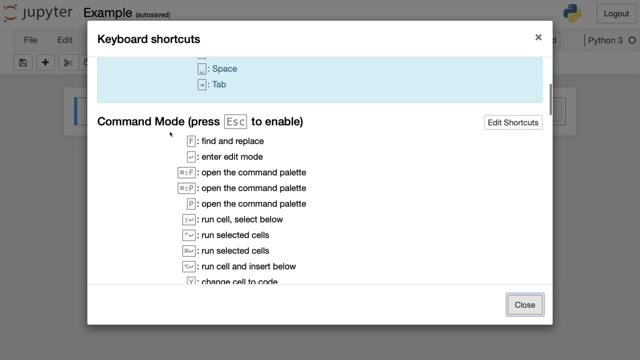 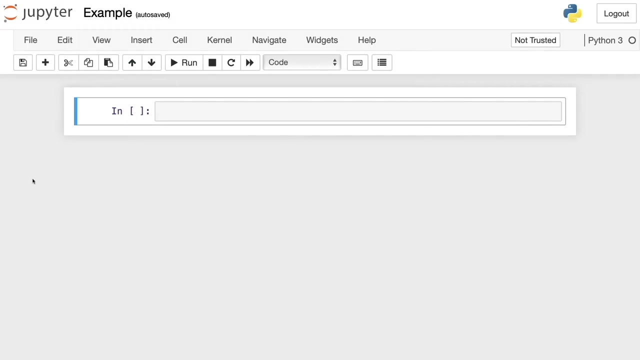 the letter H in command mode And we can see the keyboard shortcuts here. So here you can see all the shortcuts and all the shortcuts that you can apply in command mode- Now I'm going to close this one- And also you can apply different shortcuts, like for example, 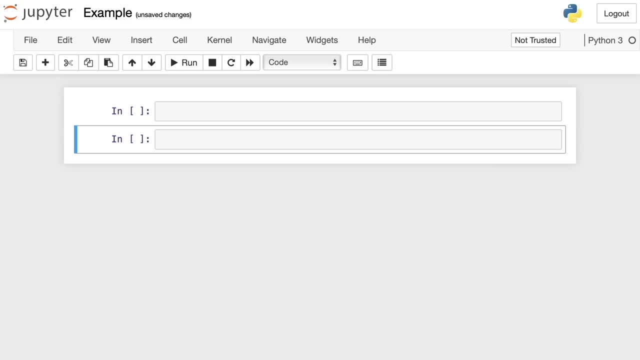 if you press B in the command mode, you will see that there is a new cell, because B is the shortcut that introduces a new cell below. Now, if we press Enter, you're going to see that the color is going to change to green. So here we have green color And this green. 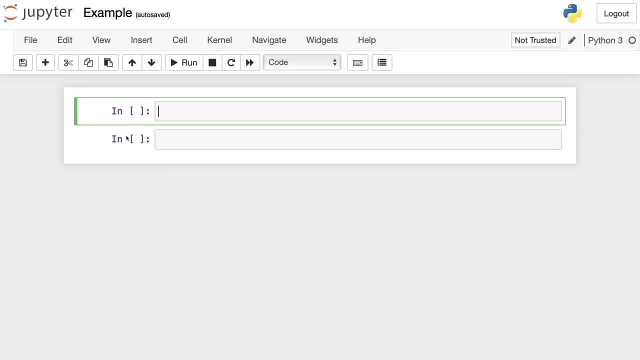 color indicates that we are in edit mode, And edit mode is for all the actions you will usually perform in the context of the cell, For example introducing text or writing code. So here I can write, say, 123.. So if I write 123, and then I click on this Run button, I'm going to run. 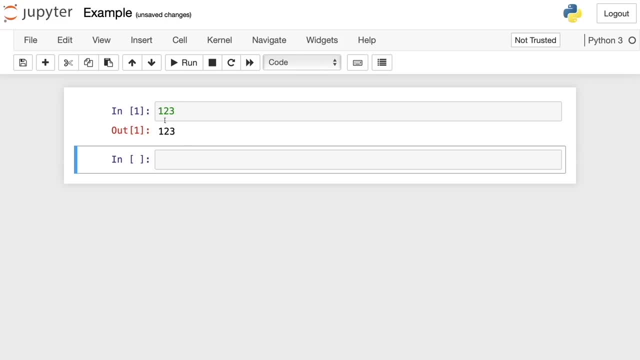 the cell And as you can see here, I run this first cell And also after running the cell, you can see that we are again in command mode. So to go to edit mode, we press Enter again And now we can edit the numbers we introduced. So for example, I can write 456 and then run. 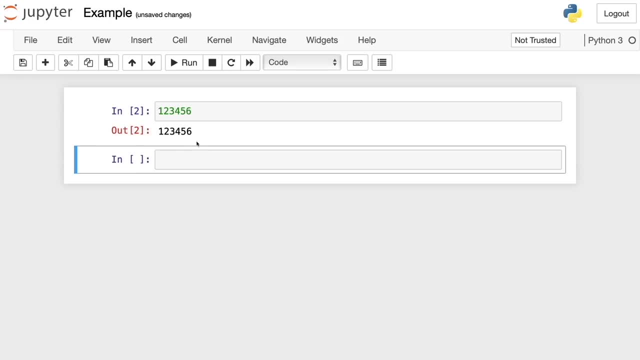 again, And here you can see that the output shows 12345 and six. by the way, if you try to use the shortcut in edit mode, it won't work here. press Enter. And now I'm on edit mode. And if I press the, 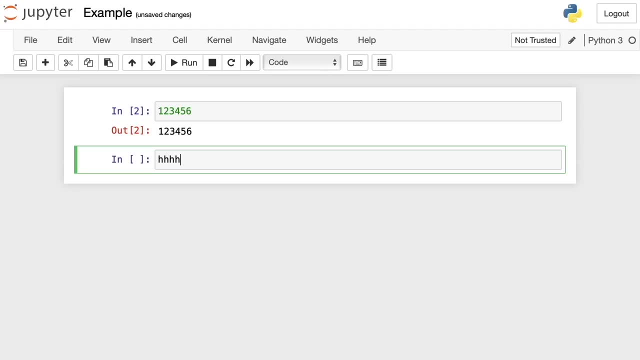 letter H, you can see that nothing happens. we don't have the shortcut window. And if I press the letter B, you can see that we don't insert any cell below. this happens because those shortcuts work only on command mode. So to escape this edit mode we have to press the escape button. So I press escape And 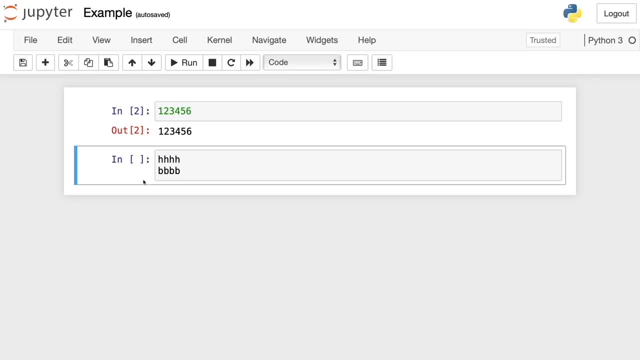 now I'm again in command mode. So if I press H, we have here the keyboard shortcut, And if I press B, you can see that we inserted a new cell. And that's it for the command in the edit mode. Now we'll see the cell types in Jupyter Notebook. In Jupyter Notebook. 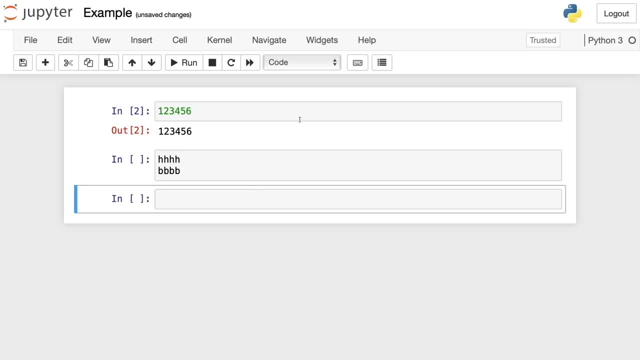 there are three main cell types And we can see all of them in this drop down here Right now. the type of this cell is code, So here it says code, But if we press here you can see other cell types like markdown and row, and be convert. So we're going to see first. 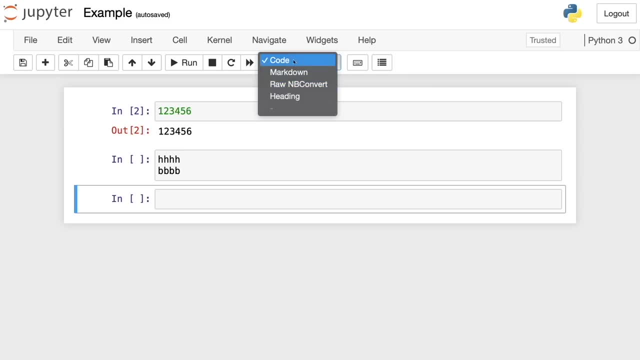 the code cell and it already has the check. So this one is a code cell. So now I press here, and now, well, it's in code cell. If I press Enter I'm in edit mode And here I can introduce any code I want. So here I can write any number- 999.. And if I press Ctrl, 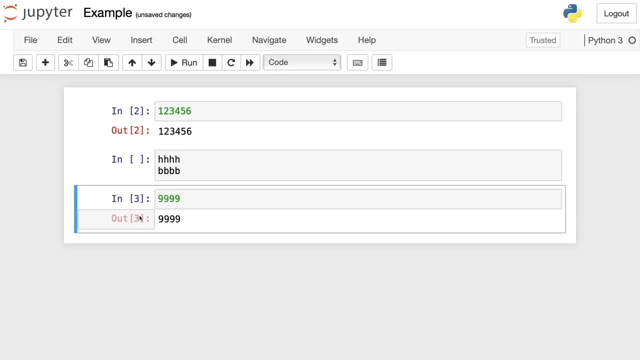 Enter here. this is the input, And here we got the output of this code. we're going to see how the code cell works throughout this course, But now it's time to see how the markdown cell works in Jupyter Notebook. So here I'm going to the cell, and now I'm going to change. 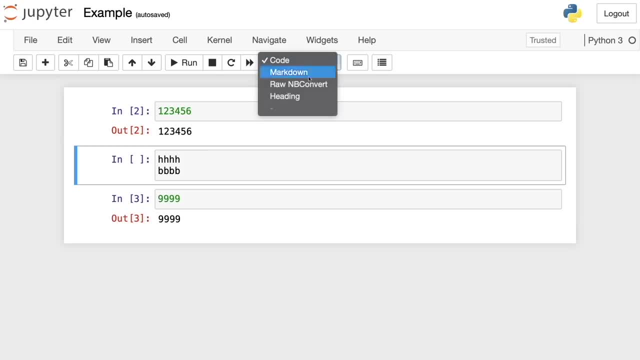 the cell type. So I press here in the drop down And now I select markdown. in the markdown cell we can introduce any type of text we want. For example we can introduce titles. So if I delete this and press the hash sign, 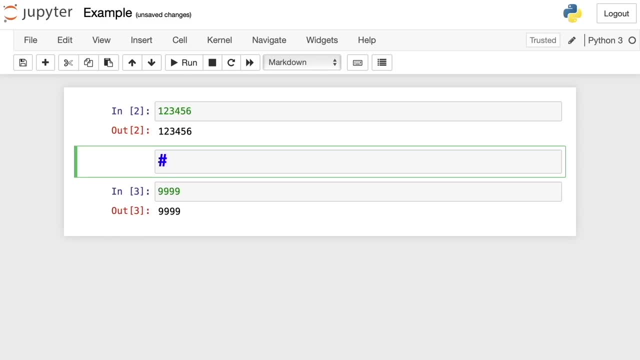 we can get TIDAL, So one hash. it means title, So here I press Space, you know I write title. Now we press Ctrl, enter or this run button to run, to turn this cell. And here we got the title. 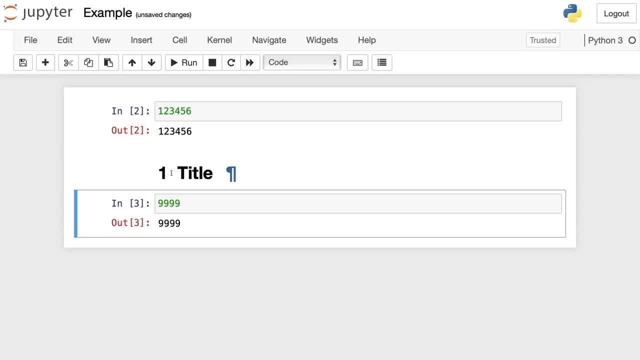 By the way, you shouldn't get this one number because I just modified the default behavior of Jupyter Notebook. So mine enumerates the titles and subtitles, But in your case you will see only the titles in the script. So now in here we've got the running up finally. 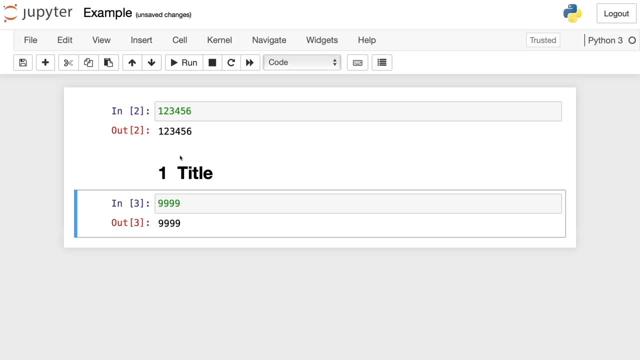 word title And if you want, you can introduce also subtitles here. So for example I'm going to insert a new cell with this button is plus button, And now I'm going to move this cell up with this button here. So I press this And now I'm going to change the cell type from 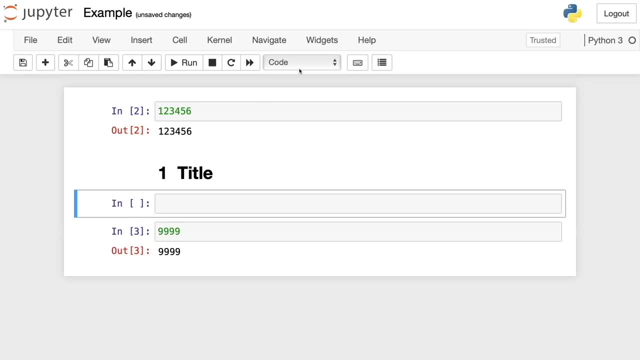 code cell to markdown cell. So I go to the drop down and select markdown. And by the way, you can change the cell type also with shortcuts. So if you're in command mode you can press the Y button to change the code cell. so I press the Y button. 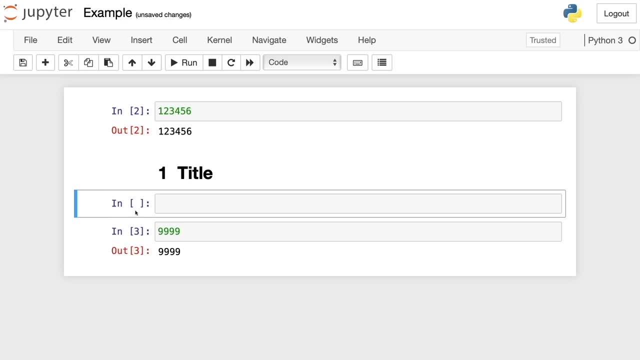 And as you can see, here it says in, and this in, with the square brackets, indicates that this is a cold cell. So here I can press Enter and introduce any code, here I introduce numbers and press the Run button, And here you can see that we have an input and an output. So this: 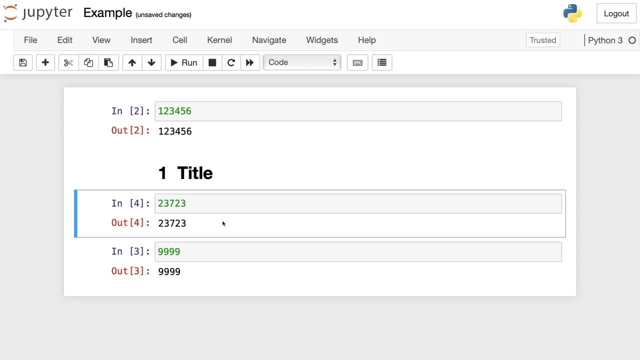 is the column we use In this example. I'm using the type that I have where, let's say, I'm supposed code cell, But now we can press the M button to make this cell a markdown cell. So now I press M. 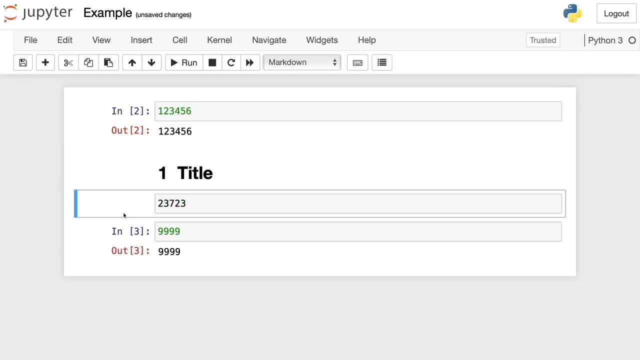 and here we are in command mode. So now we can get this markdown cell, And here you don't see the in word with a square brackets anymore. So now I'm going to edit mode. So I just press here, or well, you can press Enter to go to edit mode. And now to introduce a subtitle, I'm going to write. 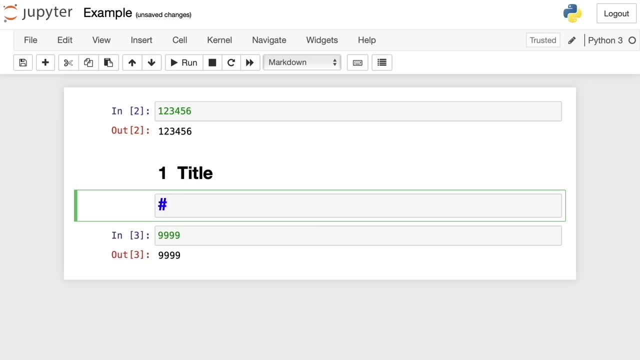 double hash sign. So I press hash sign twice, now a space. And now I'm going to write a subtitle. So I write subtitle, I press Ctrl Enter or the Run button to run the cell. And we got here the subtitle And we can also introduce text. I'm going to introduce a new cell with a plus button. 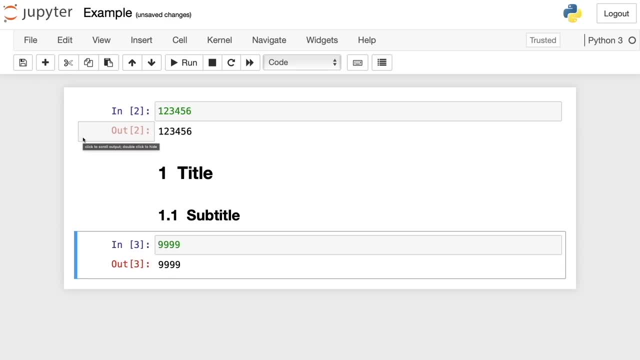 And you can also do it without B shortcut. So I'm going to do it with a B shortcut. Right now I press B And here I got this new cell And we can move this with this button here And now we have this cell in the position we want it. So here I can introduce. 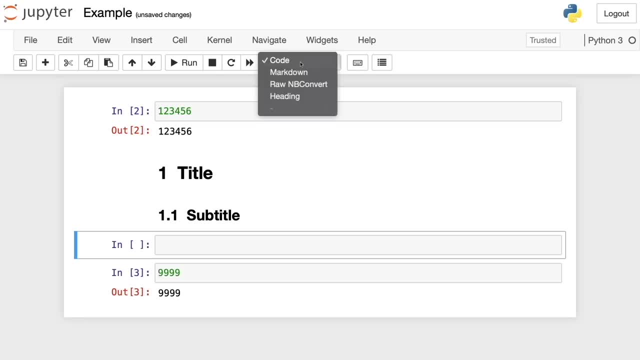 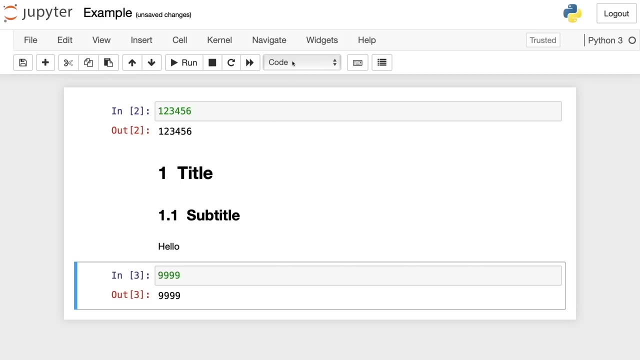 text by converting this cell to markdown. So here I choose markdown, Now you press Enter to go to edit mode And here I can introduce any text. For example, I can write Hello, I press Ctrl Enter And now we can see that we have here this text. And finally, the last type of cell is the. 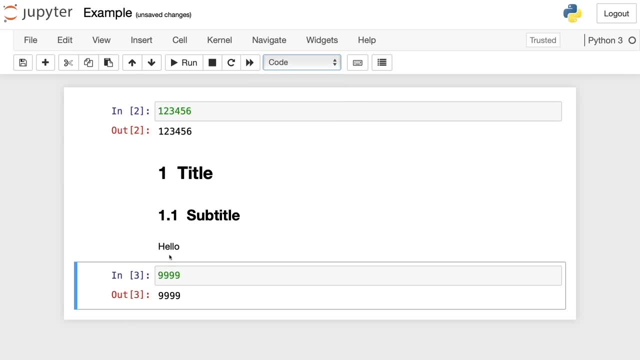 evaluated by the notebook kernel. So if we convert this code cell to a row cell, this cell won't be evaluated by the notebook kernel. So let's try here. I press row and B convert. Now we can see that this looks like a plain cell. And well, this type of cell is not used that often Actually. 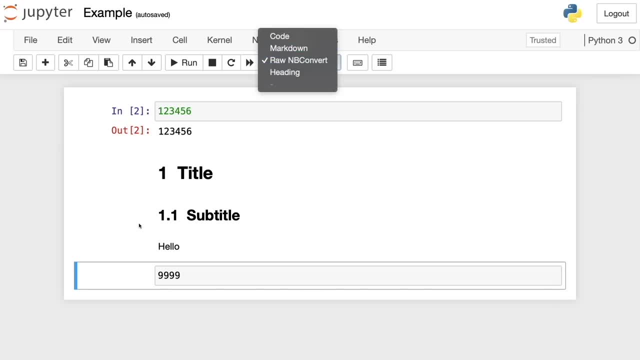 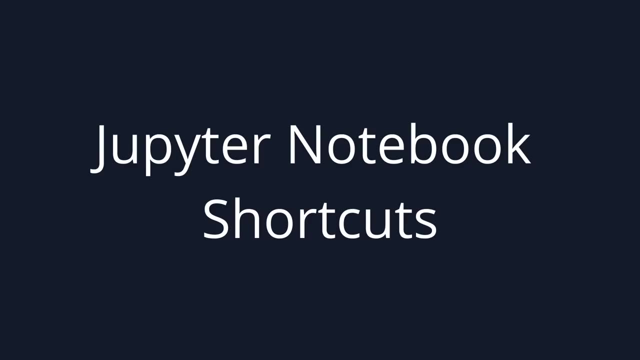 we're going to use only that code cell and the markdown cell in this course And that's it. In this video you'll learn the cell types and cell modes in Jupyter Notebook. Okay, in this video we're going to see some common shortcuts used in Jupyter Notebook And 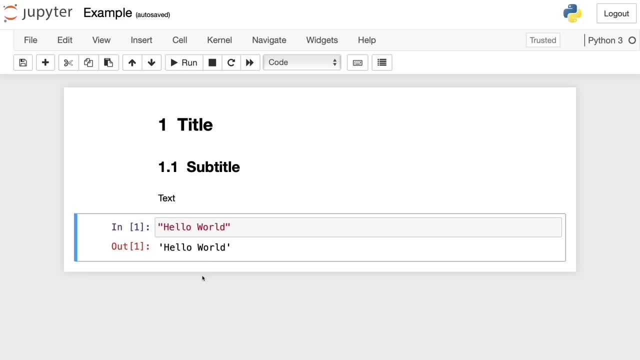 we're going to start with the F shortcut And, by the way, to use these shortcuts you have to make sure you're in the command mode and, to verify during the command mode, make sure that the cell has this blue color. Okay, now, during the command mode, you can press the letter F And you're going. 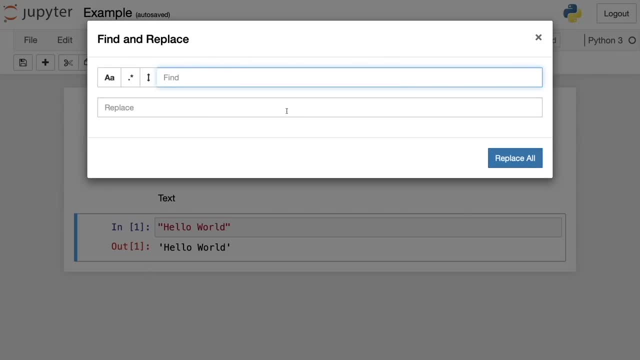 to see this. fine and replace. So this first shortcut allows us to find a word in the command mode And you can see that the cell is actually in the command mode, And we can also see that the a cell and then replace it with another word. For example, I can write here the word Hello. 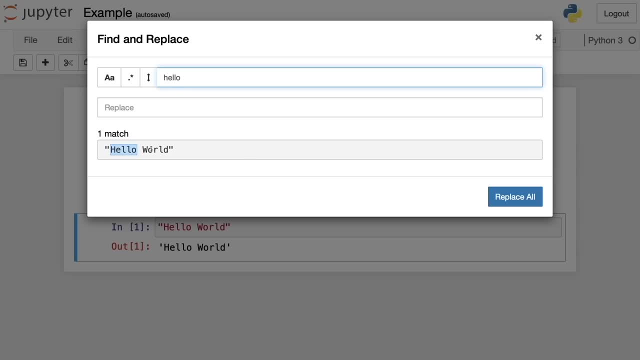 And here it found the word Hello inside this Hello world sentence, And now I can replace this word with the word say hi, for example. So here I write hi, you know, and read, we can see the match and in green we can see the word that we're going to insert. So here let's click. 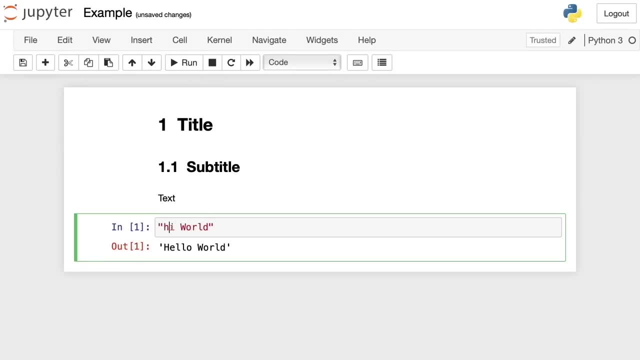 on replace all And now you can see that it doesn't say Hello world anymore, But now it says hi world. So now I press Ctrl Enter, which is another shortcut to run the cell. So you can press here on run or only press Ctrl Enter to run this cell. So I press Ctrl Enter And now we run. 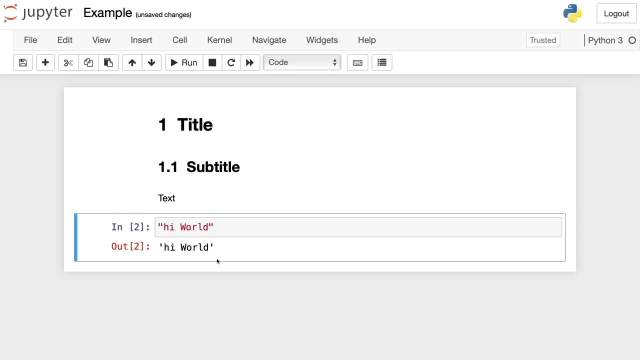 this cell in. another way to run cells is to press Shift Enter. But in this case we're going to run an insert, a new cell below. So now let's see, I press Shift Enter And not here. it ran the cell, because now it says in and three. 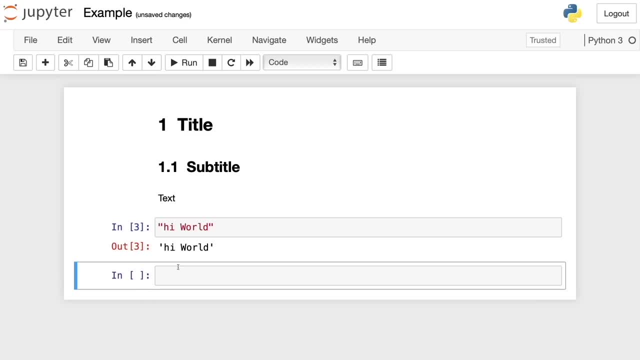 inside square brackets, And here we can see that we have a new cell. Okay now, another shortcut that is often used is the Y and M shortcut. So now this cell is a code cell, And if we want to make this a markdown cell, we only have to press the M letter. So we press M and this is going to be. 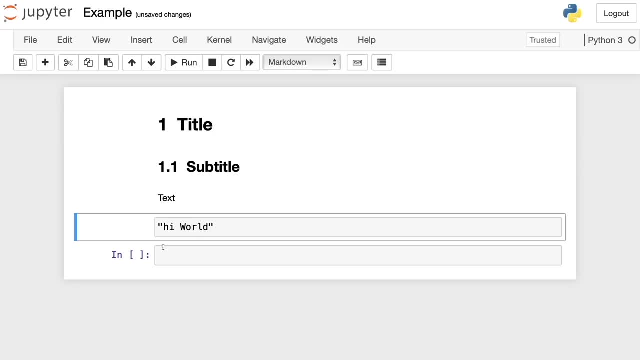 converted to Markdown cell. And if we press the letter Y, this is going to be converted to code cell. And also you can change the heading here. You can make the heading bigger or smaller. So here I'm going to locate this cell. 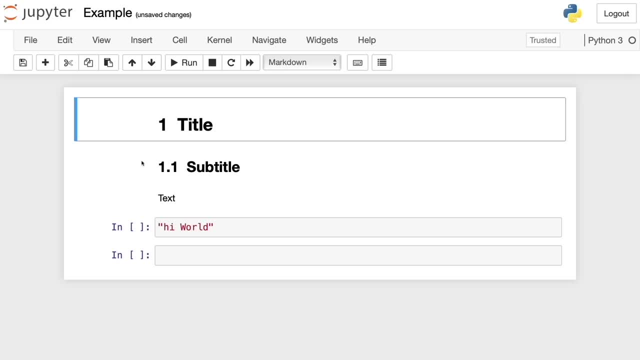 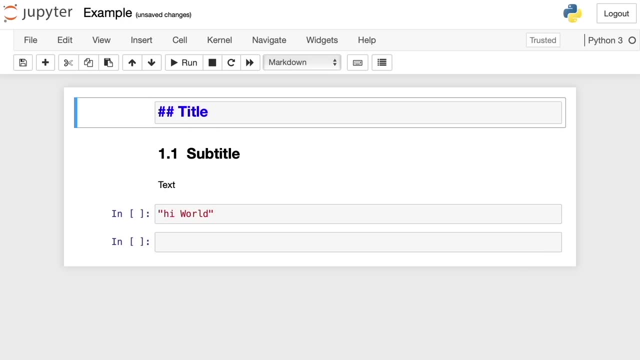 And now, to make this one smaller, we can press the numbers. So if we press the number two, we can see that this one gets smaller, And if I press number three, the title gets smaller for smaller and so on. So, as you can see, the more hash size, the smaller the text. So here I'm going to delete. 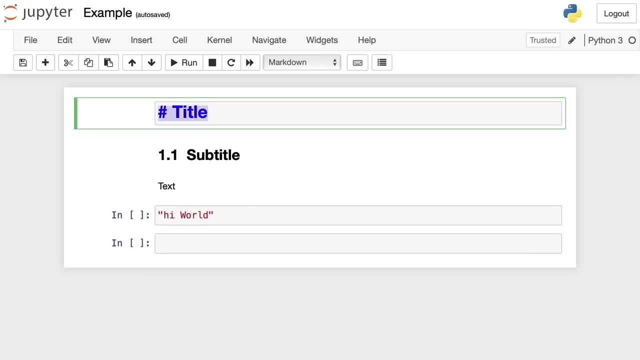 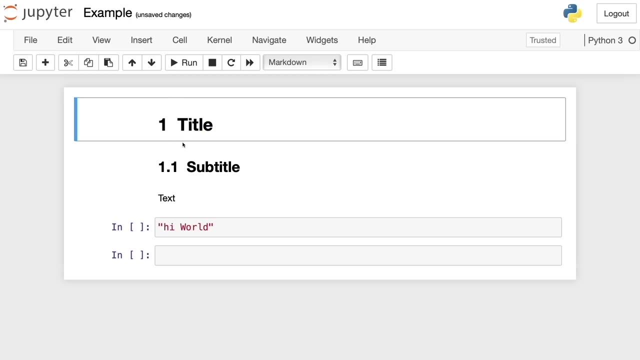 these hash signs, And one hash sign represents the biggest font size, which is the title. So now I press Ctrl Enter And now we have this in heading one. but if I press number five and then press Ctrl Enter, we can see that now this cell has heading five and it's 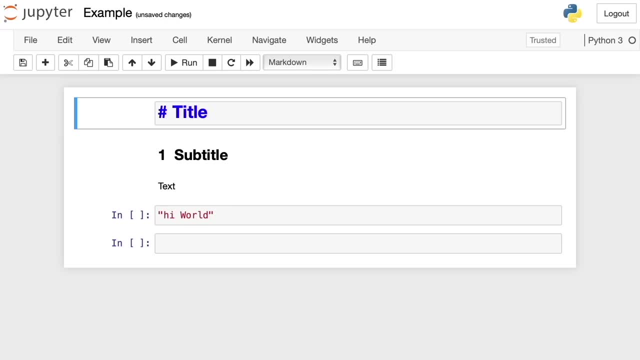 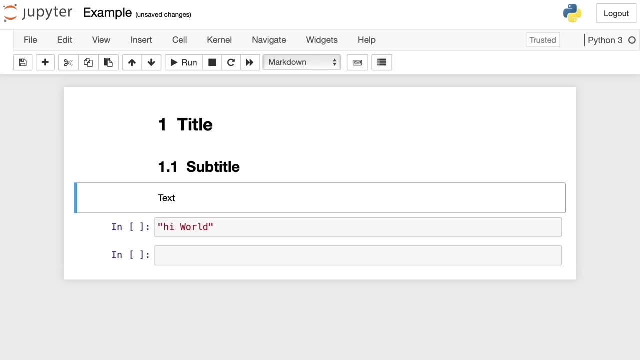 smaller. So now I'm going to revert to heading one. so I press one and then Ctrl, Enter. Okay, now we can navigate through the cells by pressing on the up or down keys on our keyboard And as you can see here, we can navigate through all the cells here Or we. 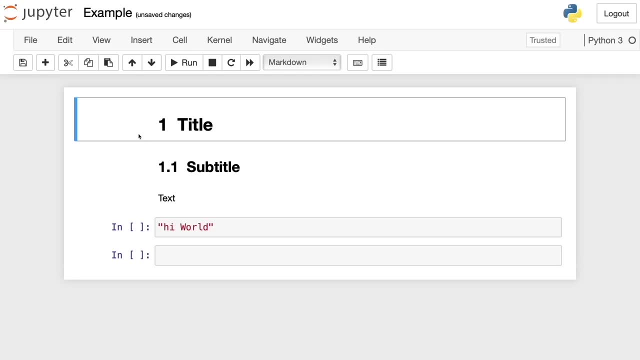 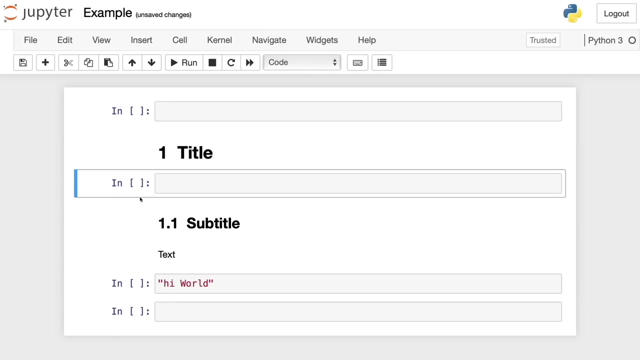 can also press with the mouse. we can press on the cells we want. Okay, now we can insert a new cell above by pressing the A key. So if I press A, we get here a new cell And above, And if I press now B, we get a new cell below. Now, if I press x, we're going to cut the. 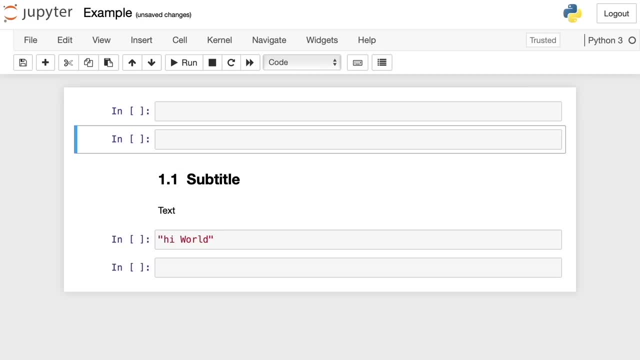 cell. So I press x And you can see that the cell was cut. And now if we press V, we paste the cell below. So I press V And now we got the cell. and if I press Shift plus V, we get the cell pasted. 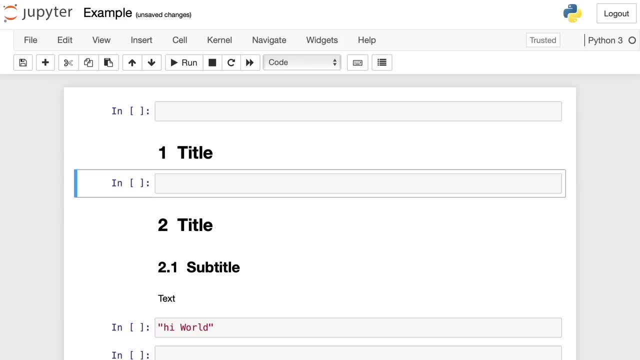 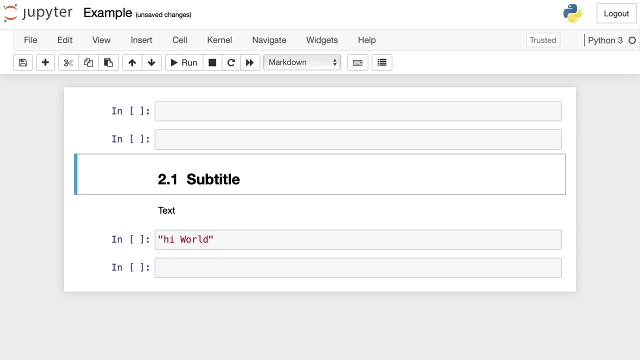 above. So I press Shift and V and we get this new cell above the cell I have here. Okay, now I can delete cells by pressing D twice. So I press D two times And, as you can see here, the title disappear. So now I tried again and we don't have the title anymore. But now if we press the letter, 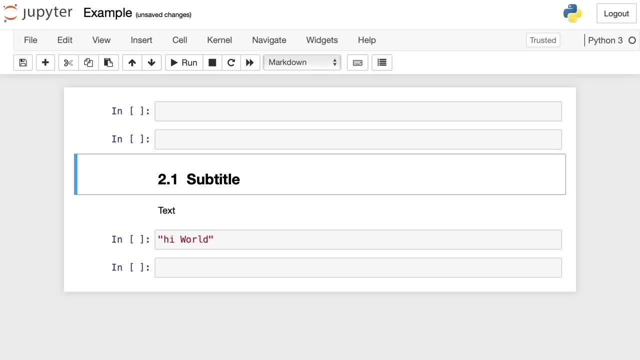 Z, we can undo those changes. So let's undo what we did before. I press Z and we get here the title back. Okay, another useful shortcut is that Ctrl s that allows us to save the changes we made in this Jupyter notebook file. So 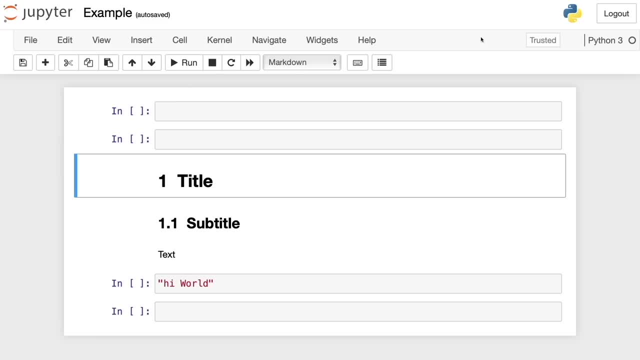 press Ctrl s And you can see here that says checkpoint created. So I'm going to press again Ctrl s And here it says checkpoint created And here also says the time. and that's it. These are some of the most common shortcuts used in Jupyter notebook, But you can see other shortcuts by 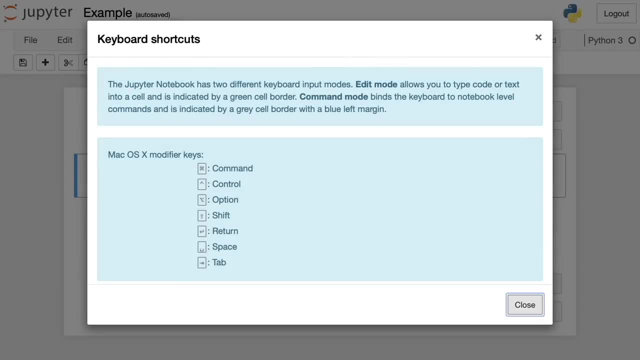 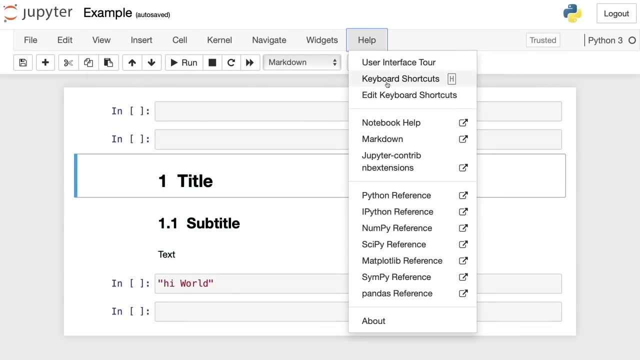 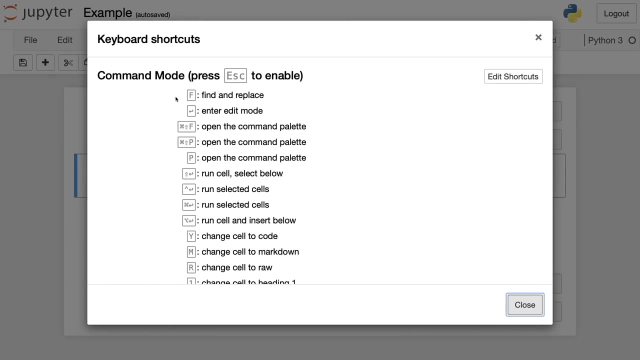 pressing the letter H. So I press H And here you can see more keyboard shortcuts. Or you can also go here to help and then go to keyboard shortcuts here And you get the same window. So here you can see a list of shortcuts for command mode And also. 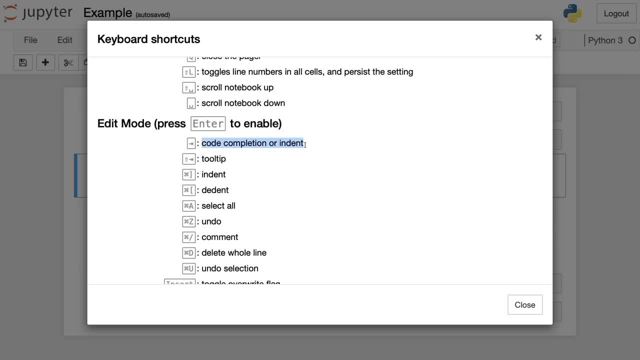 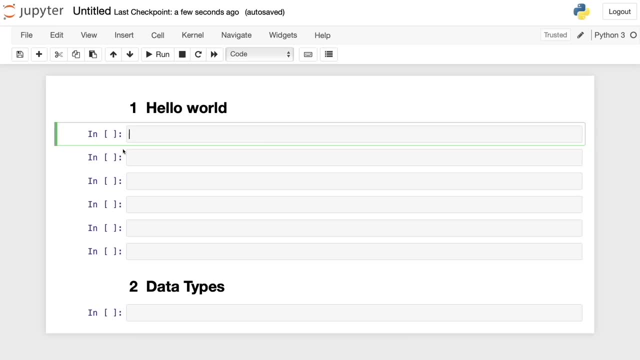 for the Edit mode. you can see the description of a shortcut and also how to do it in your operating system. One of the typical ways to get started with a programming language like Python is printing a simple message. You can write any message you want. 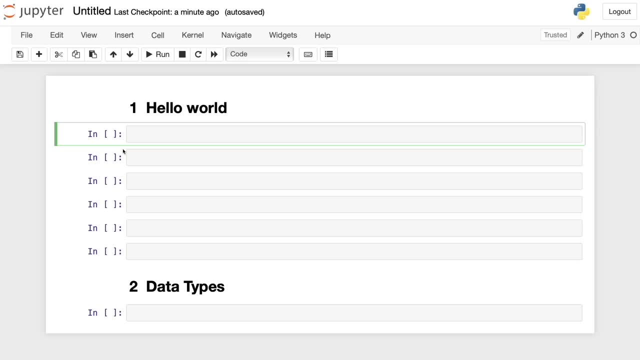 But it's traditional among coders to start with a hello world. So let's try it. Let's print our first message using the print function. The print function prints a message to the screen, So I'm going to write here, print, And then I'm going to open parentheses Every time. 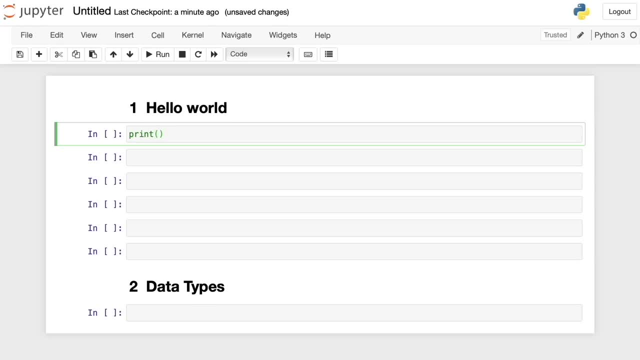 we use a function in Python, we have to open parentheses- well, in this case for the print function, And, as you can see here, the functions get a green color in Jupyter notebook, So that's not a big deal. Right now, I have to write a message, and the first one is going to be: 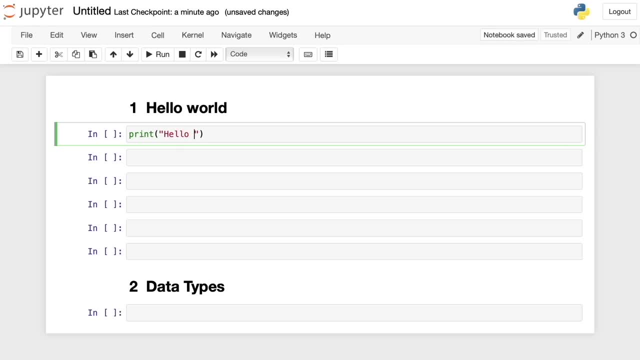 a message of workout. So I'm going to write a message like this, And then I'm going to select the message and in this case, I'm going to specify it. So, inside these parentheses, I'm going to write the message. So in this case, it's going to be: hello world. So this is our. 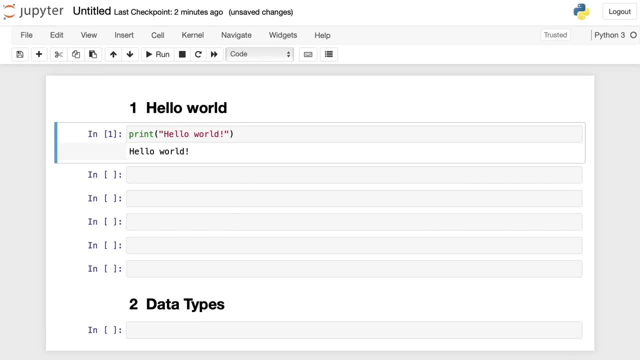 first message. Now, to execute this first line of code, we have to press control and enter, or command and enter. if you're a Mac, So way to run this first cell is pressing here on the Run button. it's going to have the same effect. So 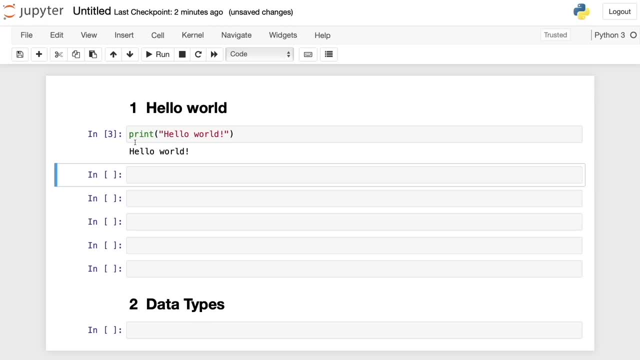 I pressed and it ran. So, as you can see here, it says: in which represents a code cell, And this is a markdown cell. as we've seen before, one of the advantages that Jupyter Notebook has is that it allows us to print the last object in a code cell without specifying the print function. So for 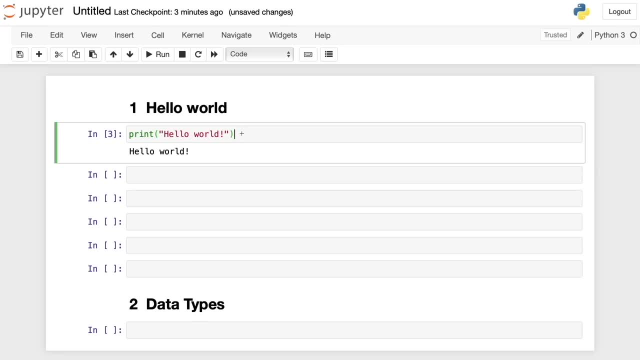 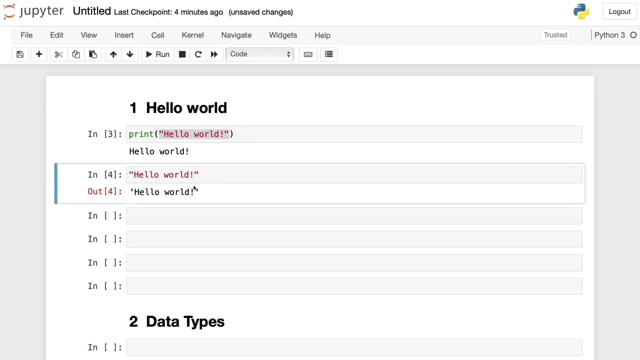 example, here I can print this Hello world with without writing this print function. So I'm going to copy this Hello world message that it's inside quotes, And I'm going to run this code. So just Ctrl Enter And, as you can see, here we have this message printed. So this one of the advantages. 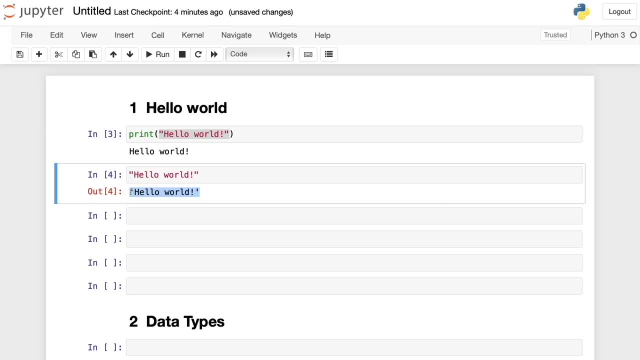 that have Jupyter Notebook has is that it allows us to print the last object in a code cell without specifying the print function. So, for example, here I can print this Hello world without writing this as Jupyter Notebook. If you do this in another Python ID it won't work. So here you can try. 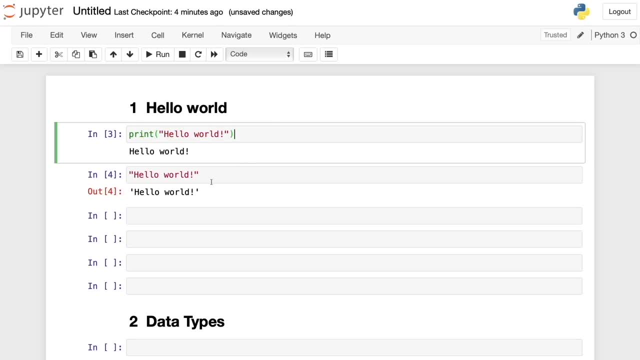 yourself. you can write any message you want, Apart from the first Hello world. you can try with your name. So we write print, then parentheses and we open quotes because we need to define a string. I'm going to tell you about strings a little bit later, But 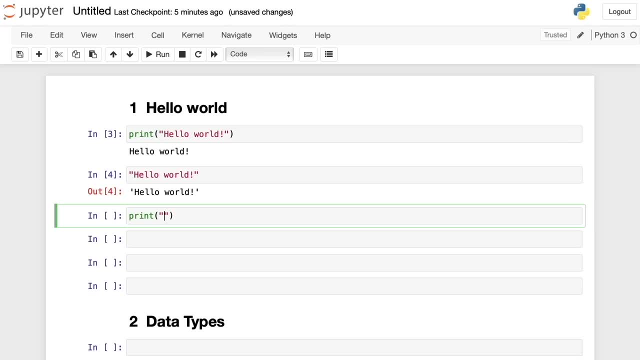 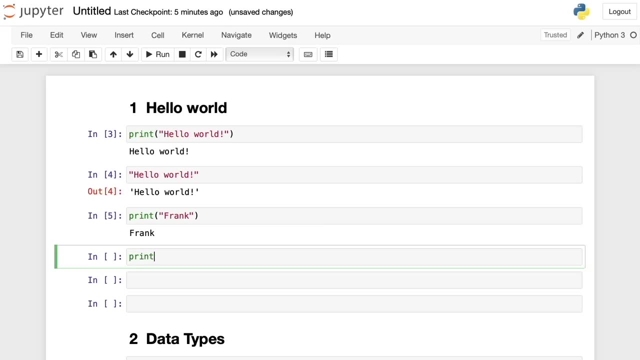 yes, so you know, right now and here, for example, I can write my name, so my name is Frank and I can print my name. then I can print also numbers, So I print my age 26.. And it's going to work too. And besides writing code, you can also add comments. Comments are a useful 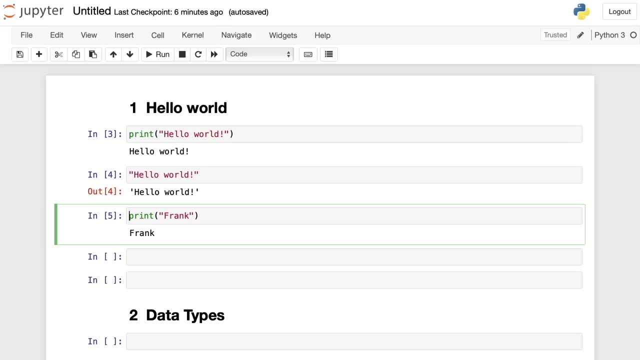 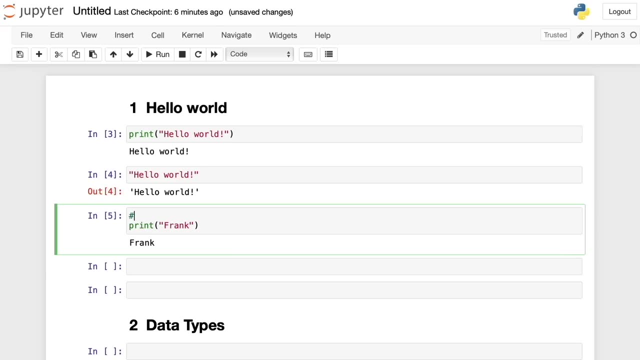 way to describe what we're doing in our code. So here we can use comments. we just have to write the hash sign, which is this one. So you write hash sign and then you write the comment. in this case, I'm going to write my name And I'm going to say printing my name. So we know what. 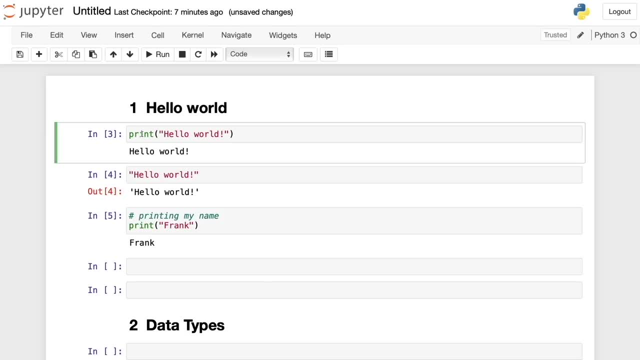 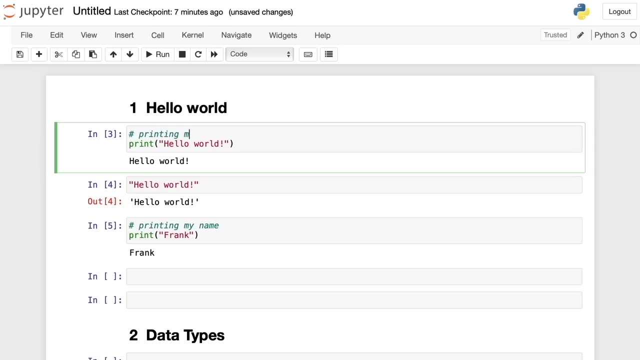 our code is doing here. in the first message we wrote we can also add the comment. So we write hash sign and then we can save printing my first message. As you can see, here the comments also have a different color, So So far we have three colors. this color for the comments, green color. 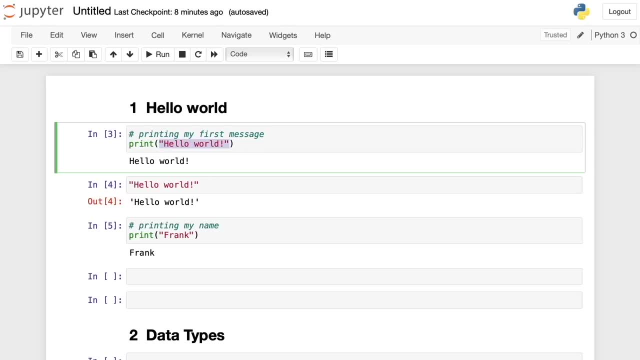 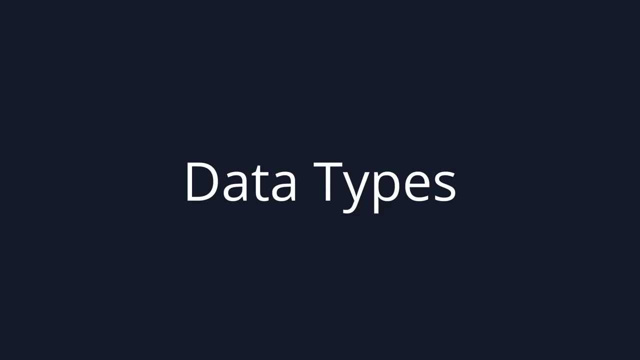 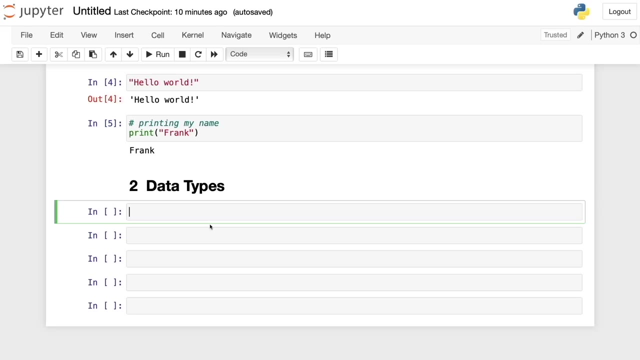 for the functions and red color for the string. this is just a useful functionality most text editor have that allows us easily read code. Okay, now let's see some data types in Python. every value in Python is an object and object has different data types. Let's see the most. 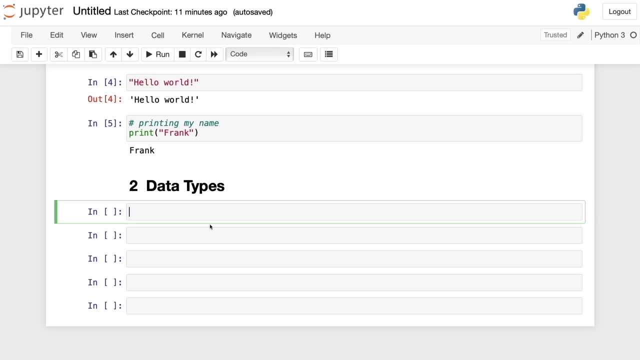 common data types in Python, So one of the most common that the types in Python are integer and floats. Both are numbers, but integers are numbers that can be written without a fractional component, just like, for example, the number one, number two, three, four, five. 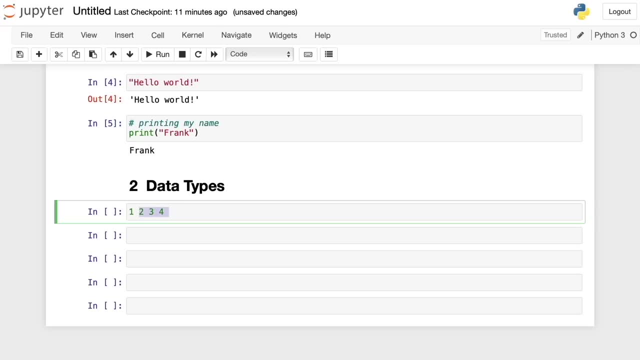 and so on. So all of them are integers And we can check this value or this data type by using the type function. So this is our second function we're going to see. so we write type, then parentheses, and we execute. we run this code And, as you can see here in the output, it says: 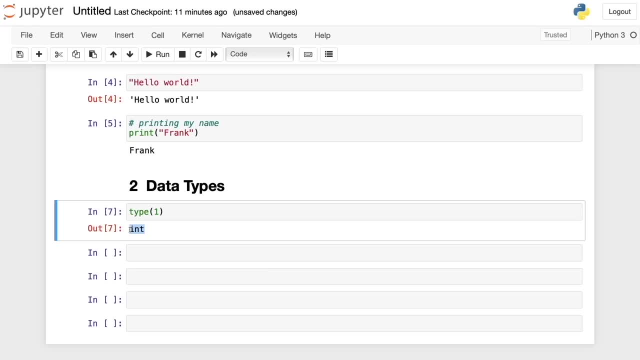 I n t, which represents integer. So this is an integer, Okay. the second type of data I want to show you is float. Floats are numbers that contain floating decimal points. So basically 2.3, let's say 1.2.. 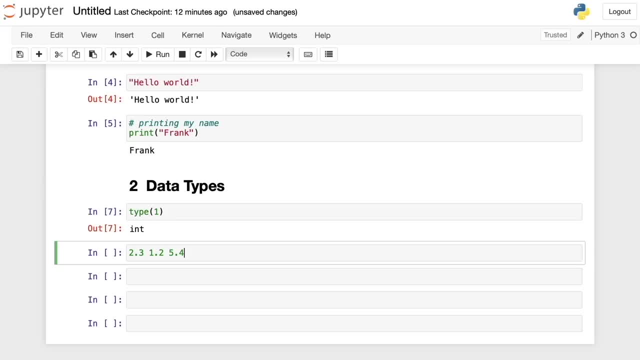 5.4, and so on. So here we have another type of data And let's check out if these are actually floats. So we use type and then parentheses and we run this code And we see that we have float. 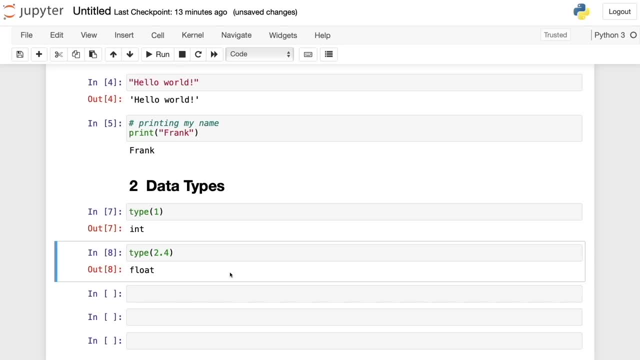 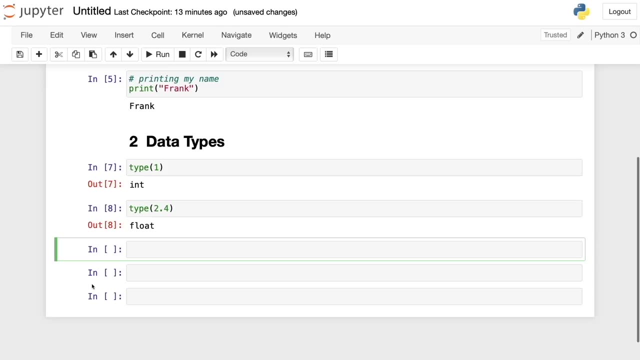 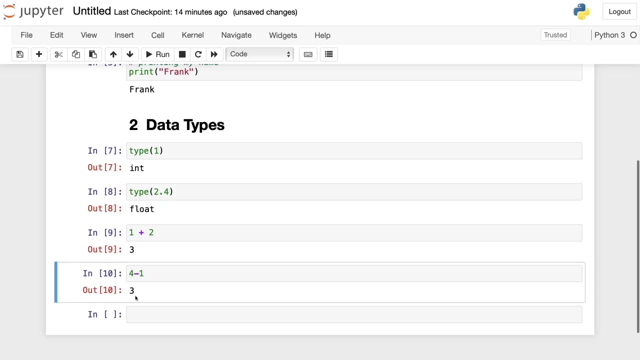 And, just like on Excel, you can perform math operations in Python using these numbers. So some operations you can use are addition. for example, you can say one plus two and then execute this code and you get three. you can use subtraction, So four minus one, execute and you run this code and you get three. 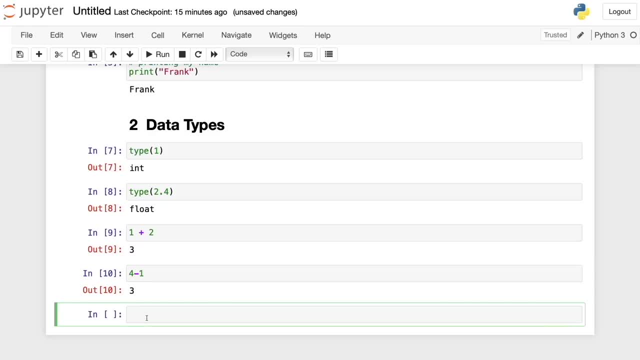 you can also do multiplication, division, exponent and more in Python. But now let's see the third data type that we will see often on Python And it's the Boolean. Boolean are true or false values And we can check this using again the type function And we write type and within parentheses. 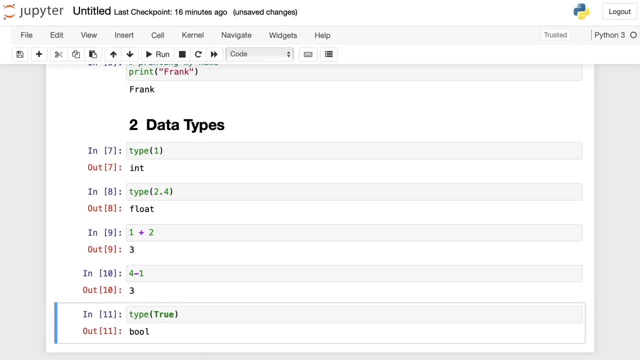 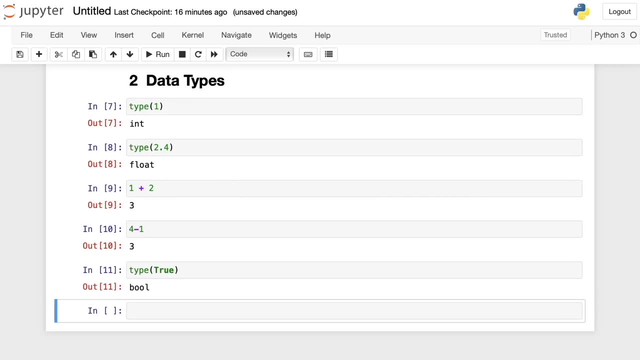 we write, for example, true, And we run this code and we see that we got that bull, which represent a Boolean data type. So we can also write type and in this case false, and run this code and we get bull again. So this is Boolean And we're going to use Boolean often. 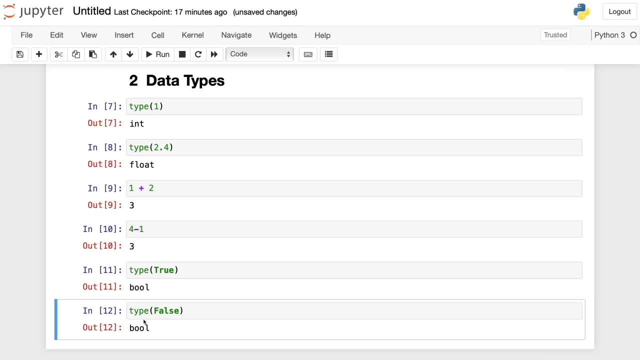 when we use conditionals. Okay, now the fourth data type I want to show you- and it's very common- is the string. A string represents a series of characters And in Python, anything inside quotes- either single quotes or double quotes- is a string. So let's see them. Actually, we already 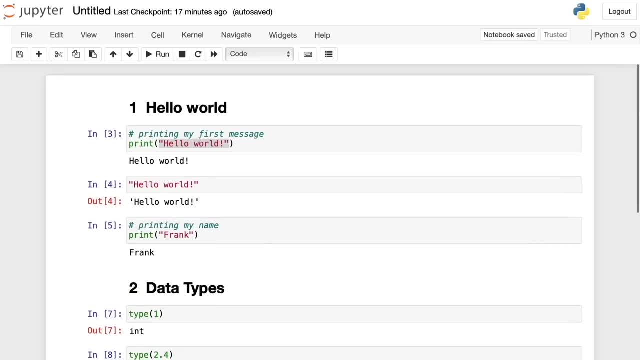 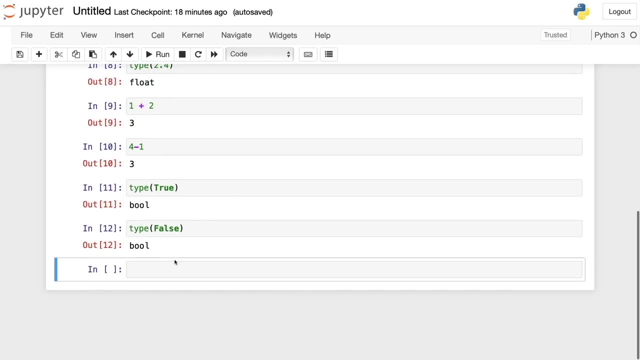 see one kind of string here. when we printed this hello world- And you're actually going to be familiar with this, but we're going to see it again- So to create a string we have to open either a single or double quotes. So in this case I'm going to use double quotes. So you see it now. 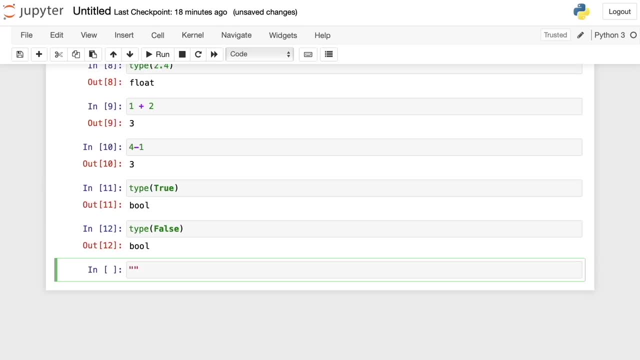 And now I'm going to write any message, So I'm going to write, for example, again: hello world. And again to verify the type, we can use the type function parentheses. run this code and we got that str. So we're going to use the type function parentheses: run this code and we got that str. 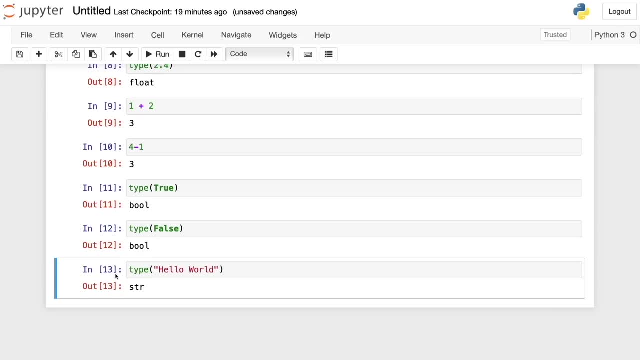 that represents a string, And one cool thing a string has is methods. we can apply different functions to strings, as we will do in Microsoft Excel, for example. However, in Python we use methods. a method is a function that belongs to an object. To call a method, we use the dot sign. 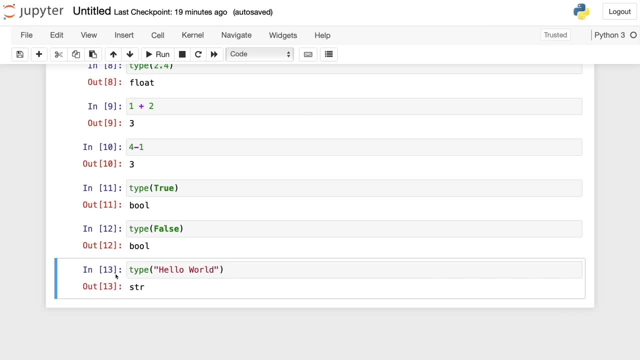 after the object, let's see some string methods to change the case of the text. So here I'm going to write again hello world. But now I'm going to use some string methods So I write Hello world. in this case I'm going to use the upper method to make this uppercase. So I'm going to use the print. 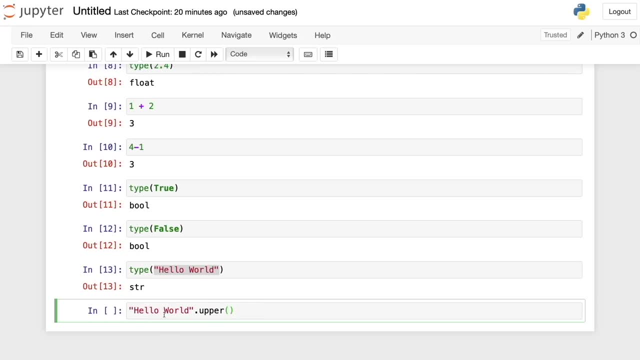 function. But actually we don't need to use the print function because, as I told you before in Jupyter notebook, we don't need to use the print because it automatically prints the last line of code. So, since this is that, 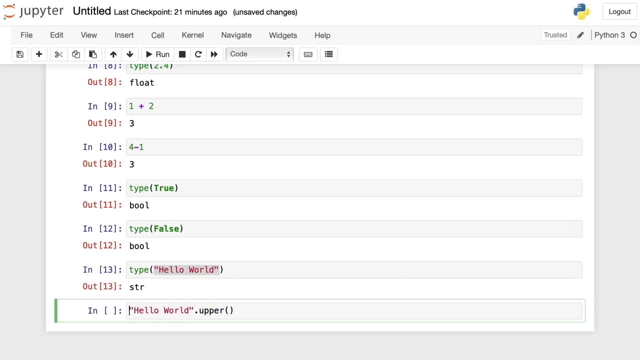 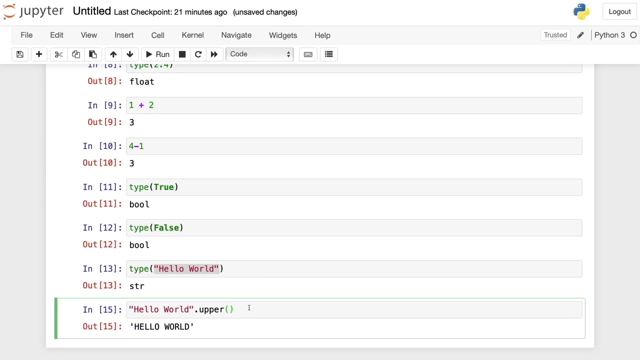 only line of code in this cell block. it's gonna print it automatically. So we just run this cell and we have Hello world in upper case. So, as you might expect, now we can also change the case of the text. In this case it can be a lower case or title case. So I'm gonna just copy and paste this. 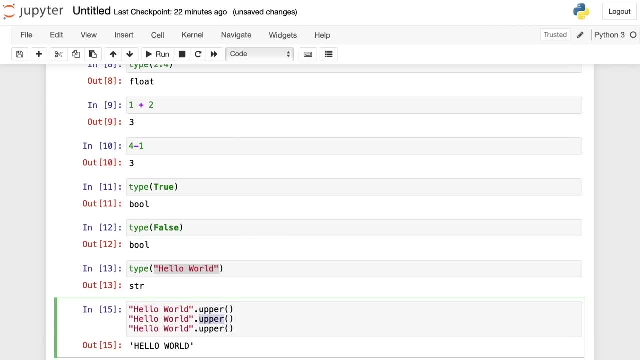 twice. And here I'm going to write: instead of upper, I'm going to use flower and then title, So you can see how it's going to change the case. So here I'm going to run and let's see what happens. 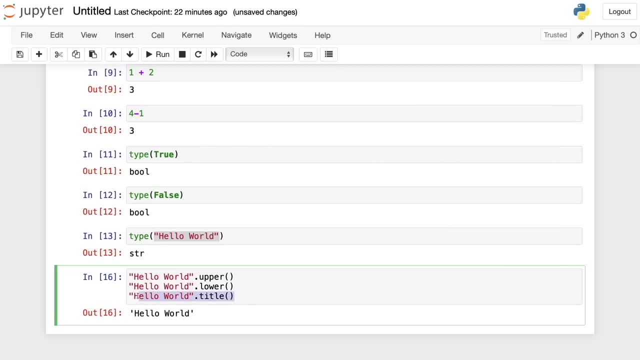 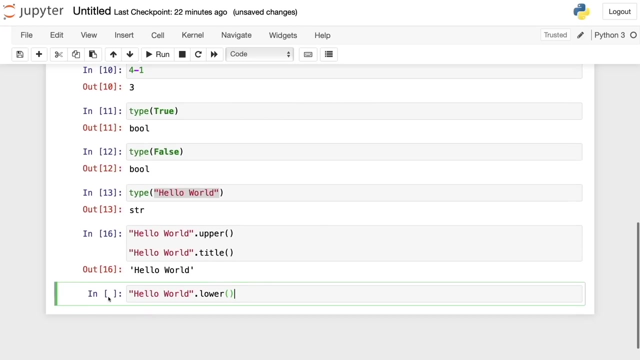 So, as you can see here, it only printed the last one, because I told you before it only prints the last one. And if we want to print the three of them, we have two options. So we can maybe here cut and paste on each cell, Or what we can do is to print each of them. So here for example, 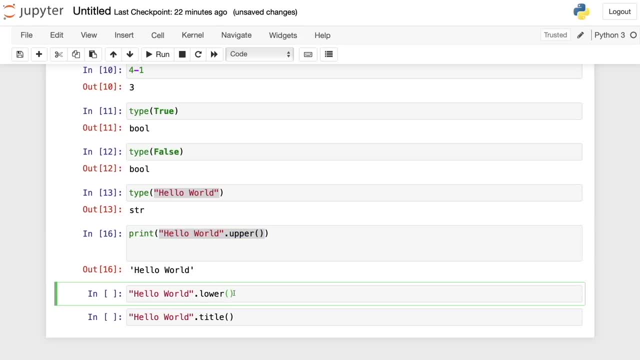 I can do print here and I can do the same for them. So instead of using more cells, we can print all of them, And here we can print this one too. actually, we don't need that. we don't need it. 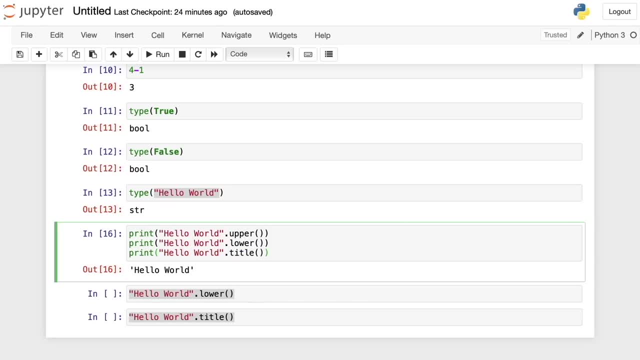 because gonna print the last line, But just for the sake of this video, I'm going to print the three of them. So here I'm going to run this code And, as you can see here, the first, it has an uppercase, the second has lowercase and the third has a title case. So that's. 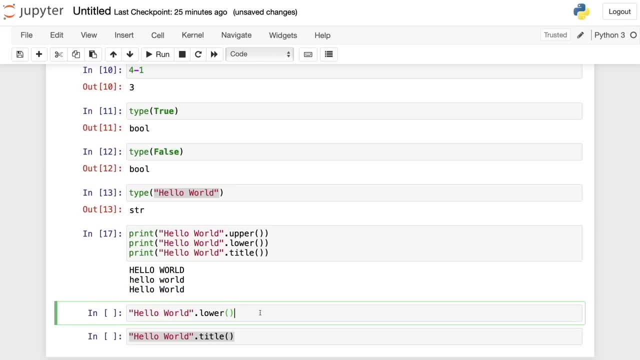 how you do it on Python. Other string method that you can find, Python is the count method. So I'm going to delete this and actually this one too, And we're going to see this now. So first I copy this And now I paste it here, And here I'm going to use the count. 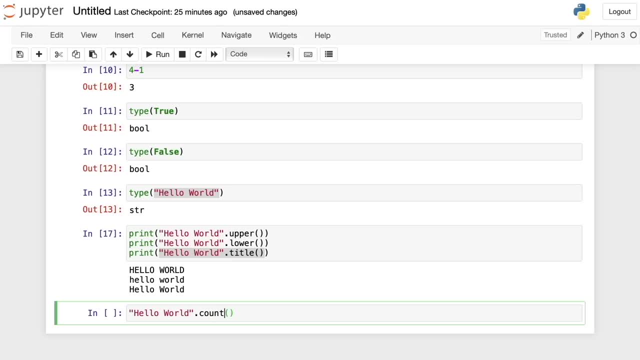 So the count method, so I write count And then here I open single quotes and I write the letter that we want to count. So here, for example, I'm going to write the L letter And what this string method is going to do is going to count how many times this L letter. 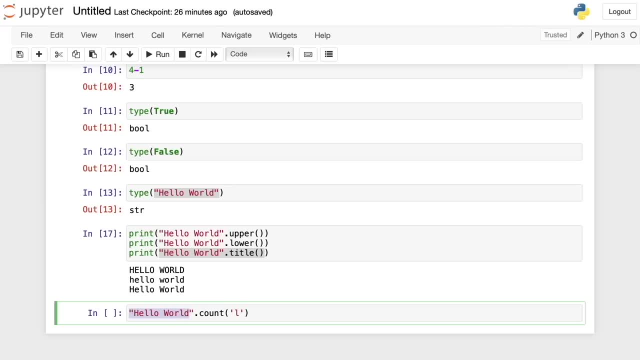 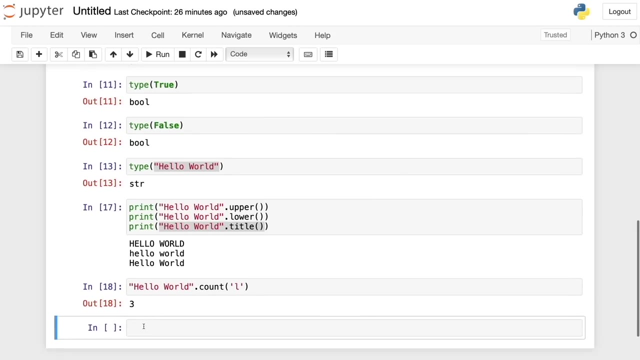 is included in this string. So, as we can see, there are two else, so it should set two times. So I run this code And actually is three, because there are two in Hello and one in world. so I was wrong And here Another string method that you can use is the replace method. 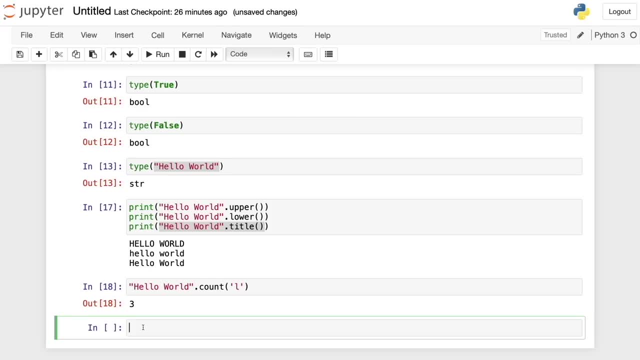 method So we can replace one letter for another. So here, let me copy this And I'm going to paste it here, And instead of writing count, I can write replaced. So here, the first letter that we're going to see here is the letter that we want to replace. So in this case, I'm going to change the 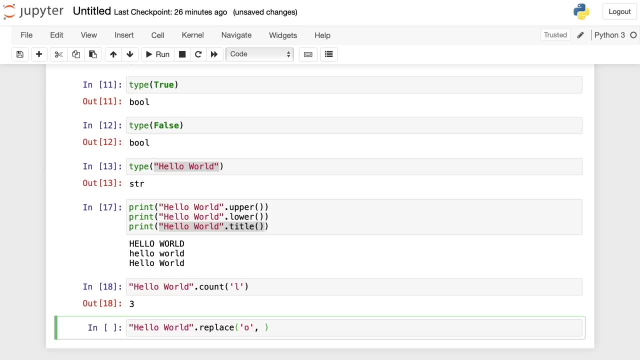 L with O, And the second letter is the letter that you want to put in that string. So I'm going to use the U, So I'm going to change every time that an O appears here in the string. we're going to replace it for a U vowel. So let's try. So I run this code And now it says: well, hello world. 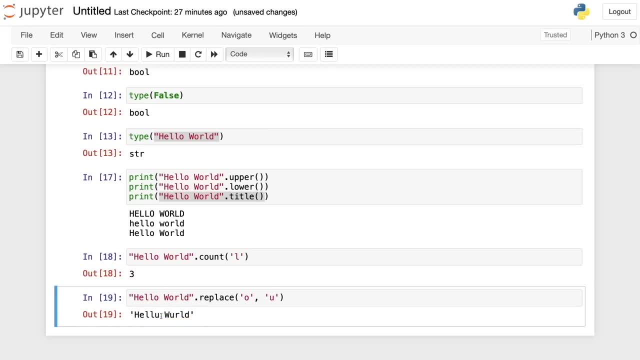 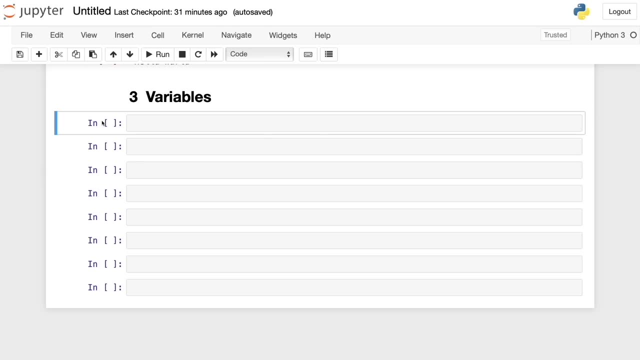 but with you, And these are some of the most important things that we're going to see here: common string methods in Python. Okay, now it's time to learn something that you're going to see often in Python, which are variables. variables help us store data values. In Python, we often 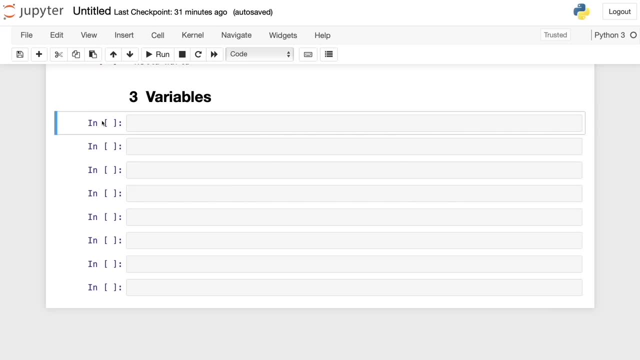 work with data, So variables are useful to manage this data properly. A variable contains a value, which is the information associated with a variable. To assign a value to a variable, we need to have a value of the value of the variable, So we need to have a value of. 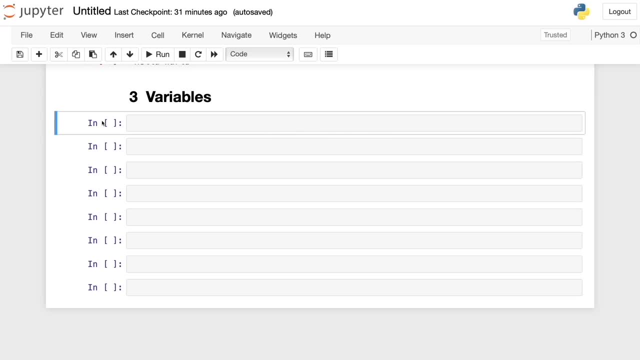 we use that equal sign. So let's create a message that says I'm learning Python and store it in a variable called message underscore one. So here I write message underscore one and we set it to that string I'm learning Python. So I open double quotes in here I write: I'm learning Python. So 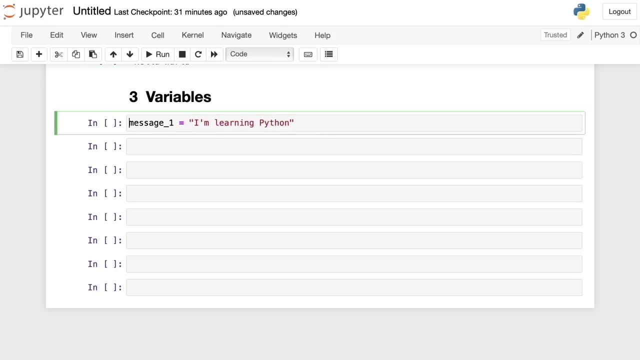 this is string- we've seen this before- And this is the variable, And we assign this value to the variable using that equal sign. Now I'm going to run this And, as you can see, nothing happens. But actually we just assigned that string to the variable message underscore one. Now, if we want, 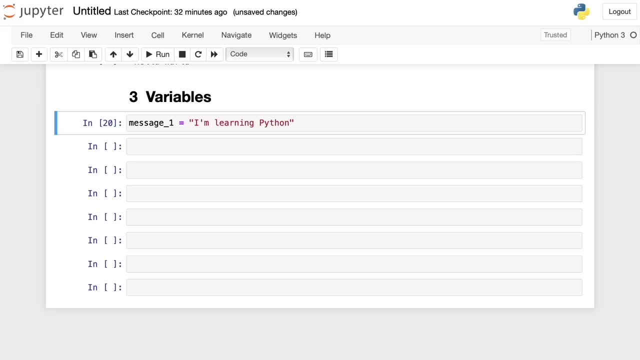 to obtain the message. I'm learning Python. we only have to type the variable name and then execute that code. So I'm going to copy and paste it here And then we run this code And, as you can see, by running this, 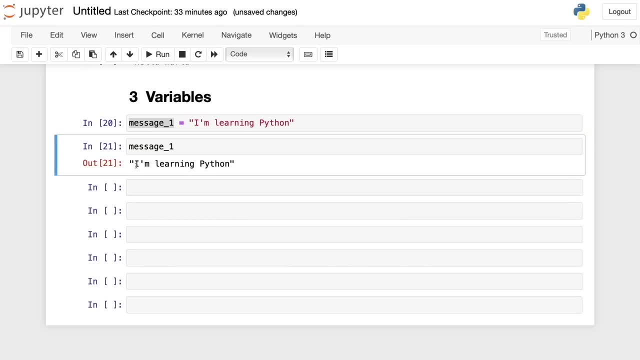 cell we obtain the content inside the variable message underscore one. we can create as many variables as we want, Just make sure to sign different names to new variables. So let's create a new message that says: and it's fun and store it in a variable called message underscore two. So 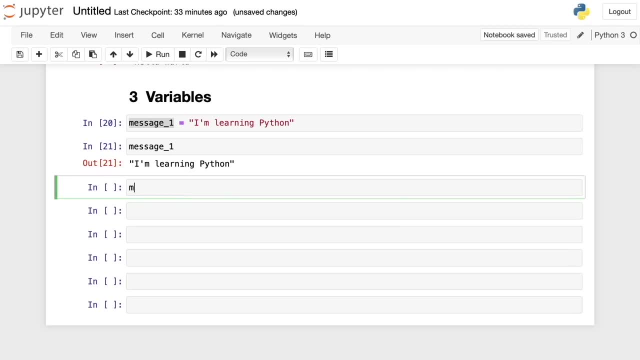 first I write message, So message, And I'm going to use this variable right and place and type this option And if you are using Dragon R, you can use this variable as a default and it's fun and protected. But I'm going to create a. 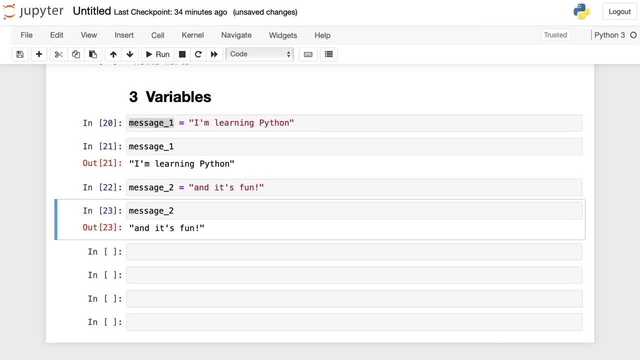 message that says now leaChate say add decoratibV robot word underscore two, And then we set these using single quotes instead of double quotes, as I'm using in this video. probably you had the following issue, So here I'm going to copy this one and paste it here So you can. 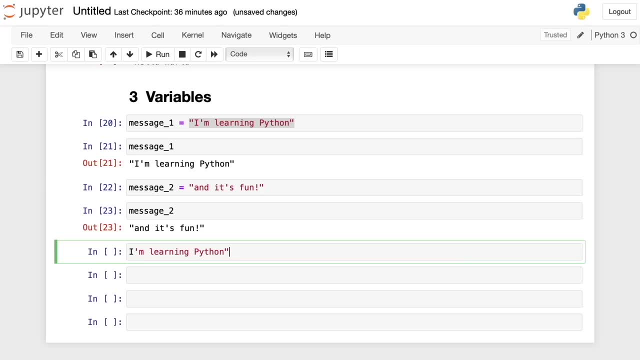 see what I'm talking about. So let's see your. let's say, you're using single quotes instead of double quotes. So you get this. this is a problem that you will have when using single quotes, because in the English language we use these apostrophes often. So a simple way. 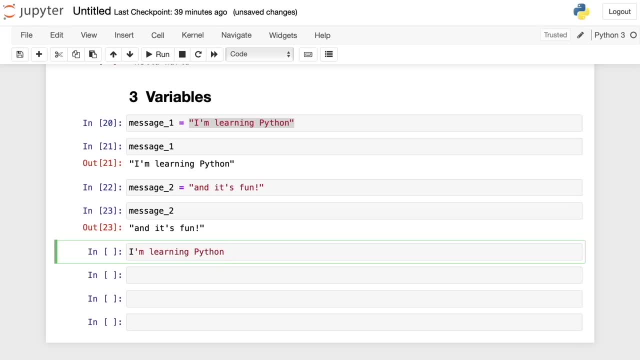 to deal with this is using double quotes. So, as you can see here, if I use double quotes, everything is okay, everything remains as a string. but with single quotes it doesn't happen. So only the- I gets this string, but the rest- it doesn't get a string value, or? 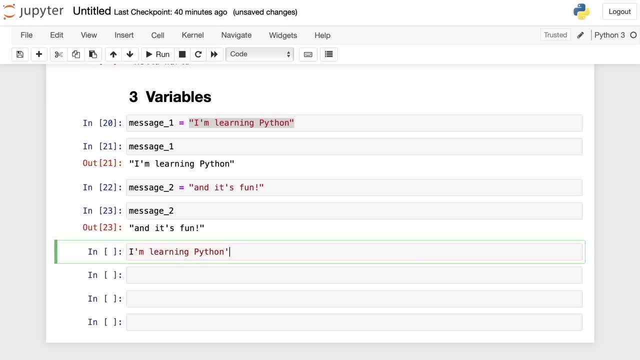 the string data type, So you use double quotes every time you have these apostrophes, and that's it. Okay, now let's put these two messages together, So message one with message two. I want to put them together. So this is called a string concatenation, If we want to put message one. 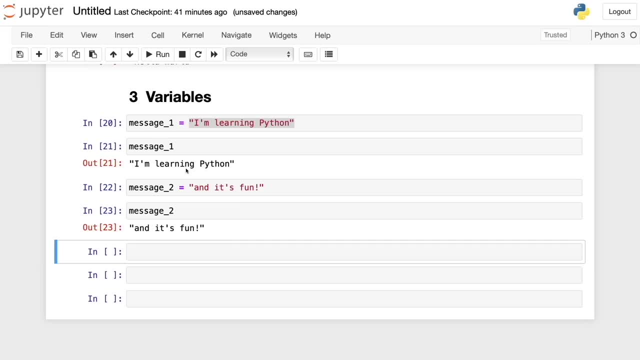 in message two together. we can use the plus operator And we can just do this. So I'm going to copy a message One or the variable message one, And now I'm going to copy the variable message underscore two, And I use the plus in the middle to concatenate this first message with this second message. 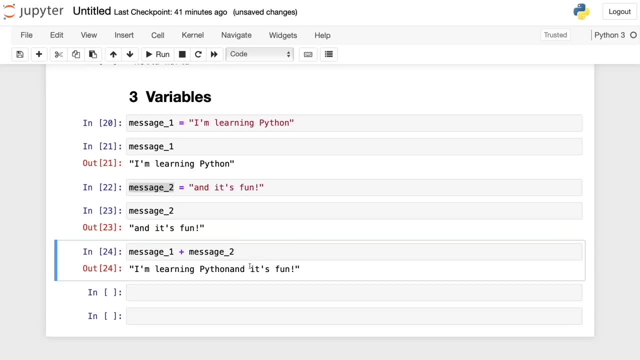 So I run in, let's see what happens. So here we can see that the two messages were concatenated, But here there is enough space between these two messages. So this is the first message and this is the second, And there isn't any blank space in the middle. So what we can. 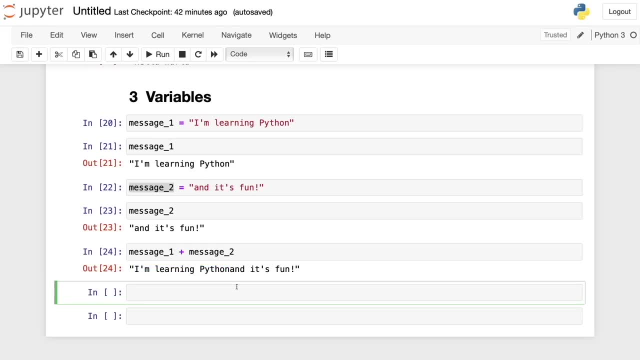 do here is to use add blank space. So I'm going to copy this one and paste it here and show you how to do it. So here I add a new plus operator. in the middle we open a string. So with single quotes or double quotes, in this case I'm going to use single quotes. 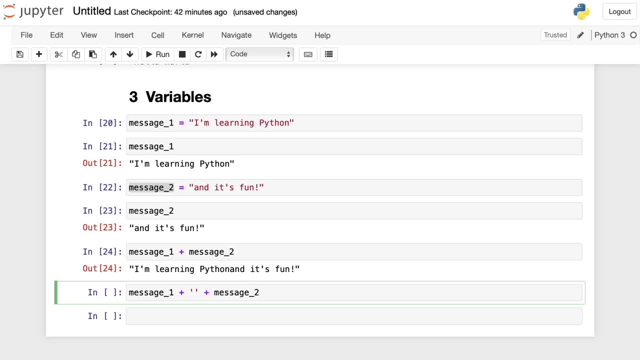 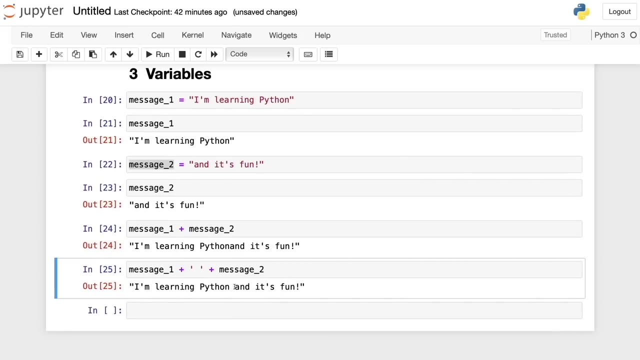 here. So I'm going to activate this blank space, I'm going to press space, And here we have our blank space here, And then we run this code And now let's see, And here, as we can see, there is a space between Python and and we have this blank space And we want. 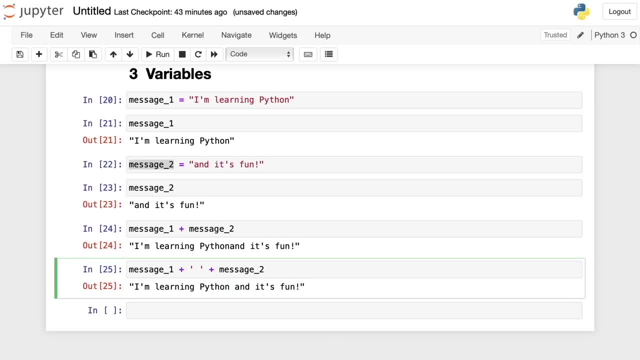 we can assign this new message to a new variable. So I'm going to assign this to a variable called message And I write message here And I include here below the code In here I can print this So, as you can see, if I 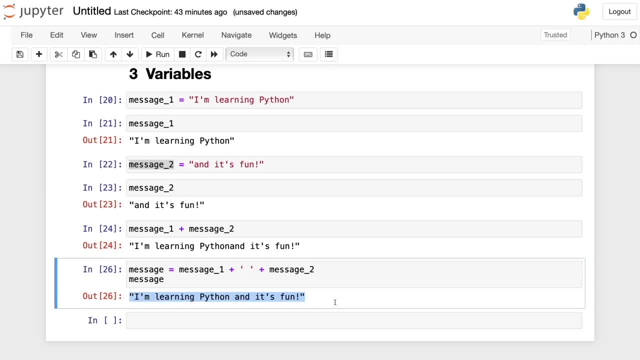 run this, we can see that the message is there. Okay, now let me show you an alternative way to join two strings. So this is called the F string And it works like this: you write F and you open a string. So we write a single quotes here. So one and two. 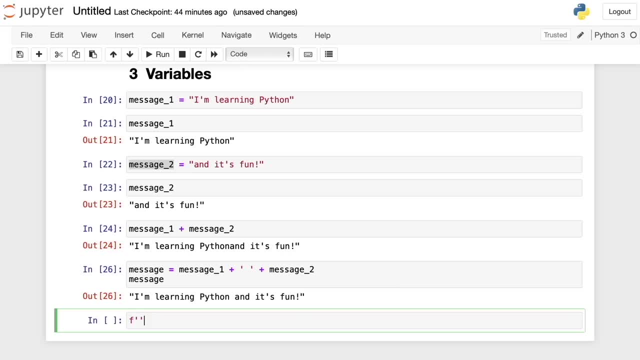 And in here, as you can see, the whole, the whole thing is red, So it's like everything is a string In here, inside we can write the message. So let's see, let's say we write the, not a simple Hello world, So hello world, And we run this And, as you can see here, 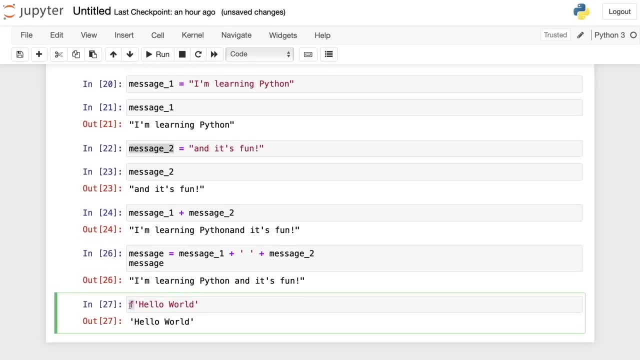 this is a string. it just has this F in front of that string. And here one of the advanced advantages that this F string has is that it can have variables inside string. So here, for example, we can write a variable opening these curly braces, So this curly braces can. 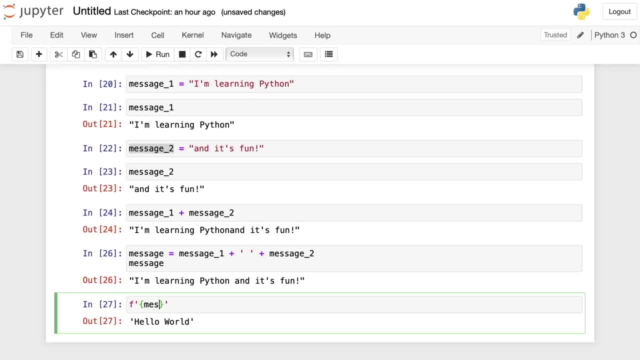 have variables inside it. So here I can write message, underscore one and we can print it. So if we print, we have this string. I'm learning Python. And now, if we want to concatenate this first message with our second message, 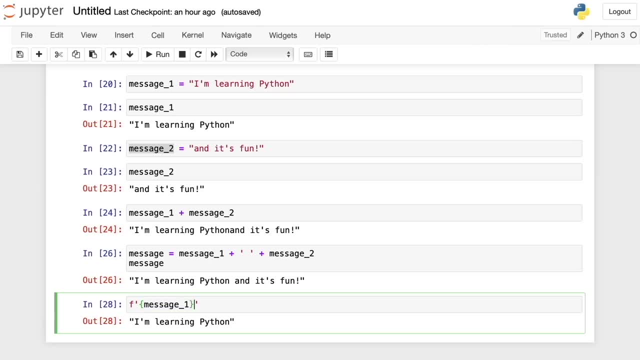 we just have to include curly braces. Again, I put it here, And now I write message two, And between message one and message two I just have to press space And we have this. So I'm learning Python and it's fun. So here we just press space and the space also appears. 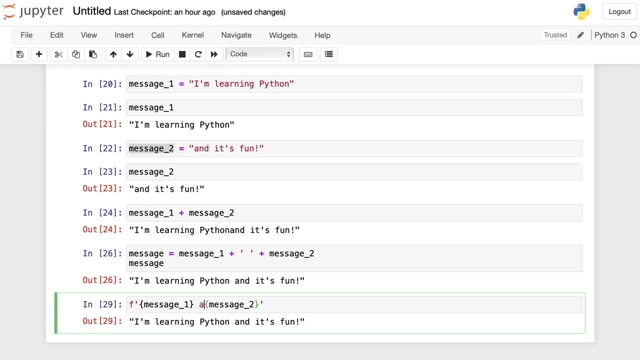 here. So, for example, if we add some random text, let's say ABC, we get this ABC between Python in between, And so this is how F string works. you just have to write the F, then open single quotes And inside. 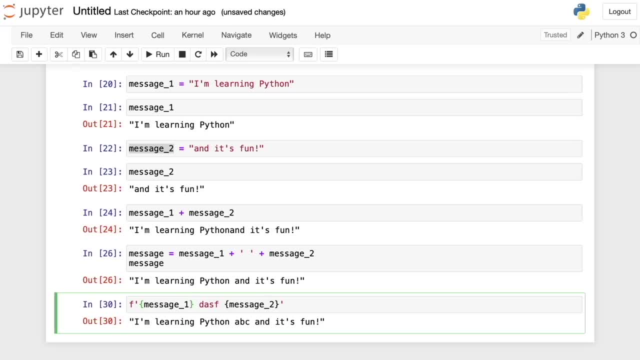 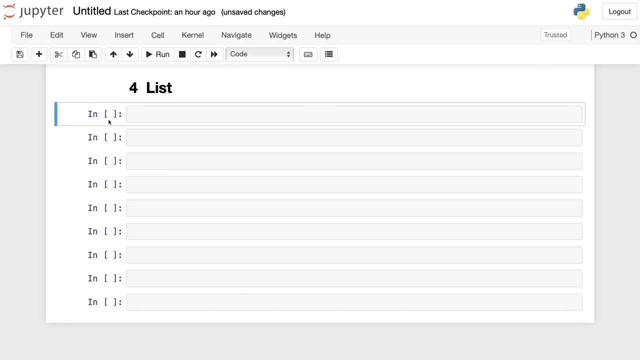 you can write any message And to include any variable, just you have to open these curly braces, write the variable name, And that's how you join strings. Okay, now it's time to see a data type that is used often in data analysis. I'm talking about lists In Python: lists. 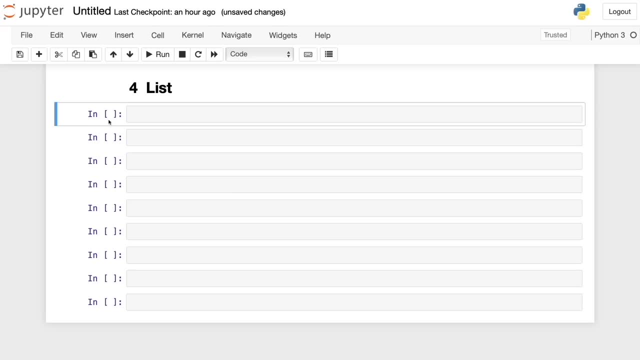 are used to store multiple items in a single variable. Lists are order and mutable containers. In Python we call mutable to objects that can change their values, That is, elements within a list can change their values. To create a list we have to introduce the element. 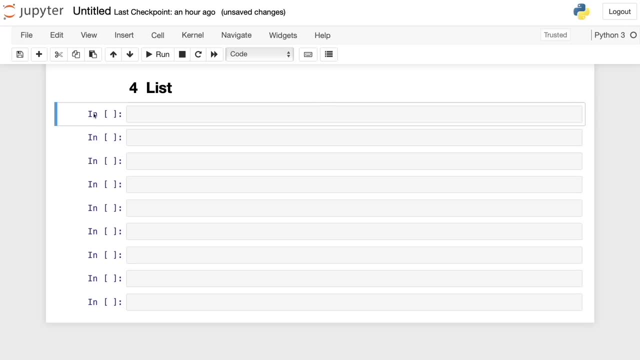 inside square brackets separated by commas. So let's create our first list. First, we have to set the name of the list. In this case, I'm going to name it: countries In. now, to create a list, we have to open square brackets, as I said before. So here we open square. 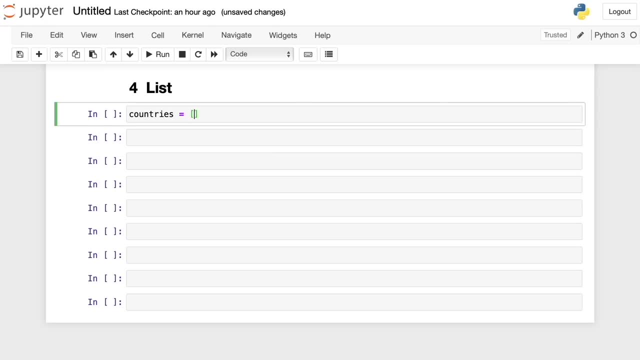 brackets And here we have to write the elements. So I'm going to include in these countries list just strings, and they're going to be names of countries. So the first one I'm going to write United States. So this is the first element in my list. 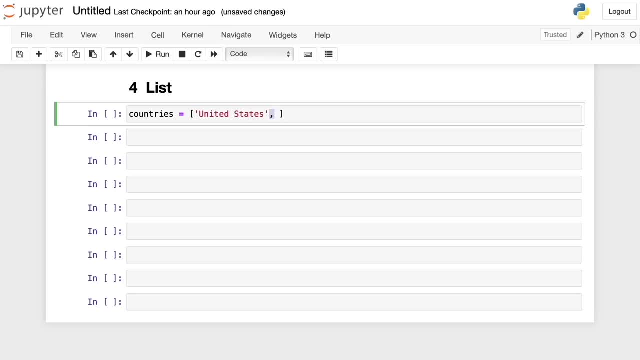 And to write the second we have to use the comma. So here comma, and now the second. So let's write India, two more, So now China and finally Brazil. So these are the four countries, as you can see here, this list. So we have the square brackets that represent the list. 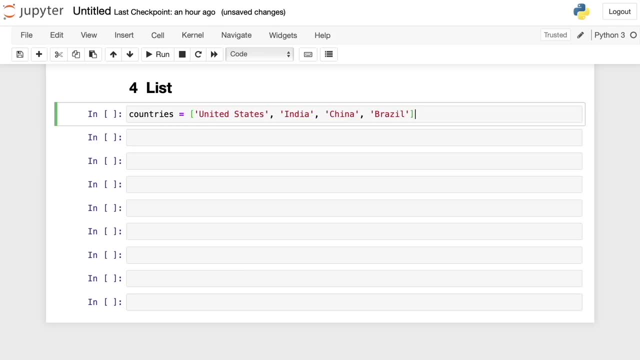 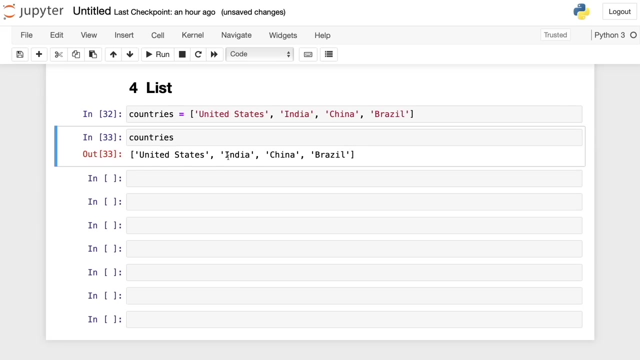 And we have four strings And this is how to define or how you create a list. So now I'm going to run this one And to see that content, I'm going to paste the name of this list And now I run here. I include only strings, But keep in mind that lists can have elements of different types. 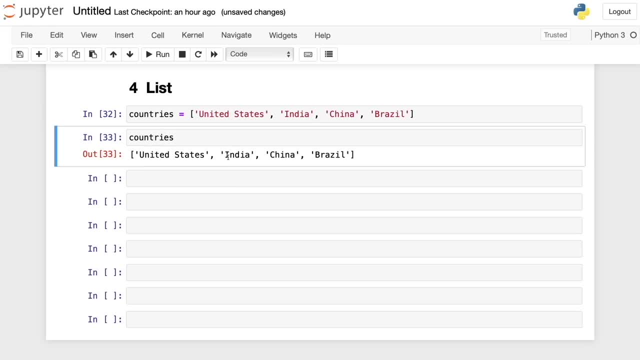 So for example one string and the other an integer and then a float and so on. And also lists can have duplicated elements. So for example I can have here United States written twice. So here for example I can write United States twice, And that's okay because lists can have duplicated. 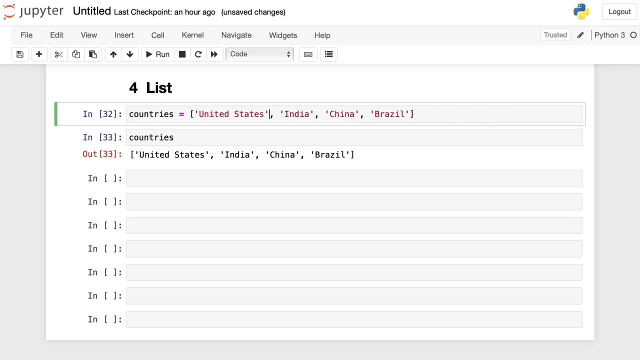 elements, but I don't want it that way, So I'm gonna delete it and leave it as it is. Okay. now, if we want to get an element inside this list, we have to use something called indexing. By indexing, we can obtain an element by its position, So each item in a list has an index. 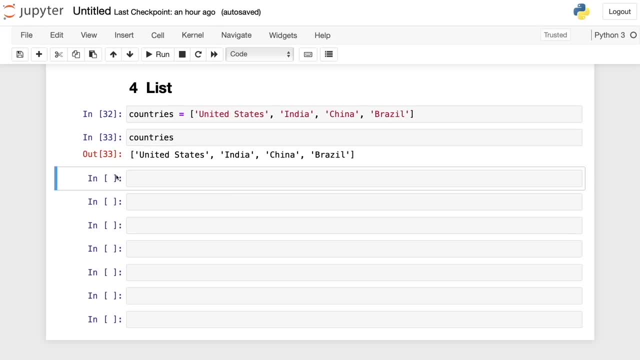 which is the position in the list. Python uses zero base indexing. that is the first element, so United States has an index zero, the second, so India has an index one, And you know one setup. but we're just drawing apples and Minuten and then we move on To access an. 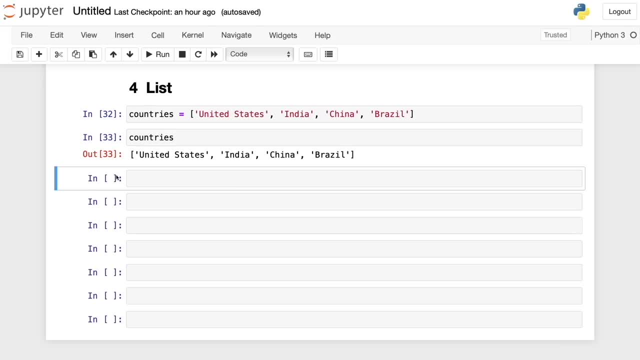 element by its index. we need to use the square brackets again. So let's see some examples. Let's start by getting the first element, so United States. so what we have to do is to write the name of the list, in this case countries, and then open square brackets And inside square. 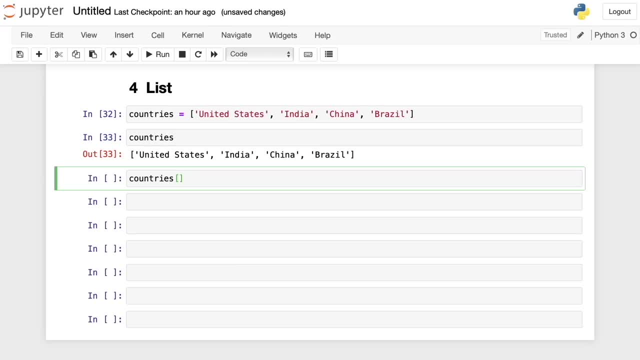 brackets. we have to write that position of this element. So it starts with zero. so we write zero to get that first element. And to get the first element we also have to reach inside of interest element And then we run this code And, as you can see, we got the first element. 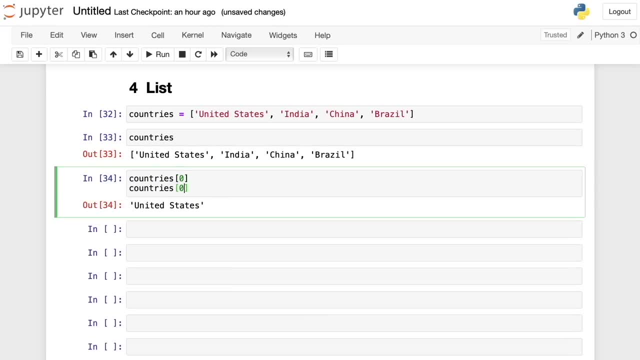 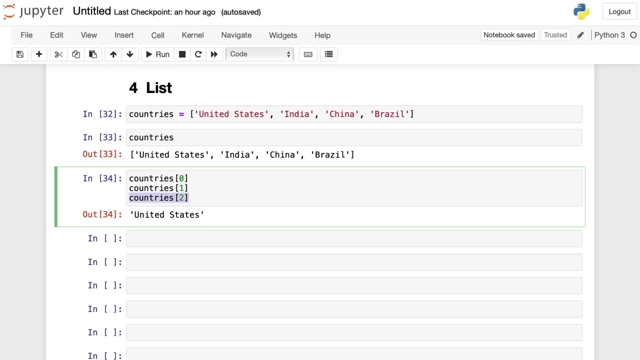 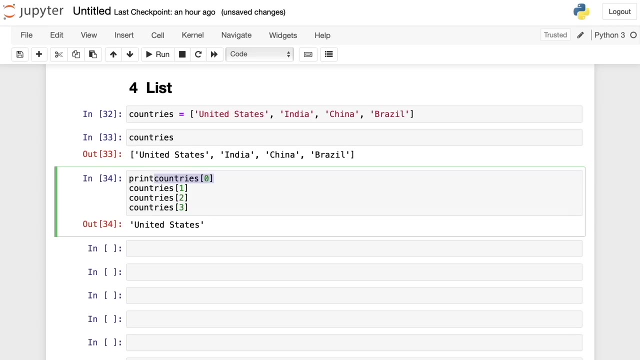 So if we write here countries square brackets one, we get India, And if we write countries square brackets two, we get China, And if we do this with the number three, we get Brazil. So to verify this, I'm going to print each of them, So let's see what happens. So here, 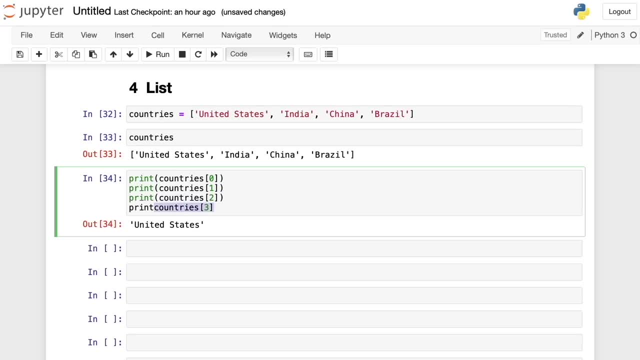 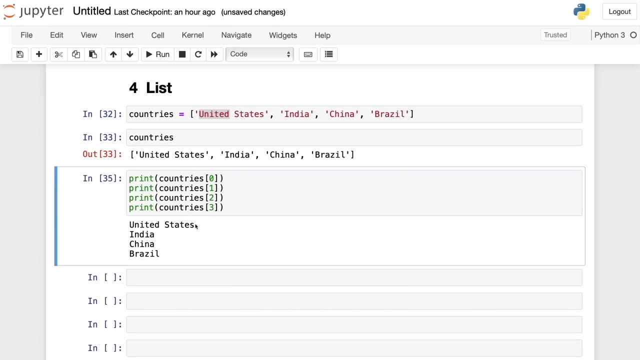 print and finally print this one. And now I'm going to run and we should get each element of the list from United States to Brazil. So let's try out. So here we have each of them: United States the first one, then India, then China and then Brazil. So it's correct. So this is the 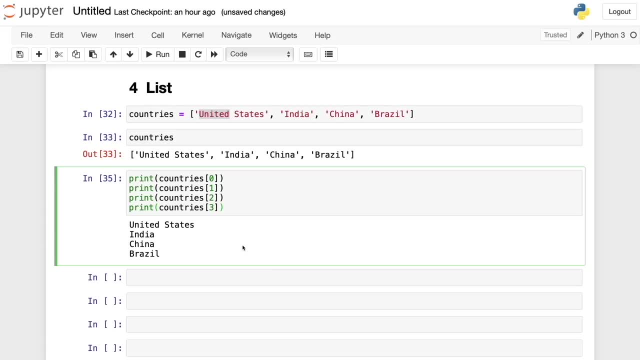 most common way to use indexing, But there is also negative index. This help us get elements is starting on the last position of the list. So instead of using indexes from zero and above, we use indexes from minus one and below. So let's get the last element of the list, But now using 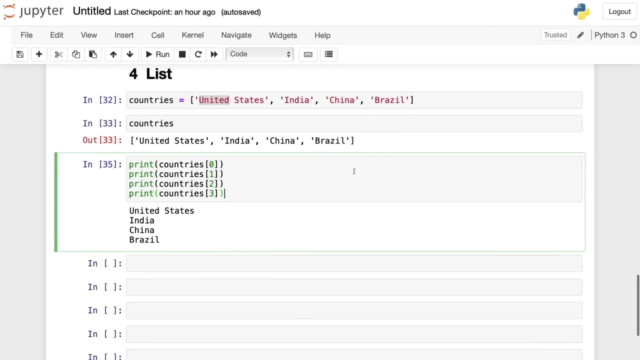 a negative index. So we want to get the last element, which is Brazil, And we did it before with countries, square brackets, three. But now we're going to do it with negative indexing. So here I'm going to write countries, copy and paste it here, And now I open square brackets. 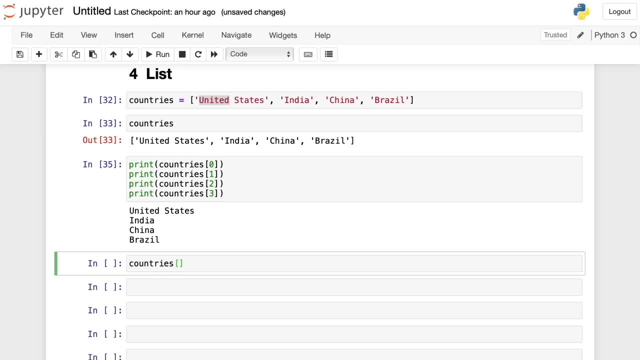 And instead of writing three, we're going to write minus one, And this minus one represents the first element, is starting from the last position. So Brazil will be minus one. China is minus two. India minus three United States. Brazil is minus two. India minus three United States. 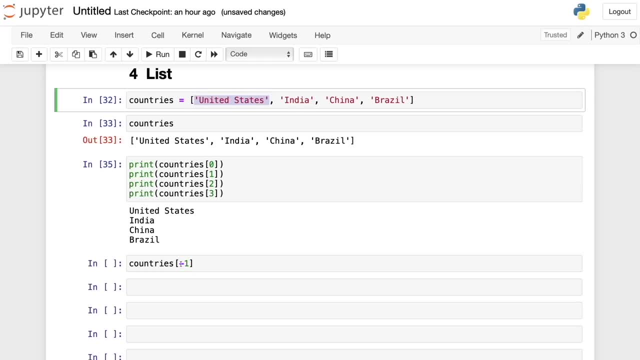 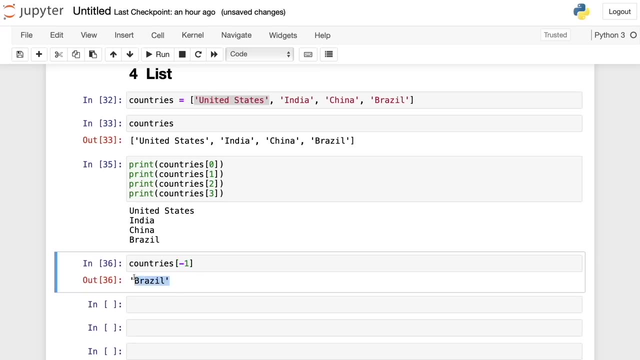 Brazil is minus four, And that's how it works. So I'm going to run this one: countries, square brackets, minus one, and we should get Brazil, and we got it. So let's do this one more time, And in this case I want to get United States, which is minus 123 and four, So its 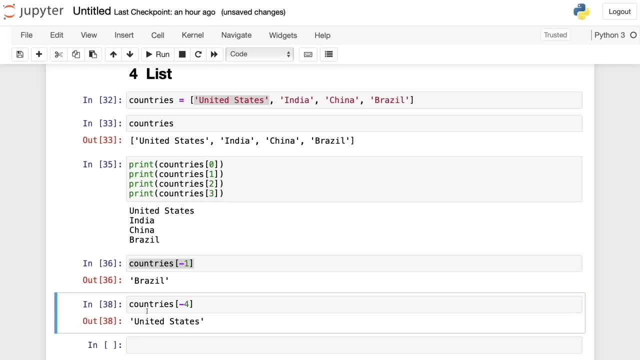 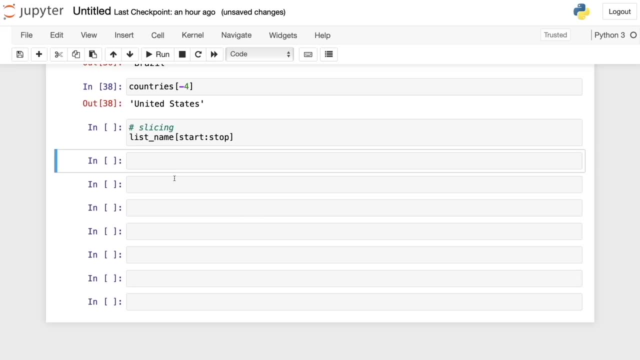 countries minus four. So we run this and we got United States, but now using a negative index. Okay, now let's see something called slicing- accessing parts of a list. A slice is a subset of list elements. A slice notation takes the form of: 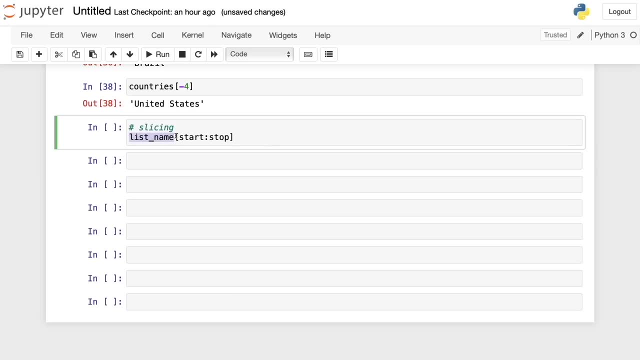 list, So the list name and then a square brackets and the start, then this colon and stop. this is: start represents the index of the first element and stop represents the element to stop at, without including it in that slice. So let's see some examples. So I'm going to use this country's 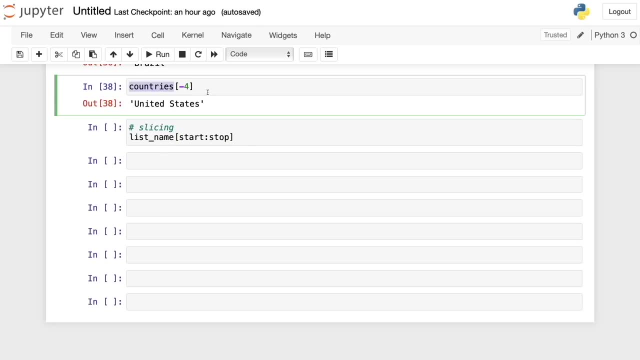 list again I use. I'm going to copy this one and I'm going to paste it here. So this is the name of my list And now I open square brackets And we're going to get, let's say we're going to. 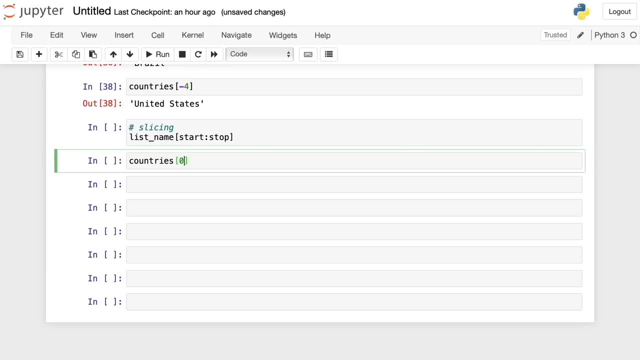 start at position number zero and then colon, And let's get from zero to the position number two, And then we're going to paste it here, And now I open square brackets and we're going to start at position number two. So we have to write three, because it stops at three without 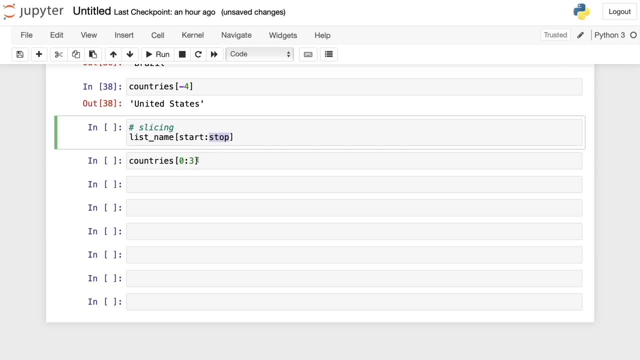 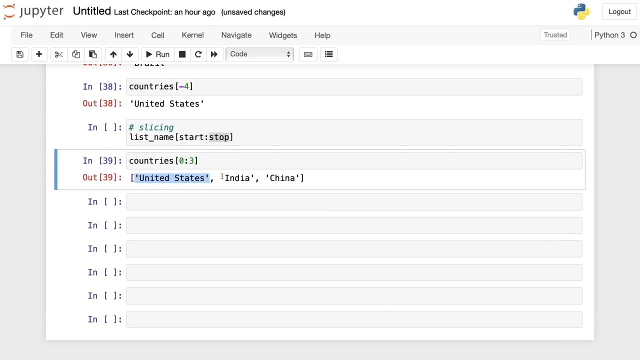 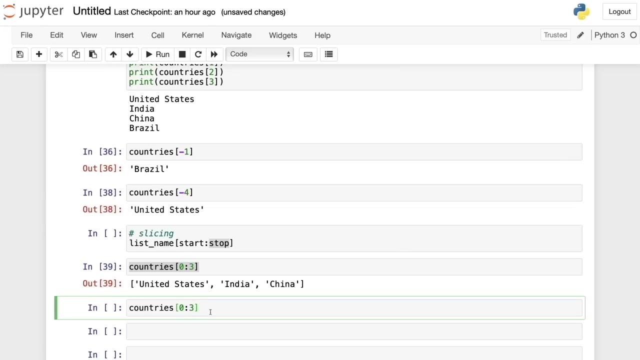 including this element in the position number three. So let's run this one And as you can see, here we have index zero, index one and index two. So it didn't include index number three. And now let's say we want just the first element, So we write from zero to one, So it's only zero. 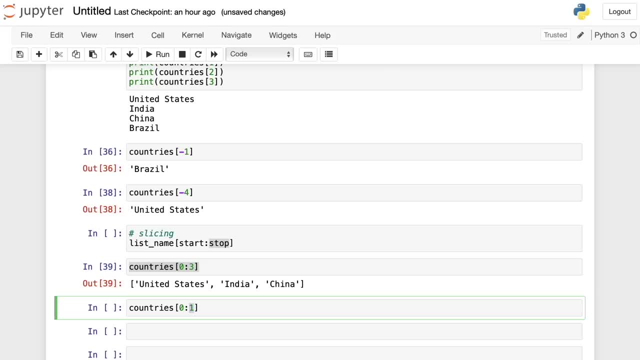 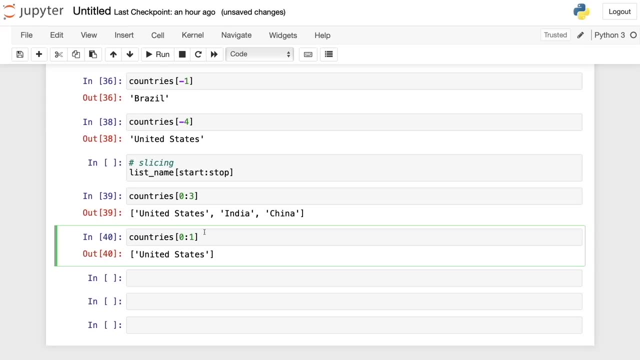 and one No, because it doesn't include one and it stops at one. So here I run and we got only United States. So now let's try something different. Let's say we want to get elements from index one to the last. 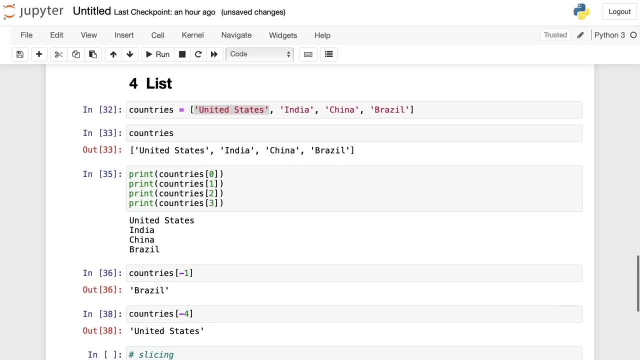 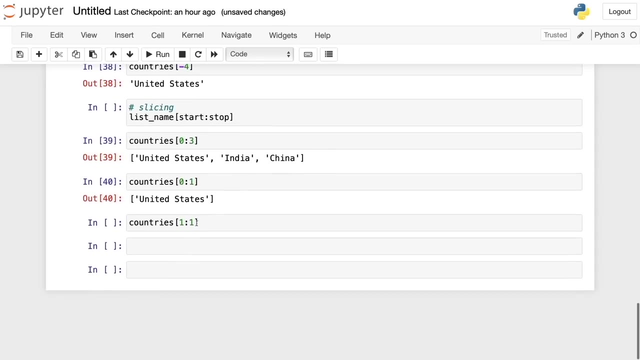 one. So let's say: let me see here, we want to get from India to Brazil, So it's one, two and three. So we have to write four because it stops at four and we got three. So let's write here one, two, four, And we should. 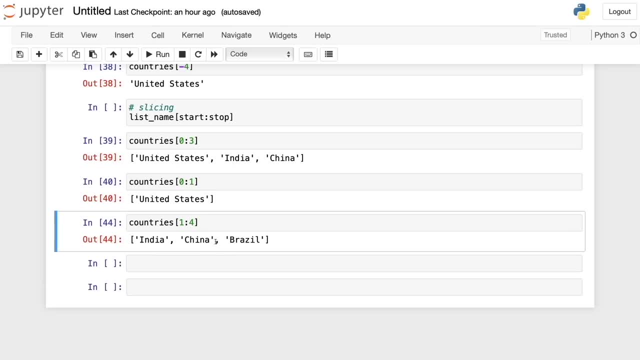 get: Yeah, India, China and Brazil. So this is one way to do it, But another way to do it is just delete this and leave it as it is, and then run the code And, as we can see, we got the same. 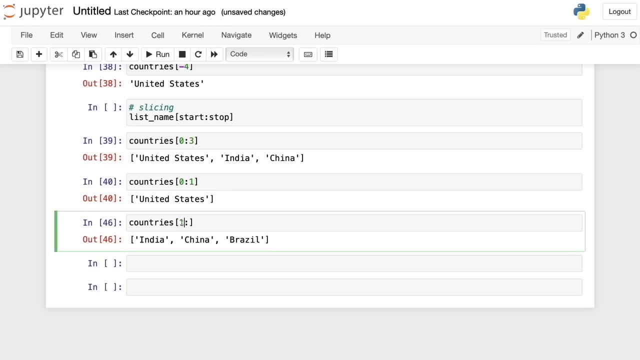 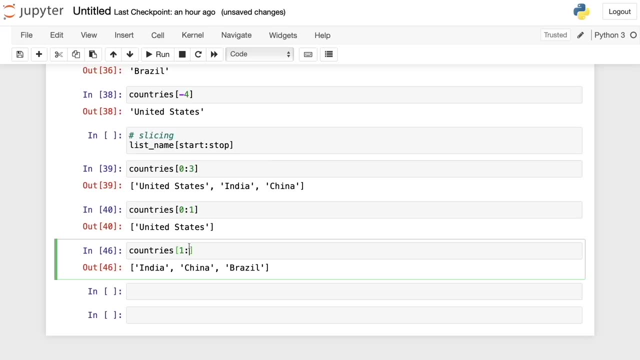 result. So every time you want to get from one position to the last one, you can omit the stop element and just leave it without that element. So just as we did here, and the same goes for the start. So let's say we want to get from the first position, So index zero. 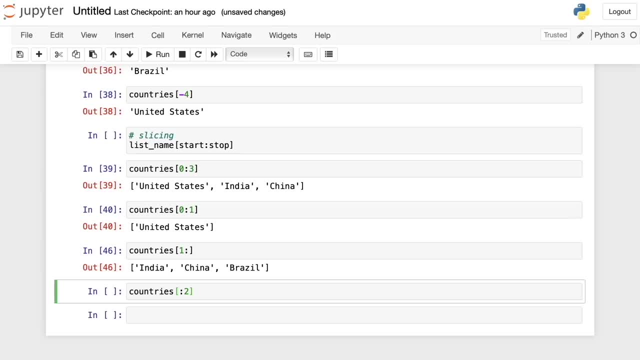 to two, So we don't include the start element and we write only colon and two. So we're on this and we get United States And then we get India, Because this is the first and this is the second. So every time we want to get from the first. 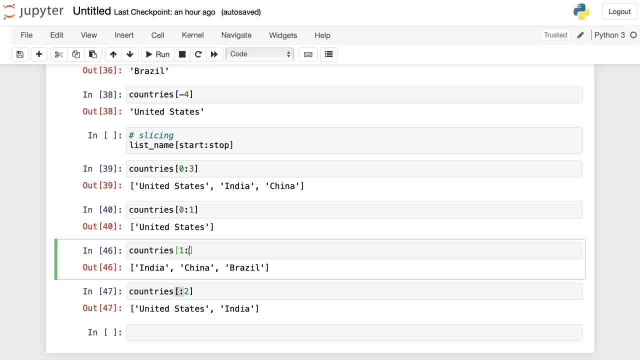 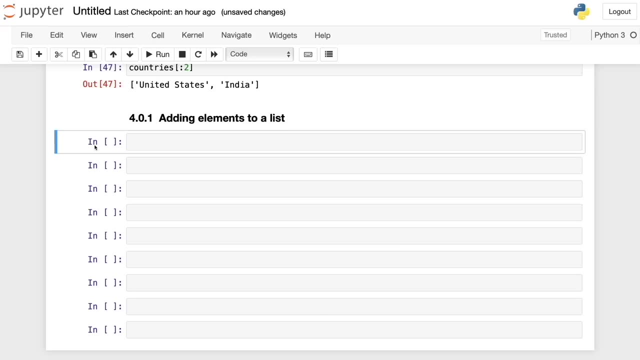 element or until the last element. we can omit that start and stop elements, as we did in these two examples. Okay, now let's see how we can add elements to a list. There are different methods that help us add a new element to a list, So let's have a look. The first one is called append, And 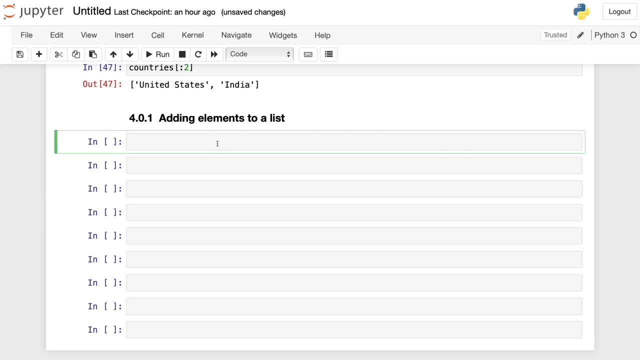 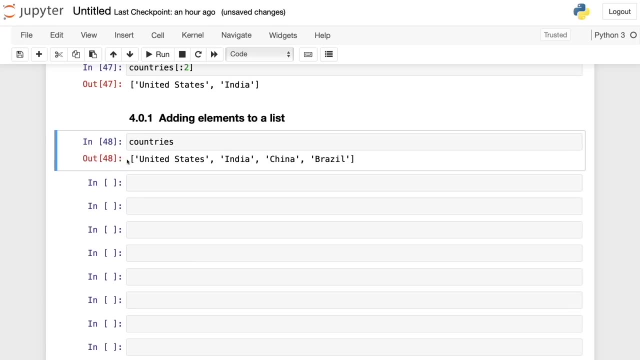 we're going to use that countries list as an example. So I'm going to write countries, just so you can remember. in here it's countries And, as you can see, it has four elements And let's say we want to add any country. 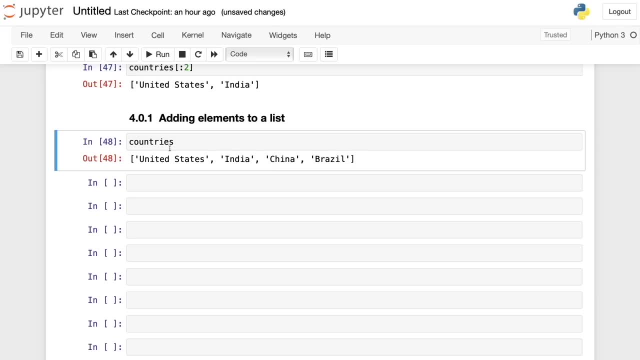 to this countries list. So what we can do is just right here or paste here countries you know, add, append or that append in here, as you can see is this is a method, So inside parentheses we can write the new country we want to add to this. 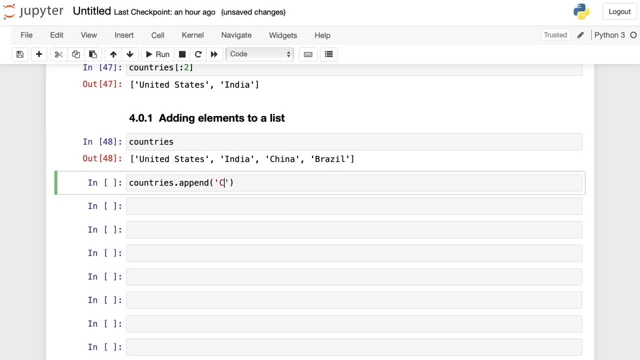 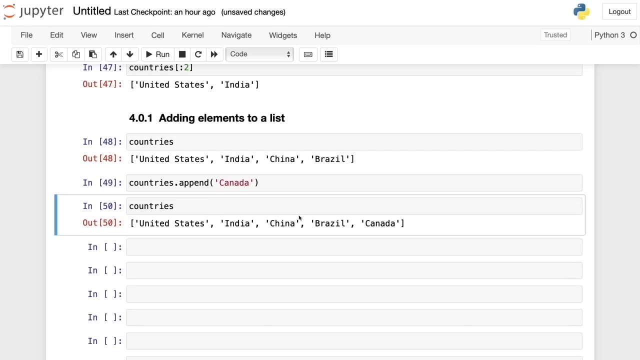 list. So let's say we want to add a country, Canada- So we write Canada And now we run this code. As you can see, nothing is printed. But if we print the countries list again, we see here a new element. So, as you can, 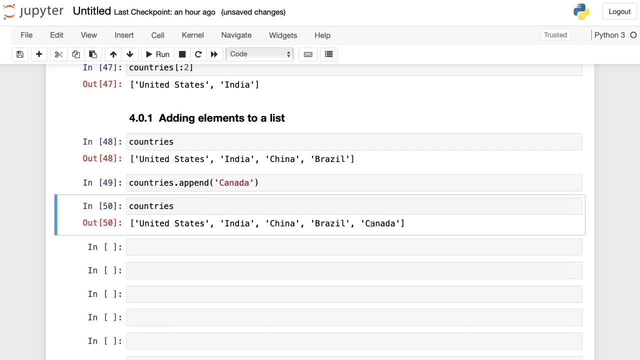 see here: append method adds a new element at the end of the list, So it is by default at the end. But what happens if you want to add an element in a different position? So here you can use another method, which is called that insert method. 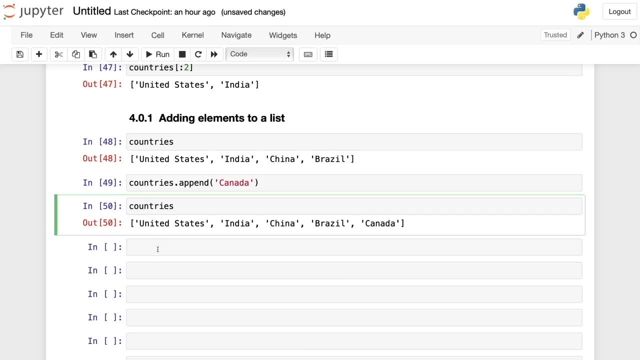 So let me show you: here I'm going to copy countries And now I'm going to use that insert method. So I write that insert, then parentheses. And this one accepts two arguments. The first one is the index, So the position of the element you want to insert. So let's say we want this are the first position. And the second argument that it takes is the new element. 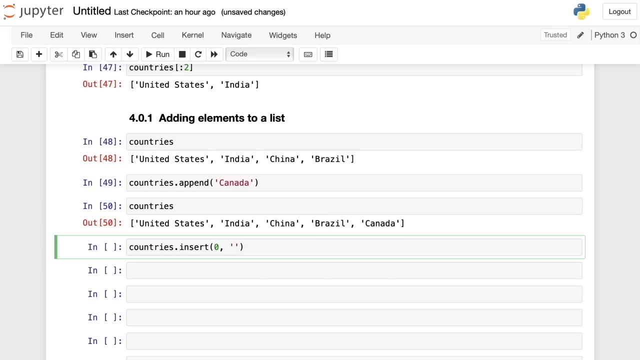 you want to add. So in this case, let's say we want to add elements pain, So these, another country and it's going to be in the first position. So index zero. So let's try. I run this one And again. nothing happens, Apparently nothing happens. And here, if I run this, 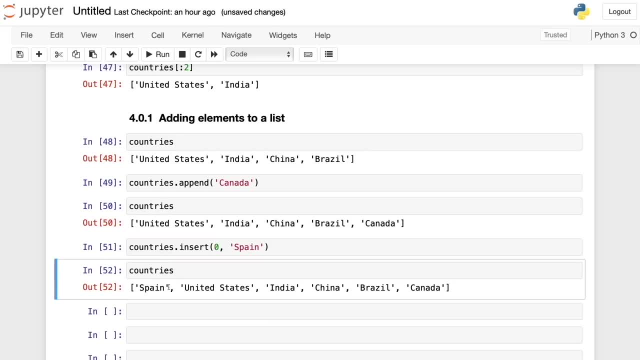 countries list again, we can see that there is a new element, And this element is Spain, And it's located in the first position, Unlike Canada that was placed in the last position. This is one of the difference between the append method and the insert method, So with 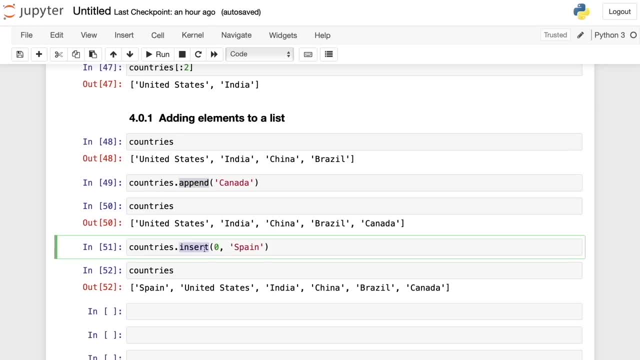 insert. we can specify the position we want to insert this new element, but with append the element is added at the last position. Another thing you can do is to join two lists using the plus operator. we use the task operator to concatenate strings before. 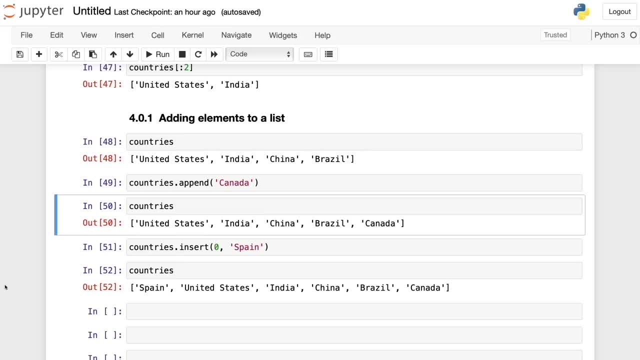 the last position And we can also use the plus operator to concatenate strings before the last position And we can also use the plus operator to concatenate strings before. but you can also join two lists, So let me show you here. I'm going to create a new. 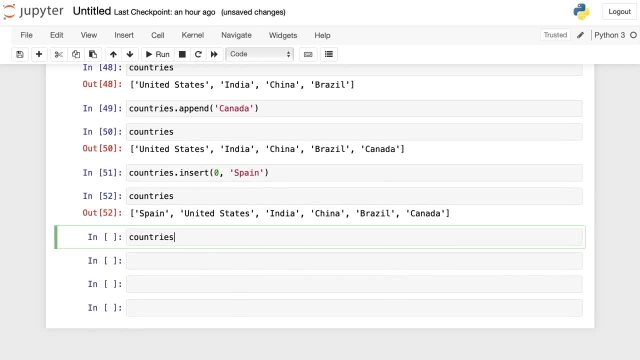 list, just to show you how it works. So my new list is going to be called countries, underscore two. So I'm going to include different countries. So in this case it's going to be the UK, then Germany Too. Let's write Austria, So we have three countries in this new list. 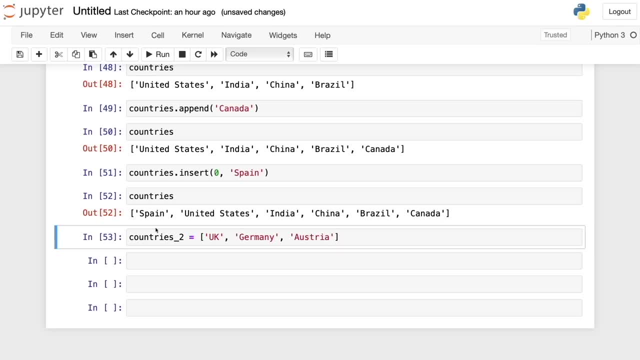 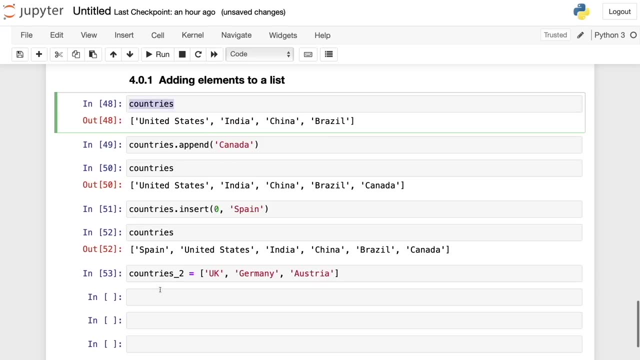 list. And now I'm going to run this one, And if we want to concatenate this first list countries with this second list, countries two, we can use the plus operator. So here I write plus and then I run this one And, as you can see, I got the five elements from. 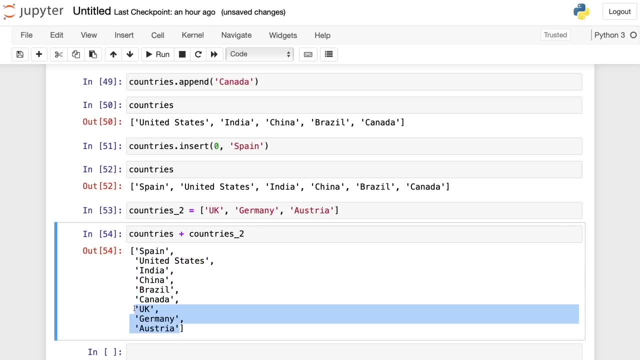 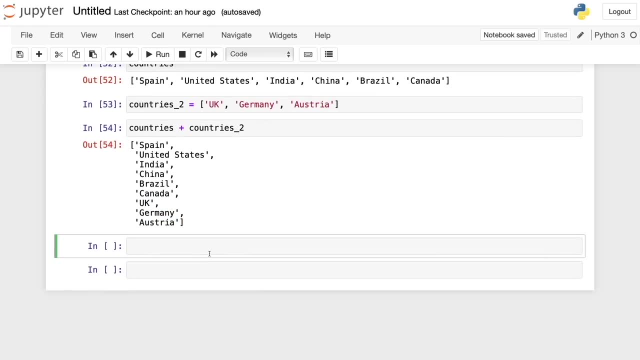 that first list and three elements from the second list. And another cool thing you can do in Python is putting these two lists inside another list which is called nested list. So let's try out. So here I'm going to create a new list And it's going to be called nested. 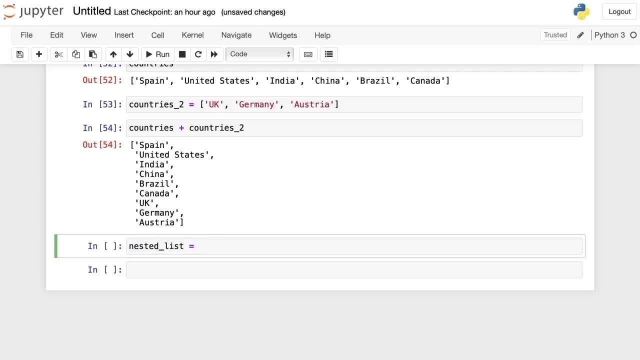 underscore list. In here I'm going to open a square brackets to create a new list And As elements I'm going to write countries, which is my first list, and then coma, and then countries underscore two, And this is my second list. 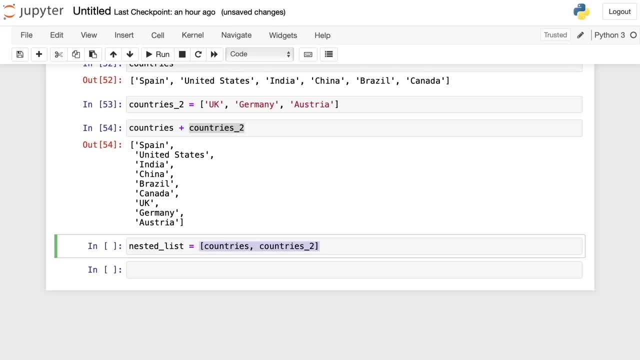 So, as you can see here, these elements inside this list- the first is a list in, the second is a list- So we have a list inside another list which is called an asset list. So I run this one and then I paste nested underscore list and we run and we get here. 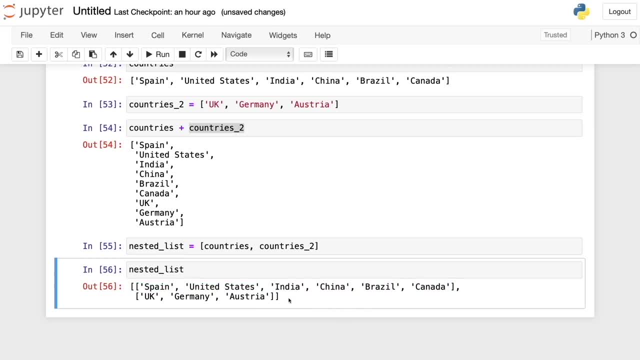 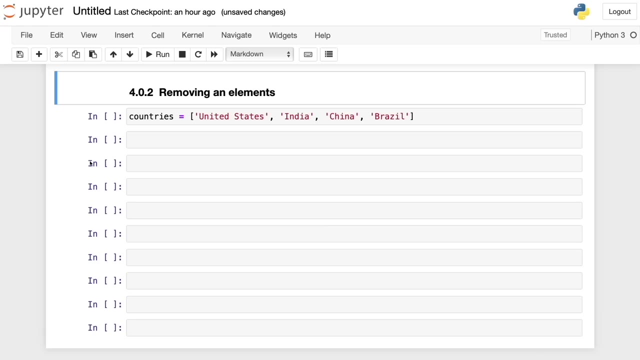 the first list as first element and the second list as second element. you will see this nested list so often, but you will encounter this a couple of times, So it's good for you to know. So now we're going to see the opposite of adding an element to a list which is removing. 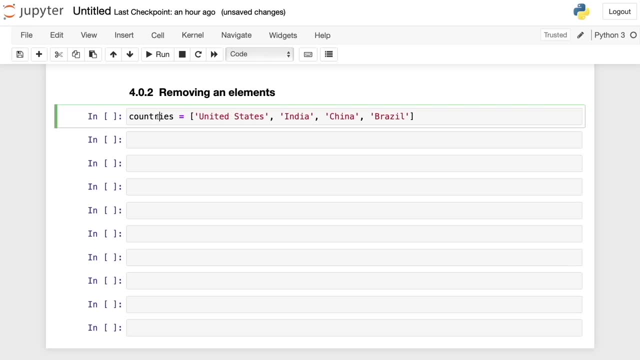 an element. So here I just pasted the countries list we had before And what we're going to do is to remove some of the elements of this list. So there are different methods that help us remove an element from a list. One of them is the remove method. 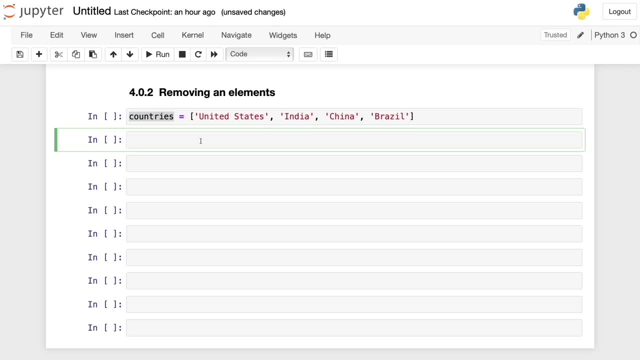 So to remove an element using this, we have to first write the name of the list and then use that, that sign and then write remove And write parentheses in inside here we have to write the element we want to get rid of. 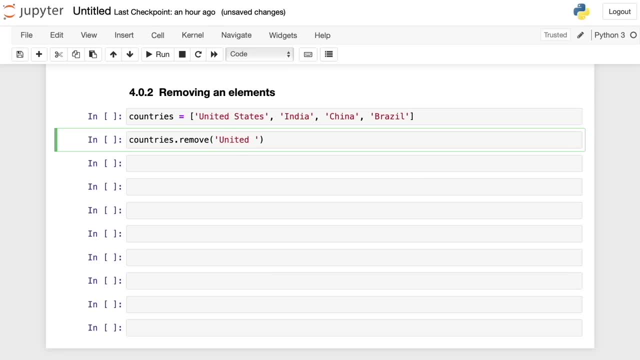 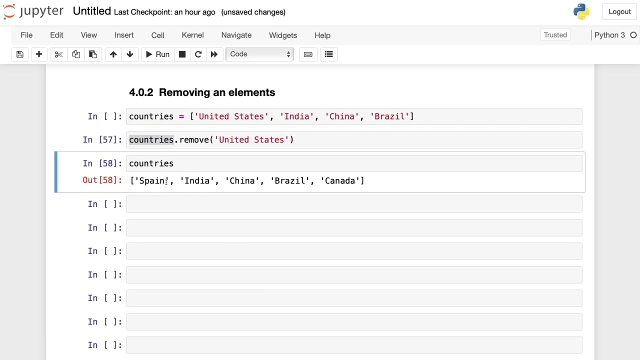 So first it's the United States, So I write United States And let's run this one And, as you can see, apparently nothing happens. bad if we paste countries here. we have all the elements, but United States is not there. 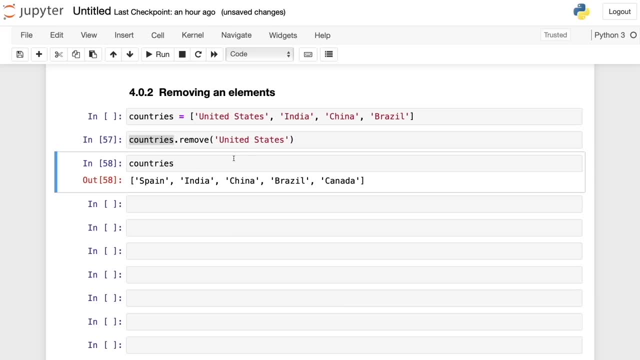 So, as you can see, the first matching value was removed, But you can also remove an element by its index, So this is accomplished with the pop method. So I'm going to copy all of this And now I'm going to paste it here. 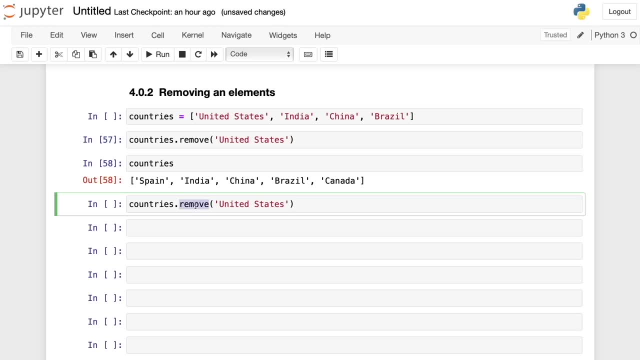 So instead of writing that remove, I'm going to write that pop in here. I'm not gonna use the name of the element, But it's index, So I write the index in this case. let's remove the last one, So it's going to be index minus one. 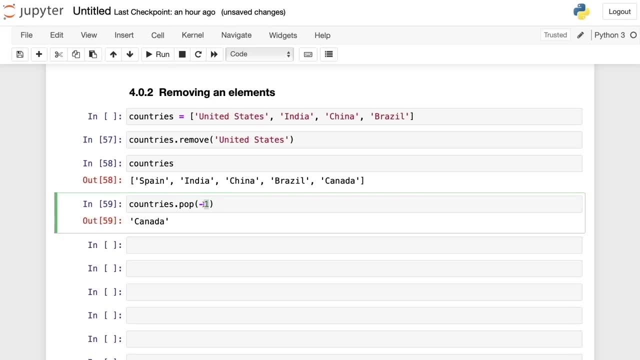 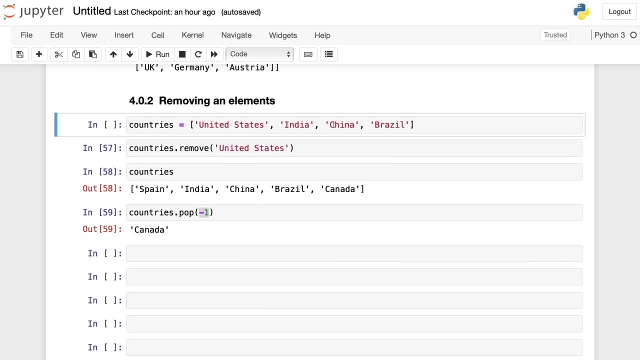 And what pop is going to do is to remove the element with index minus one and then returns this element. So this element is Canada. I didn't run this code here, So you can ignore it. So I'm going to comment this one. 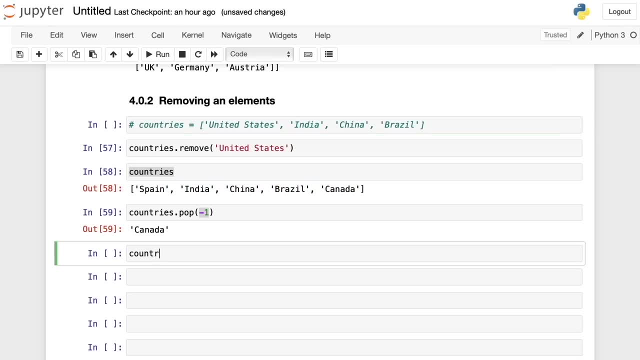 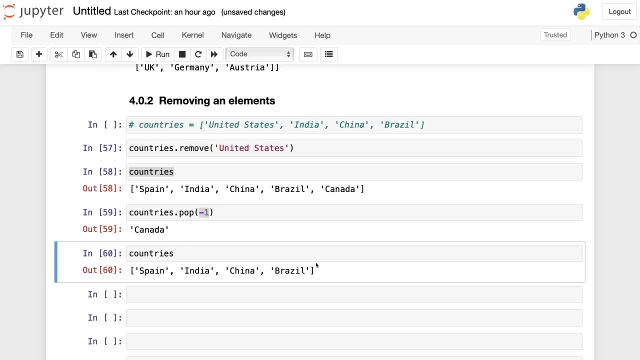 And our reference is going to be this, this list. And to verify, we just write countries and then run And here, as you can see, there isn't Canada anymore, And that's how you remove an element, using the pop method. But there's still another way to remove an item using an, a specific index, and it's the. 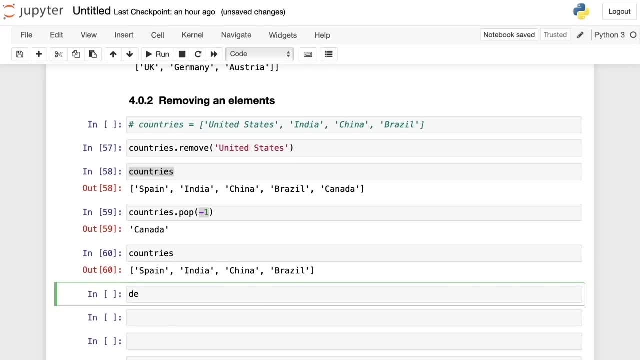 Dell. So I'm going to show you here Dell, it's the function Dell function. In here we have to write the countries list, Okay, And then again open square brackets in here, write that index. So I write here the index and, unlike the pop method, we're not going to get the name. 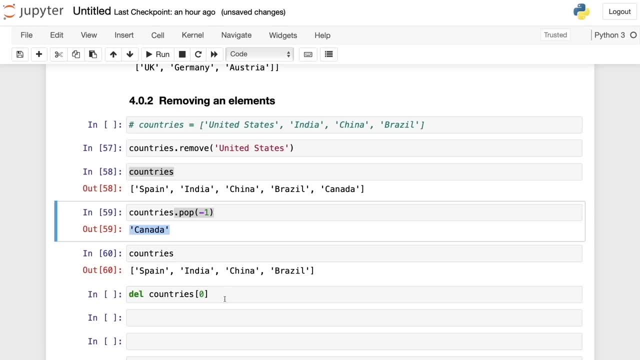 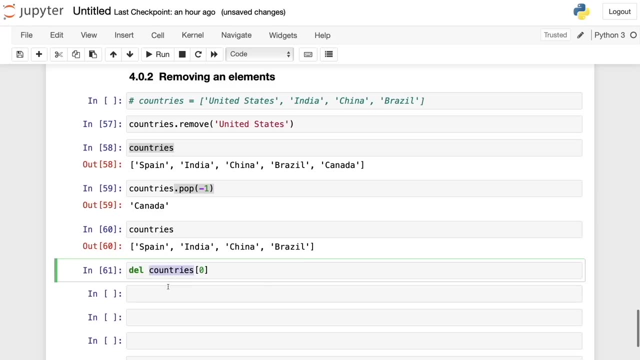 of the element we're getting rid of, but just deleting the elements. So I run this one And here we didn't get anything And I'm gonna print this. So countries, and that element at index zero was removed. Spain, because that's the first element. 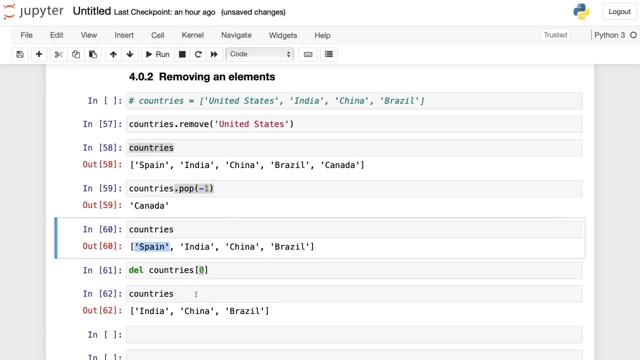 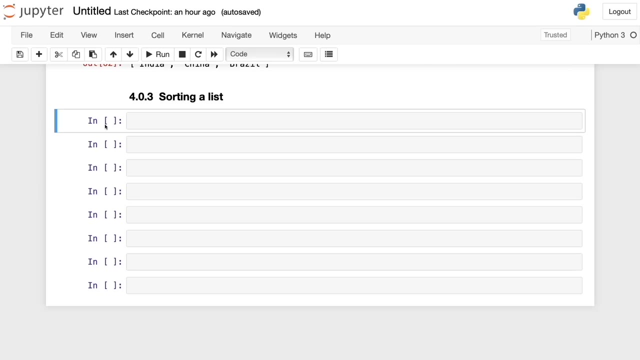 So we deleted or we remove the first element. So we only got India, China and Brazil. And there you have it: three different ways to remove an element from a list. Okay, now let's see how to sort a list. We can easily sort a list using the sort method. 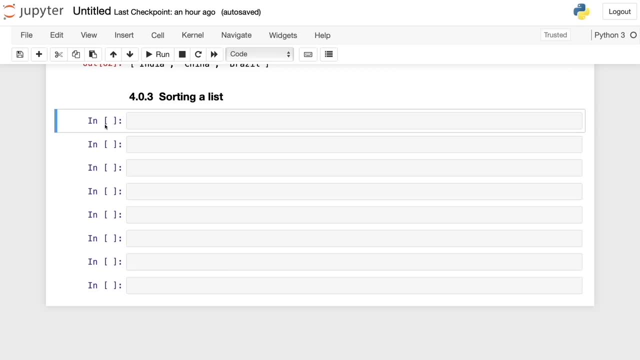 Let's create a new list called numbers and then sort it from the smallest to the largest number. So I write numbers and then open square brackets. So I'm going to write some random numbers. So first four, then three, then 10, then seven, one and then two. 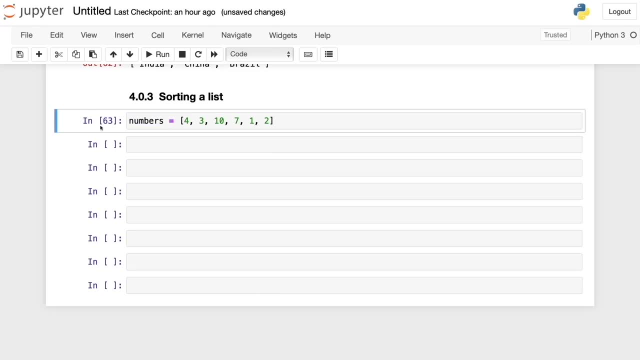 So this is my list. So I run this code And now to sort it from the smallest to the largest number. we write numbers, then sort and then open parentheses And by default this is going to be sorted from the smallest to the largest number. 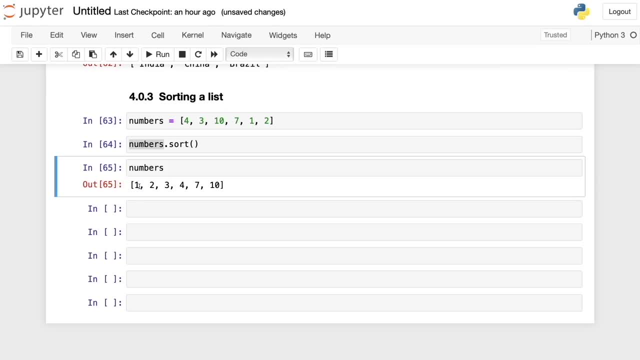 So I run numbers again in here. it starts with one and it ends with 10. And, as you can see, it's from the smallest to the largest number. So that's the default behavior of the sort method, But we can control how this works. 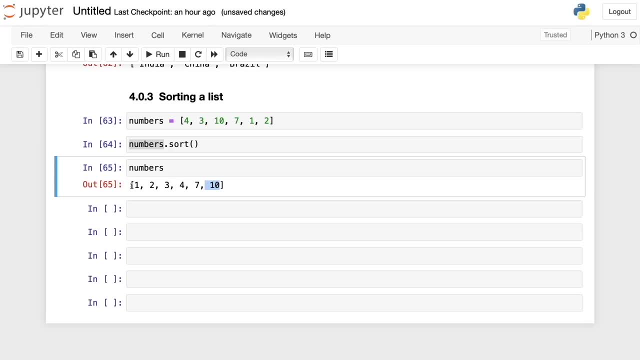 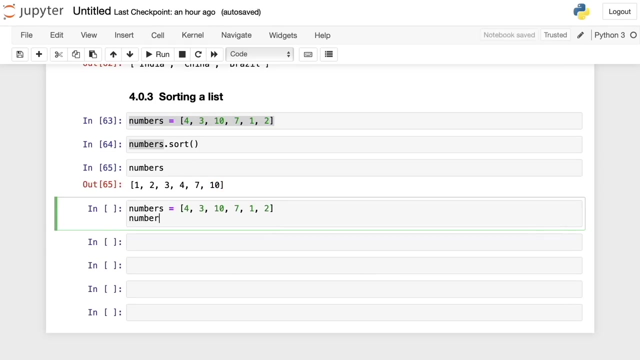 So we can add that reverse argument to the sort method. So if we want it to be descendant, we set reverse to true. So here again I'm going to create again the numbers list and then write numbers that sort in inside parentheses. I write the reverse argument and I'm going to set it. 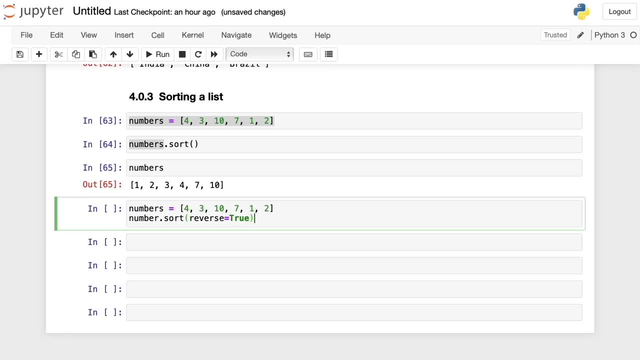 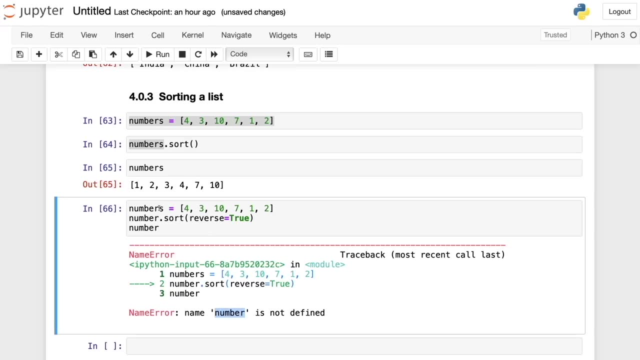 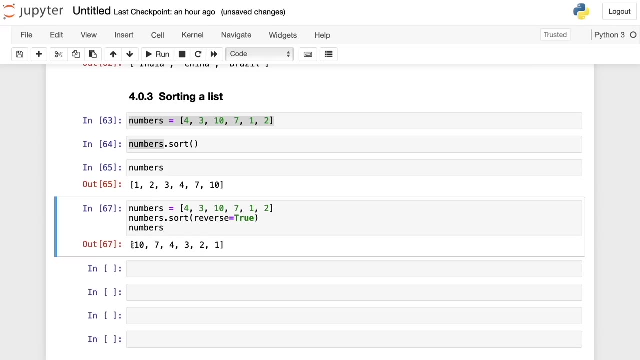 to true here. And then I'm going to print numbers. So here an error, because here it I wrote number and its numbers. So here I'm going to add the s and here s two. so run again And here we have from the in. here we see that the list is sorted from the largest number. 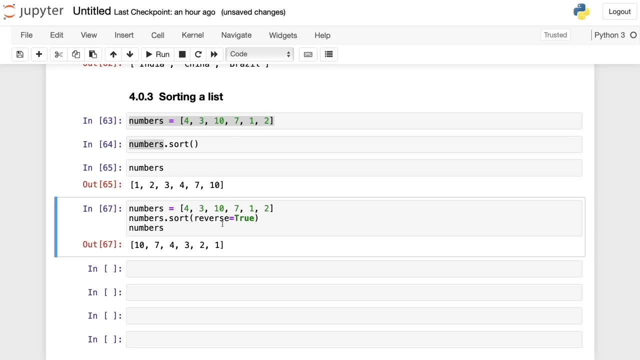 to the smallest number. So, as you can see, the default behavior of this sort method is reverse equal to false. So you can control it here By writing reverse equal to true, as we did here. okay, now let's see how we can update. 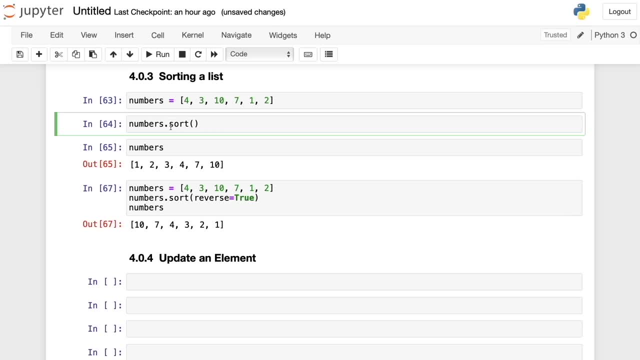 values in a list. To update a value on a list, we use indexing to locate that element we want to update And then we set it to a new value using that equal sign. So let's say we want to update the first element of this numbers list. 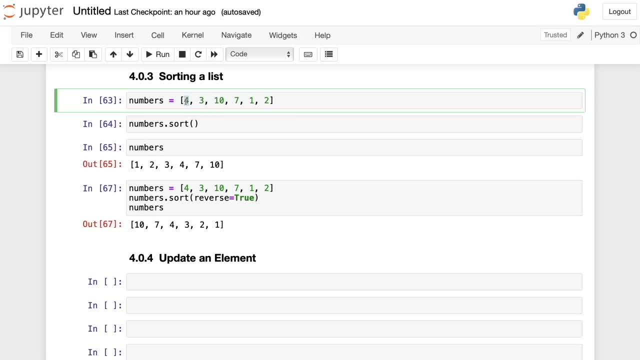 So now it's four, but we want it to be, let's say, 1000.. So we write here numbers And we use indexing. So we write numbers. the first element has index zero. So we write numbers, square brackets, then zero, then we set it equal to the new value. 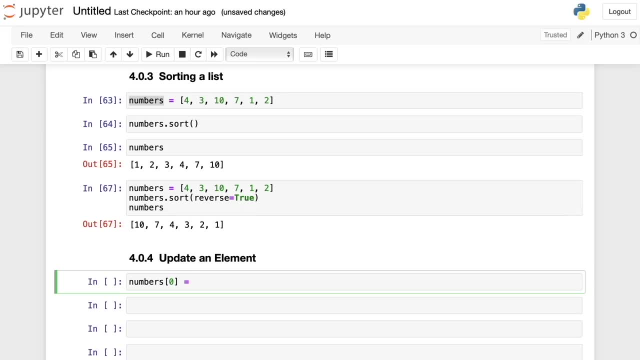 we want to include. So in this case I'm going to write 1000. And now I'm going to print the numbers, please, to see the results. So run this one And, as you can see, it's working. As you can see here, the numbers list we got is from the last change we made. 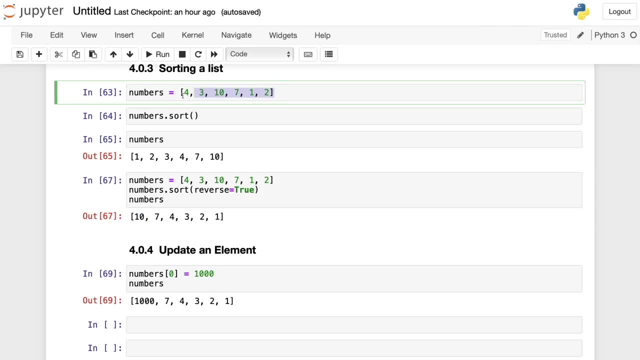 So the one that starts with 10.. So it's not this one, but this one, because it's the last one we ran. So instead of 10, we replace this one with 1000.. Because this is the first element with index zero. 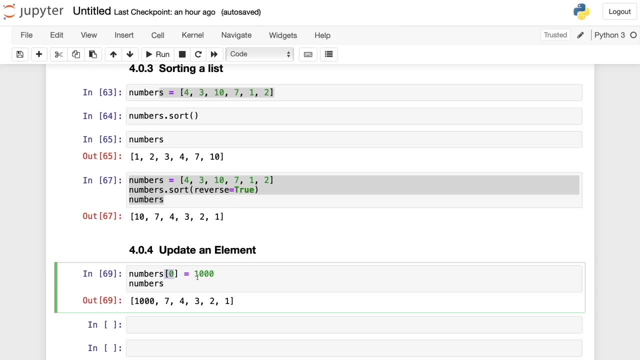 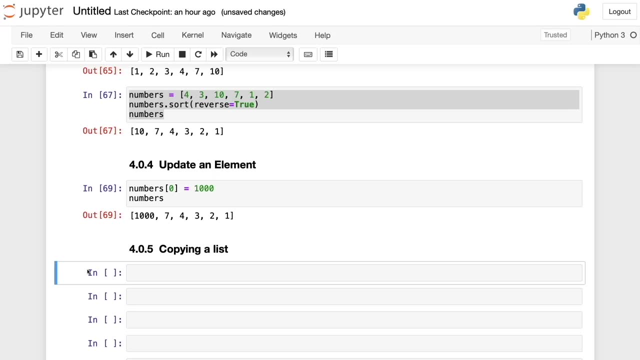 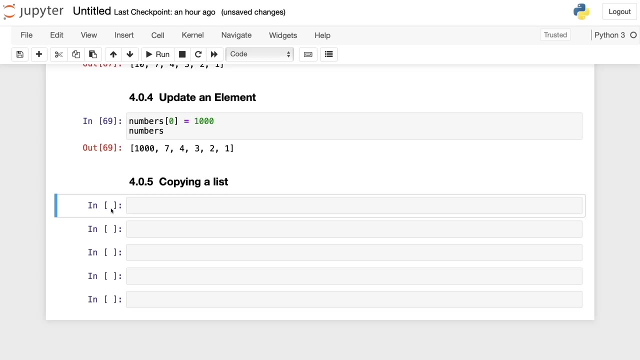 So we did numbers, square, brackets, zero, and we update that first element with 1000.. Okay, finally, we can make copies Of the list we created. So there are different options to create a copy of a list. One of them is that slicing technique. 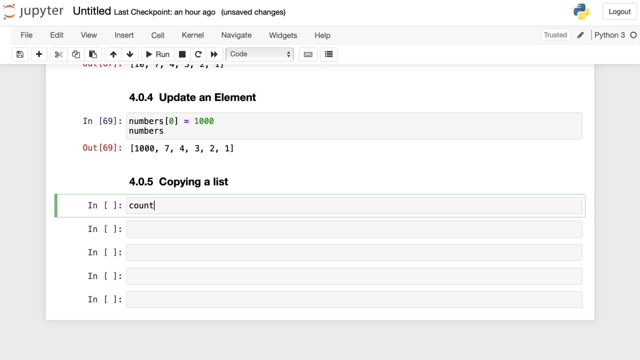 So, as you might remember, to do slicing, we have first to write the name of the list, which this case is countries, And then we open square brackets. then we're supposed to write the start and stop. So in this case, we're not going to write start and stop. 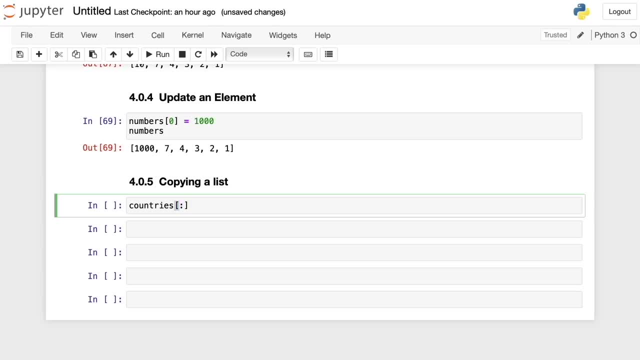 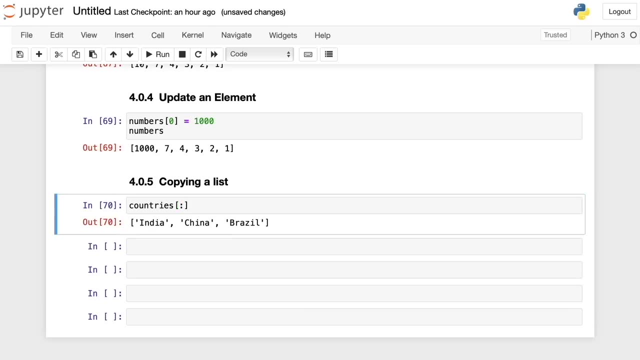 But only colon. So if we don't write start and we don't write stop, it means we want the whole list. So let's try this out. I'm going to run this one And, as you can see, here we got the whole list. 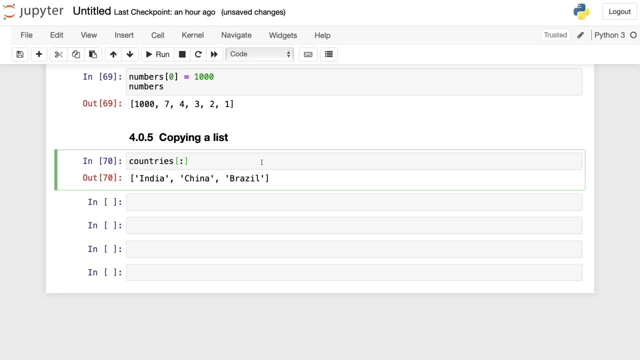 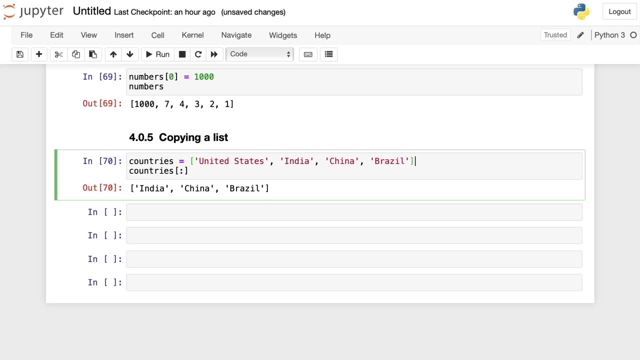 So the countries list doesn't have the original values because of the changes we made when we added and remove elements. So I'm going to paste the original countries list with the four original values, that are, United States, India, China and Brazil. 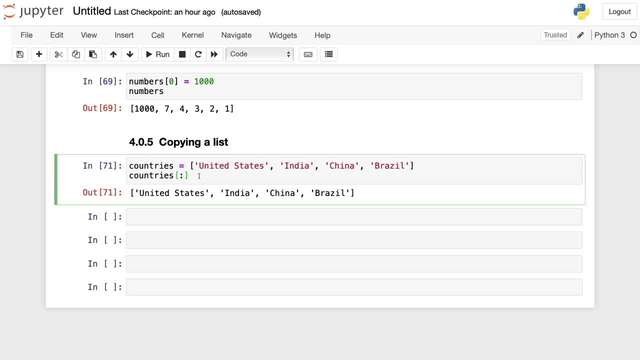 And here let's see that changes. and now we test it out And, as you can see, we got the whole list. So from the first element, United States, to the last element, Brazil, because we're slicing the whole list. So if we write here new underscore list and we set this, equal to countries with this. 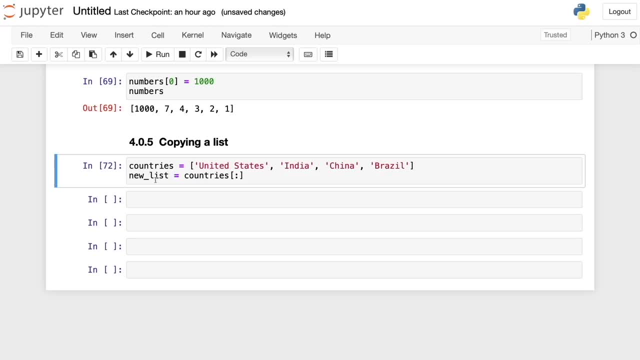 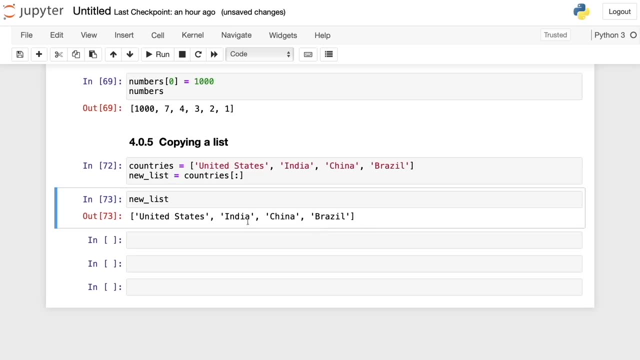 slicing. what is going to happen is this new list is going to have the same values as the country List. So I write here new list And as you can see here, it has the same values. So we created a copy of that countries list. 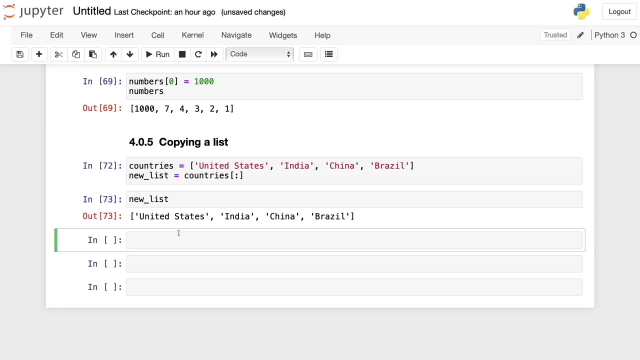 So this is one way how you can create a copy, And the second way is more straightforward or is more explicit, So is using the copy method. So we write again countries, the name of the list, and then we use the copy method. 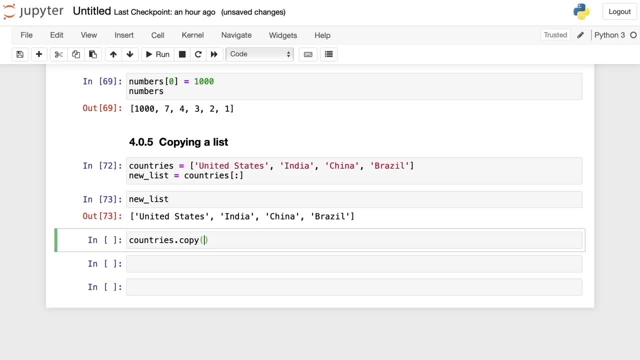 So write copy and then parentheses. So with this we create a copy of this list. So let's run this code And, as you can see here, it returns the list. But if we assign this to a new list, we're going to create a copy. 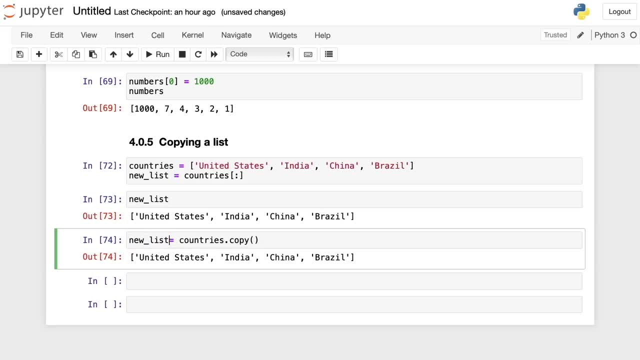 So here I'm going to write new underscore list, underscore two. So here we assign this copy to this new list. So I'm going to copy this new list and paste here And, as you can see, here We have the values of this list which are the same as the original countries list. that 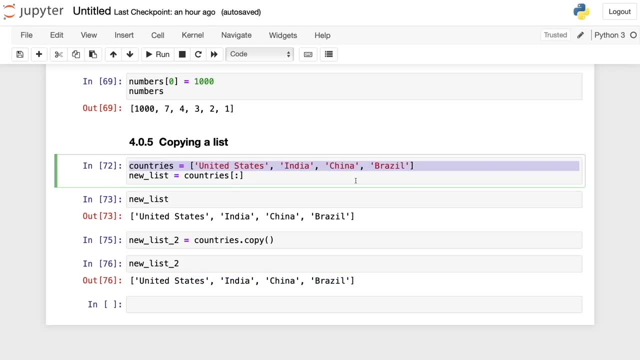 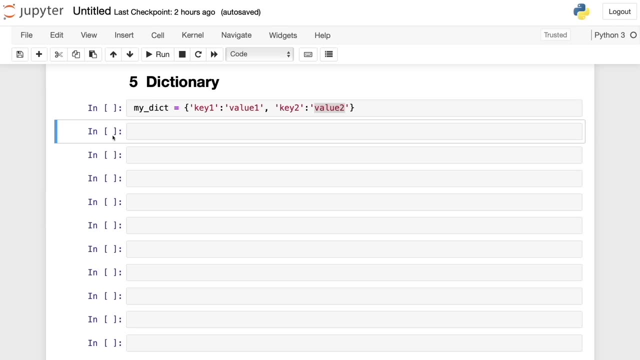 is here And that's it. That's how you make a copy of a list. So now let's see how dictionaries work in Python. In Python, a dictionary is an unordered collection of items used to store data values, And a dictionary contains a key and a value. 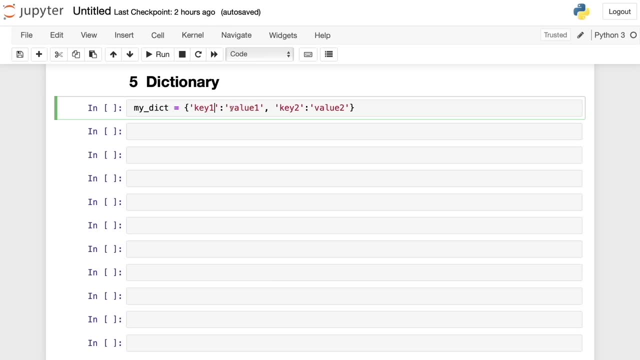 So this is what you will offer And see in a dictionary. So here, for example, the name of my dictionary is my underscore dict, And to create this dictionary we have to use these curly braces. So we open curly braces and inside we write our first item. 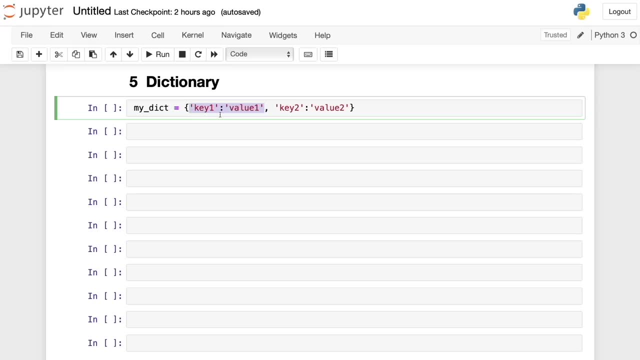 And the first item consists of a key here on the left and then a value here, and it's separated with the colon. So here we have the key, then column and then the value, And then we have here the second item. 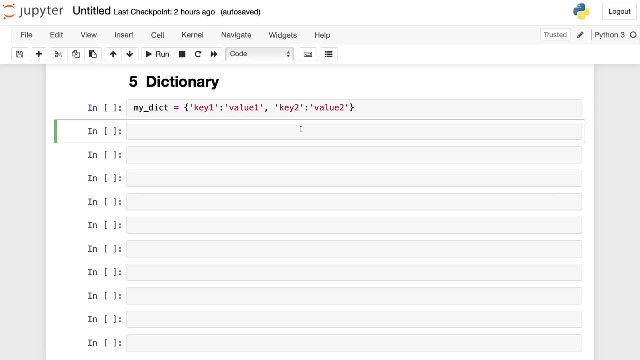 So the second key and the second value. So now let's create a dictionary that has some basic information about me. So I'm going to name this dictionary my underscore data. And now, to create this dictionary, I'm going to open curly braces. 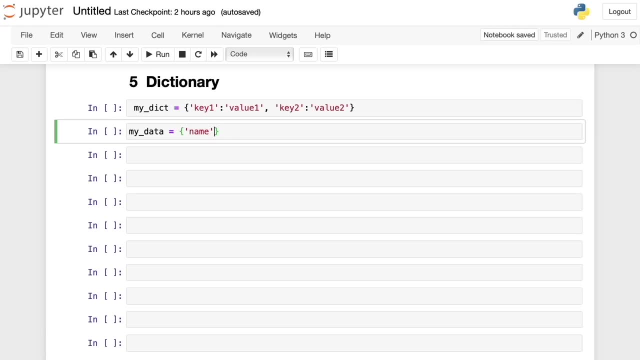 And the first key is going to be name. So I write name And it has a value: that is my name. So I'm going to write Frank, so I open single quotes and then write Frank, And then I'm going to add a new item. 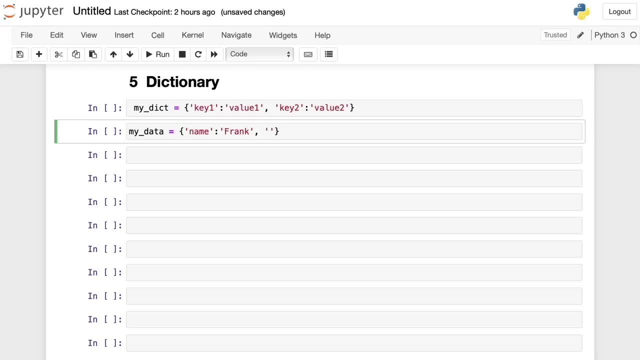 So I write comma and then the second key is going to be age And the second value is going to be my age. So in this case, I'm going to write my age, which is 26.. So, as you can see, here, the first is a string. 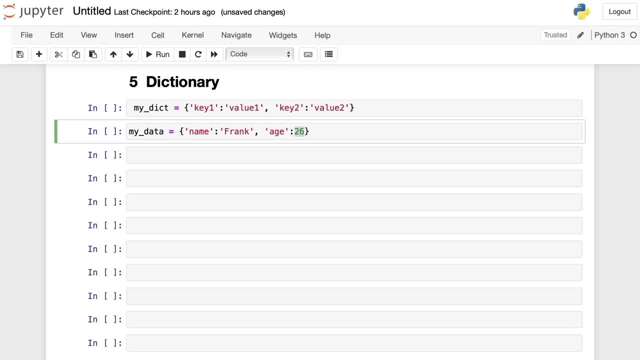 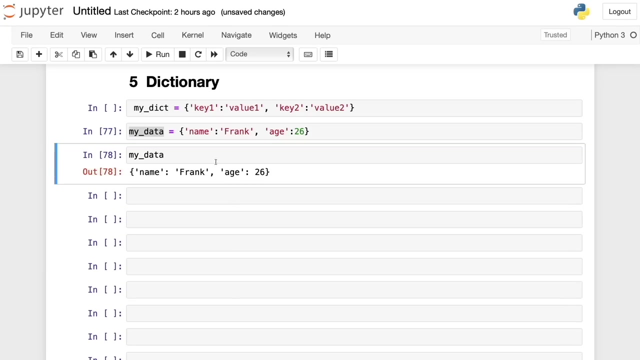 The first value is a string And the second is integer, So we can mix different data types. So now I press Ctrl Enter to run this code. and we created this dictionary. So now I write my underscore data in. here you have the dictionary we created. 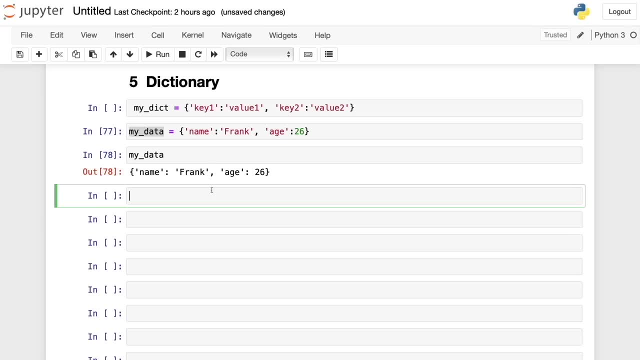 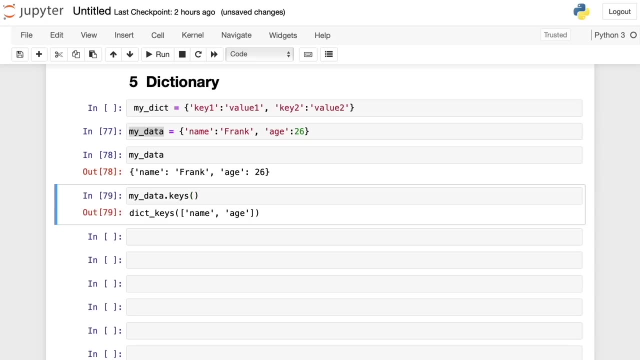 So here we can get the keys of this dictionary. we only have to write my underscore data. that keys. So this is the keys method. So we run this And we get this dict underscore keys And the values are name and age, which are the keys of this dictionary we created. 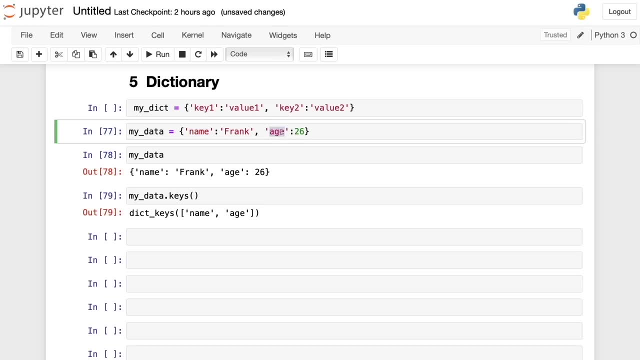 So name the first key and H the second key. Now we can get also the values, So my name and my age. So we just have to use that values method. So I'm going to paste this one here And instead of writing that keys, I'm going to write that. 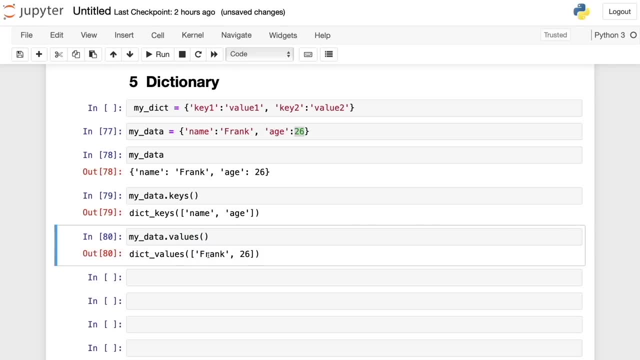 values and now run this and we get my name and then my age. So next I'm going to get the items. So, as I said before, an item is this. So this is the first item And this is the second item. 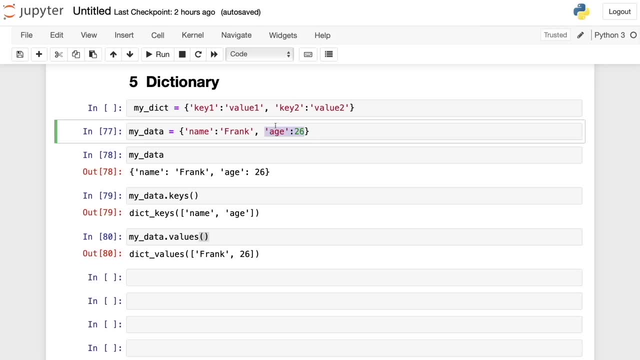 So we can say that the item is a pair of key and volume. So we can get this by using the items method. So instead of writing that value, That values, I'm going to write here that items and then run this one. 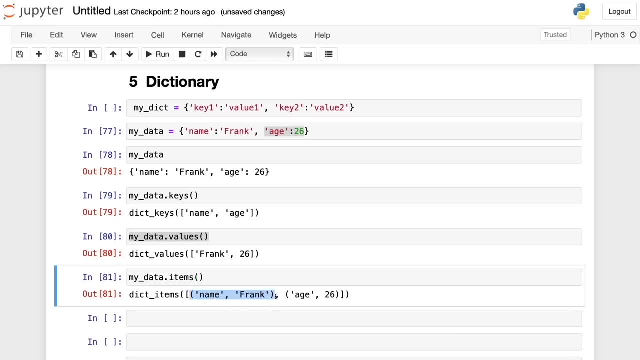 So here we got the first item, So the first pair key and value, which is my name, and well, that key name, and then my name, Frank, and then the second item, so the key name H and the H, which is 26.. 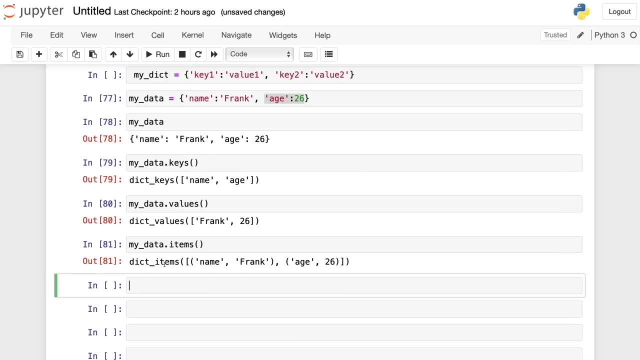 Now we can add a new pair of key value in this dictionary we created. So let's say we want to add my height, So I write my data in. let's say we want to add the key name height, So I write height. 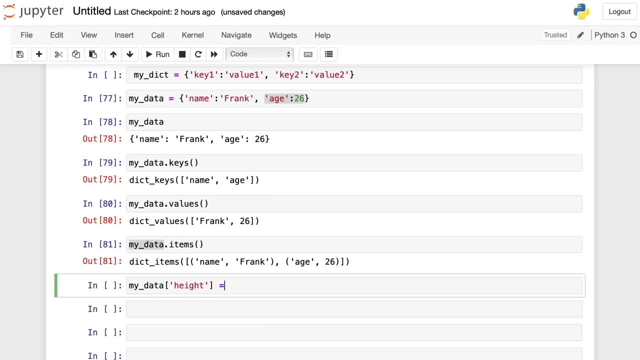 So we use square brackets here And then we set this to the value, So let's say it's 1.7. So I write my data and then square brackets, then hide inside it, And then equal to 1.7.. 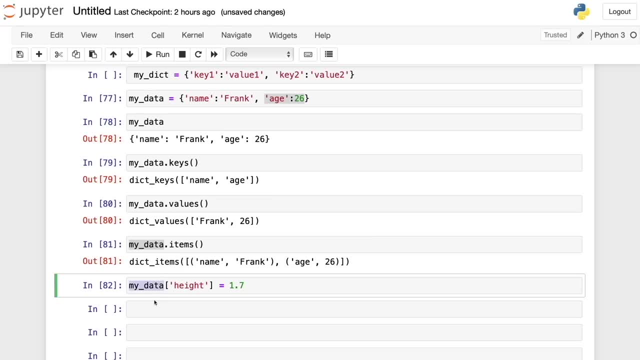 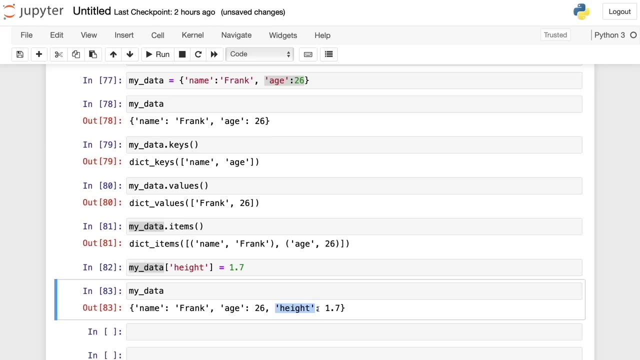 So if I run this and then I run the dictionary, we can see that there is a new item and it's the height, So height colon and then 1.7.. This is how you add a new item to the dictionary. 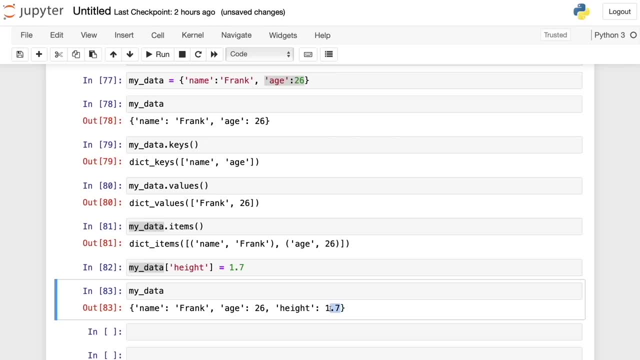 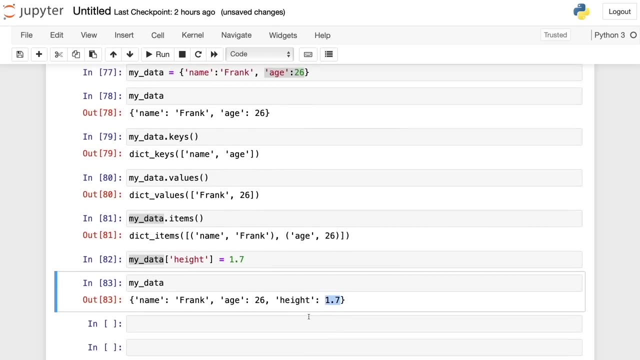 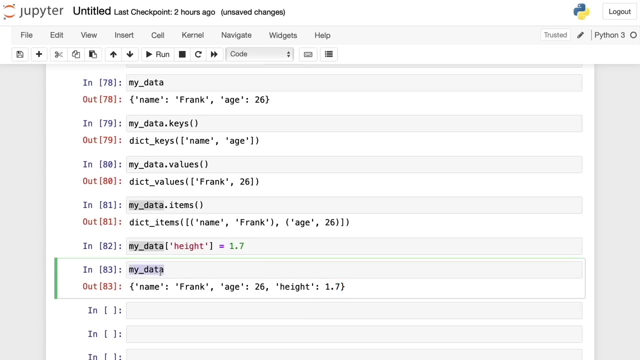 And now we can update this height. So let's say I'm not 1.7. But I'm 1.8. So what we can do is to use the update method to update this value. So I write my underscore data in here. I can use the update method. 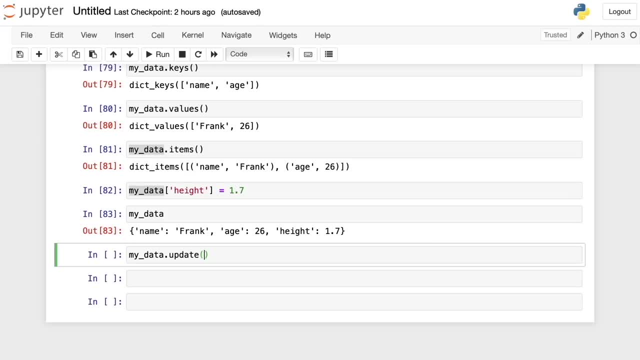 So I write update And then inside parentheses we have to open curly braces to update this new item. So I'm gonna write the key, which is height, And then I'm going to set the new height, which is 1.7.. 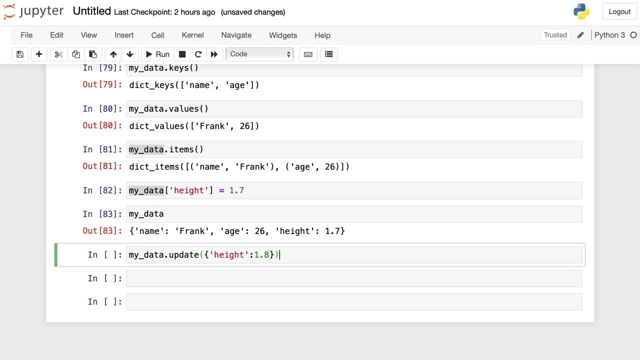 Okay, 1.8.. So let's try this out. I run this And then let's see the values. So let's see if it was updated. So I run this and we got the height 1.8. So it's perfect. 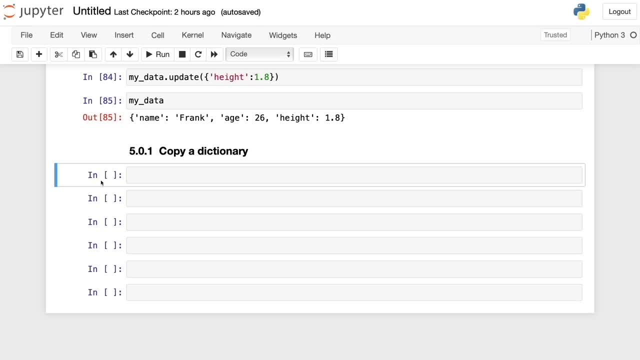 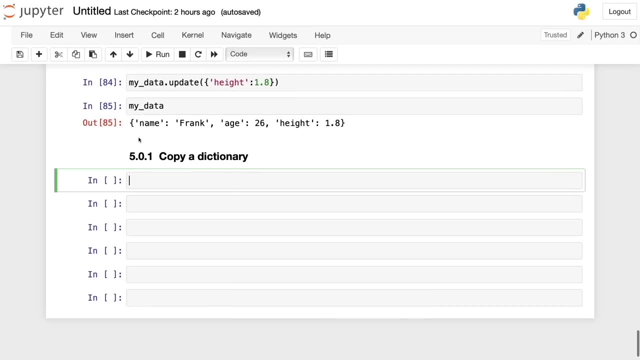 So now let's see how we can make a copy of a dictionary, the same way we did before for the lists. So to make a copy, we just have to write the name of the dictionary. in this case it's my underscore data. 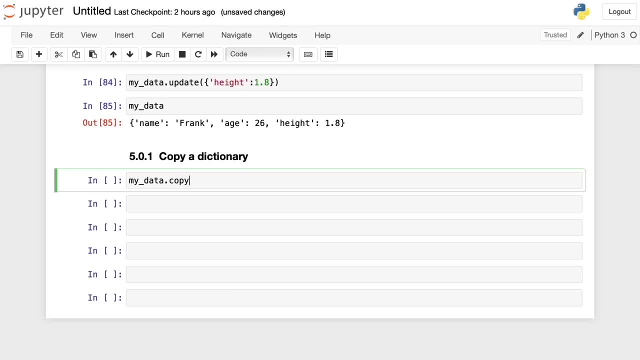 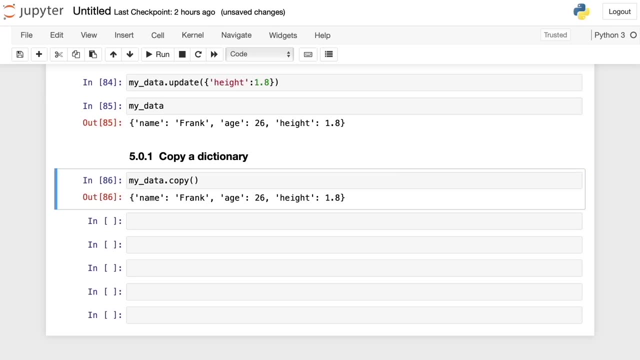 And then, as we did for the list, we can use that copy method. So we write that copy with parentheses and then we create a new copy. So here you can see the copy, And now I can assign these to a new dictionary. 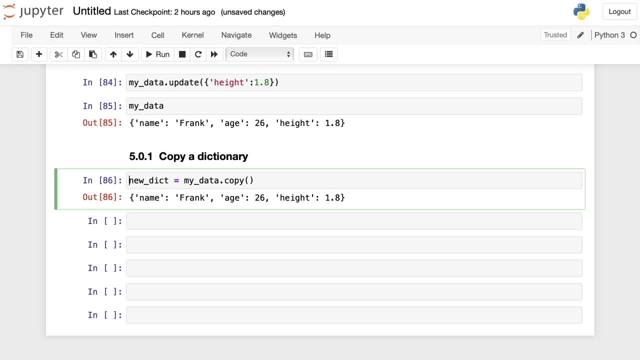 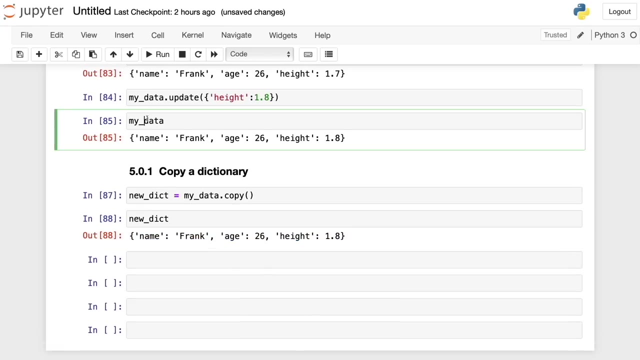 So I'm going to write new underscore dict And now I'm going to copy this one, I'm going to run, and then I write new underscore dict and run this And, as you can see, it has the value: The value of the my underscore data dictionary. 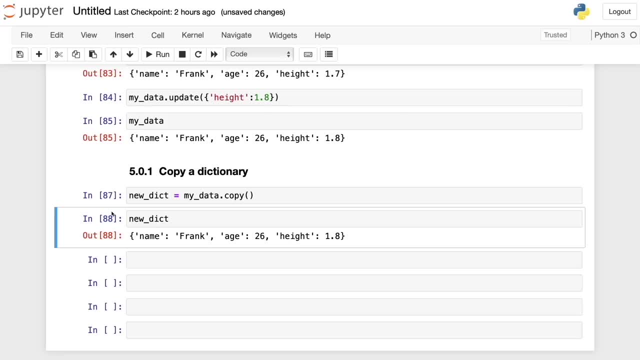 And something I didn't tell you when I make a copy of the list is that if you change the data inside my underscore data dictionary- so the old dictionary- that effect is not going to be seen in the new dictionary. So, for example, if we write one that nine and here I update this in the old dictionary. 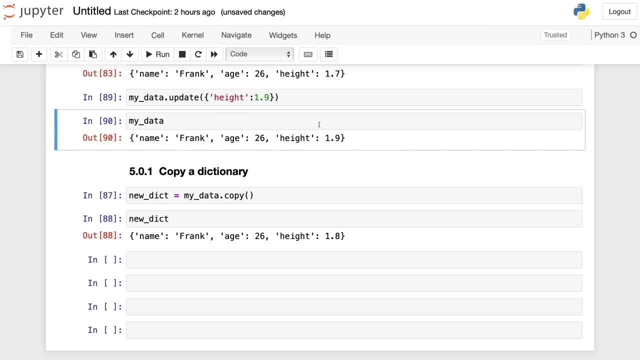 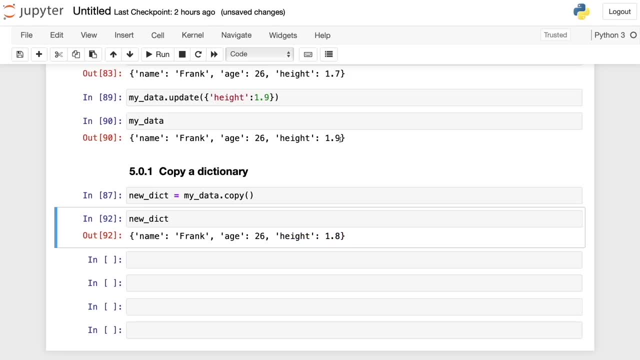 with the same value- 1.8, and it doesn't change to 1.9.. This doesn't happen. if you make one of these copies, most people do, So let me show you what I'm talking about. So most people just make a copy doing new dict, underscore, dict. 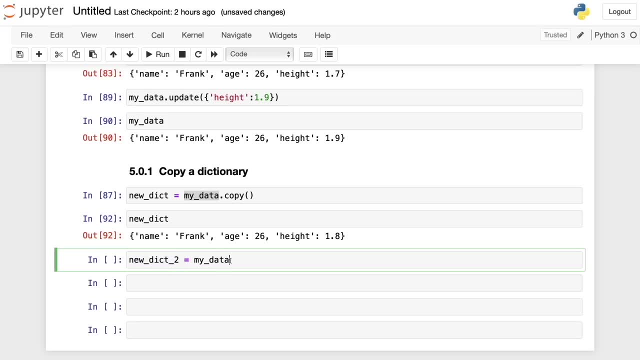 So let me show you what I'm talking about. So most people just make a copy, doing new dict underscore dict. So let me show you what I'm talking about. So most people just make a copy, doing new dict underscore dict. So this is my new dictionary. 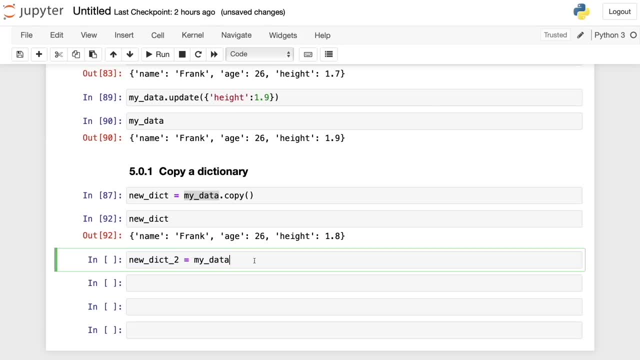 So this is my new dictionary. So this is my new dictionary. So what happens if I run this and then I will show you the values of this new dictionary? So this is 1.9.. And if I update this to, let's say, 1.95.. 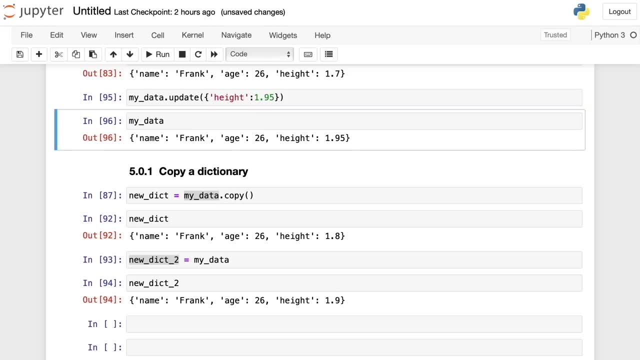 So update here, Update here: Here is 1.95.. And if I run this new underscore, ticked underscore, ticked two, we can see that the value was updated to and this shouldn't happen. So if you want to create a, 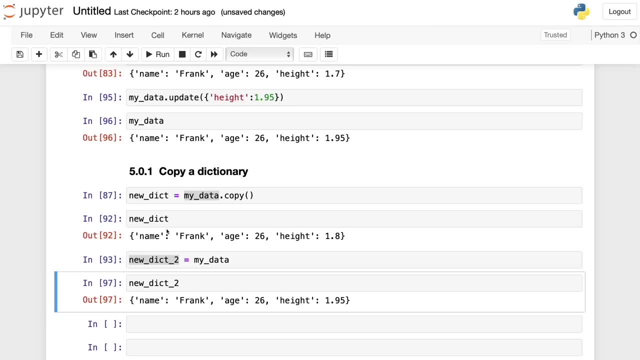 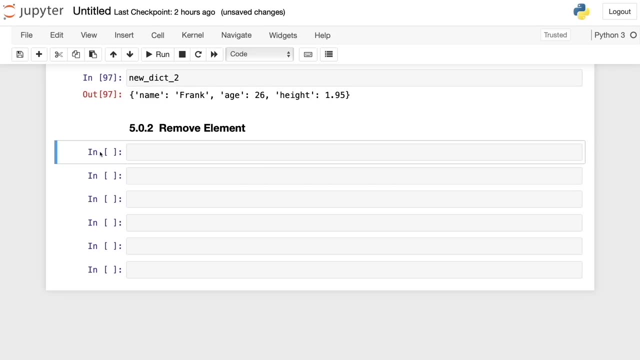 new dictionary that works independently from the old dictionary, you should use that copy method, And this is the same if you're making a copy of a list. Finally, let's see how to remove elements from a dictionary. So, just like we did with the lists, we can remove an item in a dictionary. 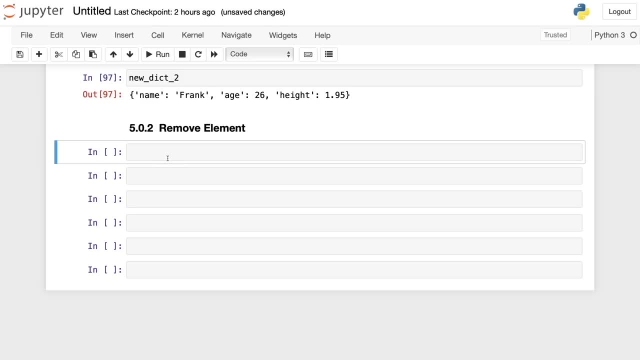 So there are different options. First we have the pop method. So right, my underscore data. I'm using the old dictionary we've been using so far, So my underscore data and I'm gonna write that pop. So this is the pop method. So here I can write the key. 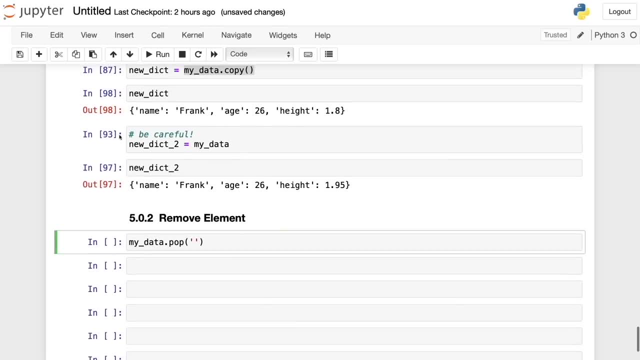 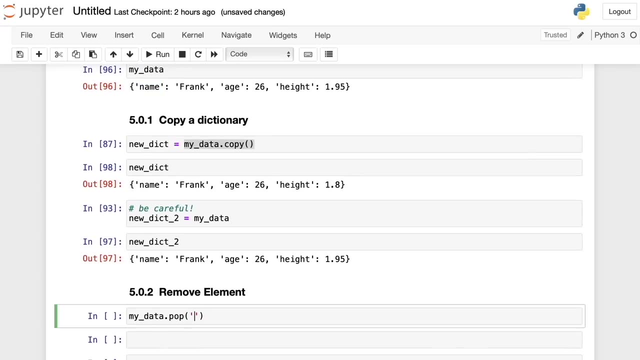 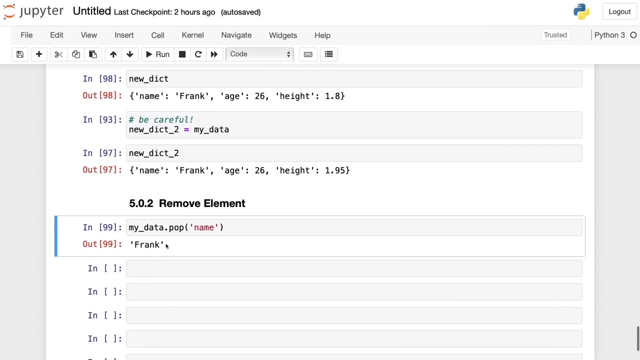 So in this case I'm going to write the key. Let me see here my underscore data: the key name. so I write pop, then parentheses them name. So, as you might remember, the pop method returns this value of the key. Before we did with the list and it returned the list element. 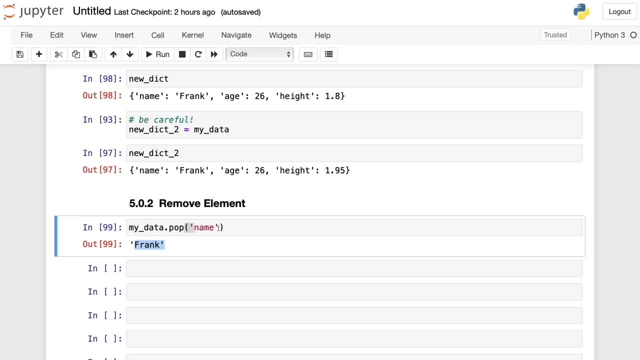 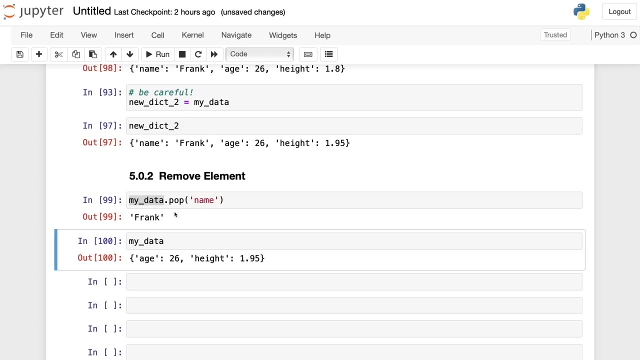 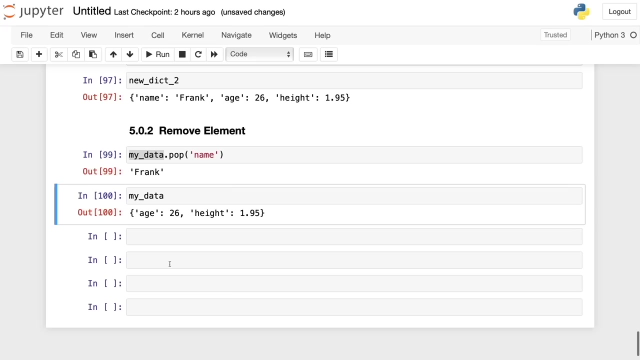 In this case, it returns the value of the key. So this is the key name in. it: returns the value. So if we print this, my underscore data dictionary, we see that this pair key value isn't here, So we successfully remove this item. Another way to remove an element. 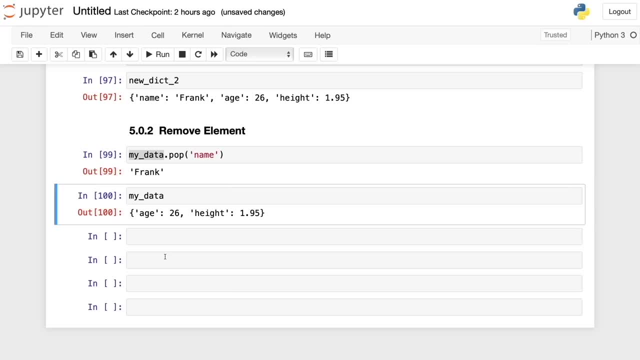 or an item from a dictionary is using that delt function. So we write del and then we write the name of the dictionary, So underscore data, And then we have to specify again that name of the key. So we open square brackets and open quotes In here. let's say we want to delete or remove the H key with 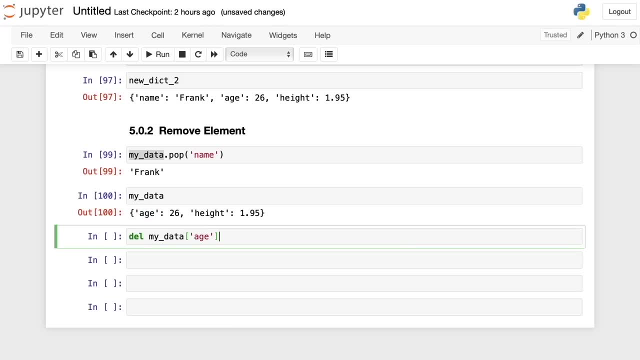 its value, So right age, and we run this And then if we print this dictionary again, we get the dictionary and we see that that H key was removed and also its value, And finally you can remove all the items in a. 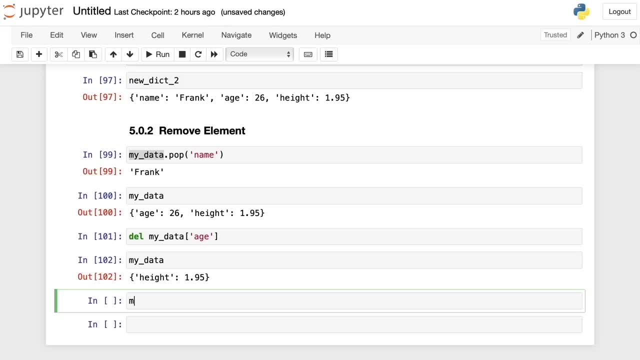 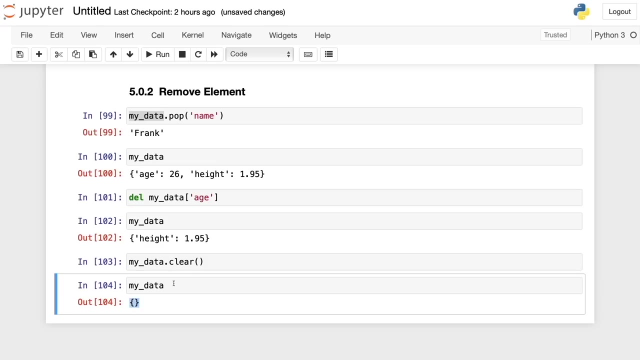 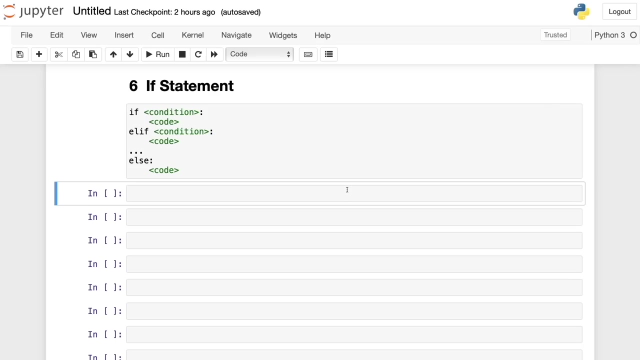 dictionary with a clear method. So we write my underscore data and use that clear with parentheses, And now, if we print this dictionary, you can see that this is an empty dictionary because we remove all the elements from this dictionary. Now let's see one of the most common statements used in Python. This is the state statement. 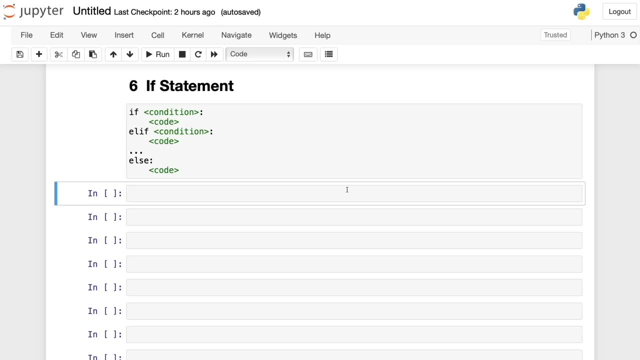 that if statement is a conditional statement used to decide whether a certain statement or block of statements will be executed or not. Here you can see the syntax of this alpha statement And, as you can see, it starts with the if keyword, followed by the condition. 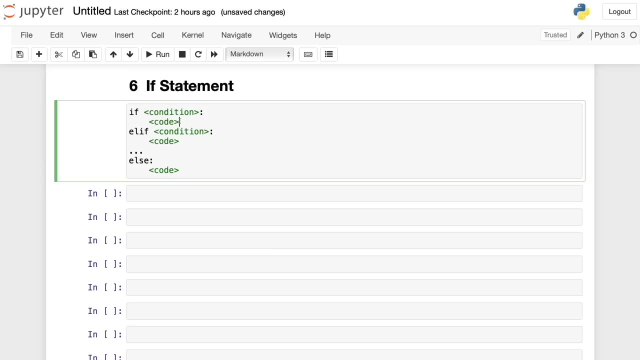 So if the condition is true, this could have Hoppack. Now you don't have to get rid of this block. statement code here is going to be executed, And if the condition is not true, so it's false, the code here in the LF it's going to be tested. So here in this LF block, this new condition will be tested. 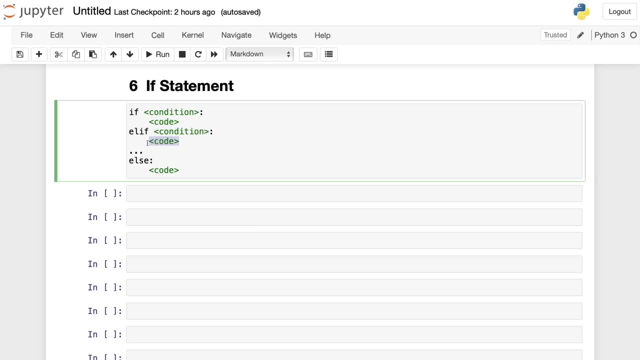 And if this is true, this code below will be executed. But if it's not true, then the else block will be tested, And here this is the last block, and automatically this code will be executed. So here, one little detail that most beginners forget to write is the column. So it's sometimes. 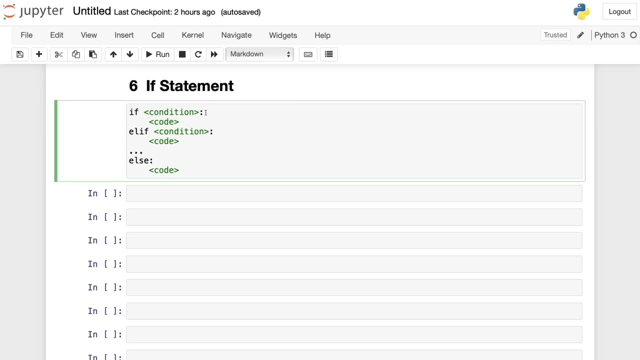 easy to forget. it's there, but you have to include it. And one other things some people miss is this indentation. So here there is an indentation You have to include after the column. So every time you're right here, colon, you press Enter. 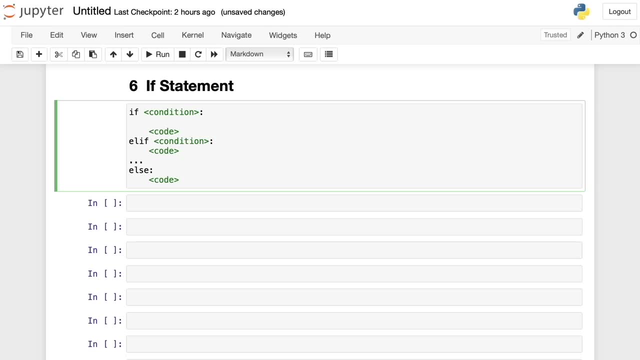 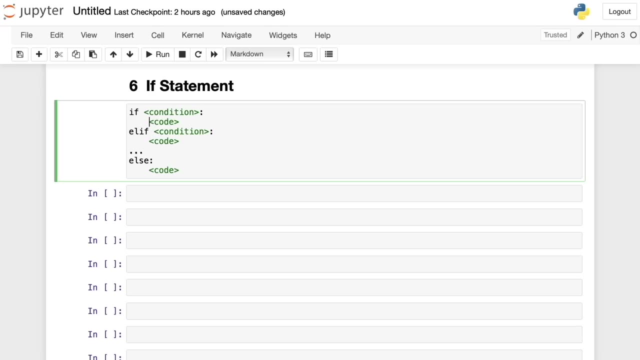 and you automatically in most test editors you're going to get this indentation. But if, for some reason, you don't get that indentation and you get something like this, you can indent this line by using that tab key in your keyboard. So just press Tab And 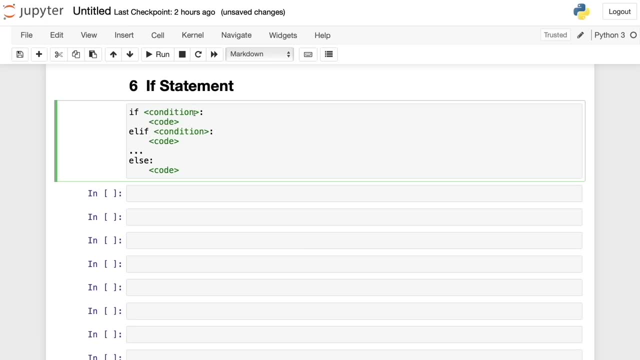 it's going to indent this line. So make sure you write that column and you include an indentation for each code that will be executed. So here, here and here. So now let's have a look at some examples to see much better how that if statement works. So first I'm going to create a new. 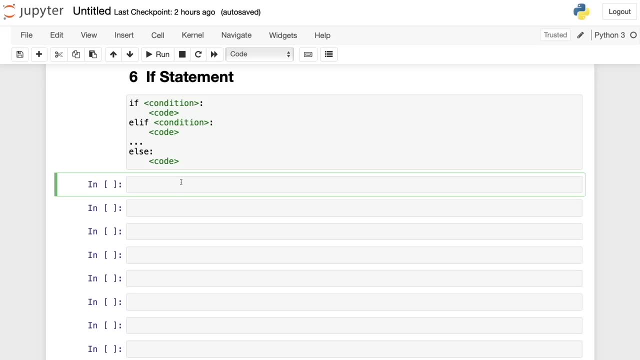 variable And, as you might remember, to create a variable, you have to write a name of this variable. In this case, I'm going to set it as an age, And then you have to set it a value. So in this case, this is going. 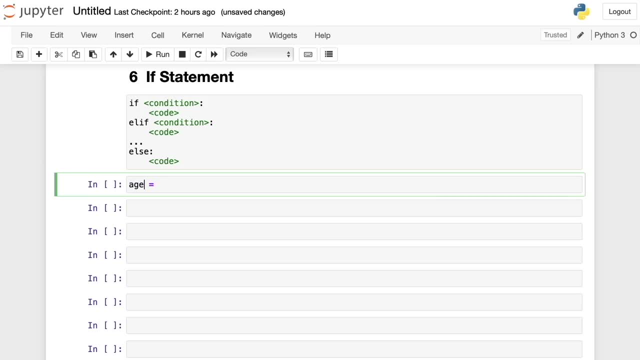 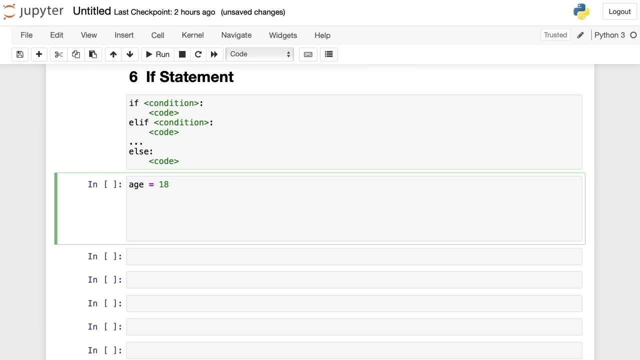 to be a number. So I'm going to set this age to the number 18.. And now I'm going to write this if condition or if statement. so I write: if H is greater than or equal to 18, then column, and then 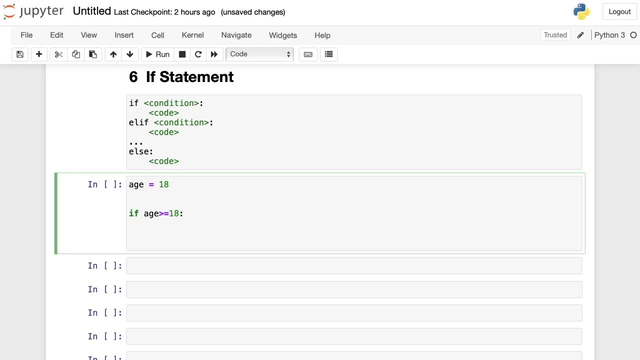 this code is going to be executed. If this is true, I'm going to write print and then a message. So if this person or if the age is equal or greater than 18, I'm going to write the message: you're an adult And, as you can see, here I'm using single. 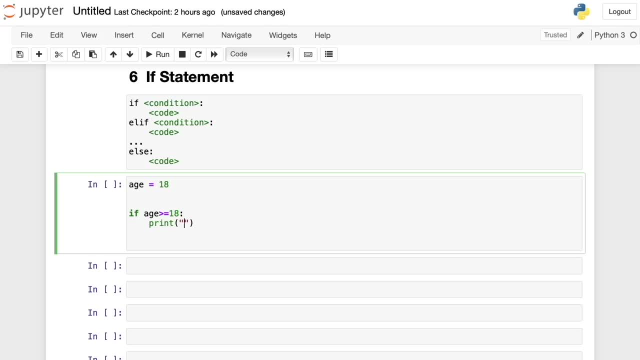 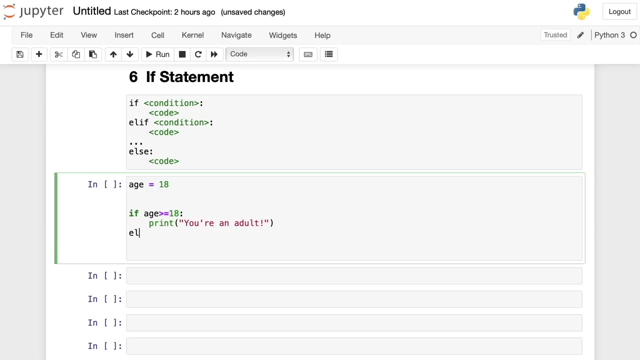 quotes and I wrote the apostrophe, So I'm going to use double quotes. and everything is fine now. So here, print then the message: you're an adult. So if this isn't true, I write else and then column and print here a new. 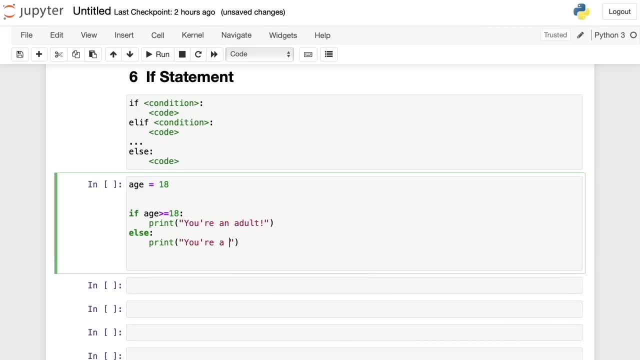 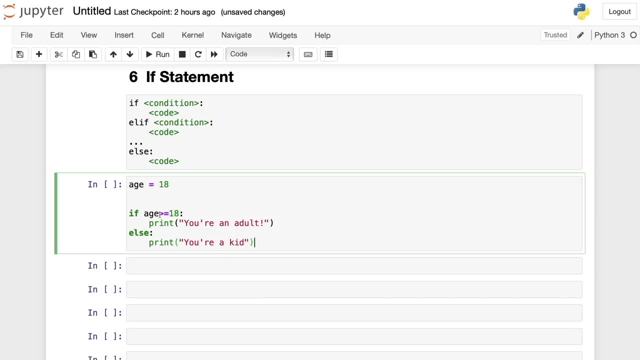 message, which is: you are a kid. So let's see this again. So if the age is equal or greater than 18, then we print you're an adult, but if it's less than 18, we print you're a kid. So here we run this code and we should get this, because 18 is equal to 18.. 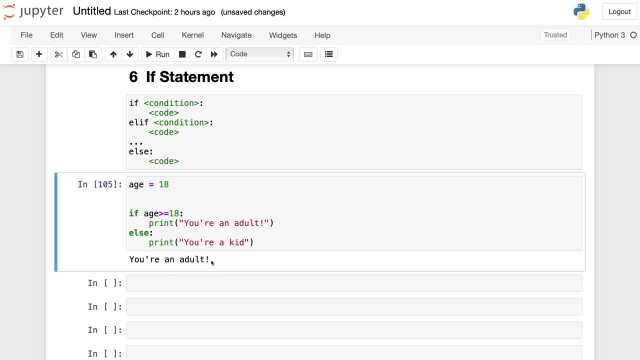 So let's run And, as you can see, we get the message: you are an adult. So now we can play with this. we can change the age value. So here I'm going to set it to 15.. So I run and, as you can see, here 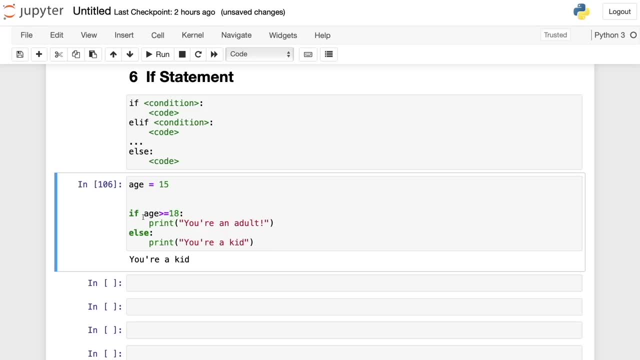 15 is less than 18.. So this is false And this code is executed. So this block here it's going to be executed. So we got- you are a kid, So we can try this one more time. So in this: 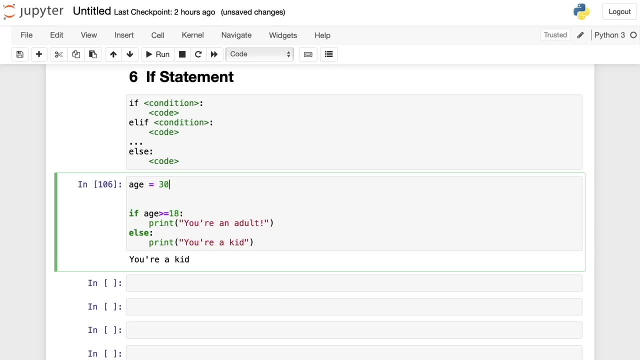 case, I'm going to write another age, So 30. And again, 30 is greater than 18.. So this is executed. So you're an adult. So now let's add a new block, And I'm going to add a new block, And I'm going to. 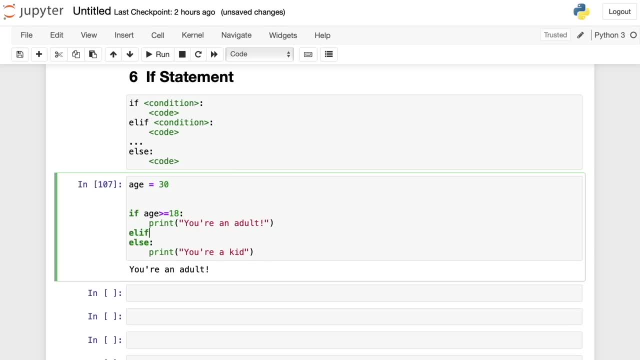 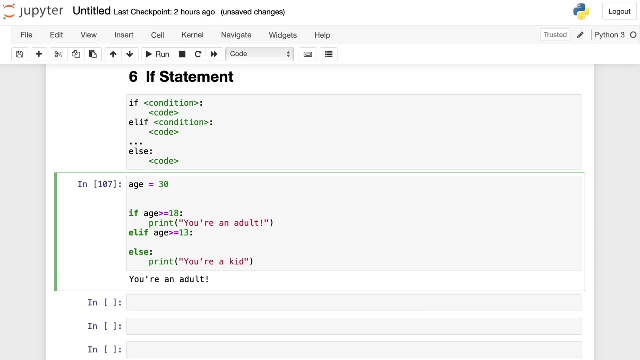 use that elif. So I write elif and then age and then greater than, let's say, 13. And then column press Enter and we got this indentation And then we print another message. So if the age is equal to or greater than 13,, we write the message: you are a teenage. 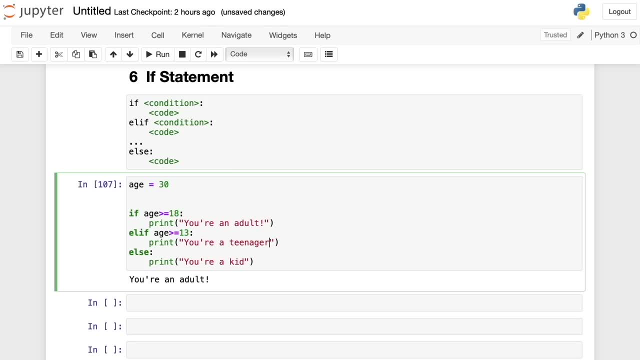 So teenager. So if it's between 13 and 17,- or well, less than 18,, it's going to be you're a teenager, But if it's less than 13, it's going to be your kid. So let's try this out. So I write. 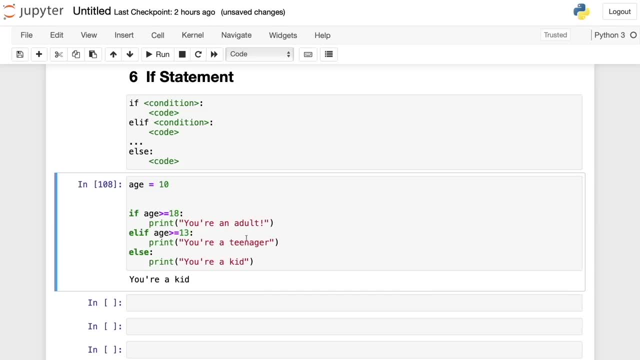 first 10.. And then we get your kid, because it's less than 13.. Then we're going to change this to 14.. And then we get your teenager, because 14 is greater than 13.. And finally we write 20.. And we get your an adult, because 20 is greater than 18.. And that's it. 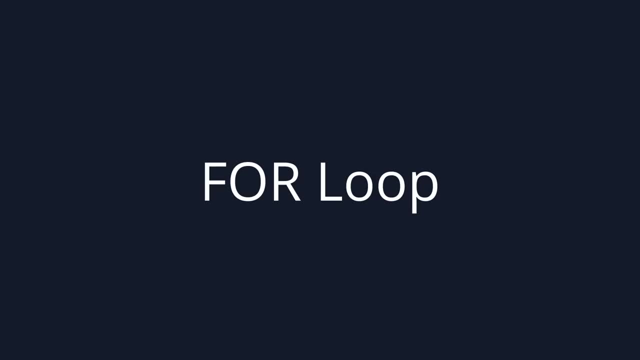 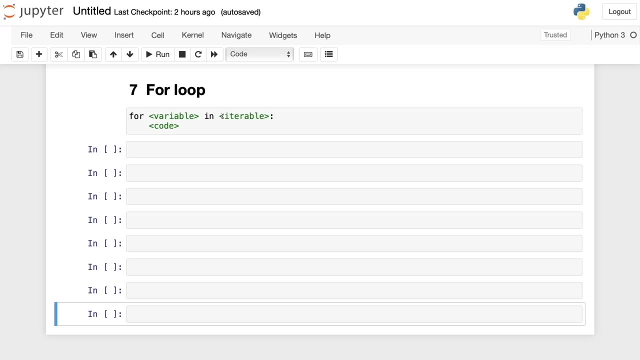 That's how the if statement works. Now it's time to see one of the most common loops in Python. This is the for loop. For loops are used to loop through an iterable object and performs the same action for each entry. One example of an iterable object is a list, So we can loop through each element of a list. 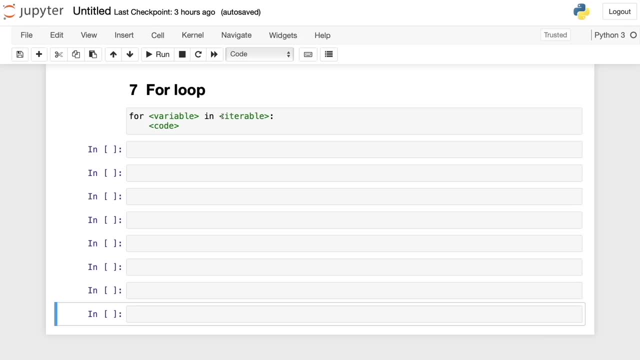 and perform the same action on each element of that list. Here you can see the syntax of the for loop And, as you can see, here is the for keyword. and then we have to use a variable, then we have to write that in key. And then we have to use a variable, And then we have to write that in key. 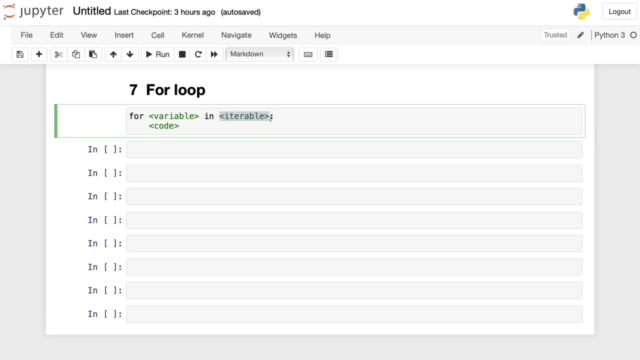 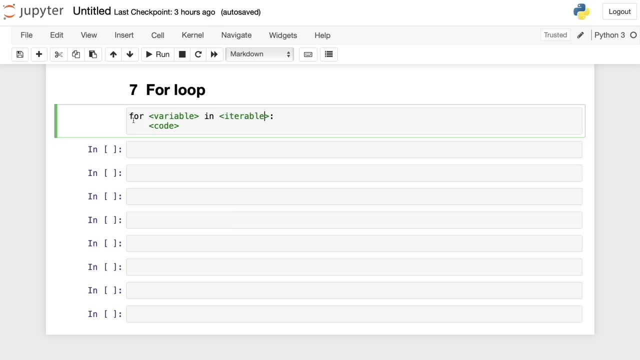 most common is the list. So you have four variable in list. I'm going to write here list so you can see much better. And then we have to write a column And then after a column it goes an indentation. So here we have the indentation and the code that will be executed for each iteration here that we 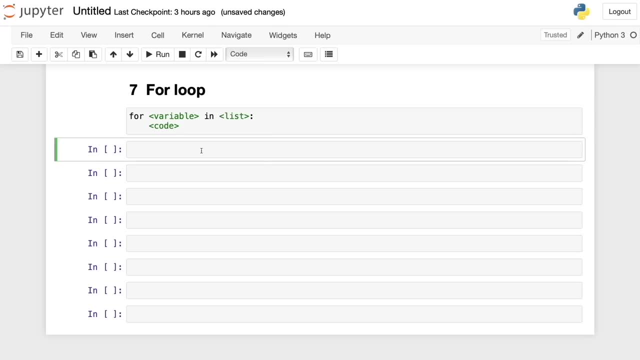 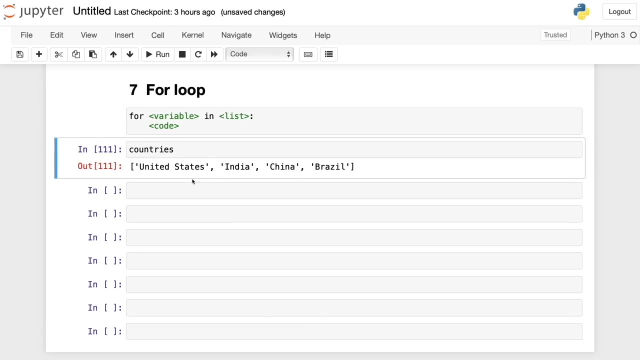 make with the for loop loop. So to see this much better, I'm going to use that countries list we created before. So this is the countries list And I'm going to loop through this list. So I write four and then we have to set a variable that is going to be just just temporarily, So this: 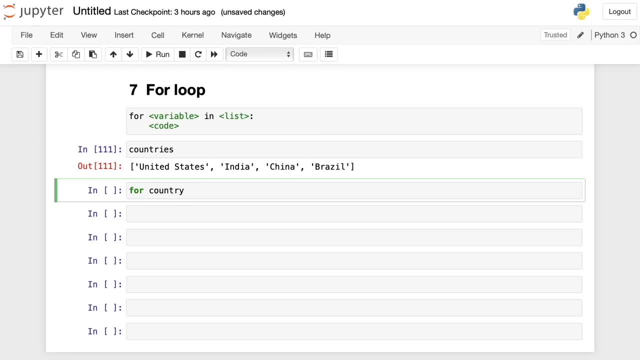 variable is going to be called country. So this variable doesn't exist. we just created temporarily. So for country in, and then we have to write the name of that iterable, which is, in this case, a list. So countries. So for country in countries, and then column. 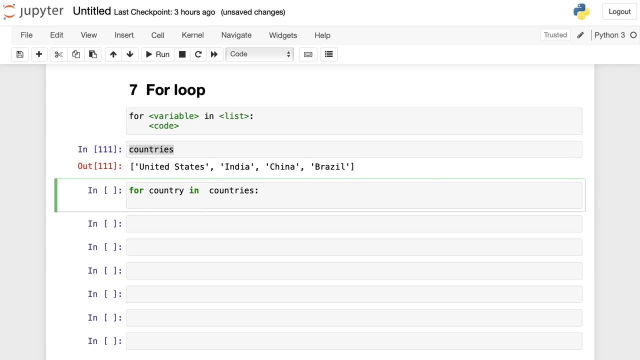 and then enter and we get this indentation. then we say print country. So for this variable in this iterable, which is a list, print each element. This is what we're saying in this for loop. So we run this as you can see each element. 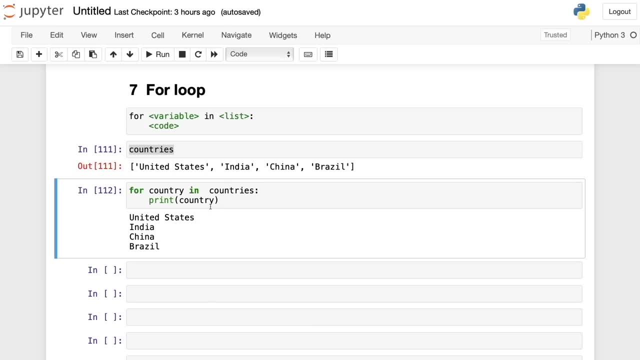 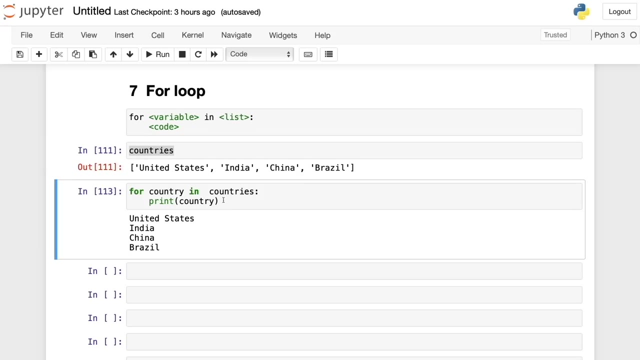 of the list country is printed. So we're looking through the countries list and printing each element. So the first is United States, then India, then China and Brazil, And this is how the for loop works. Now let me show you a new function that you can implement along. 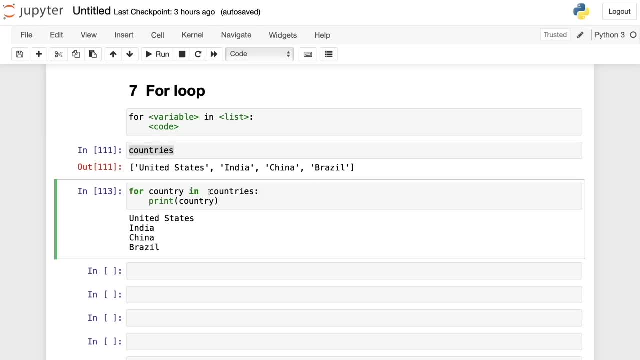 with the for loop And it's called enumerate. So I'm going to write here: enumerate. In here I'm going to put this countries list inside this new function. So what this enumerate function does is to enumerate each element of the countries list as we look through the list. So I'm going to add here a new variable. 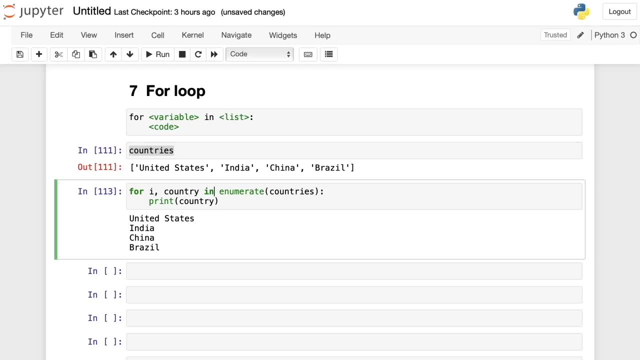 and it's going to be. I, then comma and then country. So this enumerate will return two elements. the first one is going to be the number of the loop And the second one is going to be the element itself. So here I have to print, apart from the country, the 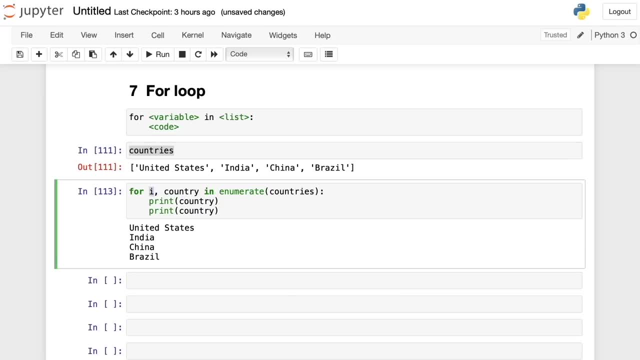 I variable that I just created here or it's just temporarily here. So right, print I and then print country. So here we're going to print here that number of that iteration and that element. So I run Ctrl Enter and here we got it. So first is the United States in that iteration. 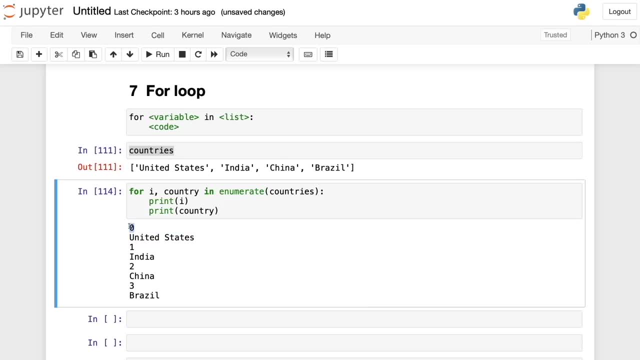 the first iteration, with each, which is zero, then we got India in the second iteration, which has one, and so on. So, as you can see, here the eye starts with the zero. So this is how enumerate works: It starts with the number zero and it returns the number of the loop and that. 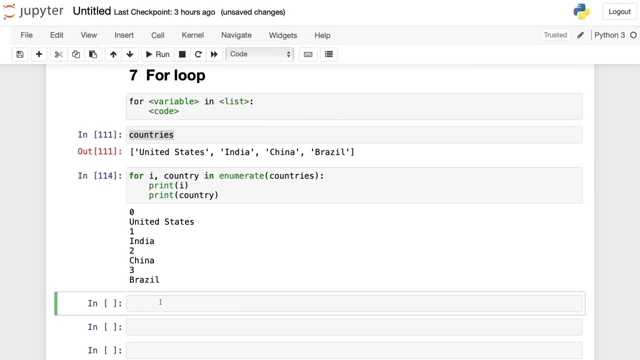 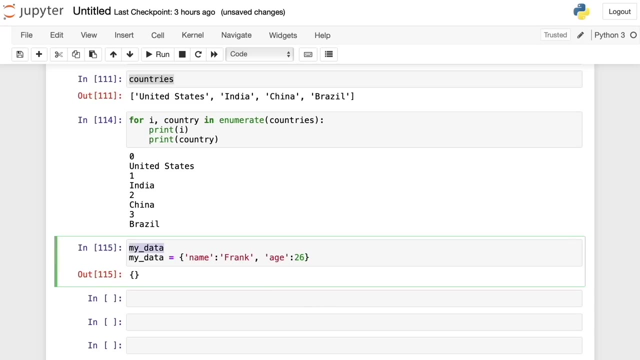 element And finally, let's loop through elements in a dictionary. So let's use that dictionary we created before. that was my underscore data. Well, this is empty, So I'm gonna use the original dictionary. So here I have the original dictionary and it's here, so I'm just going to print it. So 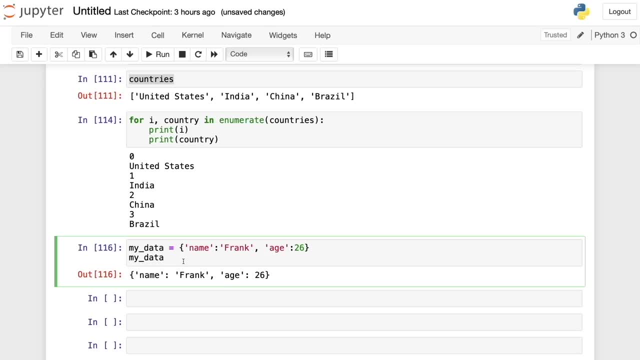 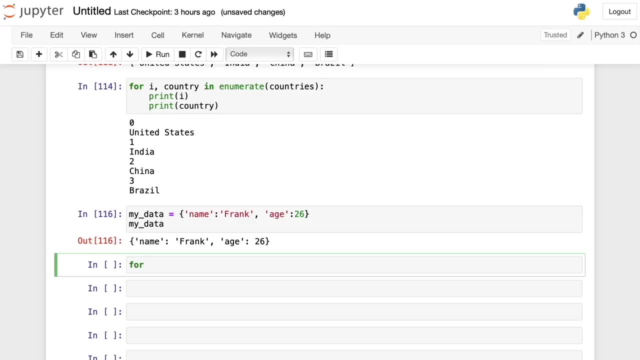 this is the original dictionary and it's here, So I'm just going to print it. So this is the a dictionary, And now we're going to loop through this dictionary. So let me show you here. First we have to write four, And then we write key and value, because one item, as you might remember, 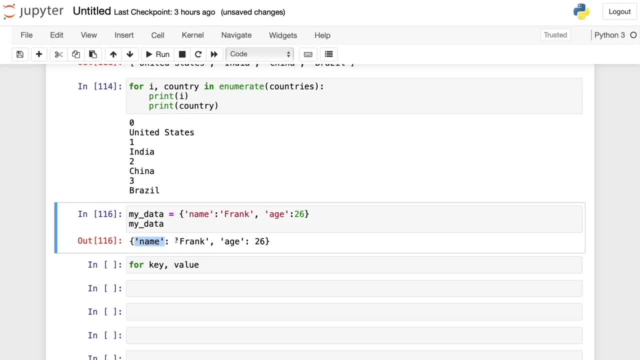 is made of a key and the value. So key and value, So we say for key, comma, value in and then the name of the dictionary. So right, my underscore data. And now to get the items of this dictionary we have to use the items method. So we write that items and then parentheses, then we 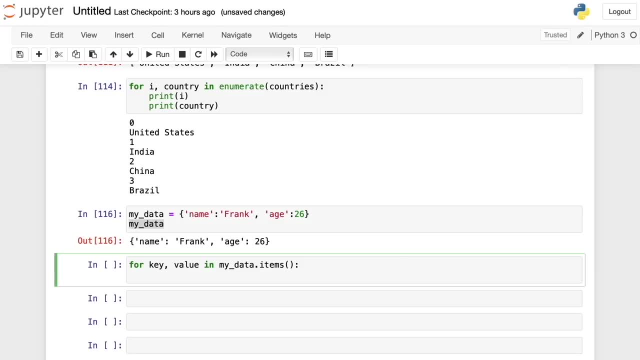 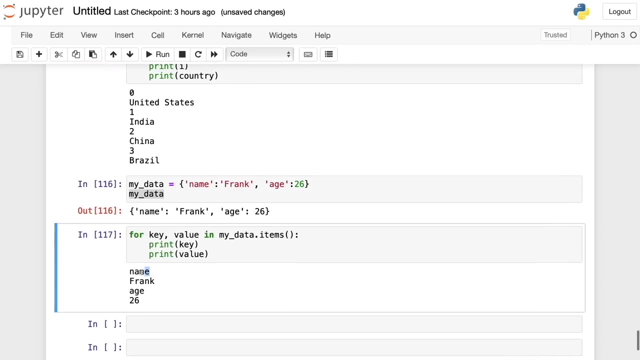 write column and we press Enter, So here we can print the key And we can also print the value. So key and value. And then we run this code And, as you can see, here we get the key, the first key. 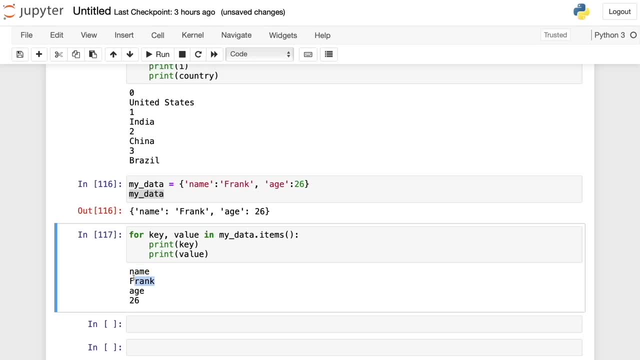 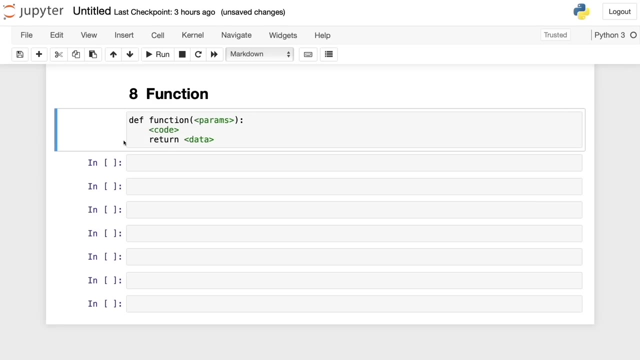 and we get the value, we get name, and we get Frank and then the second key, age and age 26.. So this is how you look through elements or items inside a dictionary. Okay, now let's see how functions work in Python. A function is a block of code which only runs. 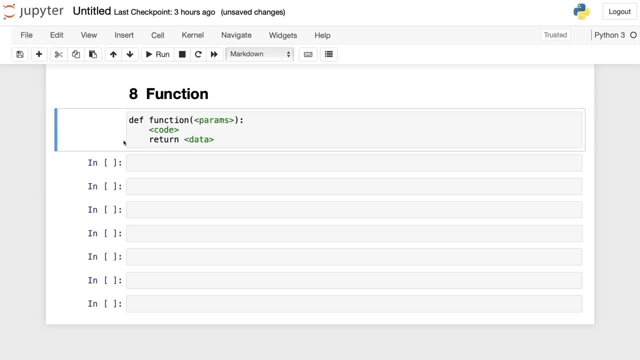 when it is called. So in Python, you have to use the function. So in Python you can pass data known as parameters into a function. So here is the syntax of a function And, as you can see here we have first to set the keyword def to create this function, And then we have to write the name of this. 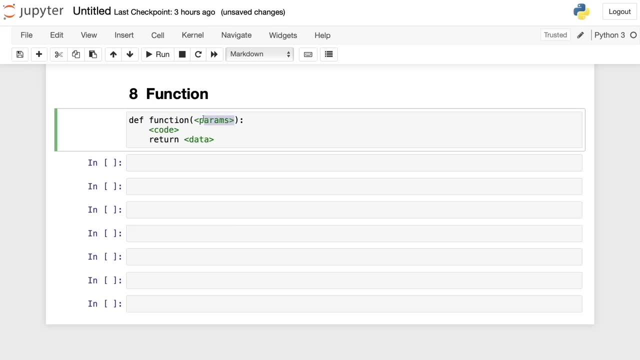 function And inside parentheses we define the parameters of the function that we're creating. then we write column and below you have to write the code And every function should return some something. So we have to use the return keyword and then return something like a variable. 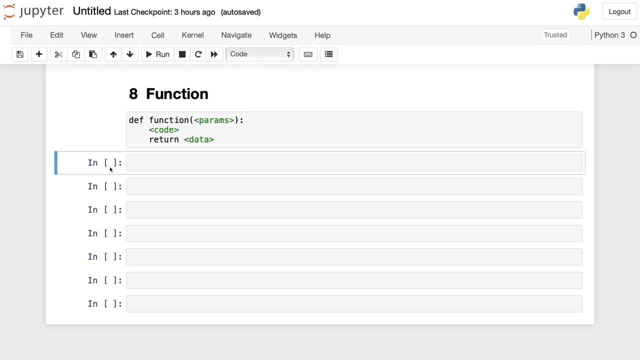 for example. So now let's create a basic function. So first we write def and then we write the name of the function. So this function is going to do something really simple: it's going to sum the values we pass into it. So it's going to be named sum underscore values. 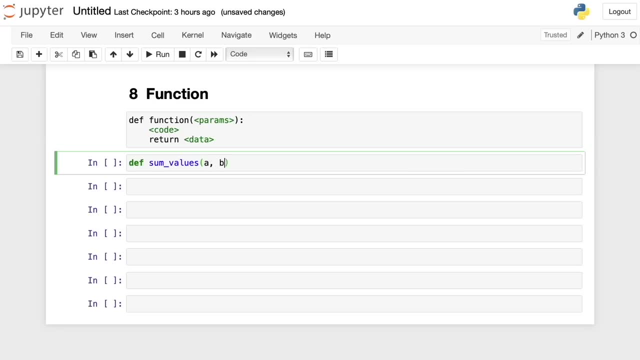 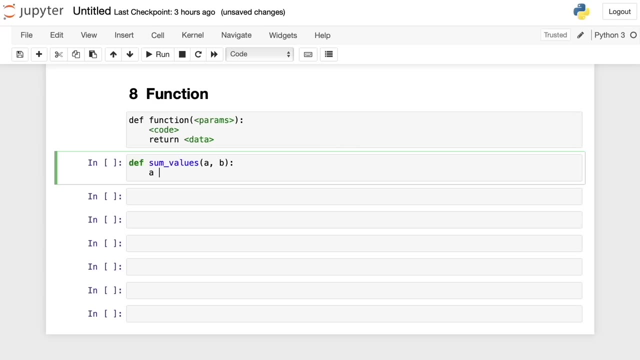 And as parameters we set a comma B, then colon and press Enter. Then what this function is going to do is to add the A plus B values And we're going to set this equal to x. So we write x equal to A plus B And, as I told you before, you should return something after. 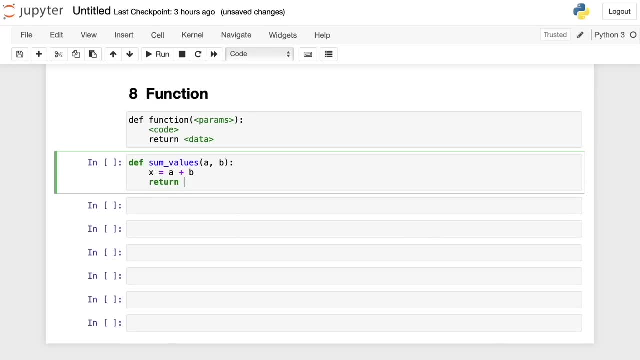 we finish the function, So we write return, And here we're going to return the x variable. So right, x, And that's it. That's how you create a function. I ran this code And, as you can see, apparently nothing happens. but this function was created, So to use this function. 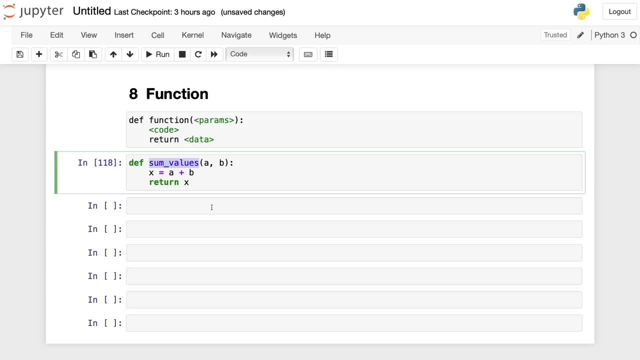 we have to call it. So to call this function, we have to write the name of the function And then we pass some parameters in. In this case it's called arguments when you call the function. So I'm going to write the. 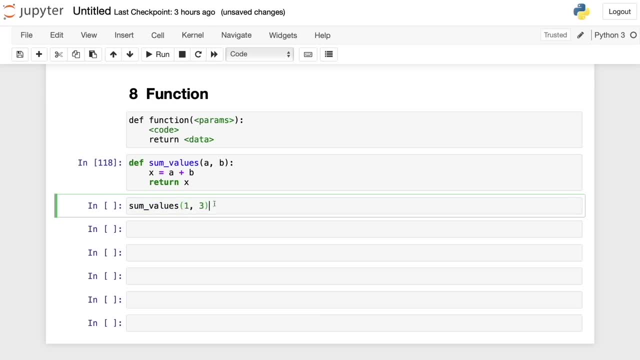 argument one and argument free. So once you call this function is going to go to the function here in is going to set this one equal to a and this three equal to B. So you have one plus three and this is four. So x is going to be equal to four, And then this function is going. 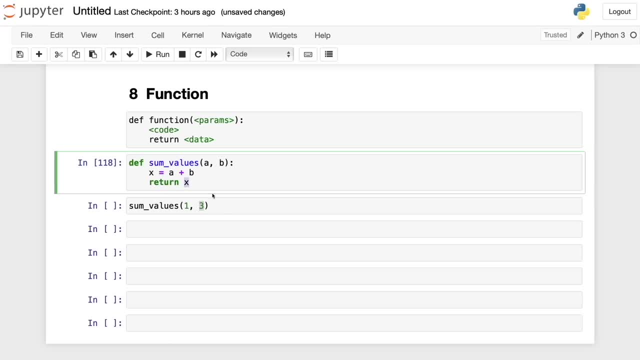 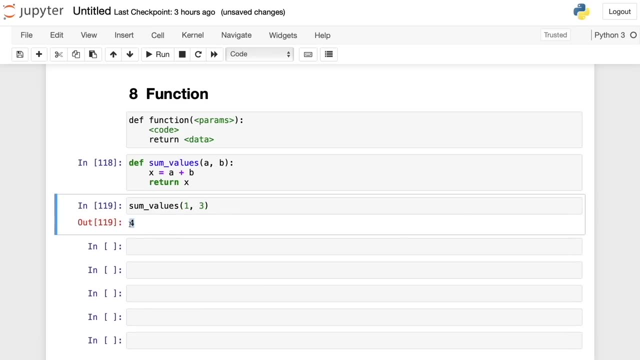 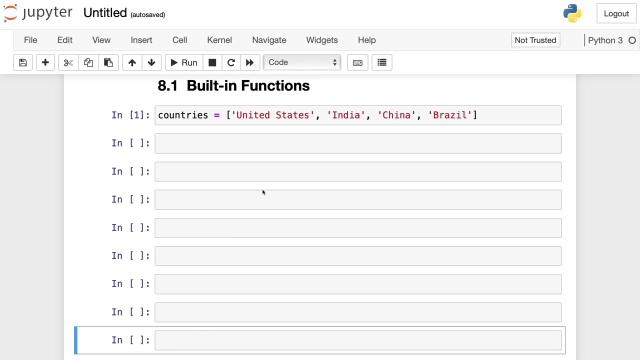 to return the value of x, which is four. So this is supposed to return the value Now of four. So we run this and we got a value of four. So this function is working properly. Okay, now let's see some built in functions that Python has. Python has lots of built in functions that. 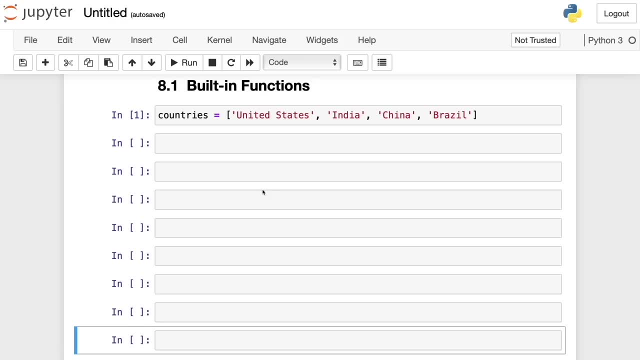 can help us perform a specific task. Let's have a look at some of them. So let's start with the land function. we only have to write the word land And then we open parentheses And, as you can see here, Jupyter Notebook gives the green color to functions. And now let's calculate the. 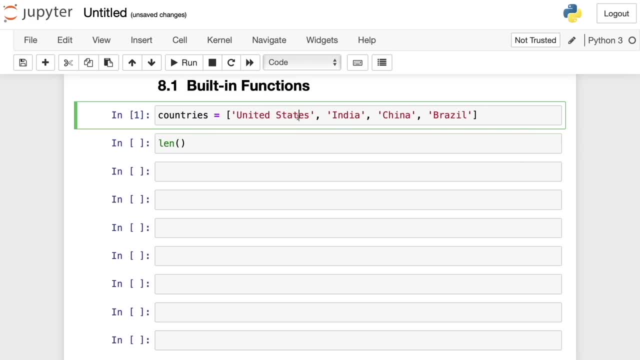 length of the countries list. So I have here the countries list, And now I'm going to copy this one, paste it inside parentheses, And what the land function is going to do is to calculate the length of any iterable object, In this case the country. 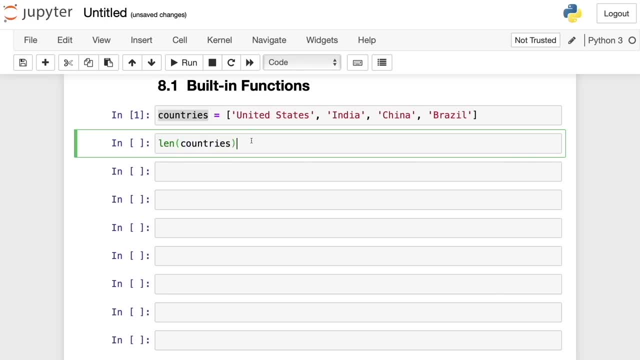 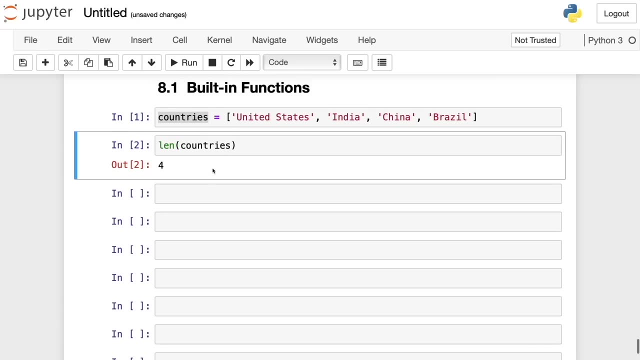 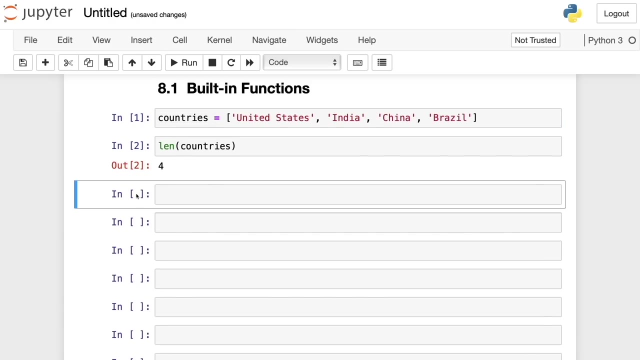 this list is an iterable object And now I'm going to run to calculate the length of this object. So I run this one And, as you can see here, the length is four. And this is how the land function works. Now let's see a different function. In this case I'm going to create a 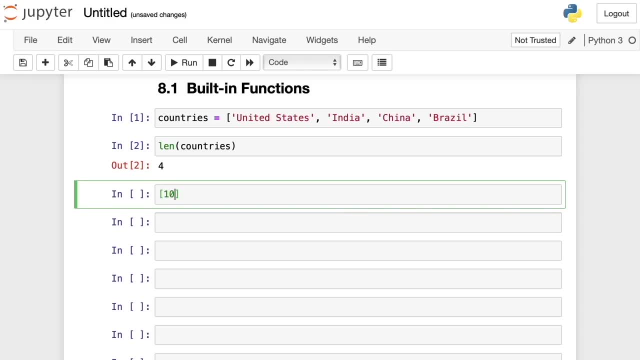 new list that contains only numbers, So I'm going to write random numbers here: 10, 6381, then 99.. So this is my new list And I created this list with only numbers to try the max and min function. So the max function is this one. we write max and then parentheses, And this one. 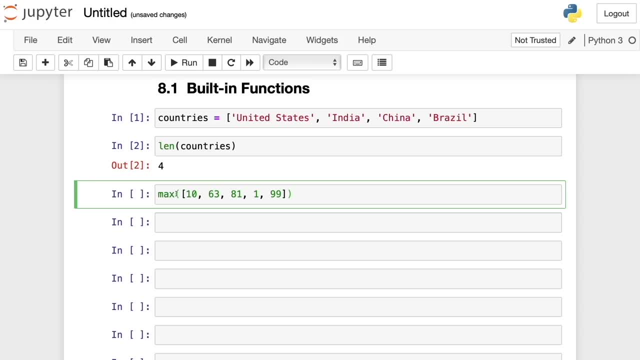 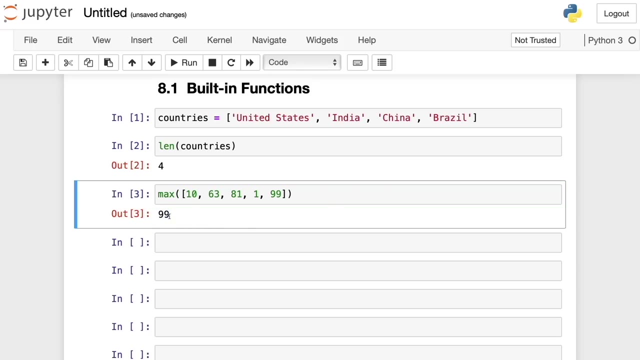 returns the item with the highest value in an iterable. So my iterable is this list and we're going to get the highest value of the elements inside this list. So we're this one And as you can see here the maximum value is 99. And we can do also the mean function. 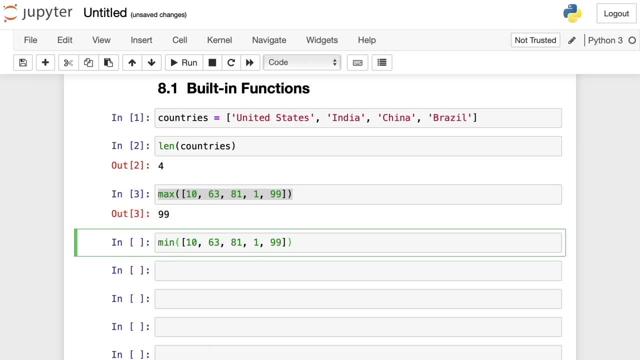 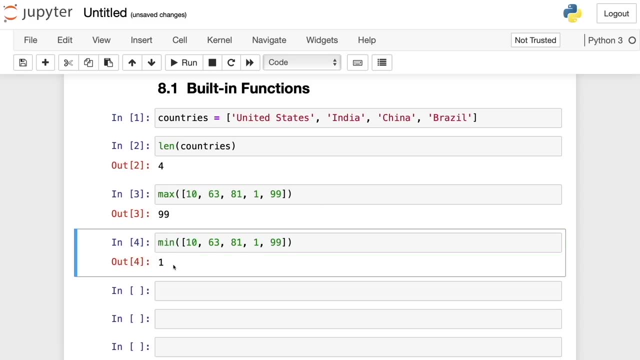 and it's going to have the opposite effect. In this case, we're going to get the minimum value of this list. So we run and we get one. Okay, another common function used in Python is the type function, And this function give us the type of the object. we only have to write type. 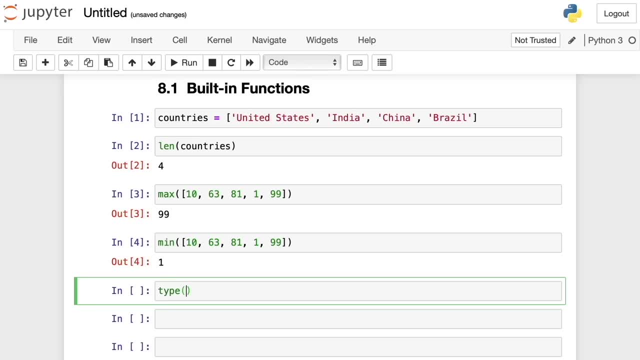 And what this function does is to return the type of an object. So in this case, let's copy and paste the countries object And if we run this, we can see that this object is a list, And that's correct, because here we created a list with square brackets. So that's what the type function does. 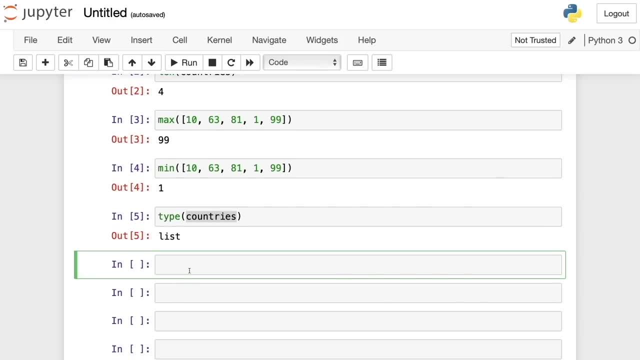 And finally, the last function we're going to see is the range function. This one returns a sequence of numbers that start with a number and ends with another number. So let's see how it works here. So this one has three arguments. First, the start number. 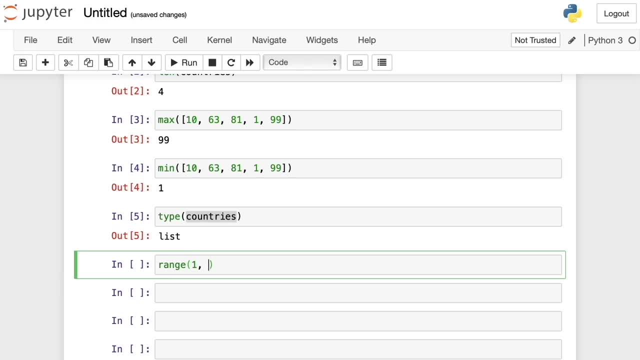 This one, I'm going to write one. then the number where the sequence stops. In this case, I'm going to write: write, let's say 10.. And then the last argument is the increment. So how that this sequence is going to grow by how much. so, in this case, I'm going to say that this sequence is going. 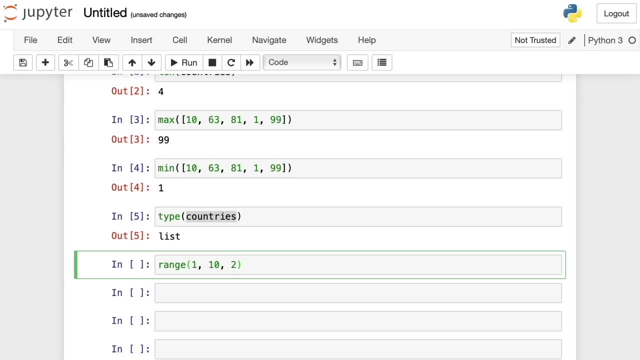 to grow by two. So right to know I run in. as you can see, nothing happens. we only get the same text here. But if we make a loop here, so I write for I in wrench now print this I. So these are for loop. we saw this before And here we run And, as you can see, 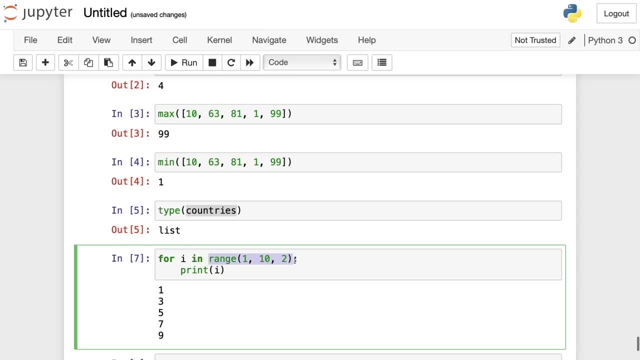 here we're iterating over this wrench and we're getting the elements inside this wrench. So the first element is one, the second is incremented by two. So one plus two is three, then three plus two, five, then seven and then nine. And 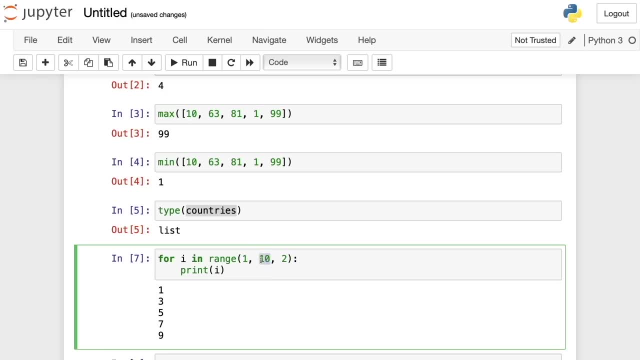 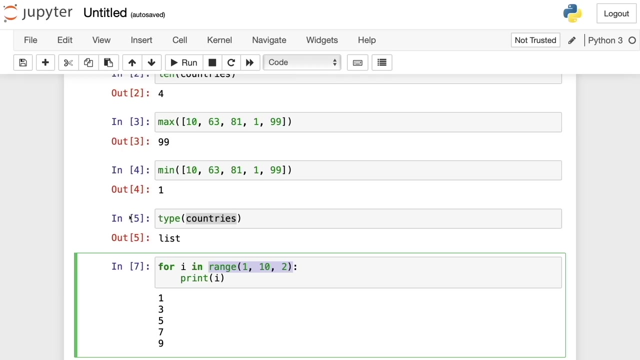 then we should get 11.. But the last element here, it's 10.. So this sequence stops at 10.. So we only get until number nine, And that's how the range function works in Python. And that's it Now. you know the most common built in functions in Python. 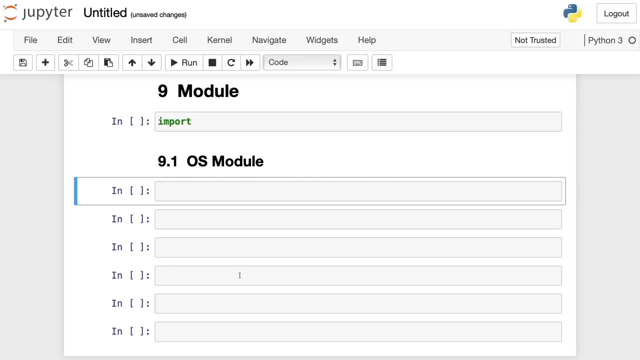 Okay, in this video we're going to see what are modules in Python. In Python, modules are files that contain Python code. a module can have classes, functions and variables and even runnable code, And to get access to a module we have to use the import keyword. 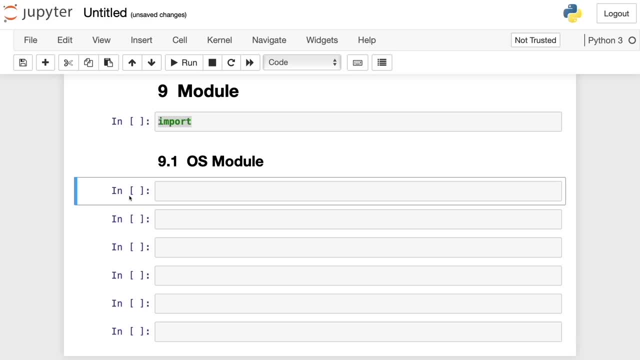 this one And to see a module in action. we're going to see the OS module And this one comes with Python, So you don't need to install it. So to get access to this OS module, we have to write import OS And that's it. 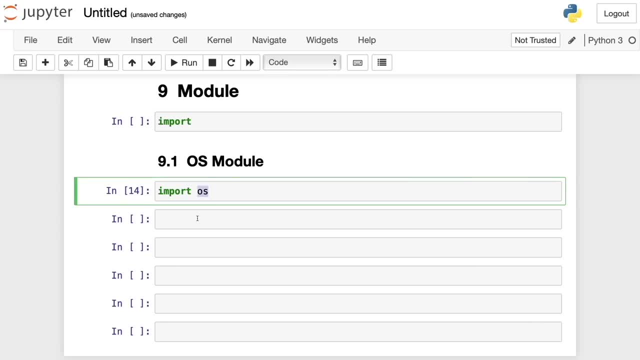 we only write this, And now let's see some functionalities of this module. So the first one that we're going to see is the get current directory method. So to get access to that method, we write OS, then get C, W, D and then parentheses. 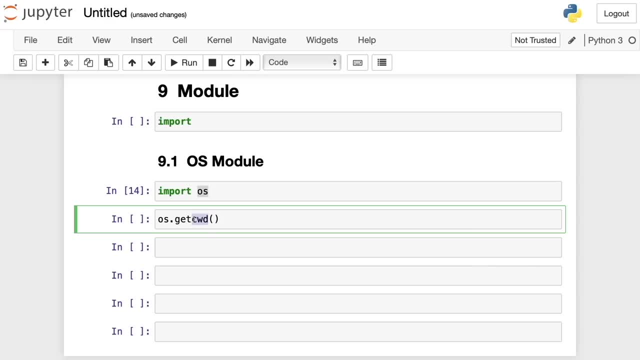 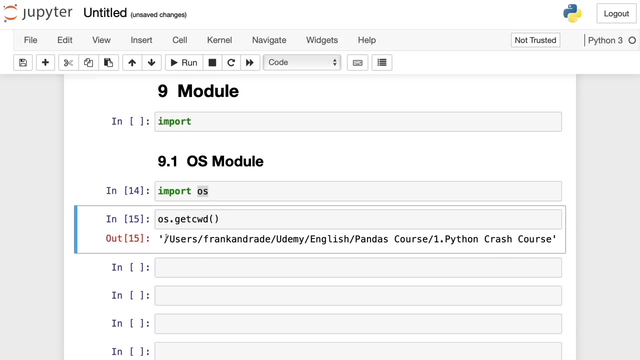 So this CWD stands for current working directory, So we're going to get the directory where our Jupyter Notebook file is located. So this file I'm working with right now. So let's run and let's see what happens. So, as you can see, here I have the path where the Jupyter 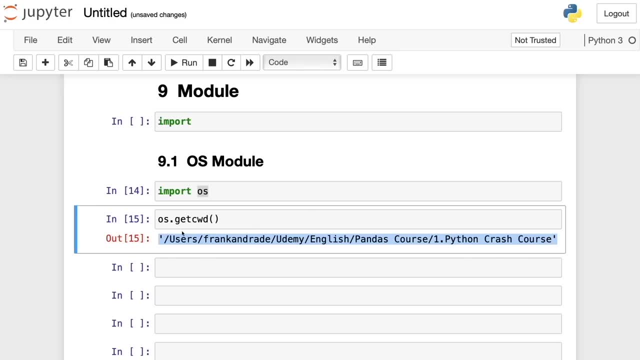 Notebook is located. So this is the complete path, And you can see it by using the get CWD method. So now let's see another method, And in this case we're going to list all the elements in the folder where this Jupyter Notebook file is located. So here to do that we're. 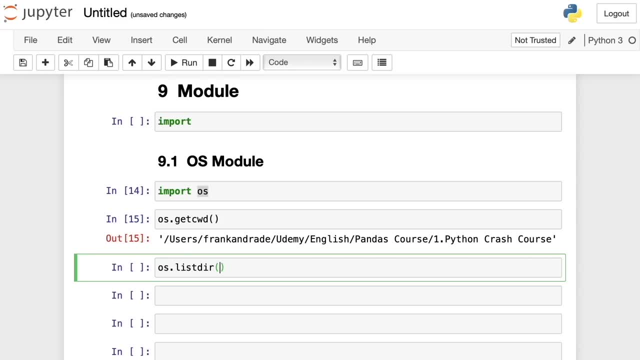 going to use the method list dir. So this means list directory and I'm going to run it And, as you can see here, I have this Jupyter Notebook file that is named untitled. As you can see here, the name of my file is untitled And these other elements you can ignore it. they are not files. they 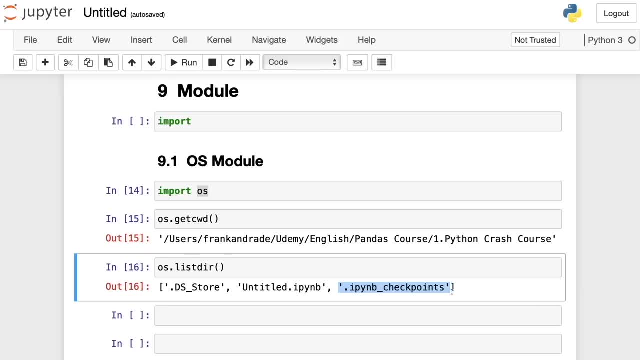 are just some hidden elements in my folder, but they don't matter. So right now the only file I have in this folder is this untitled file. So this is what that list dir does. So it lists all the elements in the folder where this Jupyter Notebook file is located. 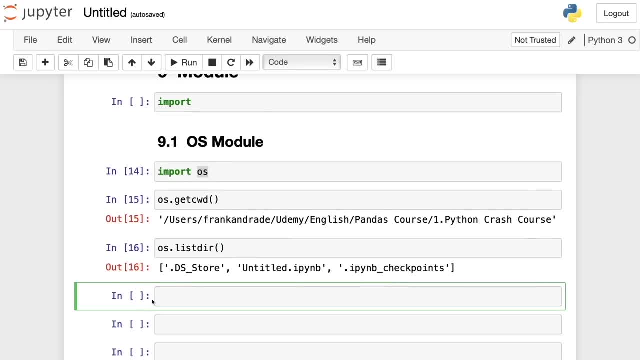 And now let's see how it works. So let's go ahead and run this Jupyter Notebook file. Let's see the last method, which help us create a new folder. So this method is called make dirs And we have to write OS that make dirs and then parentheses and inside parentheses. 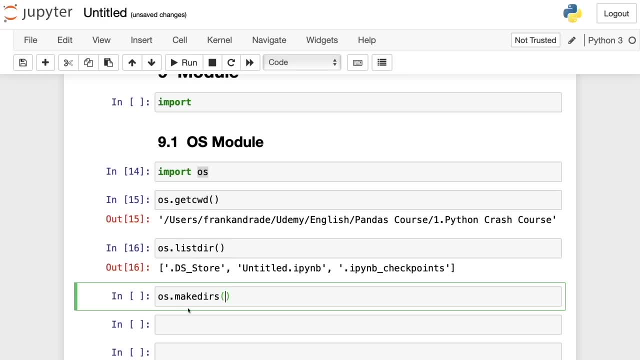 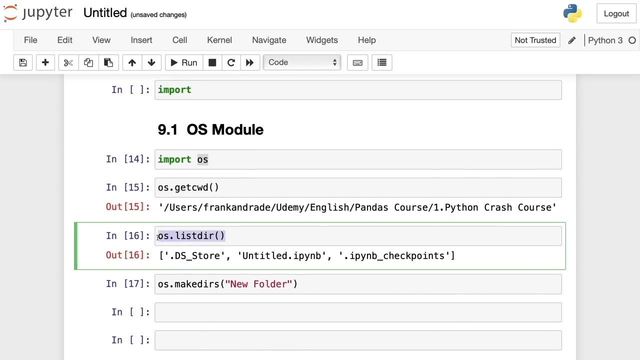 we have to write the name of the folder we want to create. So in this case, I'm going to name it new folder, simple as that. And now, if we run, we're going to see that nothing happens. But now, if we use this list dir method to list all the elements in my folder, we can. 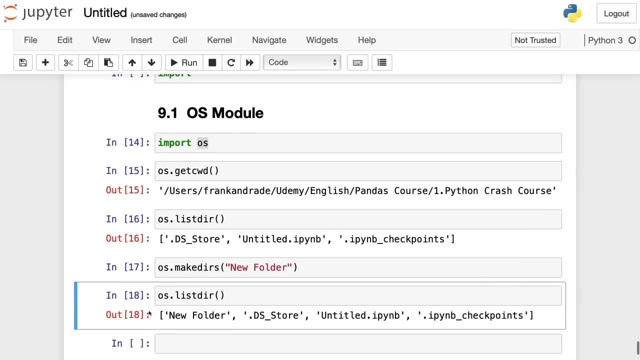 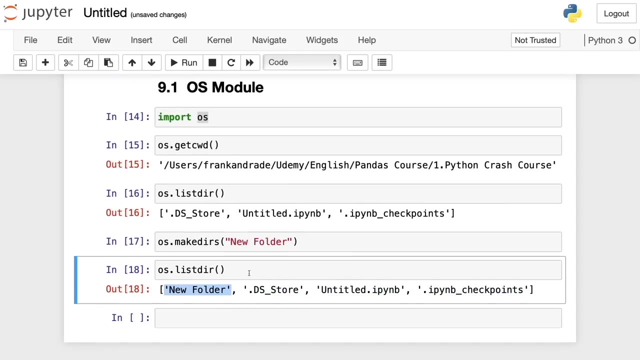 see that there is a new folder. So here, if we compare this result we got before with this new result, we can see that there is one new element, And this element is that new folder element which is the folder we created using the make dirs method, And that's. 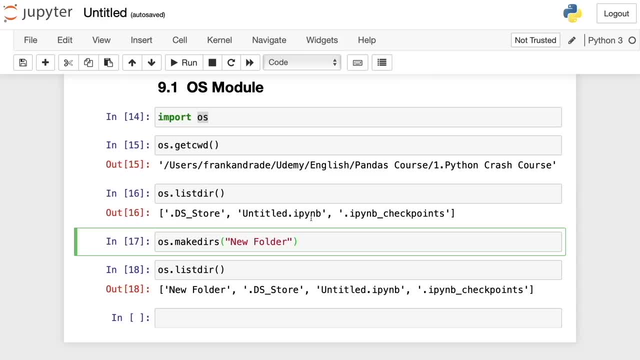 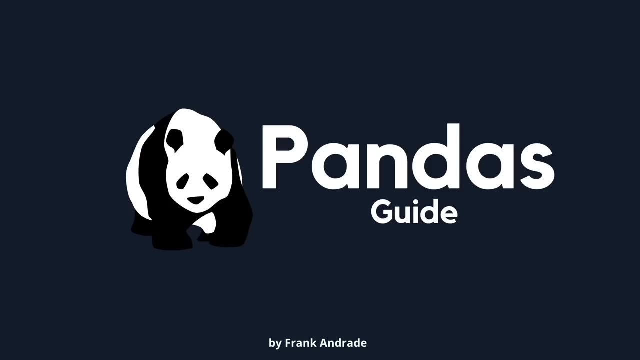 it. So these are some basic things you can do with the OS module. In the following videos we're going to install different libraries, packages and modules so we can do even more things in Python. In this first introduction to pandas, we're going to learn what is pandas. we're going 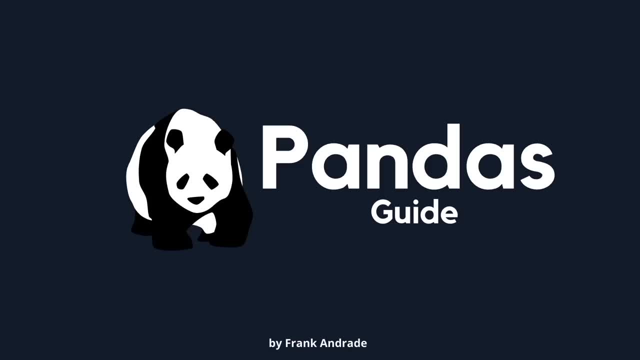 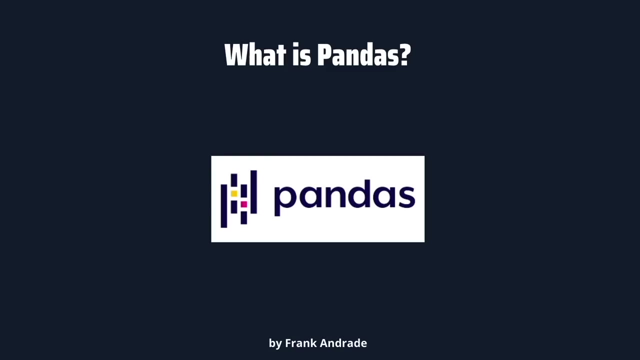 to compare pandas with Excel, And then we're going to learn what are pandas dataframes. So first, pandas is probably the best tool to do real world data analysis in Python. It allows us to clean data, wrangle data, make visualizations and more. You can think of pandas as a supercharged 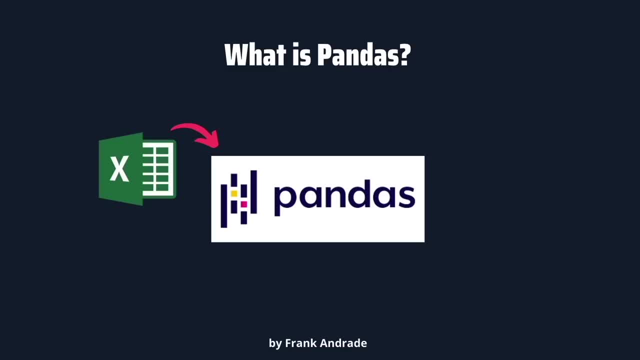 Microsoft Excel, because most of the tasks you can do in Excel, you can also do it in pandas, and vice versa. That said, there are many areas where pandas outperforms Excel. So before you learn pandas, let me show you why you should learn pandas. 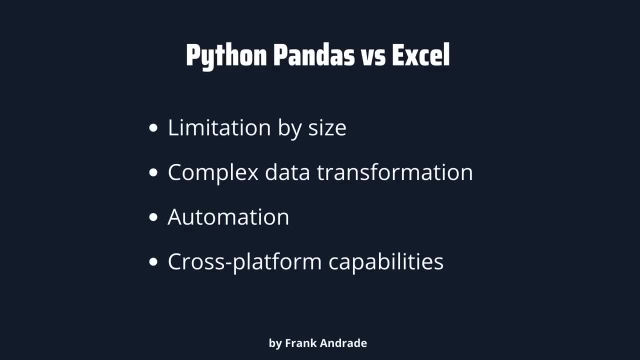 especially if you already know Excel. So there are some benefits that pandas has over Excel or Python has over Excel. So before dedicating time to learning pandas and also Python, let's see what are these benefits. So first, limitation by size. 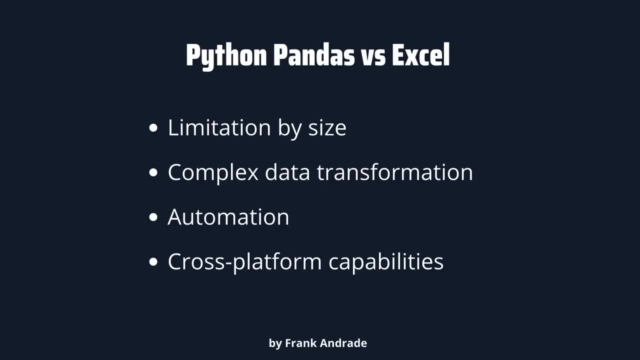 Excel can handle around 1 million rows, while Python can handle millions and millions of rows. Another benefit that Python and pandas have over Excel is that complex data transformation. So in Excel, memory intensive computations can crash a workbook, While in Python when 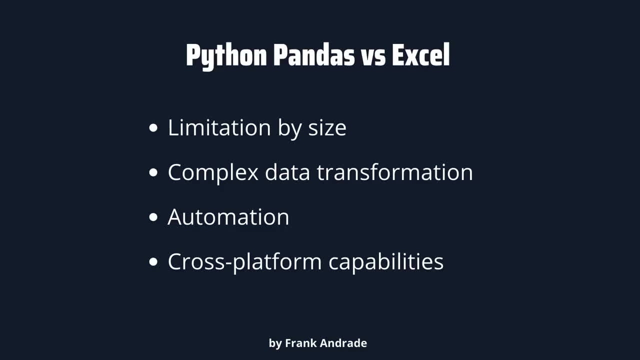 you work with pandas, you can handle complex computations without any major problem. Also, Python is good for automation, While Excel was not designed to automate tasks. you can create a macro or use VBA to simplify some tasks, But that's the limit. However, Python can go beyond that with its hundreds of free libraries available. 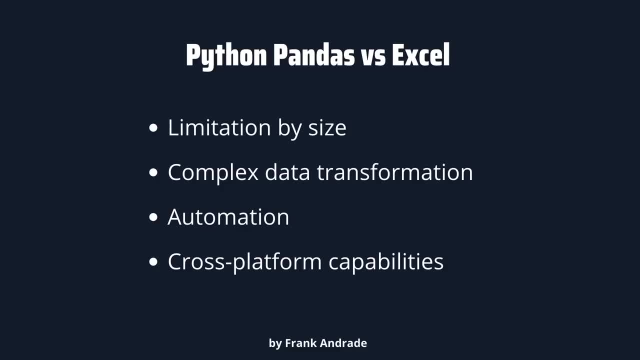 And finally, Python has cross platform capabilities. This means that Python code remains the same, regardless of the open source code. Python has a lot of features that can be used to create a new version of the operating system or language set on your computer. Okay, before. 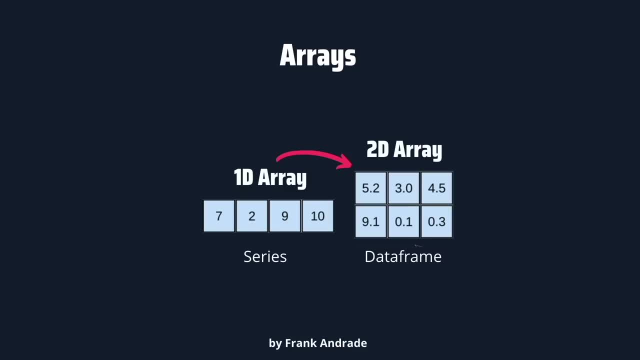 we start writing code. let me explain to you the core concepts of pandas. So we're going to start seeing the concepts of arrays. So arrays in Python are a data structure like lists, So you can find like one dimensional array or two dimensional rate, also known. 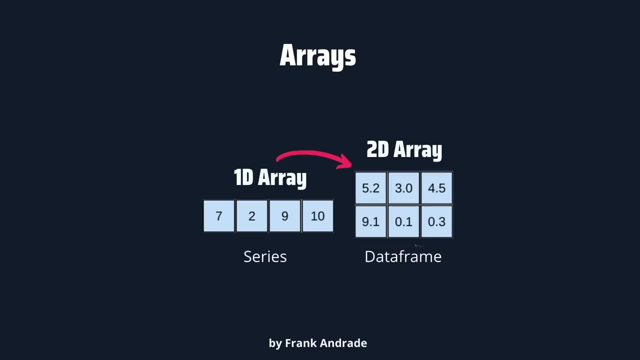 as 2d array, And the two main data structures in pandas are series and data frames, So the first is a one dimensional array while the second, a data frame, is a two dimensional array. In pandas we mainly work with data frames, But if you didn't understand so much the definition of a data frame with 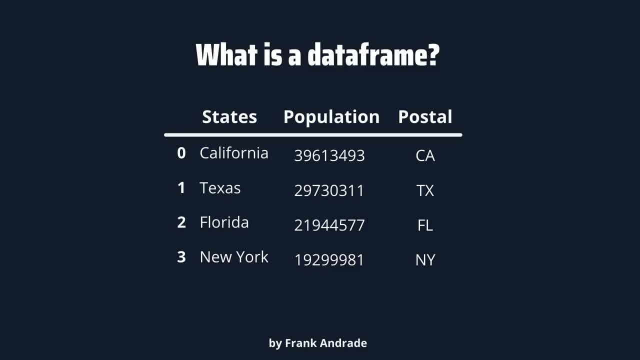 arrays. let me show you another definition, this one using Excel. So it's not even a data framework, it's just a different formula for various data structures. So a pandas data frame is the equivalent of an Excel spreadsheet. pandas data frames. 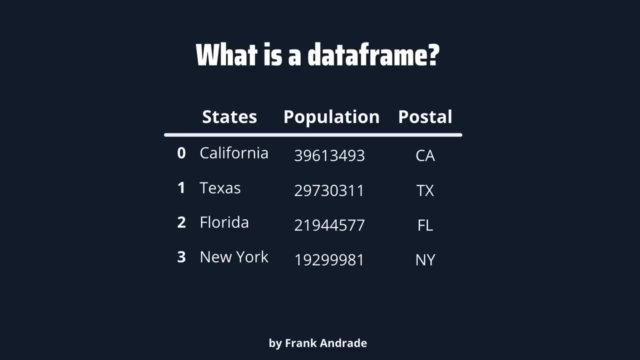 just like Excel spreadsheet, have two dimensions or access. So there are two axis, and one is the row and the other is the column, So the column is also known as series. So what we've seen before, this one dimensional array series, is a column. So what we've seen before is one dimensional array series, is a column in which the column is divided into two dimensions, meaning the Lieutenant column or the Pandas column, And then, of course, we can call this one dimensional array series, which is the connect function. 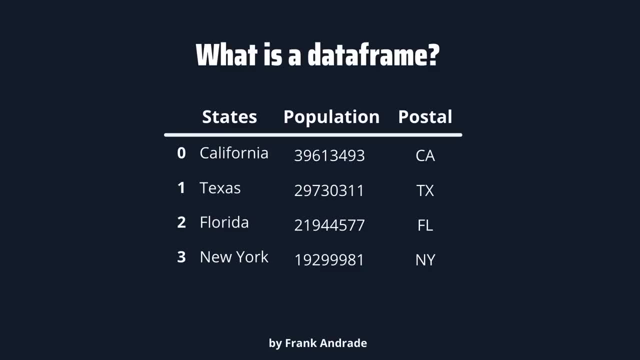 So that's all for this video And if you liked this video, don't forget to subscribe to our channel. this is another name to call the columns in in a pandas data frame. On top of the data frame you will see the name of the columns And on the left side there is that index by default index. 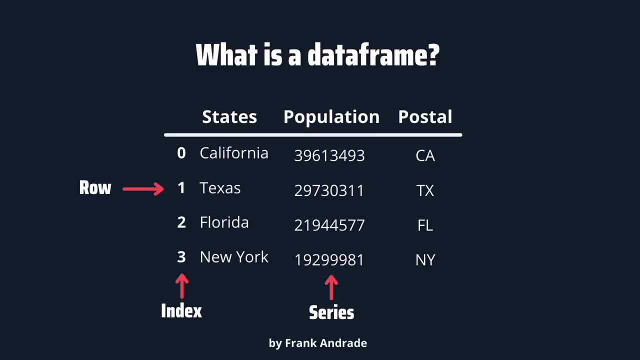 in pandas start with zero. the intersection of a row with column is called a data value or simply data. we can store different types of data, such as integers, strings, Boolean and so on. Right now you see on the screen a data frame that shows the US states ranked by. 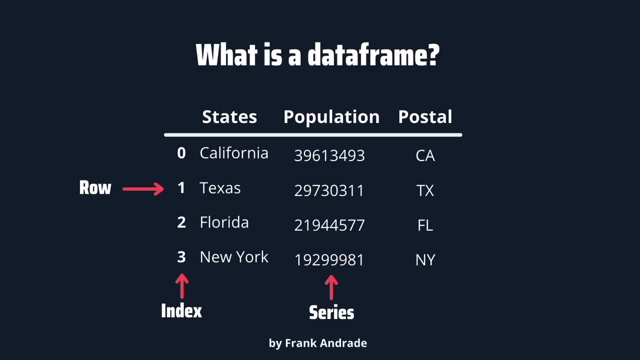 population. I'm going to show you the code to create a data frame like this later, But now let's analyze this data frame. So the column names are also known as features, So our column names are also known as features. So our column names are also known as features. So our 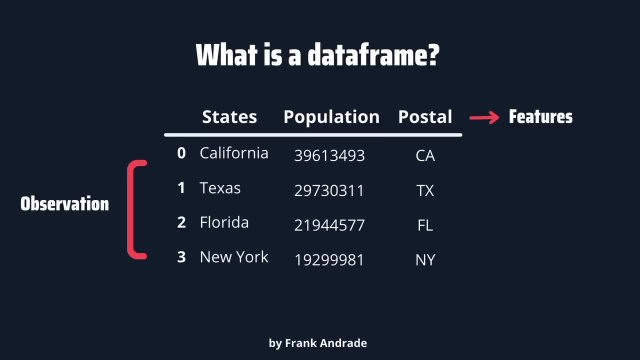 features here are states, population and postal, While each row value is known as observation, we can say that there are three features and four observations, because there are three columns and four rows. Keep in mind that a single column should have the same type of. 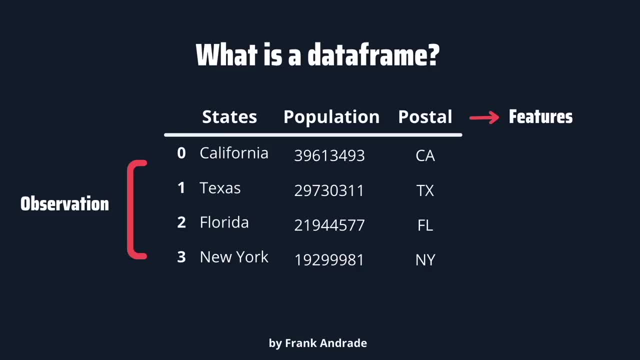 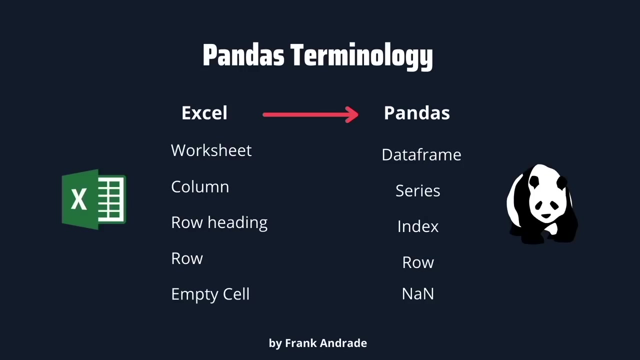 data. In our example, the states and postal columns only contains strings, while the population column only contains integers. we might get errors when trying to insert different data types into a column, So avoid mixing different types of data. So now let's see that terminology translation between Excel and pandas. So, as I mentioned before, 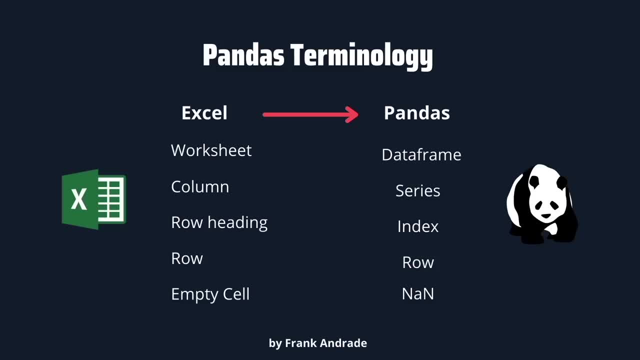 in Excel we work with worksheets. in pandas we work with data frames. So the columns in Excel are also known as Syrians in pandas. But we also mentioned or we also say often the word columns, And in pandas we worked with index. So the index are those numbers that are on the left. 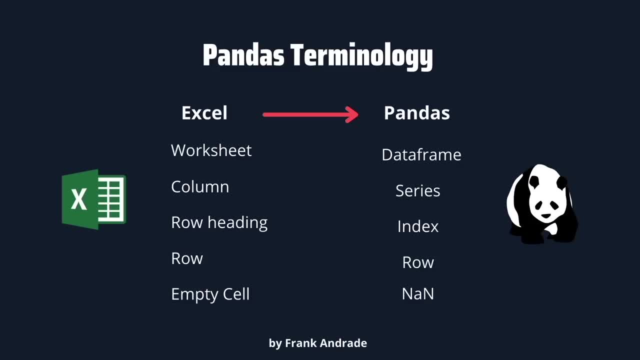 And in pandas we also say rows. we have many rows. well, observations too, but rows are fine. And finally, in pandas we work often with this n? a? n, that stands for not a number, And this is the equivalent of an empty cell that you might. 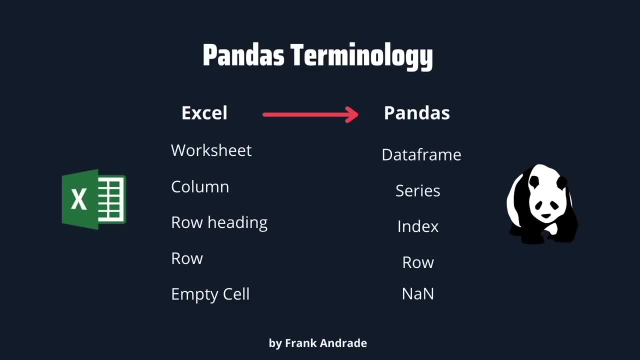 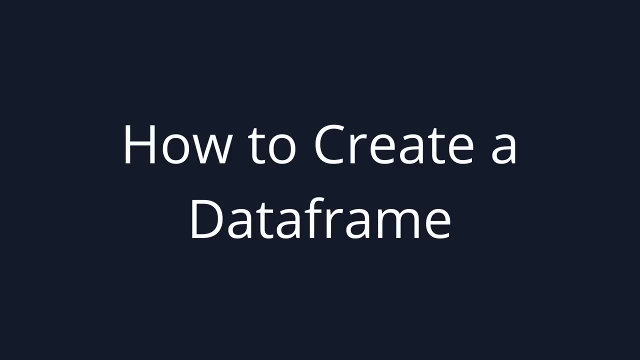 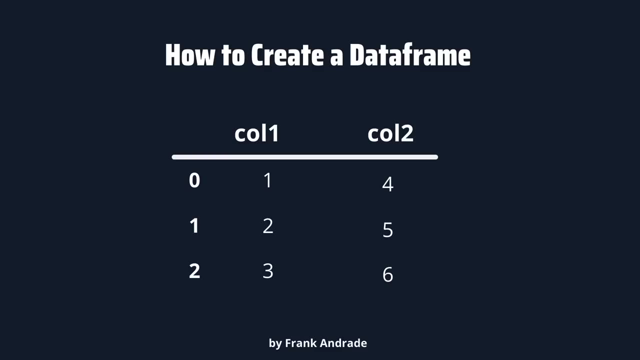 find in Excel. So that's it for now. In the next video, we're going to learn how to create a pandas data frame from scratch. Welcome back. In this video, we're going to learn different ways to create a pandas data frame. So, as you might remember, a data frame looks like this. It's a. 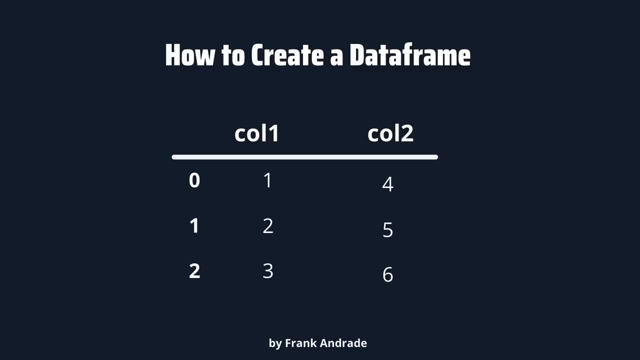 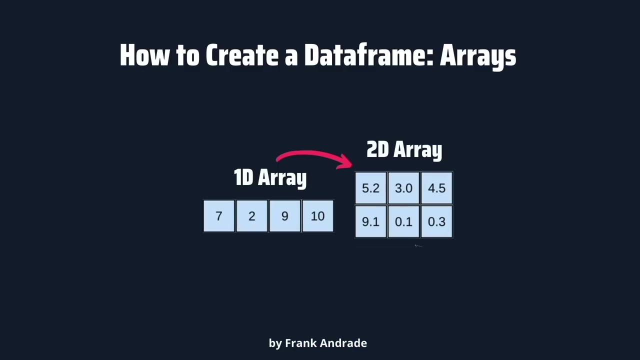 has columns and rows and the columns are series, So series are one D array And arrays is how we create a data frame. So this is the first way to create a data frame with arrays. So these are arrays. we have one D arrays to D arrays and one D arrays are basically columns, while two D arrays. 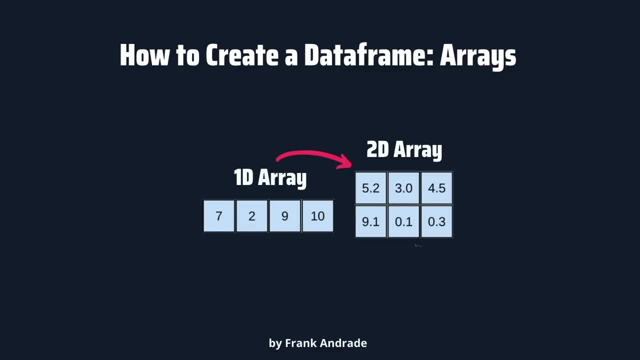 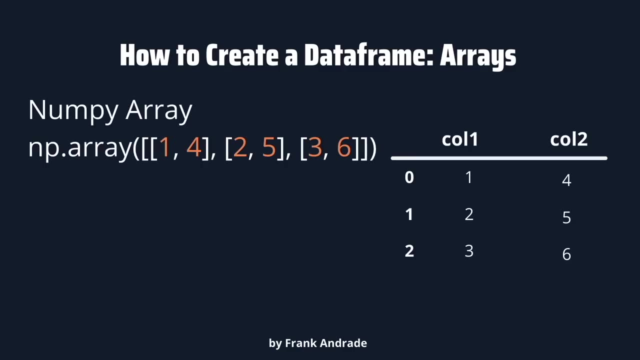 are data frames. So usually to use arrays we use a library named NumPy, And NumPy is what is under the hood of pandas. So to use NumPy we have first to import NumPy. we're going to do that a bit later, when we 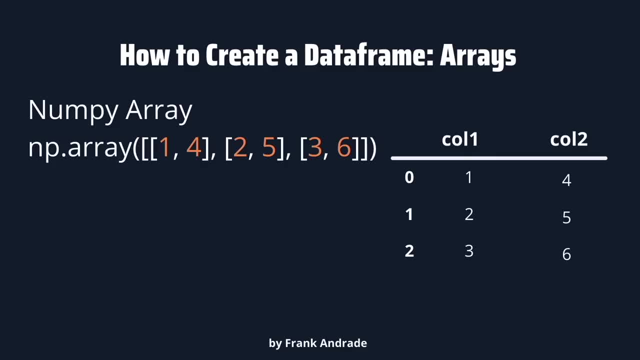 write code. But just to give you an idea of what a NumPy array looks like, here I wrote basic array. we have to use NP, that array, to create this data frame that you see on the right. And well, this is one way to do it. You can also use lists, as I'm showing you right now And as you can see. 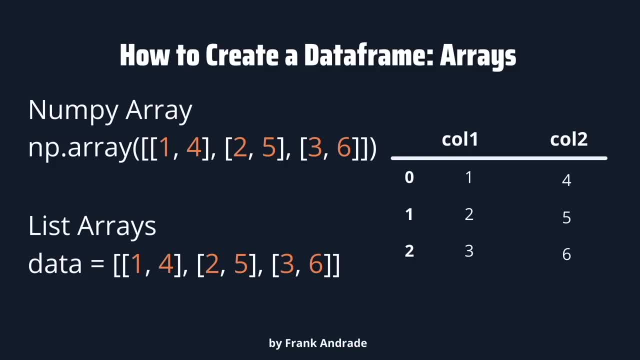 here and the second option: when you create a data frame with lists, you don't need to use NumPy arrays because you're using some kind of list arrays. So we're going to write the code to create a data frame with arrays. But let's see the second option: to create a data frame. 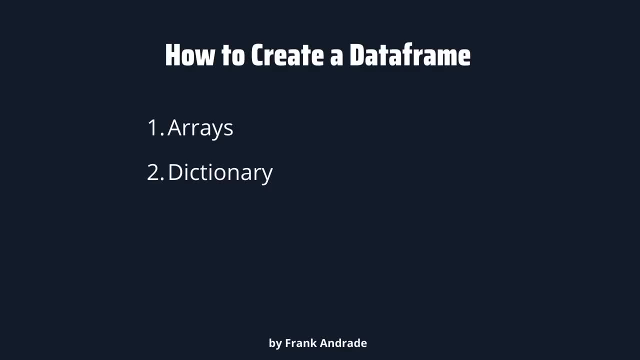 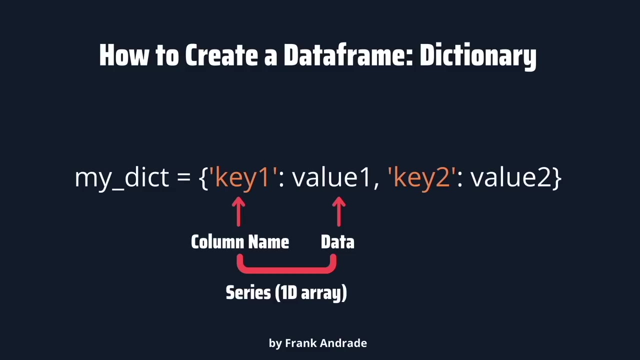 So the second option is dictionaries. you can create a data frame with dictionaries And, as you might remember, a dictionary has a key and a value. So we can use the key as column name and the value as the data. So the value can be a list. 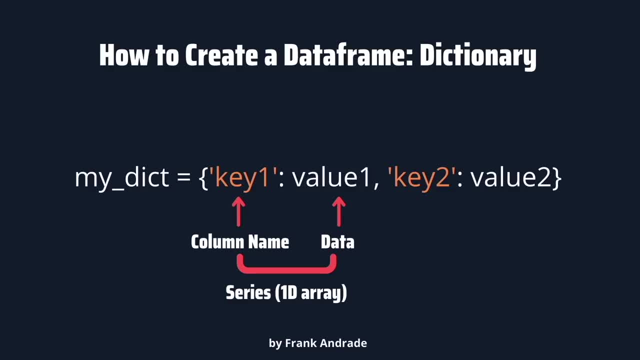 So this data will be many elements inside the list. So a pair of key and value is known as item in a dictionary And in this case is going to be a series, because it's one column what we have here. So this is the second way to create a data frame with dictionaries And we're going to see 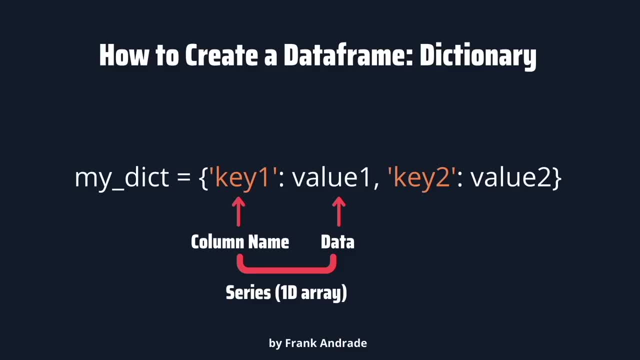 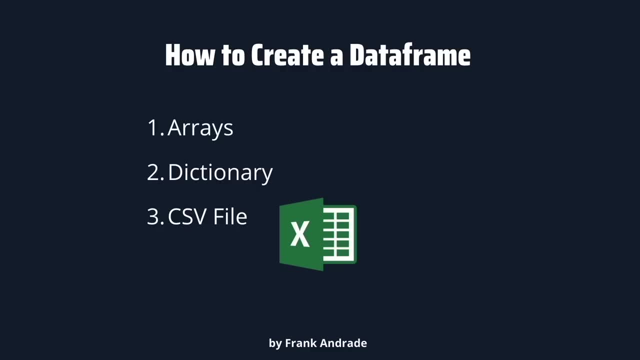 that with code a little bit later. But now let's see the third way, Which is with CSV files. So CSV files are files that can be open in spreadsheets like Excel, And this is the easiest way to create a data frame, because we only need to read the CSV file and then 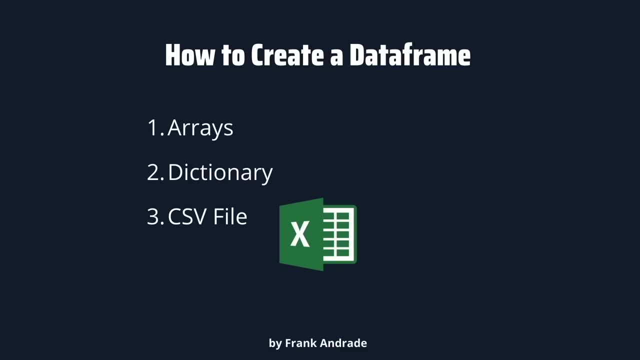 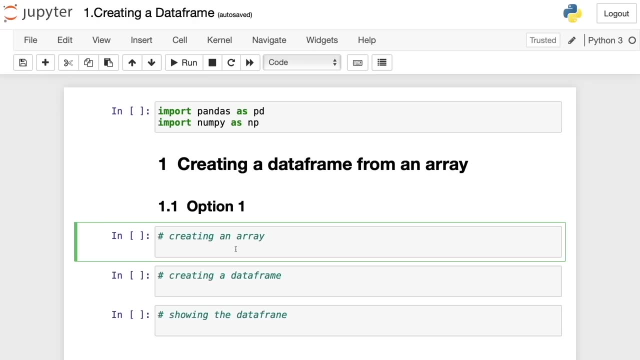 the data frame is created And that's it. So now let's go to Jupyter Notebook to create a data frame writing some code. Okay, now we are on Jupyter Notebook, In here, we're going to write the code to create a data frame And we're going to use the three ways I showed you before. So the first thing: 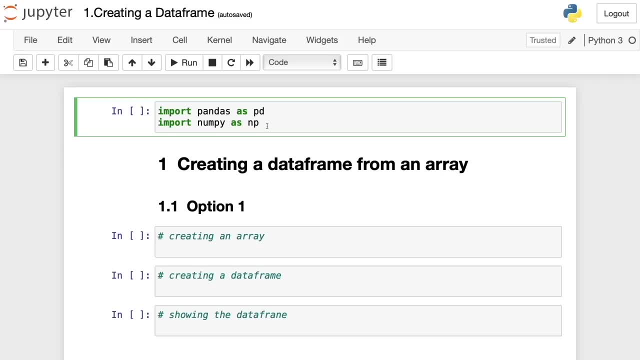 we're going to do is to import the libraries we're going to use to create a data frame. So that's the first line of code And I already wrote that, So it's here. So first we import pandas And then we import NumPy. So import pandas as PD. PD is just a convention to name pandas. 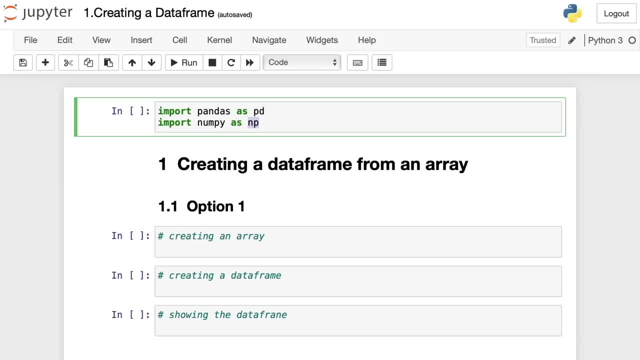 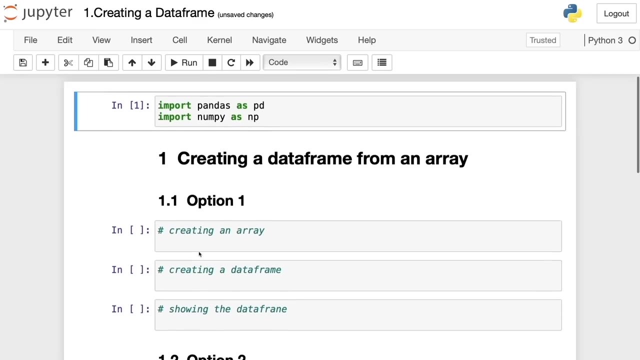 And NP is a way to name NumPy. So to run this code just press Ctrl Enter And now just wait, and we imported pandas in NumPy. So let's see the first way to create a data frame. So the first is with arrays, And to create an array we have to use a NumPy. This is the first. 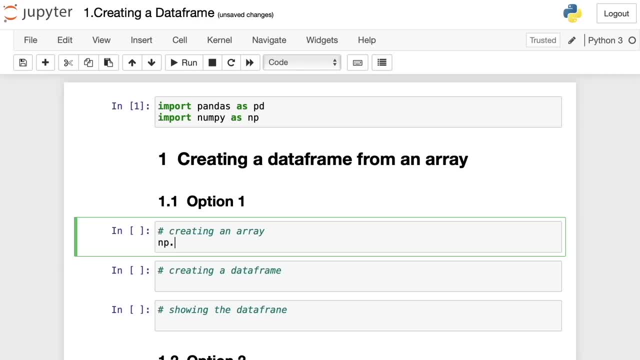 option. So we write NP, which is the short name for NumPy, And then we use the array method. So we write array, open parentheses, And inside we write the array we want to create. So I'm going to create, I'm going to write random numbers, just for the 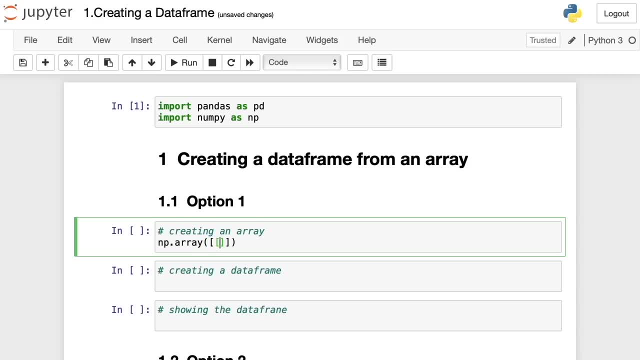 sake of this example. So I open double square brackets And then let's write, let's say one and four, And then let's say two and five, And the last one is going to be three and six. So each pair of- let's call it- list- Actually they are lists- Each list represent a row, So 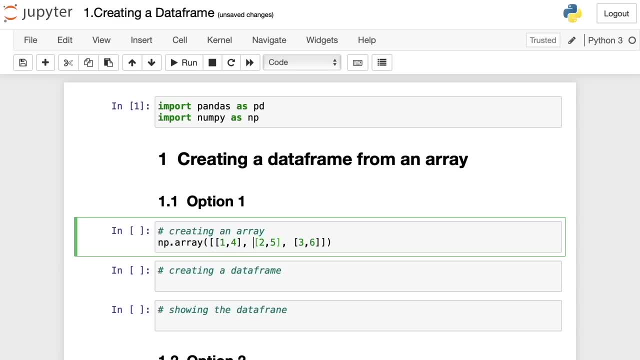 this is the first row, or this is going to be the first row, this is going to be the second row in our data frame And this is going to be the third row. So here we can name this rate and I'm going. 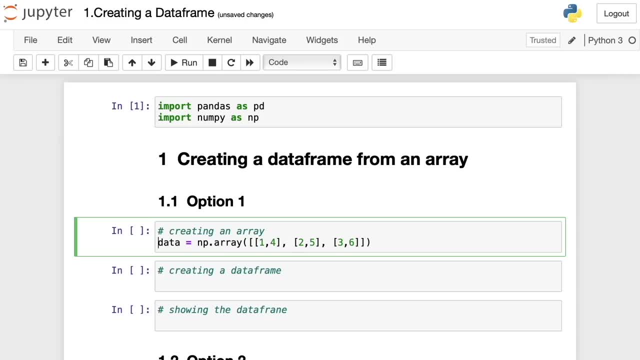 to name it as data. So that is equal to this NumPy array. So I'm going to execute this code. And now we have this data. So we created a rate using NumPy. Now let's create a data frame with pandas. So to create a data frame with pandas, we have to write pandas. In this case, 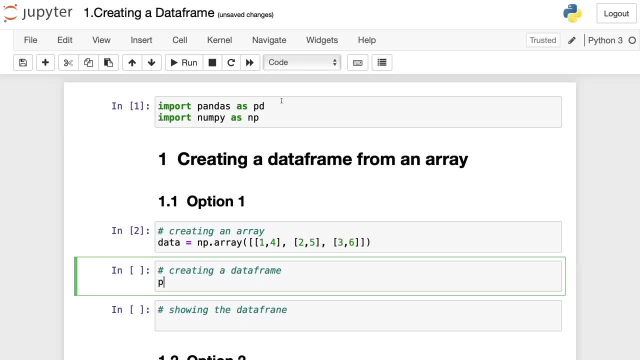 I can write PD, because I named it like this here in my first line of code. So I write PD And then to create a data frame we use the data frame method. So we write that data frame and then we open parentheses, And here we have to fill some. 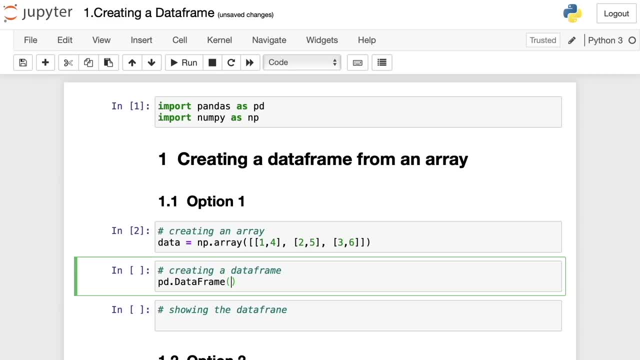 arguments. So the first one- and that's what- something that you always have to include in this data frame method is the data, because you cannot create a data frame without data. So first we include the data. So first copy here our array and then you paste it here. 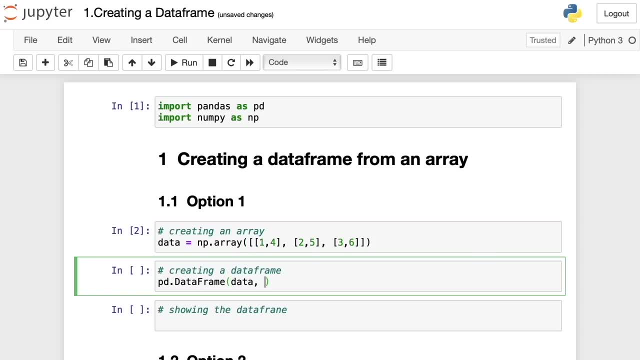 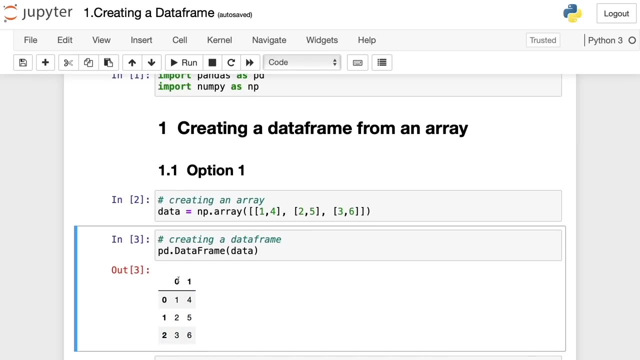 That's the first argument, So you can create this data frame as it is. I'm going to show you here, just Ctrl and enter. So, as you can see here, here's my data frame, But as you can see, it's full of numbers and column names also have numbers and the row names. 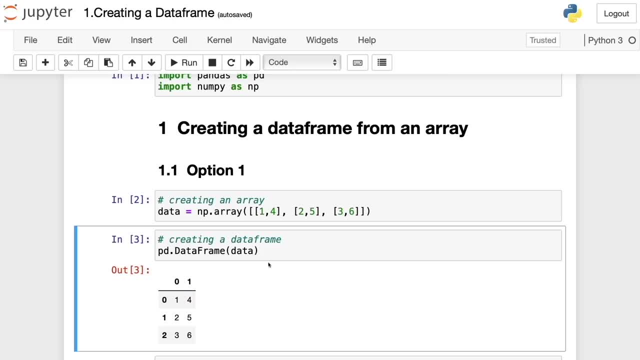 also have numbers. So to make it more understandable, we can rename these, this column names and row names, And you must have successfully created develops. you must name these columns as you want to open retired. Feel free to type any arguments you like in the comment box and you can even add basic reasons if you want to. So, for example, there is a 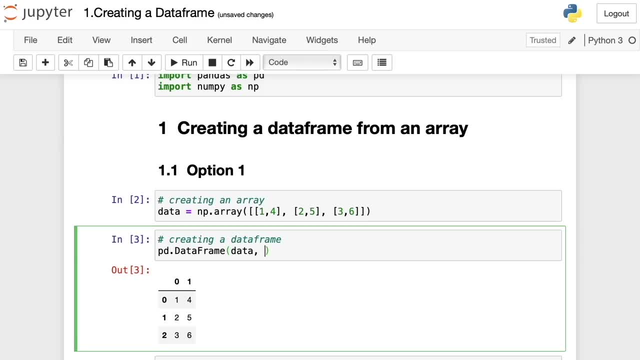 and row names or index. actually, the name of the row names are index. So first we can name this index as rows, For example we: you only need to add the index argument, as I'm writing right now, And then you have to specify the names you want to set. So you have to. 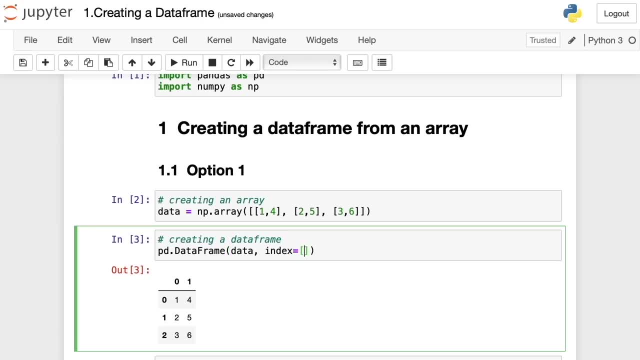 open a list. So this first or the second argument has a form of a list. So the first element is going to be the first index. So here zero. So in case you don't want it to be zero, you can set here another name. So in my case I'm going to set it as row one, then comma. 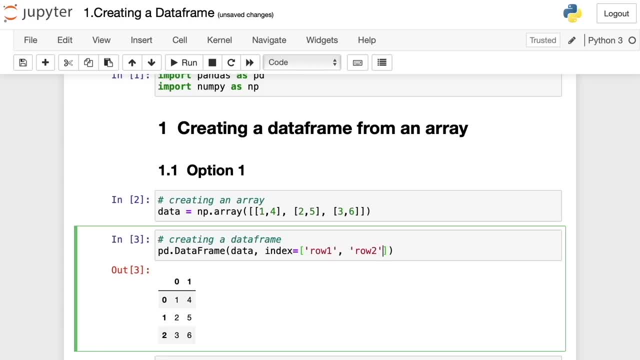 to set the second index as row two and the third as row three. So now we can add also or we can modify also the column names. we have to use that column argument And here we write it columns, And then we open square brackets because it's 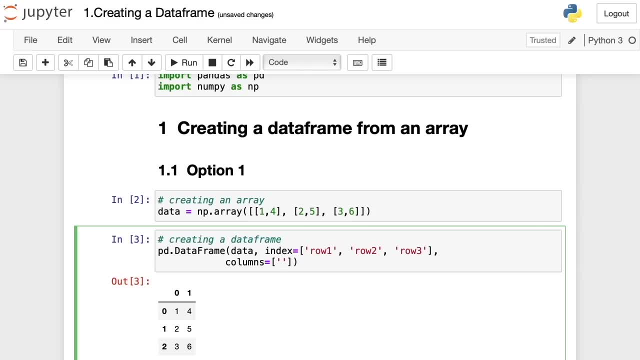 a list here that we're going to edit, And in this case we have to modify only two elements. So the first is going to be- I want to name it- call one And the second call two. So I'm going to write this one And actually I'm going to name. 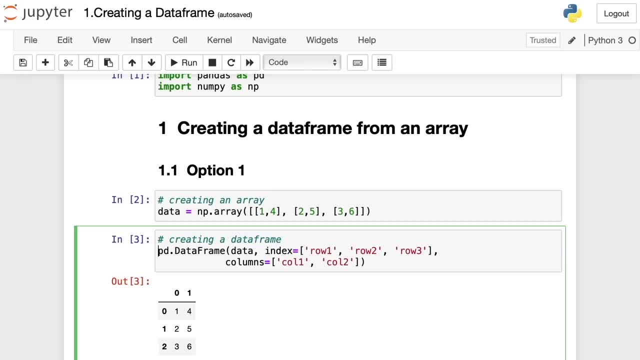 this data frame, So I'm going to set it to a variable And this is going to be equal to the F. the F it's the common way to name a data frame, So the F stands for data frame. So I'm going to run this code now And, as you can see here, 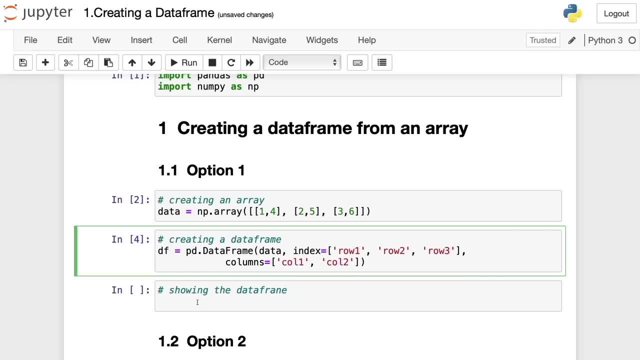 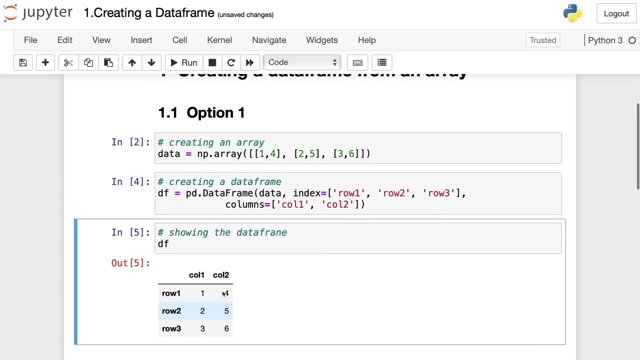 it ran in out to show the data frame. I can write here the F, so the F, And now we have here the data frame And, as you can see here, the first row, one four. it's my first, my. 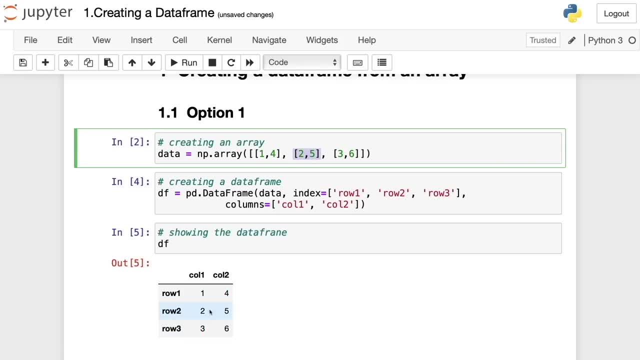 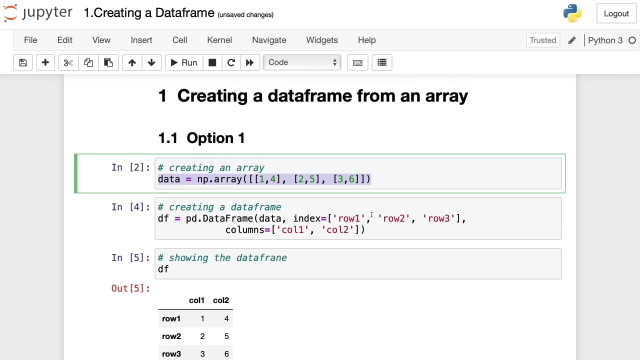 first list And the second is the second row And the first column. well, that's a series, as we discussed before, So we have also the column names that we modified And the row names. So now let's quickly see how to create a data frame with arrays. but 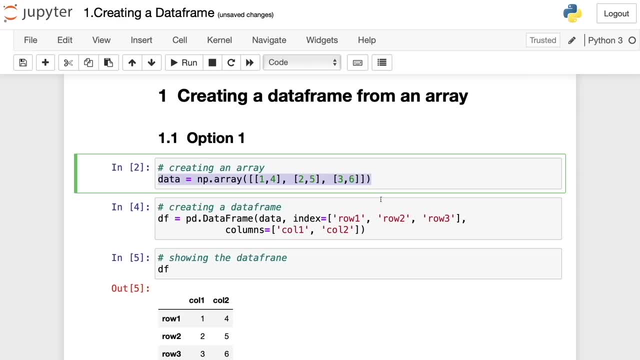 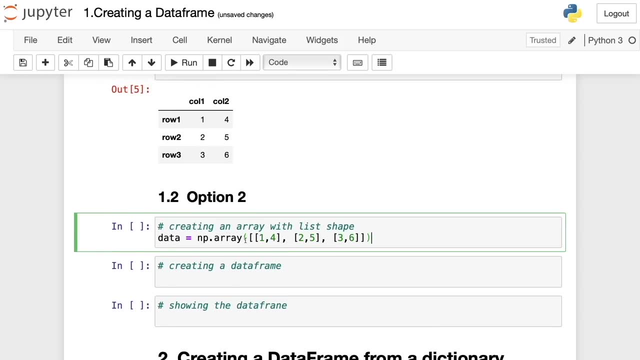 in this case without NumPy. So I'm going to copy this line of code and I'm going to paste it here. option two: So here I'm going to paste this, because this is the base of this arrays with list shape, And I'm going to just delete this. So I don't want NumPy. 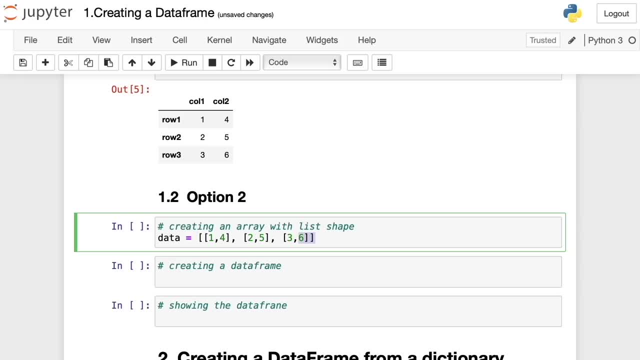 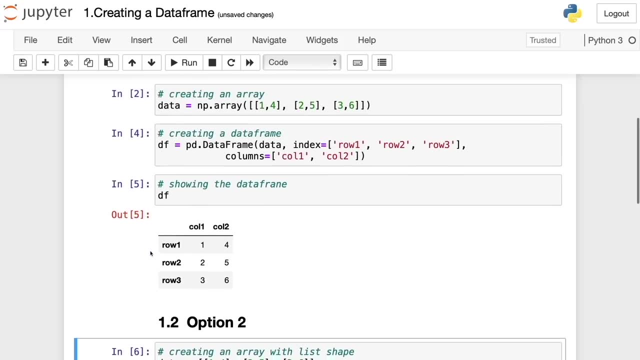 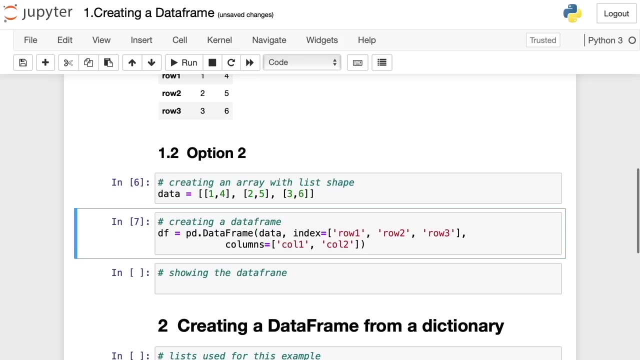 array anymore, just this double square brackets. So I run this Now to create a data frame is the same way we did before, So just copy this and paste it here. So run this And now I can run the. I can write the F and now execute. 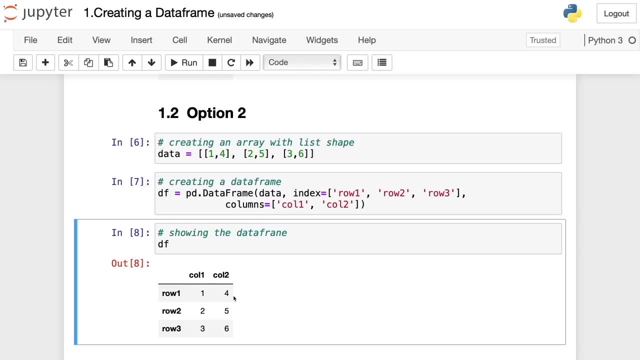 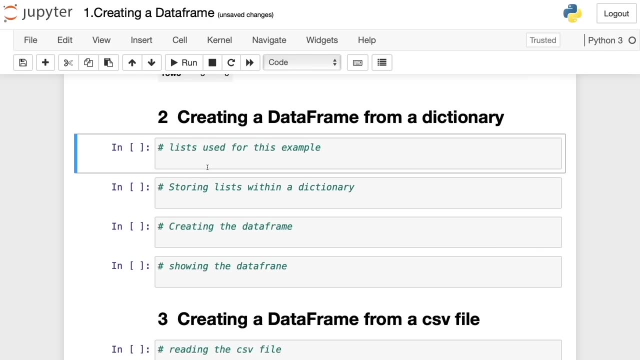 this code. So, as you can see, we have the same result. I'm just showing you the second way, So you don't have to worry about learning right now: NumPy. Okay, now let's create a data frame from a dictionary. 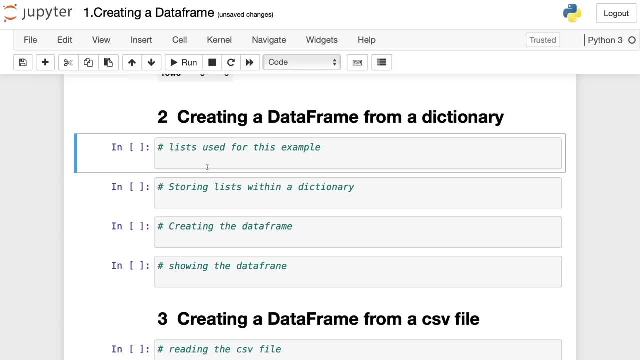 Okay, now let's create a data frame from a dictionary. So let's create a data frame from a dictionary, And we're going to use lists in this example, And we're going to create a data frame using more meaningful data. So in this case, to create a dictionary, I'm going to use two. 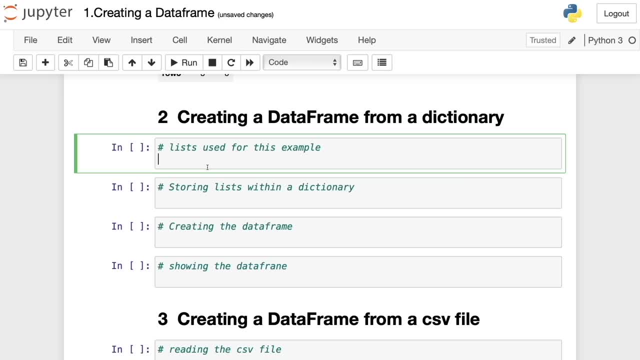 lists. The first is going to be a list named states. In the second it's going to be that population and it will contain the population of each state. So the first list is states And I'm going to write it here And I open square brackets because this is a list And 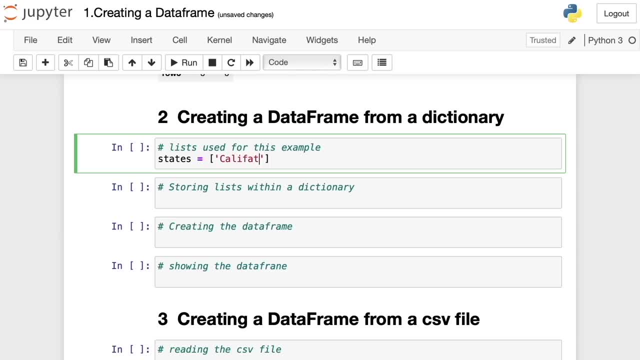 now I write some states in in the US. So the first is California, The second is going to be Texas, Let me write it here. The third is going to be Florida and the last one New York. So I quickly write it here, And now I'm going to create a population list, So in this case I'm going 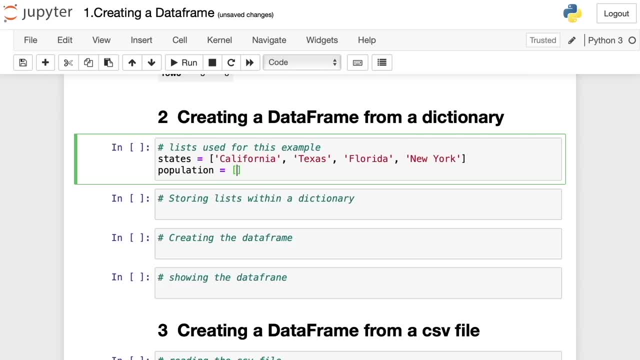 to pay. So in this case I'm going to paste this data. So I paste it: the population fromamorphic loss text. here I paste the list data basis on each state, And now I'm going to create a dictionary from these two lists. So I'm going to 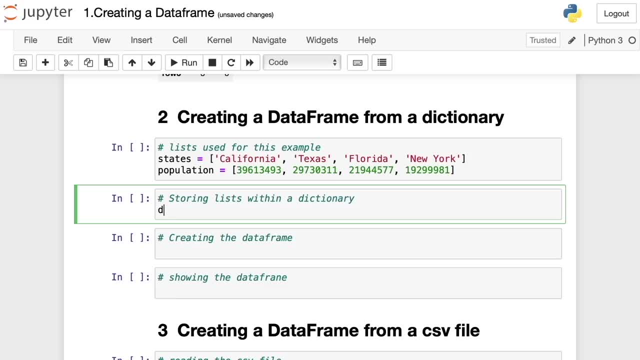 write the name of the dictionary. So the name is going to be dict, underscore states. then this is a dictionary, So I should use square brackets, sorry, curly braces. And now I'm going to set the name of the key. So the first key is states, then colon and now the element or the value. So 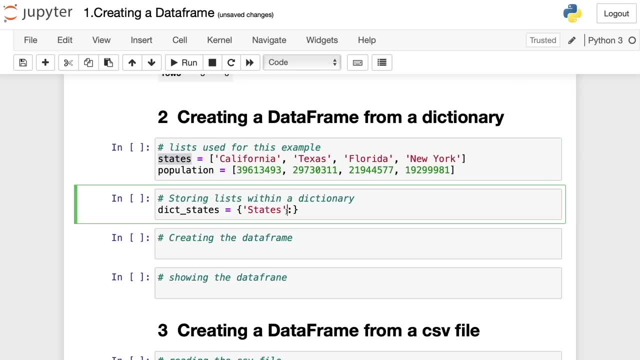 this is states, the first value And the second key and value is population. I'm just going to set it to with capital letter, And the second is the least population that we have here. So with this we create a dictionary. And now I'm going to create a dictionary, So I'm going to create 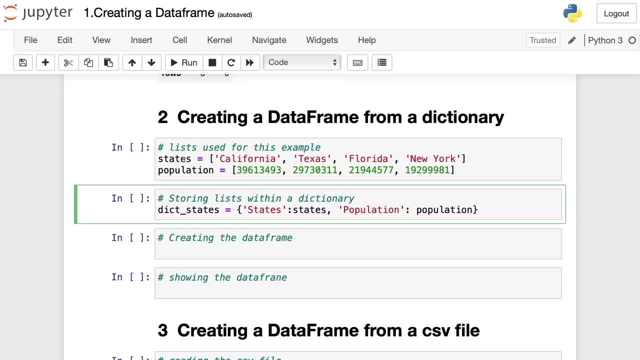 our dictionary. So I'm going to run these two And now we have lists and a dictionary. So now we can easily create a data frame using the data frame method that we used before for the first option. when we create a data frame with an array So to do it, just write PD, then that data frame. 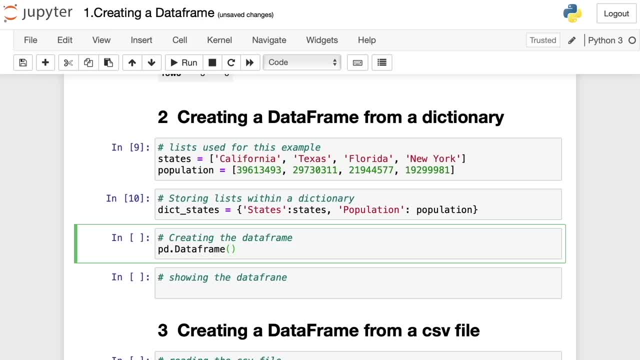 And now we have to write inside parentheses the name of the dictionary. So I'm going to copy dict: underscore states And I'm going to set this to new variable. So I'm going to name this DF underscore population. So data frame about population. So now I run this And here I 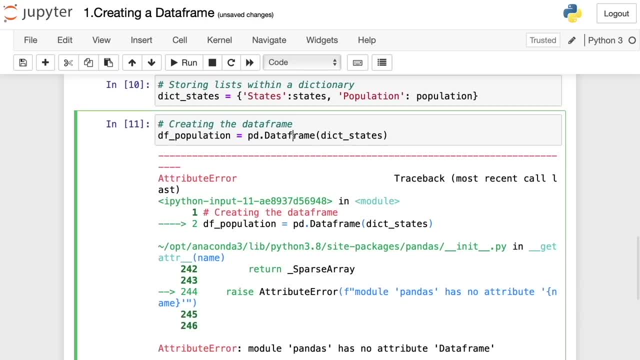 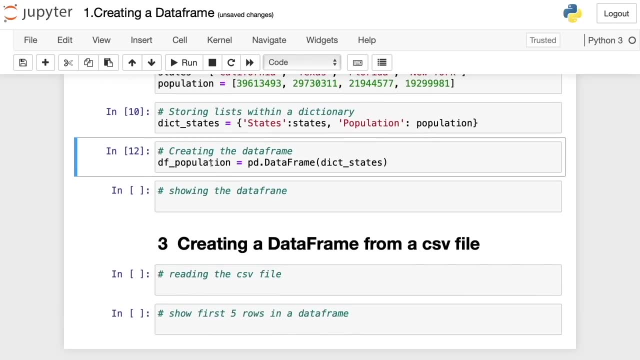 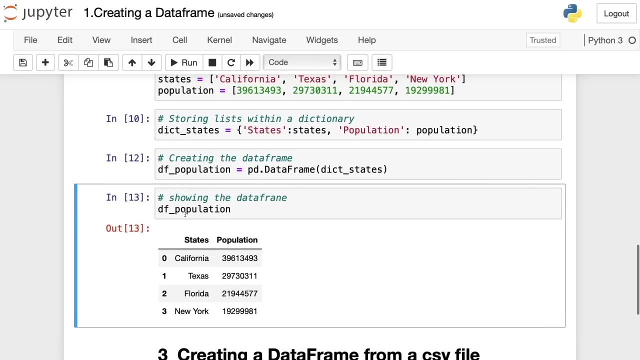 got an error because I didn't write data frame correctly. Here is in capital letter, So I run again And now everything is okay. So now to show the data frame, I just paste this one here And now I run. So here we have this data. 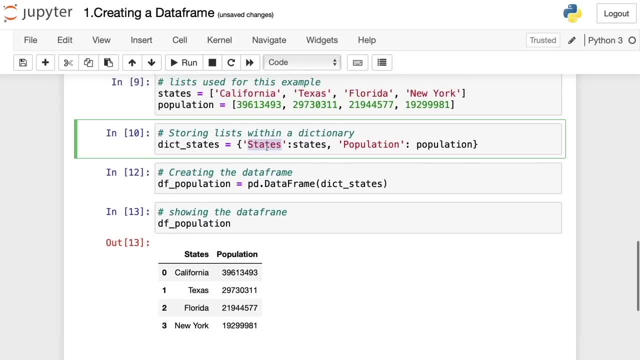 frame And, as you can see here, my first key states is the name of my first column And the data inside the states list is here. So here is my first column, or my first series, And the same goes for population with its data. 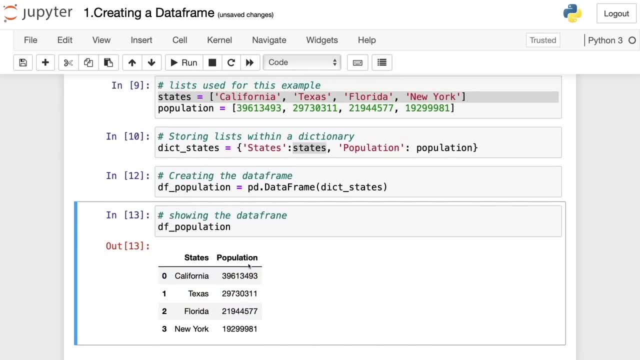 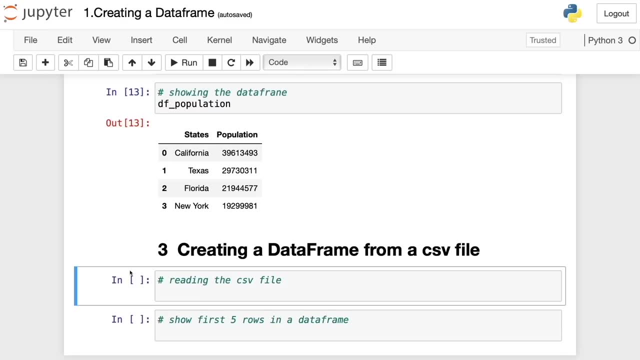 So here we created a data frame, And now I'm going to create a dictionary. So here we have this data frame using a dictionary. Okay, finally, let's create a data frame from a CSV file. To create a data frame from a CSV file, we have to use the read underscore CSV method. So first we write as: 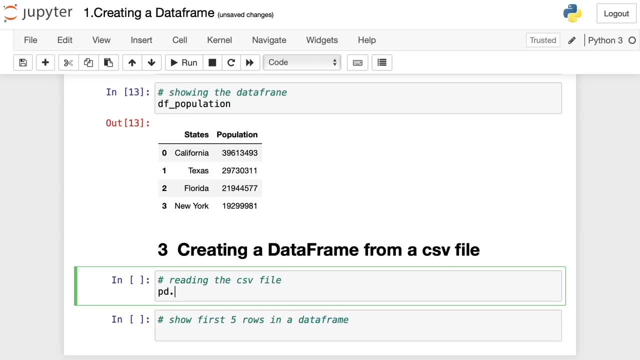 usual PD that stands for pandas. And then we use the method So we write: read underscore CSV- open parentheses. And then we have to write the name of this CSV file. Here I'm going to paste the name So it's named students performance that CSV And download this data. 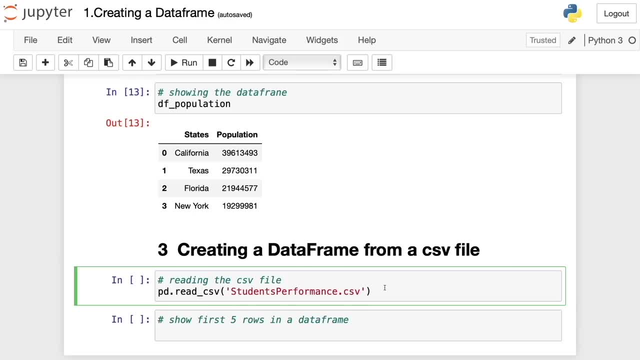 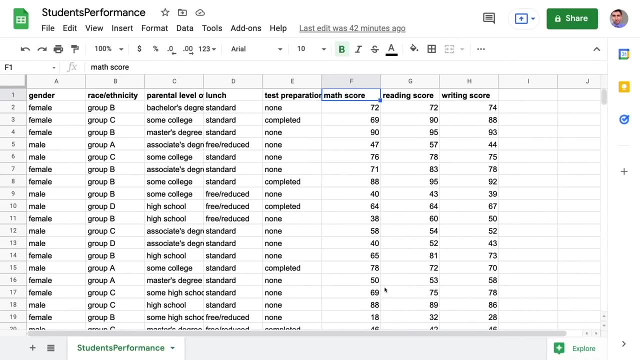 you can check the notes of this video And actually we can have a look at this data before importing into pandas. So it's here, I have it in Google Sheets And, as you can see, here we have this course of some. 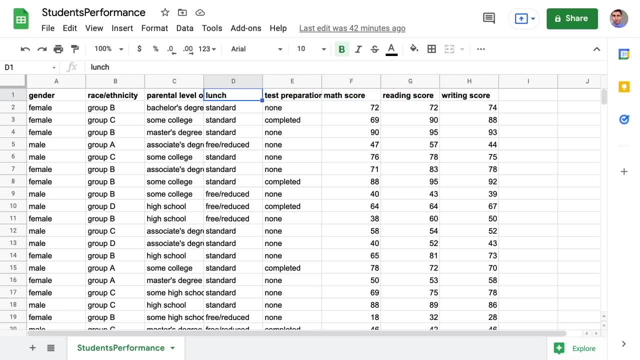 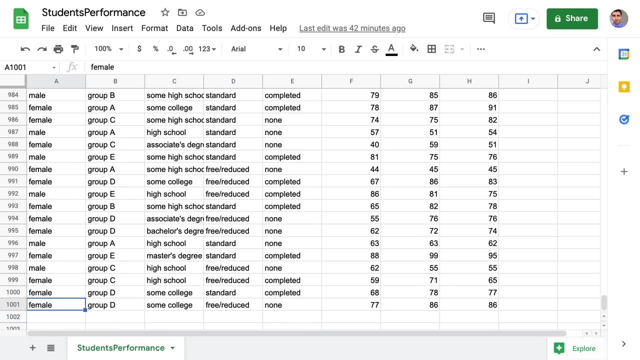 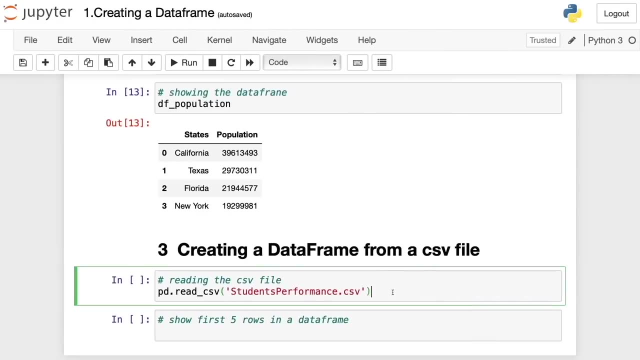 exams, math, reading and writing, And we have some other data, So we can import all of this data, all of the 1000 rows in pandas, So all of this is going to be here. So here we only have to define the name of. 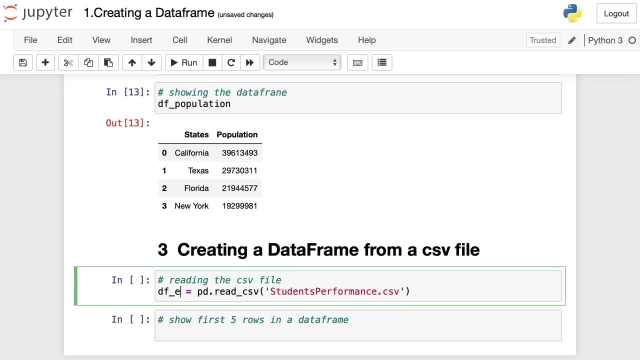 this data frame. So here I'm going to name it DF underscore exams. So now I run and to show now the first five rows of this data frame, we can use a method named head- that we're going to see later, But just to give you an idea. 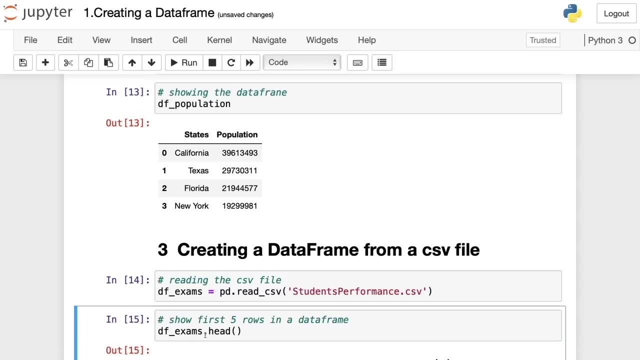 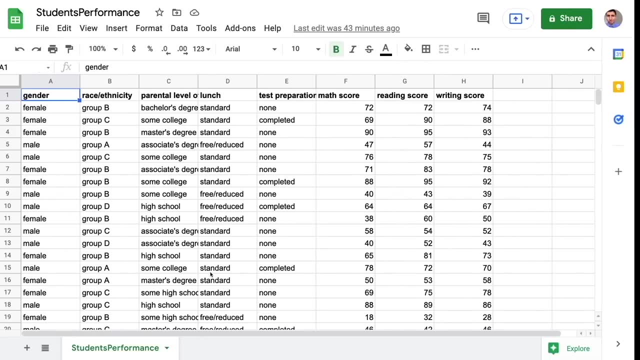 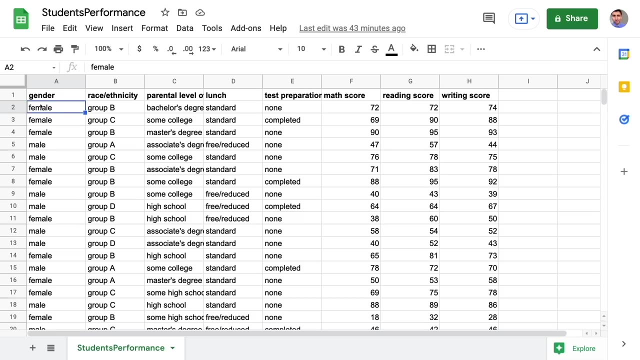 this. we can write that head and we get the first five rows. So, as you can see here we have the first five rows of this Excel, or actually CSV file, And you can see here, for example, the first row. it says: 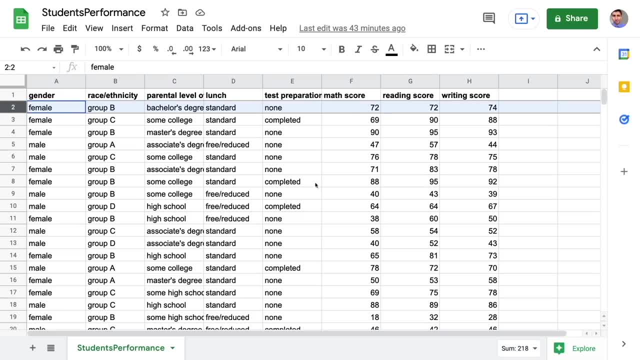 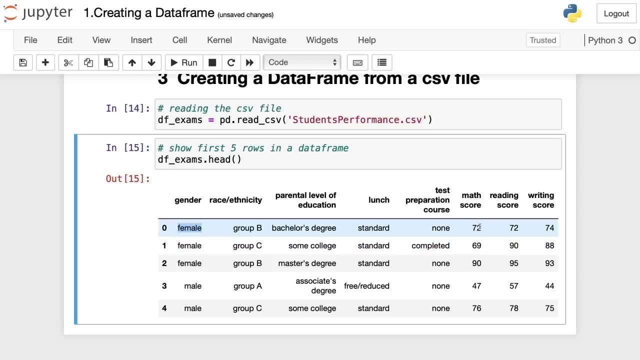 female group B and math score 72. So let's check if that data is the same here. So we have female group B and math score 72. So we have all this data here in this data frame. So if we want to see all of them, all of the rows here we 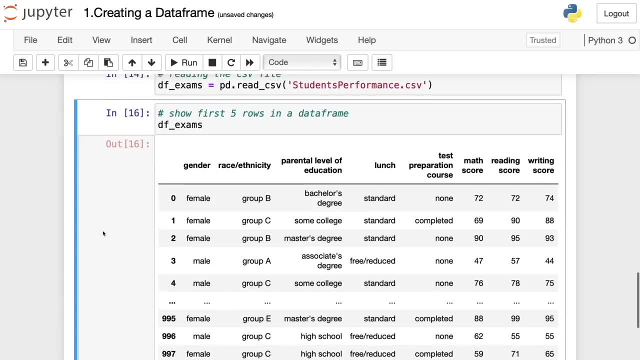 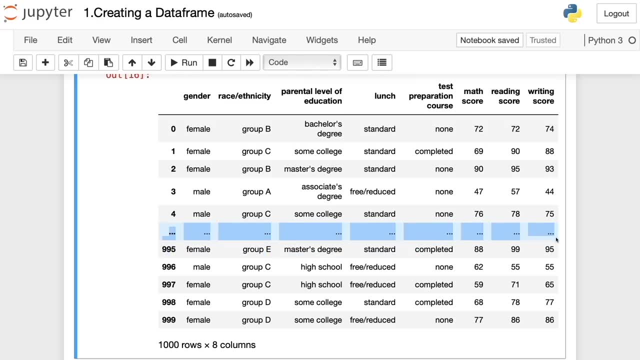 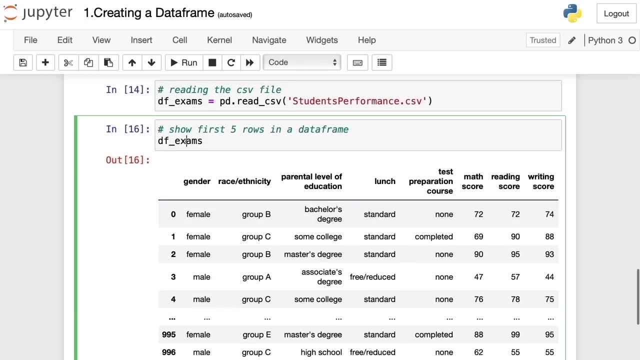 can forget about the dot head. And now we have all the rows. Well, here we cannot see part of the rows. I'm going to show you how to see that part later in this course, But now, as you can see, if we run this DF. 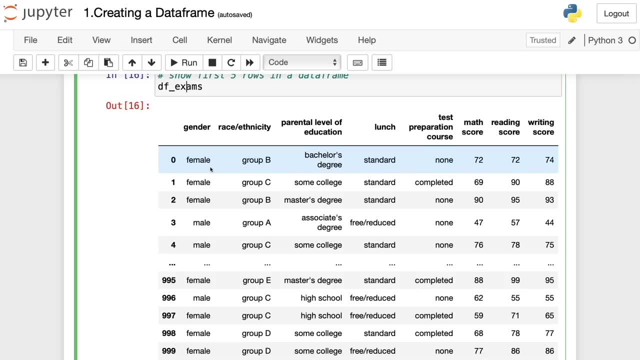 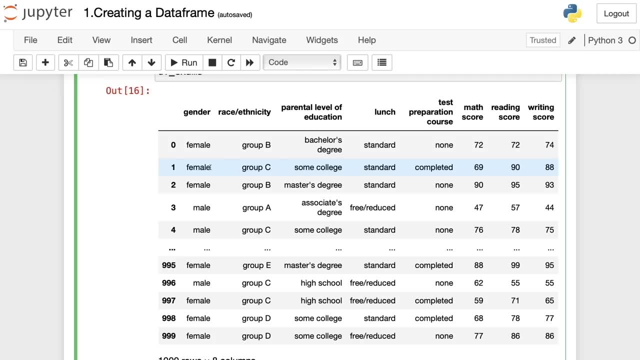 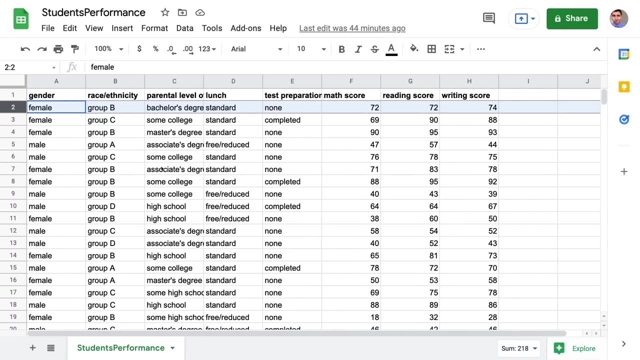 underscore exams. we can see, like the summary of this data set or well, data frame- this case, by the way, in pandas or when we work actually in Python, we usually call this type of CSV files, we call it data sets. And when we read a data set using well, pandas, the result is a data. 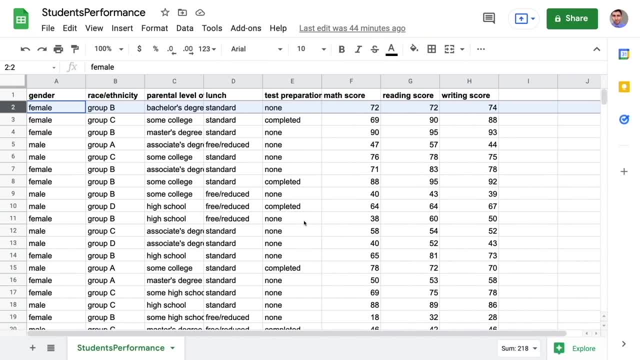 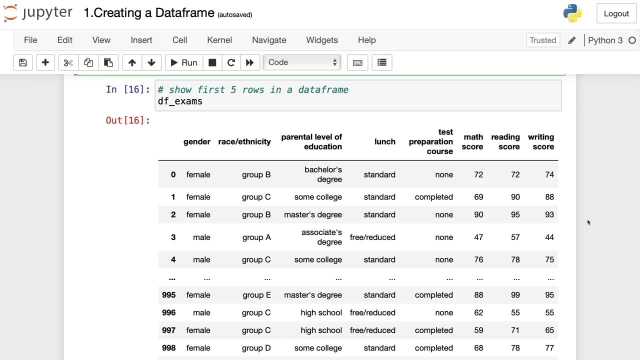 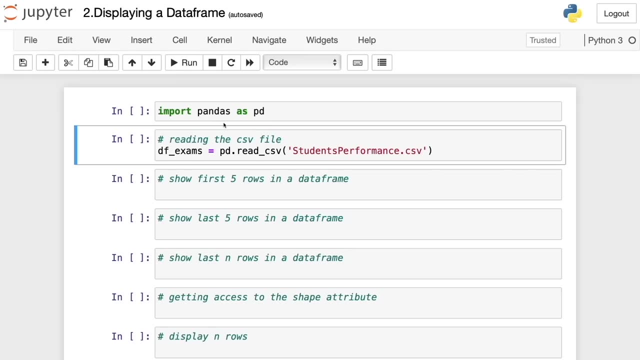 frame. what we have here, So the CSV file, is a data set, And this, when we read it with pandas, is a data frame, And that's it. This are the three ways to create a pandas data frame. Okay, now it's time to see how to display a data. 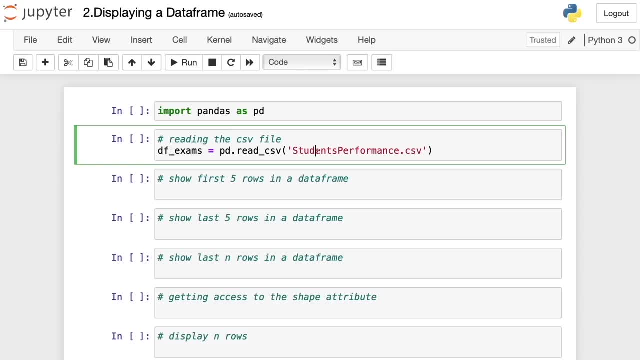 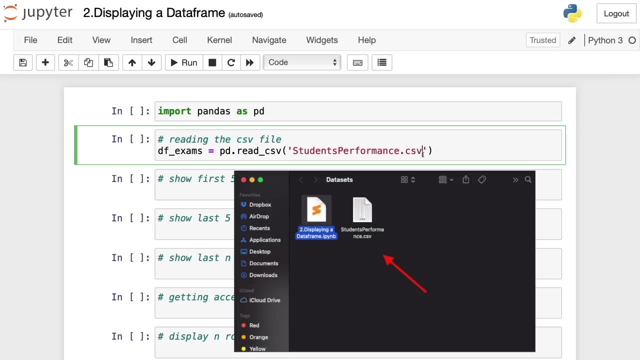 frame in pandas. So here I have the CSV file we use before to create a data frame, And a little detail I forgot to mention before is that this CSV file should be located in the same directory where your Jupyter notebook script is located. So 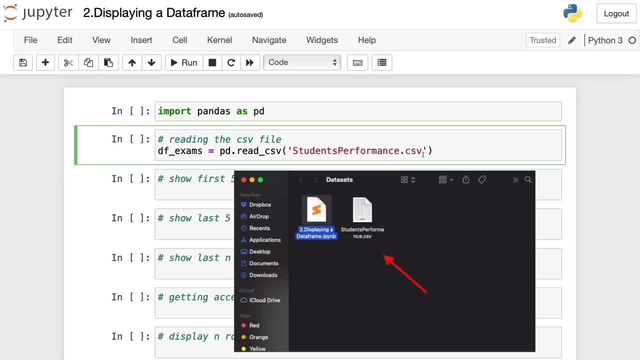 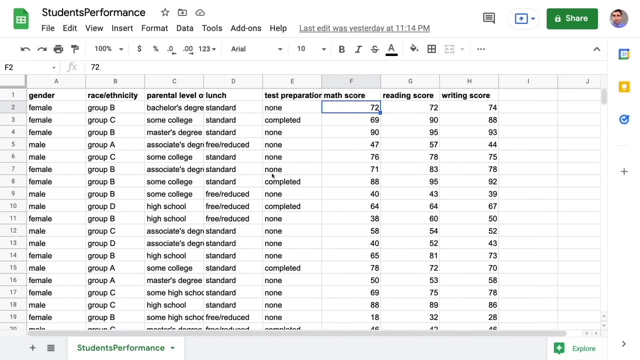 so what I mean by the Jupyter notebook script is what we're seeing right now. I mean the. what we're working right now is a Jupyter notebook script, this, this file that we're working right now. So what you have to do is to download this CSV file and 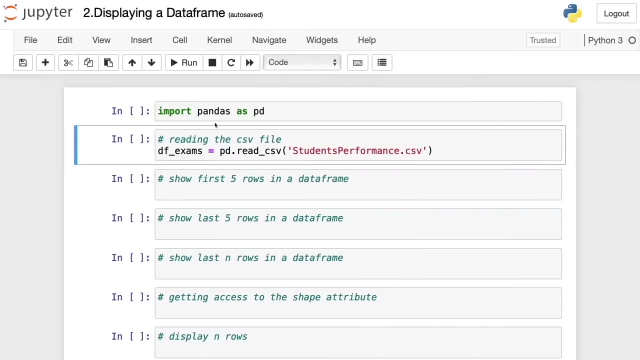 place it in the same folder where your Python or your Jupyter notebook script is located in the same folder, And this is how you're going to read this CSV file: the read underscore CSV method. So just make sure both the CSV file and the Jupyter Notebook script. 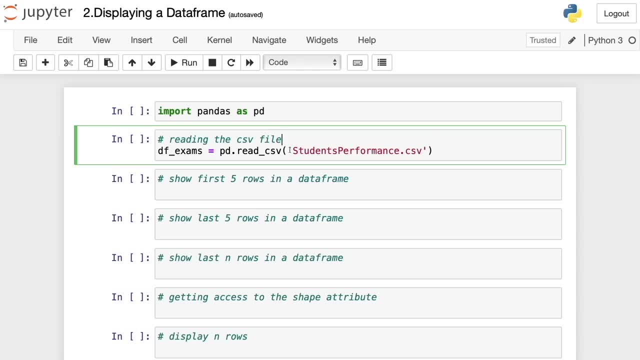 is in the same place, in the same folder. Okay, now I'm going to run these first two lines of codes that we've seen before. So the first import pandas and the second reads this CSV file. So I run this And now we have this CSV file stored into these DF underscore exams. This is my data. 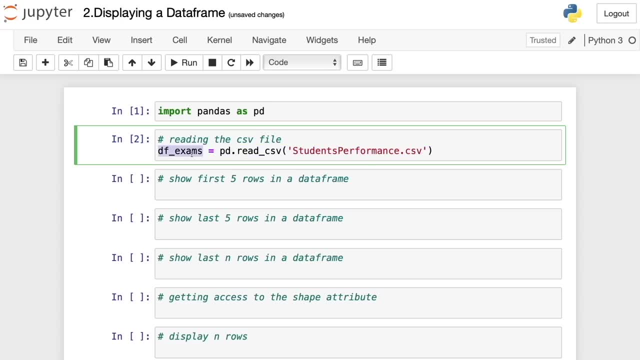 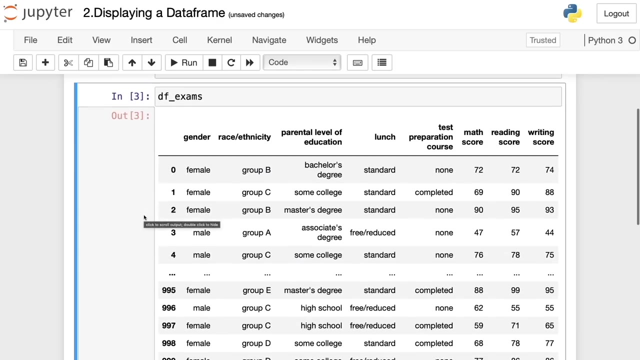 frame. So now let's see how we can see this data frame. So the easiest way to see this data frame is just copying this name, this variable, and now pasting here. Now I execute this, you know, we have the data frame. Actually, this is a summary of the data frame, because not all the 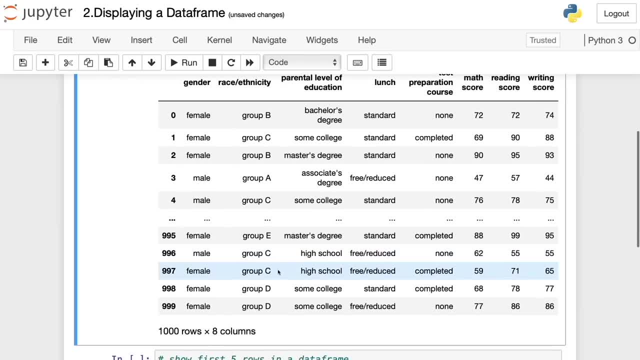 rows are the same. So I'm going to copy this data frame and paste it here And now. I'm going to now copy this data frame. Actually, this is my data frame. Actually, this is my data frame Because notes are seen here. So here we scroll down a little bit. we can see here that there are 1000. 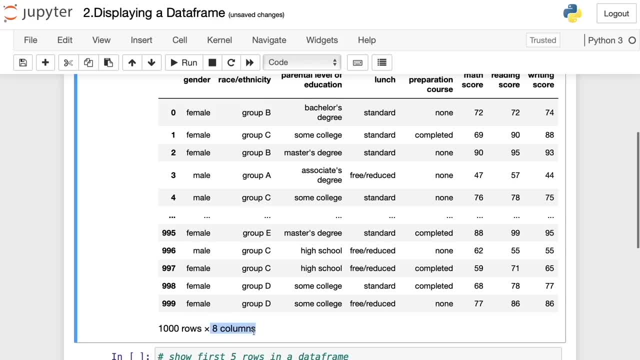 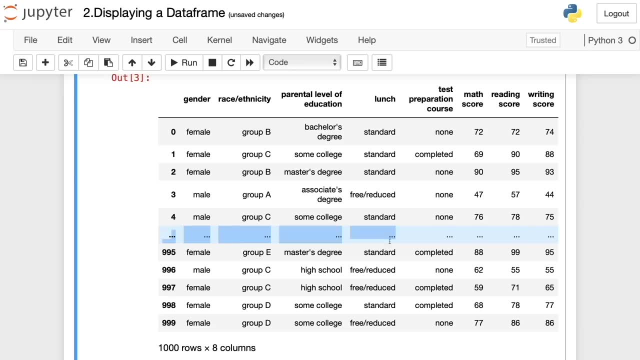 rows and eight, eight columns. So here we can see all these rows and columns, But as you can see, here in the middle we cannot see the rows. So it's until four and then it continues with 995.. So usually when we work with pandas we 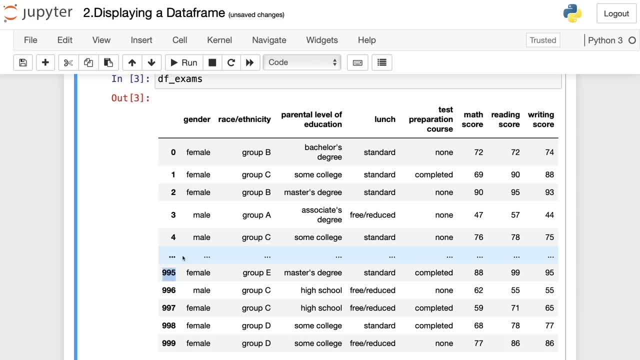 we don't need to see the data one by one, So row by row. that's not how we do it with pandas, But if for some reason you need to see all the data in pandas, as you will do it here in Excel or in Google Sheets. I'm going to show you a way to do it a bit later, But first. 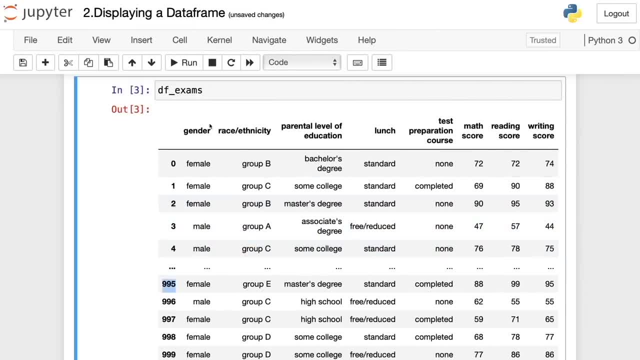 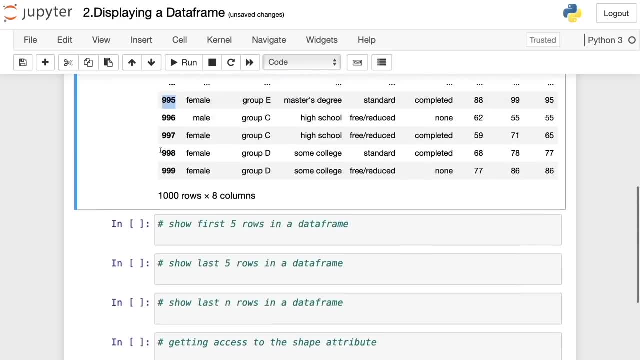 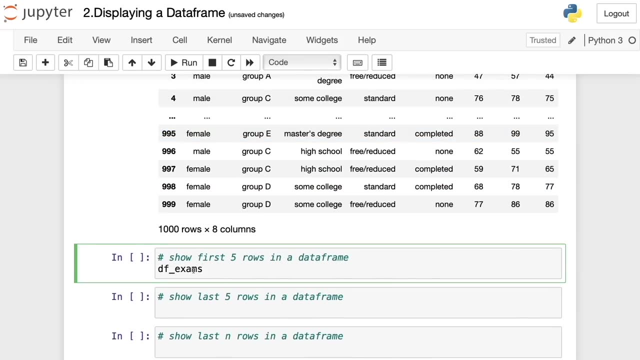 I'm going to show you different ways how we usually display a data frame in pandas. So the first way to do it is using the head method. So here, to use the head method, we only have to write the name of the data frame, in this case the F underscore exams, and then 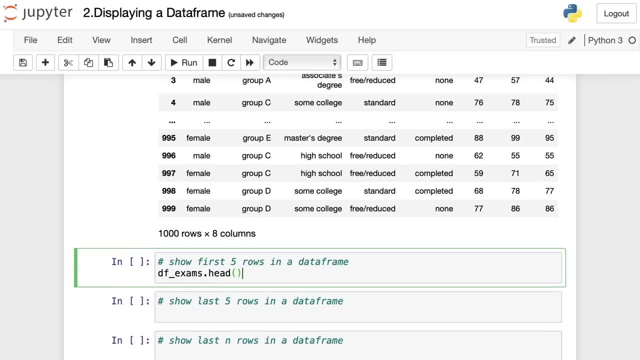 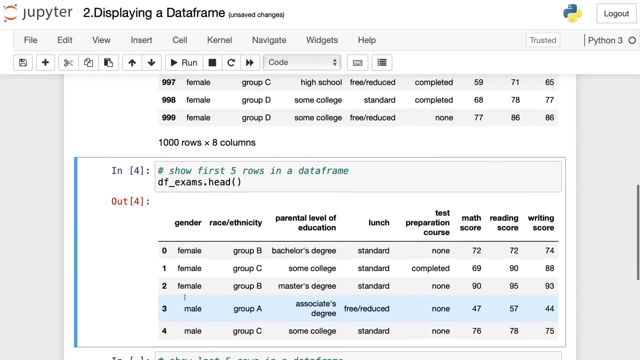 write head, then parentheses, then we run this And this is how we get the first five rows in a data frame. So you can see, here we have from row zero to row four And this is how we got these first five rows. 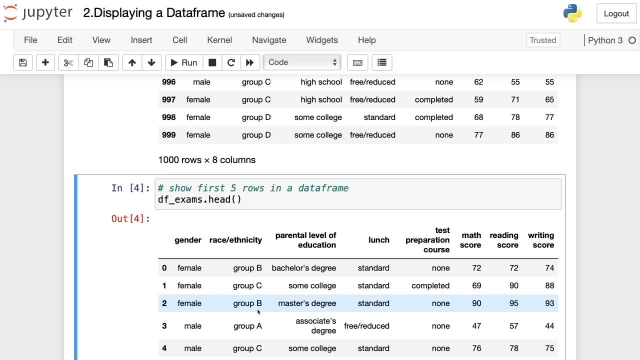 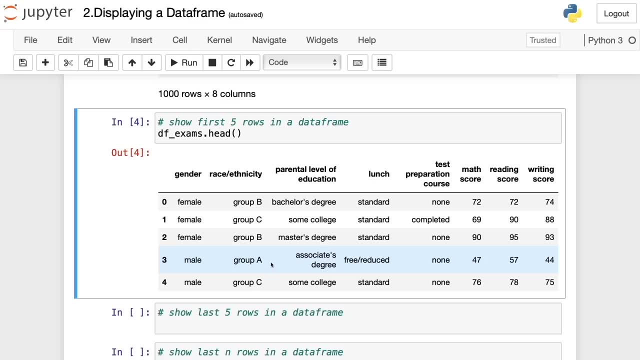 So this is the head method. In the same way, we can get the last five rows of this data frame by using the tails method. So here we only have to write again the name of the data frame- in this case, well, the same DF, underscore exams- and then write that tails, then parentheses. 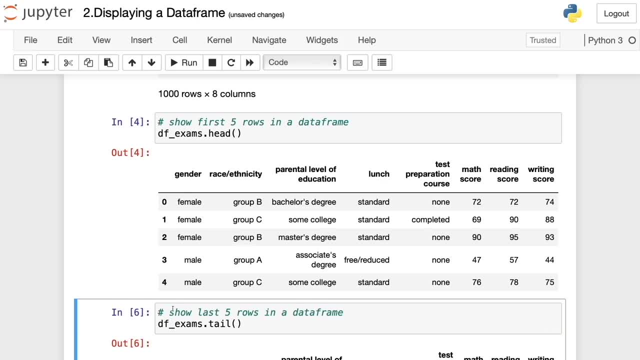 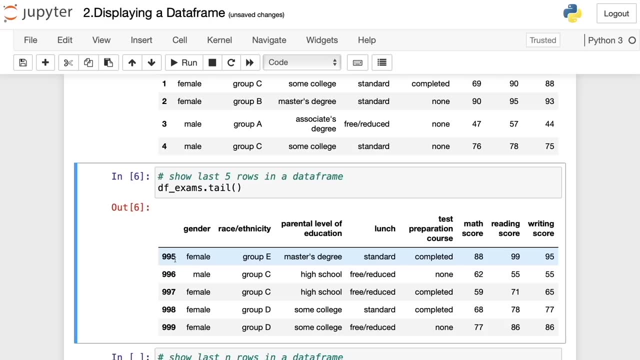 run this And actually I think it's tail- Yeah, it's tail in singular- And now we get this, we got the last five rows, So it's from 995 to 999.. So these are the five rows, the last five. 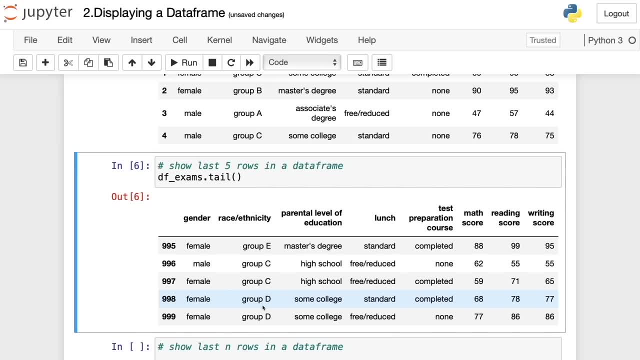 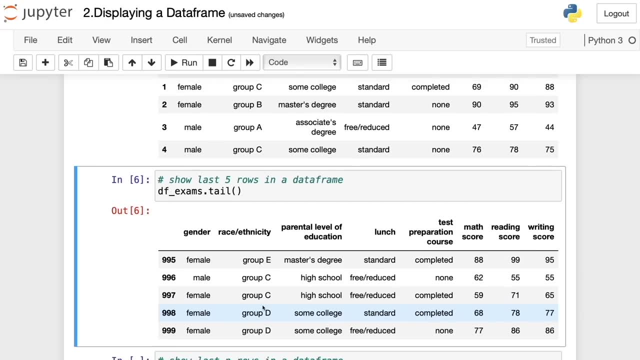 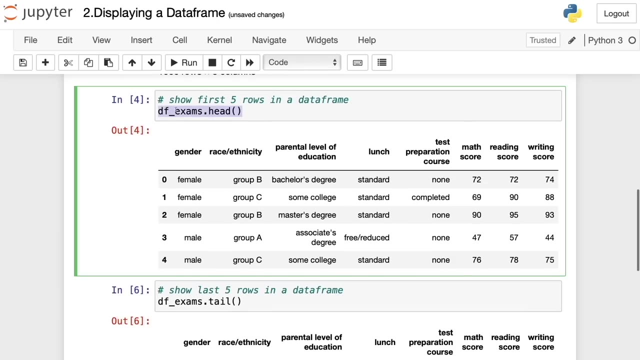 rows. And now, in case you want to get more rows- so not only the first five are the last five rows- you can add an argument to the either the head or the tails method. So I'm going to use here the head method as an example activities. So here I copied these ked ена. let's say, here I: 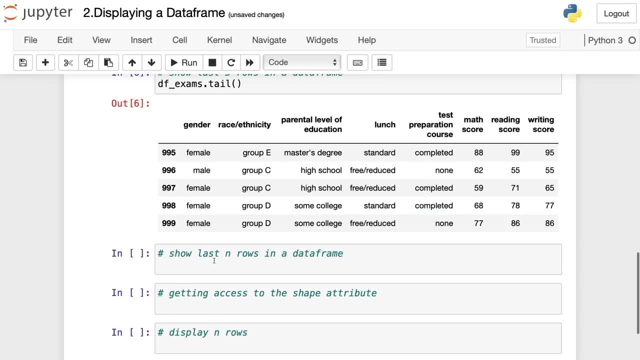 are going to read 5 rows on the rough test, which is usually the first five rows in a year, And now I'm going to paste here. So let's say, now we want to get the first 10 rows, So we write here inside: 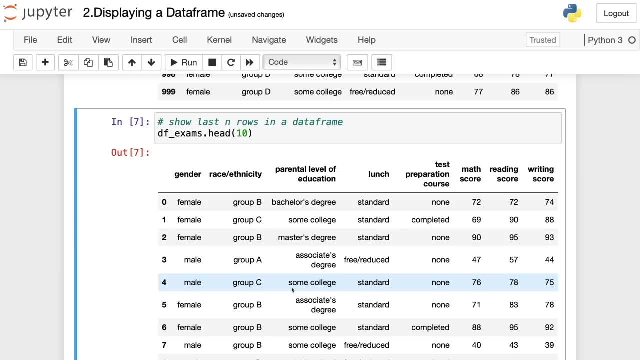 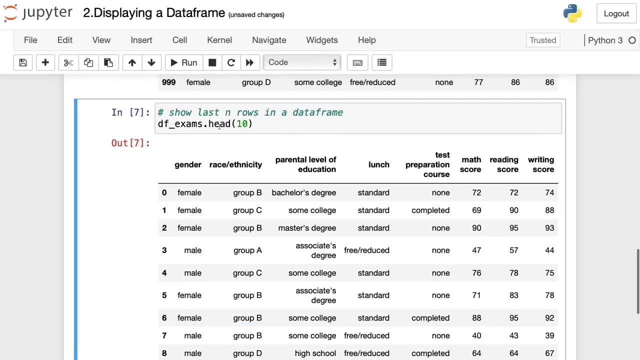 parentheses 10.. And now we run this and I scroll down here and we can see that the first 10 rows are here And we can do the same with tail. So here I write tail And, as we can see, the last 10. 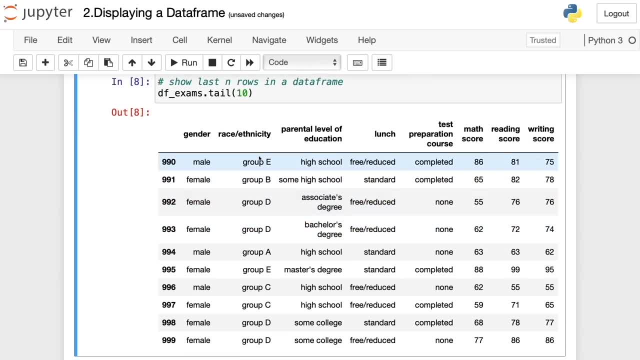 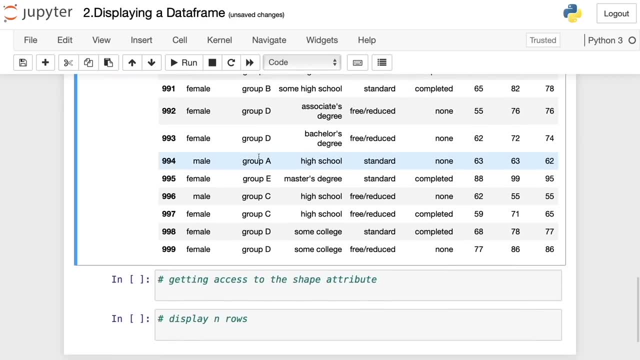 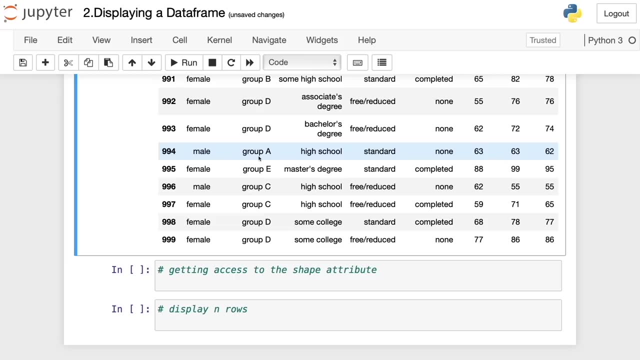 rows are displayed here, So you can specify the number of rows that you want to display, And that's how you do it. So now I'm going to show you how to display all the rows of this data frame, as you will do it in Excel or in Google Sheets. To do so, first we have to know how many columns. 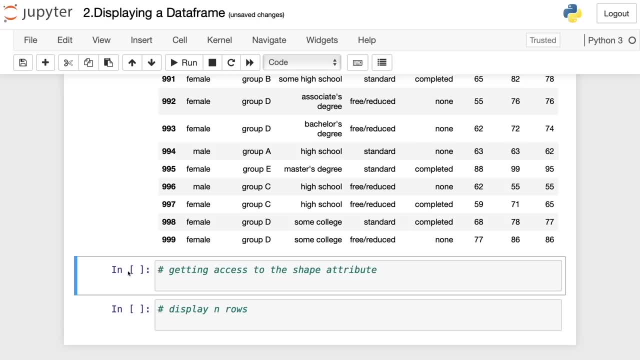 this data frame has. So an easy way to get the number of columns is using the shape attribute. to get the shape, First we write the name of the data frame- So in this case DF, underscored exams- And then to get to this attribute, to get access to this attribute, we use that, that and then the name. 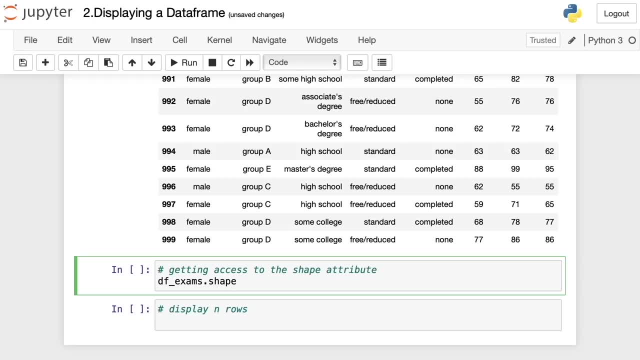 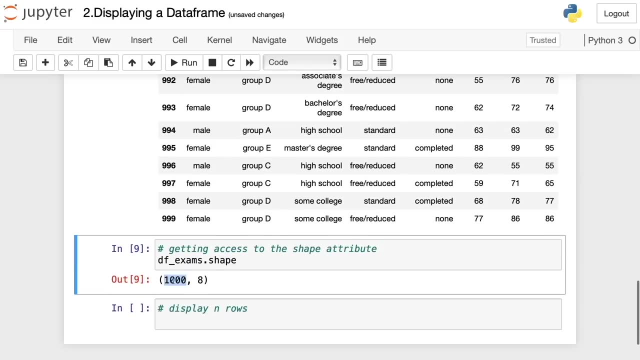 of the attribute, in this case shape. So now we run this and we get 1008.. The first is the number of rows in, the second is the number of columns. So we have 1000 rows. So now to display all the rows. 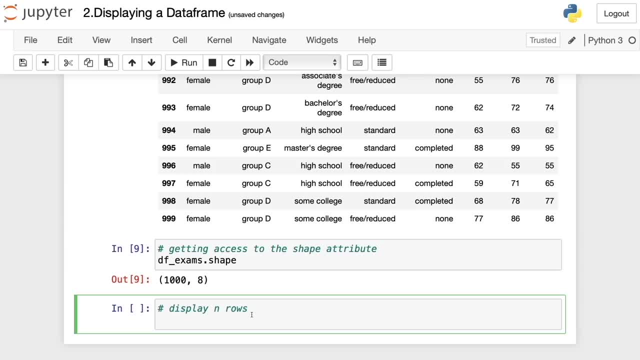 we have to use that set underscore option method. So we write PD that set underscore option And inside parentheses, our first argument is going to be the following: display that max underscore rows. So here we have to specify one more argument, And this is going to be: 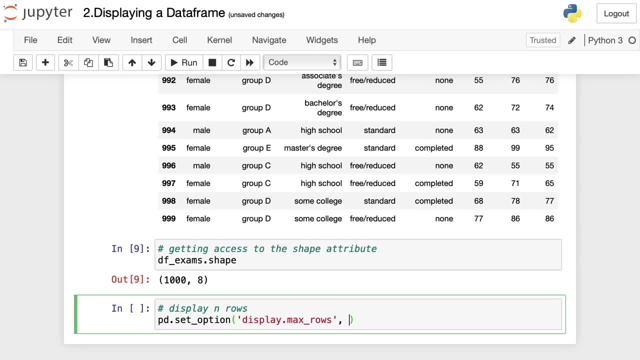 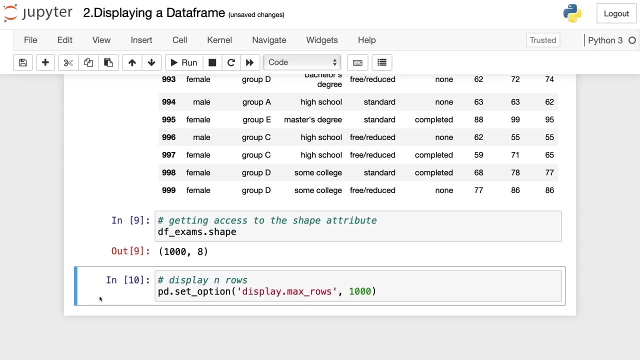 the number of rows we want it to to have. So here it's 1000, because we have 1000 rows And we run this And, as you can see here, nothing happened, because we only modified the default behavior of pandas. So if we want to get the data frame, we just press Enter. 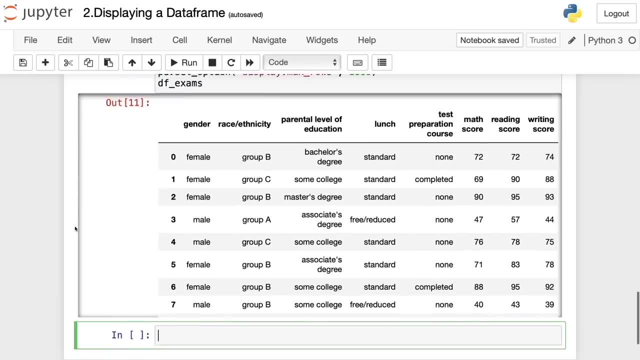 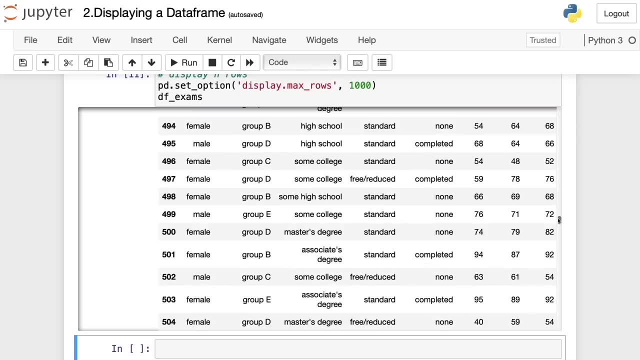 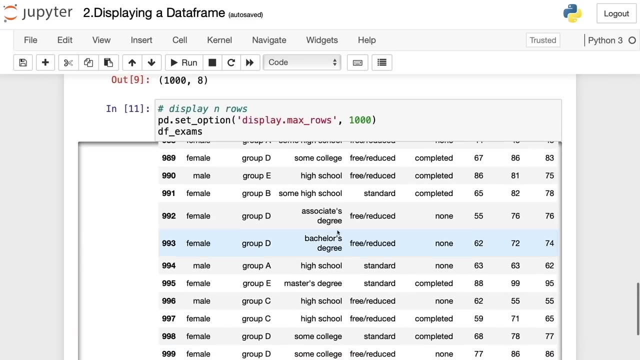 and execute this data frame. I'm going to scroll down in here. as you can see, here there are all the rows of this data frame. So I'm going to scroll all the way down here And, as you can see, it says 999.. So all the rows are here displayed And that's it for this video. 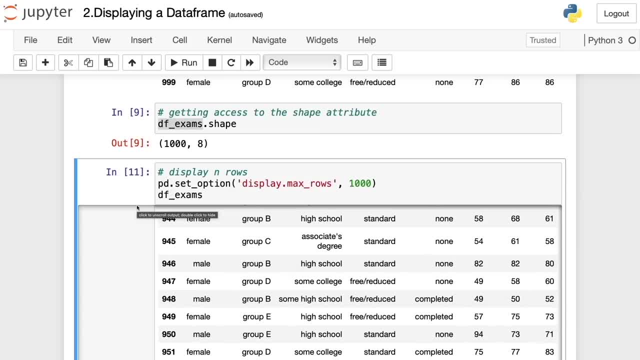 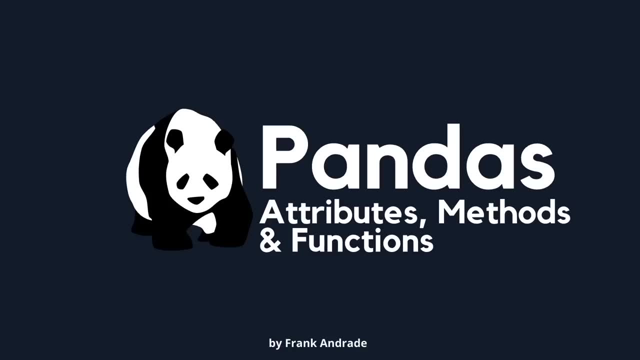 In the next video I'm going to show you the different attributes, methods and functions dataframe has in pandas. Welcome back. in this video we're going to see some basic attributes, methods and functions that we can use in pandas, But first let's learn what are each of them. 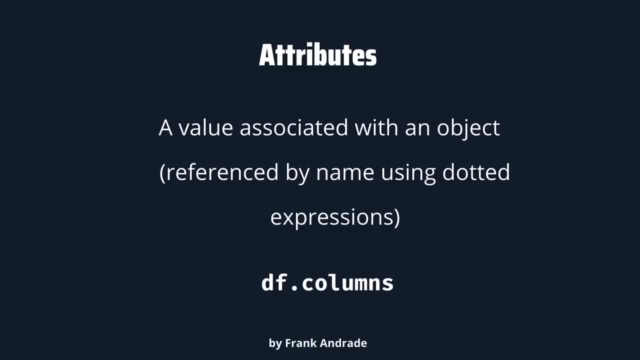 So first, attributes are values associated with an object And they are referenced by name, using dotted expression. So to get to an attribute we have to use the dot sign. So for example, below you can see that we have a data frame named DF. And to get to the columns, 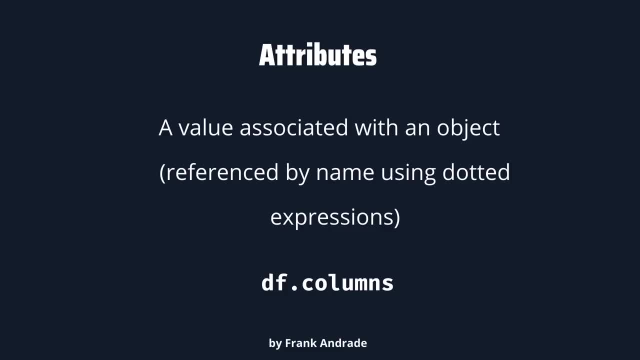 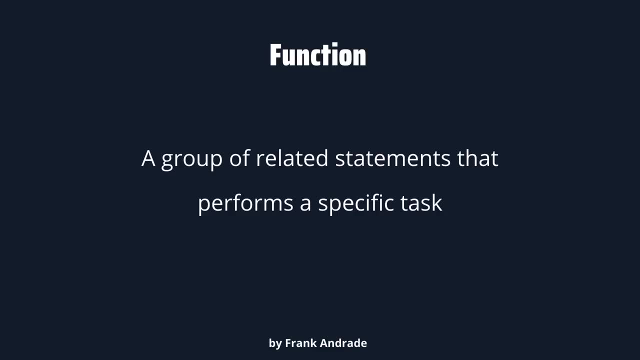 we have to use that, that columns, So columns, it's an attribute And that's how we get this attribute of this data frame. So now we have a function. a function is a group of related statements that performs a specific task. So we've seen functions before in Python we've seen some. 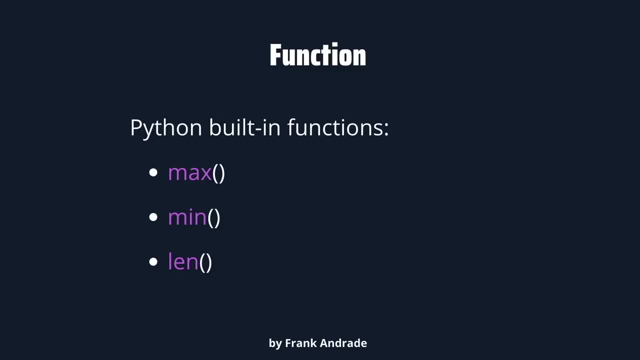 Python built in functions like the max, that gets the maximum value of a list, or mean, that gets the minimum value, or length, that gets the length of a list. So those are some Python building functions that we can use in pandas too. And finally, methods are functions which are defined inside a class body. So we 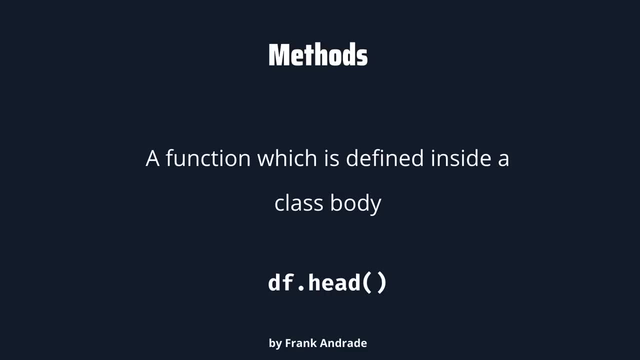 haven't talked anything about classes because it's not the main topic in this course. So just keep in mind that functions are inside a class. So when the creators of pandas build pandas, they use many classes And those functions inside some classes are known as methods. So, for example, below you can see: 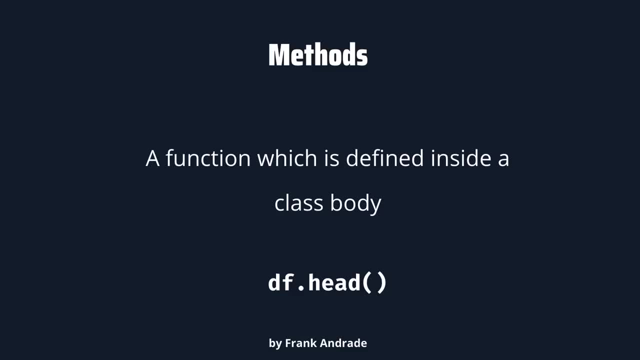 the head method And we've seen also the tail method and some other methods so far. as a rule of thumb, when we use methods, we have to write the parentheses, But when we want to get access to attributes, we only write that, that and the name of the attribute. 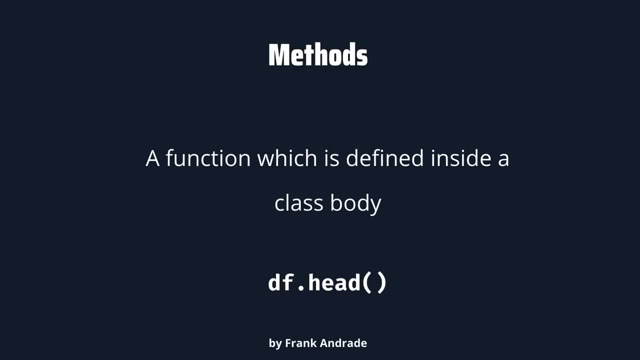 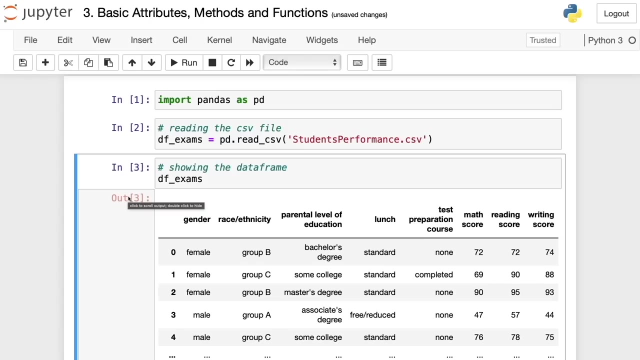 So the methods? it's with that in parentheses and the attribute is with only that in the name of the attribute. So enough talk, Now let's write some code in Jupyter Notebooks. So here we're going to use the same CSV file we use in the previous video And we import pandas as we did. 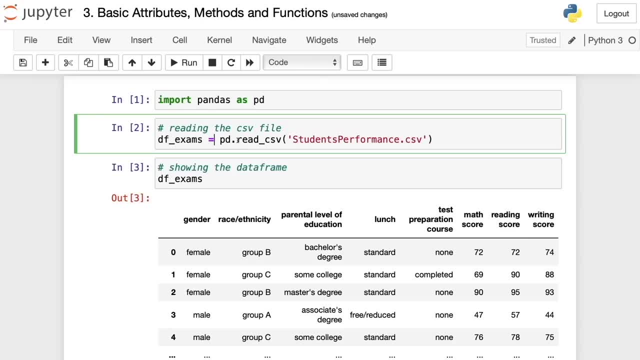 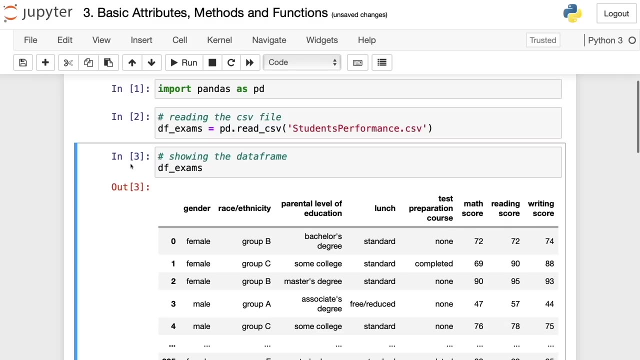 before. then we read this CSV file with the read underscore CSV method, And now we show the data for simply by writing the name of the data frame. So we've seen this before. I'm just reminding you, and now we'll see some basic attributes, methods and functions that we can use in pandas. So first, 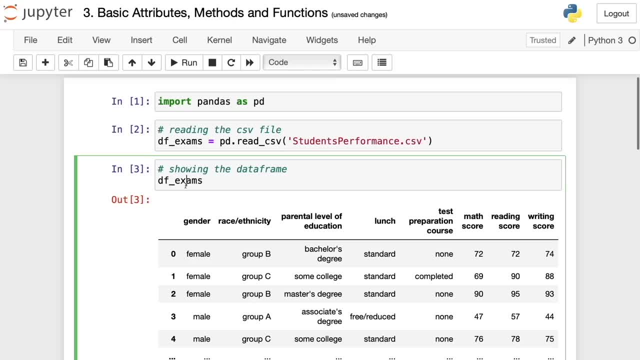 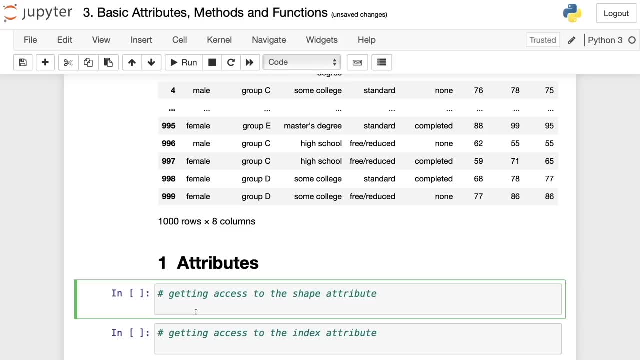 let's check some attributes of this data frame. So first I'm going to copy the name of the data frame And now let's check. So the first attribute it's going to be the shape. So we've seen this before, I believe. And to get to the attribute, we write the dot and then we write the name of. 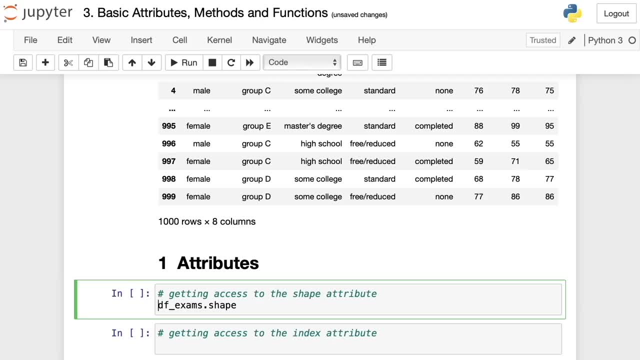 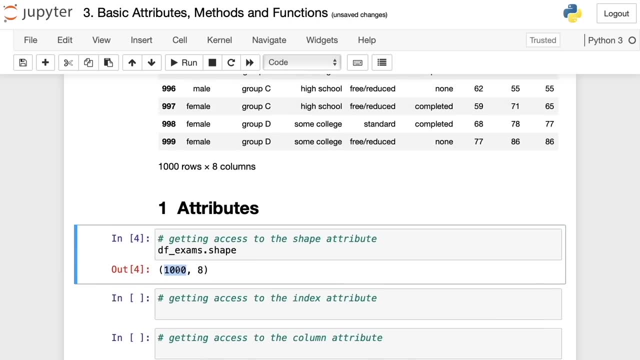 the attribute. So it's shape. So DF exams that shape and we get the name of the attributes. The first is the number of rows And the second is the number of columns. So let's go to the next attribute. The next attribute is going to be the index attribute And, as you might expect, 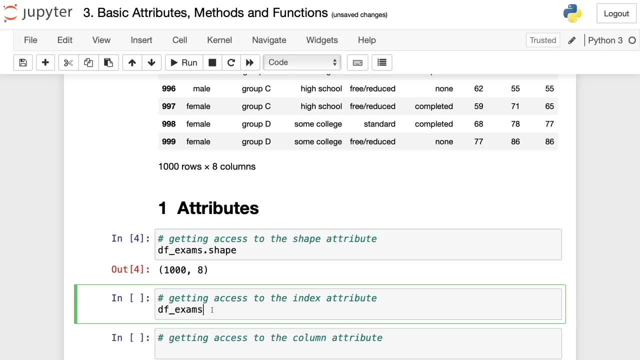 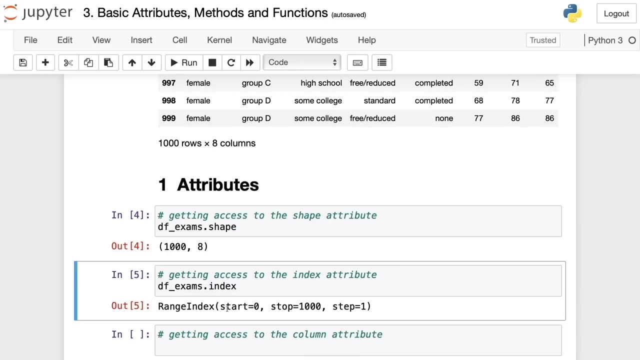 we have to write only the name of the data frame, Then that and now index, And this is how we get the index of this data frame. So, as you can see, this has some form of range. a range, as you might know, has three arguments And actually, 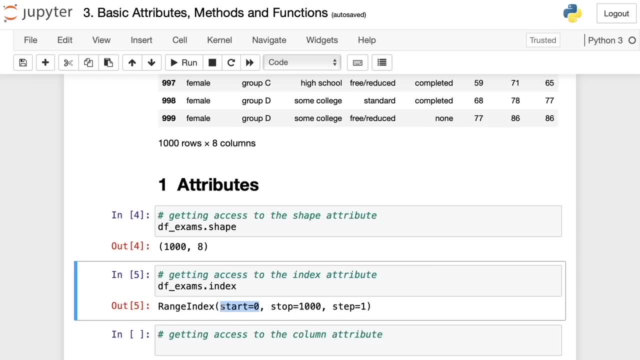 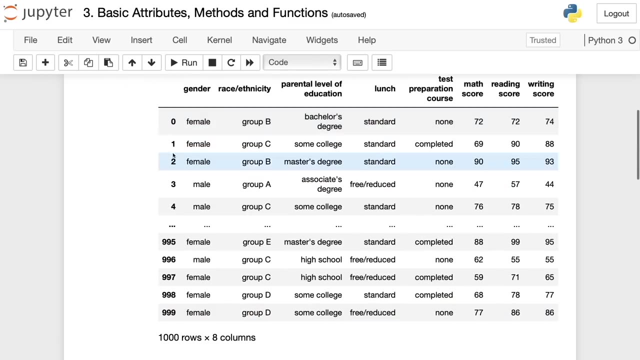 two are necessary. The first is the start, in this case starts in zero, And the second is the stop, So the last element, and stops at 1000.. So this is true because here my data frame starts with zero and and finishes with 999.. Well it's. 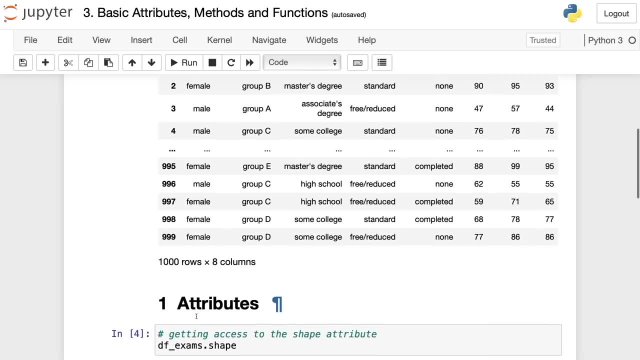 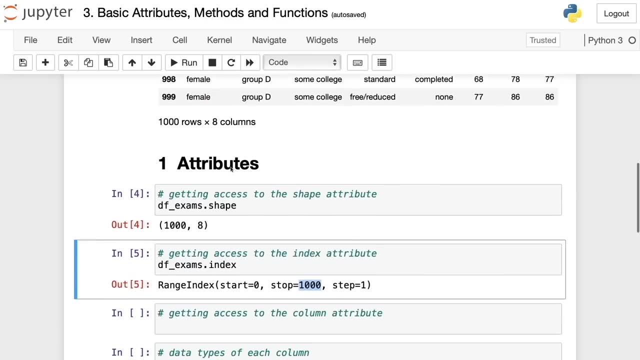 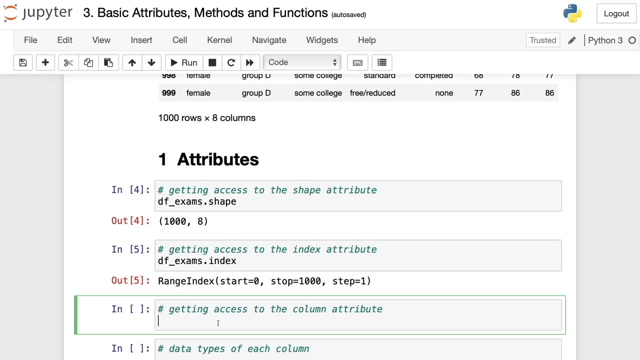 1000, because tops one before 1000.. And here it increases by one, so 012, and three and so on. So the step is one. So this is my, my index attribute. So now let's continue. And now let's get access to. 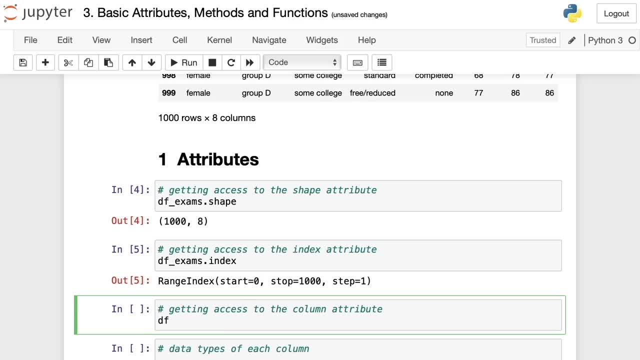 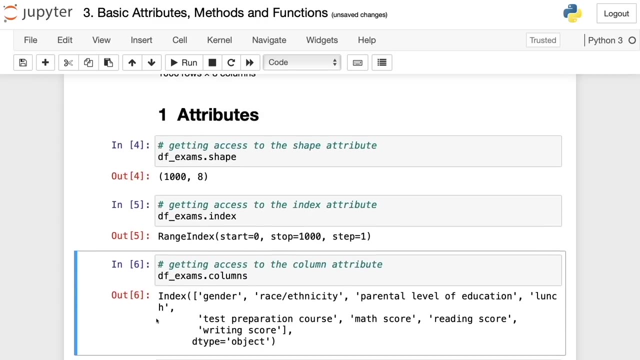 the column attribute. So to do so, we write the name of the data frame And then we write the name of the attribute, So in this case column, and it has to be written with s, So in plural. so we run this and we get the name of the columns. So as you can see, here we have eight columns: the gender: 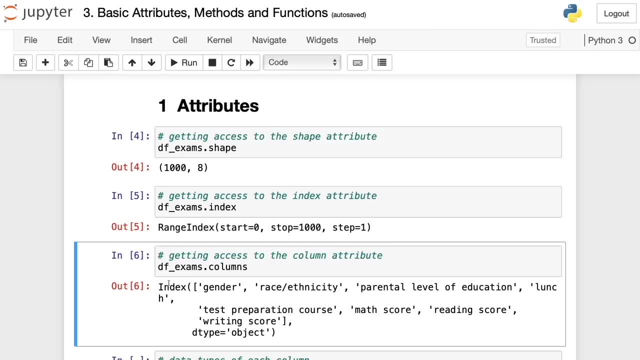 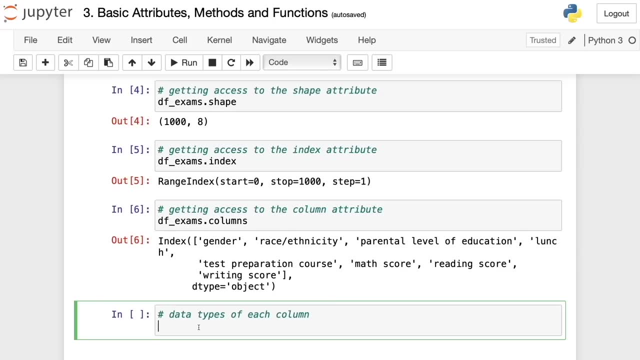 race, ethnicity and so on. And we can use this attribute even to modify the name of the columns. but later and now let's see how we can obtain the data types of each column. To do so we have to use the D types attribute. So we write well the name of the data frame again, and then D types. 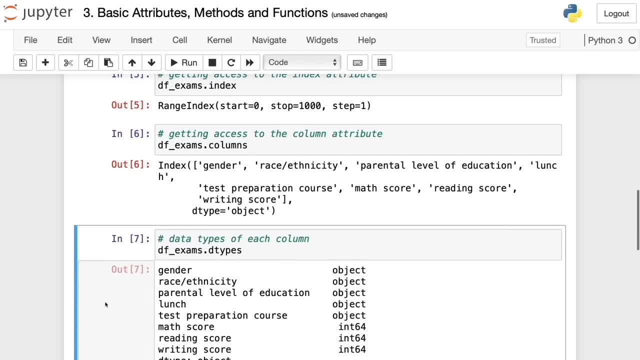 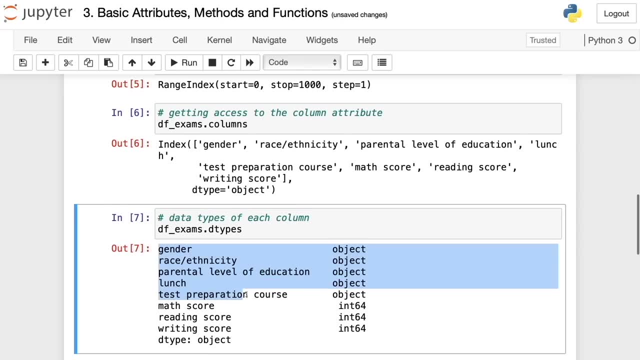 And this is gonna give us the type of each column. So the gender is object And actually, from the gender to the test preparation course, we have two types of objects. while the math score, reading score and writing score are integers. So 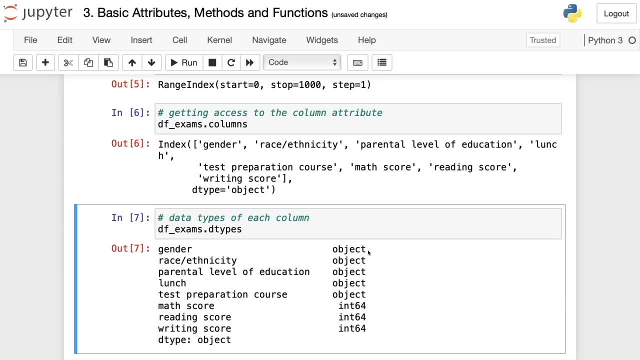 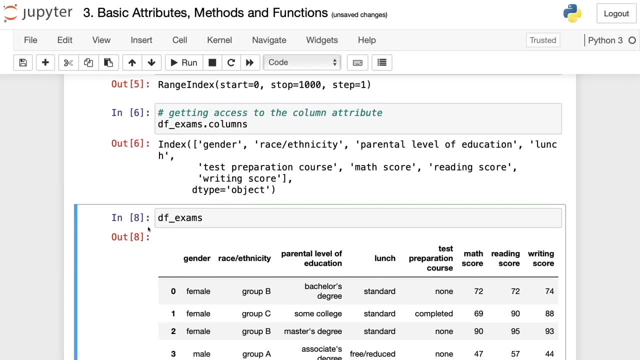 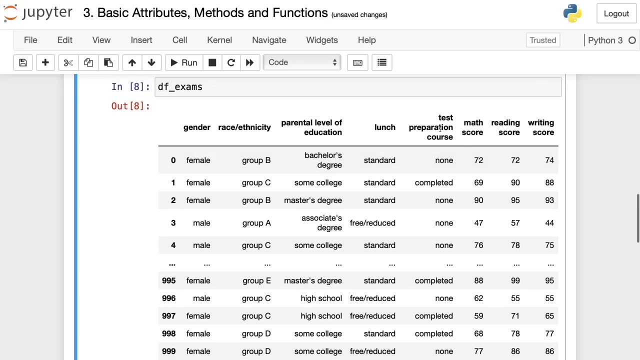 numbers by default. anything that says object is some kind of string. So I'm going to bring this so you can see much better. So here is the data frame again And, as we've seen before, from gender to test preparation, has that type object And, as we can see here, all of them are strings. 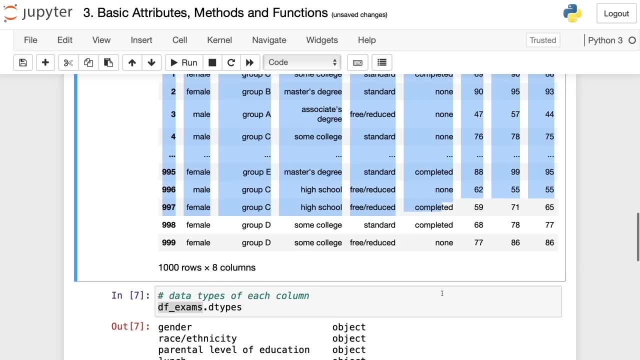 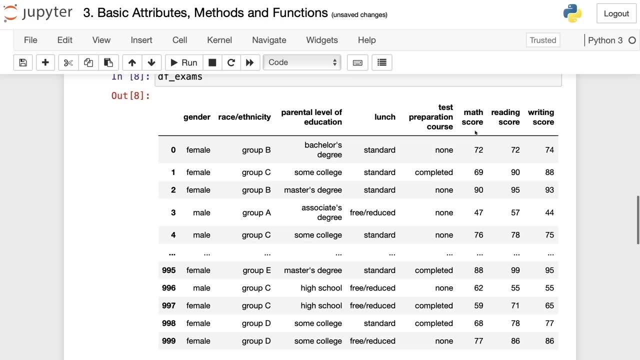 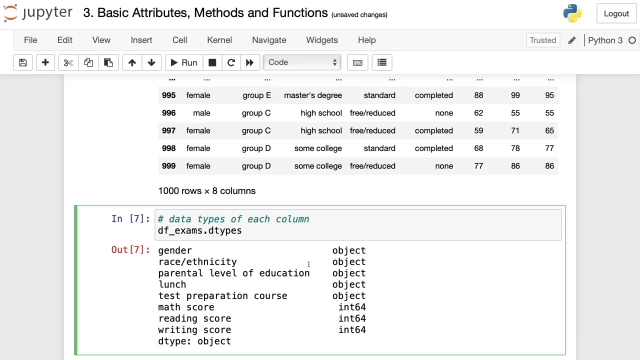 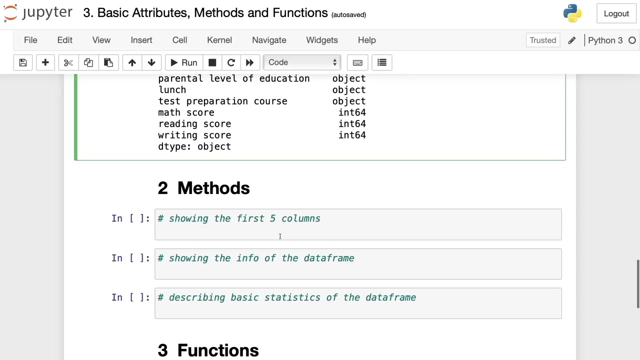 So we can say that objects are the same as strings here, And also anything that has a score here represent some kind of number. So that's why we get here integers, So in 64.. So these are the most common attributes in a pandas data frame. Now let's review some methods. So first let's 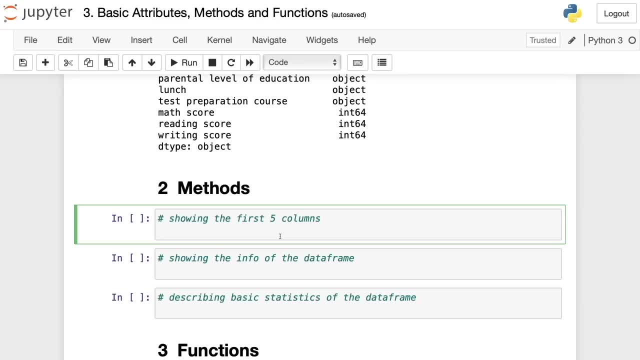 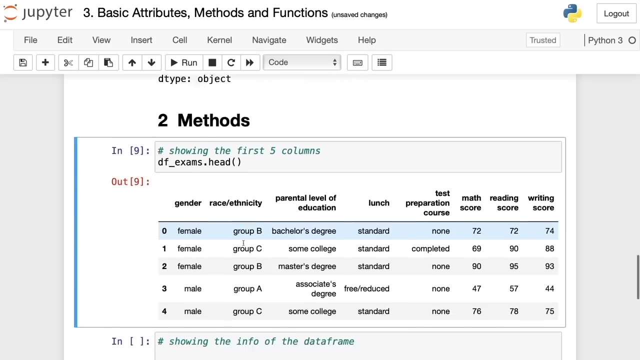 see the first five columns And, as you might know, it's with the head method We only write the name of that attribute, sorry, the name of that data frame, And then we write the head method, So head and parentheses. So we run this and we obtain the first five rows. So we can. 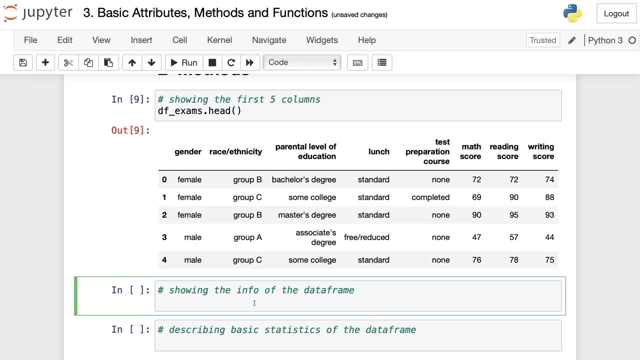 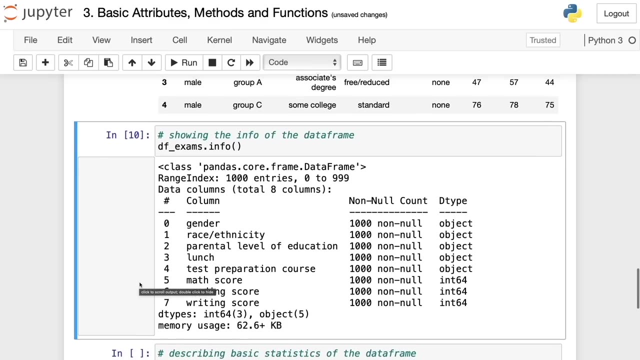 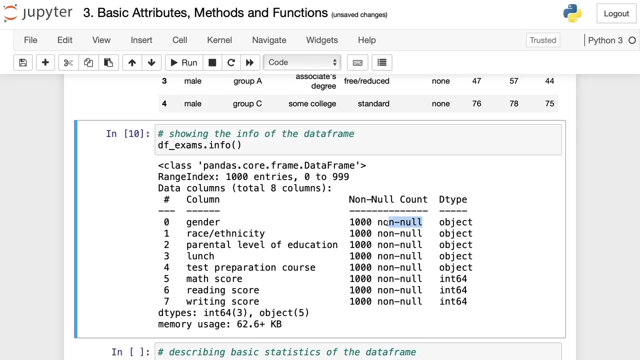 also obtain some summary info, the data frame, by using the info method. So here we write the name of the data frame- info- parentheses- and execute this. So here we have some information about this data frame And here we have again the data type here And also how many rows are non null. So 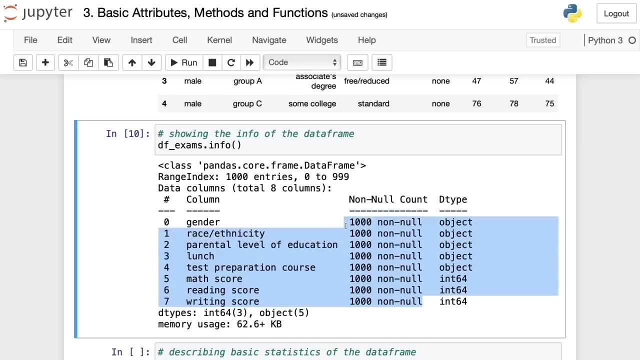 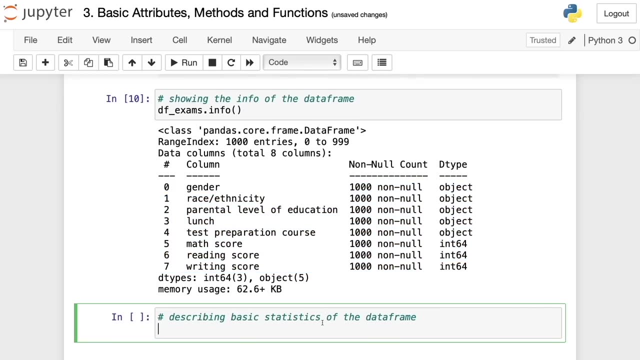 as you can see here, all the data that we have in this data frame are non null, So there isn't any empty data here in this data frame. Okay now, if we want to get some basic statistics of a data frame, we have to use that describe method. So we write the name of the data frame. 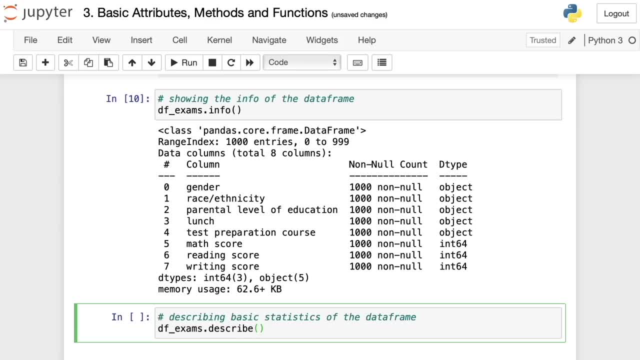 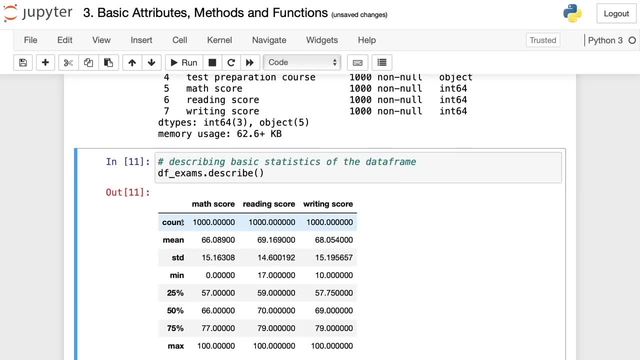 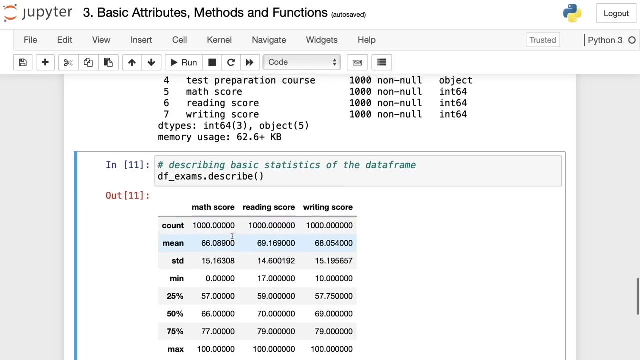 and write describe parentheses- to execute this. So we run this code And we have some basic statistics. So first the count, So this indicates how many rows each column has. So each of them have 1000 rows. then we have the mean. So it's basically they assume each of the data here that 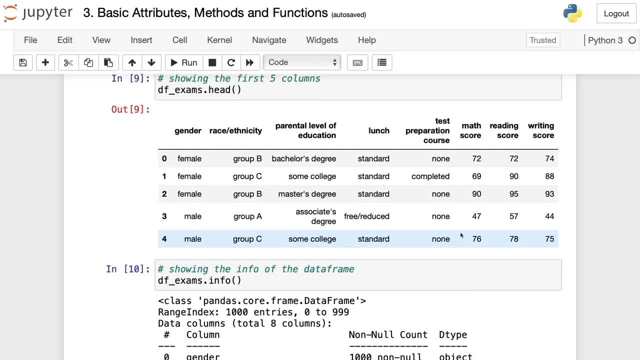 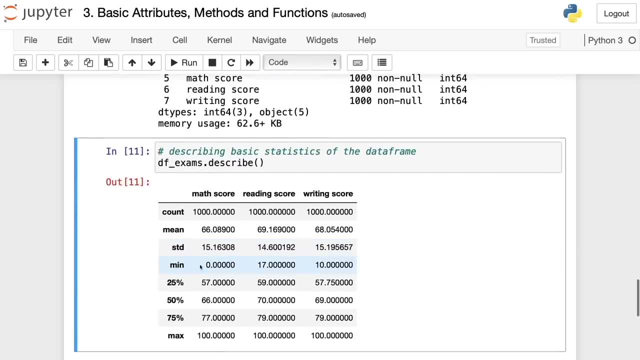 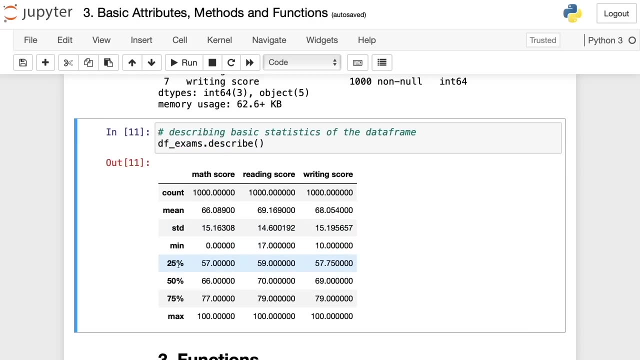 numeric data divided by 1000, because there are 1000 rows- then the standard deviation, the minimum value. for example, in math score the minimum value was zero, then 25% represents the percentiles. So this is q1, 25%, q2 is 50% in q3 is 75%, Then we have the maximum value on each score. 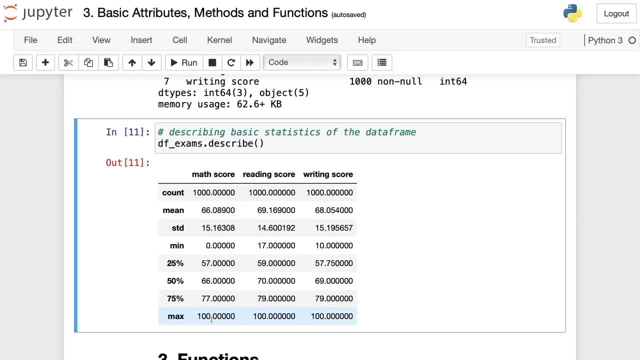 on each exam And we see that the maximum score is 100 on each of them. So that describe method is a useful method whenever we want to get some basic statistics of the data frame, especially of the numerical data that we have in our data frame. Okay, now let's see some. 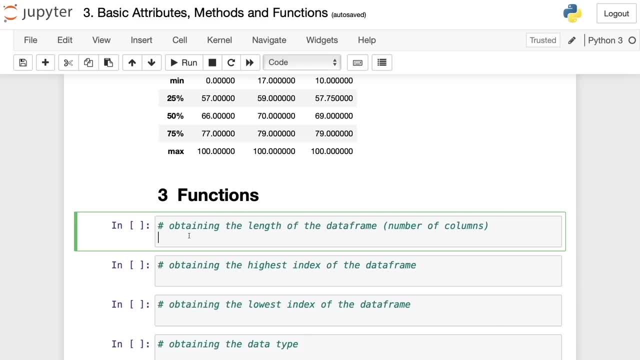 functions that we can use In pandas. We can use some built in functions that Python has in pandas, For example if we want to get the length of a data frame. So, for example, if we want to get the length of a data frame, we can. 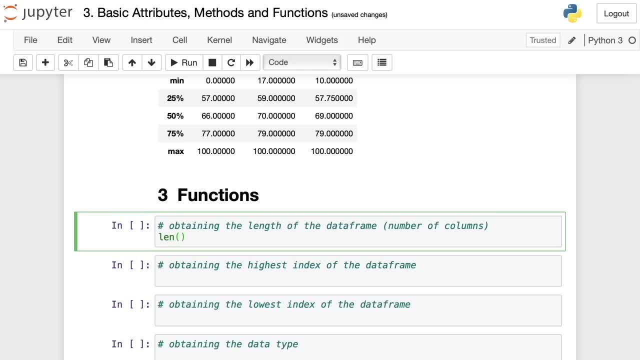 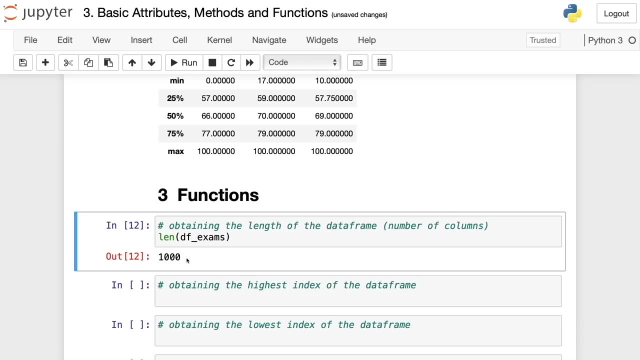 use a data frame. we only have to write land and then, inside parentheses, the name of the data frame. So we run this and we obtain that the length of this data frame is 1000.. Actually, the length of a data frame indicates only the number of rows, So here I made a 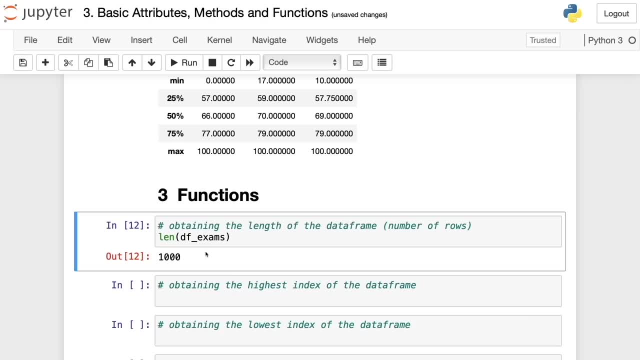 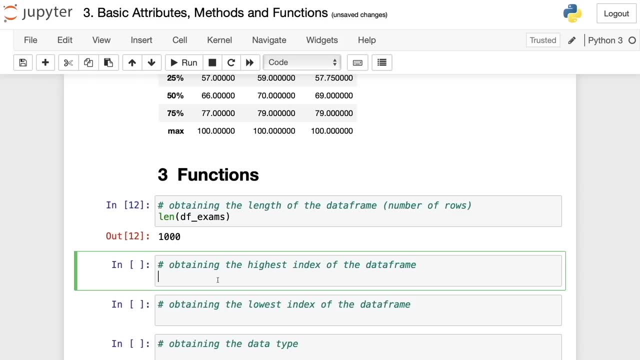 mistake is rows, And this is how we obtain the number of rows of data frame. So also we can use other built in functions that Python has, Like the max function. So we write max, then the name of the data frame we run In this. 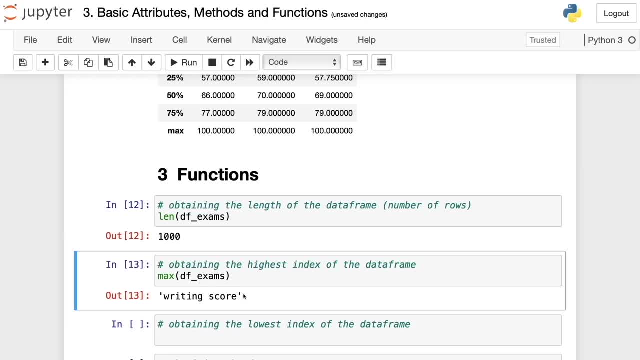 case, we didn't get anything, anything meaningful, because we get like a string. But if we write here the index and we write max, as you might remember, if we use this, this attribute, we're going to get the list of index. So if we use the max function, we're going to get. 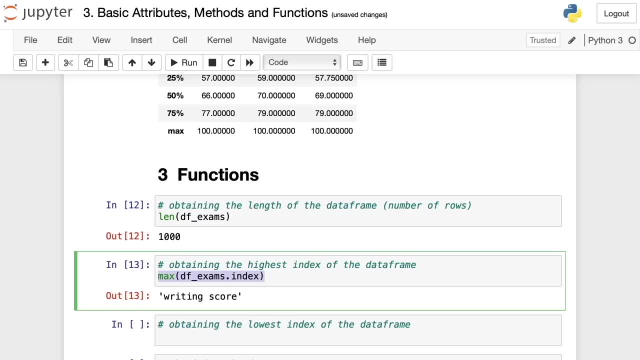 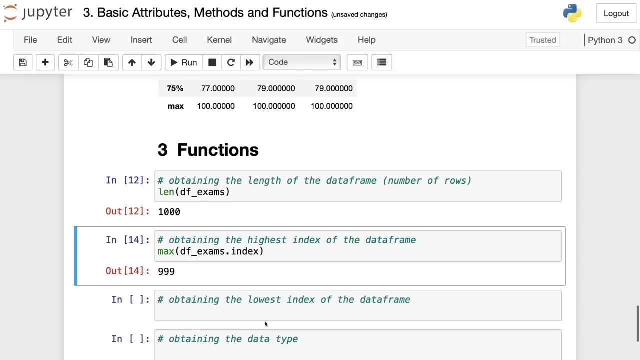 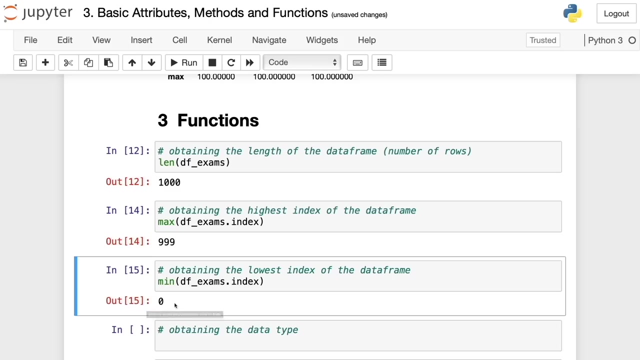 the maximum or the highest index here. So run n is 999.. So we can also get the lowest index of a data frame. we only have to copy this, And instead of writing the max function we write min. So in this case we get that minimum index n is zero. So now we can obtain. 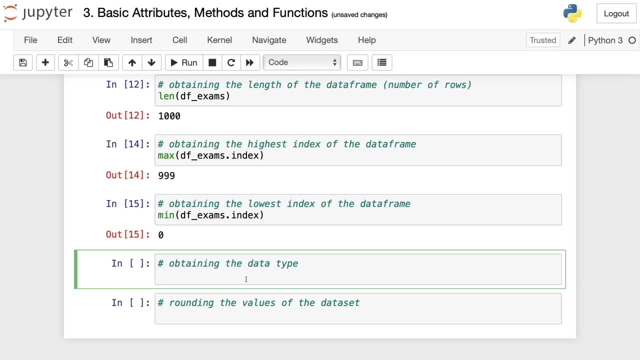 the data type Of the data frame. Well, the data frame has a data frame type, but we can verify that using the type function. So we write type. then, sorry, write only the name of the data frame And we run. So here, as you can see, the type of this object is a data frame, And 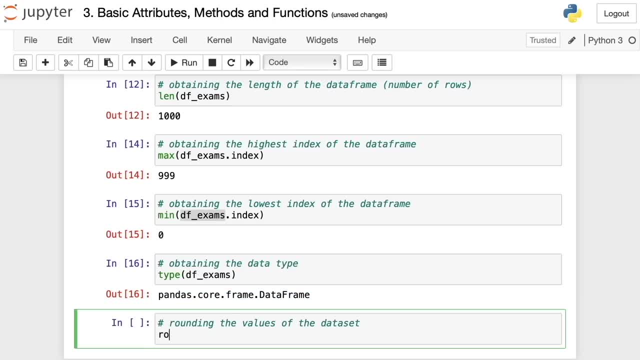 finally, we can use a common function, that is the round function. So we'll write n, we'll write only round, And this has two arguments. So, first, the object that we want to run, and in this case is our data frame, And the second argument is the number of decimal points. 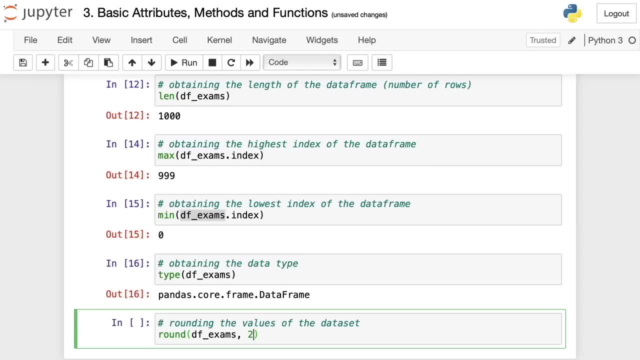 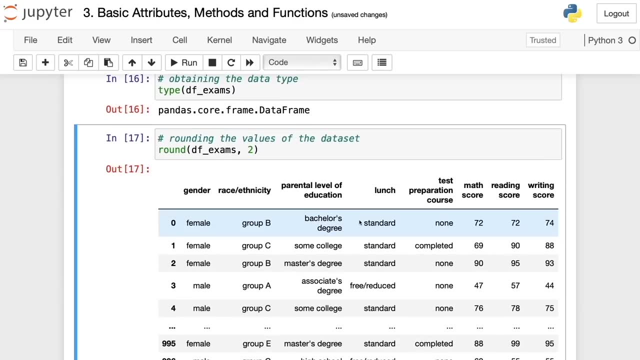 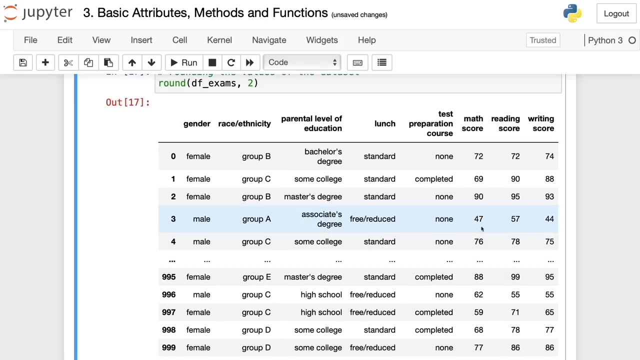 that we want to have. So in this case I want two decimal points. So we run this And we're not going to get this number of decimal points in this particular example because the numerical data we have here integers, so they are not floats, So this doesn't have any effect. But if you have a 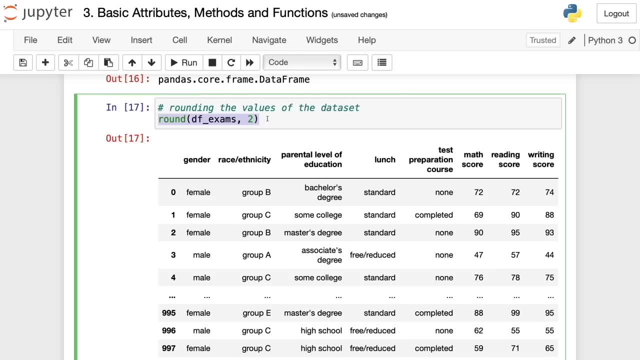 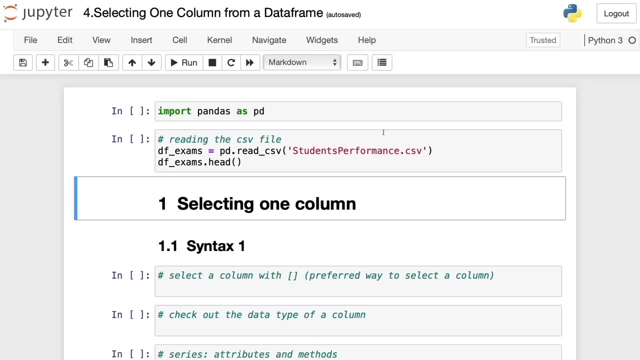 data frame with float numbers. you can round those numbers using the round function, And that's it. These are the most basic attributes, methods and functions that we will see often in pandas. Alright, now it's time to learn how to select a column from a data frame. 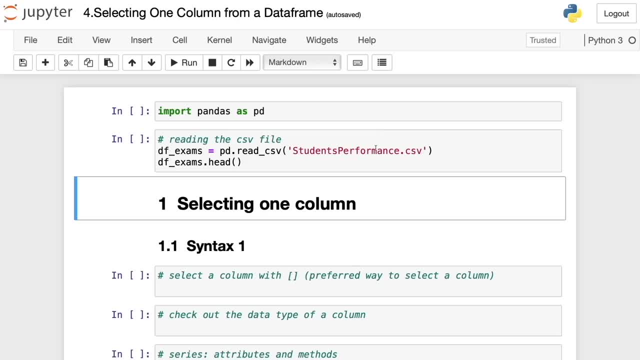 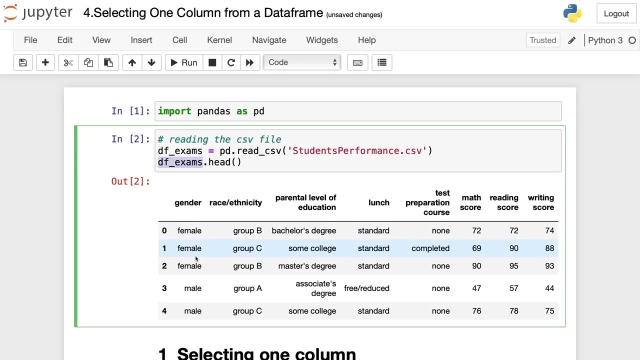 So here I have the same CSV file we've been using in the previous videos. And well, let's import pandas And let's read this CSV file. So I have this in the same data frame And I'm just showing the first five rows. So now to select one of the columns of this data. 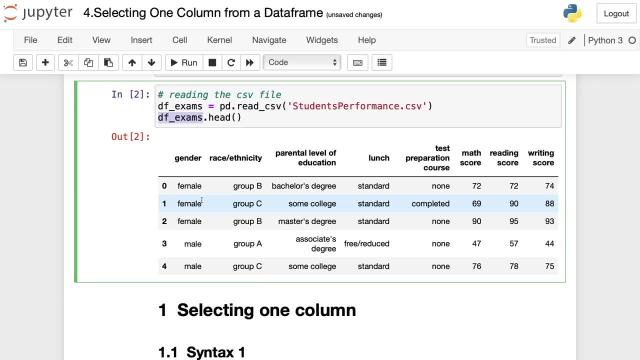 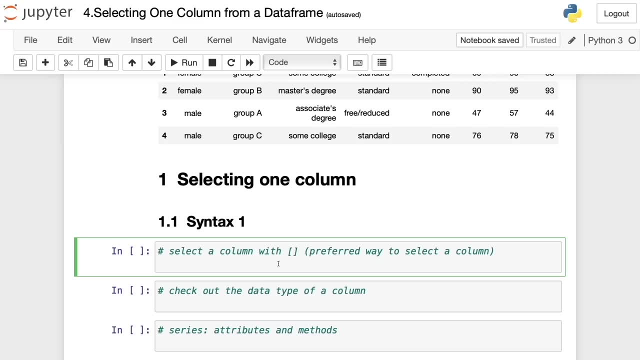 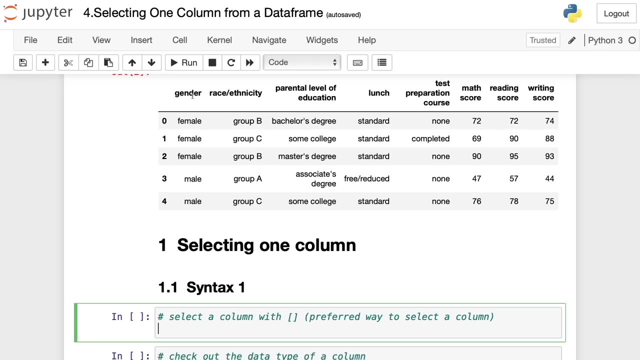 frame. we have two options. So let's see the first option. The first option is using the square brackets. This is the preferred way to select a column in pandas. And let's see how to select the gender column. So the first one here. So the first thing we have to do is to write the. 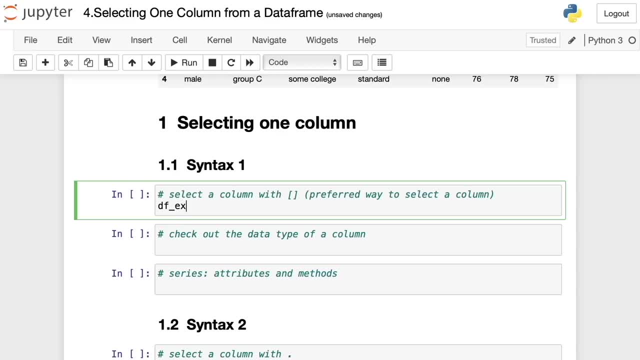 name of the data frame- in this case DF underscore exams- and then open square brackets. So I open square brackets And now we have to write the name of the column. So we open quotes And now I'm going to copy the name. 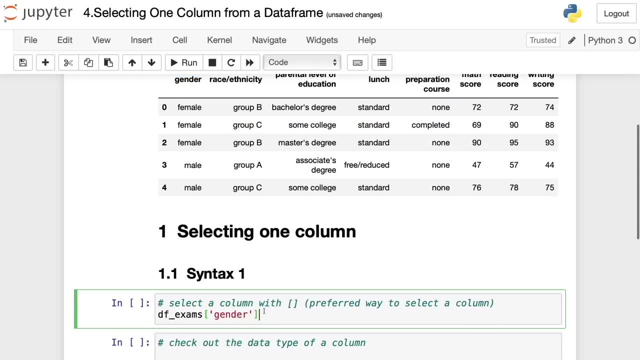 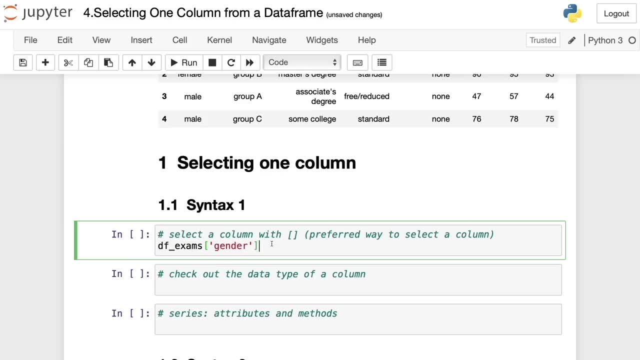 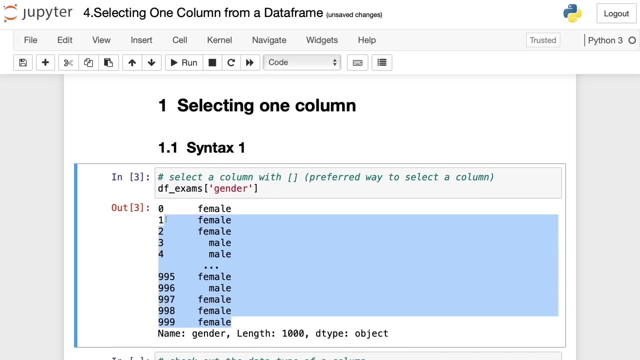 of this column And I'm going to paste it here. So we have here the name of the data frame and then the name of the column we want to select. So now we press Ctrl Enter to run this code And, as we can see, we have the first column of this data frame. So here we have this. 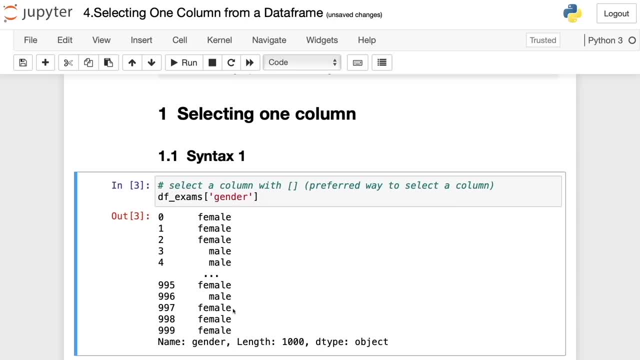 and, as you might expect, this is an array. So this is one d array And, as you can see, once you remove the arrow from the column you get an array. So here's the second array And you output fn d. So remember the first column and now we can add the next column and 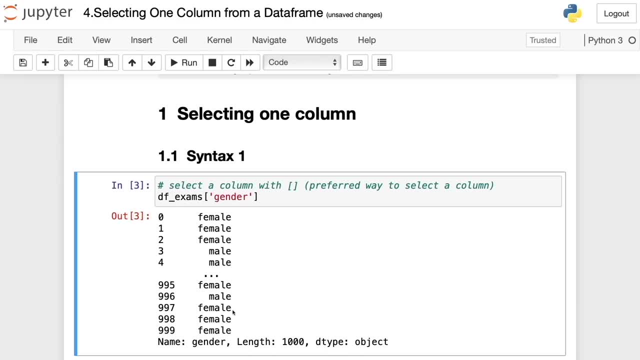 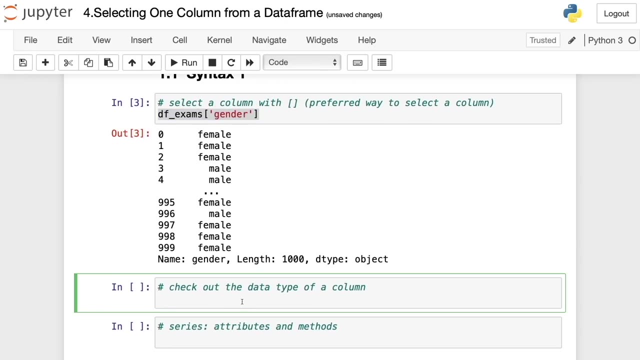 we discussed before in previous videos. one D arrays are serious, So we can verify if this is true. So we can do this with the type function. So I'm going to copy this column, this selection. you know what we're going to do is to use the type function. So we write type, then open. 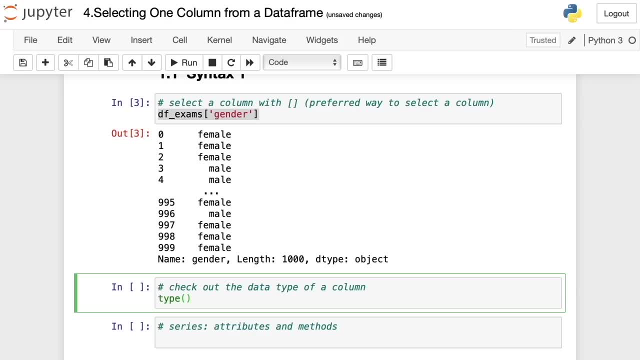 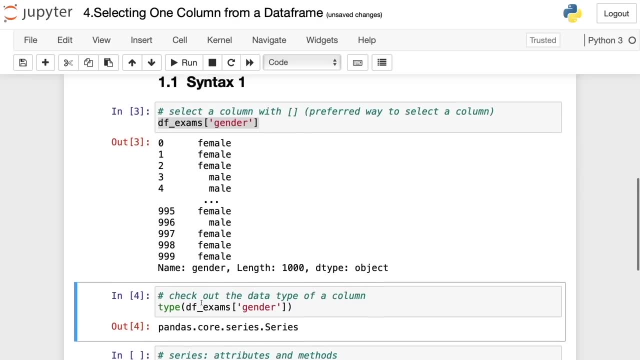 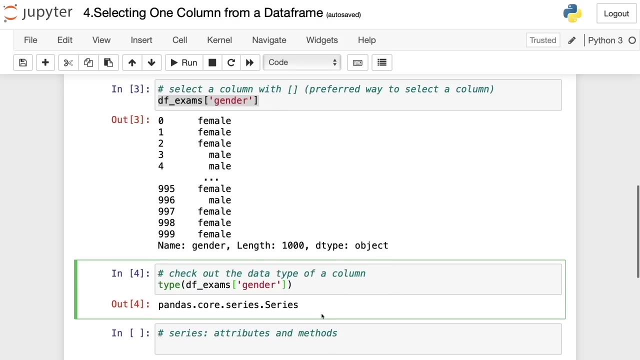 parentheses And then inside parentheses we write the object we want to evaluate. So in this case is this: And now we run this And, as you can see here, we get a series and series. just like pandas, dataframes have attributes and methods, So we can access those attributes and methods And actually 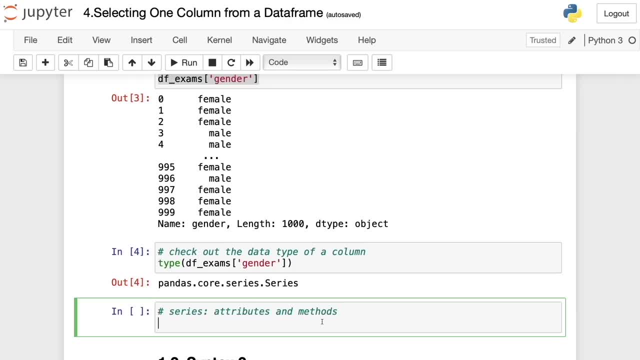 the attributes and methods between a series in a data frames are very similar. So, for example, we can write a series and a data frames. And we can write a series and a data frames are very similar. So, for example, if we want to get the index attribute of this series, we only have to write that name of the 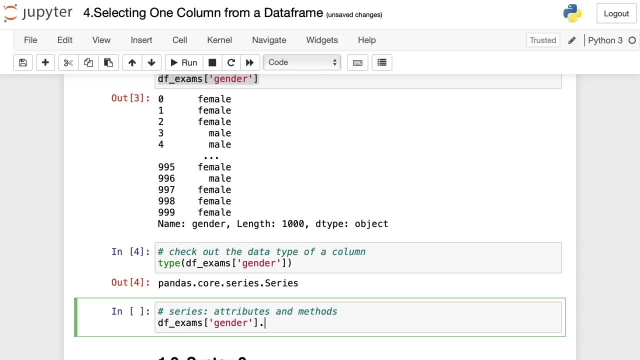 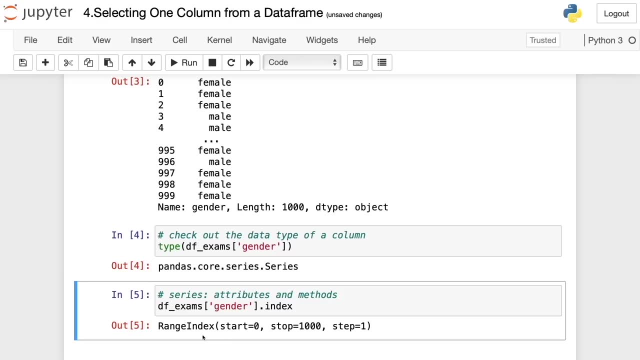 series and then write that and the name of the attributes or index. So we run this and we get this index in form of a range that starts with zero and ends with 1000.. So another method that share pandas in series is the head method. So we can also get the first five rows by 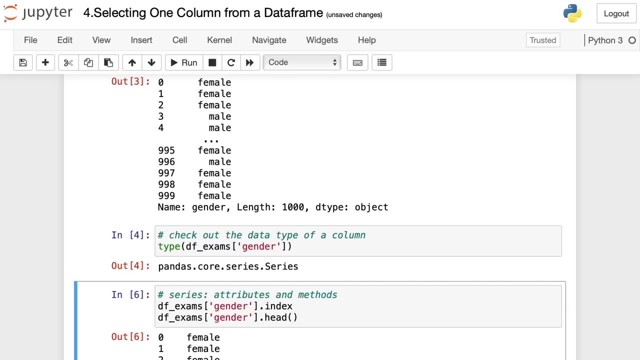 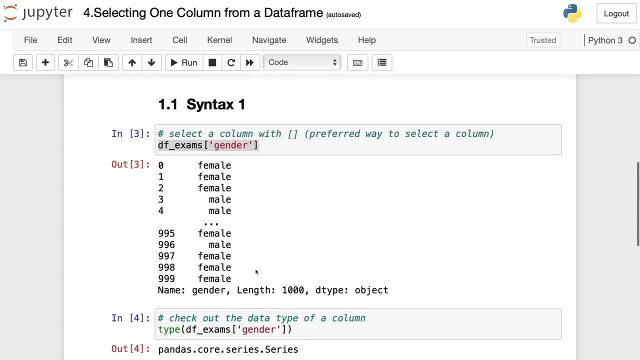 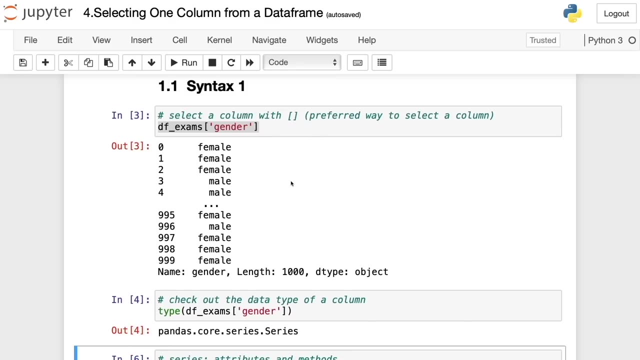 writing that head and parentheses. So, as you can see, here we get the first five rows of this series. Alright, that's it for the first syntax. This is my favorite syntax And actually most people use it because it's the most practical. you know, it's time to see the second syntax to. 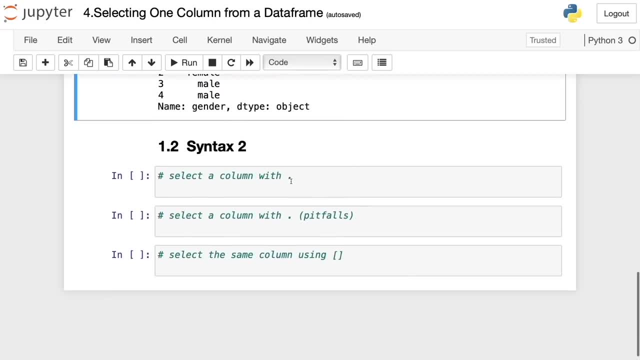 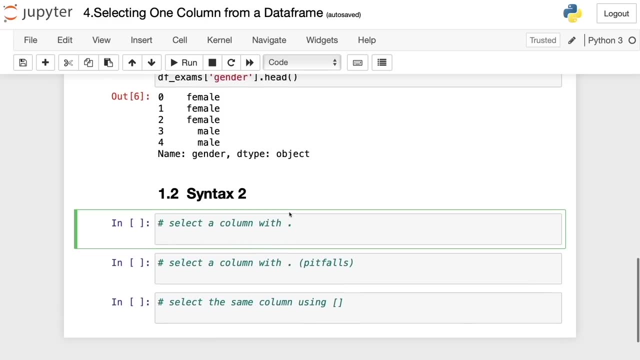 select a column from a data frame. So this syntax involves writing that, that sign which is here. So let's say we want to get the same gender column. So we write the name of the data frame, followed by that and the name of the column. 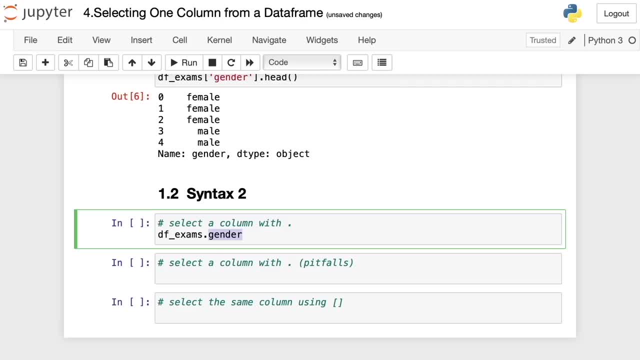 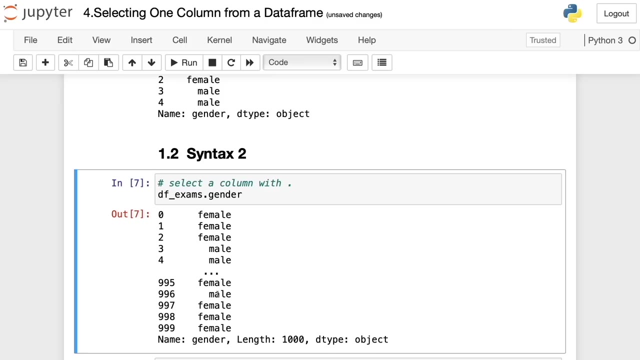 So gender. in this case we don't need to open quotes and we don't need the square brackets, So we run this code and we get the same series. So it's here, And probably now you might be thinking that this is more practical than the first syntax, But this syntax has some pitfalls. So now let me. 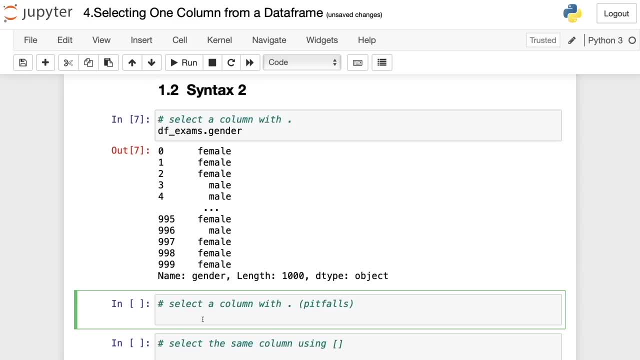 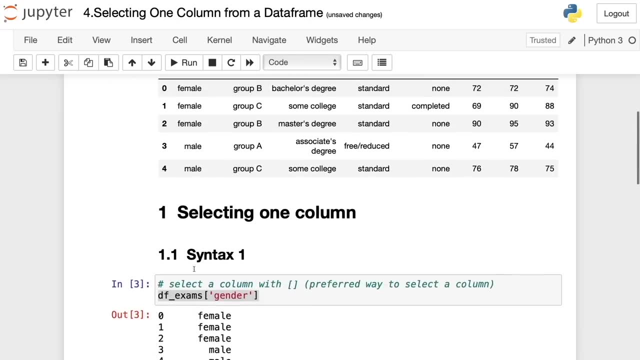 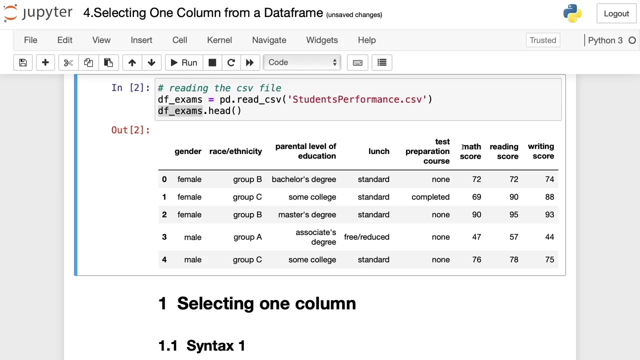 show you here. So what if you want to get one column that has two words, for example? what if you want to get- let me show you here- this column that has as name math score? So now let's try to get access to this column. I'm going to copy this column name and now scroll down. And now let's. 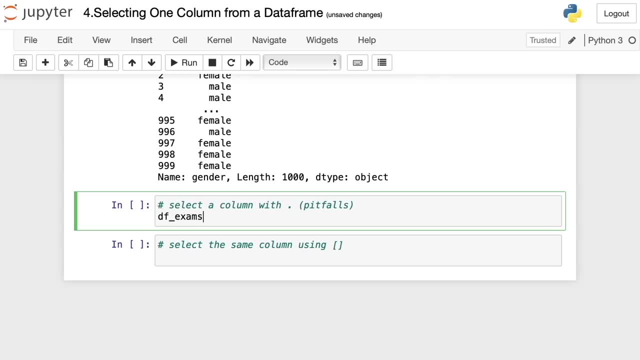 try. So I'm going to write first the name of the data frame and now the dot. So to get access to this or to select this column, we have to write the column name. So this is the column name. But, as you can see, if I run this we get an error because Python doesn't work. 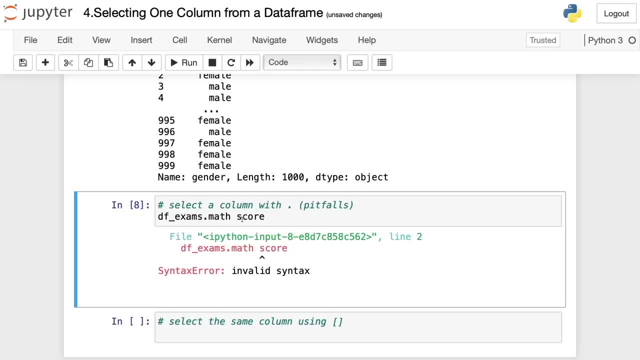 like that. In Python, when we have two words, we usually add an underscore. So that's how Python understands this, that this is a variable. But if it's like this, Python will not understand what you're trying to do. However, if you use the first syntax, so the square brackets- 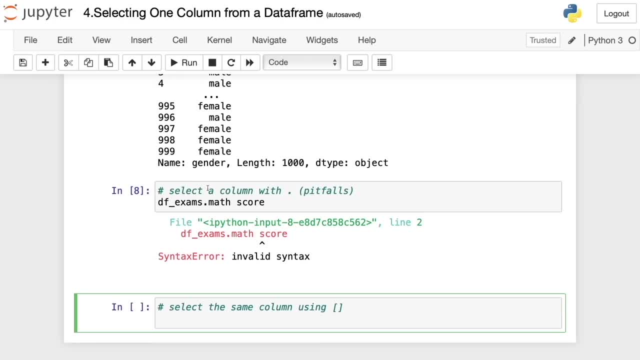 you won't have this problem. So let me show you here. Now I'm going to write this, I'm going to copy and now I'm going to paste it here. And instead of having this only dot notation, I'm going to open the square bracket. So open square brackets and then add the. 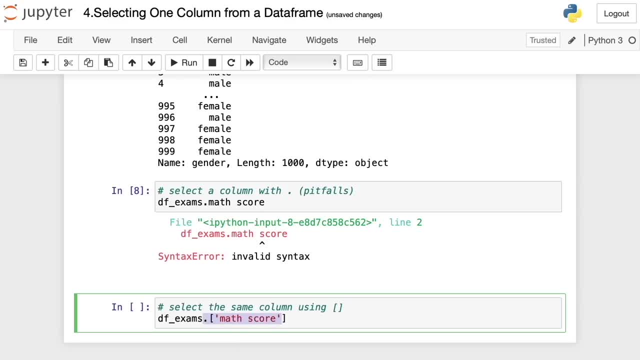 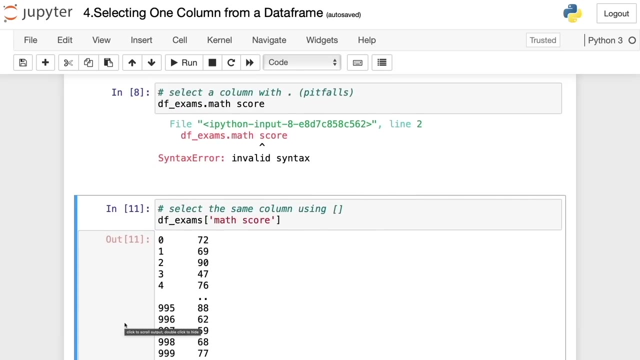 quotes. So, as you can see here, the column names has a string type And now Python know that this is a string And now, if you delete this dot sign and you execute this, you get this column without any error. So this is one of the advantages. 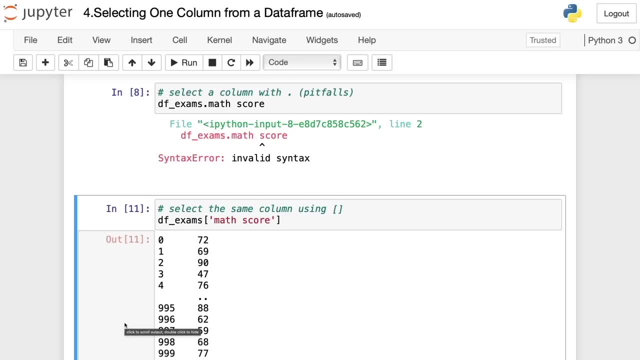 that the square brackets has over the dot sign. And that's it. In this video, we learn how to select one column from a data frame, And in the next one we're going to learn how to select two or more columns from a data frame. 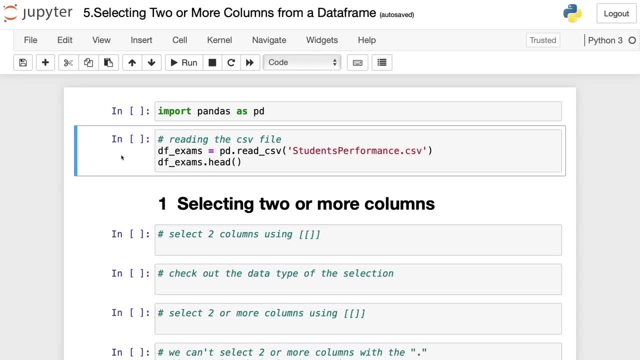 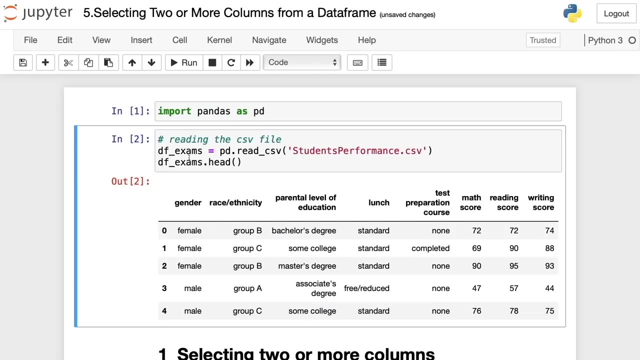 Okay, in this video we're going to learn how to select two or more columns from a data frame. So, as usual, we're going to start by importing pandas and reading the CSV file we've been using so far. So we execute these two lines of code and we get here that data frame. 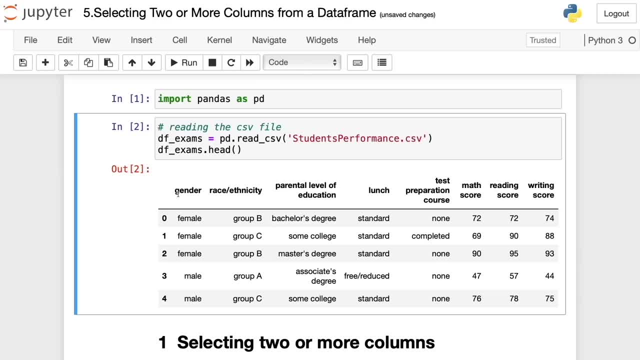 So what we're going to do in this video is to select two random columns from this data frame. So first let's pick some columns. So I'm going to select that gender column and also the math score column. So to select these two columns, we have to 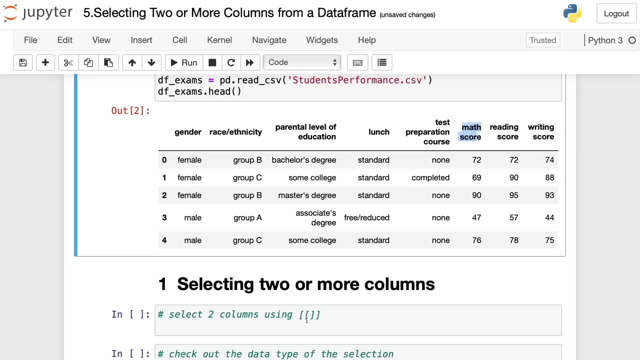 use the square brackets again. So here, in this case, we have to use two square brackets to select two or more columns. So to do this we have to write first the name of the data frame, So it's the F underscore exams. And now we open square brackets, So we write one. and two, two, three, four, five, six, seven, eight, nine, ten, twelve, twelve, thirteen, fifteen, sixteen, twenty, thirteen, fourteen, nineteen, twenty, twenty fifteen and twenty sixty. So we have to column the data file twice. 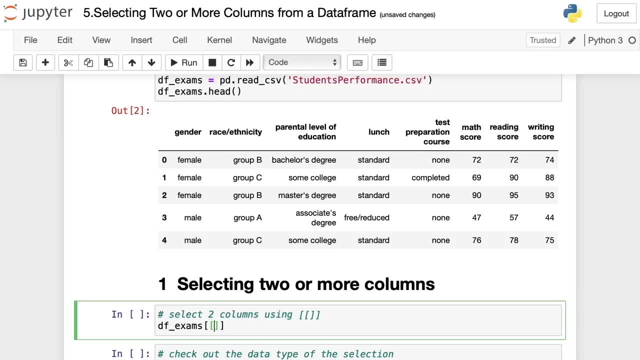 So we have two pairs of square brackets and inside we have to write the name of the columns we want to select. So we said that we wanted the gender column, So we write gender. And the second column that we chose was that math score. So I open these quotes and now we write: 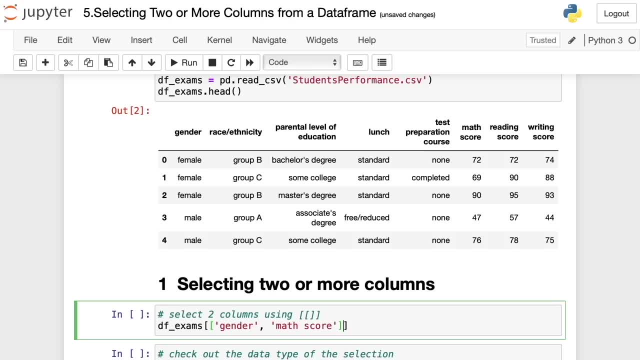 math score. So here I have these two columns And, by the way, the order that we write these columns is the same order that we're going to get that data frame. I mean, we can define the order of the columns inside this square bracket. So 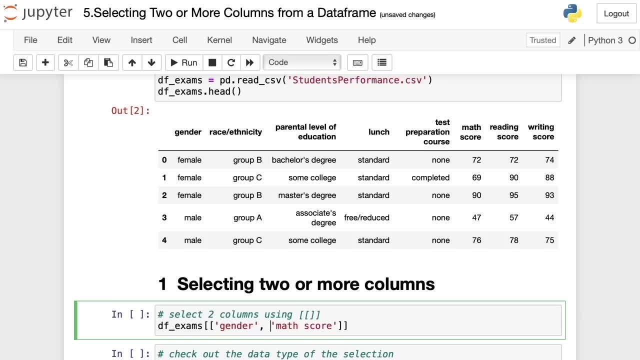 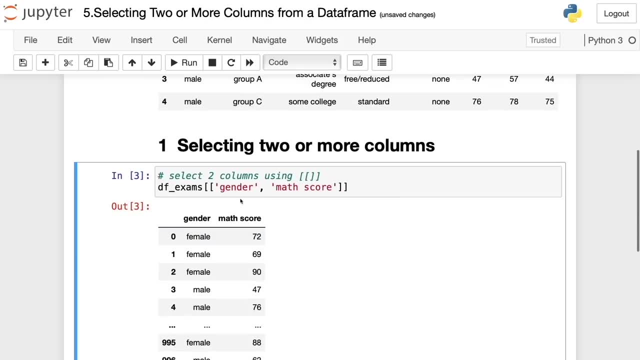 here we're saying that first is the gender column And second it should be the math score column. So now let's run this And, as you can see, here we obtain first the gender column and second the math score column. So here we can see that it's a data frame, and 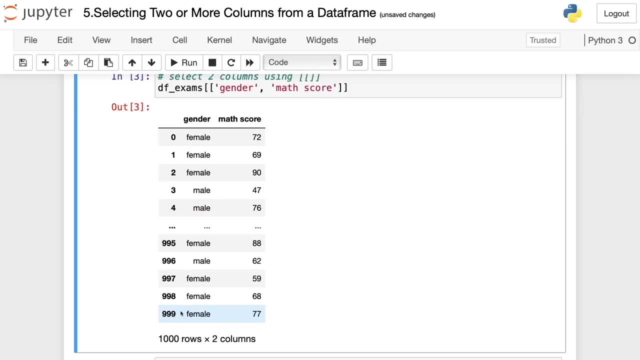 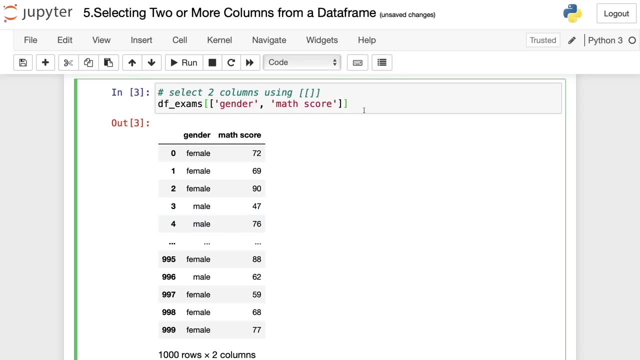 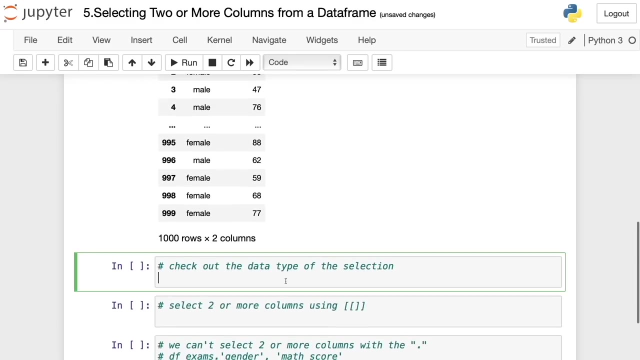 there are 999 rows. So now we can verify that this is actually data frame by using that type function. So let's check if this selection is a data frame. So now I'm going to copy this in here. Let's check out the data type of the selection. So here I paste it, And 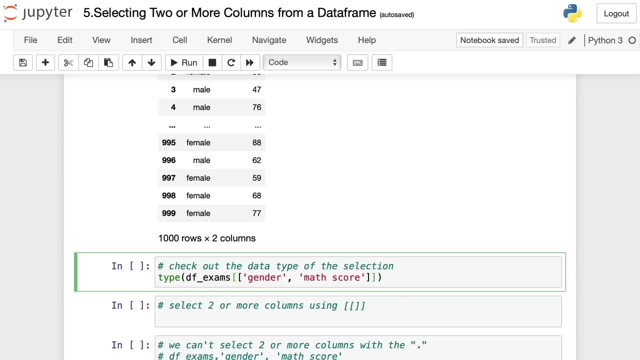 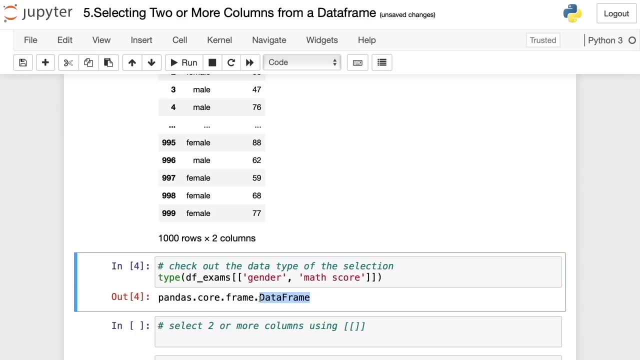 now we use the type function, we open this parenthesis And now we execute this code And, as you can see, here we got that this is a data frame. So here, one little detail I want to tell you is that when we use these two square brackets, or two pairs of square brackets, we're always 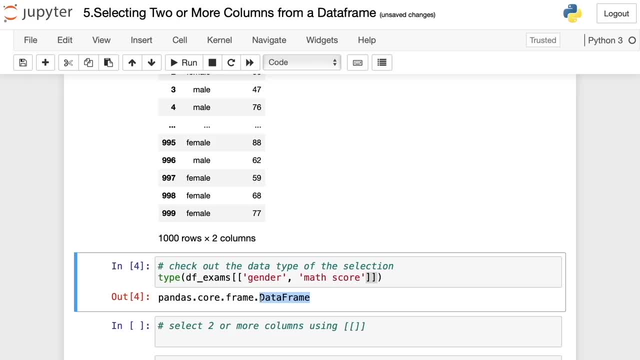 gonna get a data frame. But when we use only single pair of square brackets, as we did in the previous video, we get a series. So one pair of square brackets is for a series and two pairs of square brackets it's for a data frame. 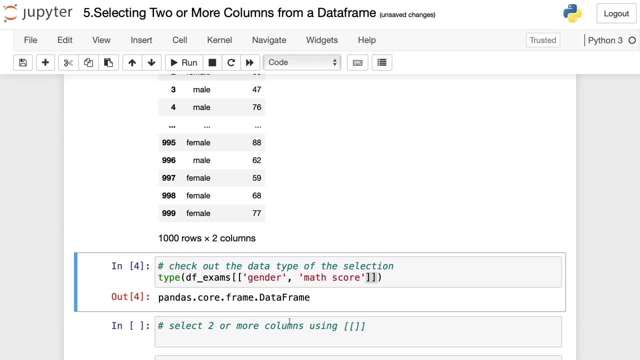 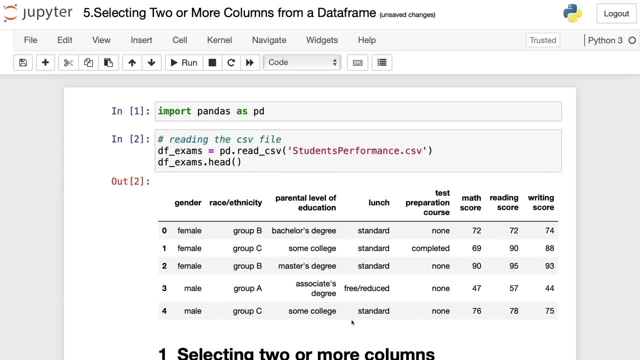 Okay, so to continue with the video, I'm going to select two or more columns using these two pairs of square brackets. So now let's choose the columns that we're going to get. So in this case, I'm going to get that gender column and all the scores that we have here. So the 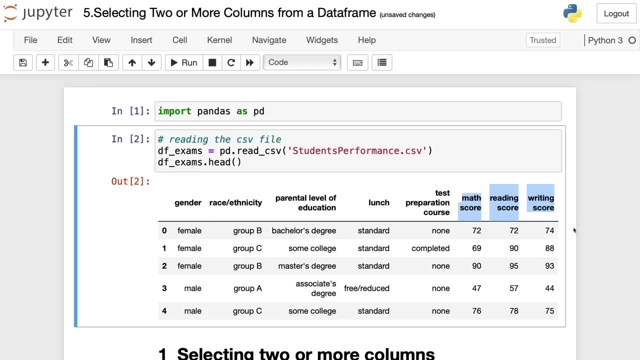 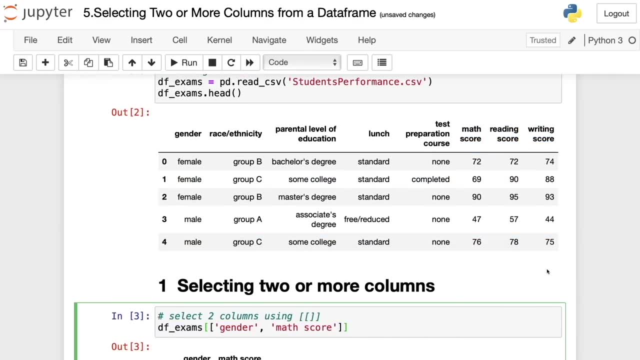 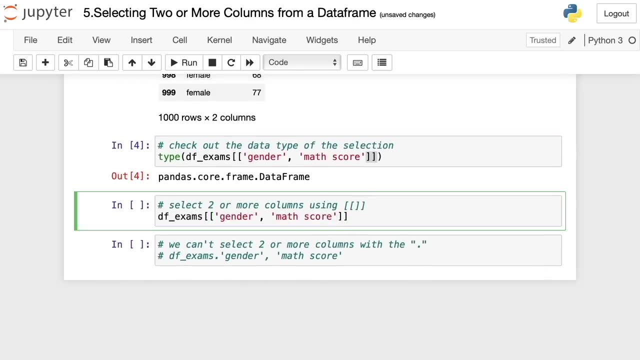 math score, reading score and writing score. So to do so, first I'm going to copy this first selection with it to have it as a reference, And now I'm going to paste it here. So I'm going to save it in my folder. So here, so far, we have two columns, so let's add the 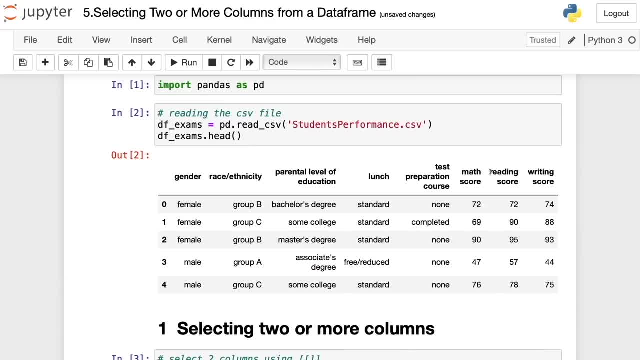 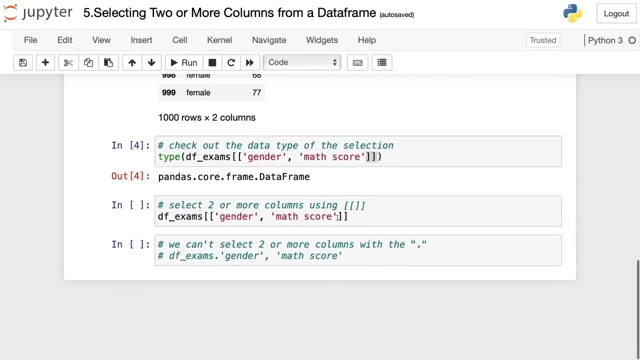 two remaining columns. So here, an easy way to write these columns is just by copying this in the data frame And here we can paste it. So instead of writing those names we can just paste it here. Now I delete and I put it inside puts. So here are inside quotes: 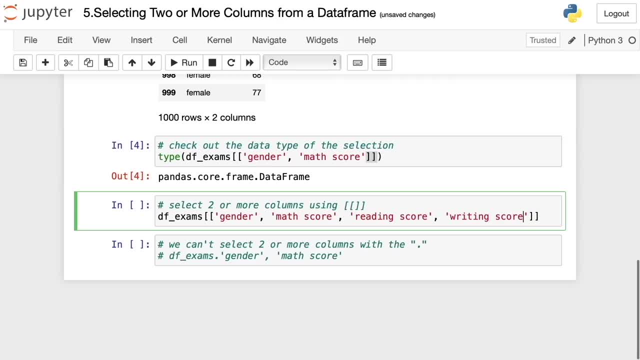 And here we have it. So here, as I said before, I'm going to add my Wi contradiction And I'm going to enter this, Or you can activate this, And you know this, of course. I've already doing this And 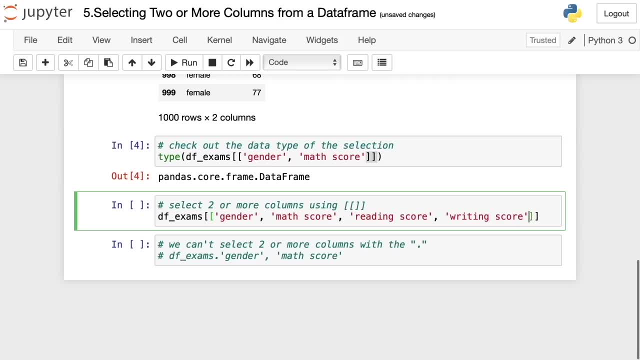 we can change the order of the columns, we just have to. for example, here I cut this And let's say we want to have the writing score in the beginning, So here I paste writing score, And now what we're going to get is first the gender column, then writing score column and then the 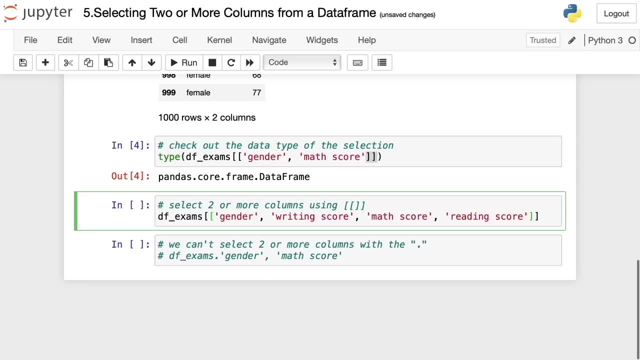 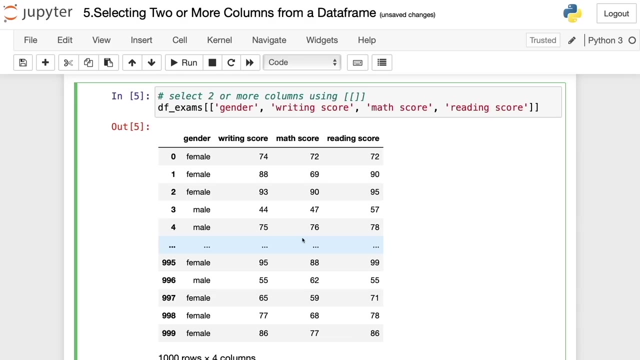 math score and reading score columns. So now let's run this code And, as you can see here we have this data frame in the order that we defined here. Okay, now you might be thinking if there is a way to select two or more columns using that that sign. So let's check if that's. 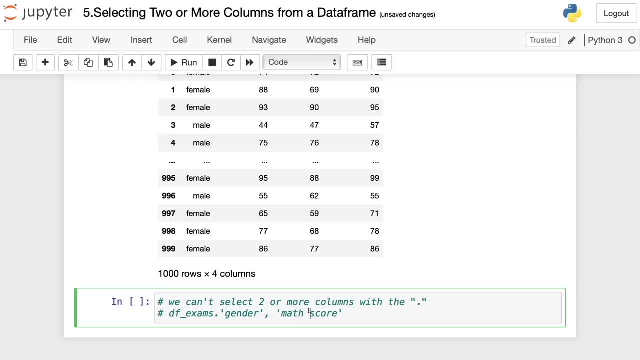 possible here. For example, let's say we want to get a gender in the math score column using that notation. So here I have it And as you can see here this doesn't look right, Because if you have two strings separated by a comma. but 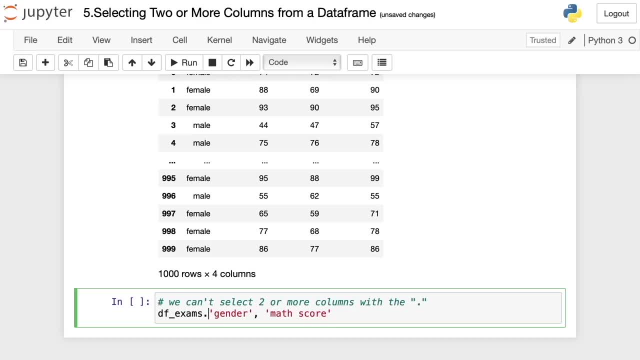 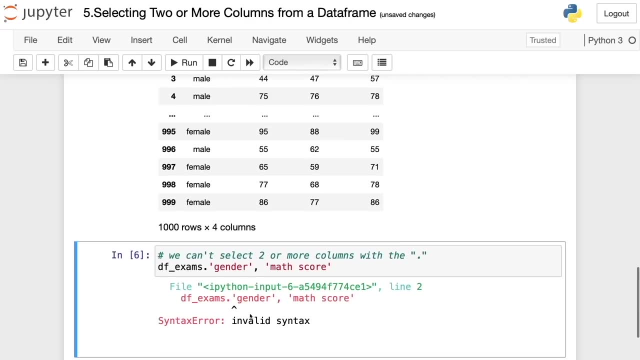 you don't have a list, you don't have square brackets. this is probably going to fail. So let's check. I'm going to run this code And, as you can see, here we got an invalid syntax, So it's a syntax error. So, as you can see, we cannot select two or more columns with that. 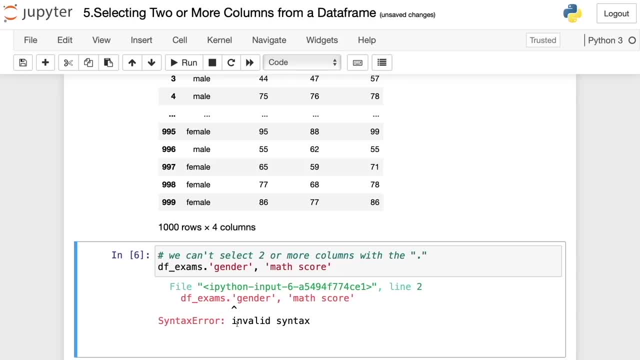 sign, And this is one of the disadvantages that that sign has over the square brackets. This is why most people prefer to use the square brackets instead of that dot notation. And that's it for this video. In this video, we learn how to select two or more. 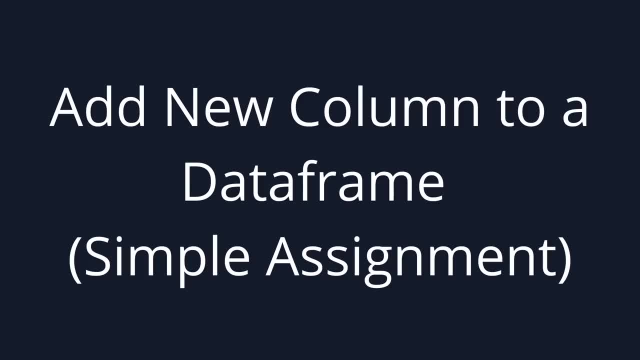 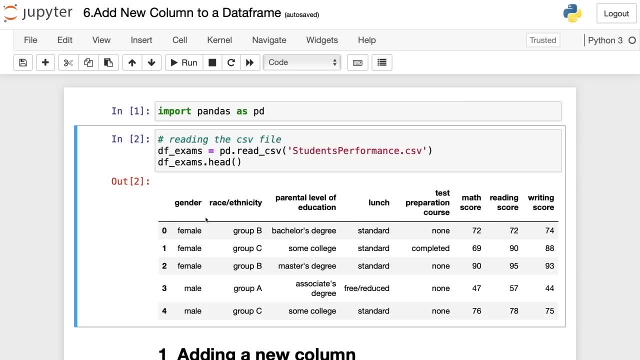 columns from a data frame. Okay, in this video we'll see different ways to add a new column to a data frame. So here is the same students performance data frame And, as you can see, we have three columns with scores: math score, reading score and writing score. So let's say we 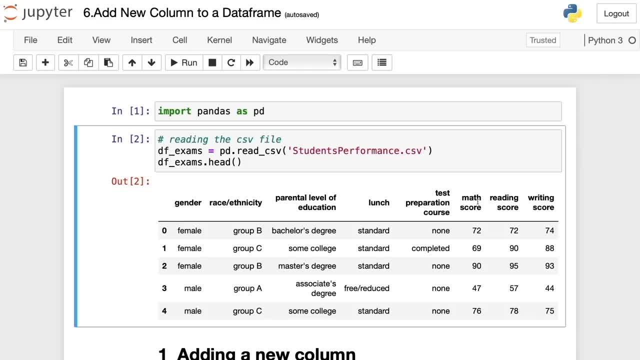 want to add a new score. So in this case, we want to add a new score. So in this case, we want to add a language score. So in this case, let's add a language score. So to add a new column in. 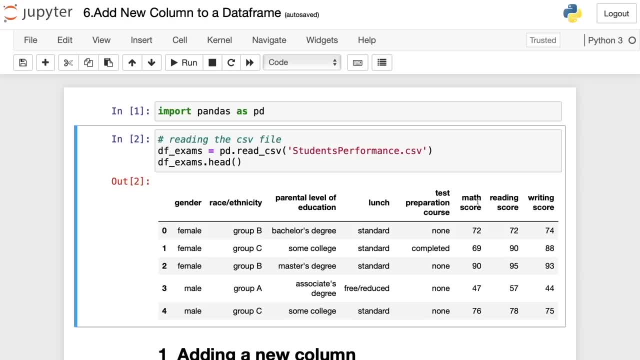 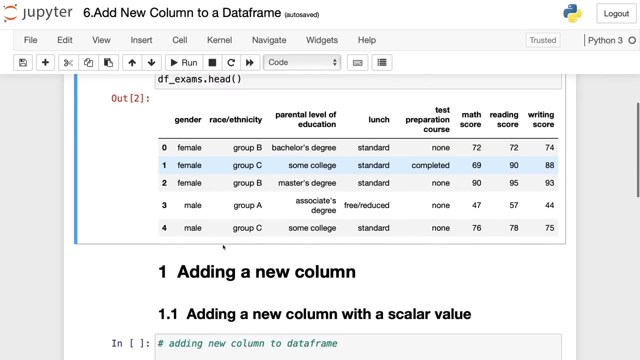 spreadsheets like Google Sheet or Microsoft Excel, we'll simply insert a new column And that's it. But in pandas we have to use different methods or different ways to allows us to insert a new column. So let's see how to do it here. So first let's add a new column with a scalar value. 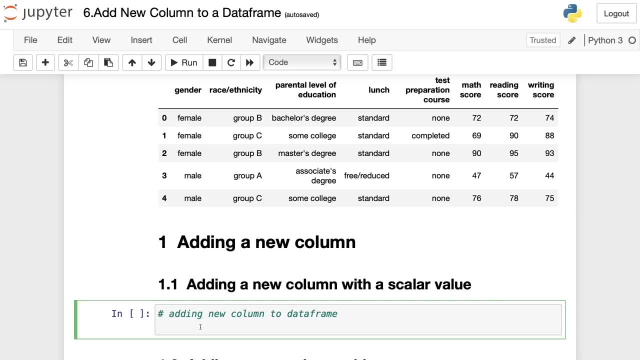 So a scalar value is simply a single value And in this case it's. the column is going to have one single value, So all the rows is going to have the same value. So to do so, we're going to have to select this imaginary column, because 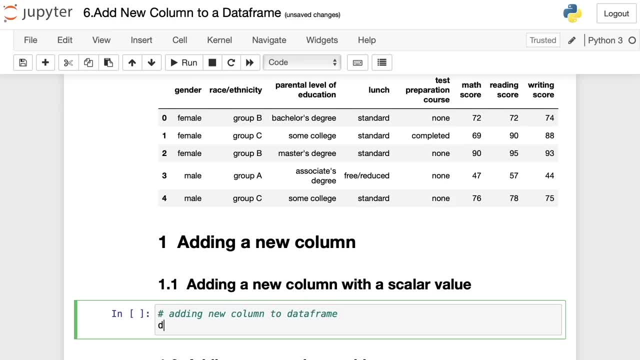 this column doesn't exist so far. So what we're going to do is to select a column, as we will do with any other column. So first we'll write the name of the data frame, in this case the F underscore exams, And then we open square brackets and open quotes, as we will do in any column. So 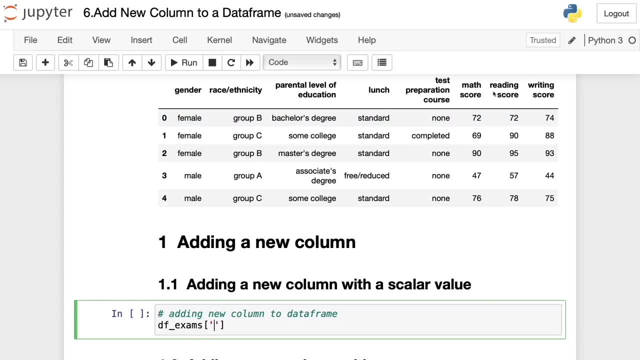 here. instead of, for example, writing math score, I'm going to copy this: Instead of selecting math score, we have to write the name of the column we want to create. So in this case, let's write language score. So this is a new column we want to create And now we have to assign to this. 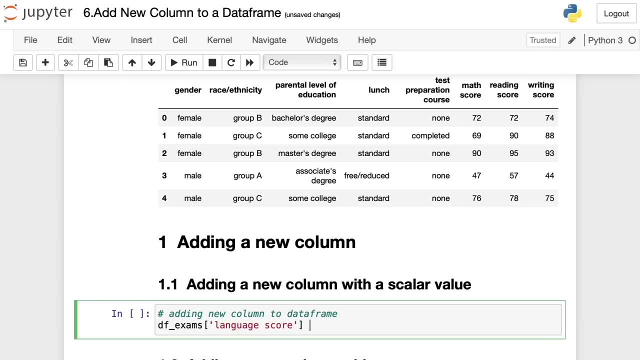 new column, we have to give it a new value or a new scalar value. In this case, I'm going to add a value of 70.. So now, if we run this code, we're going to see that nothing happens, that if we now 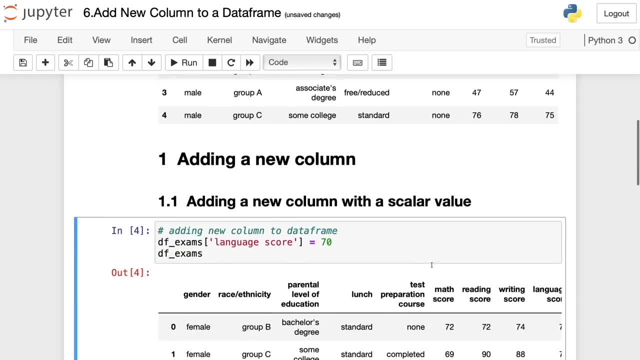 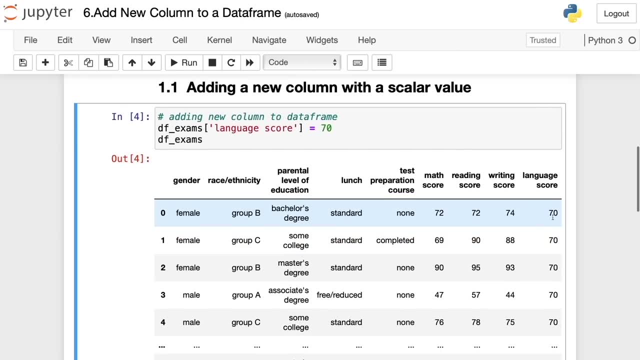 show the data frame. we're going to see that we have a new column And this column is named language score And the value that this column has is the same value. So it's 70 in all its rows, So we have 70.. 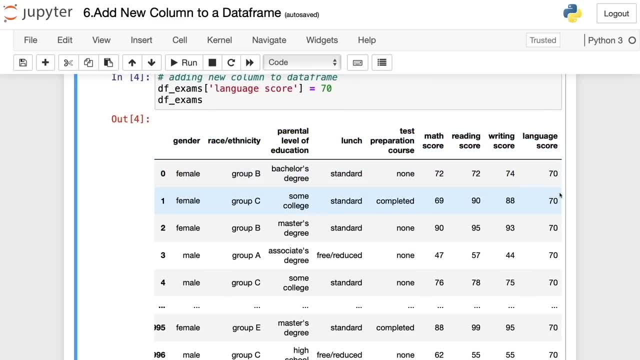 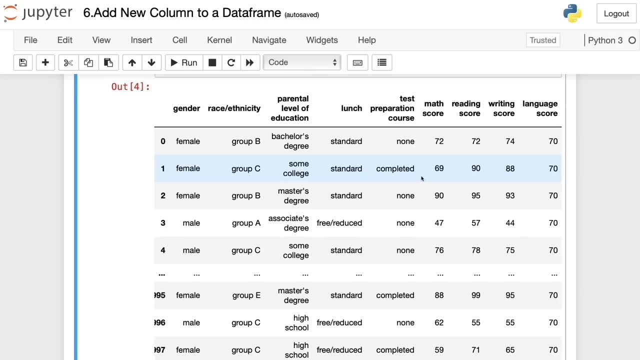 In row zero And if we scroll down we're going to see that it's 70 in all the rows, So even in row 999.. But it's a bit weird that in an exam you will have all the students with the same score So. 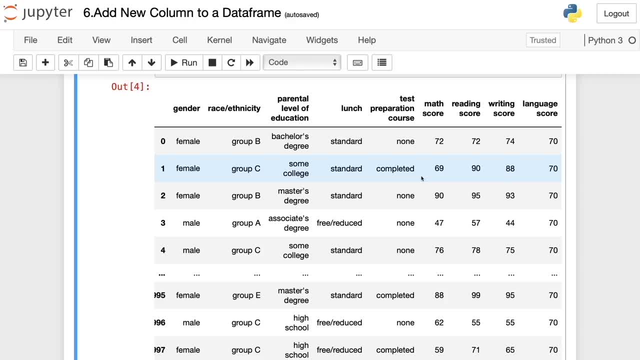 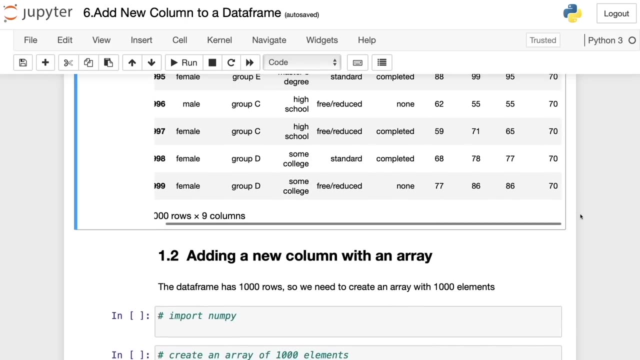 what you will usually do is to add some different values to this column. So to do this we have to use arrays, And to create arrays we have to use numpy. So here, in the second way, to add a new column, we're going to use arrays. So in this case, 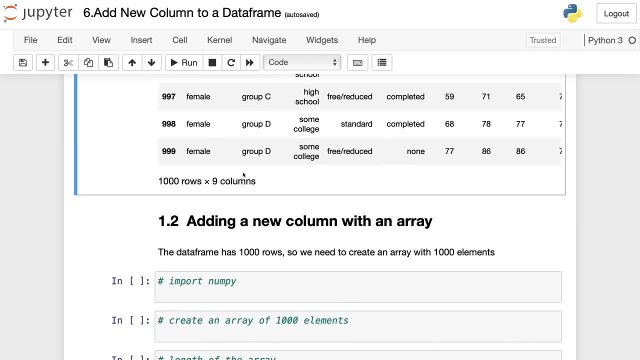 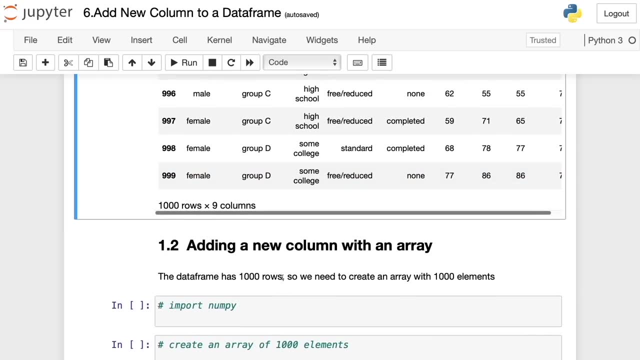 we have first to see how many rows this data frame has. So in this case it has 1000 rows, And this is important because the number of rows has to match with the number of the rate we're going to create. So let's create this array And first let's import numpy. So we write import numpy as. 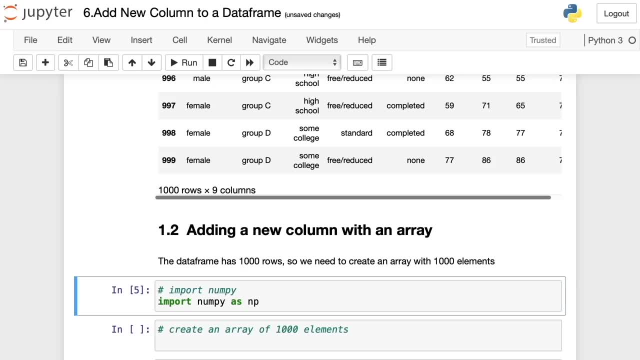 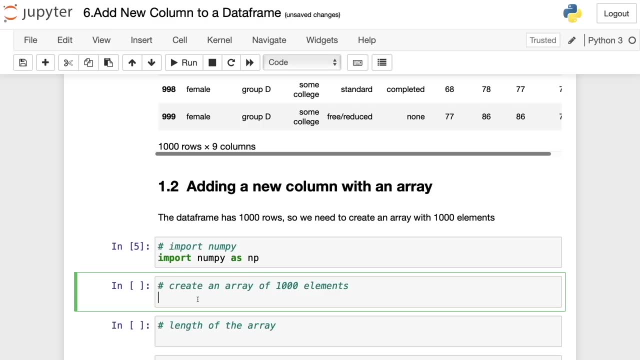 numpy And p. so we run this code And now we import it numpy. So now we have to create an array of 1000 elements, And to do so we're going to use a method called arrange. So it's written like this: 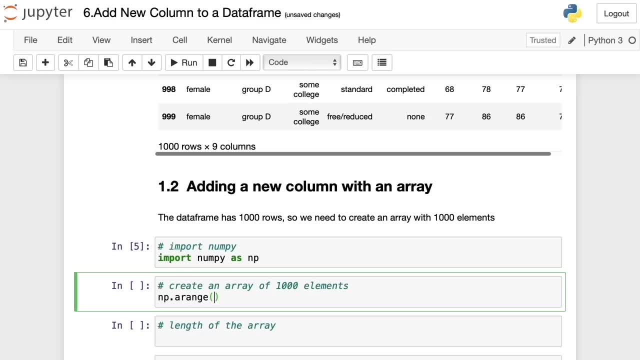 orange, And this gives us an range of numbers that start with the first argument and that I'm going to write zero, And the last argument that in this case it's going to be 1000.. So these are the limits of my range. So I execute this And, as you can see here, 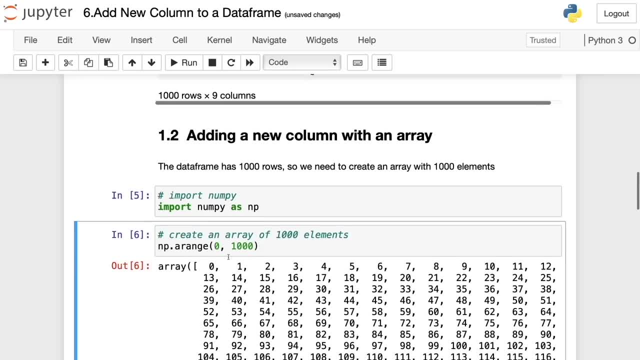 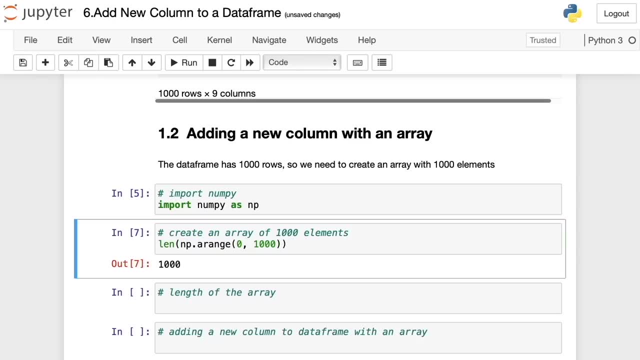 it starts with zero until 1000.. So to verify the length of this range we have to use the length function. So, as you can see here, the length is 1000. So the rate has 1000 elements. So now I'm going to assign this to a new variable And I'm going to name this. 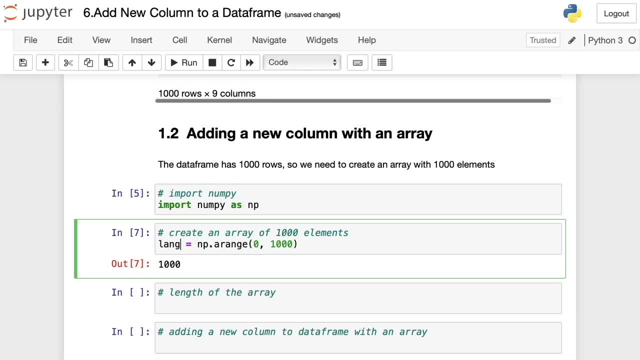 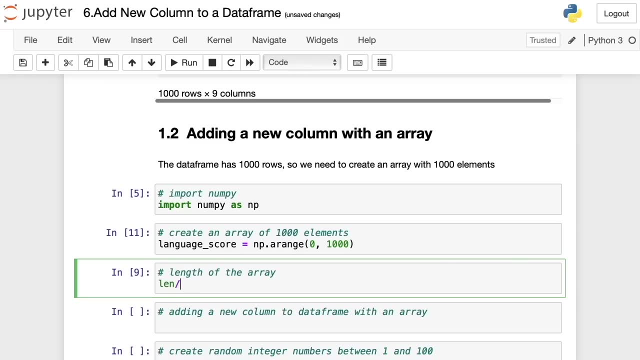 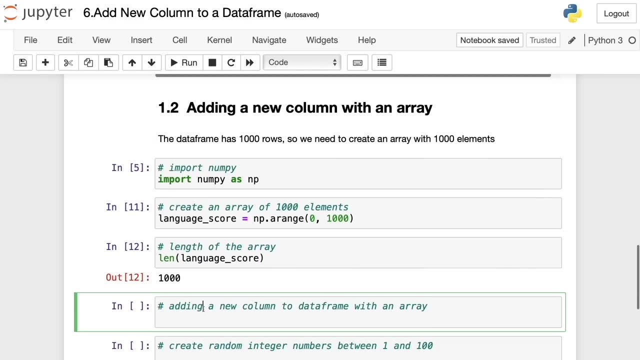 variable language score, So language underscore score. So we execute this, And here I was planning to see the length of this array, So I quickly do it here. So we did it before. So land in, we have the length of the array. So now we have to add a new column to a data frame with this array. 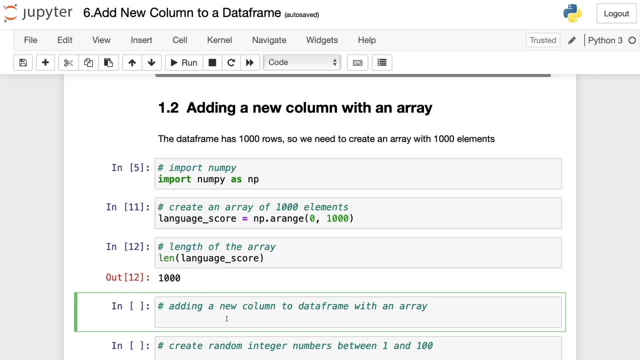 And to do that we have only to use the same way we did before. So first we write the name of the data frame And then we make the selection. So this selection is going to be with a new column- Well, in this case is not new, because we already created it, But let's imagine it's a new column. So 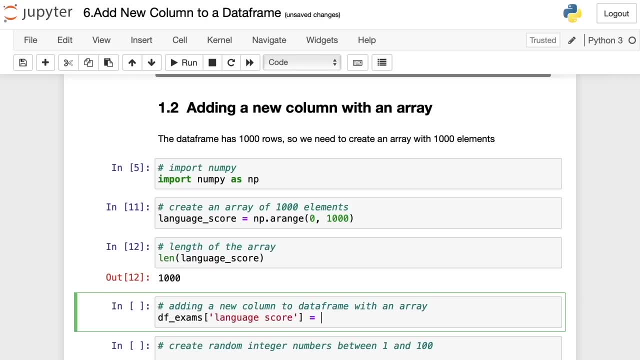 it's language score, And now we have to set the array to this column. So we write language score here And we set it to this new column. So now to see the results, we only show this data frame And, as we can see here, we have a new column And this new column starts with zero. 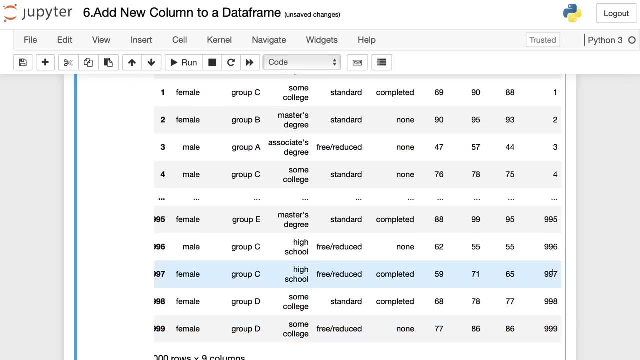 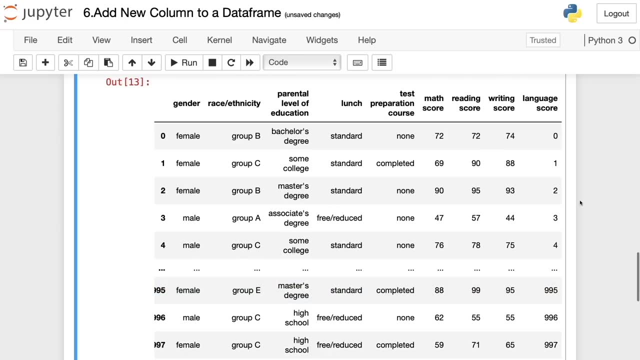 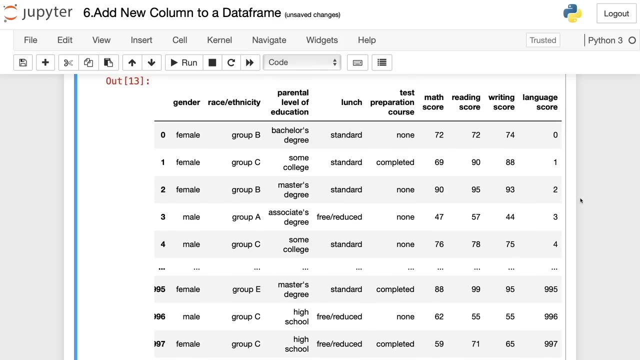 and it ends with 999.. So it doesn't have a single value anymore. But now it has a range of values, And now there is a little detail we have to take care of. So scores are supposed to be between zero to 100. And we have here from zero to 999. And now we have a new column. And now we have a new column. 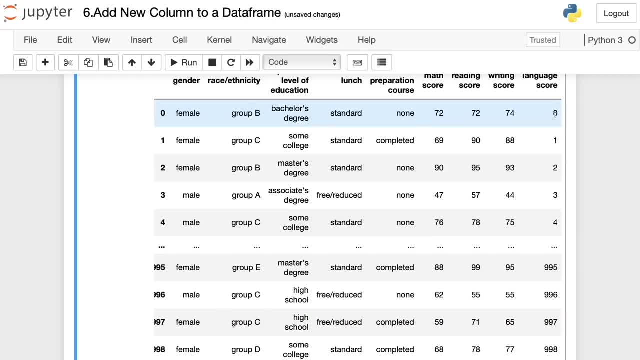 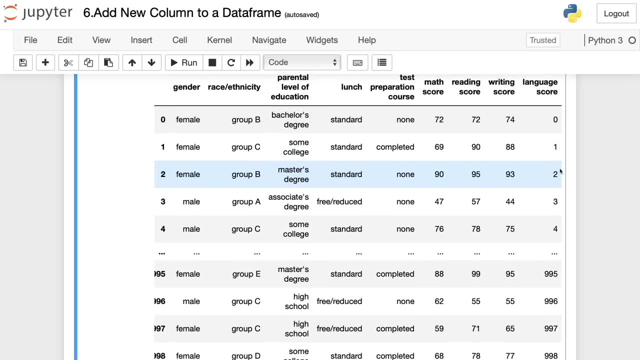 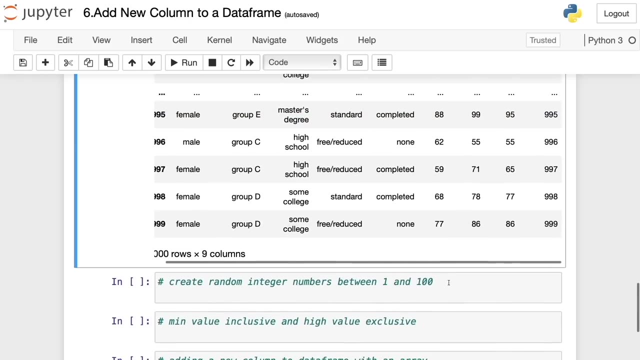 And also here we have a sequence of numbers, So it's from zero and then one, and it increases by one, And usually in scores you will see that students have random scores. So we have to create here an array with random numbers, And to do that we have to use NumPy again, But here we have to. 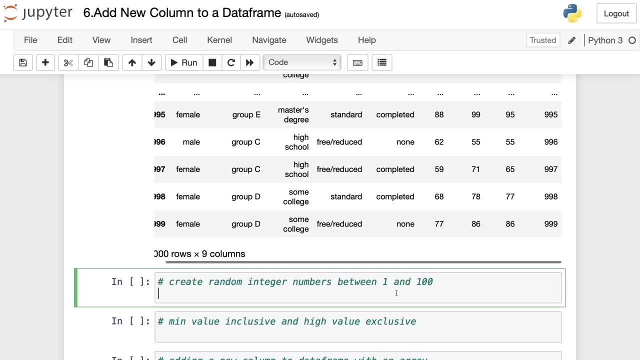 use a different method. In this case, the method is named random dot rant, int. So let's write it here: NP dot, random. And then we have a new column, And now we have a new column, And now we have a new column that ran, And then I n t. So the first argument is the lowest value of these random. 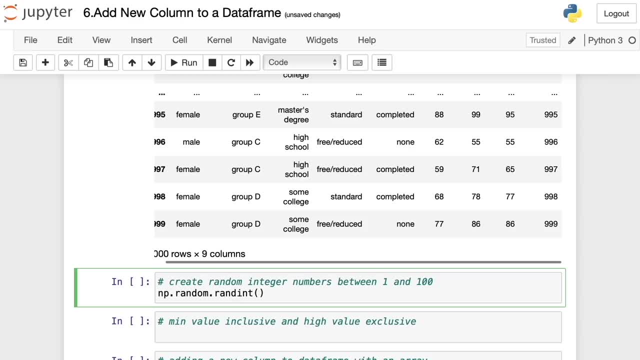 numbers- And, by the way, these are random integer numbers, because scores are usually integer numbers, And in this case I'm going to set this, this, to one. And the second score is the highest number or value in these random numbers, and I'm going to set it to 100.. And the 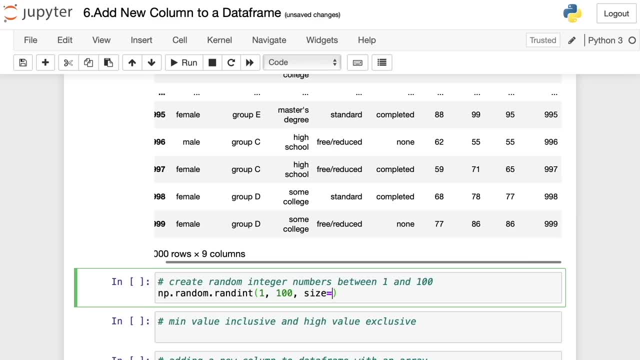 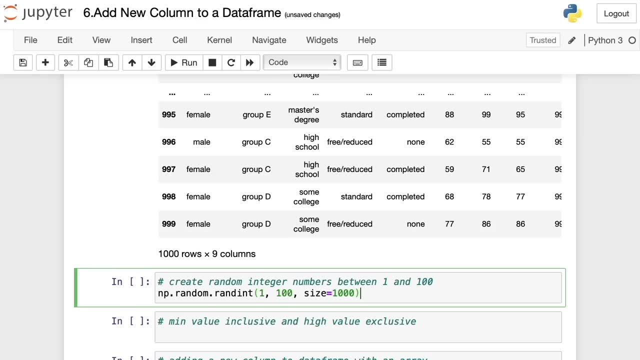 third argument is the size. In this case, we want an array of 1000 elements, So we set the size to 1000.. Now we execute this, we run this, and I'm not going to see this rate Again, I'm just going. 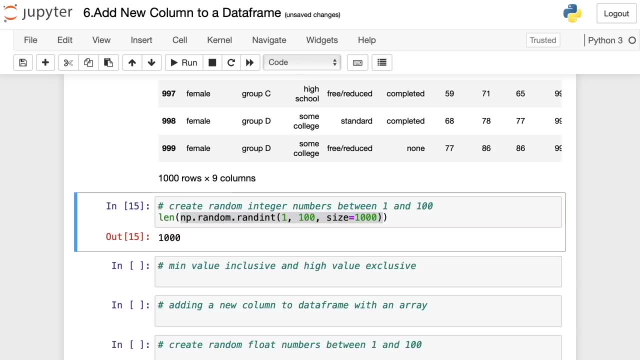 to check that it has the length we want by using the length function. In here we have 1000 elements, So now let's create a new variable and store this in the variable. So here this is going to be: I n, t and then language, underscore, score, And this is going to be: 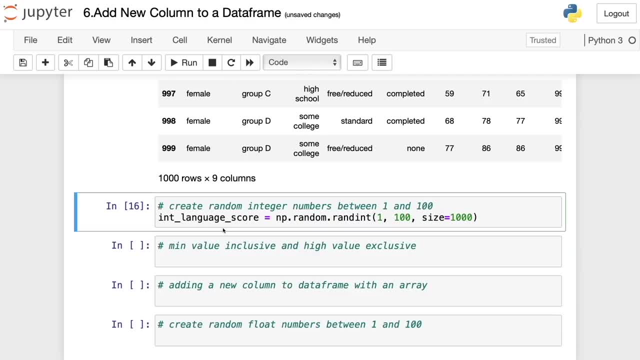 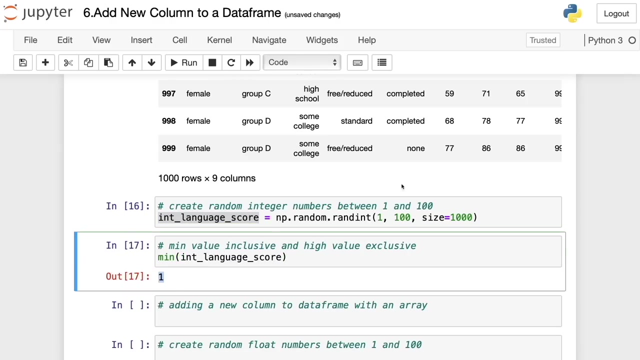 our new variable. So here, one little detail you should know is that the first argument is inclusive and the last one is exclusive. So this means that if we here, let's say, we get the minimum value of this new array, we're going to get that the minimum value is one because this first argument is inclusive. 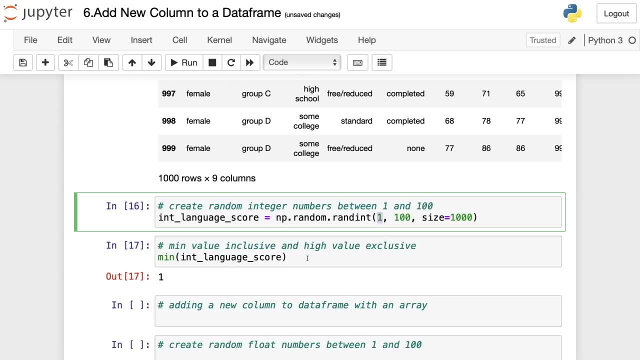 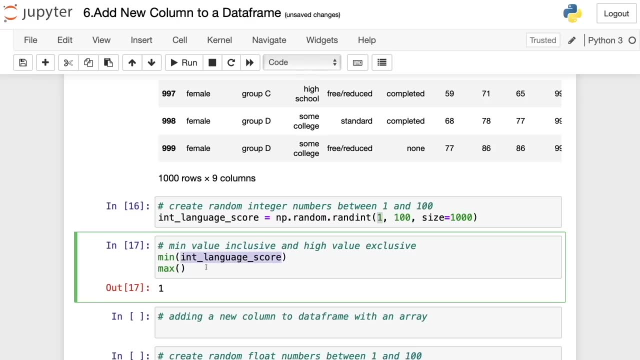 which means that it can be included in this new array. However, if we print now the maximum value of this array, we're going to get that 100 is not there because it's exclusive, which means that this second argument shouldn't be included in this array. Okay, finally, let's insert this: 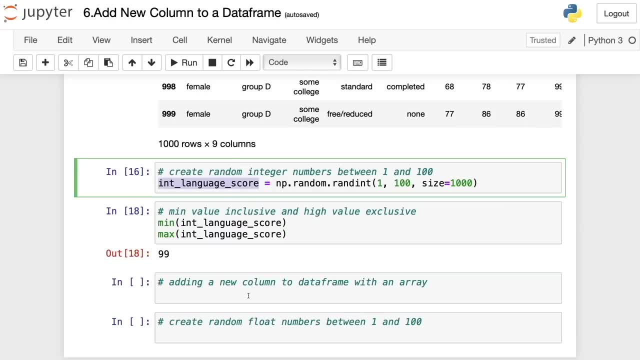 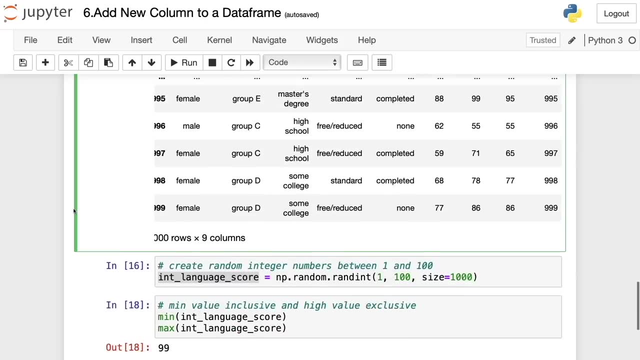 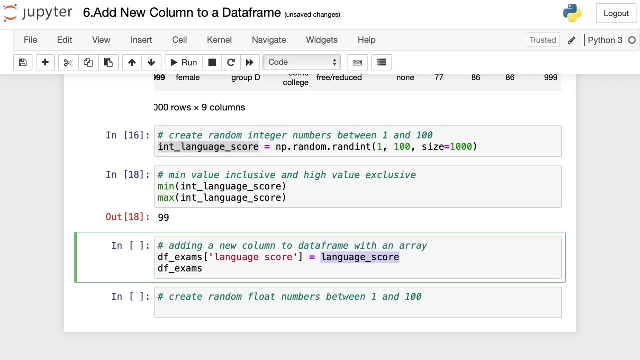 random integer numbers in the new column that we created. So we have to just use the same way we did before. So here I copy and now I paste it. So here, instead of assigning this language underscore score, I'm going to use this int language underscore score. So here I'm going to. 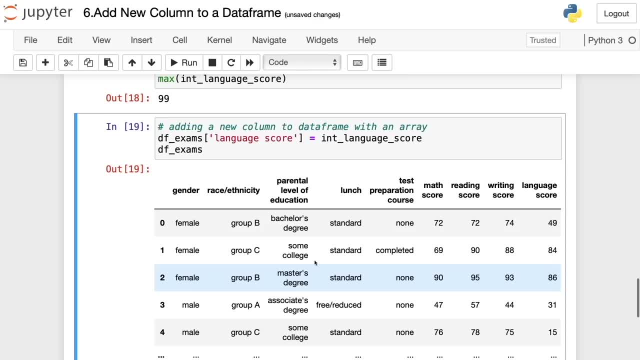 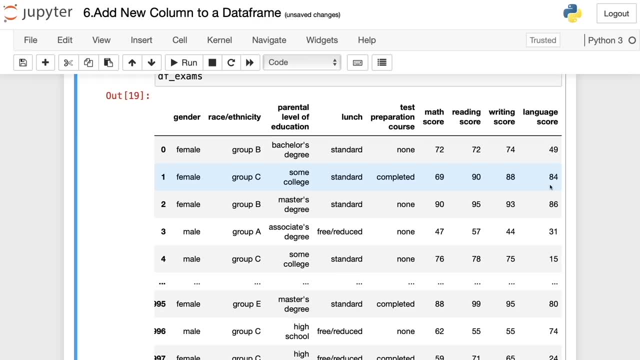 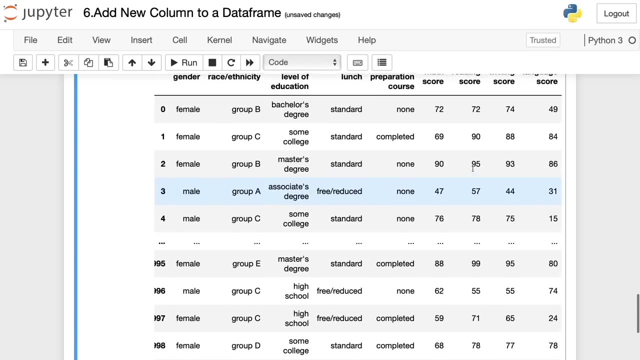 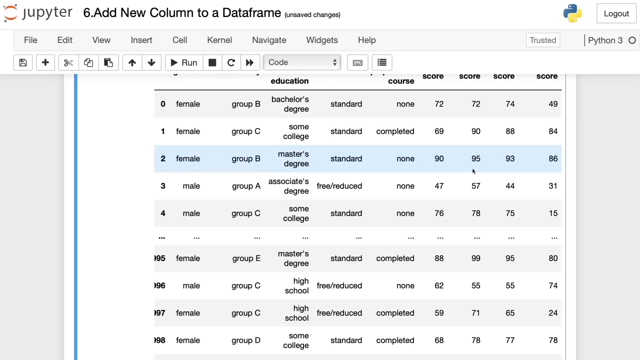 run this code. See, here we have this, the same column, and we have now this data, that is, random, random integer numbers from the row zero to the row 999.. So now this new data looks more like scores, like real scores, because these are random numbers and these are between zero and 99.. And that's it Now. 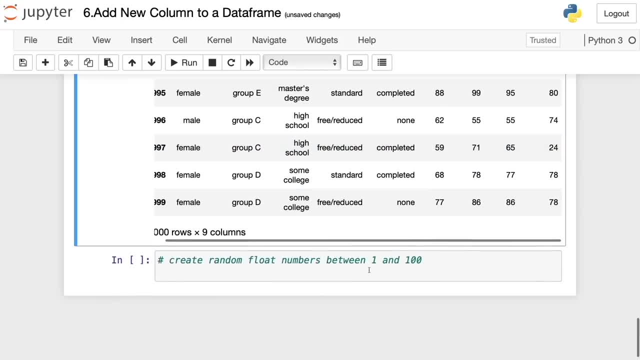 one more little detail I want to share with you is how to create random float numbers, because before we created random integer number. but if for some reason you want to create random float numbers, there is a way how to do it with NumPy. So we only write NP, then that random, then that uniform. 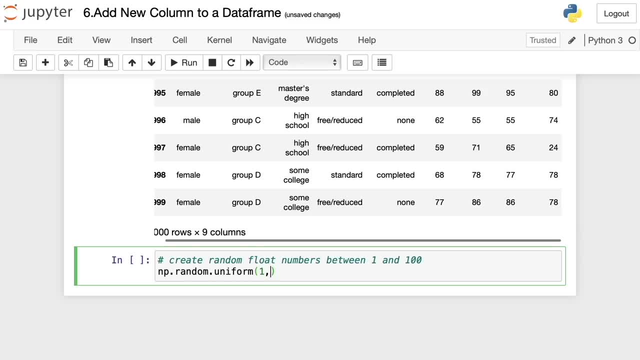 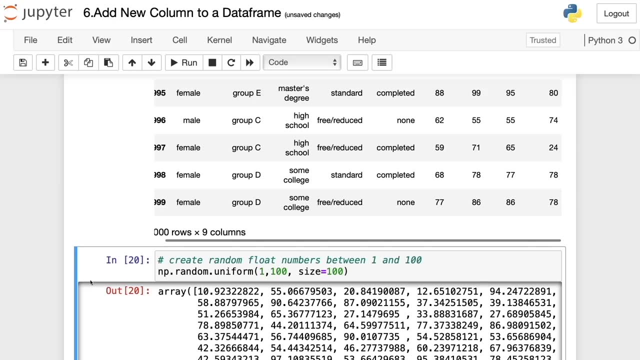 And the arguments are the same. So the minimum value, then the maximum value, then the size, which is 1000.. Then you run this: And well, it's similar to the one we got before, But now we have float numbers. 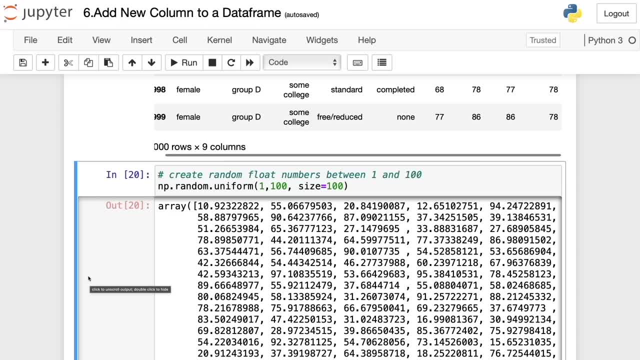 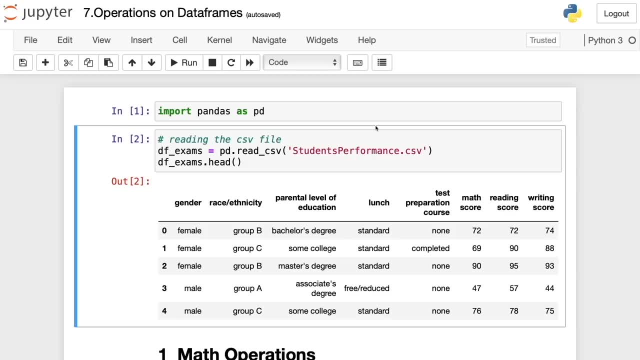 And that's it. In this video we learn different ways to add a new column to a data frame. All right, now it's time to see some operations we can perform on data frames. So here we have the same data frame- DF, underscore exams- And here we can apply some common operations to the. 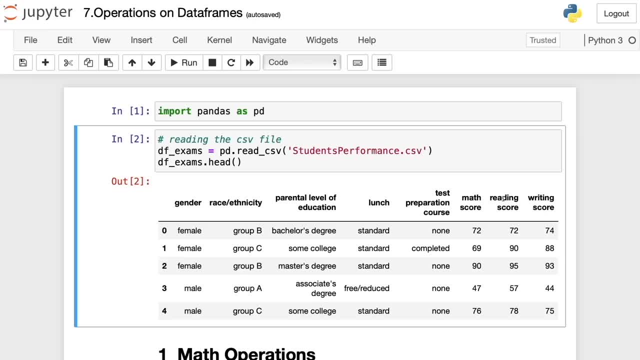 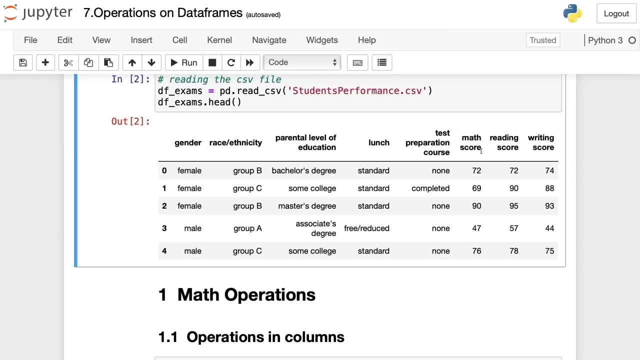 numerical columns like this. And here we can apply some common operations to the numerical columns, like math score, reading score and writing score. So let's see how to do this in pandas. So first we're gonna see how to make operations in columns. So our first task is to calculate the total sum of. 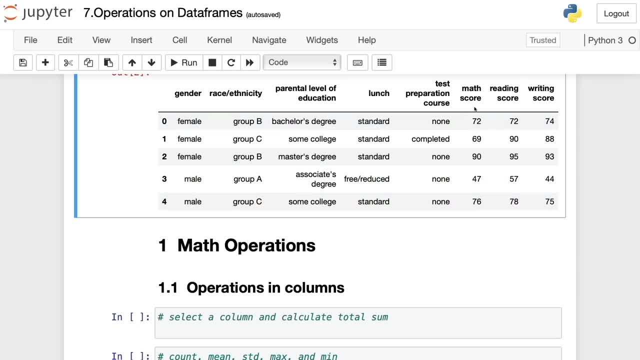 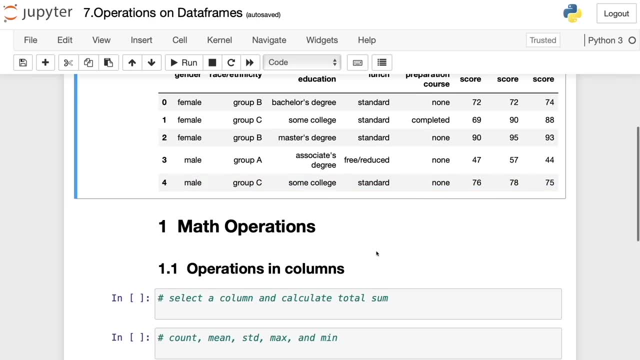 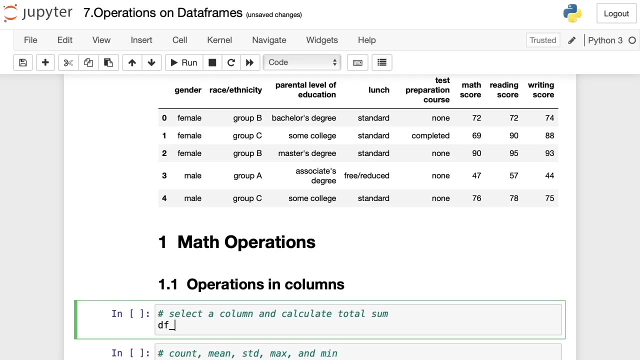 a column. So let's pick first our math score And let's calculate the sum of this column. So to do that, we have first to select a column And, as you might remember, to select a column first to write the name of the data frame, in this case the F underscore exams. then we open. 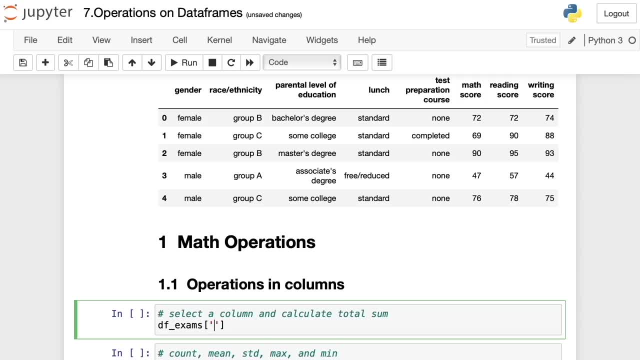 square brackets and then write either single or double quotes, then have to write the name of the column, And in this case it's this one math score. this is the column we want to select, And now, instead of selecting, we're going to perform operation. So in this case, 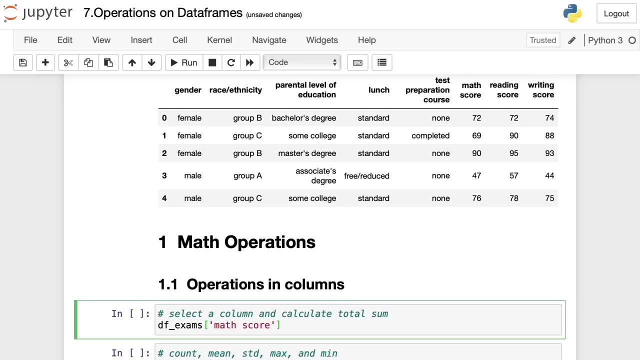 I want to calculate the total sum of this column and we have to use the sum method. So we write that sum in parentheses And this is how you calculate the total sum of this column. So to verify this, we run this code And here we got 66,000. And this is the total. 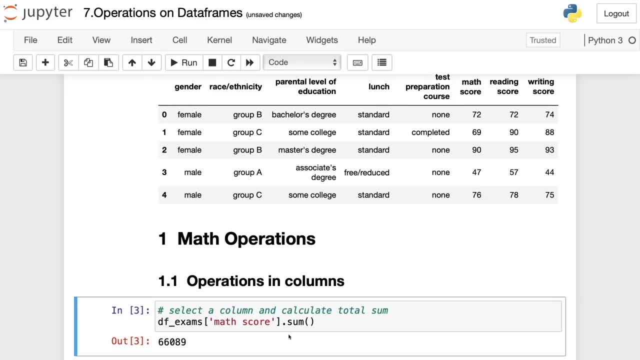 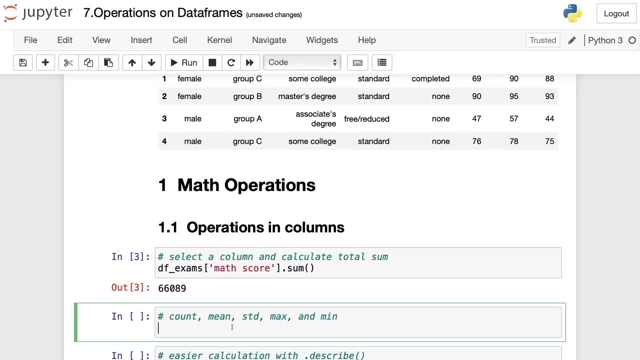 sum of this math column. Great. Now we can make some other operations. you will do the we'll do in Excel, for example, we can calculate the number of rows using the count method. So here we can easily do that. I'm just going to copy this one, And now, instead of writing, 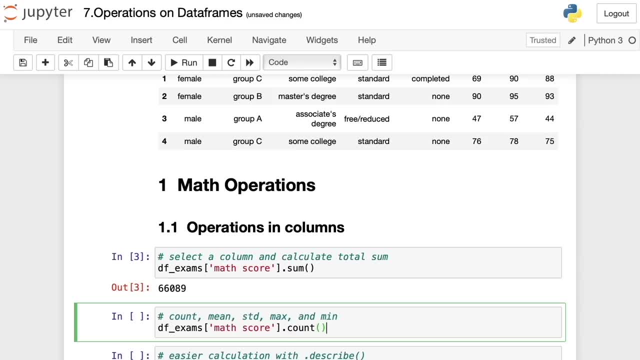 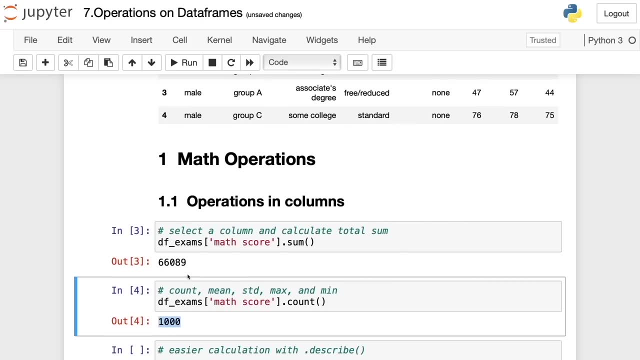 the sum method. we write count, So here count, you know, let's see. So we see 1000 rows. And yeah, this is correct, because this data frame has 1000 rows. So now we can calculate the mean of this. 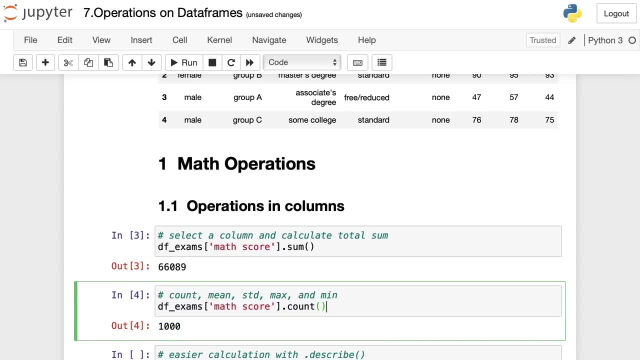 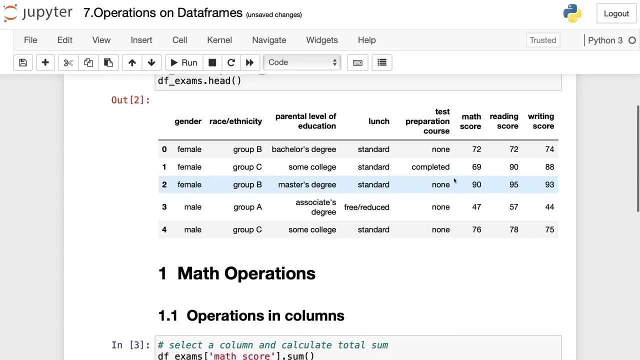 math score column. we have to copy this one now, paste it And instead of writing count, we have to write mean, And here we got the average value of this math score column. So to get the average we have to sum all the rows in this math score column and then divided. 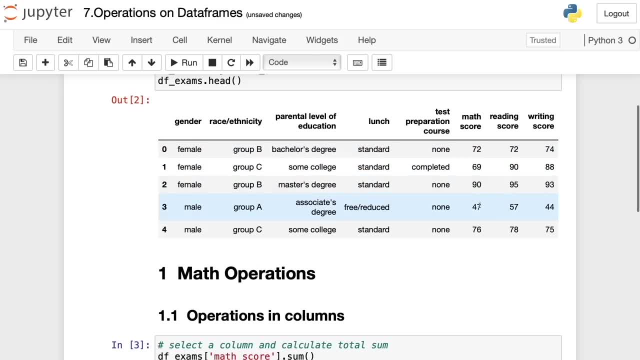 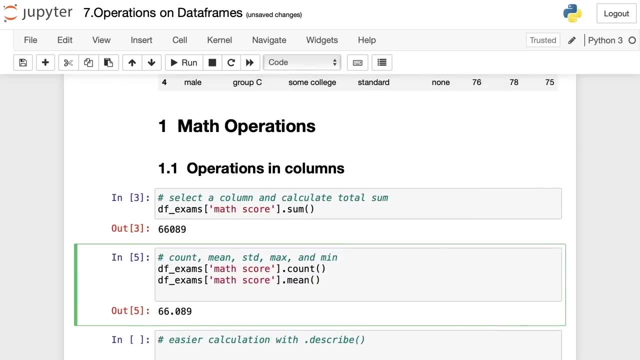 by the total number of rows, in this case 1000.. And this is how you get this mean value. then we can get other other operations using the method. So here, for example, we can get the standard deviation by writing std. So we execute this and the standard deviation of this math. 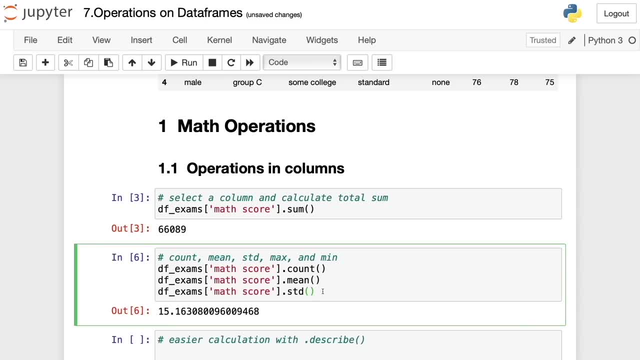 score column is 15.. And we can get also the maximum and minimum value. Let's do it quickly here, So first the max and then the mean value. You can actually do it with the Python built in function, But we can also do it with methods. 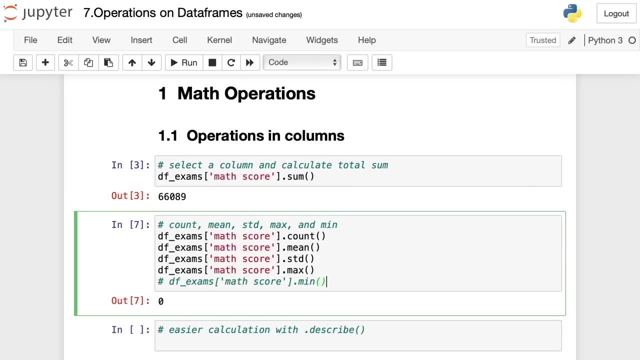 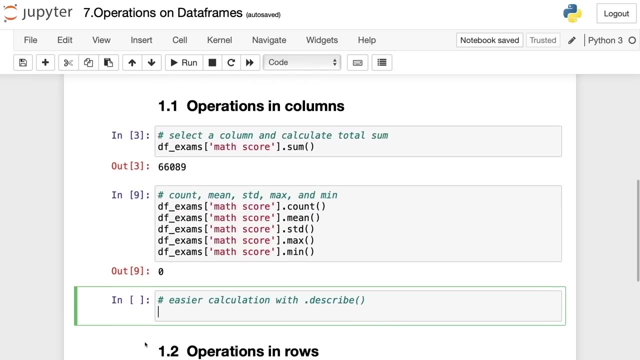 So here I ran in. as you can see here, the minimum value of the math score is zero in, the maximum is 100.. Okay, now I'm going to show you a quickly way to make the same calculations using that described method. I think we saw that described method in previous videos. 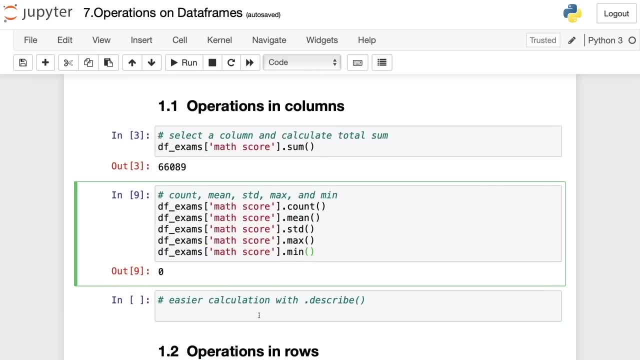 But in case you don't remember it, I'm going to write here The name of. actually, we only need the name of the data frame. we don't? we don't need the name of a specific column, we only need the name of the data frame. And now we can. 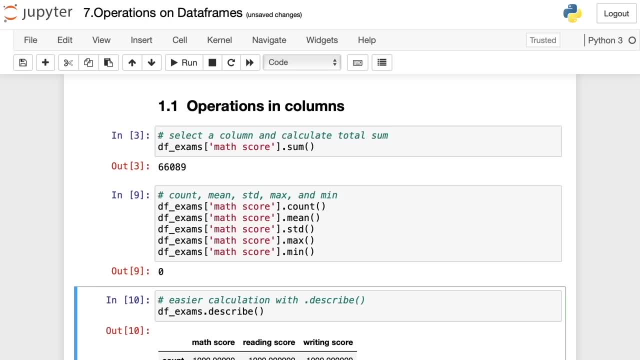 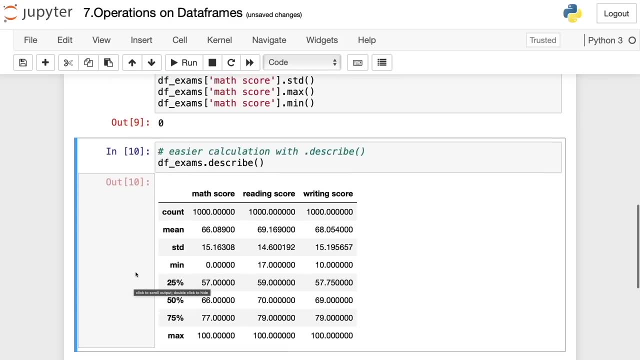 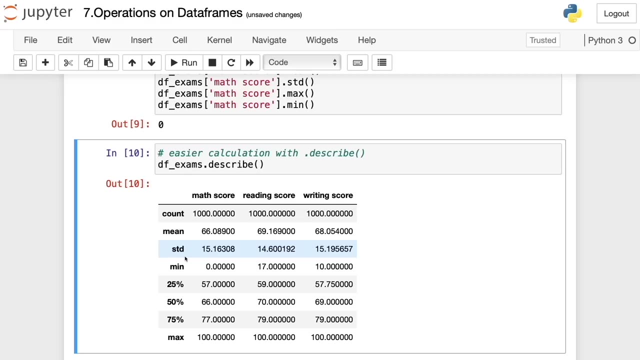 use the describe method, So we write that describe with parentheses. And now we got like a summary table with some important statistical values And here we have the count that mean, the standard deviation, the minimum and maximum value, And as you can see, here we got all. 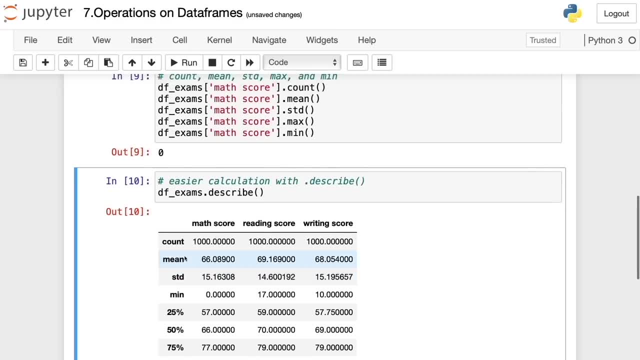 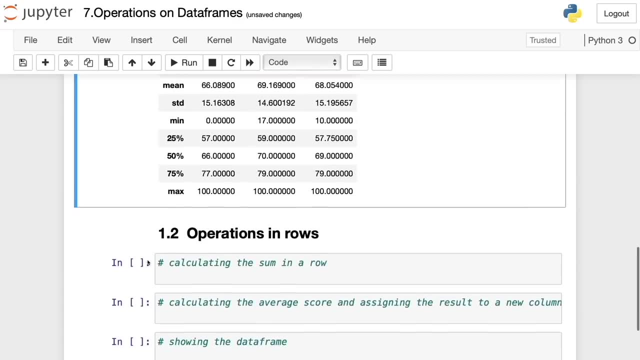 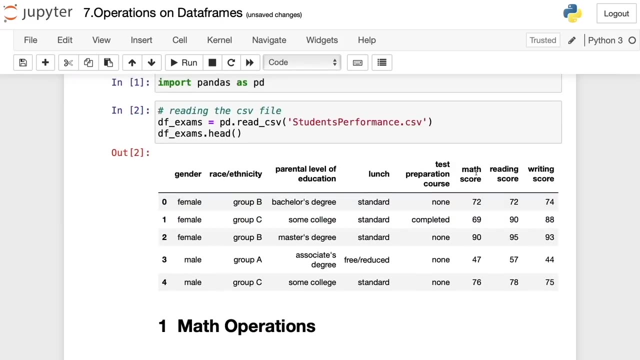 of these values. So we're going to do the same thing with one method. Okay, so far, so good. Now, instead of making operations in columns, we're going to learn how to make operations in rows. So now let's calculate. let's say, the sum of the math score, reading score and. 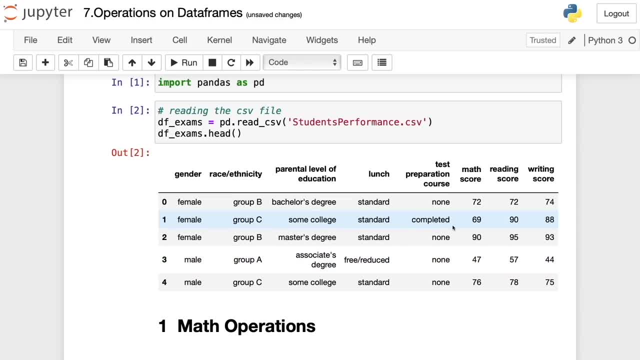 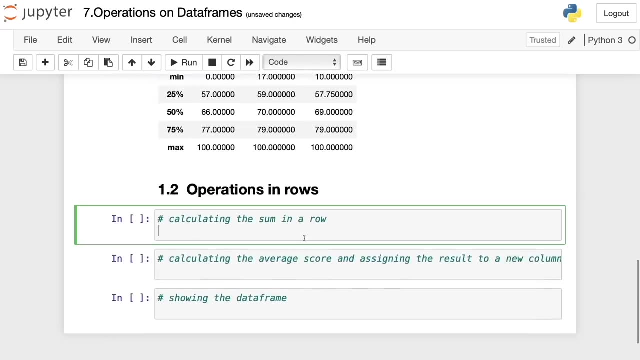 writing score. To do so, we have to make some selections, And in this case we have to make some independent selections. So, to show you, I'm going to copy the name of these three columns. I copied it And now I paste it here. And now we have. 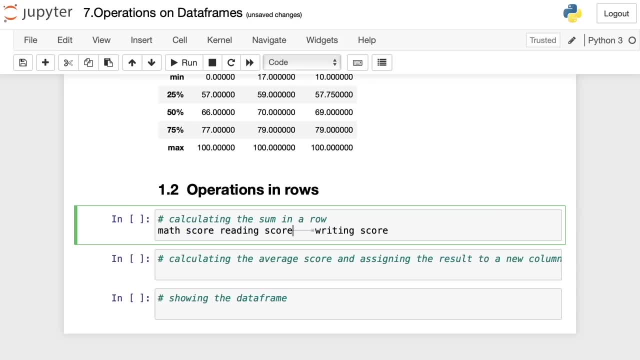 math score, reading score and writing score. So now let me delete that sign. And now we have to make some independent selections. So first we write the name of that data frame, So DF exams, And now to make the selection, we open square brackets and quotes. So now, 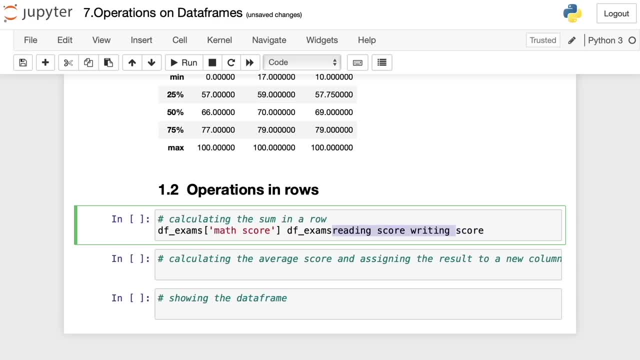 let me do it Quickly in the orders, Now here. so I open square brackets, And now let me do it here too. And now it's ready. So here we made some independent selections, And now to make to calculate the sum in a row, we have to use the plus sign. So here the plus operator. 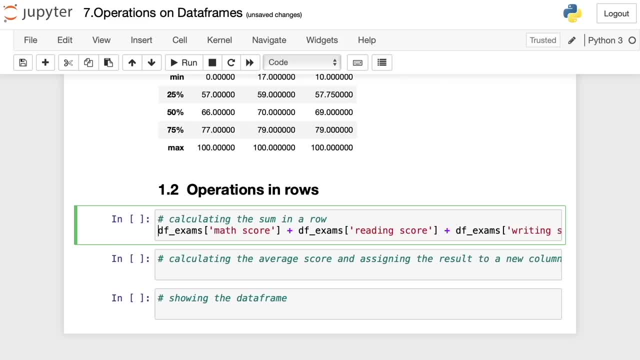 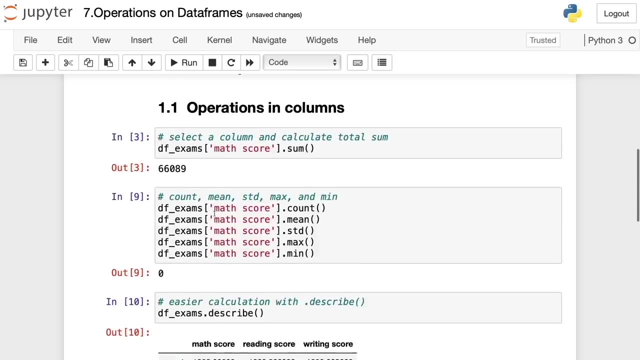 we have to write it here and here. So basically, here we're making some in each row. we're making some in each row. So to verify this, we run this code And, as you can see, here we got the sum of the scores column. So here let's verify fast the sum of the first row. 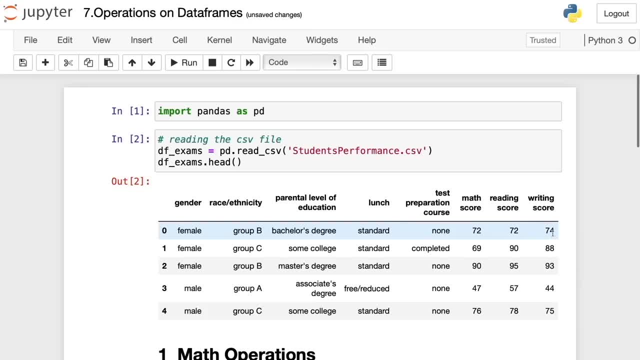 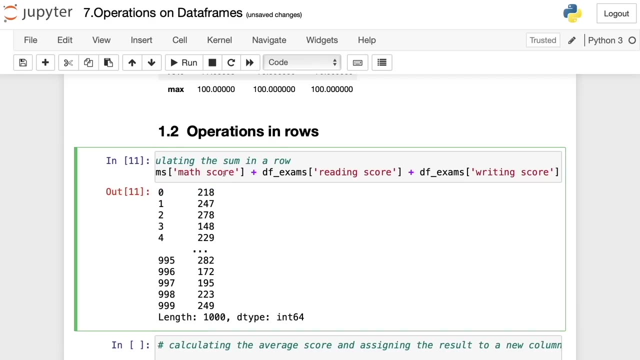 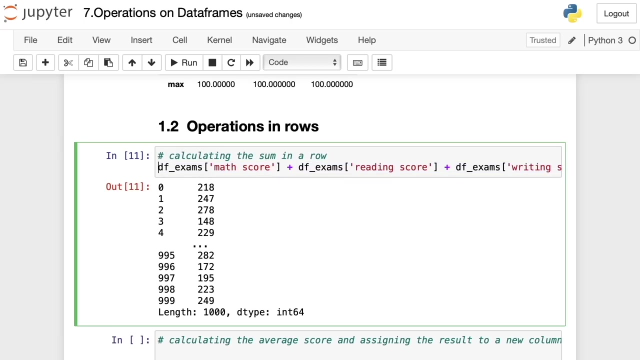 And it's 72 plus 72 plus 74.. So 72 with 72 is 144.. And with 74 is 218.. So here we have it in, it's correct. So now, let's do it. Let's do something else. So now, instead of just summing these three rows, or actually, 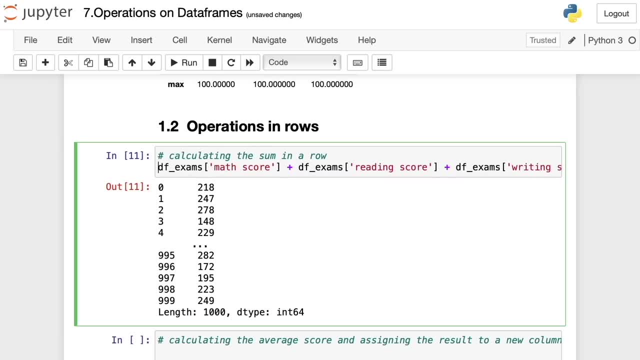 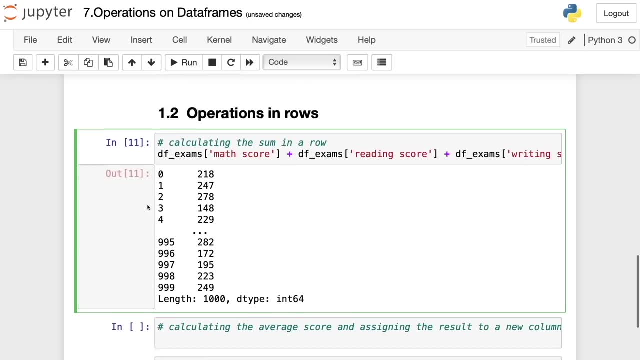 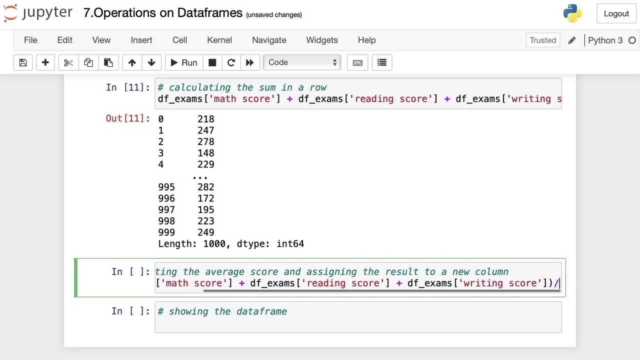 these three columns. what we're going to do is to calculate the average to get like an average score. So here let me copy this. And now here we're going to calculate the average by summing this and then dividing this by three. So this is how we calculate. 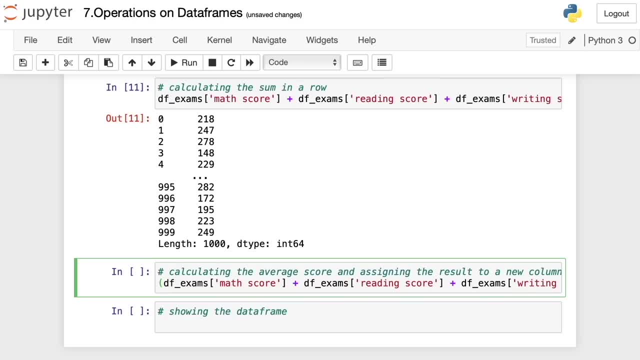 the score. And now let's assign this result To a new column. To do so, we only write equal in them. As you might remember from previous lessons, we have to add a new column by writing the name of this column, So we: 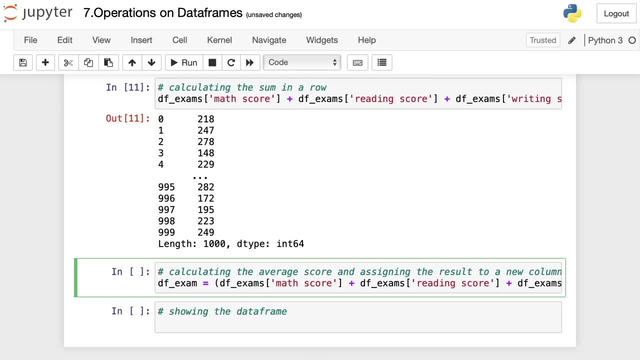 do that, writing the name of the data frame and then making like a selection. So we open square brackets, then open quotes. In here we write the name of the column that we want to create. So this is the same as we did in previous lessons. 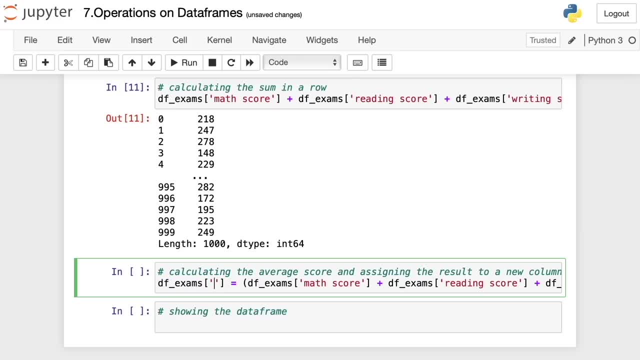 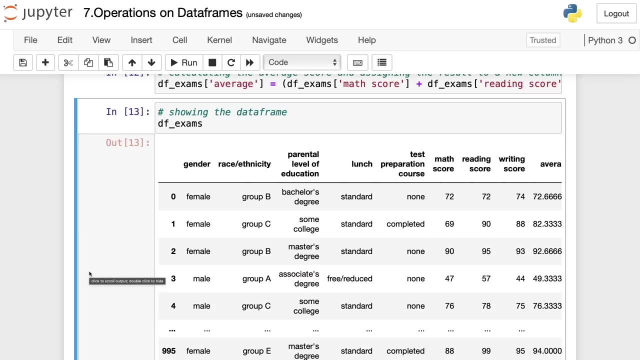 we added a new column, So in this case, I'm gonna name this new column as average And I'm going to execute this. And now, to verify that this new column was created, I'm going to show this data frame here below, And here is our data frame. So now, in the last column, 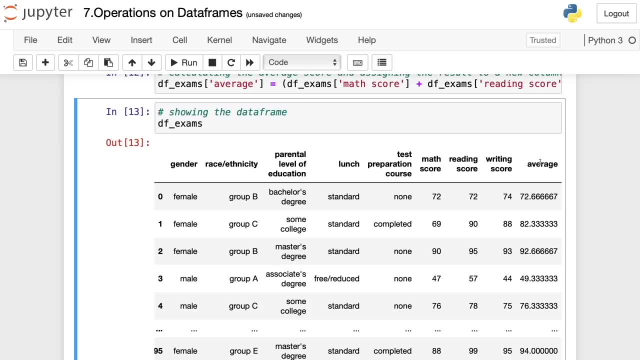 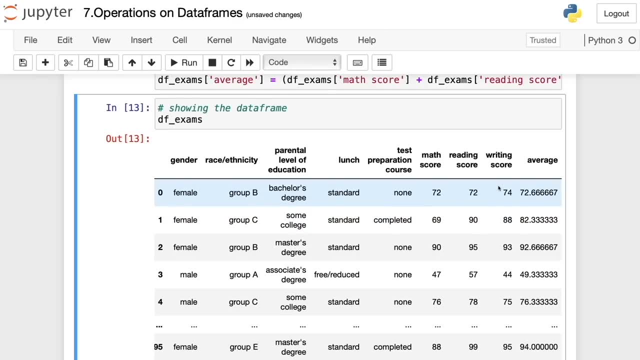 you can see that there is an column named average and it has the average value of this math score And writing score. And now here we can control the number of decimals. we can just use the round function and write the number of decimals we want to get. So in this case I want only 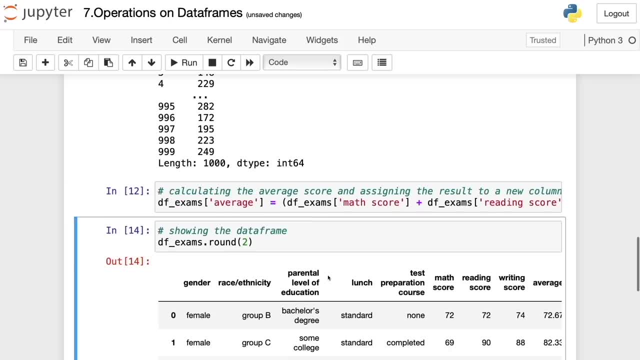 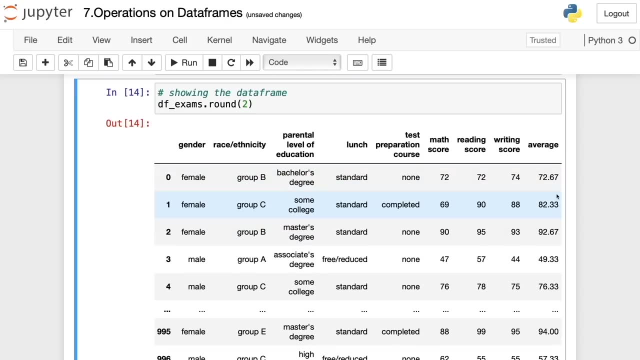 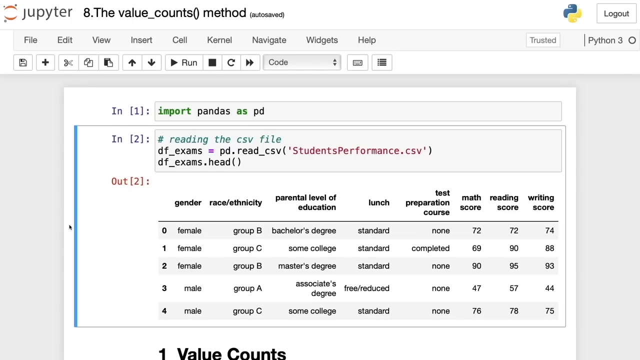 two decimals. So I run this And, as you can see here, our data frame looks much better because we only have two decimals And that's it. In this video, we learn different ways to make operations in columns and rows On data frames. All right, now let's have a look at the value counts method. So so far. 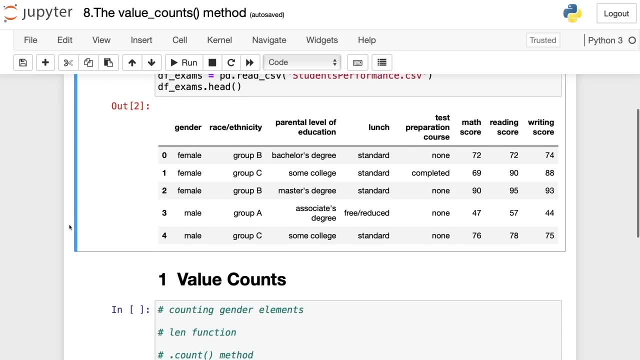 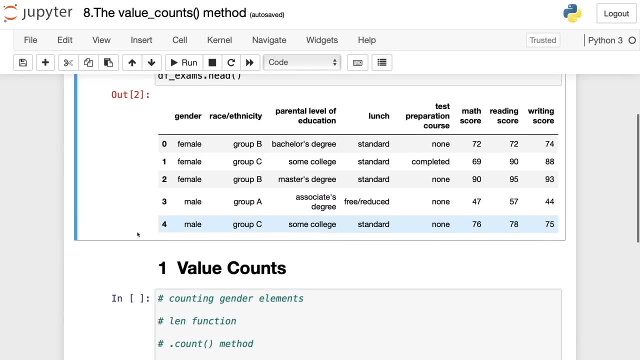 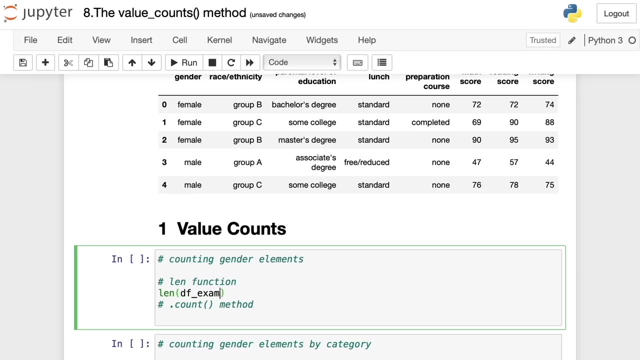 we have seen how to count the number of rows in a data frame. So, for example, if we want to count the number of rows in the gender column, we either use the length function, So we write length, then the number or the name of the data frame. 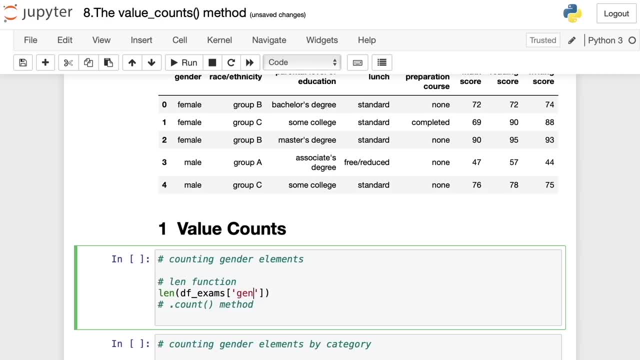 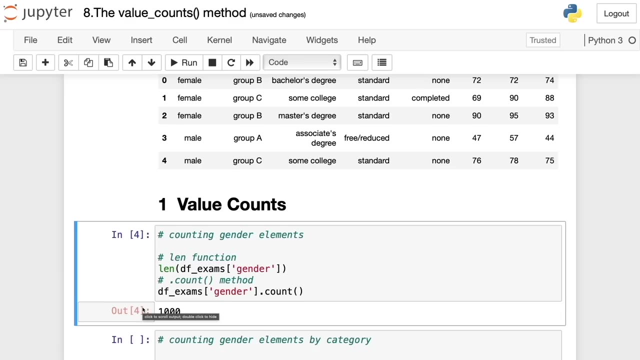 We only have to write the name of the column. So, as you might remember, this give us the number of rows, And we can also use the count method. So here we write, count and we get the number of rows. But what if we want to count the gender elements by category? so 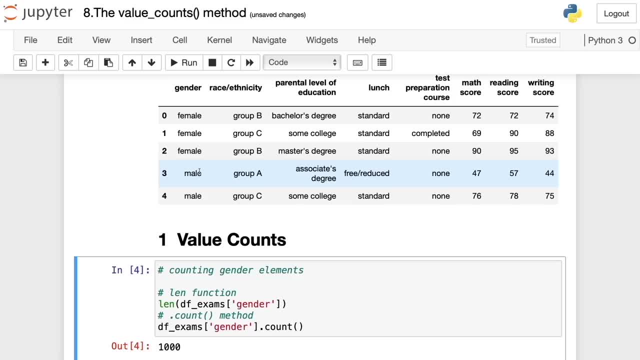 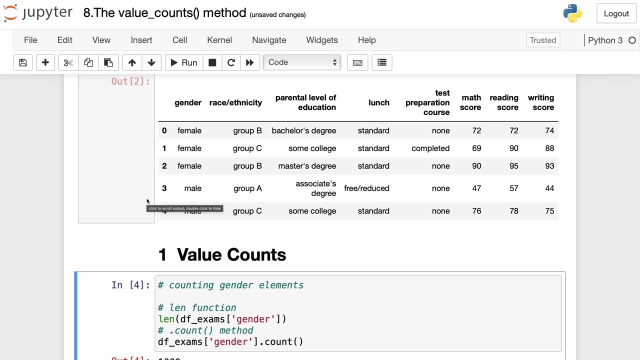 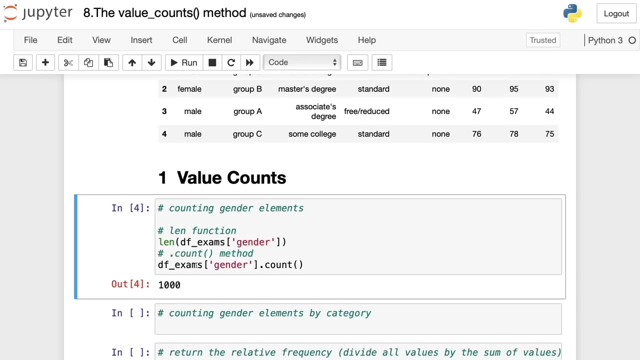 female or male. What if we want to know how many female and how many male elements are in this gender column? So this is when the gender column is created. So if we want to count the gender elements, the value counts comes in handy, So we can use this method to count each category of. 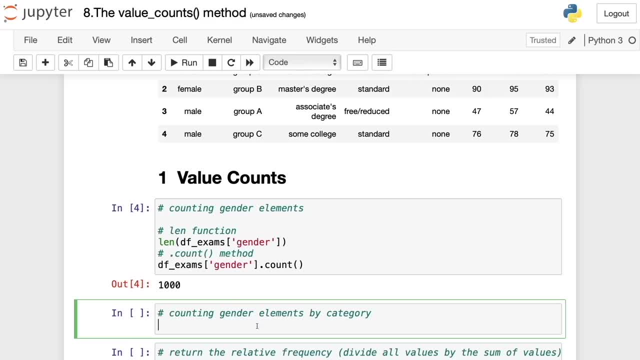 the column. So to use this method, we only have to write the name of the data frame followed by the column that we want to count. So in this case is that gender column? And then we have to use the value underscore counts method, as you can see here. So now we actually 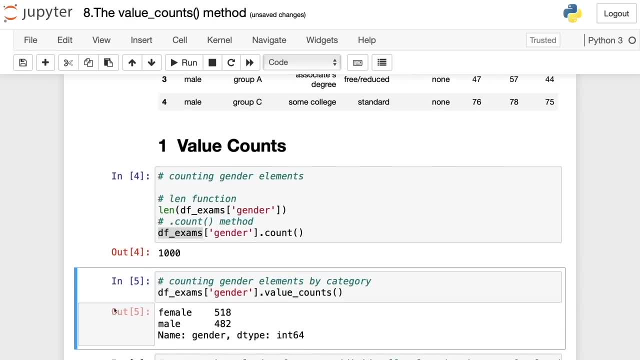 have to use the value underscore counts method. So now we actually have to use the value underscore counts method. So now we can execute this And, as you can see, here we have not only the total rows in this gender column, but now it's divided by category. So we have that. 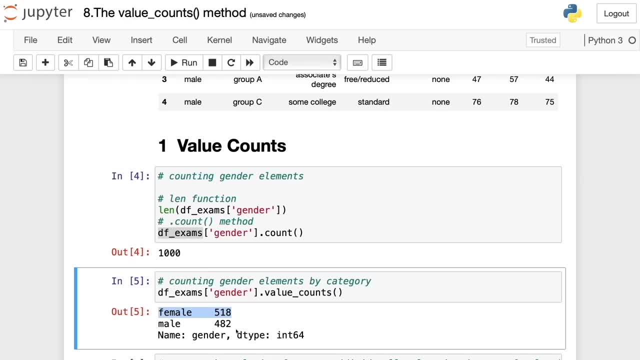 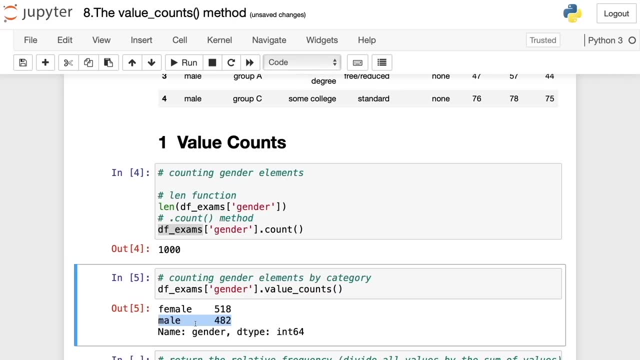 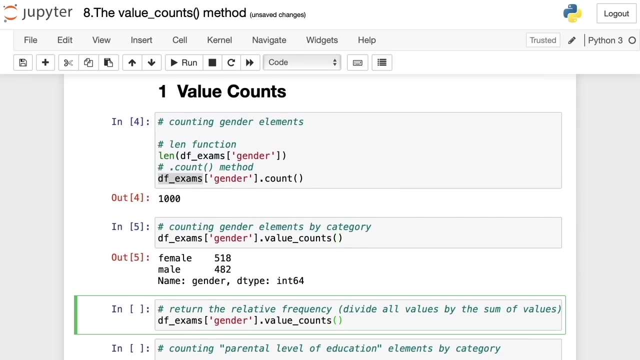 there is 518 females and 482 males. So this is how the data is spread in the gender column. So now we can do more with a value counts method So we can get the percentage that each category represents All column. So here I'm going to copy this And now to calculate the percentages also. 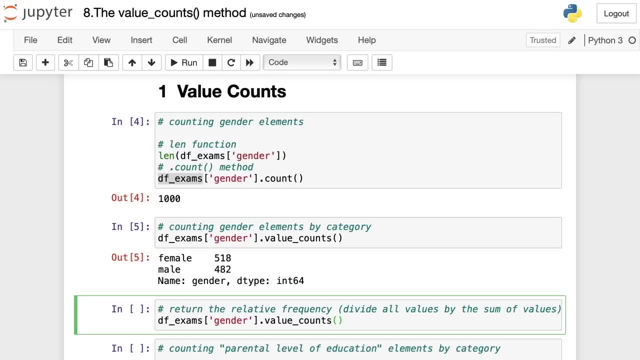 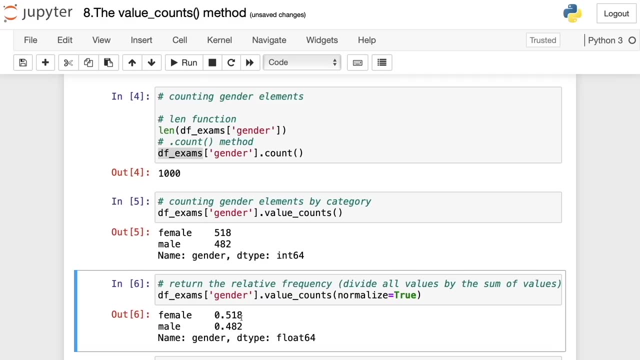 known as relative frequency. we have to add an argument named normalize. So we write normalize equal to true And then we execute this And, as we can see here, female represent 51% of the total observations in the gender column, While male only represents 48% of the total observations. So, as you can see here, the 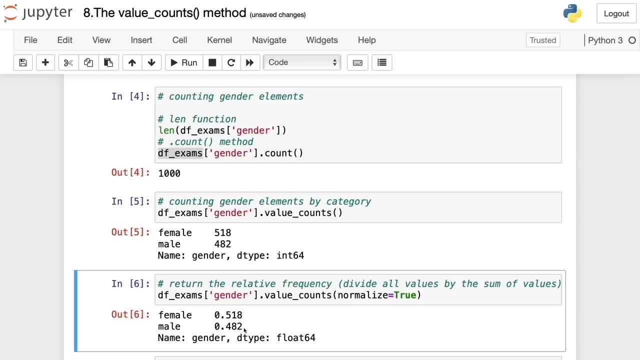 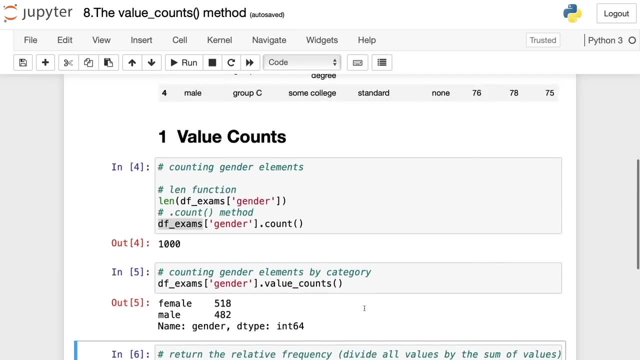 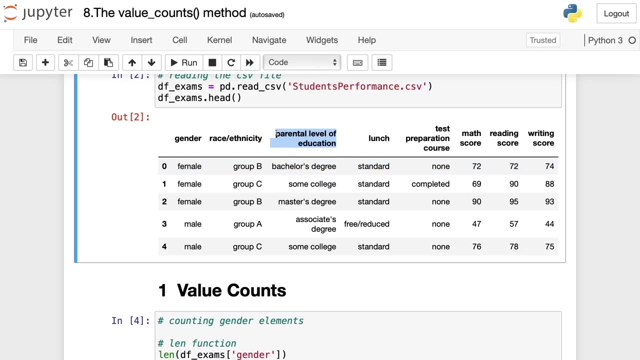 value counts method is useful when you want to have a look at the data by category. Okay, now let's see another example, And in this case let's pick a different column. So here I'm going to choose this parental level of education column. I copy this, And now let's 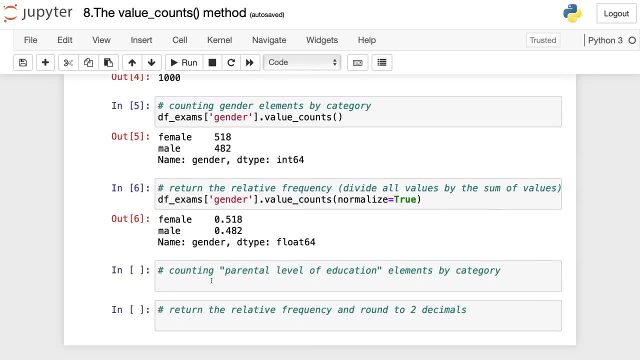 calculate. let's count the elements by category. So here I'm going to write the name of the data frame, the exams, And now I open square brackets, quotes, in here I paste this column now to count the elements by category. In this column we use the value underscore counts. 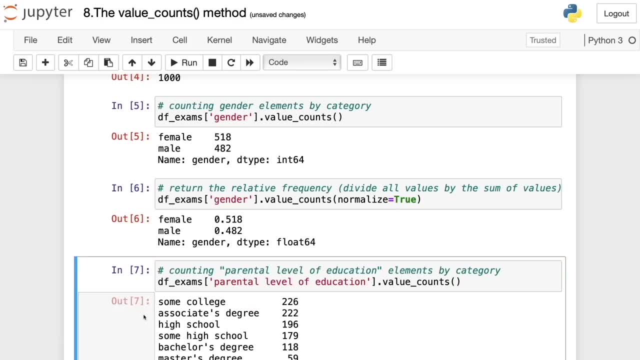 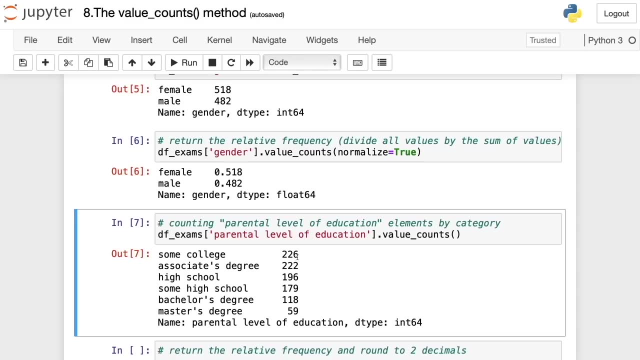 method. So we run this code And here you can see how the data is divided In this column. so most people have some college level of education, while just a few people have a master degree. And now if we want to get the percentages that represent each category, 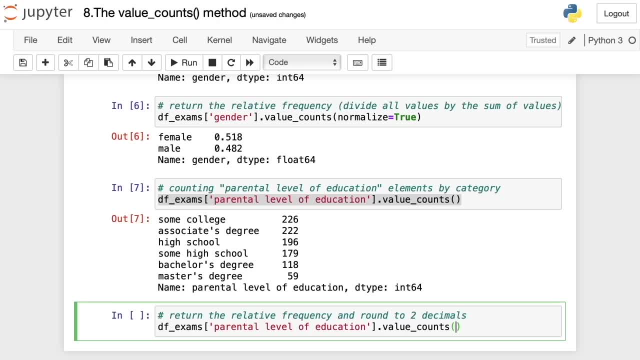 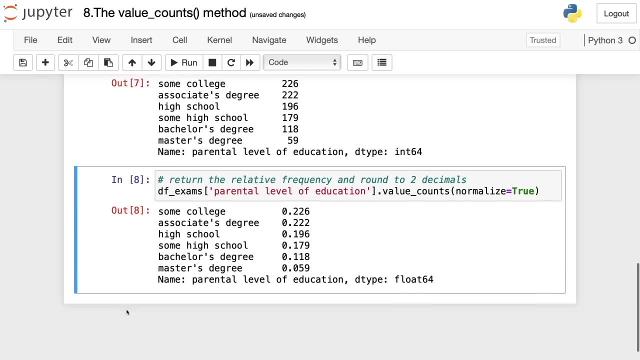 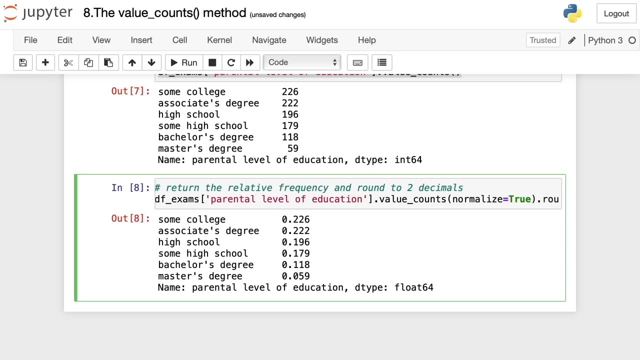 we again use the normalize argument. So we write normalize equal to true. And now we're going to get the percentages, So we can see the percentages. And if we want to round this to two decimals, we use the round method. So we write that round parentheses. and now 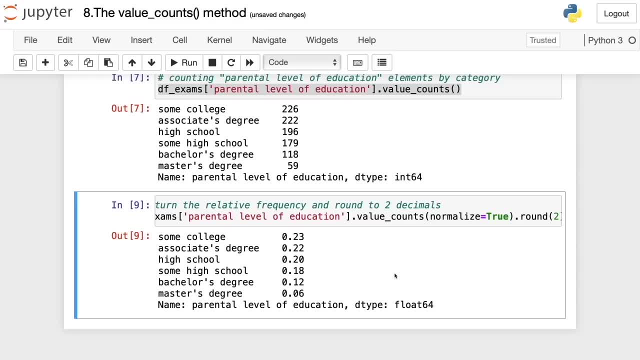 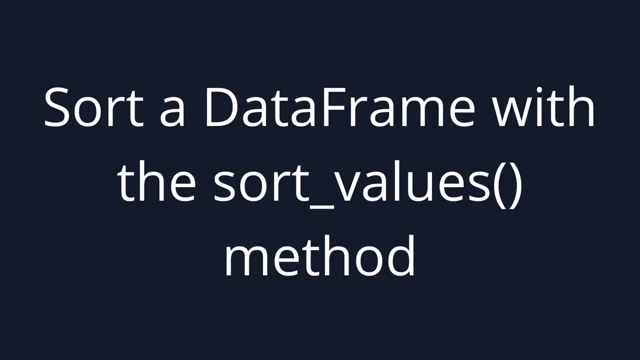 two decimals, And, as you can see here, we round it to two decimals, And that's it. Now you know how to use the value counts method. Okay, in this video we're going to see how to sort a data frame using the sort underscore. 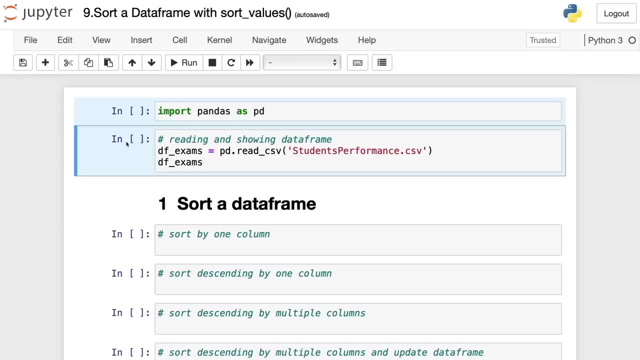 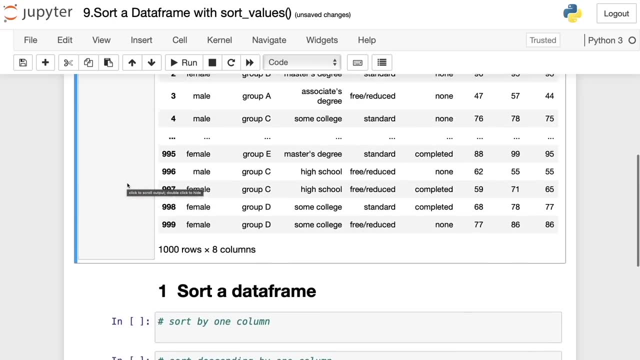 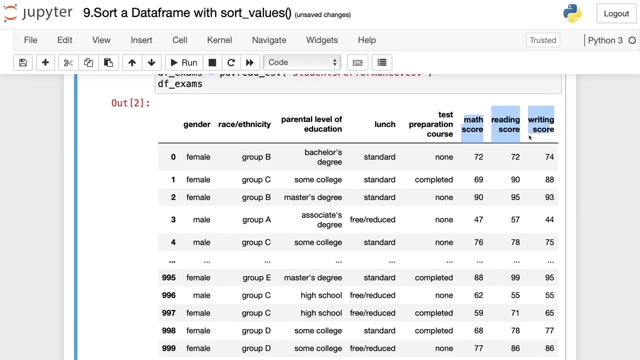 values method. First let's import and read the CSV file that we've been working with in this tutorial, And now let's sort the data frame. So here we have the data frame And, as you might remember it's it has these three numerical columns, And now I'm going to sort it using one of 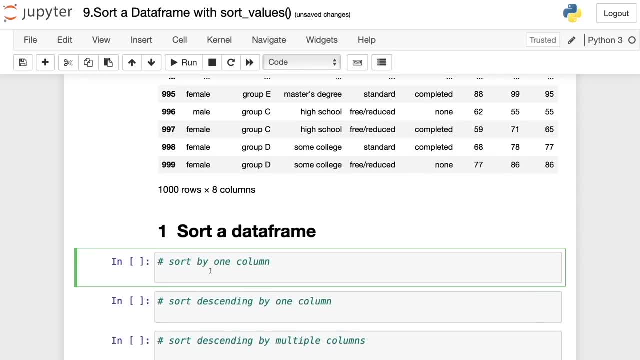 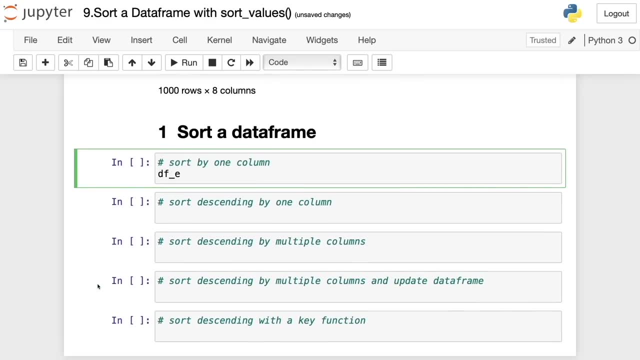 these columns. So let's use the sort underscore values method And first I'm going to write the name of the data frame, which is TF- underscore exams- and then write sort underscore values. Now I open the data frame and I'm going to say sort underscore values And I'm going to 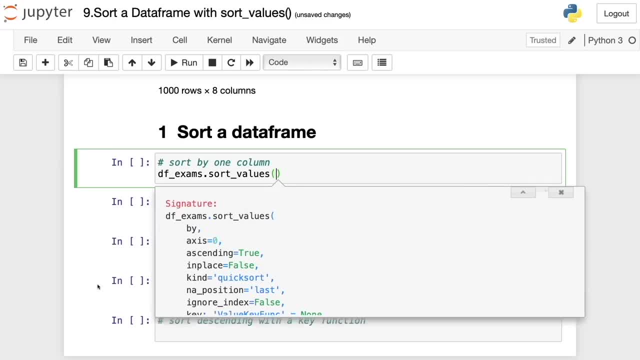 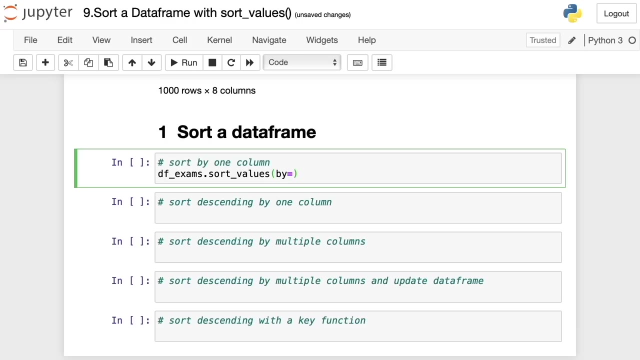 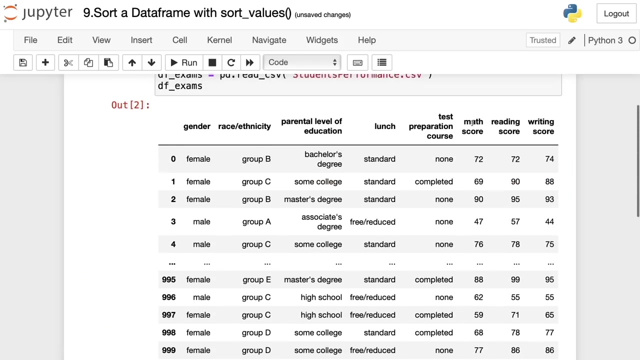 parentheses. And now I can use this help here And, as you can see, the only mandatory argument is by. so we can use this one by and this one. we have to specify the name of the column we want to sort by. So in this case I want to sort by the math score, So I'm choosing this numerical column to start. 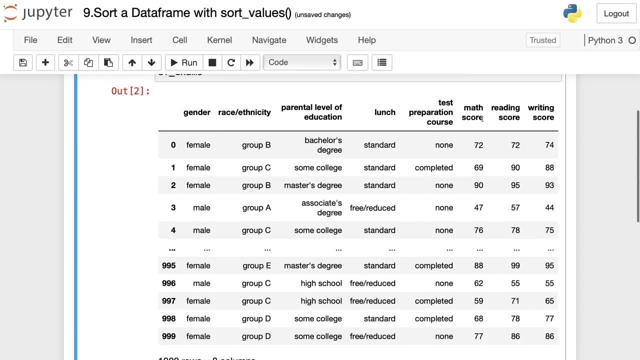 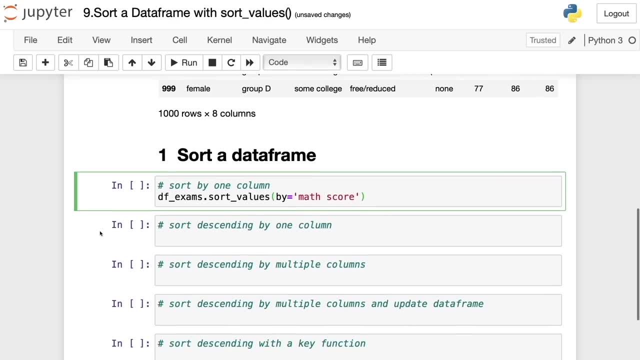 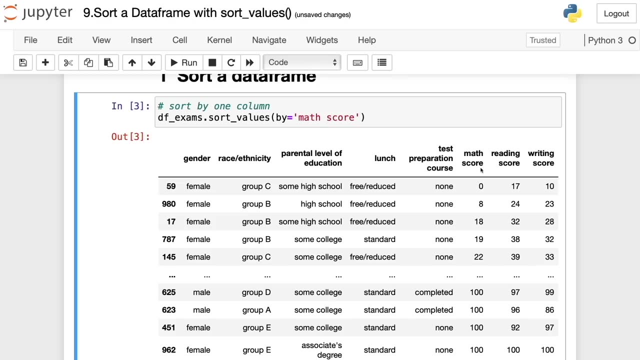 with. So I'm going to write math score- Actually, I'm going to copy this one and paste it here. So by math score and sorting this data frame is as simple as that. Now we can run this code And, as you can see here the data frame was sort ascending by default, So it starts with zero and it ends. 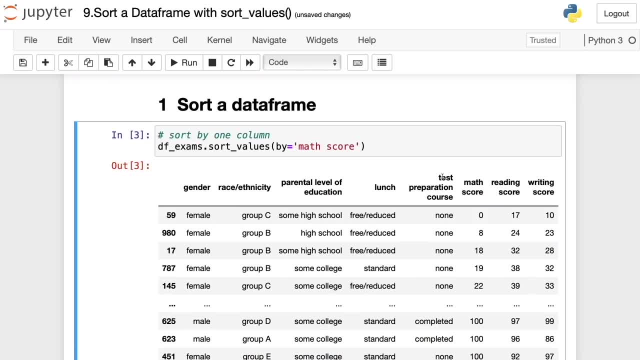 with 100 in the math score. So this is how the sort underscore values behave by default. And here one little detail: you don't need to specify the byte word, we can omit it And we run this And as you can see here it still works. So here we can modify that default behavior of the sort. 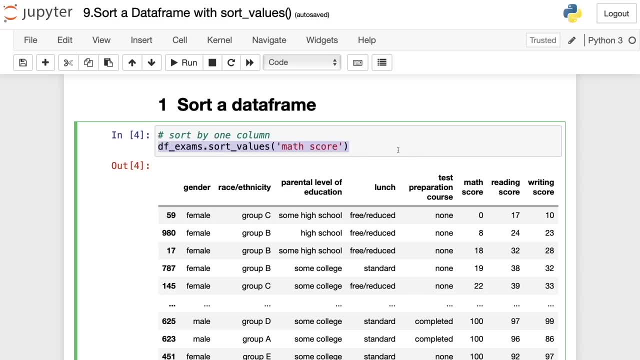 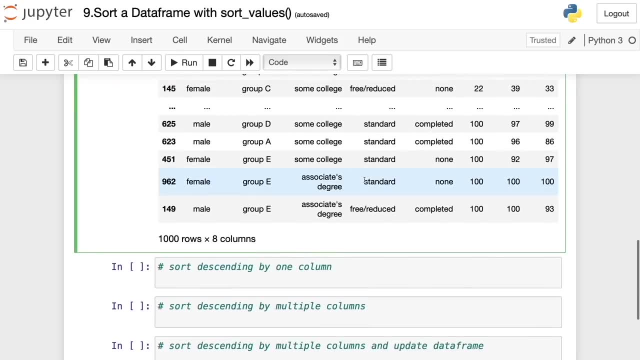 underscore values method. we only have to add a new argument, and is that ascending argument. So let me show you here. I'm going to copy this one first and show you here. So in this case we're going to sort descending by the same column. 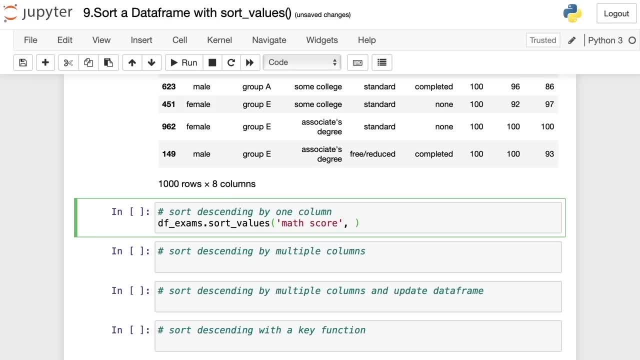 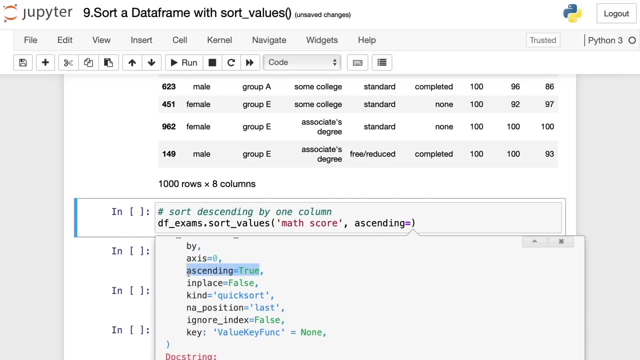 So we only write comma and then we specify the sending arguments. we write ascending equal to. and here I want to show you something in this little help here. here the sending is set to true by default. This means that is ascending by default. But we can change this. 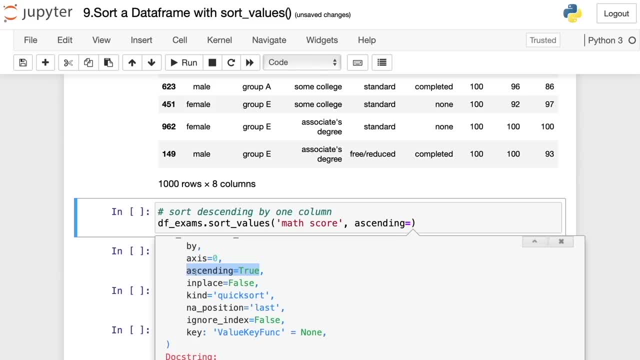 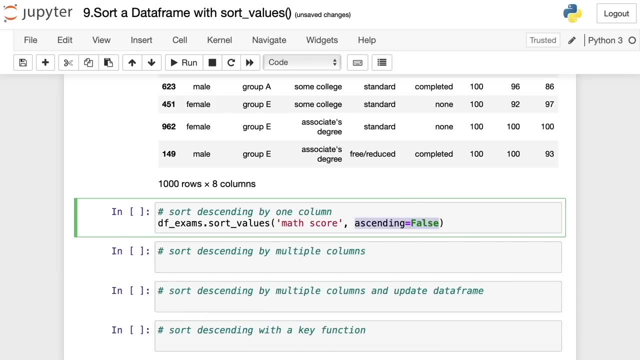 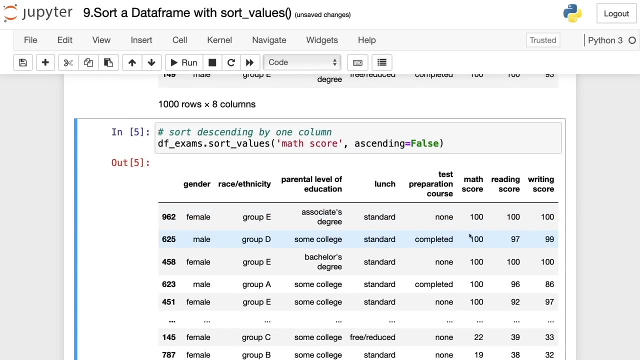 default behavior by setting ascending equal to false. And that's what we're going to do here: ascending equal to false, So it means descending. And now I'm going to run this one And, as you can see, here is sort descending by the math score column. So here it starts with 100. And it ends with zero. 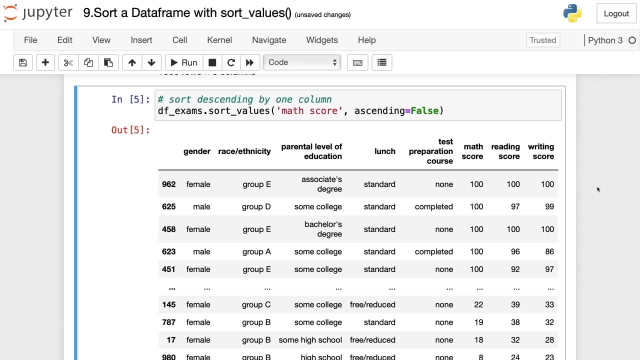 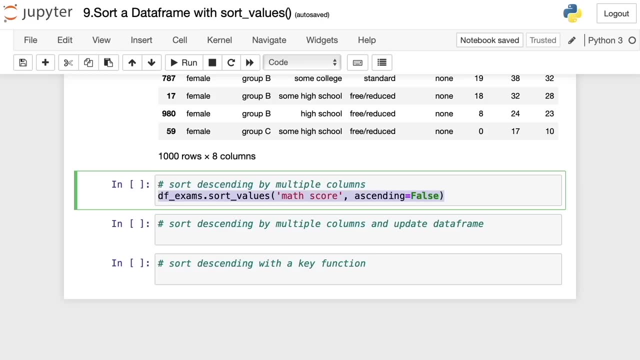 But that's not all. we can do much more with a sort underscore value method. So first I'm going to show you here how to sort by two different columns. So here let's copy and paste this one. So in this case we're going to sort descending by multiple columns. So instead of 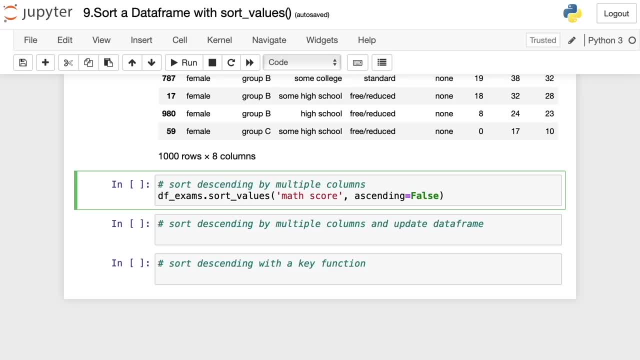 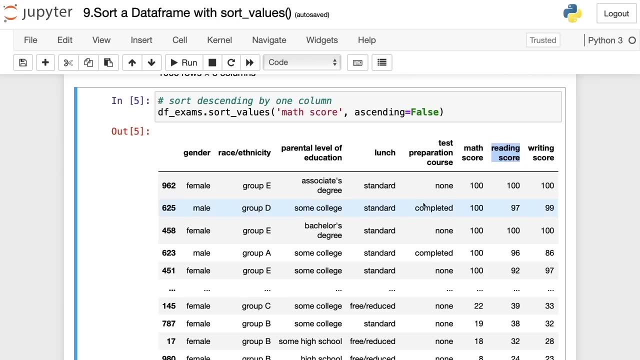 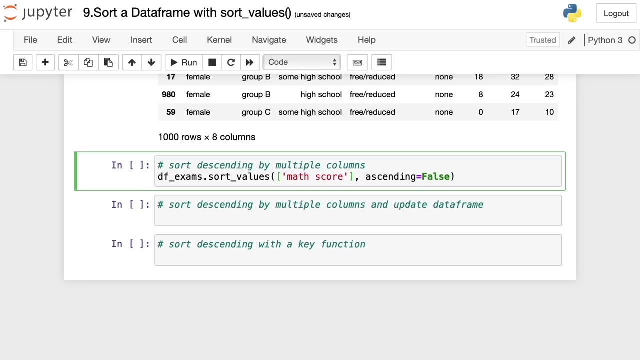 writing only math score. we're going to add here one more column and it's going to be the reading score column. So here I copy this one. I'm going to copy and paste it here, But first we have to add the square brackets because, as you might remember, when we write two or 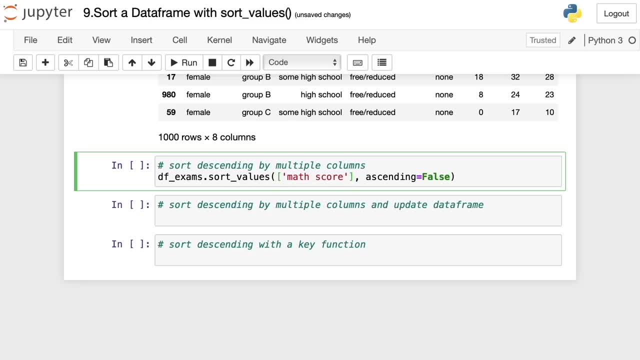 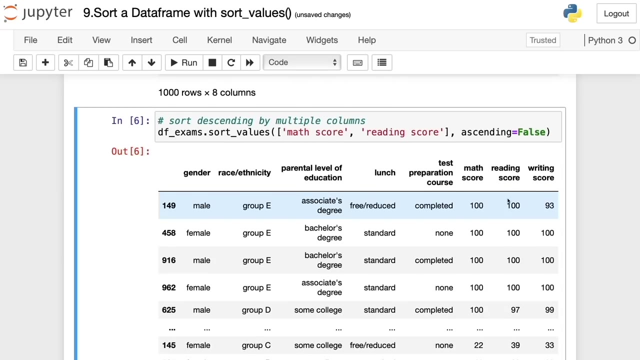 more columns. we need the square brackets. Now we write comma and I paste this reading score. Now I add quotes And that's it. That's everything you have to do to sort by multiple columns. Now I'm going to run this one And, as you can see, here it was sort. 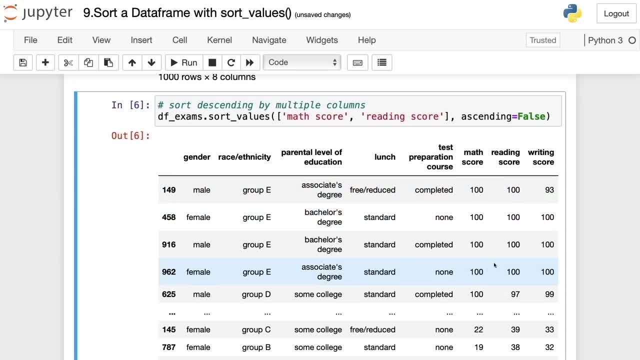 descending first by the math score column and then by the reading score column. So the priorities are set here in the list that we include the here. So first is the math score column, first priority And the second priority is the reading score column, And that's what you can see here. 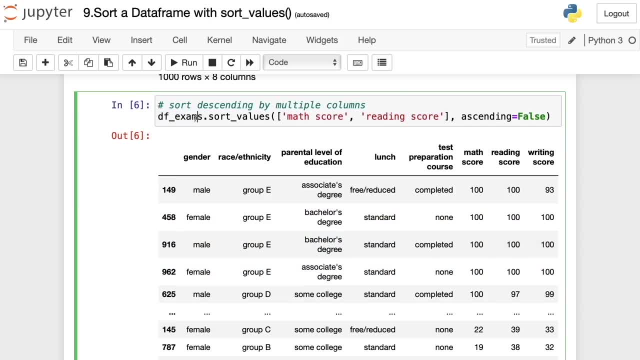 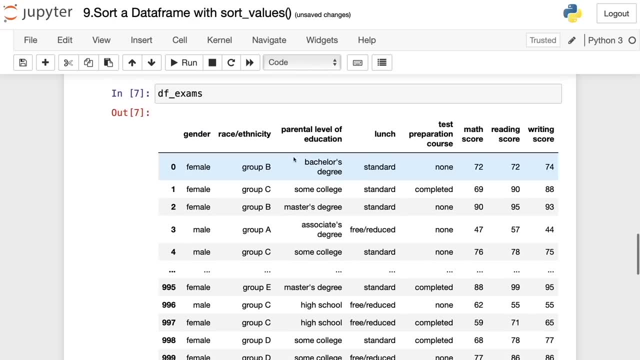 Now I'm going to show you a little detail here. Let me copy the DF underscore exams And if I print this one, you can see that the changes we made weren't updated. So this here, the math score column has the original values. This happens because the sort underscore values method 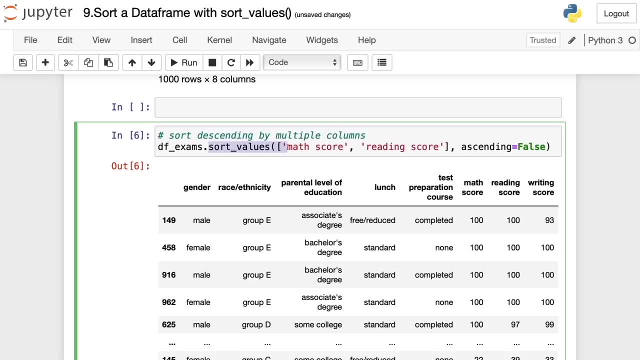 like many other patterns method only create a copy of the data frame. So here we obtain a copy. this one is a copy, but it doesn't update the values of the data frame unless we add a new argument, which is the in place argument. So I'm going to show you here, But first I'm going to delete this. 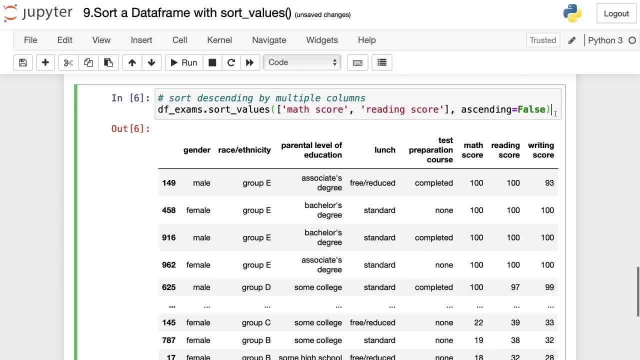 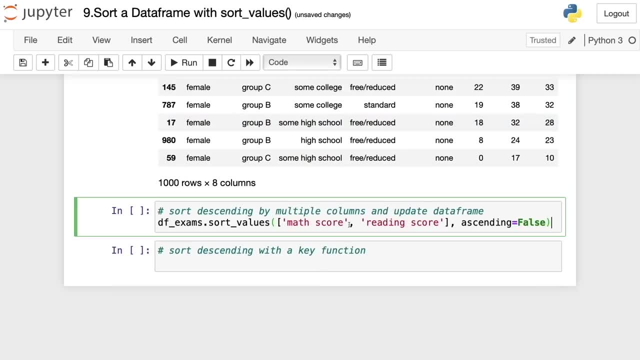 DF underscore exams. And now I'm going to copy this one and show you how to update the values of this data frame. So here I'm going to copy: those are the same values. But now I'm going to add a new argument, which is the in place argument. So here, right in place, equal to 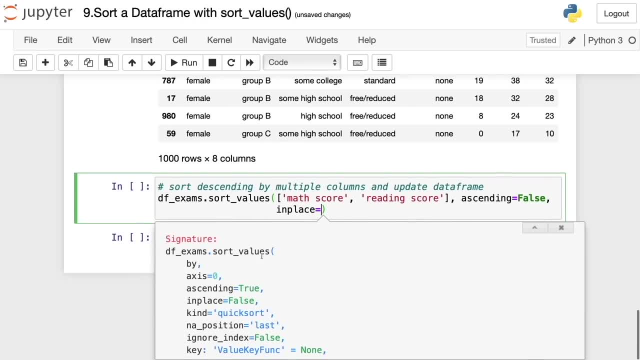 you know I'm going to show you the default value. So here the default value of in place is false. This means don't update the data frame, but only create a copy. But if we set it to true, it means update this data frame. So here I'm going to set it to true, to update the data frame. So here: 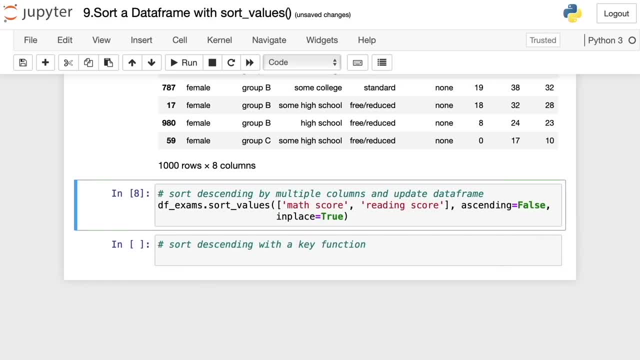 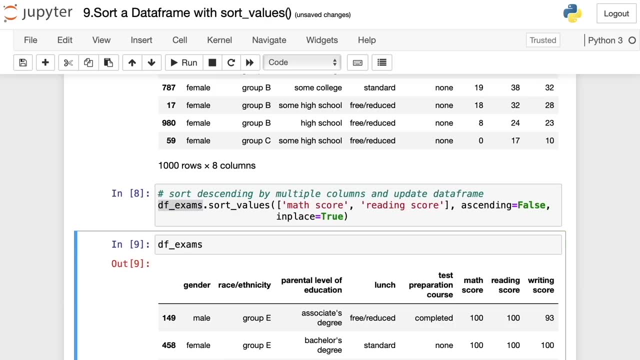 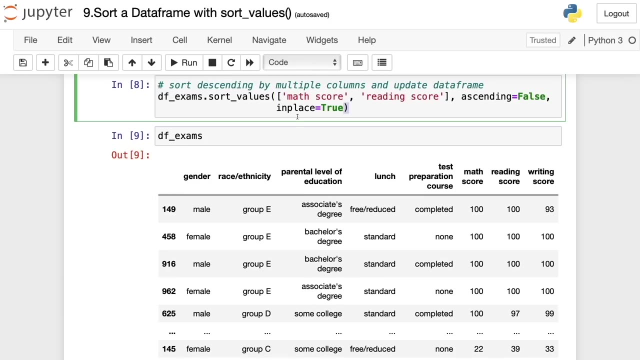 I write true And now I run this and apparently nothing happens. But if now we print that DF underscore exams data frame, we're going to see that we have the data frame sorted. In case you don't want to add the in place argument and you want to update the values of the data frame, you 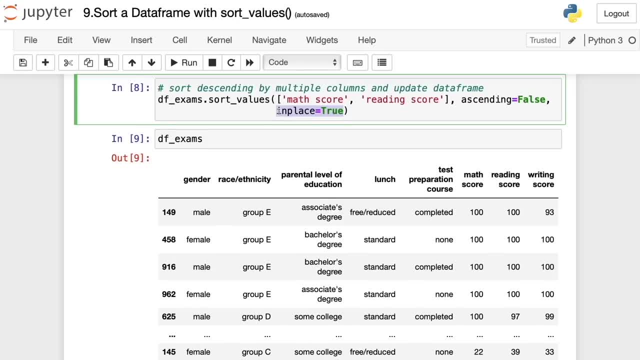 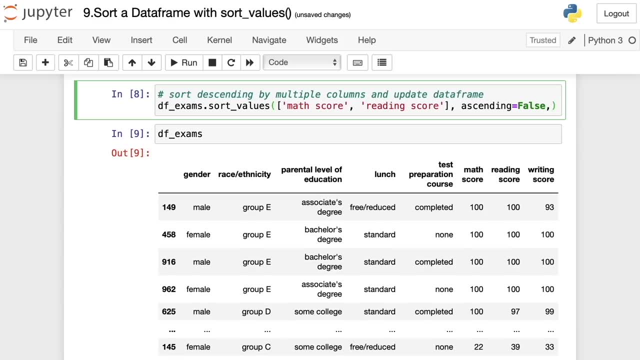 have another option that we used before, which is overwriting the values of this data frame. So, for example, you can only delete that in place argument and write DF underscore exams equal to this. So this is overwriting the values, But in this case we're not going to do that. We're going to 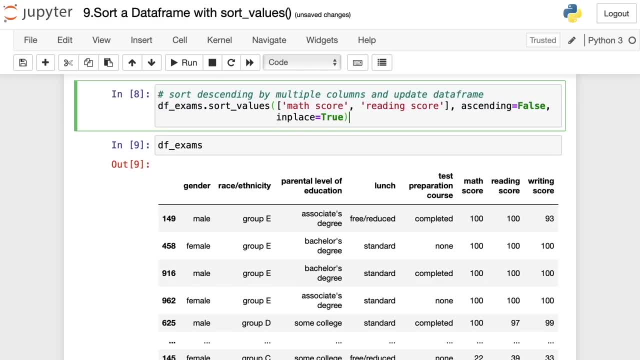 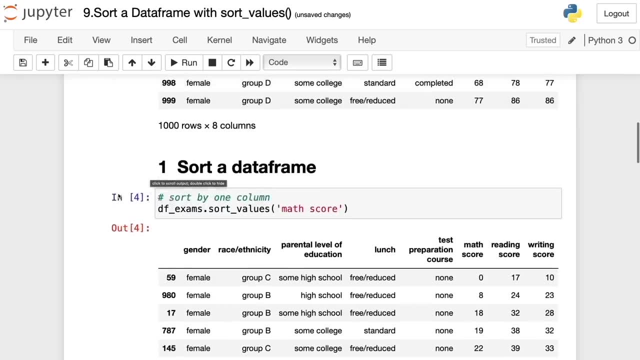 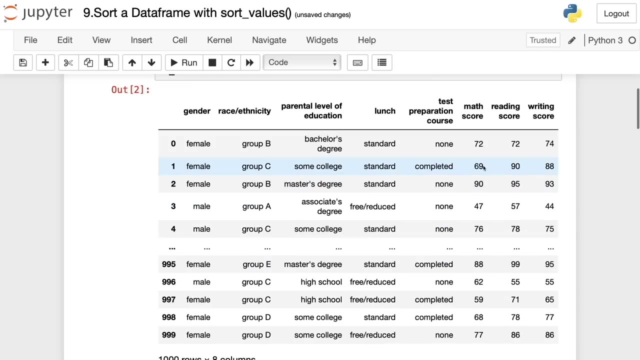 add that in place argument, as you can see here. Finally, we're going to see how to sort, but now not with numerical data, but with text. So, as you can see here, we before sort this data frame by the math score column And this one has this numerical data. But 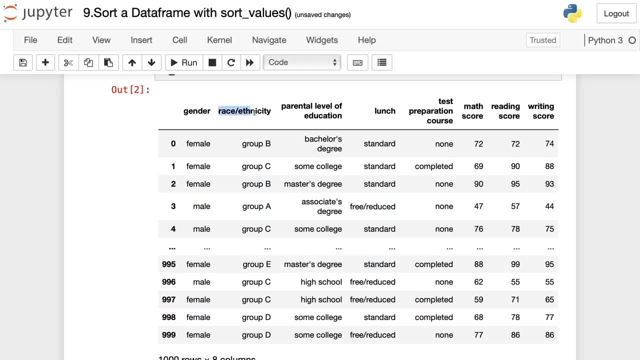 in this case we're going to sort it by that race, ethnicity which has this text. So we're going to sort this one. So first we're supposed to get group one and then group B, C, D, E and so on. 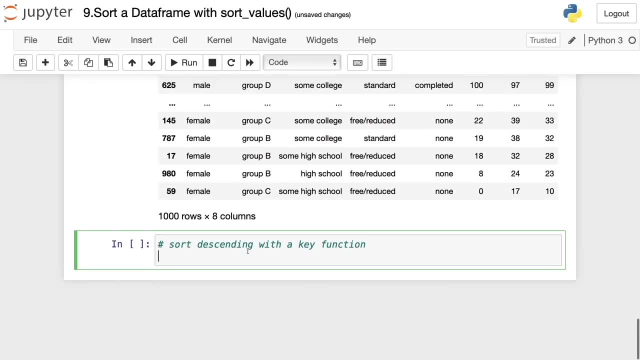 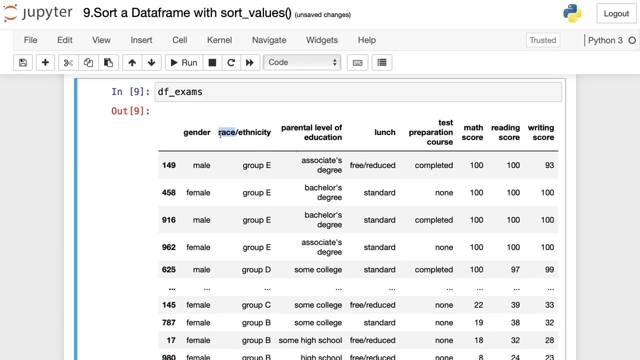 So let's do this here. I'm going to scroll down And first we have to write the name of the data frame, followed by the sword underscore values method, And now specify the name of the column. So here I'm going to copy race ethnicity here. Let me copy here And it's done. Now I have the 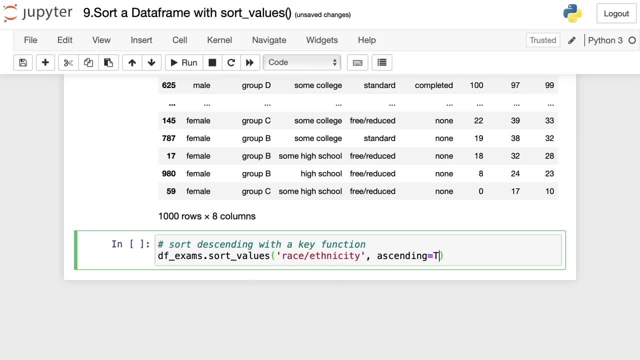 name of the column I'm going to set to ascend into true. And now that new argument we have to add to sort This is that key. So I add key then equal to. in this case, we're going to use the lambda function. I'm 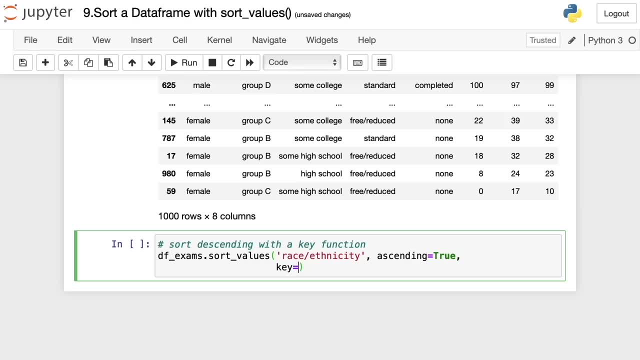 not sure if you're familiar with the lambda function, But it works. similar to an average function we've seen before in the Python crash course, But in this case it's going to behave a little bit different, So let me show you here. 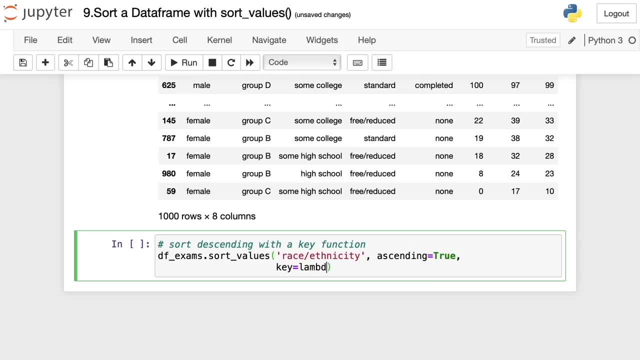 First you have to use the lambda keyword, So we write only lambda. And now we should write the object that is supposed to return. In this case, I'm going to write call that stands for column. And then we have to write column in a specified operation. we have to 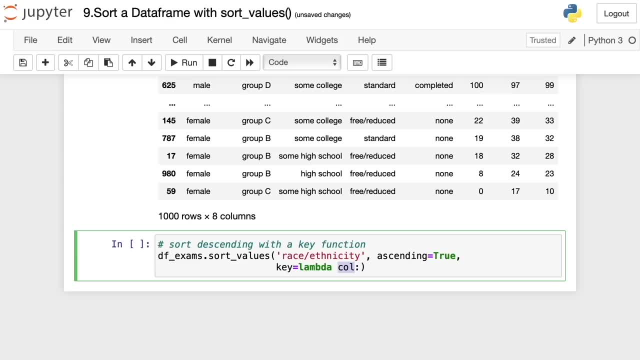 make over this variable. So in this case I want to write column or call and then access the string attribute. So I write that str and then use the lower method. So what we're saying here is get the string values of the column and then transform it to lowercase. So here: 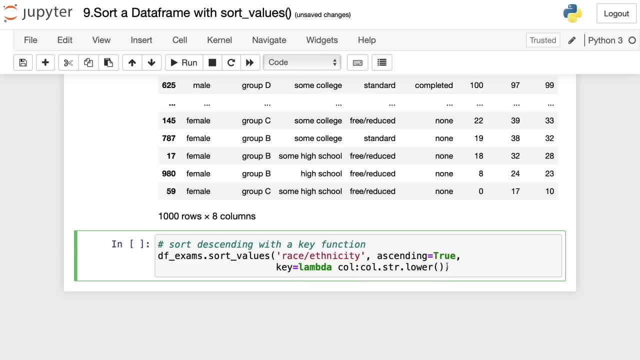 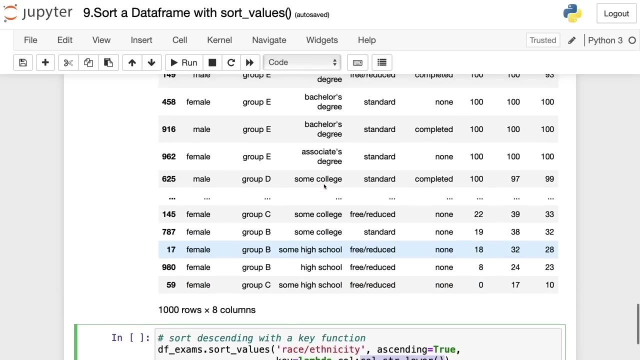 we get that textual data in lowercase And with these three arguments we're saying: sort the values inside the race ethnicity column and sort it ascending and then sort the textual data of this column in lowercase. So here we have this A, B, C, D, E in uppercase, but we're going to get it in lowercase and 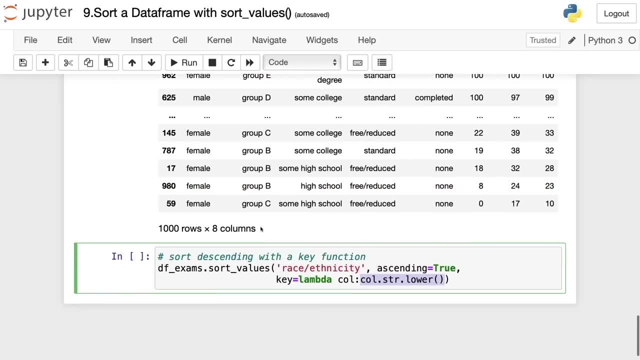 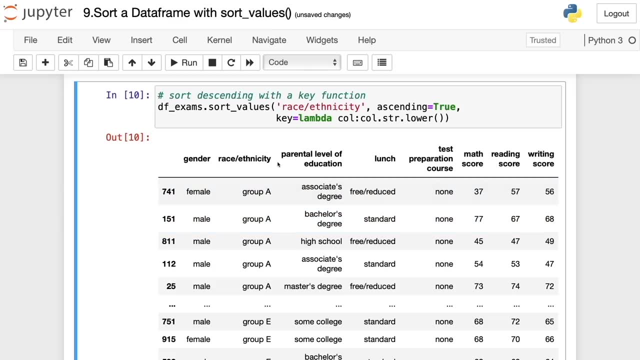 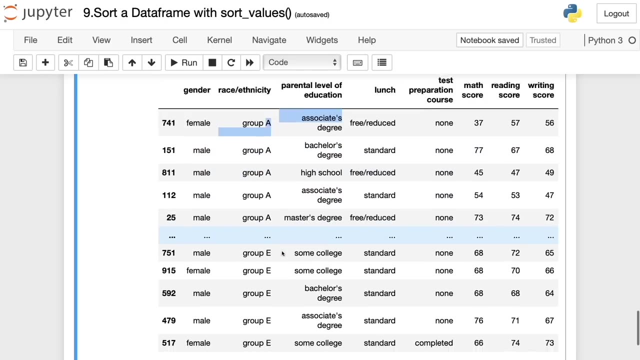 sort it by this text data. So now let's run this one And let's see the results. So, as you can see, here we have this race ethnicity column and its order ascending. So here we got the A and B and C and D and so on, And that's it. These are the different ways. 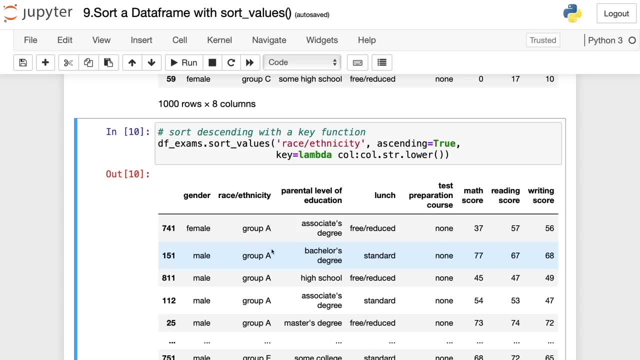 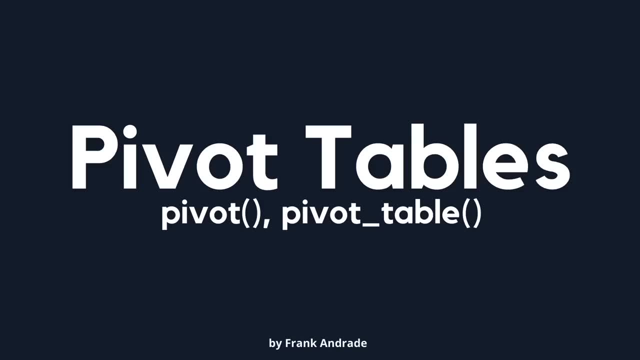 to sort a data frame using the sort underscore values method. Welcome back. In this video we're going to see different ways to make pivot tables. If you're an Excel user, probably you made many pivot tables in the past. In pandas we can also make pivot tables And 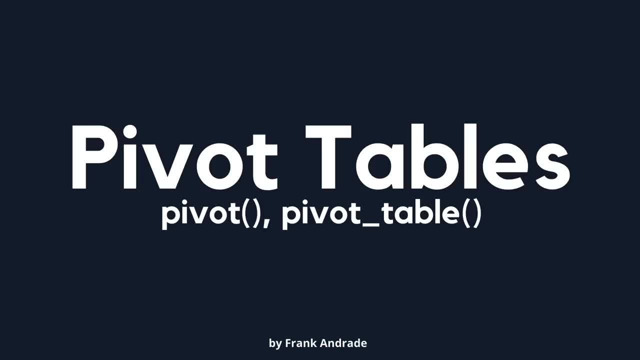 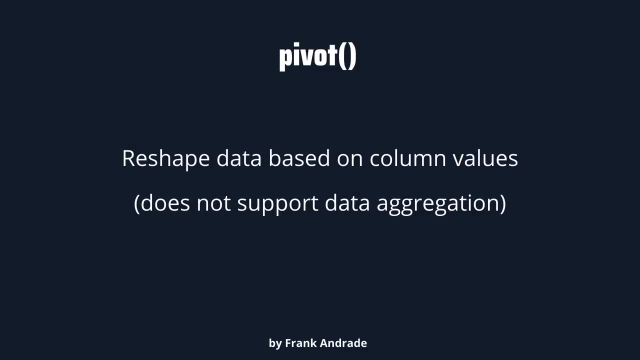 in this case, we use two different methods: the pivot method and a pivot underscore table method. In this video we're going to see the difference between the two of them. So first let's see what's the pivot method. So the pivot method reshapes data based on columns, values and 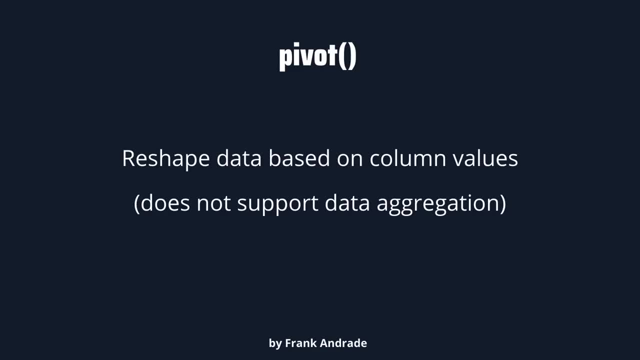 it doesn't support data aggregation. So this means that this is not a regular pivot table. you will see in Excel, because you can only reshape data with the pivot method And you cannot do anything else. to explain you better what the pivot method does, I'm going to show. 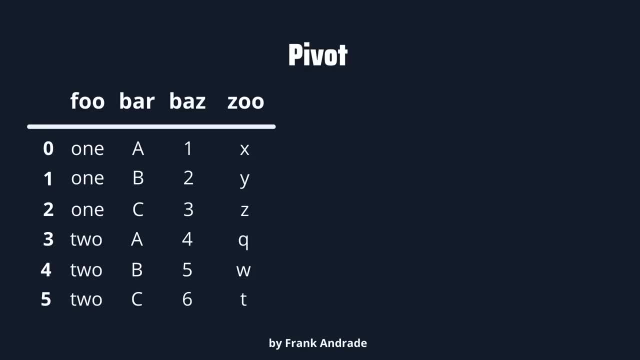 you an example. So here we have a little data frame, And this one has six rows and four columns And, as you can see, here there are many duplicate values. For example, in the column foo the one value is repeated at least twice, And the same goes for the two value. 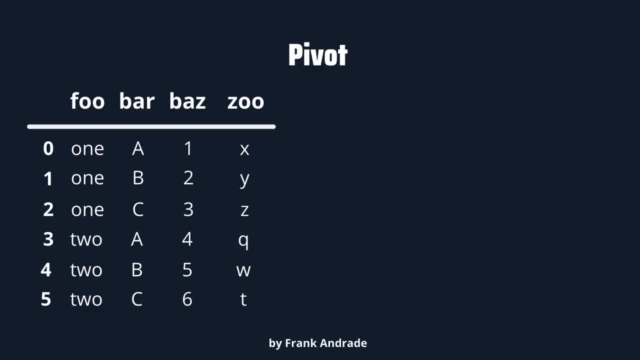 Also, in the column bar you can see that the A, B and C is duplicated. So when we have this type of data frame, we can reshape data. We can reshape it to have a different view And to make a better analysis. In this case, 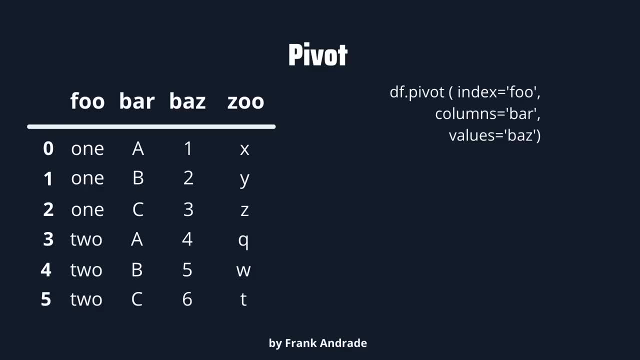 we can use the pivot method, As I'm going to show you right now. you only have to write the name of the data frame, followed by the pivot method, and then specify three arguments. So the first one is the index. In this case, I'm going to reshape this data frame, choosing. 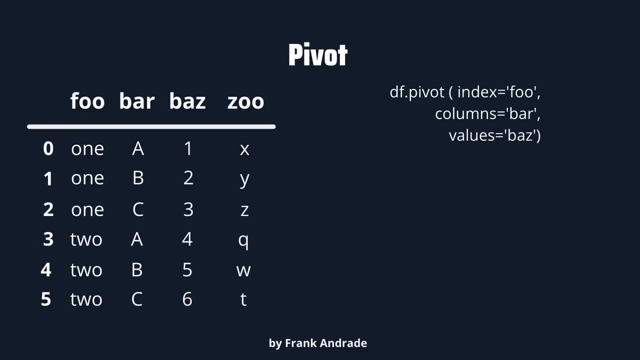 the column foo as an index, And the second one will be in the position where is, right now, the numbers from zero to five on the left. Next you have to define that column. So these are the new columns that we're going to see in our new data frame, the one that we're going to reshape. So in 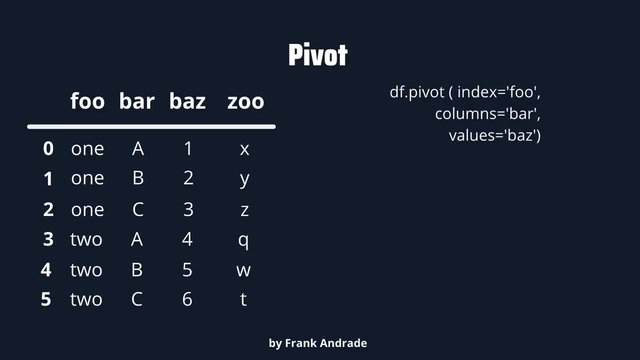 this case I'm selecting the data inside the bar column as new columns. This means that A, B and C will be the new columns in our new data frame. Finally, we have to choose the values we wish to show in this new data frame. So in: 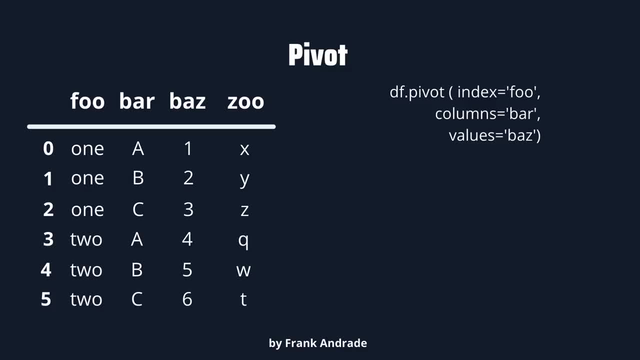 this case, I'm choosing the best column, So all the values inside there will be shown in our new data frame. So this is the column that I'm selecting, And now I'm going to show you the result of this pivot method. So here it is, And, as you can see, here we have the 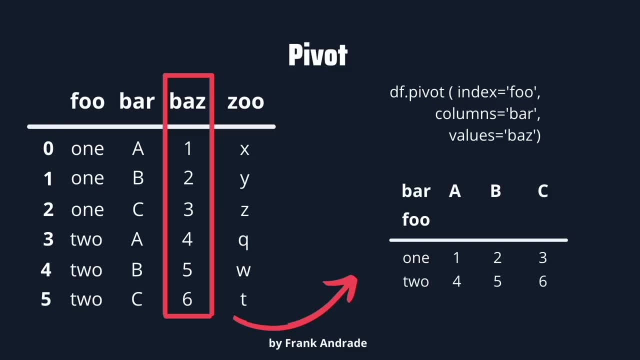 foo in the index, as I told you before, And the A, B and C that are data from the bar column now are columns in this new data frame. Also, all the data inside this best column is the only data that is displayed. 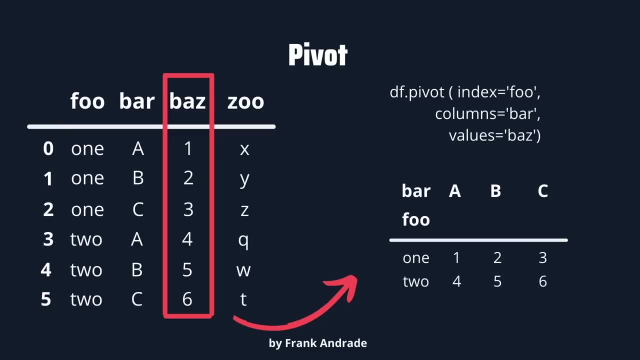 in this reshaped data frame. And now let's see why it's sorted this way. So why one is here, two is here, three is here, and so on. So here the value is defined by the index or row in the column. So between one index one and column A is one, And why that happens. 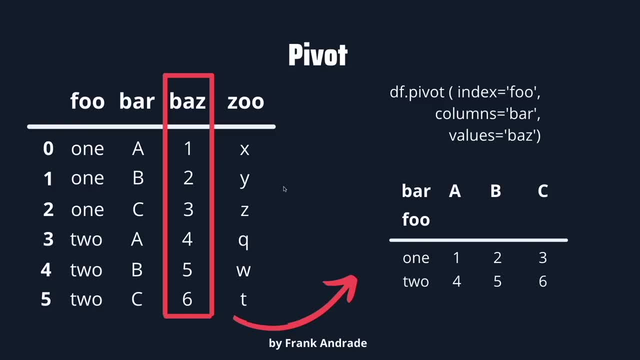 Because if we go to the our previous data frame, or the original data frame that is here, we can find that here is one a and the value that corresponds to that pair is the number one. So let's pick another one, for example five. here we have two, and 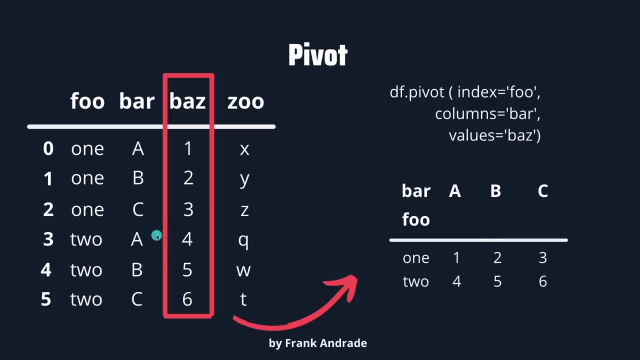 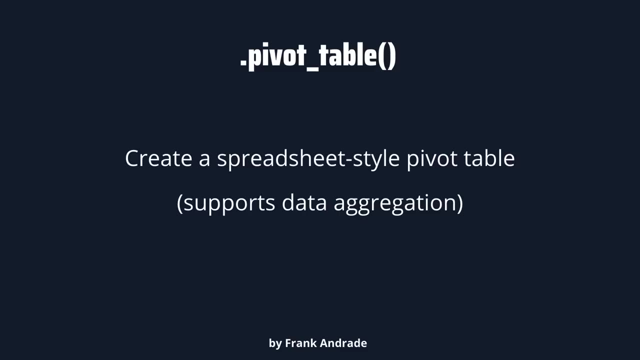 B, And if we go here to our original data frame, we have that two and B, the value that corresponds to that pair is five. So that's why this value is here And that's how this new data frame was reshaped. Okay, and finally, we have the pivot underscore table method. 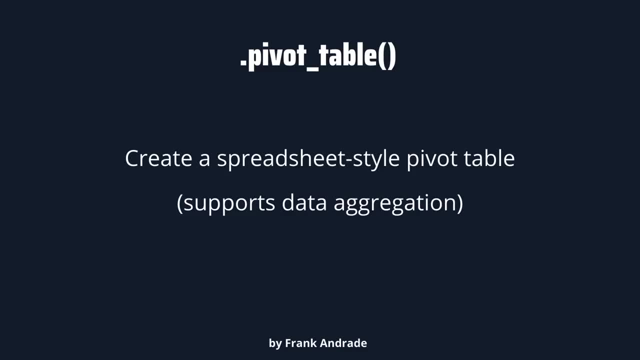 And this one creates a spreadsheet style pivot table. So this is similar to the pivot table that we will focus on in the next video, find in Microsoft Excel, for example, and this one supports data aggregation. And to explain you more about the pivot underscore table method, as well as the pivot method, 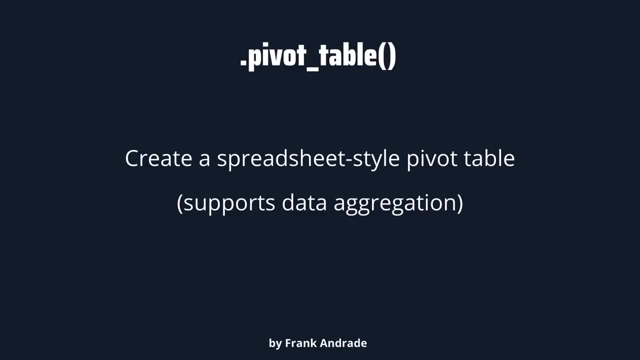 we're going to see some examples in the next video, And this time we're going to write some code so you can understand much better what we're doing. Alright, now it's time to see how the pivot method works in action in pandas. So first, 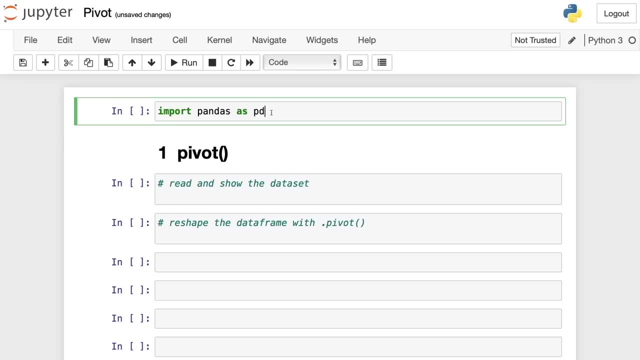 as usual, we import pandas as PD. So here I import this library And then we're going to use a different data set to work with this pivot method. So to read this data set, we use the PD, read underscore CSV method And insert parentheses. we write the name of this. 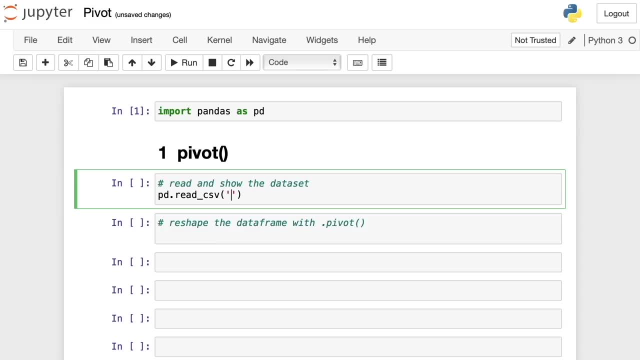 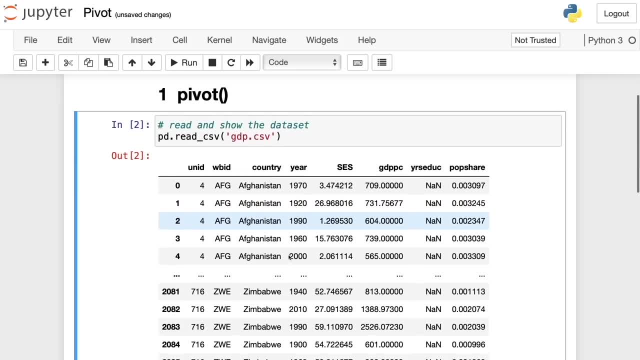 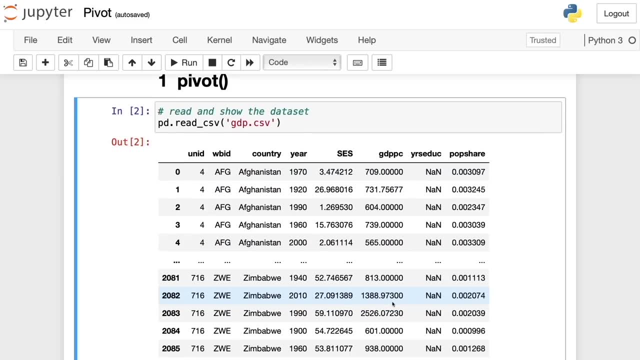 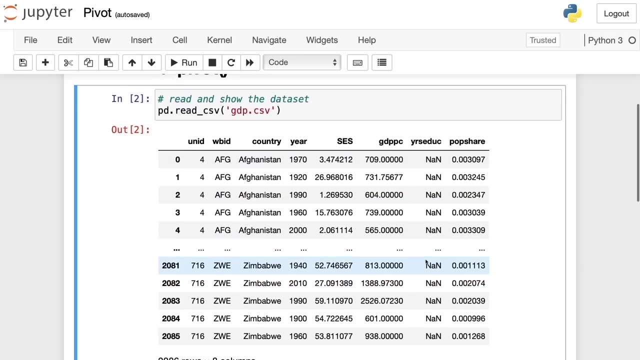 a look, I'm going to run this one And, as you can see, here we have data about GDP per capita. that is in this column, And basically this is how the GDP grow over the years for each country. So here I'm going to tell you which are the columns we're going to use for. 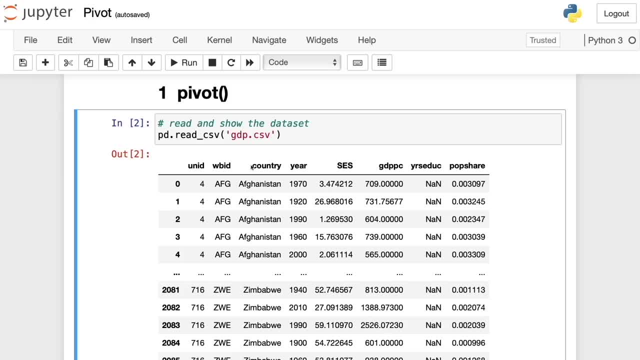 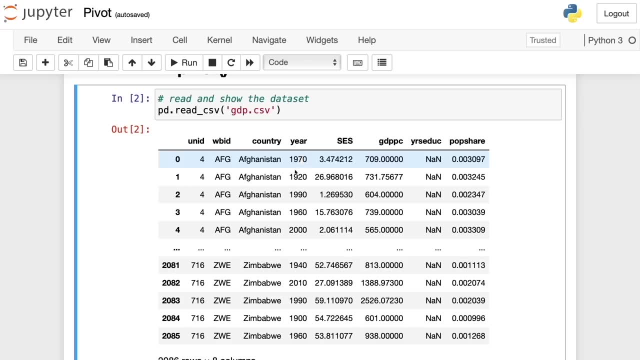 this example. So first we're going to use the country column that contains data about different countries, then we're going to use that year column that well, contains different years and that GDP per capita that it's in this column. So, basically, what we want to do in this exercise is to 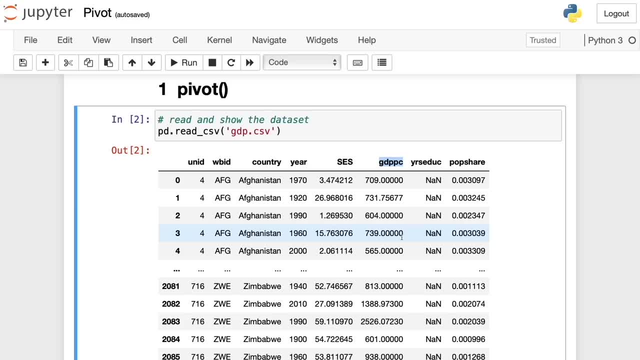 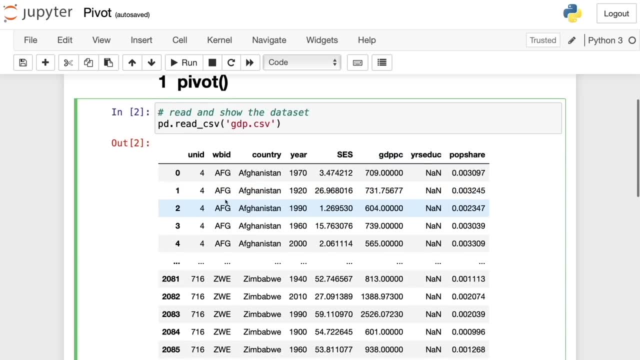 obtain a different view of our original data set. So this data set that we're reading here on this canvas has this view that we want to get a different view, to have a better analysis. So the goal of this exercise is to see the evolution of the GDP per capita over the years. 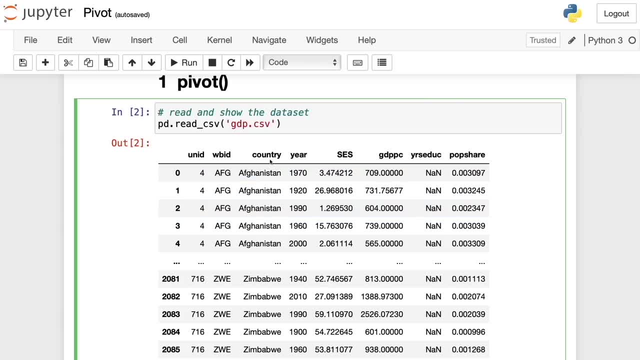 for each country And then we're going to put the country names in the columns. So the only data we're going to show in our new data frame is going to be that GDP per capita. that it's here. So I want to show you now this with code And let's write it here. But first, 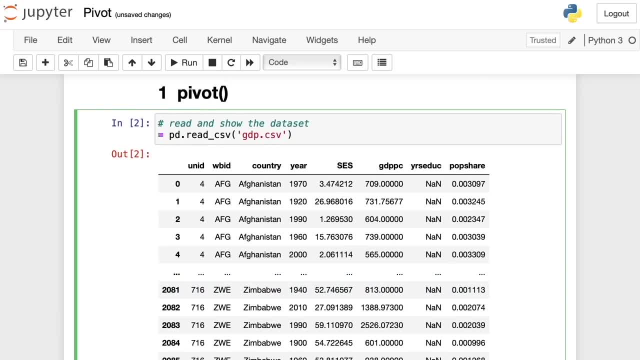 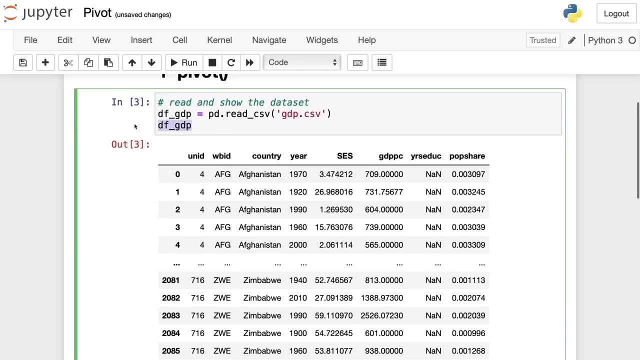 let's assign a variable to this data frame. So here I'm going to write the F underscore: GDP. So this is the name of my data frame And now I'm going to show it and it's here. So now I'm going to copy this data frame And to use the pivot method. I'm going to 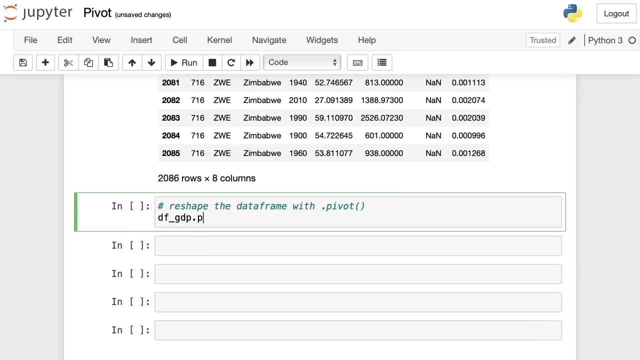 paste this one And now write that pivot. Now we open parentheses And now, as you might remember from the previous video, we have to introduce three different arguments. And if you don't remember the three different arguments we have to introduce, here you can. 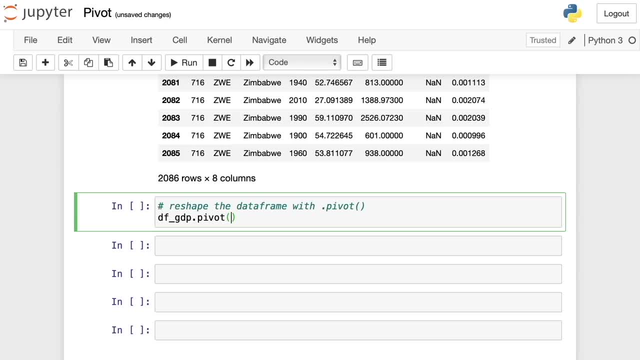 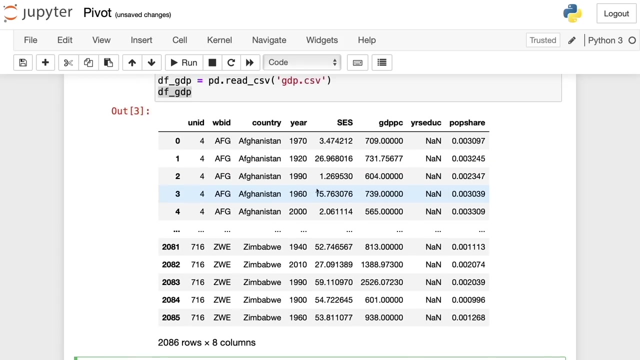 only press the Shift and Tab keys on your keyboard and you will get this. And here you can see the three arguments I'm talking about. So first we have to write the index argument, So we write index And, as I told you before, I want the year column to be the index of my new, reshaped data frame. 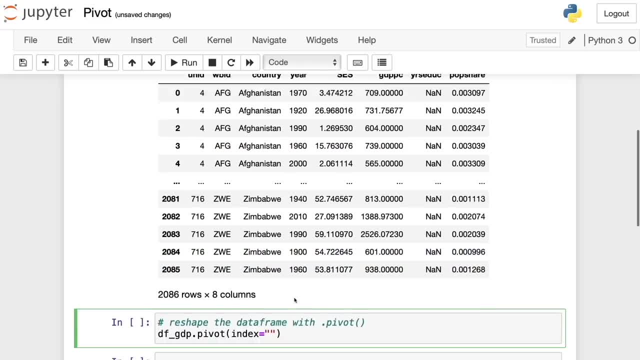 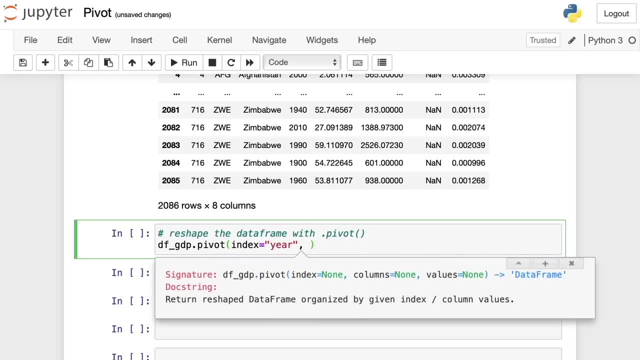 So I'm going to set this year as the index of my new data frame. So I write here year Next we write comma and press Shift and Tab to show this. So the second argument is the columns. So we write columns, then equal and open quotes. So here, as I 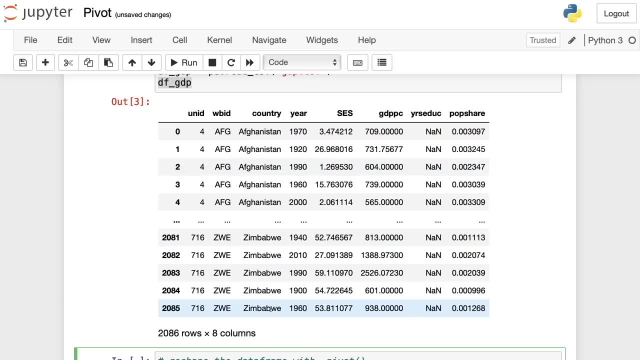 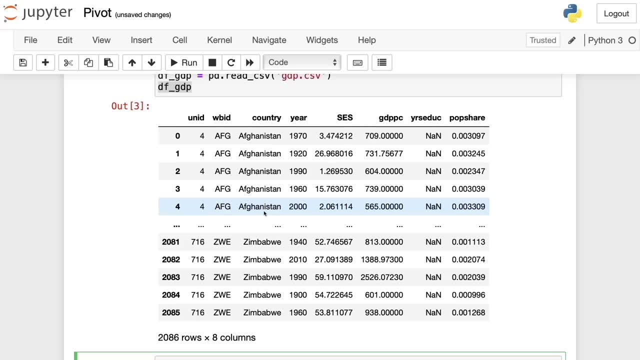 told you before, I want the countries here listed in the country column. I want each country to be an independent column. So for example, here let's say we have the United States, So I want the United States to be column number one, then column number two. 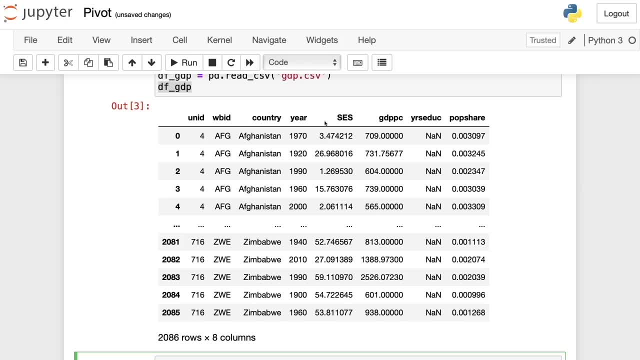 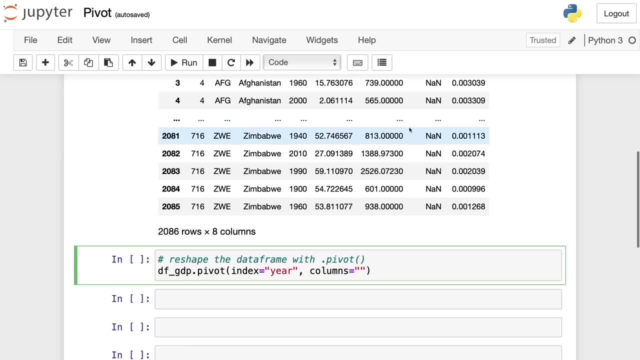 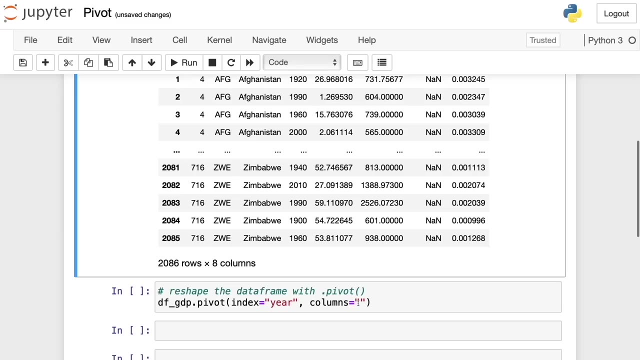 China, then Australia, then Spain and so on. So each country should have one independent column. So that's what we want, And to get that we have to set the country column here to the columns argument. So here, country, and that's it Now. 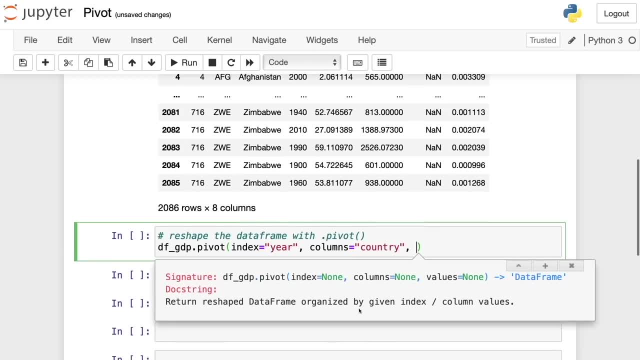 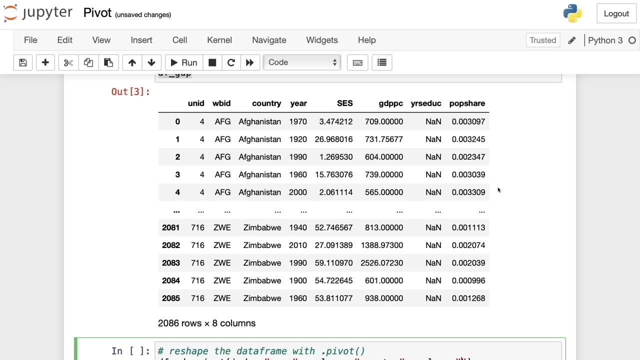 again. Shift plus Tab to show this window here. And now the third argument is values. So here I'm going to write values equal to open quotes And here the only data I want to show here in my new data frame is going to be that GDP. 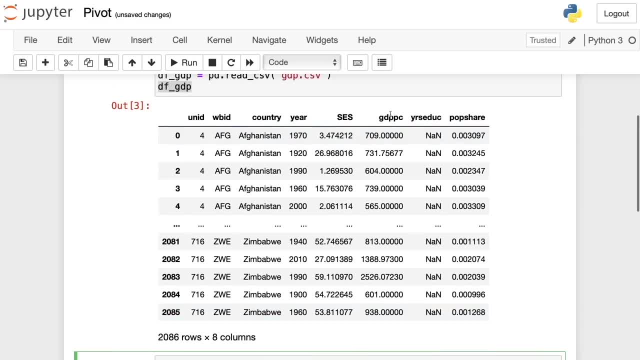 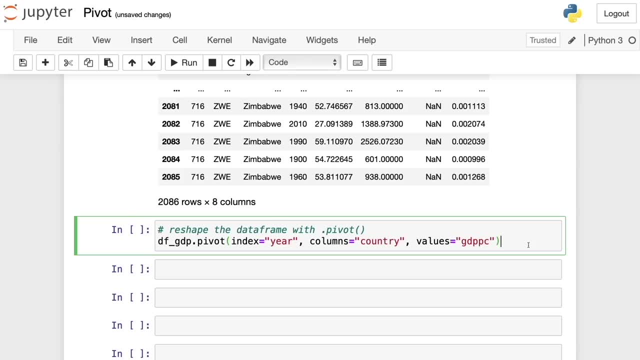 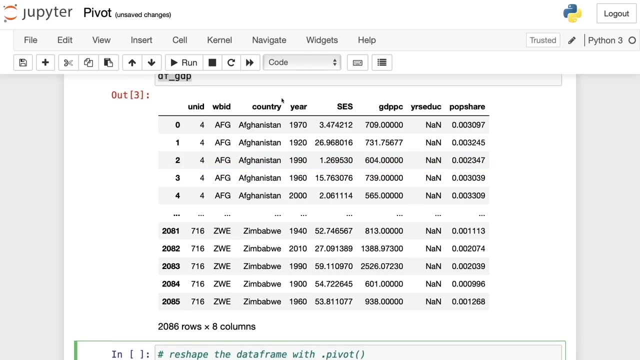 per capita, which is the one that is here And now I'm going to copy this one and paste here. So remember our goal. our goal is to see the evolution of the GDP per capita over the years for all the countries listed here in this column. So here we're going to execute. 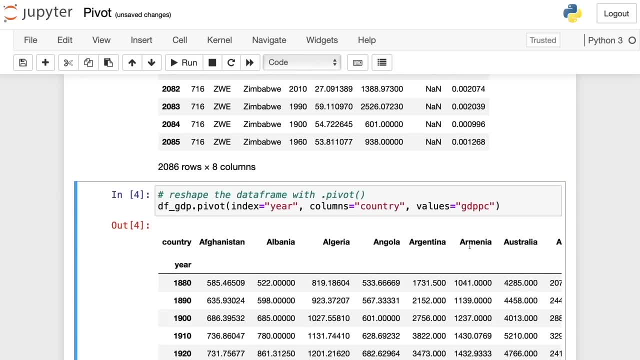 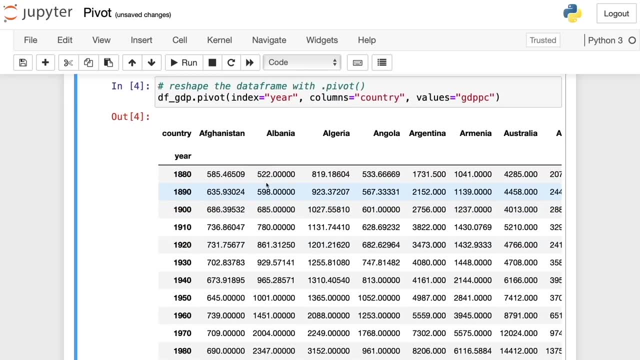 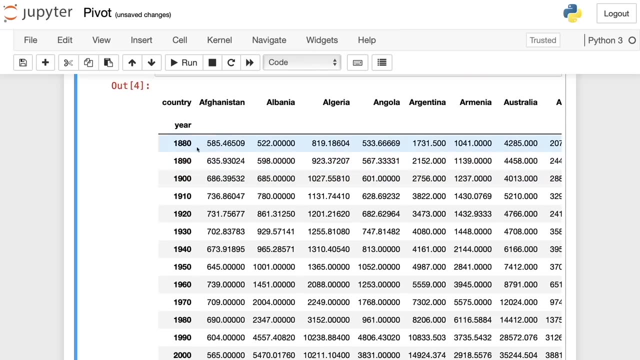 this code And let's see the result. So here, Ctrl Enter And, as you can see, here I have the new view of this data frame And it looks much better. it's more readable because we can see the GDP evolution over the years for each country. So now let's verify, if everything. 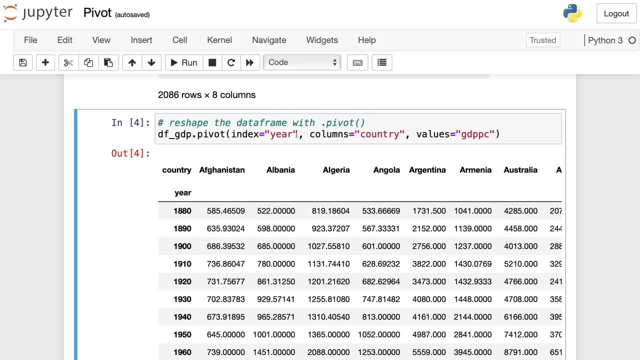 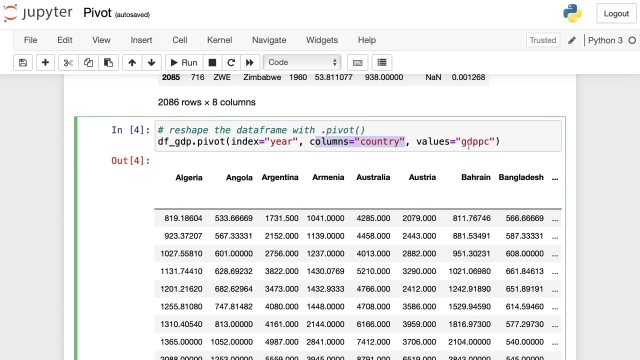 is correct. So here we have the index year And here we have the year as index. So let's say everything's fine. then the columns should be country, And now we have each country in the columns, So it's correct. Next, the values are the GDP per capita. And yeah, we have. 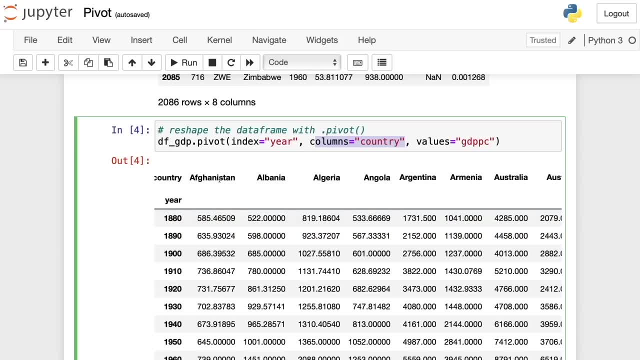 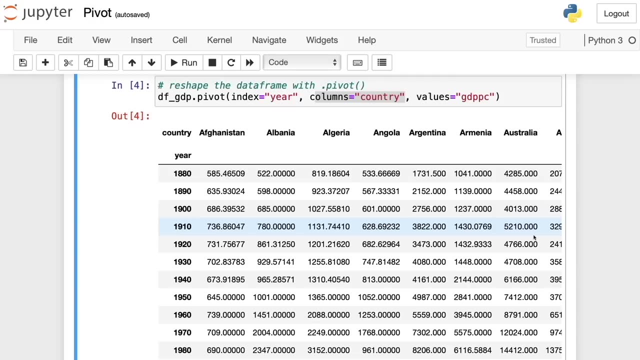 here, the intersection between the row and a column is a value that corresponds to the GDP per capita of that country in that year. So everything is working fine. And there you have it. Let's see how this works in pandas. Okay, now let's see how the pivot underscore table 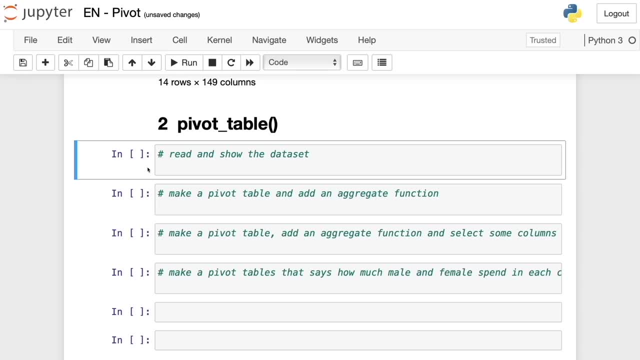 method works in pandas. So in this case we're going to work with a different data set And to read it we're going to use the method PD- read underscore Excel, because in this case the data set is not a CSV file but an Excel file, So we use read underscore Excel. 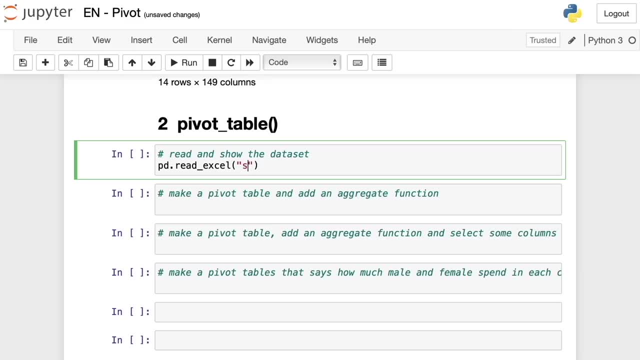 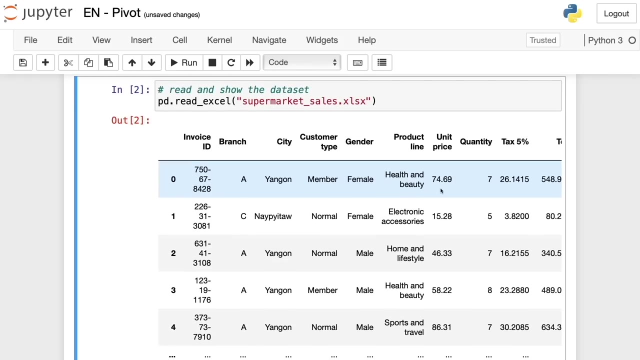 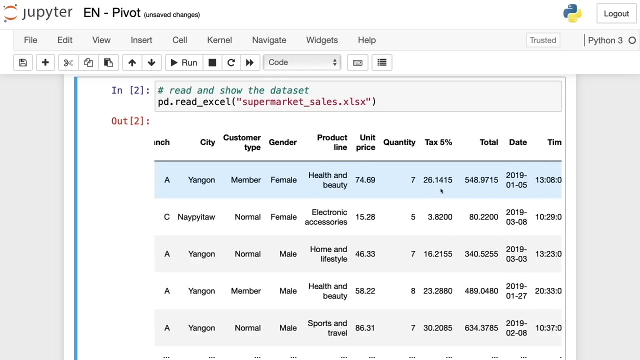 for an Excel file. So in this case, the name of this data set is super market, underscore salesxlsx. And this is what we're going to see after you run this, And here you can see that we have different columns about what specific person bought in a supermarket. And here, well, we have the branch, the CD. 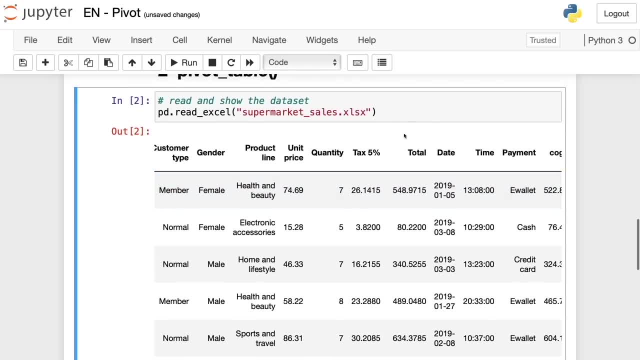 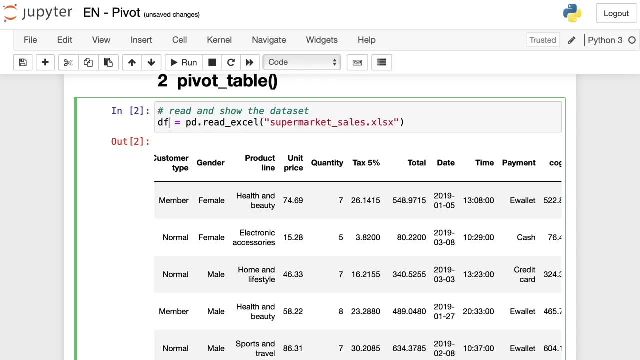 the gender and different data. So here, to make a pivot table, we're going to first name this data frame and I'm going to name it the F underscore, sales, And now I'm going to show it here And okay, now it's. 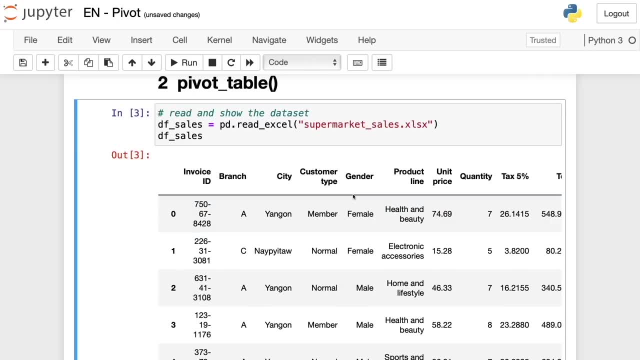 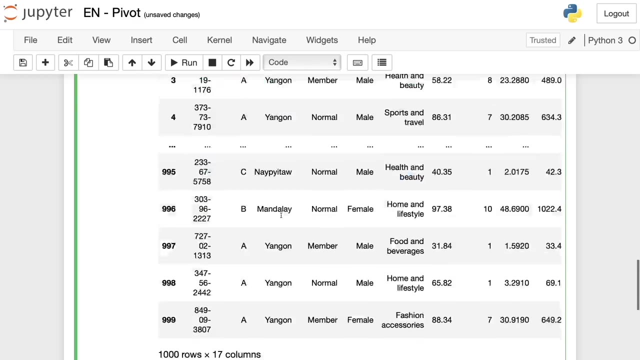 here. Okay, the goal of this task is to see how much female in male is spent their money in this supermarket. So to do that, we're going to use that pivot table method in pandas. So first I'm going to copy this data frame And now I'm going to paste it here And now. 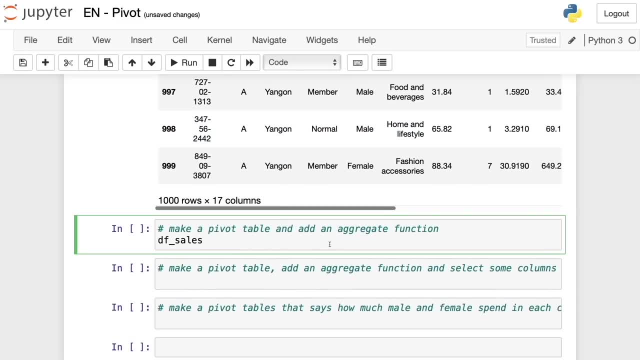 we're going to make a pivot table and add an output function, Because remember that the pivot underscore table method allows us to add an aggregate function and pivot method doesn't support that. So we're gonna use the pivot underscore table this time And now. 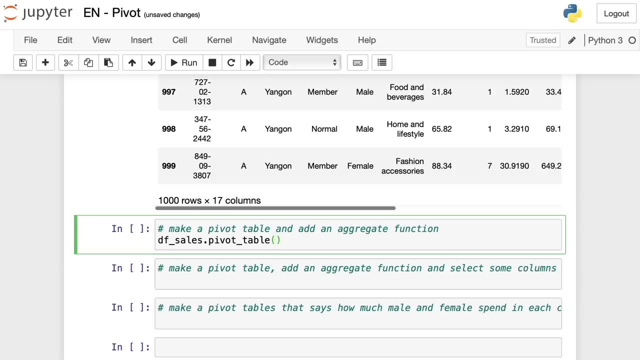 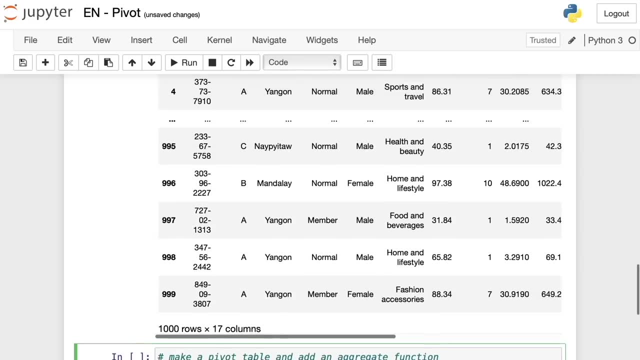 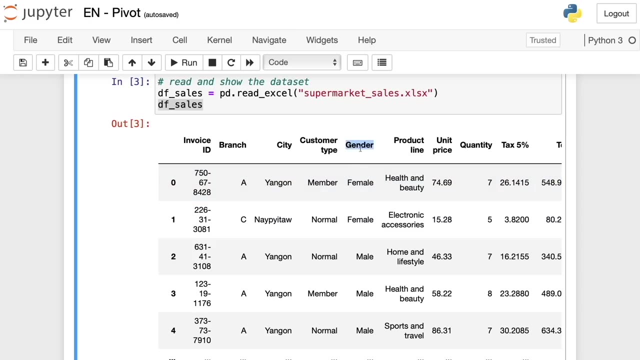 we're going to introduce some important argument. So the first one is that index And in this case, if we want to see how much male and female spend in this supermarket, that index is going to be the gender. So here I'm going to copy gender here, And it's going to be 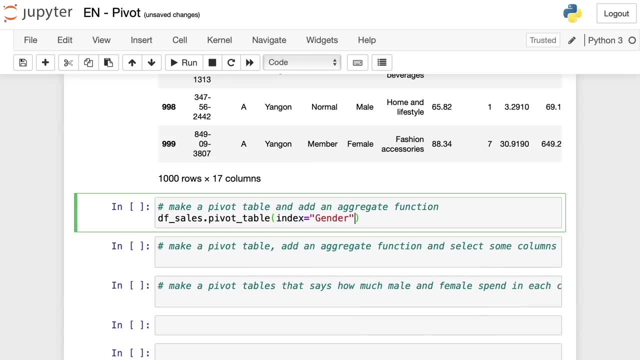 here index equal to gender. So this is the first necessary argument, And the second one is going to be the aggregate function. So we have to write a double G, F, U and C, and then equal to, and then write the aggregate function we want to perform. So in this case is going to be: 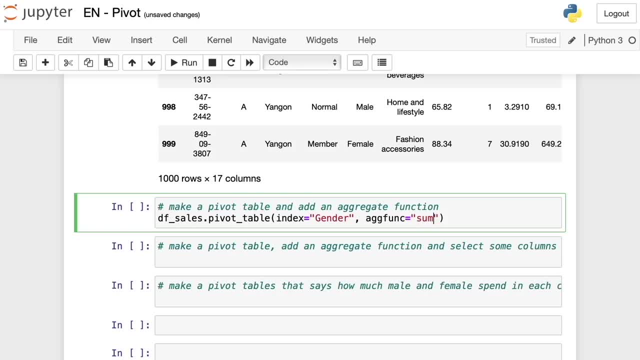 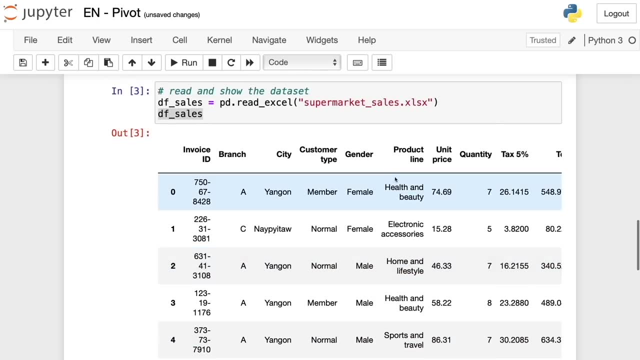 a sum, So we write some and now everything is ready. So what we're supposed to get here is the information about the sales here in this data frame, but now divided by gender, so we have the female category and then the male category. So let's verify this. I'm 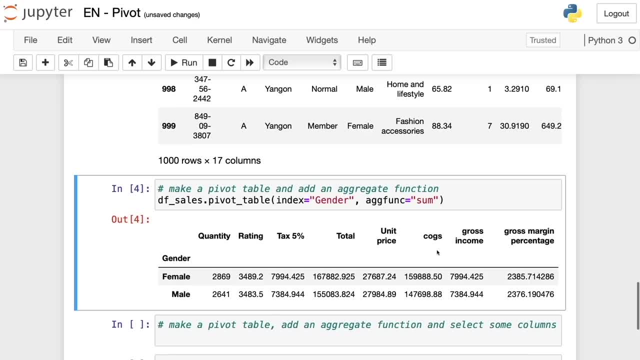 going to run this one And, as you can see, here we have this summary table, or pivot table, and now it's divided by gender, So we can see how much female is spent here in the total column and also how much males spent, also in the total column and here 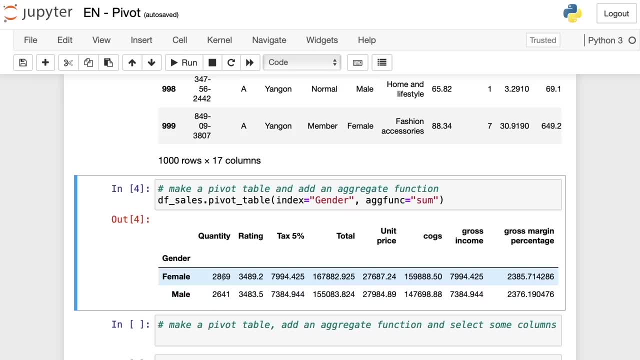 in that quantity column. So if I go to the options then this is the track here. So here you can see that I have see how many products they bought, how many products female and male bought in this supermarket. And one detail you might have noticed is that only the columns that contain numerical data 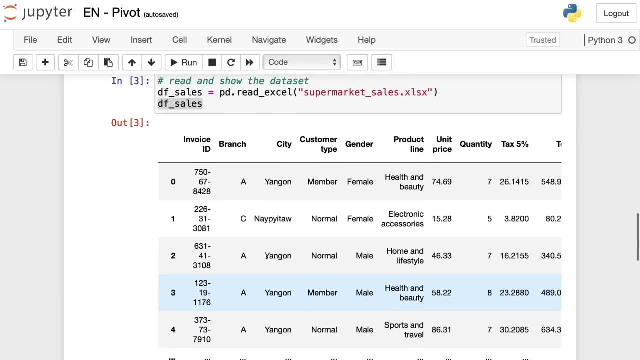 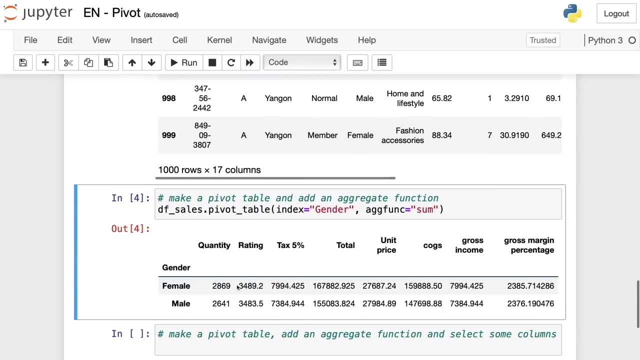 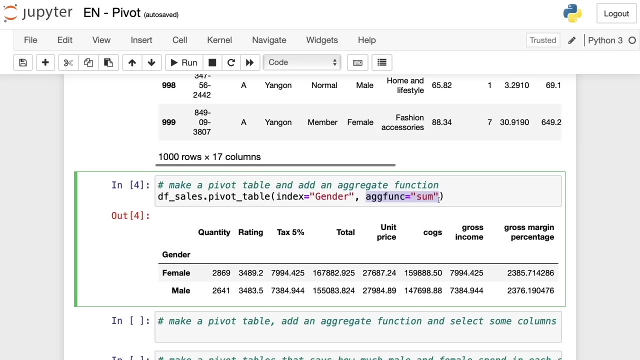 are displayed here. So for example, here branch and city that contain only text aren't here in this pivot table, because here in the argued function argument we indicated that we want to sum, And when we sum values we cannot sum text but only numerical data. 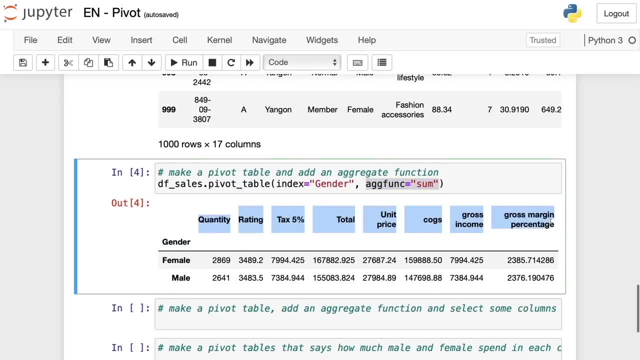 So only the columns that have numerical data are displayed in this new pivot table. Okay, that's our first pivot table And we can do even more. For example, we can select a pair of columns that we're interested in. So let's say we only care. 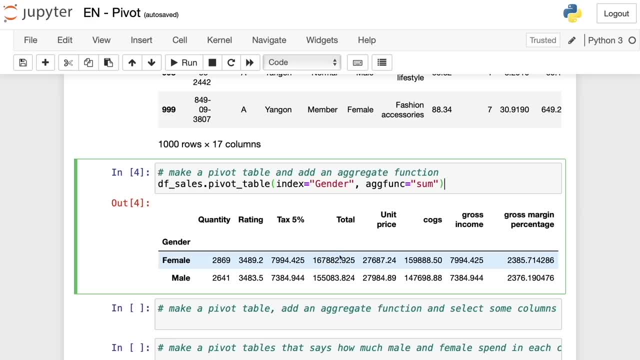 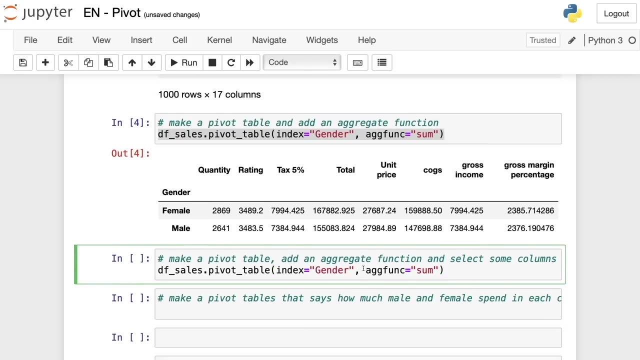 Speaker 2 about the quantity and the total column. So we want only those columns. So we can get that. I'm going to copy this one And to show you how to get only those two columns, I'm going to add a new argument. So here I'm going to write, in this case the name of the. 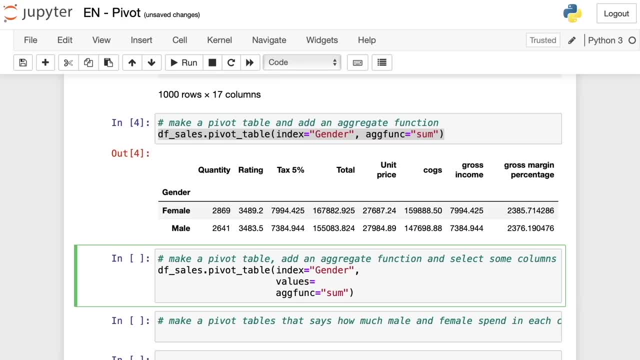 argument is values. So I read values equal to: And in this case I'm going to select the quantity and the total columns. So I open square brackets because I'm going to select two or more columns And inside I write the name of the column. So 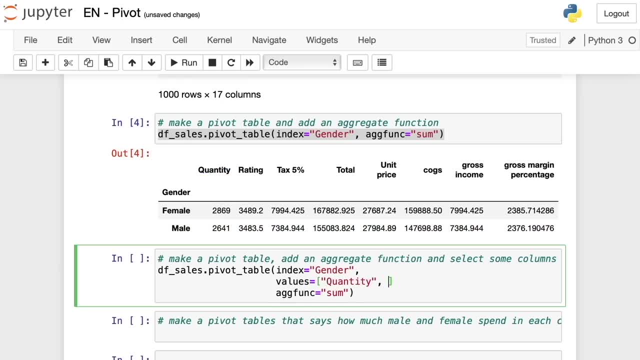 first quantity I write here, and then total, So here too. So we're going to get the same pivot table, But in this case only the quantity and the total columns are going to be shown, shown in this table. So I'm going to execute this one. And here I got an error, because 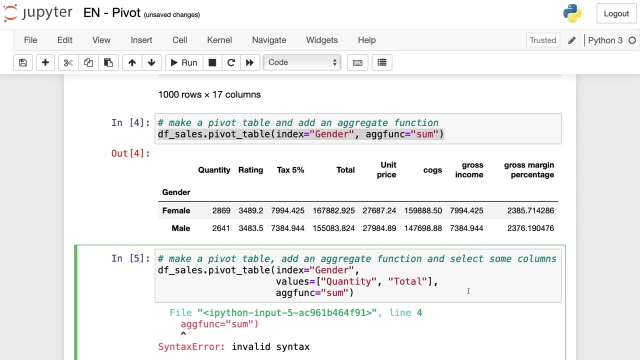 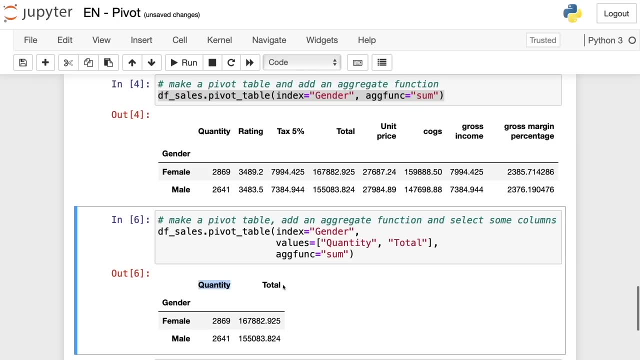 I didn't include this comment, So I'm going to add it here And now. everything should be fine And yeah, we got the same pivot table, but only the quantity and total columns are displayed here, And here we can clearly see that female spend more than male in this supermarket. 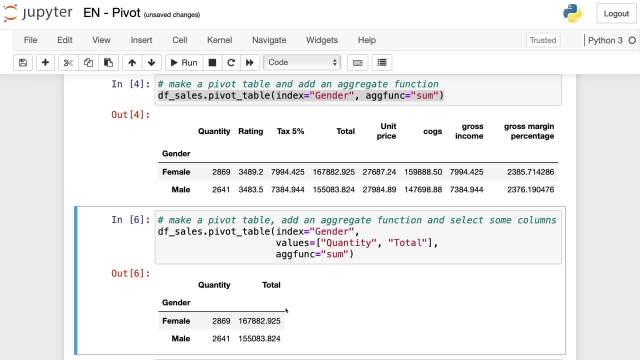 But we can get even more detail here. So far we know that female spend 167,000 in this supermarket. But with pivot tables we can even know in which product lines this money is spent. So let me show you here we can see how the money is spent in this product. 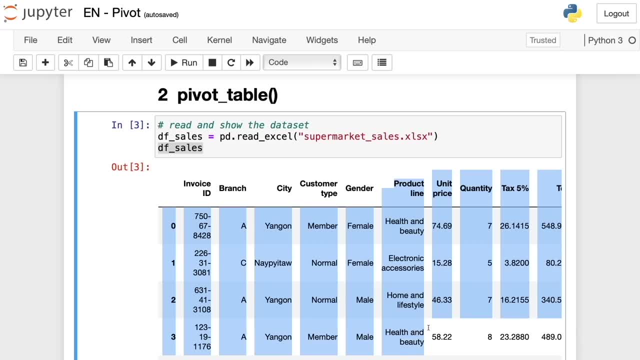 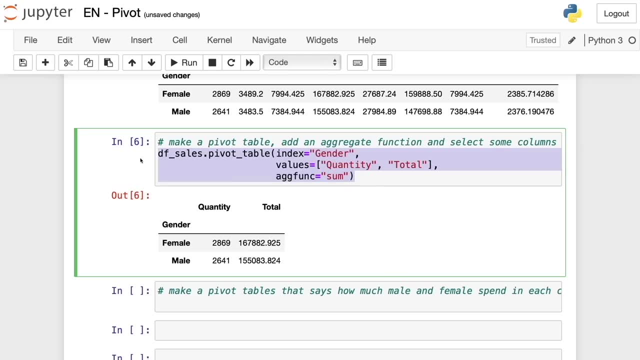 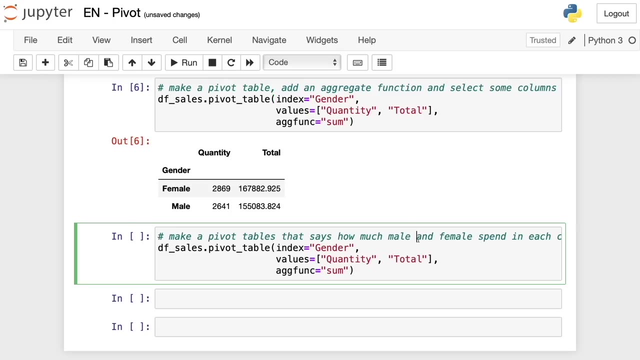 line column. So we only have to add a new argument to this pivot table method. Let's see, So I'm going to show you here. First we copy this And now I'm going to paste it here, And we're going to make a pivot table that says how much male and female is spent in. 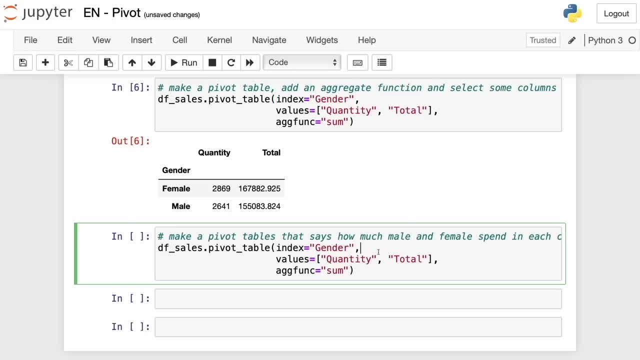 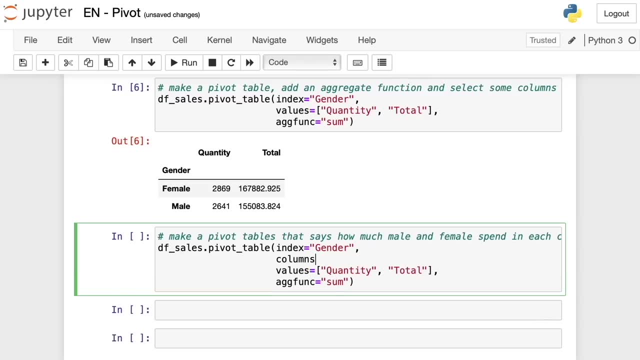 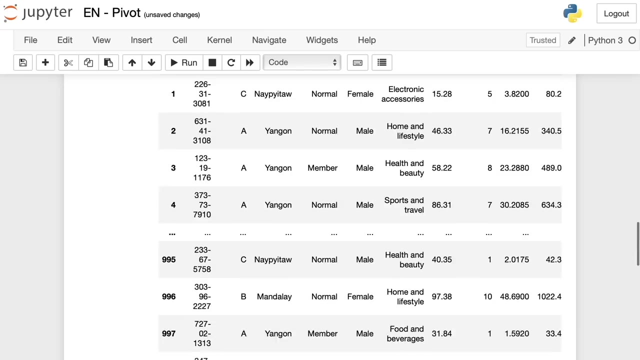 each category, or well, product line. So we add a new argument And this one is going to be that columns argument. So I write columns, then open quotes. I add the comma In here, I write the name of this column, that is, product line. So I scroll up, I copy this column: 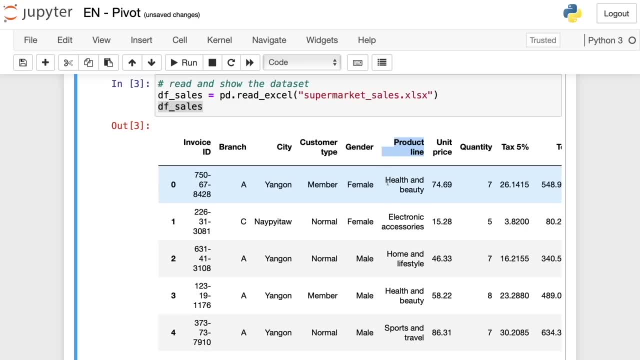 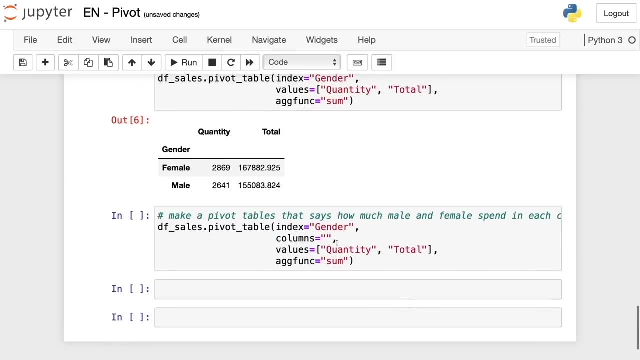 And then we're going to see in which category is to spend the money, So health and beauty, or sports and so on. So now I scroll down in here, I paste it, And before I run this code here, we only want to display the total, because we only want to see where the money 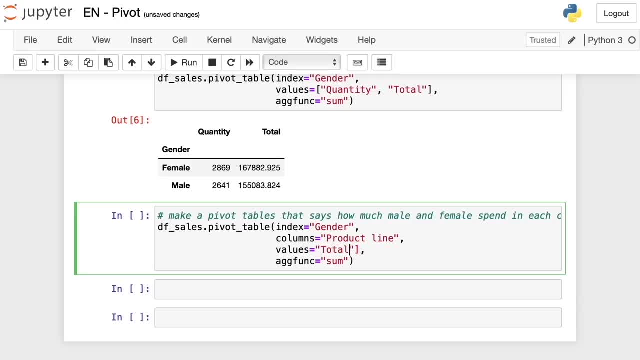 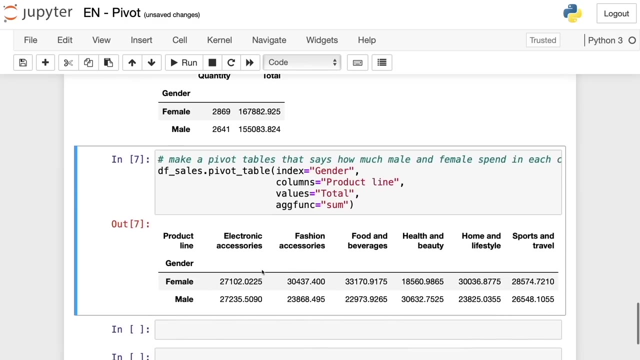 goes, not the quantity, So only total. so I delete the square brackets too, And with total we're going to see where the money goes, divided by gender. So here I run because it's ready And now, as you can see, here we can see how much female in male spent in each product line. So we can 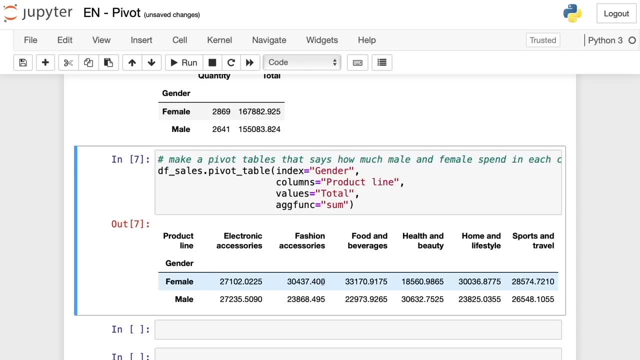 quickly see, for example, that female is spent more money on fashion accessories than male in that kind of way- Yeah, makes sense. And also in sports, women spend, or female spend, more money than male. So we could easily see all of that by using the pivot underscore table method in pandas. 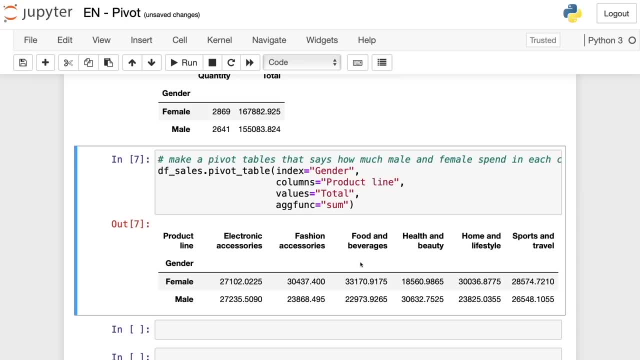 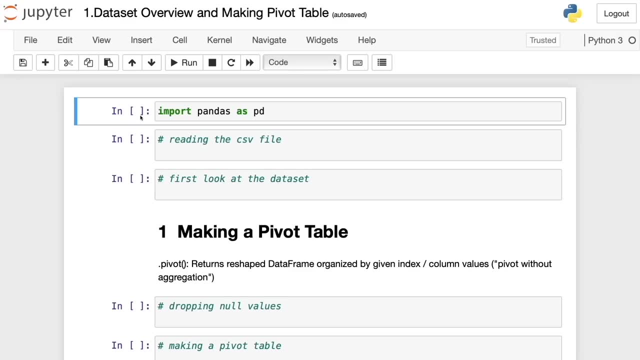 And this is similar to the pivot table you will find in Excel. And that's it. That's how you make a pivot table in pandas. All right, before showing you how to make visualizations with pandas, First we have to check the data set And also we have to make a pivot table, So we 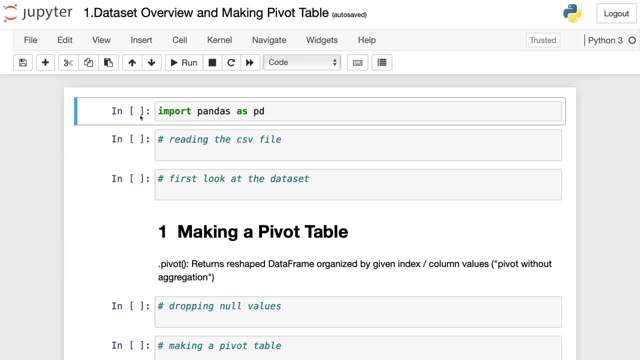 can easily make the plots with pandas later. So first we have to import pandas to read this CSV file. And well, I have this, import pandas as PD, So we just run this code. And now let's read this new data set. So, as you might remember, to read a CSV file, we have 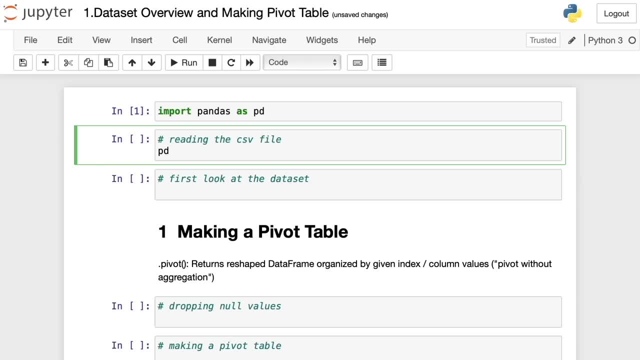 to use that read underscore CSV method. So we write PD that read underscore CSV And then we write the name of the CSV file. So in this case the name is population And I'm going to use this population underscore total that CSV. So I pressed Tab to get this the name. So we 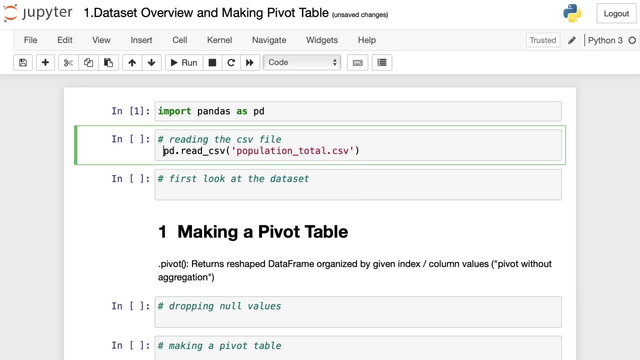 have now the name And now I'm going to sign this to a new variable. So the variable is going to be DF, underscore population, underscore row. So this row data, and now we're going to have a first look at this data set. So 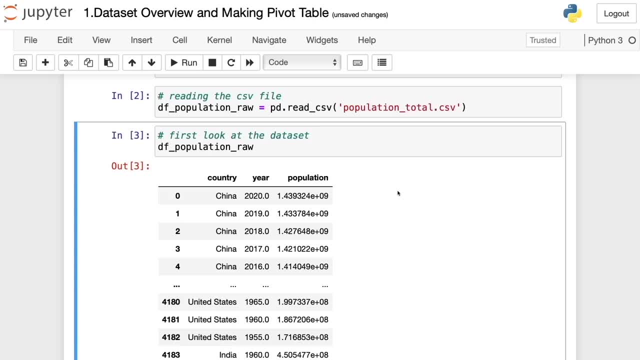 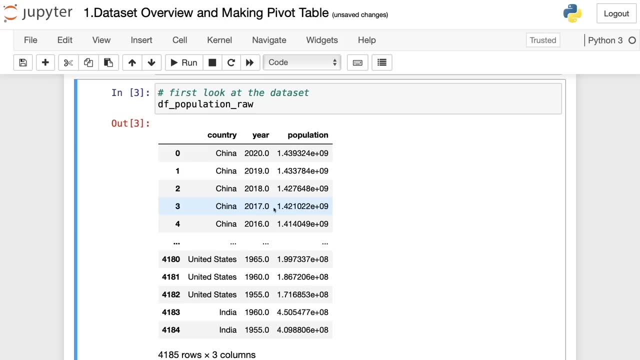 I paste this And now I'm going to run this too, And now we have this data frame. So here, as you can see, we have that population Of many countries throughout the years. So, for example, we have China here, United States, 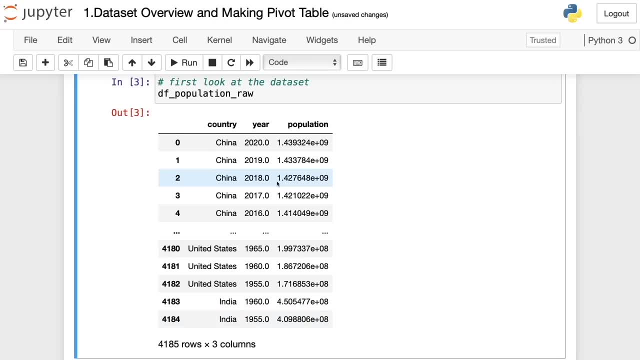 and India. So we have the population. And here I wrote the name row, because this data set was extracted using some web scraping techniques and then it wasn't modified. So now we have to make some changes to reshape this data frame. So we make it easy for us. 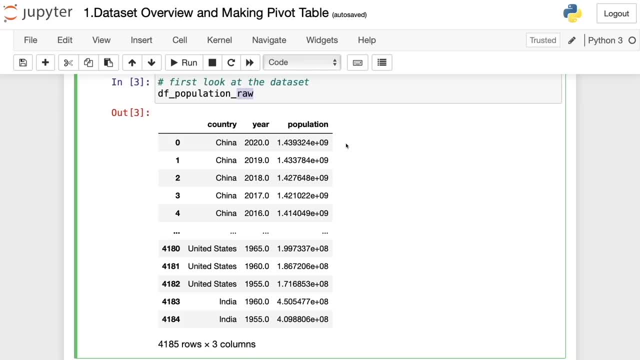 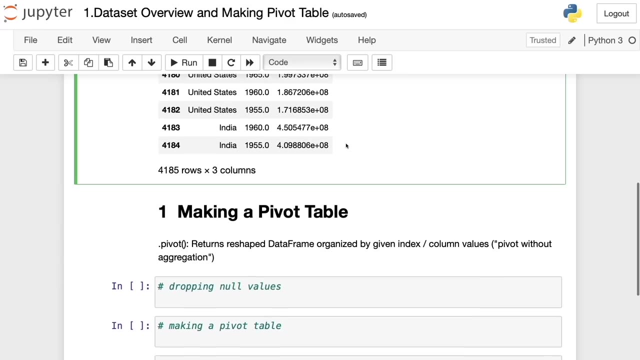 to make visualizations With pandas later. So what we have to do here is to make a pivot table to reshape this data frame, And that's what we're going to do here below. So we're going to make a pivot table And we're going to use that pivot method. So, as you might remember, the pivot method. 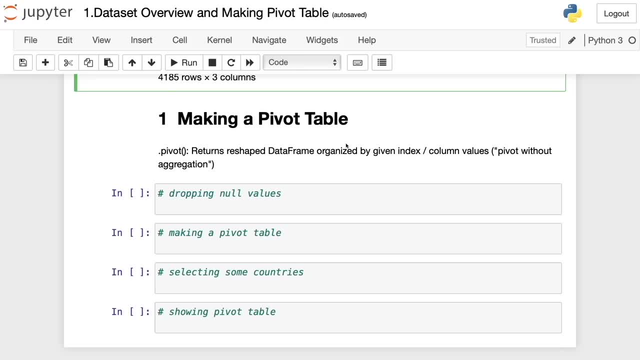 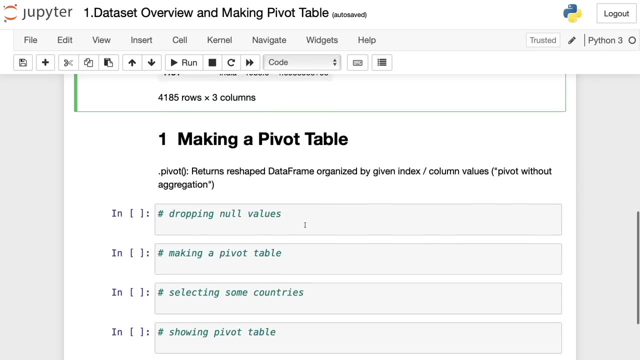 returns a reshape data frame organized by given index column values, But it's a pivot without aggregation. So this is what we want. So we only want to reshape this data frame. So we're going to start by dropping null values. So we do that by writing the name of the data frame And 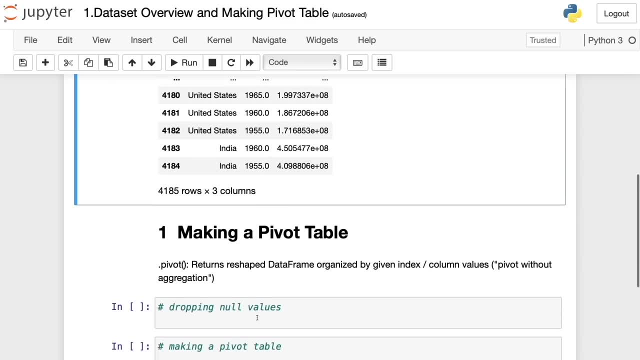 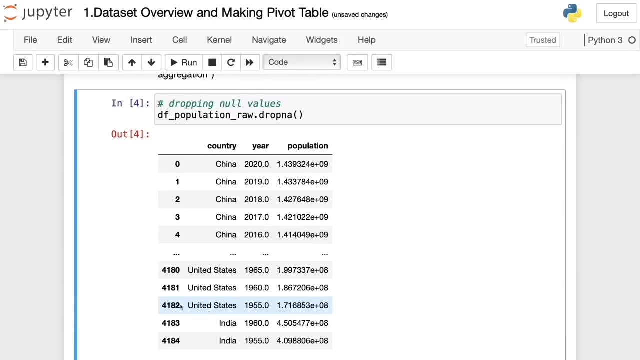 now I'm going to just copy the name and I paste it here And now. to drop null values we have to use the drop in a method. So I write drop in a, and then we have to run this And, as you can see here, we have the result and it's a copy from this data frame. But 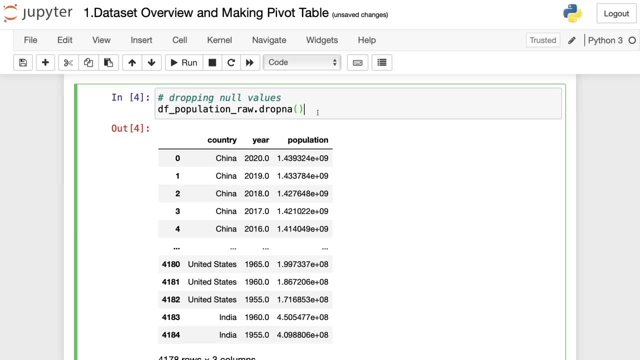 if we want to save the changes that we make to the data frame, we have two options. The first option is to use the in place argument. So I write in place and then set this to true. So if we do this and we run, all the changes that we make to the data frame are going to. 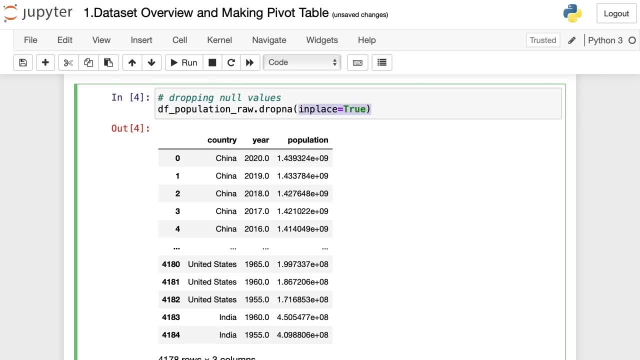 be saved. And the second option is to do something like this to overwrite the content inside this data frame. So we do something like this: we write the F underscore- population underscore row is equal to the same data frame, but that drop in a. so we're overwriting the content inside this data frame. So I'm gonna. 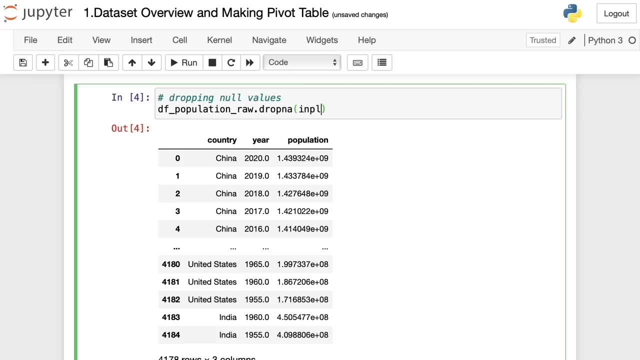 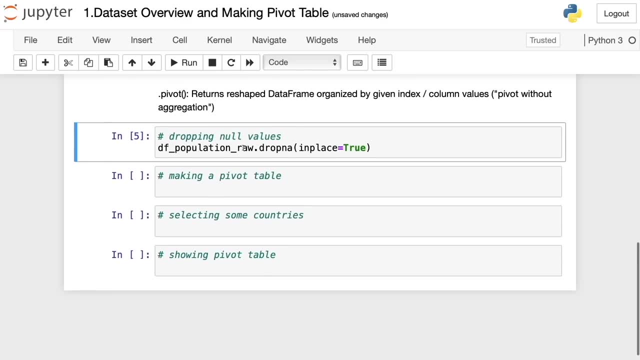 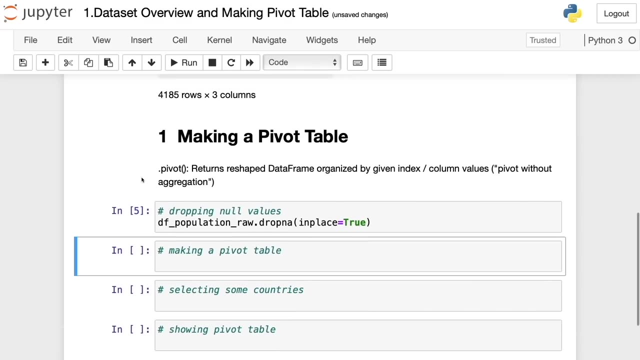 choose the first option. just to reduce some code. So I write in place equal to true in our run And this new data frame shouldn't have any new values. Okay, now it's time to make this pivot table. So first I'm going to show you what I'm going to do So we have a better 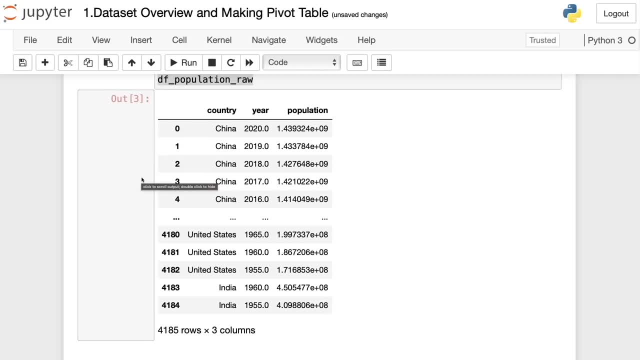 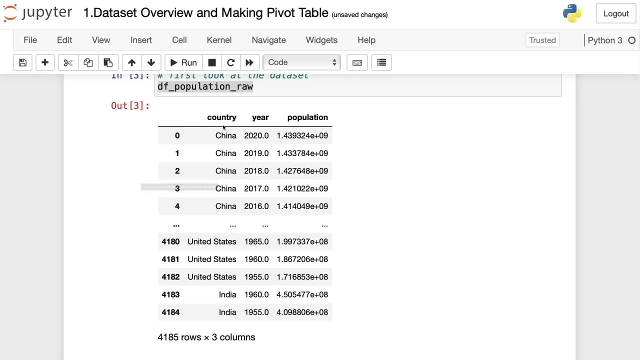 idea before writing the code. So here we have the original data frame And what we're going to do is to reshape this data frame. So I want that year to be in that index, so that your column, I want it to be here in the index instead of 01, and so on. And then I want that country. 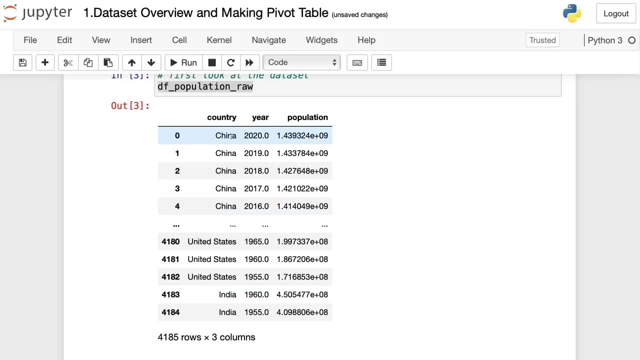 column, or the country, the values inside the country column. I want it to be here in the columns. So, for example, I want China here in one column, then United States in another column and then India in another column, And I want the population data Inside the 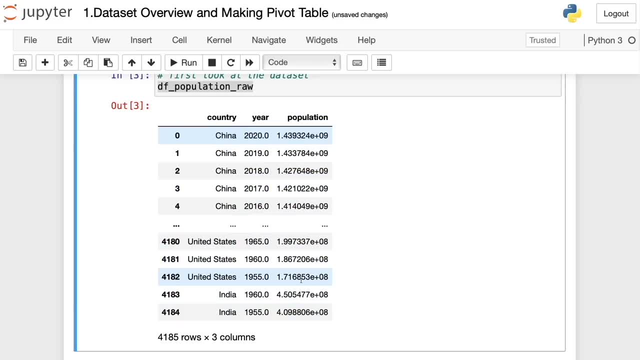 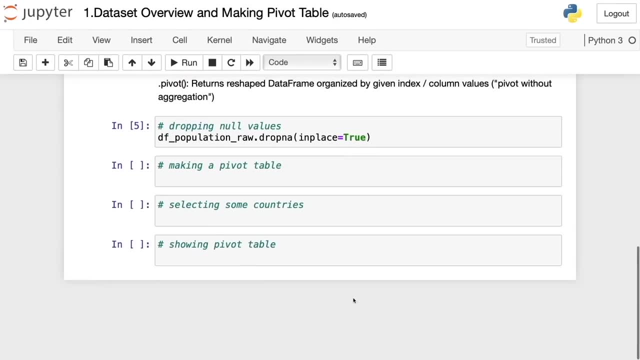 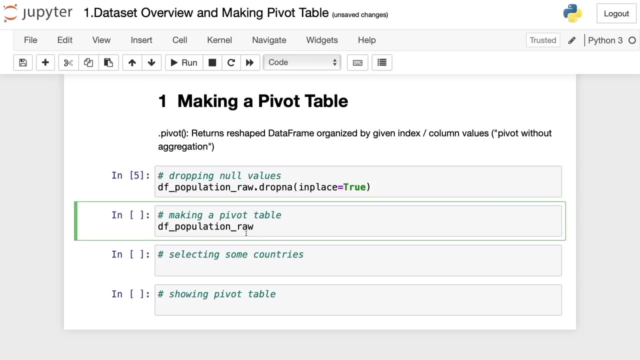 data. I want it to be the only data here. So to do that we have to use the pivot method, And that's what we're going to do here below, So let's do it here. So first we have to write the name of the data frame, which is this one, and then write that pivot. then 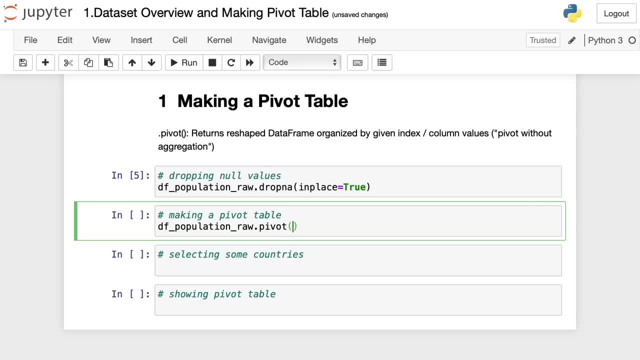 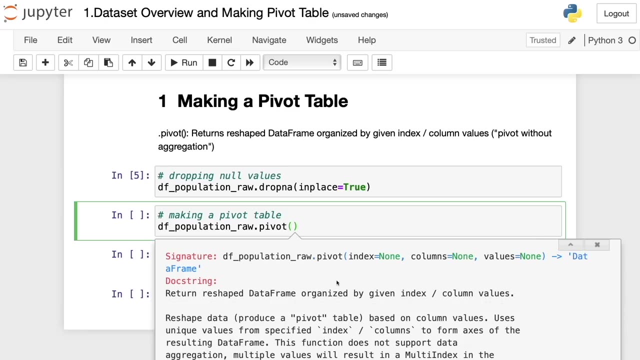 we open parentheses In here. let's see the arguments that this pivot method accepts. So I press Shift and Tab. to get this help Helpful, let's call it cheat sheet. And now we have the arguments that this pivot method accepts. So first is the index, then the column and then the values. So, as I told you before, 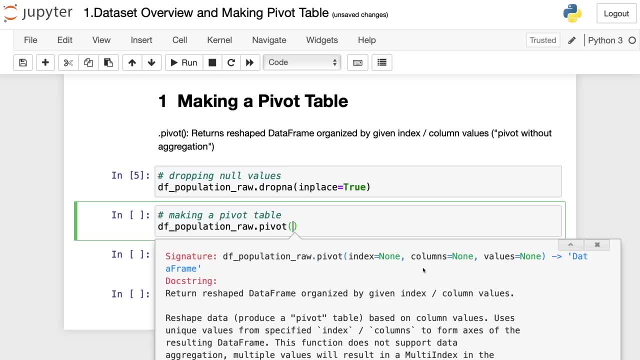 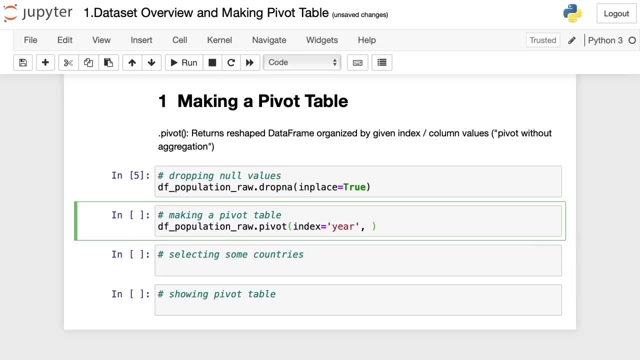 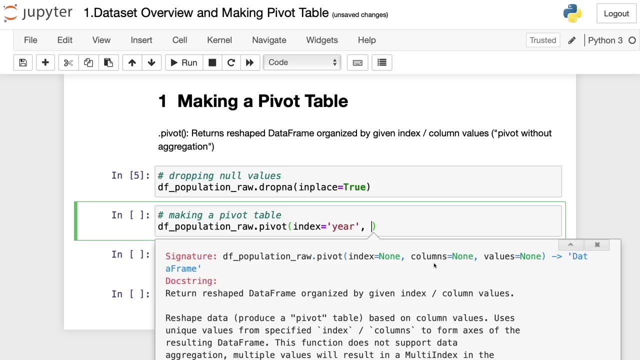 the index. I want it to be the year column, So we have to write index equal to open quotes and I write here, then coma, And let's check another argument. So the next argument is the columns. So I want the columns to be the country, So the data inside the country, columns. 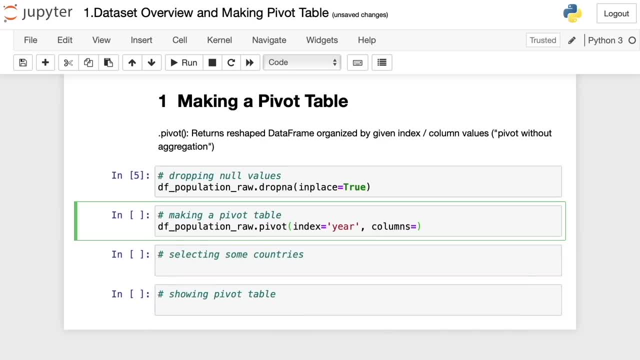 So here I write columns, then I open quotes in here I write country, so country, And now the last one I think is values. And yeah, it's values. So I want the values to be the population data. So let me see if that's correct. And yeah, it's here. 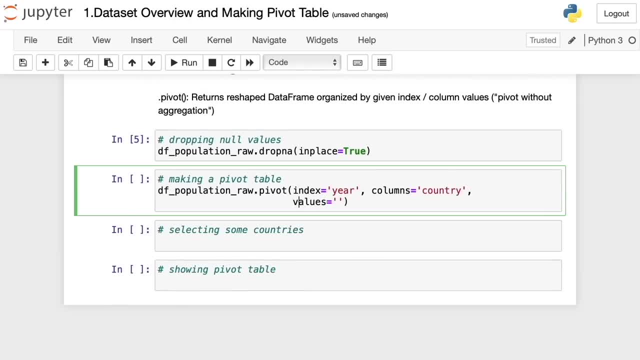 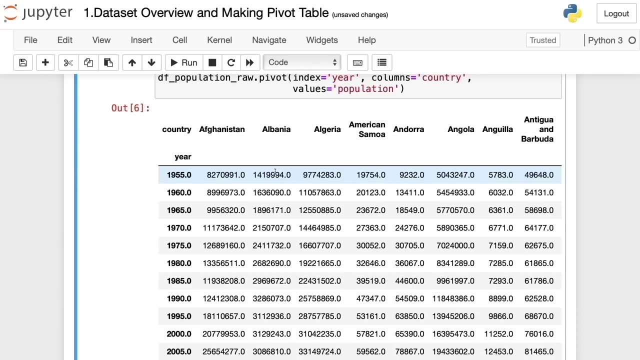 So population, and I'm going to press Enter here So it looks much better. And now population is here. So I have the three arguments that index the columns and the values, And now I'm going to reshape my original data frame. So here I press Ctrl Enter Now, as you can see, here we have the countries. 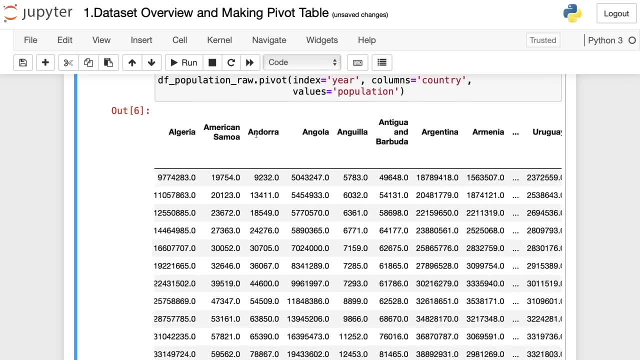 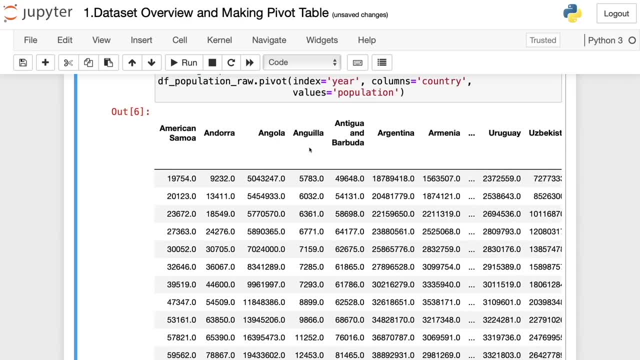 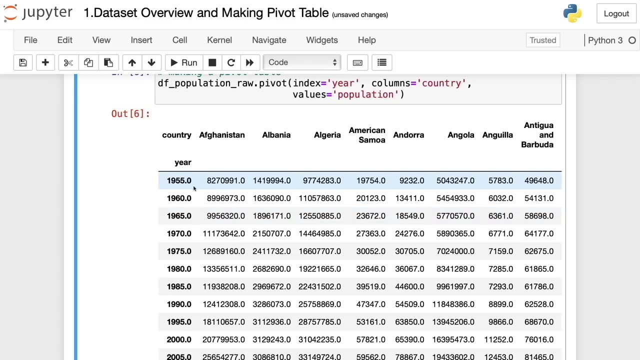 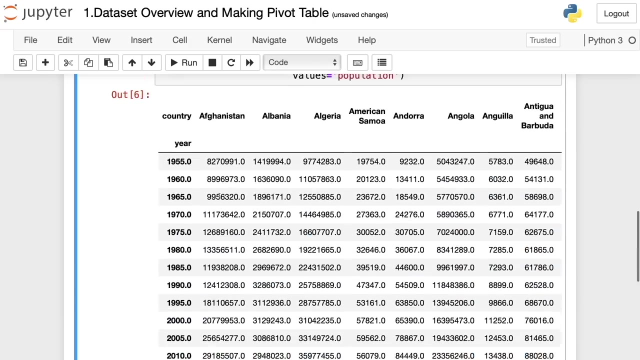 in the columns. So here we have many countries. It's from the first country, Afghanistan, to Andorra, Argentina, ur way, and many other countries. So we have also that year. so it's here that you're from 19, 55, to 2020.. So we can see here the evolution of the population throughout. 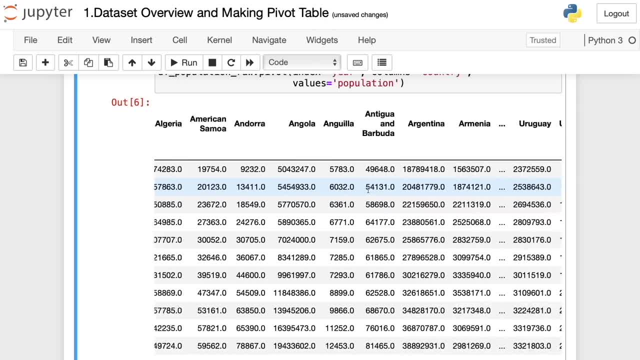 the years for all the countries in this data set. But, as you can see, there are many countries, So what we can do here is to select these three subtle column values And I'm going to switch it to yellow And I'm going to choose this redYellow, any of these tables. And here 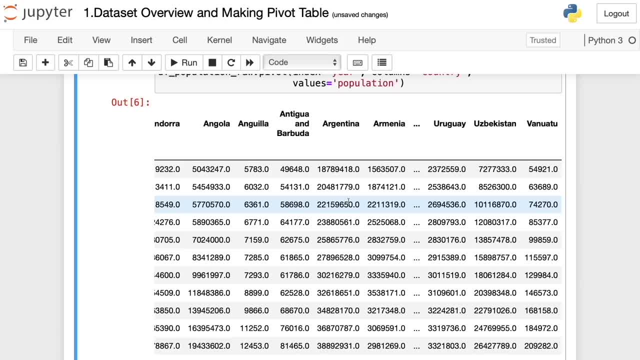 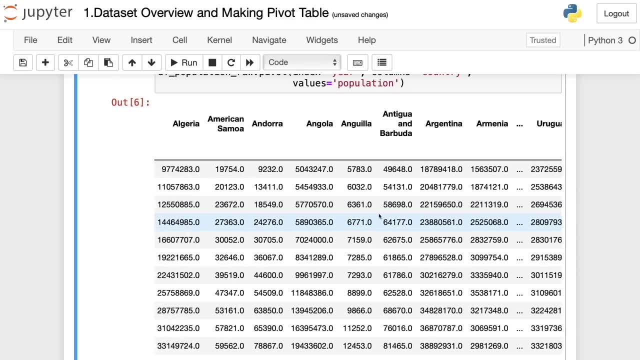 we can choose to select two different Movies, alternating values And people are going to just some countries, So we can simplify our visualizations later in pandas. So here I'm going to select some columns, But first I'm going to name this new data frame. I'm going to 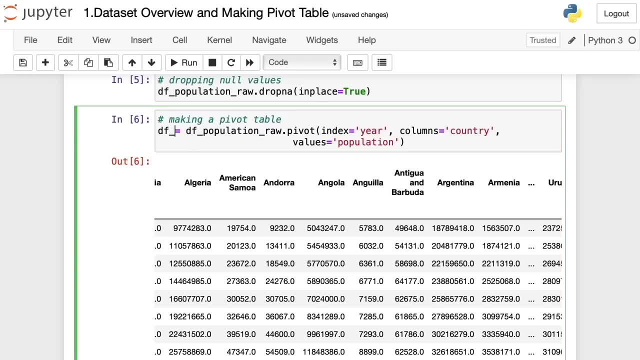 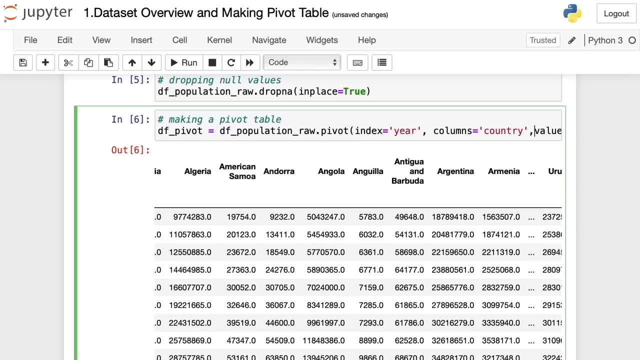 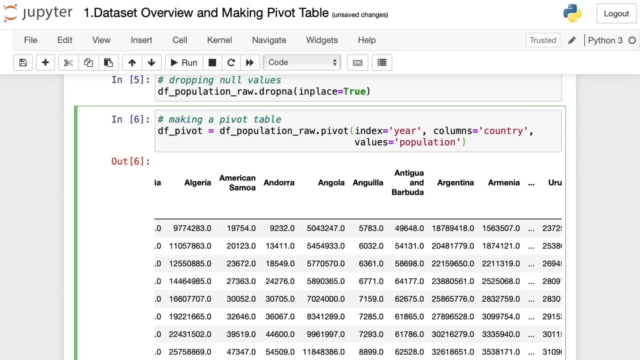 give it a name, So I'm going to name it the F underscore pivot. So this is my new data frame. Now I'm going to rearrange this, And now it looks much better. So now I'm going to run this, And now. 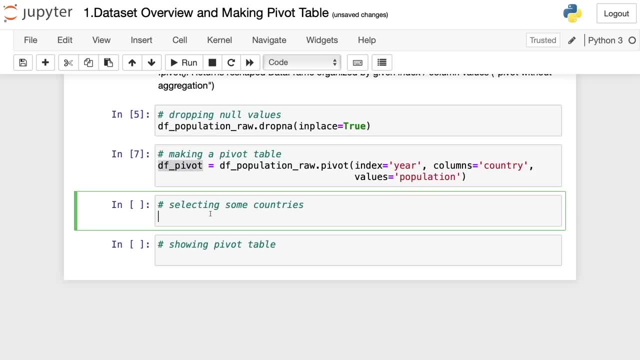 let's select some countries. So I copy this pivot data frame. you know, we open square brackets, double square brackets, to select two or more columns, And here let's write some countries. So first United States, then let's say India. 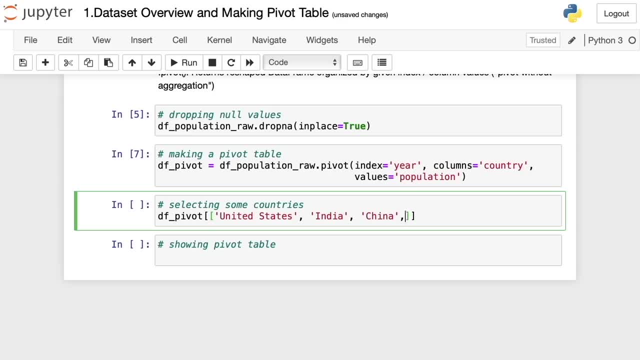 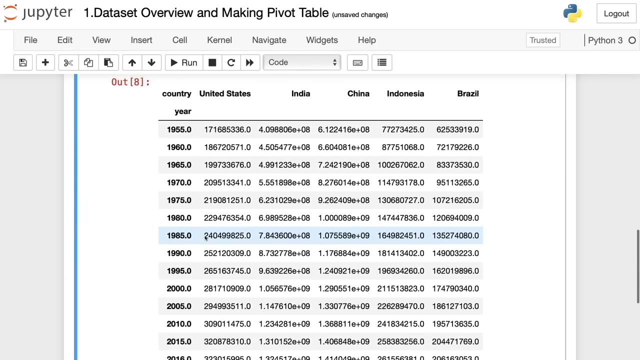 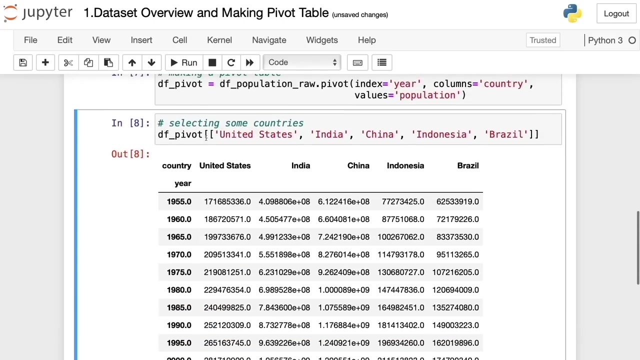 then China, to more countries, Indonesia And, last but not least, Brazil. So here we have the five countries. So I ran here and we have these five countries and population from 1955 to 2020.. So great. Now we simplify this data frame And now I'm going to overwrite the 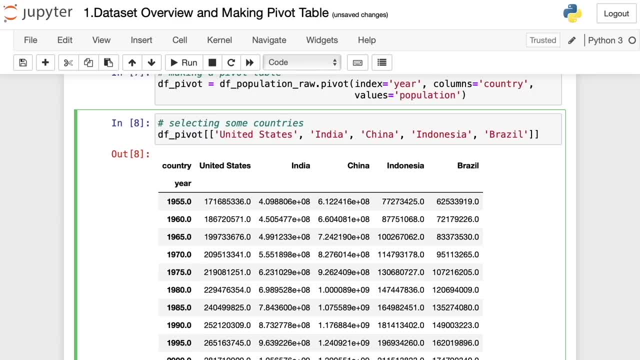 controlいきます. This is our in base code. So let's define this��elteamb harm in one county and to baixar this, So that unfair one. so let's define three in base planners. remember content inside the data frame: DF underscore pivot, And I'm going to write here the F pivot. 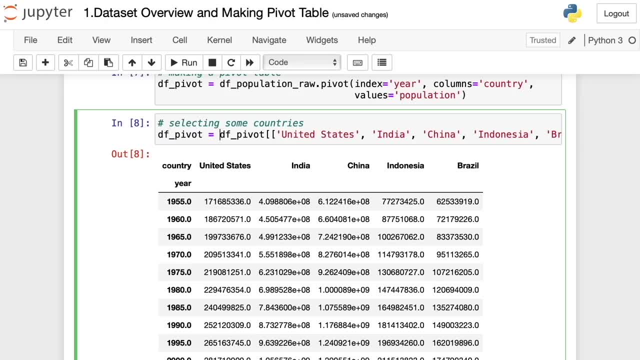 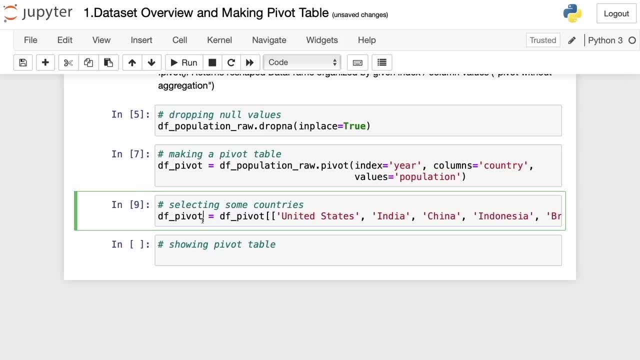 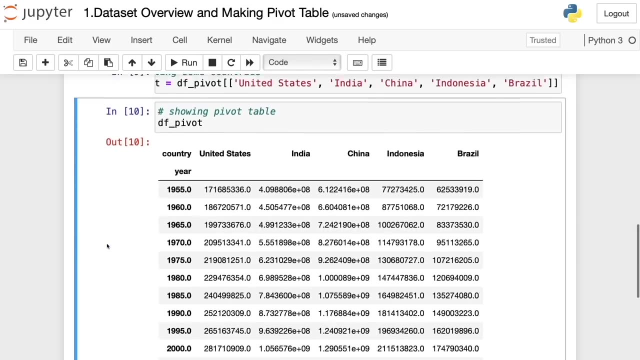 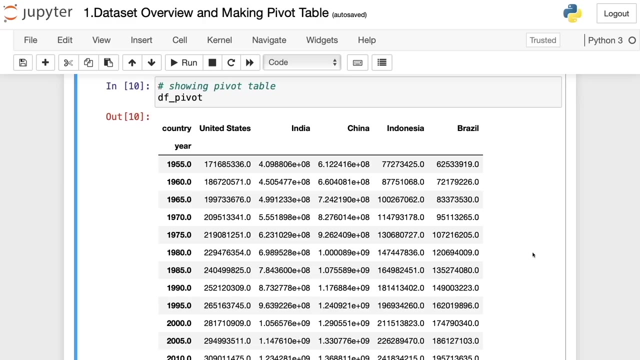 equal to the F pivot And with this selection, so I'm overwriting the content, So I press Ctrl Enter And our new DF underscore pivot is here. So we have it here And now I'm going to show it to you, And this is our new DF underscore pivot data frame, And that's it. Now our data is ready. 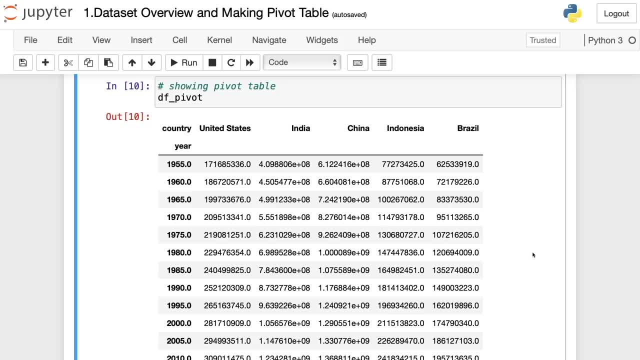 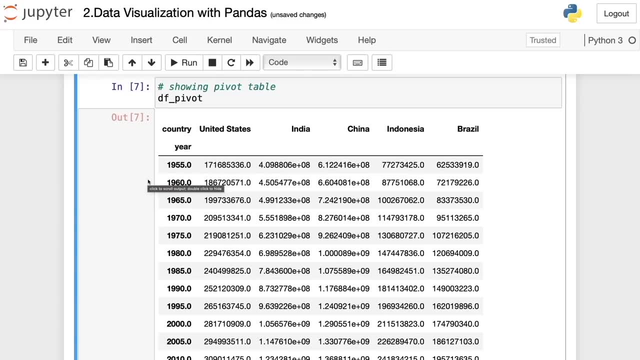 So we can use it to make very visualizations with pandas, And that's what we're gonna do in the next video. Okay, now it's time to make some visualizations with pandas. In here I have the data frame that we created. This is the pivot table we created in the previous video And, as you can see, here we have the pivot table that we created in the previous video And, as you can see, here we have the pivot table that we created in the previous video. And, as you can see, here we have the pivot table that we created in the previous video And, as you can see, here we have. 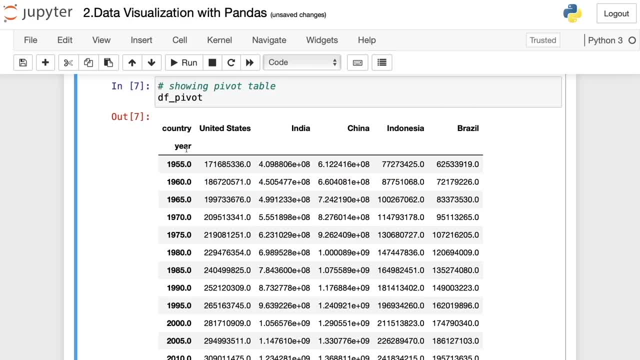 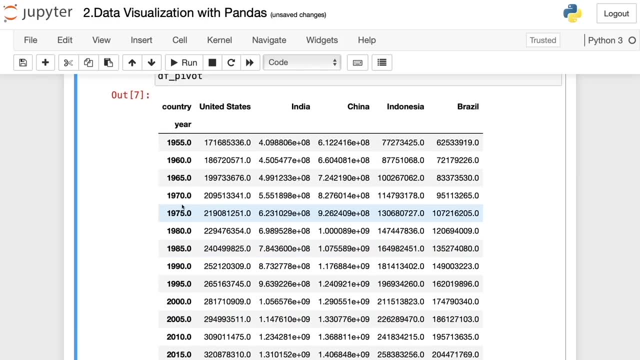 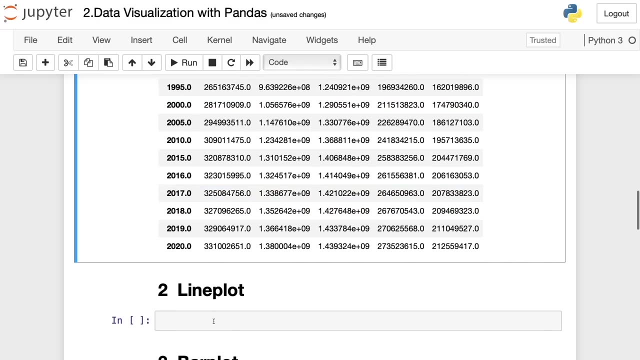 five countries in the columns And here we have the year in the index, from 1855 to 2020.. So what we're going to do now is to make our first visualization. So I scroll down here, And the first one is going to be line plots. So here, first to make this visualization, I'm going to 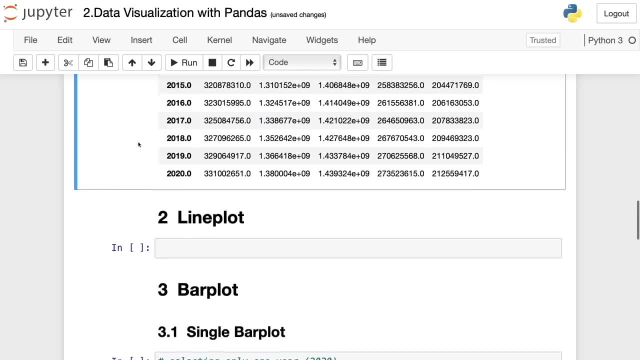 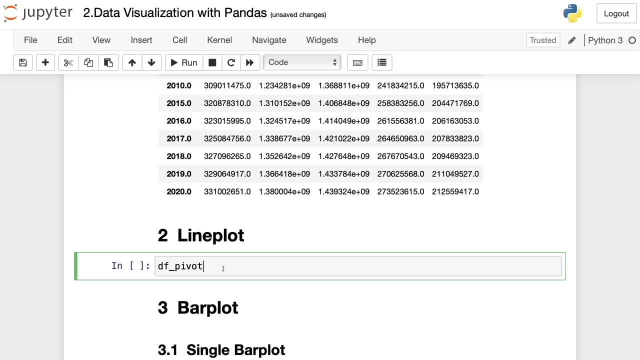 copy the name of the data frame And I paste it here. So now to make plots with pandas we have to use the plot method. So we write that plot Now I open parentheses And one necessary argument we need to introduce is the kind argument. So I write kind now equal to, and here I have to write a kind. 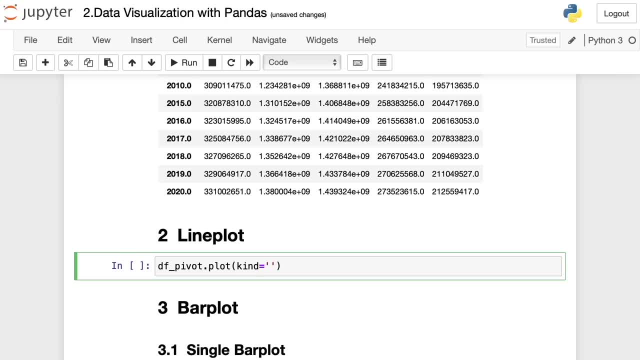 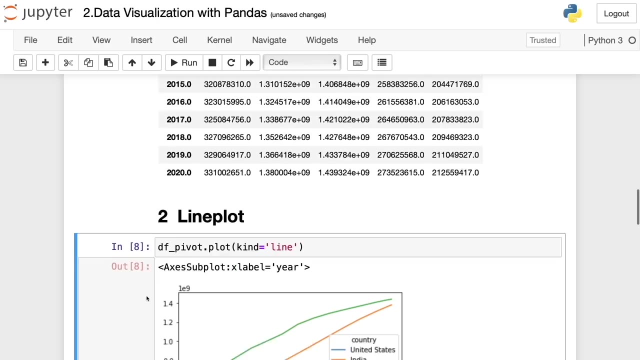 of plot we want to make. So in this case is a line plot, So we write line And this is actually the mandatory argument to make. So now we're going to merge into a plot and we're going to modify the we have to introduce here, And now we can run this code. So I press Ctrl Enter And, as you can see, 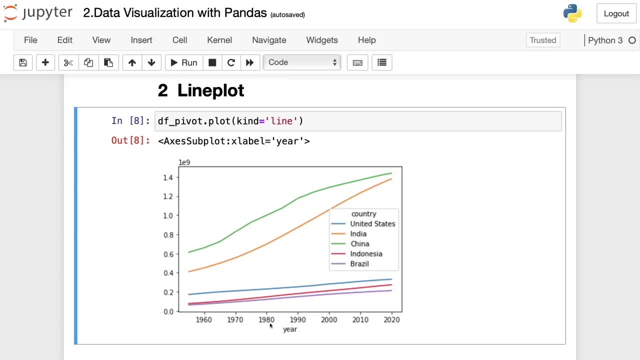 here I have the line plot. So in this line plot we can quickly see the evolution of the population throughout the years. For example, China and India, which are green and orange lines, they had some fast growing population, while United States, Indonesia and Brazil, they have a. 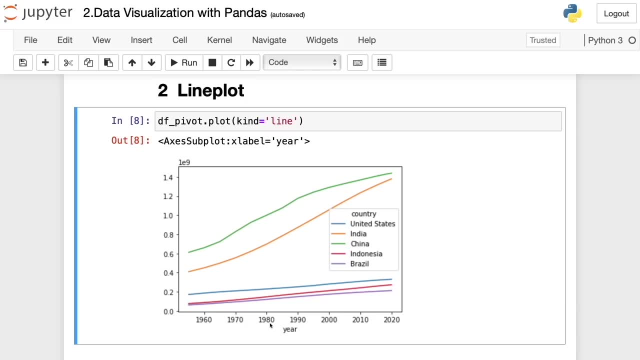 lower population being also the population didn't change so much in the past 50 years. Here we can add more arguments to this plot method to customize this line plot. So here we can introduce another argument, which is the x label. And this x label is: 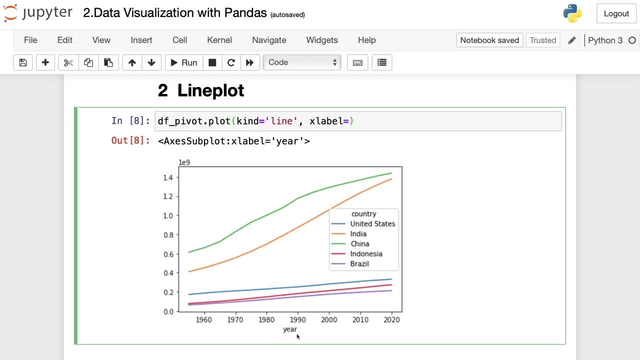 what you can see here here. when we created this line plot, by default it was assigned this year label, but we can change it. So, for example, let's say we have, we want to write year, but now with capital letter. so we write year here. And now let's say we want. 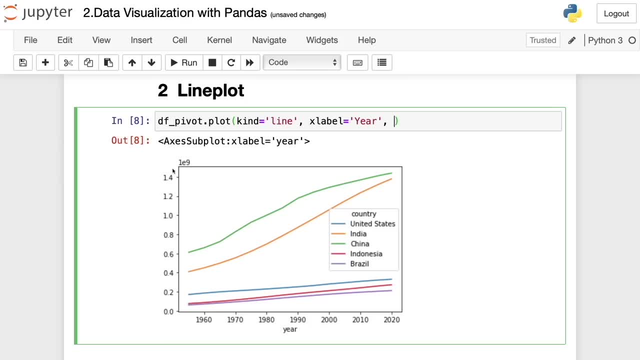 to add a new label here in the y axis. So here we have only to write y label and then equal to open quotes, And here we have to write the name we want. So in this case I'm going to write only population And finally we can also add a title. So we can add any. 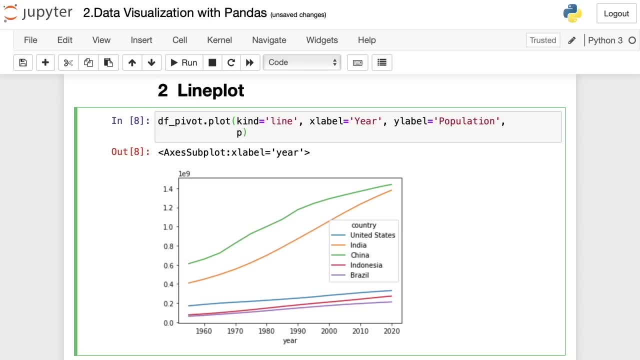 title we want. In this case, I'm going to write a. well, the name of the argument first, title, then equal to, and then the name of the title is going to be, let's say, population from 1955, and to 2020.. So this is the title. So 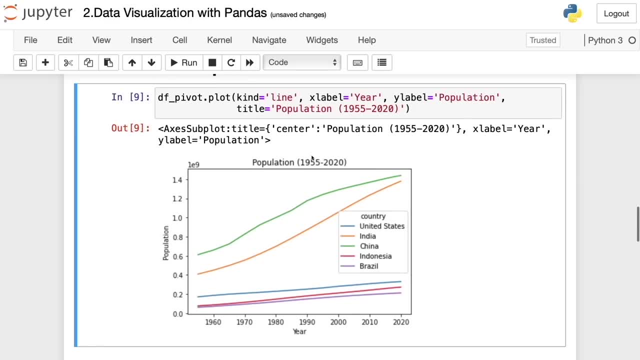 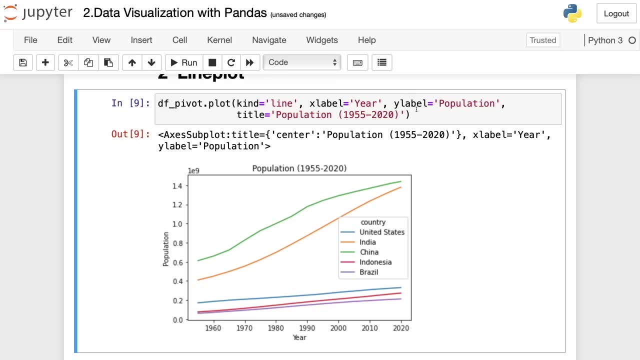 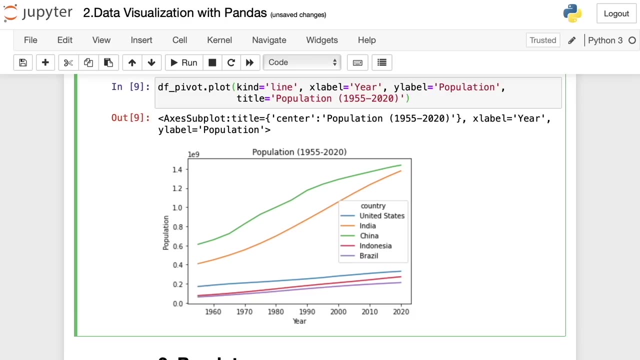 let's run this And now, as you can see here, we got the title population 1955 to 2020.. And the X label and Y label were modified to last. Finally, we can add one more argument. in this case, the argument is the size of. 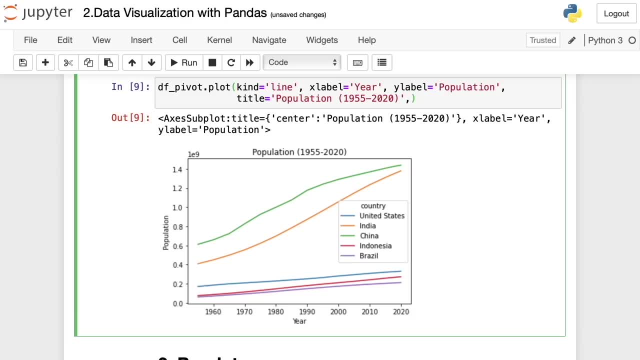 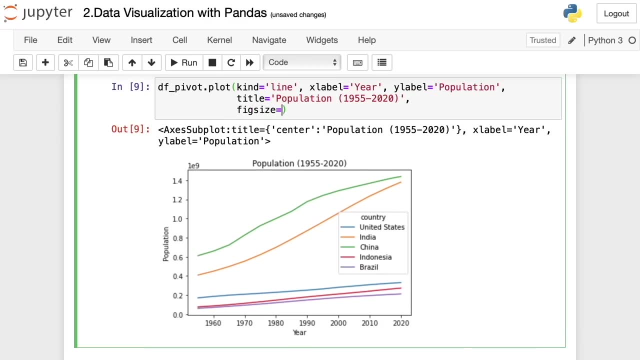 the figure. So to change the size of this figure we can add the argument name: fixed size, And this is a tuple. So we have to open parentheses. And now to edit the size we have to add two arguments. The first is the size of the x axis. 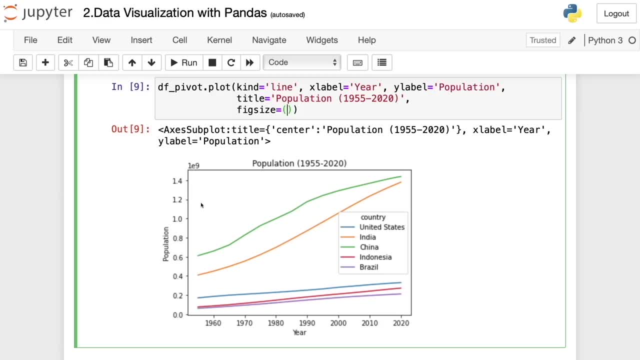 and the second size of the y axis. So in this case I'm going to set it to a and then four, which means that x axis is going to be large, while the y axis is going to be short. So here I'm going to run this code And let's check it out. So here, 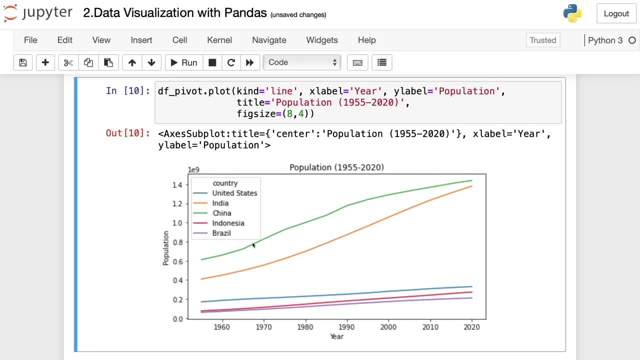 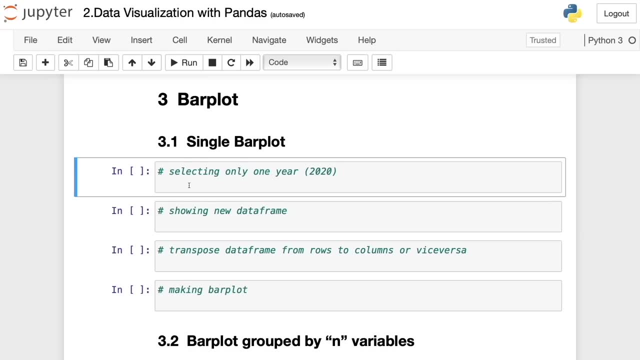 the figure has a different size, And that's how you can customize this line plot. Okay, now let's make a bar plot with pandas. So the first thing we have to do is to select only one year, So the bar plot only accepts just one year, and we can plot the population of. 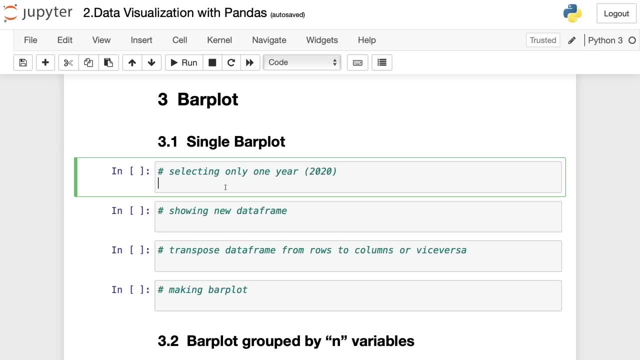 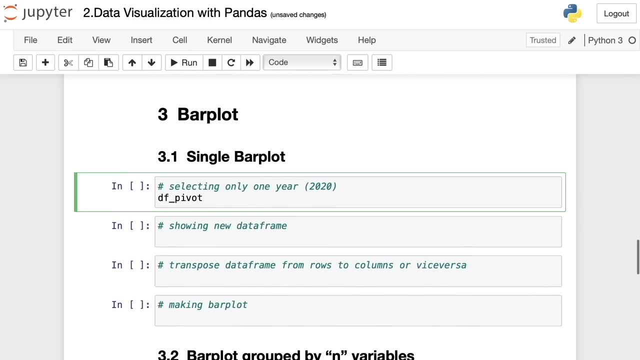 different countries. So let's select one year of this data frame we have before. So I'm going to copy the name of the data frame So you can check it out again. So this is the data frame and we're going to select one year, So 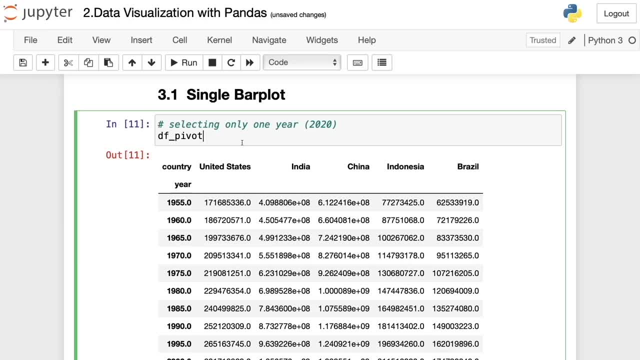 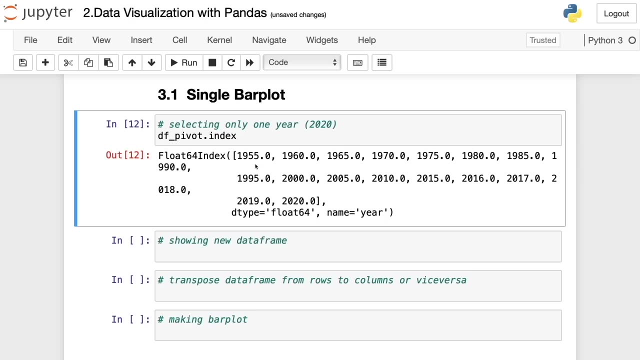 to do that we have to use the index attribute, And then that is in method. So first I'm going to show you the index method, in case you don't remember. So here the index. sorry again, that index attribute allows us to see all the index in this data frame. So we have here from: 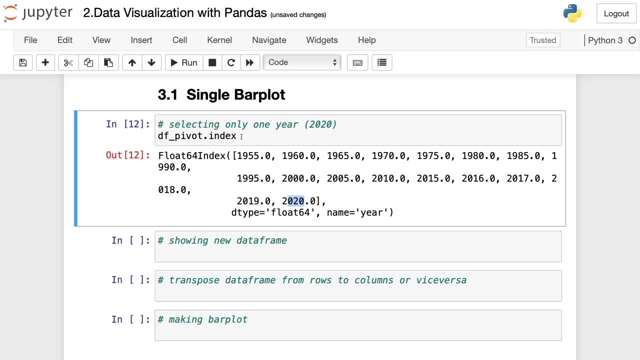 1955 to 2020.. So that's what the index attribute does. And now, if we use the is in method, we can filter out some index. So here let's say we want to select only that 2020.. So I copy: 2020.. And now here I write: equal to n. first I'm going to make the selection. 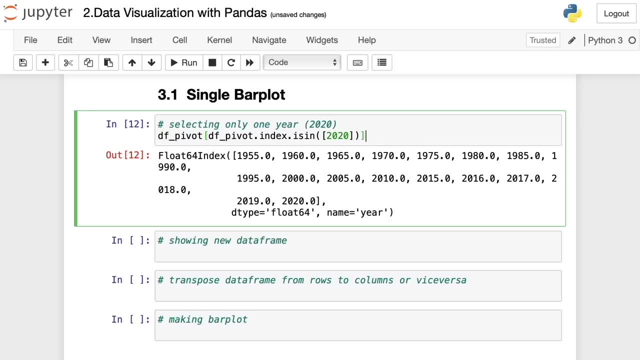 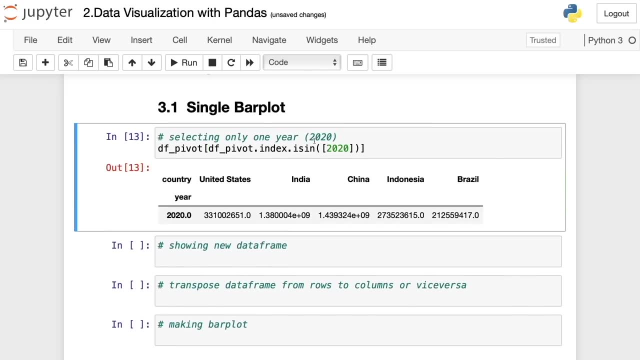 So it's here, And now I'm going to show you what's the result. So here, I press Ctrl Enter And the result is this little data frame that only contains the population in the year 2020.. So this is important, because the bar plot is supposed to show only the population. 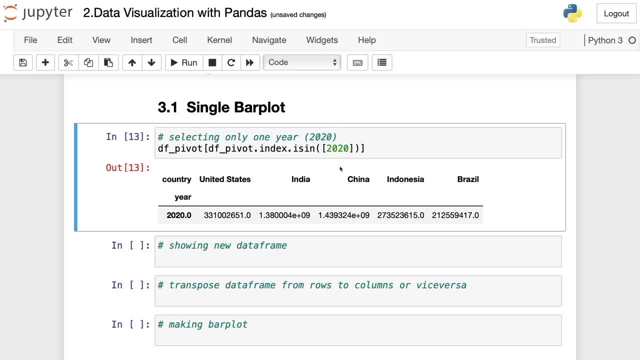 in this year. So here we have it, And now what we're going to do is to name this data frame. So here we write equal to, and then let's give it a name. So I'm going to name it: df- underscore, pivot, underscore 2020.. So here I press Ctrl Enter And now 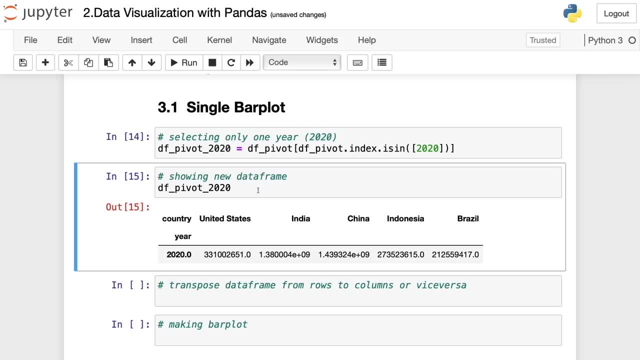 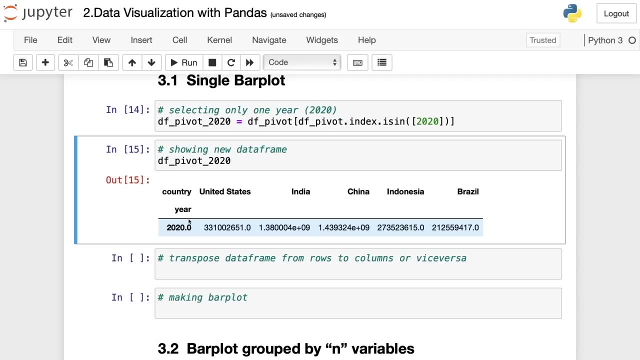 I'm going to show this new data frame Well again here and here. one little detail I have to tell you is that when we make bar plots we have to put text data in the index. So here the name of the countries should be in the index. So to do that we have to. 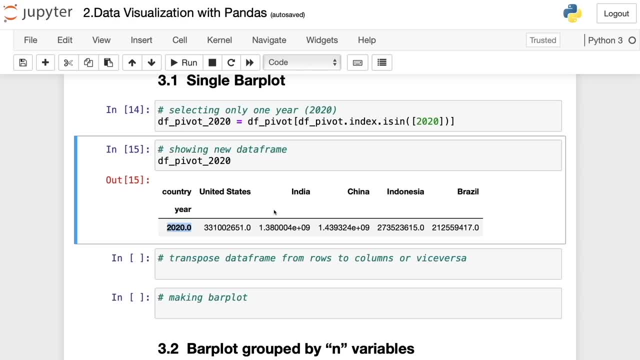 use the transpose method. So this transpose allows us to switch rows and columns and vice versa. So here we can easily do that by writing the data frame, the name of the data frame, you know that: T. So if now we run this code, we can see here that we have this. 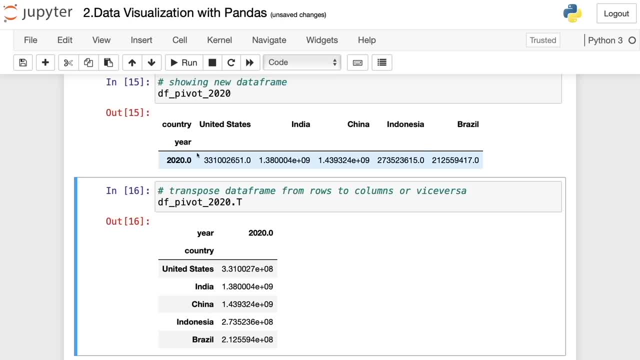 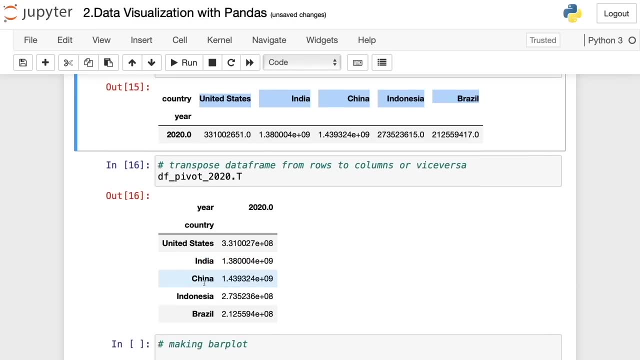 So now the year 2020 is in the column and not in the index anymore, And country names are in the index here. So this is the format we need to have before making the bar plot. So now I'm going to overwrite the content in this data frame, So I write the F underscore. 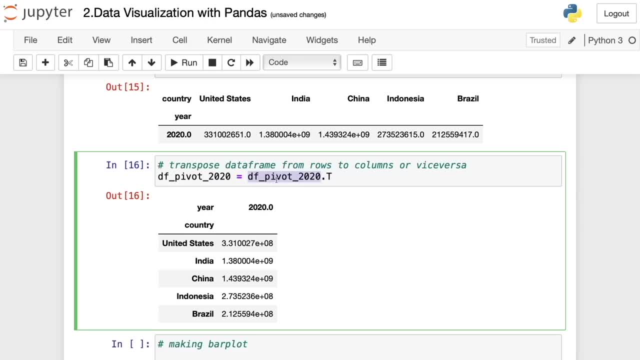 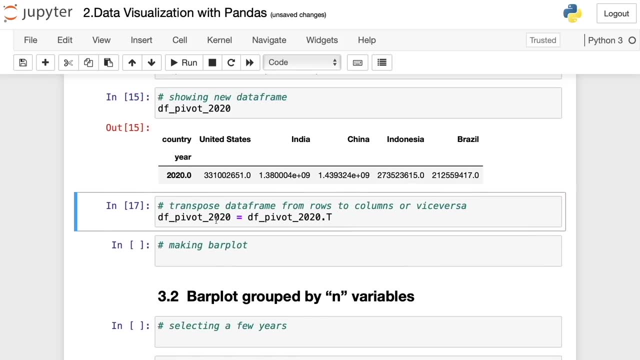 pivot underscore 2020, equal to this same data frame, but that T. So here I run this and now it's time to make the bar plot. So here I copy the name of the bar plot, And now I'm going to use the plot method. So I write plot again, open parentheses and the first argument. 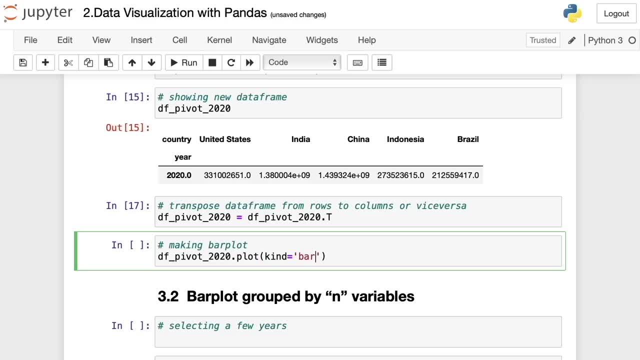 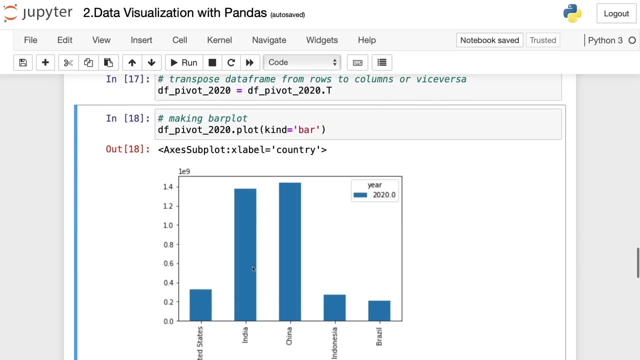 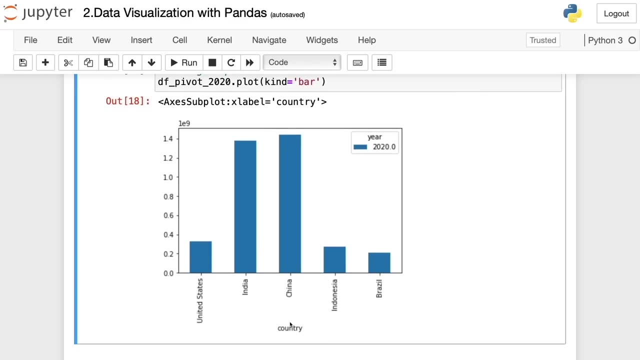 is the kind. So I open quotes and we write bar. So now it's ready and we can run it. So, as you can see, we have a basic bar plot And it has some default values, like the name of this x label And also the default color is blue, And we can customize this bar plot. 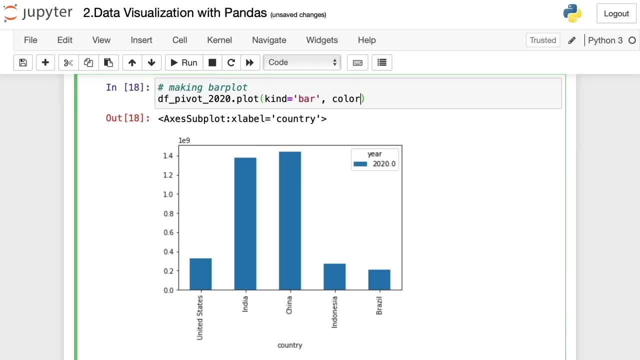 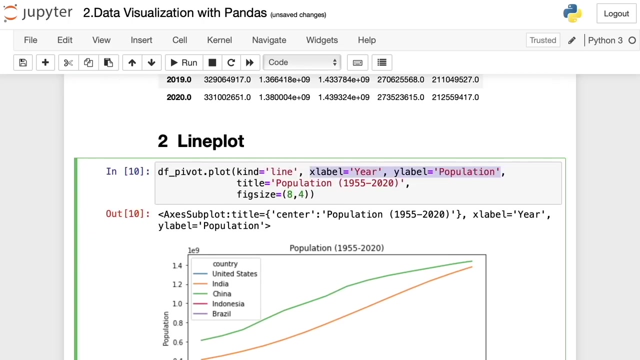 for example, I want a different color, So I write the color argument and then open these quotes And let's say, I want it to be orange, So I write orange. And also we can change the x and y label. Actually I can copy this here So I can save some time here. So x label and y label are here And 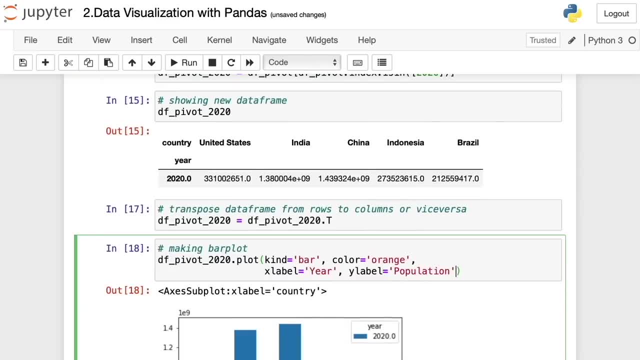 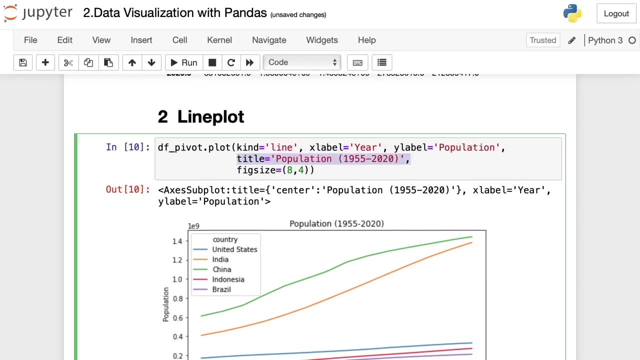 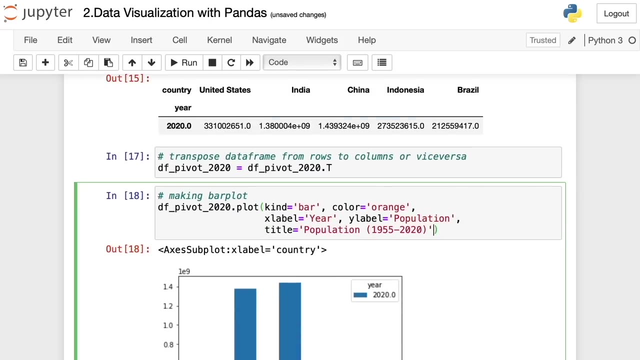 let's paste it here. So x and y label. And finally, I can add also the title, which was here. So I copy and paste it. But in this case the title is a bit different, because in this case it's not from 1855 to 2020.. But it's only 2020.. So here I have only 2020.. And now let's run this: 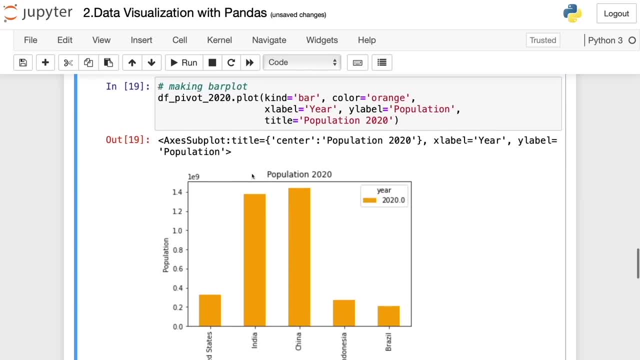 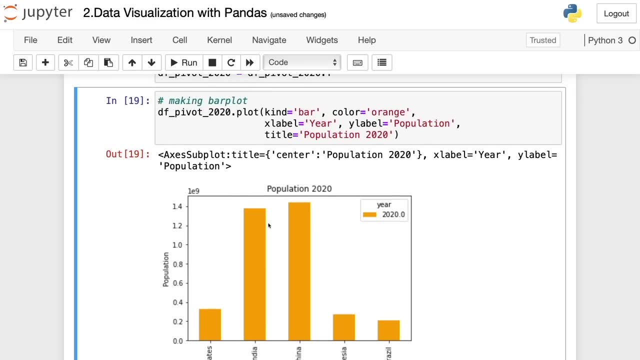 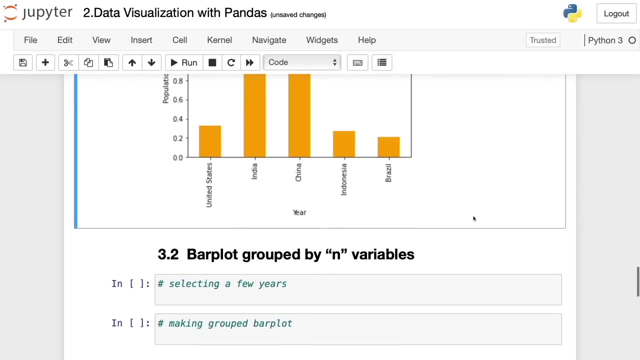 to see the results. So you can see: here we have a title, the x and y label And bar plot is in orange. So that's how you customize the bar plot. Alright, so far, so good. Now let's go one step further by making bar plots grouped by n variables. 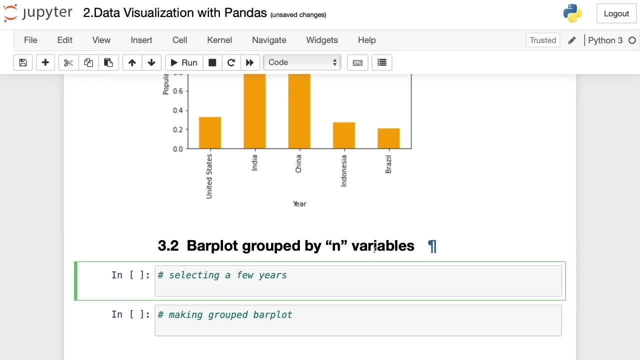 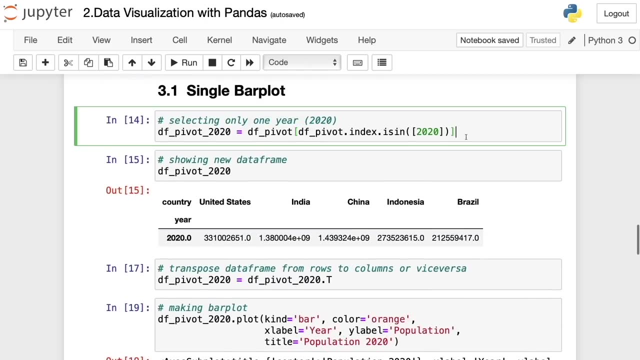 So here we have to select a group of years to make these bar plots grouped by n variables. So I'm going to copy this code we use before to select only the year 2020.. I'm going to copy this And in this case I'm not going to select only one year, but a group of years. 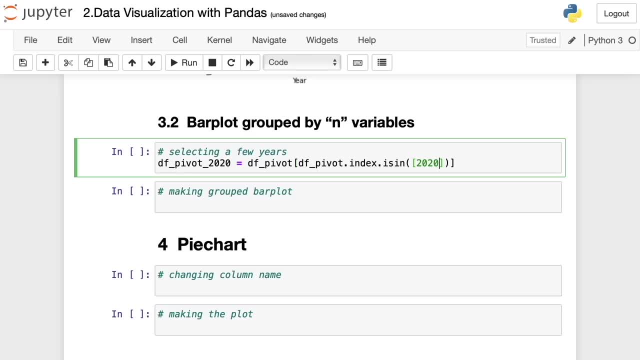 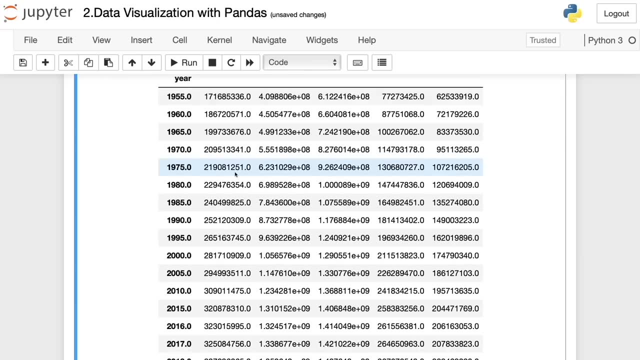 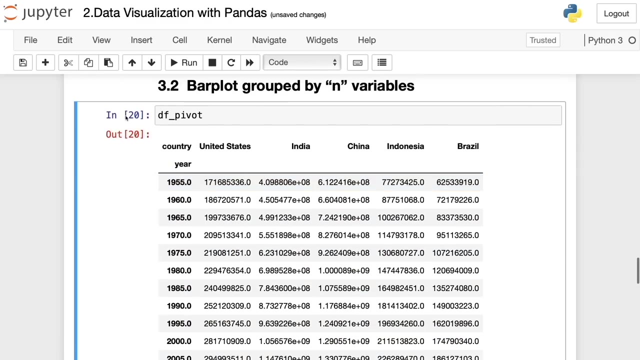 So let me show you here, instead of choosing only 2020.. I'm going to show you that people table again So you can easily understand. So, instead of choosing only 2020, I'm going to choose some other years here. So I'm going to delete this And I'm going to write it here. So let's say 1980,. 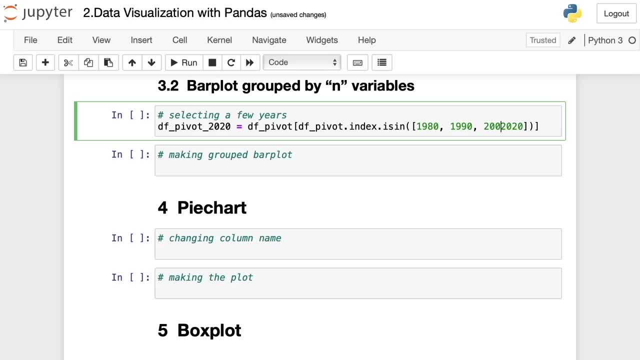 1990,, then 20,, then 2000.. And 2010.. And well, finally 2020.. So we have a group of years here And we're selecting this using the index and is in method. So here I'm going to give it a different. 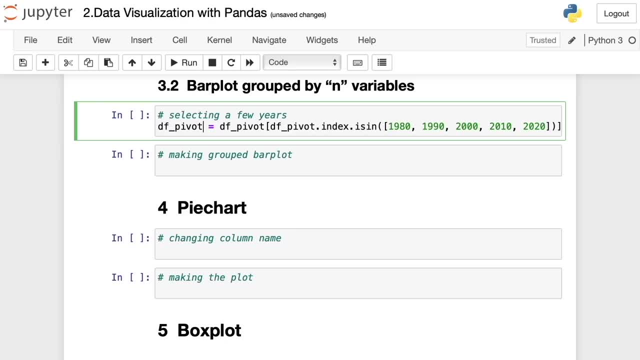 name. In this case, since it's a sample, I'm going to write the F underscore- pivot underscore- sample. Now I'm going to. first, I'm going to show you this one So you can see what this looks like. So now we have five. 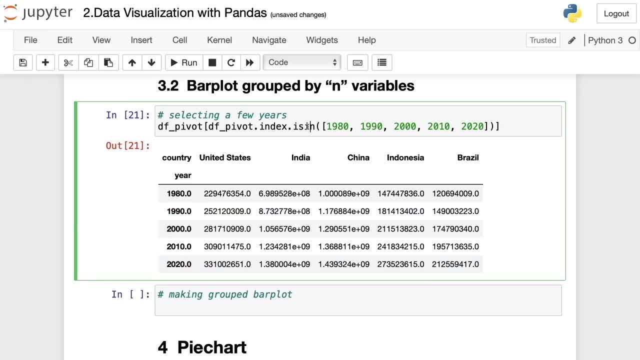 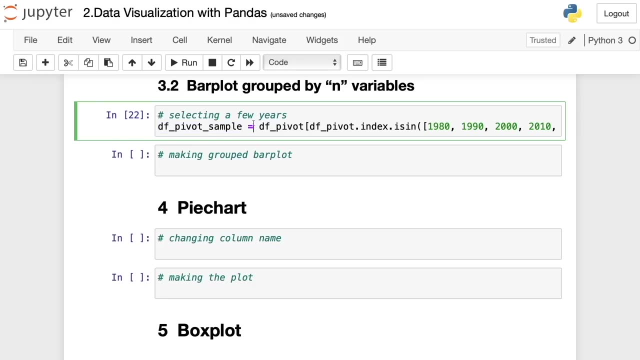 countries and now five years. So now I'm going to assign these to my data frame. So the F underscore, pivot underscore, sample. I run this And now we have this new data frame. So it's time to make these grouped bar plot. So here we write the name of the data frame. 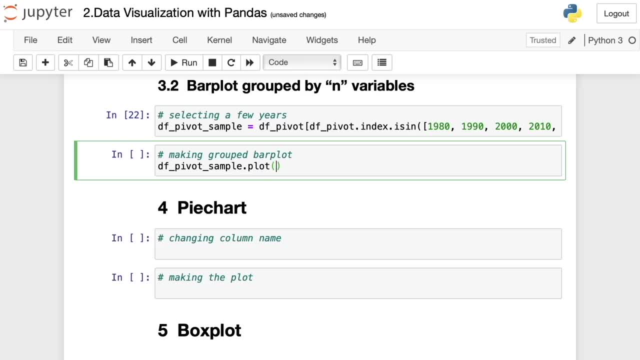 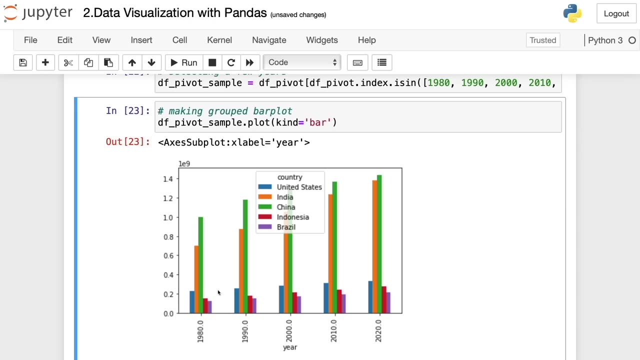 and then that plot method. So here we write the name of the data frame and then that plot method. So write that plot. And now let's add the first argument, which is kind and equal to bar. Now we run this And, as you can see, here we have the plots, or the bar plots, grouped by year. So here's. 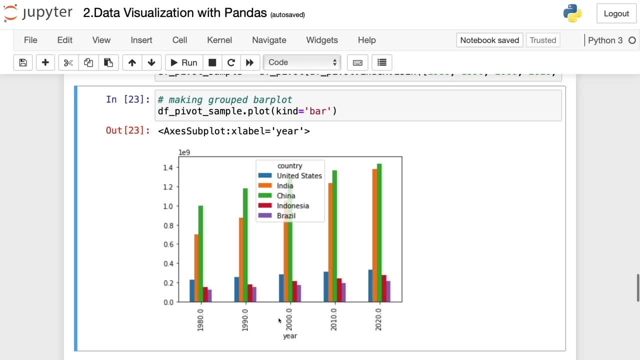 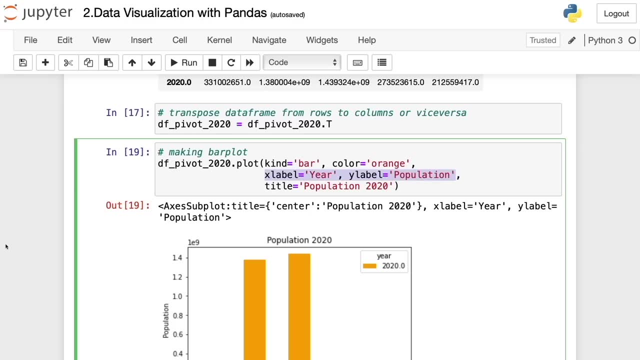 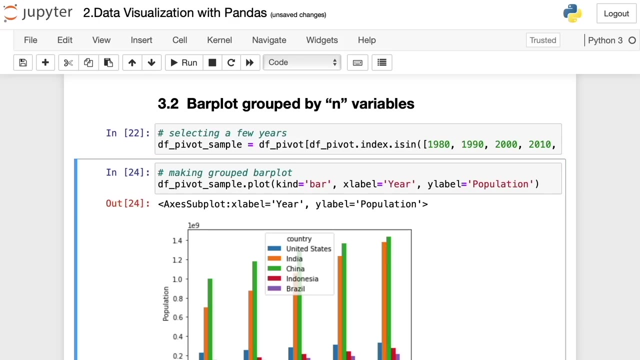 1980, in 1990, and so on. And you can also add the same arguments we added here. So for example, I can add x and y label. so I can do it here. I'm gonna do it fast, So here I run in, as you can see here. 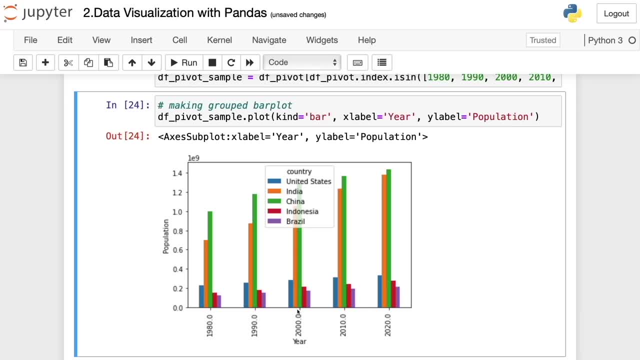 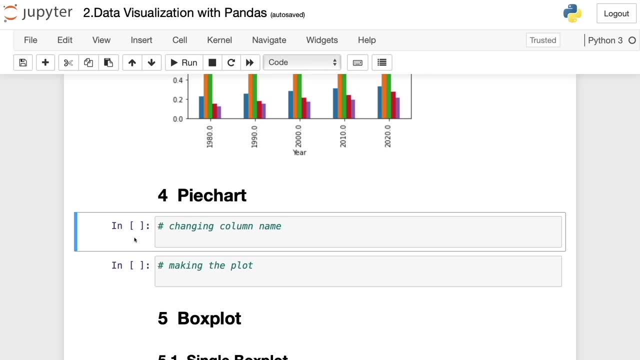 we have the, we modify the x and y label And that's it. That's how you make bar plots with pandas. Okay, in this video we're going to learn one of the most common charts that we can make in pandas in actually in any other visualization tool, And these are pie. 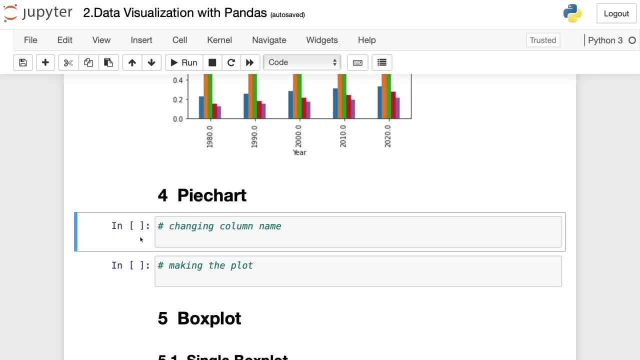 charts. So before we make this pie chart, first let's give a look to the data frame we're going to use In this case to make a pie chart. we're going to use the same data frame we just for making the bar plot, because it follows the same logic. So here I'm going to copy the data frame. 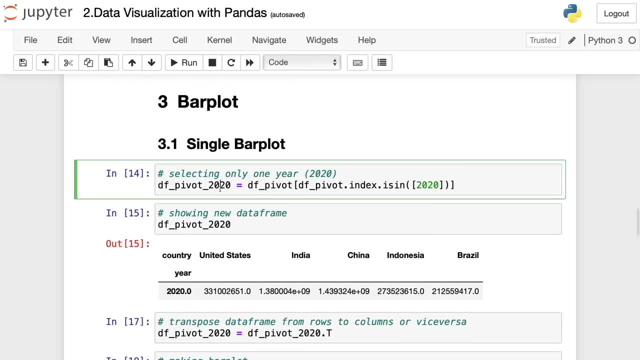 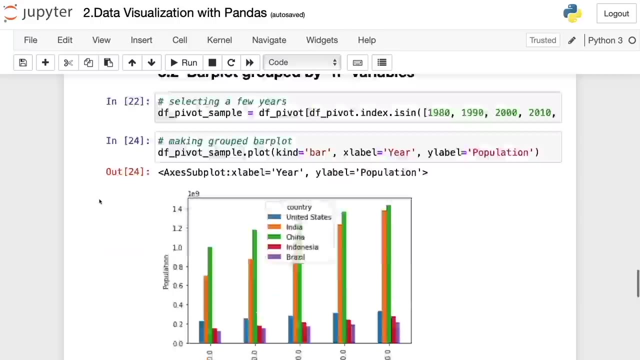 we created for the bar plot, which is this one: the F underscore, pivot underscore 2020.. So this is what we created before by using the index attribute, and that isn't method. So here I'm going to copy this And now I'm going to show you here, so so you can remember what's inside this. 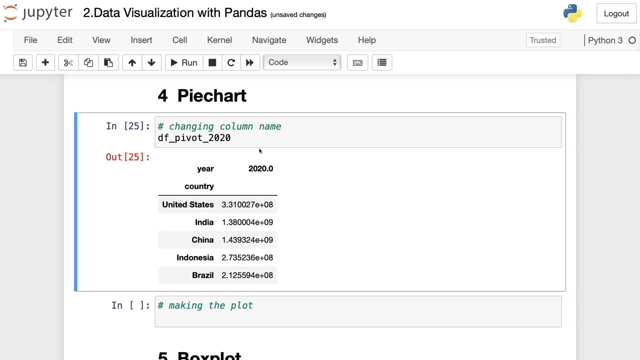 data frame And it's here. So here, as you can see, we have the column 2020.. And the countries are in the index, So everything is fine. That's what we need. That's the format we need for making. 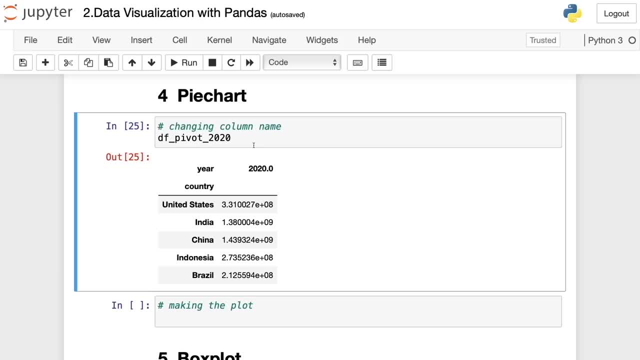 the pie chart. But there is one little thing we have to modify, And this is the column name, because now it's 2020.. And this is a number. It's actually, I think, it's an integer, So it's not a good practice to have numbers in columns. So what we have to do is to make this a 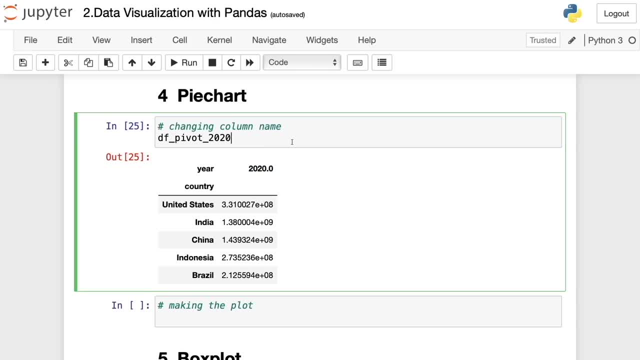 string And to do that, we use that rename method. So we write that rename, open parentheses. And now we use the columns argument. So we write columns, then open this curly braces, And now we write the name of the column we want to change, which is 2020.. And we're going to make this integer. 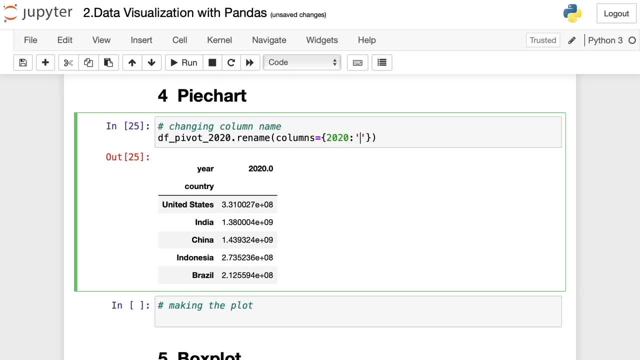 value into a string. So we open quotes and write 2020.. So apparently they are the same, but the green one is integer and the red one is a string. So now to make, to save this- changes, I'm going to write in place equal to true And I'm going to run this. So now we can. 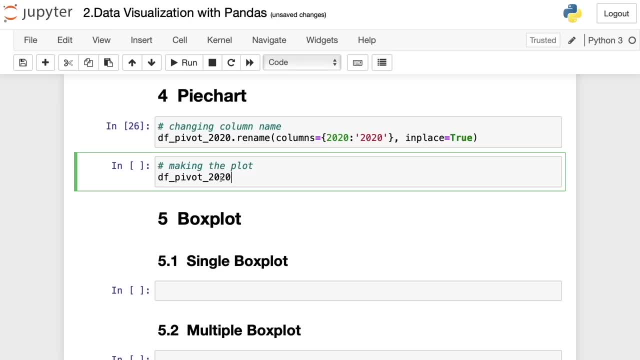 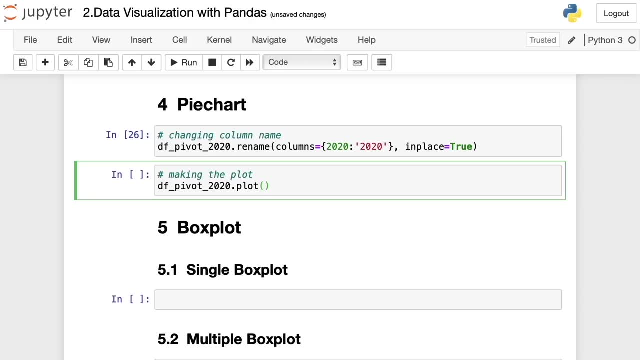 make the plot. Here I'm going to write the name of the data frame, And now I'm going to use the plot method. So here I write that plot, So the first argument is kind. and here I write pi, So the kind is pi. And now I run this, And here I forgot to. 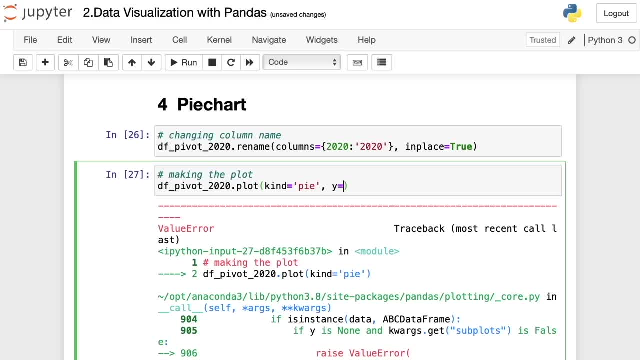 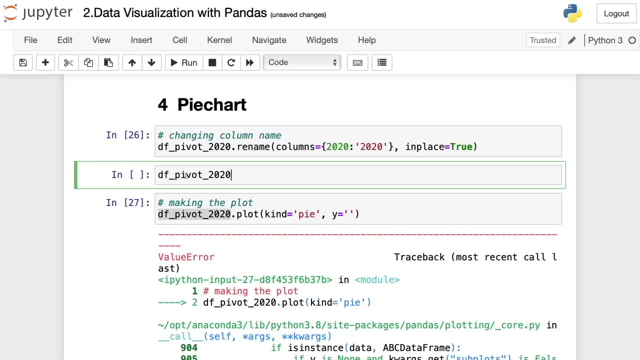 include that y argument And I'm going to write here. So the y argument is supposed to have the data. So in this case, I'm going to show you here again the data frame. So the data is here in 2020.. 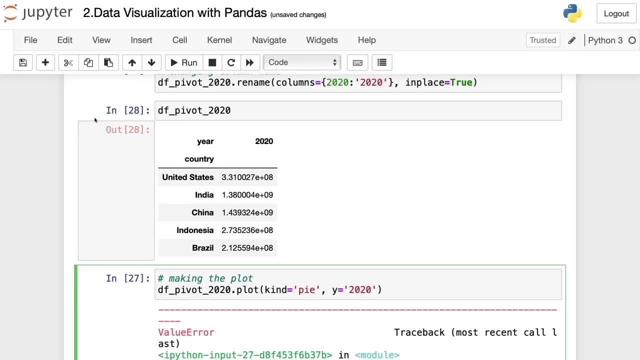 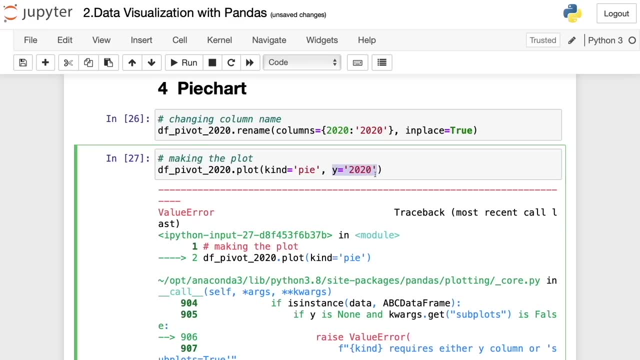 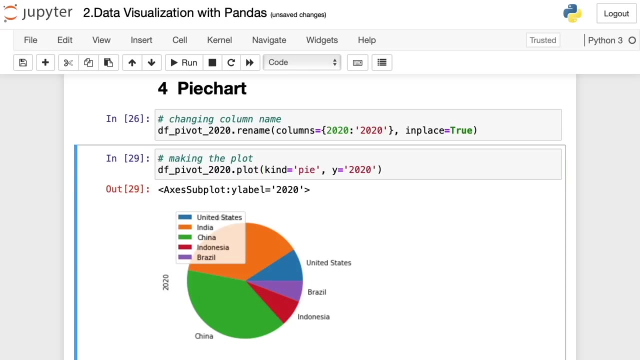 So we should write here: 2020.. So I'm going to delete this. And here in the y argument, you write the column that has the data. So that's what we did. So now I run this And now we finally have our pie chart. So here is the pie chart. So that's how you make a pie chart. 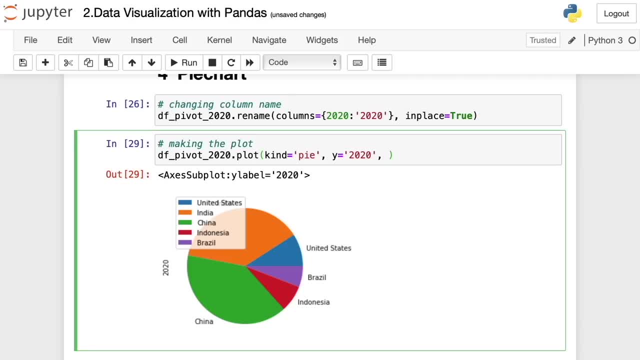 If you want, you can even add another argument, like the title. for example, here I can say that this is a population in 2020.. But in this case in percentages. right, this, and now we have this title. So that's how you make a pie chart in pandas. 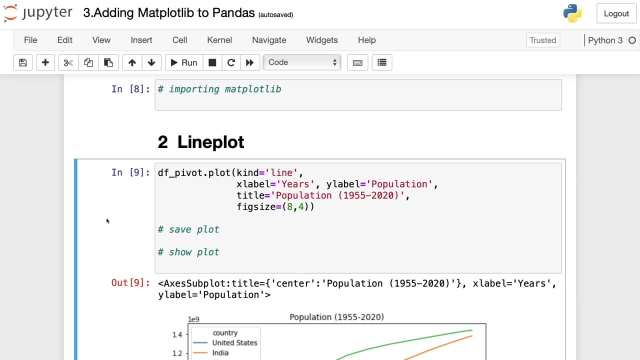 All right. so far, we made a pivot table in many plots using pandas And in this video we're going to learn how to export the pivot table and also the plots we made with pandas. So let's start by exporting the plots we made with pandas, And to do that, 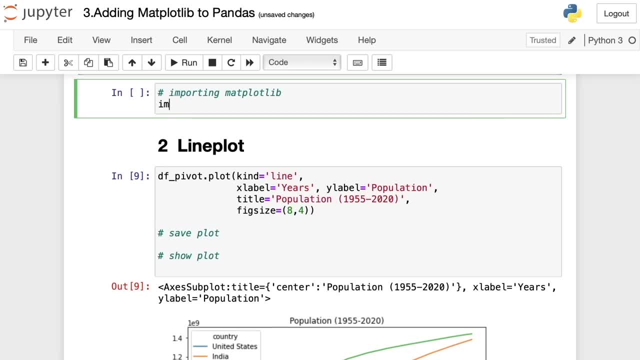 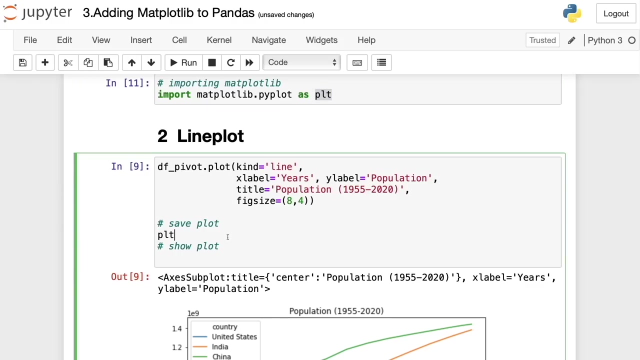 first we have to import matplotlib. So we write: import matplotlib dot pi plot. And then we write as PLT, So this PLT represents this matplotlib dot pi plot. So now we run and we imported matplotlib, And now we can use this PLT to save the plot. So we write: PLT dot save fig. 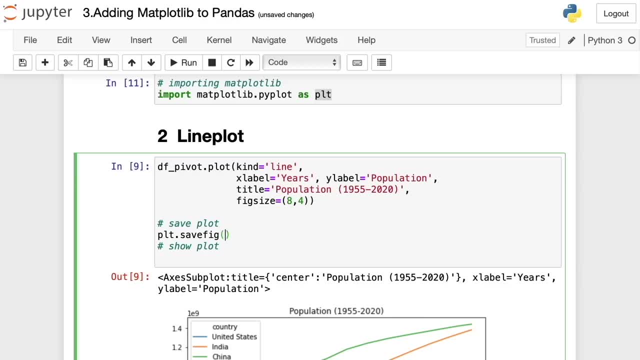 And now we open parentheses And here we have to write the name of the file we want to export. And here I'm going to write my underscore: test that PNG. So this is the extension, This is the name of the file. And now, before exporting this file, I'm going to show you. 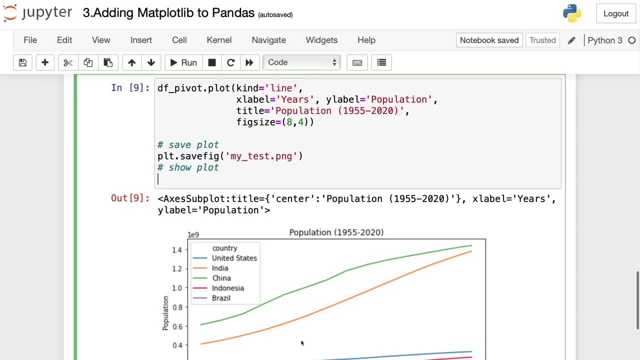 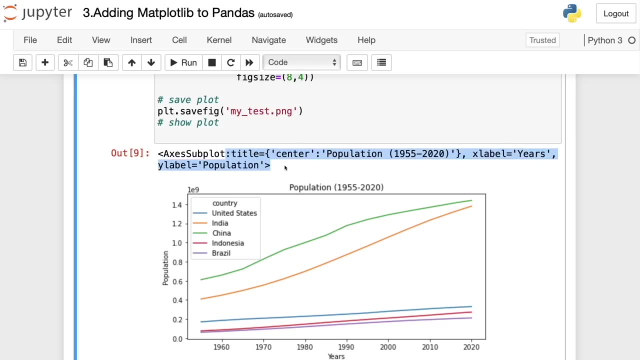 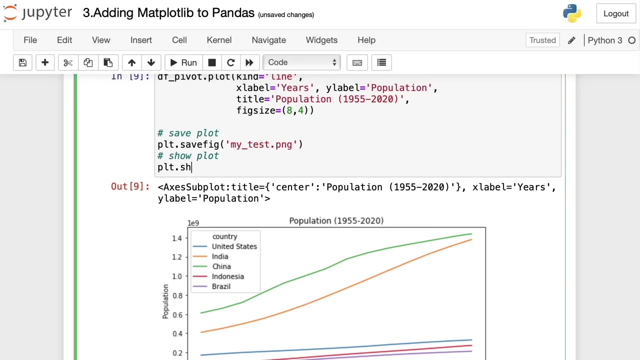 something here. So probably you notice that when we make the plot with pandas we get these words here that says access, subplot and all of this. So we can get rid of these words by using the show method. So we write PLT, that show with parentheses, And if we run this,